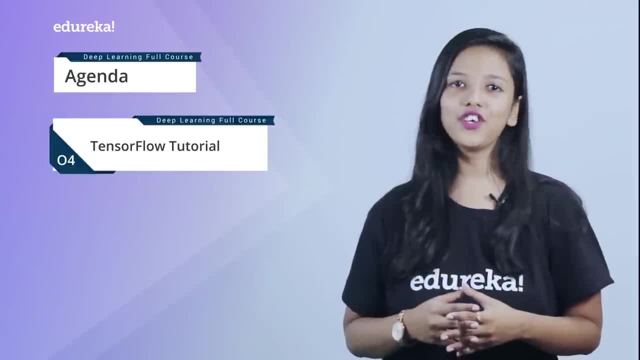 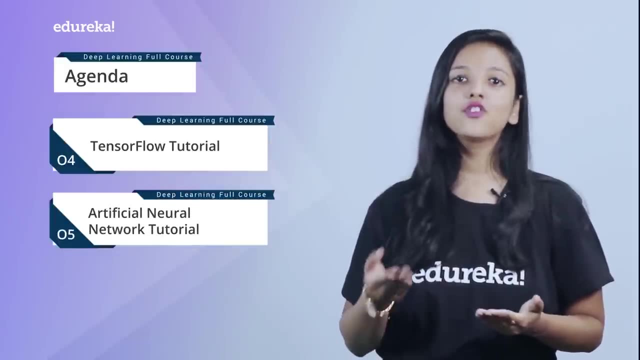 graphics visualization and also increase the efficiency of the model. Now moving on to the next module, we will talk about artificial neural networks. So in this module we will see what are neural networks and how they actually work, and then we will get into the 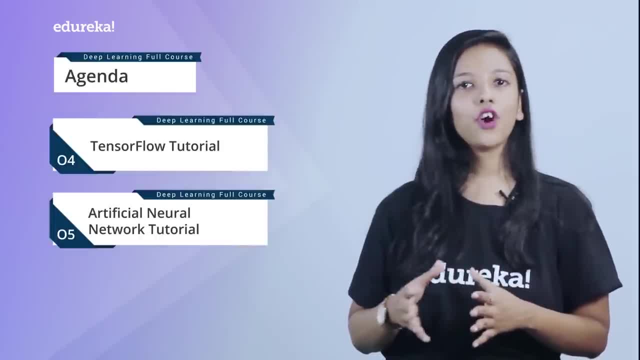 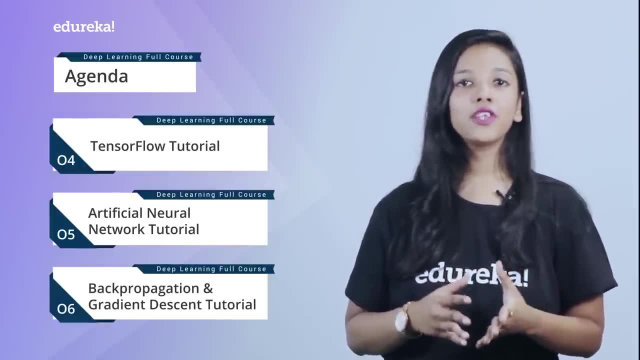 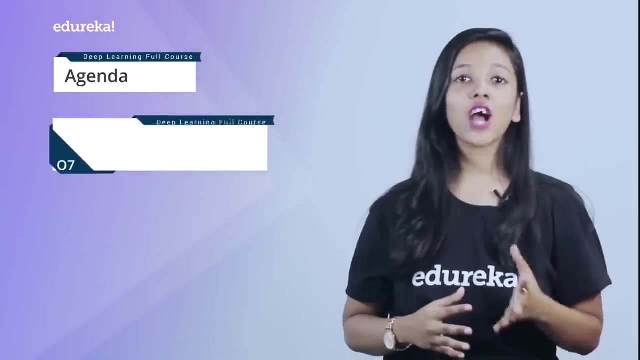 depth of artificial neural networks. Now, moving on to the next module, we will see back propagation and gradient descent. Now, in this module, we will discuss about these two terms with the help of the MNIST dataset. Now, moving on to the next module, we will talk about RNN, that is, the recurrent neural 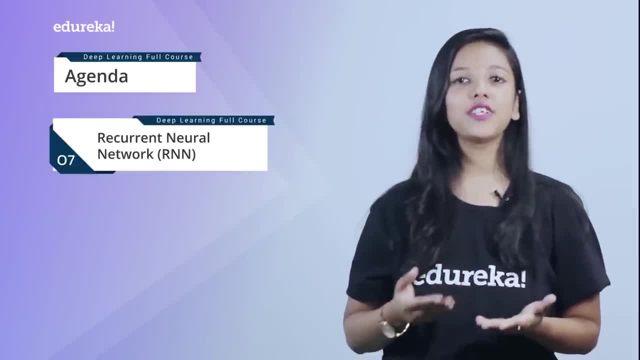 network. So here we will see what are recurrent neural networks and how it works with the help of the LSTM dataset. Now, after RNN, we will talk about CNN. So again, we will talk about CNN in our next module, that is, the convolutional neural network. 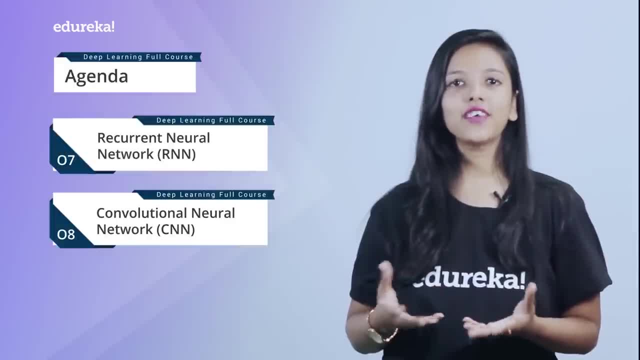 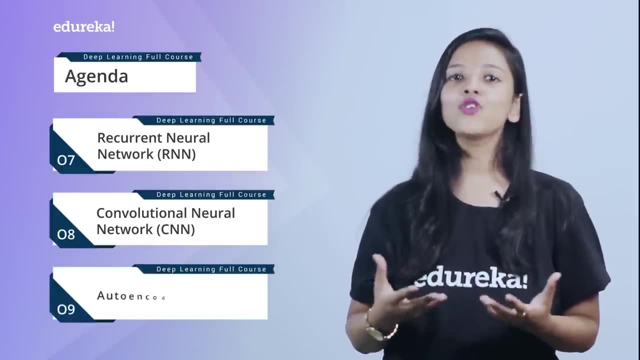 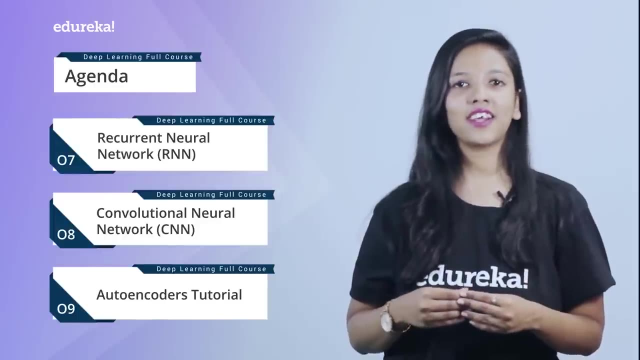 Here we will see what are convolutional neural networks and how they work with the help of different use cases. Now, after RNN and CNN, we will see what are autoencoders. So here we will see what are autoencoders, how it works, different types, properties and architecture of autoencoders. 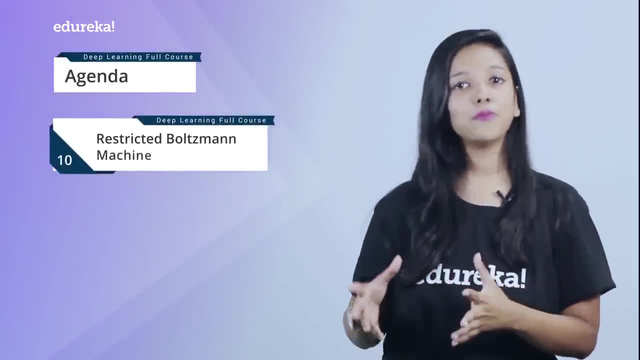 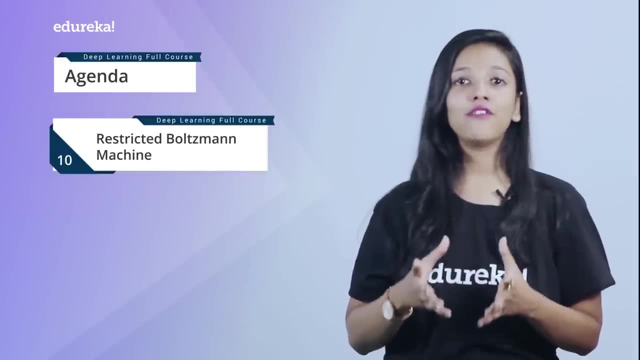 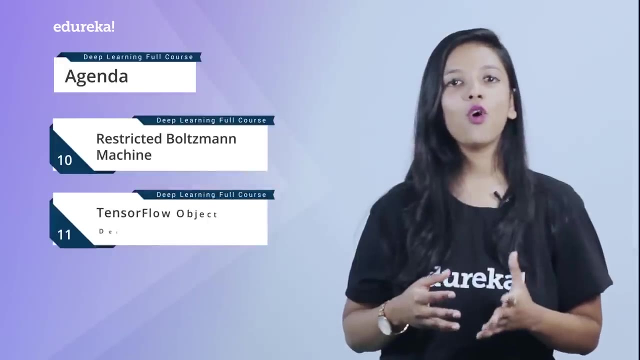 Now, after autoencoders, we will discuss about Restricted Boltzmann machines. So for that we need to understand the different between RBM and Autoencoders, and also we will have a look at the different working procedure of RBM. Now in the next module we will talk about Tensorflow object detection. So here we will. 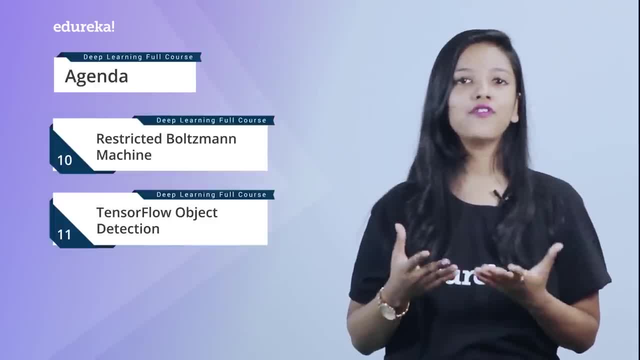 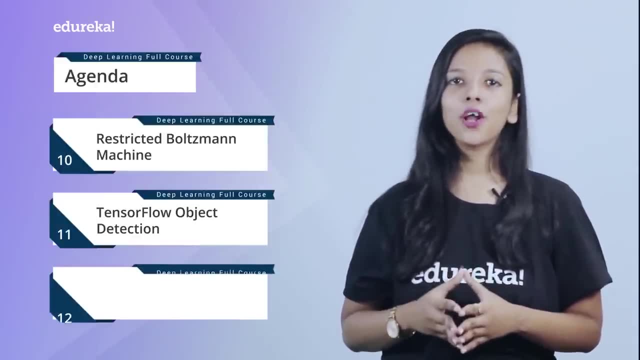 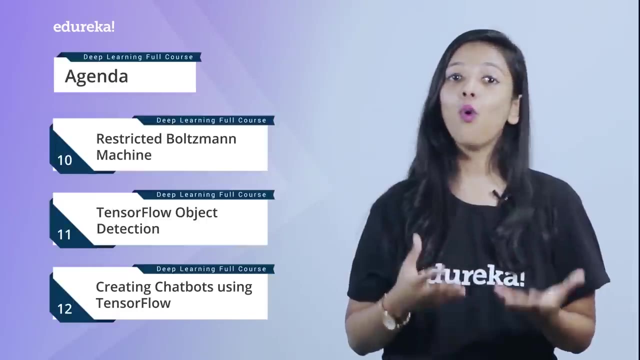 understand what is object detection and how, with the help of tensorflow, you can detect different objects in your surrounding. And finally, in the last module, we will talk about CHAT BOTS using Tensorflow. So here you will have a step-by-step guide on how you can build your own chatbot with the help of tensorflow. 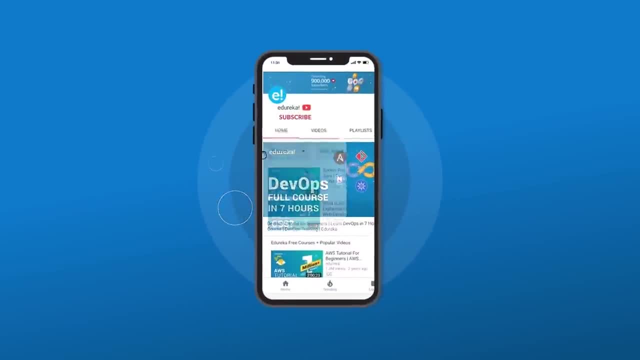 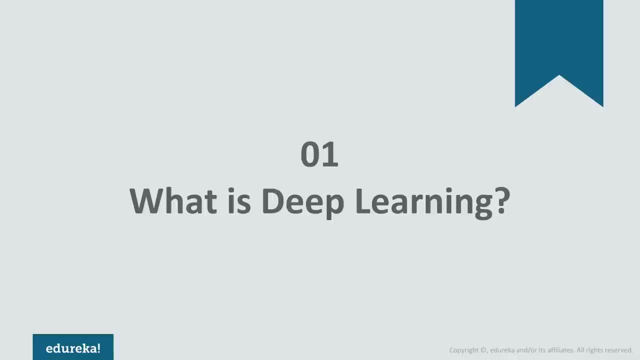 now, before we begin the session, don't forget to subscribe to edureka's youtube channel to stay updated on trending technologies. hello everyone, this is saurabh from edureka. welcome everyone to today's session on what is deep learning. well, understand how deep learning emerged. that is, what are the limitations of the? 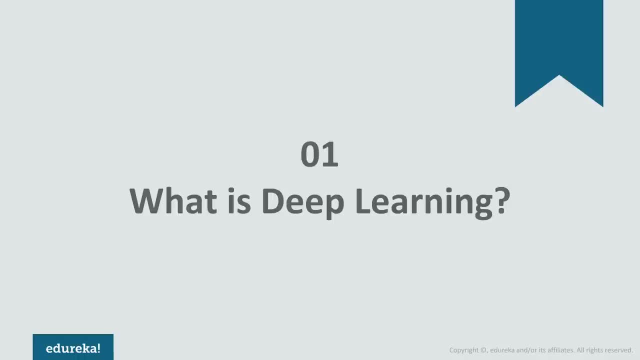 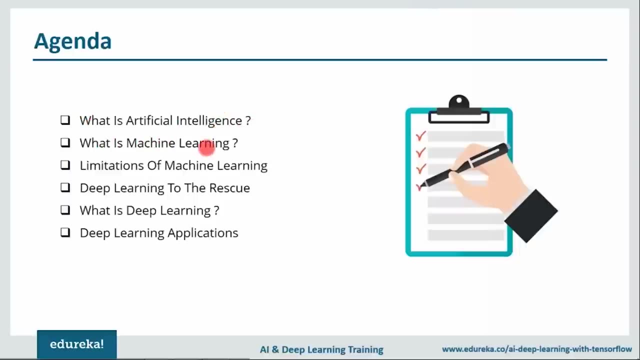 previous technologies that led to the evolution of deep learning. so let us have a look at the agenda for today. first we'll understand what is artificial intelligence and what exactly is machine learning. then we'll look at various limitations of machine learning and how deep learning solves or overcame those limitations. after that we'll understand what exactly is. 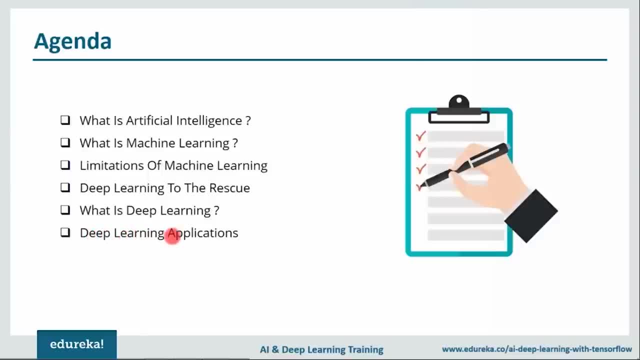 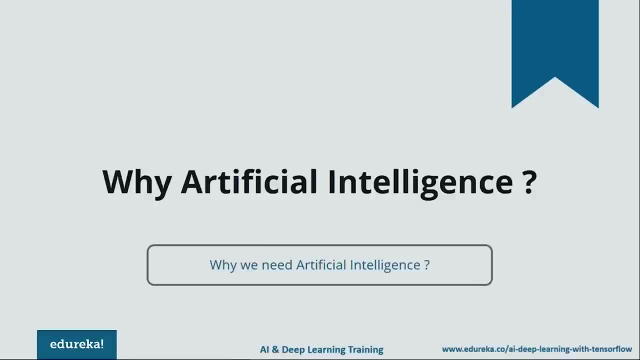 deep learning, and we'll also look at various applications of deep learning. so let us move forward and understand artificial intelligence. but the first thing that we need to focus on is distinctért today, why artificial intelligence? Why do we need artificial intelligence? Now, let us understand. 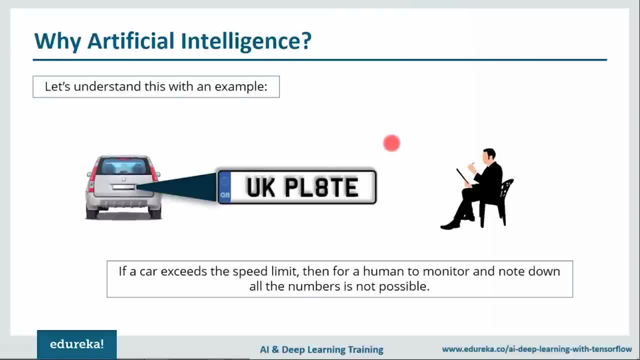 this with an example. So nowadays, if you have noticed, if your car exceeds the speed limit, so you'll get a letter, or basically a chalan at your home. How do you think that happens? Do you think that there is a person who is sitting in a chair and actually noting down all the number? 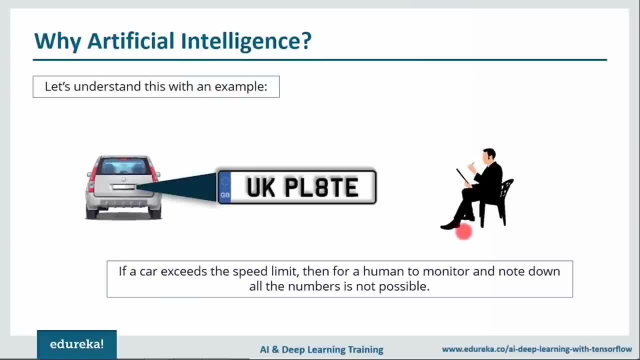 plates that crosses the speed limit. Well, that is not possible because there might be millions of cars that pass through that road, and at once there might be many cars that would be passing through that road. So for a human being to actually do this task is next to impossible. Now let us see. 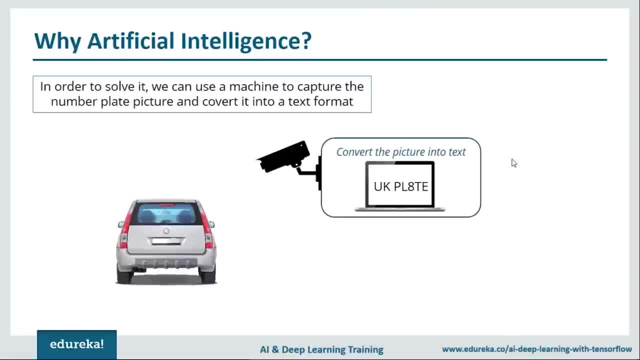 another approach to this particular problem. So what we can do, we can actually make use of cameras that will click the picture of the car that exceeds the speed limit and then we can convert that picture into a text. For example, we have UKPLATE. So in this way, the human error, the risk, 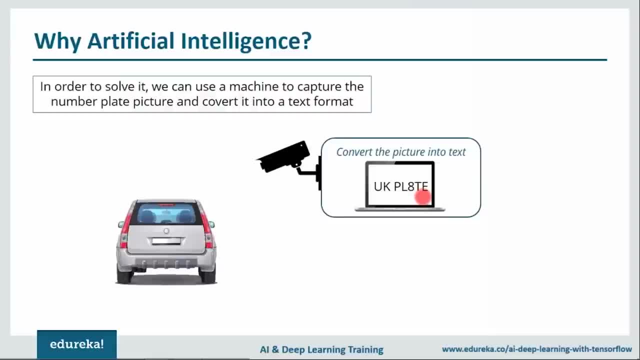 of human error has been reduced and, at the same time, machines. they never get tired. So because of that, you can capture all the images of cars That actually crosses the speed limit. Similarly, you can think of many other examples as well. It is used in order to recognize a sign that is in banks, if you want to authenticate whether that. 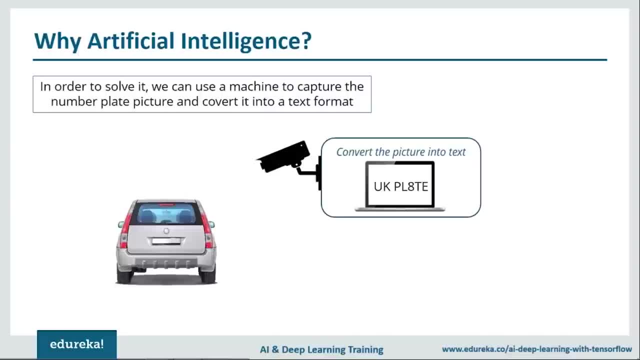 person is the bank customer or not. Apart from that, it is even used for self-driving cars as well. So in US, around 30,000 people die every year because of road accidents. So that can be completely removed if we use the self-driving cars, which is based on the concept of artificial 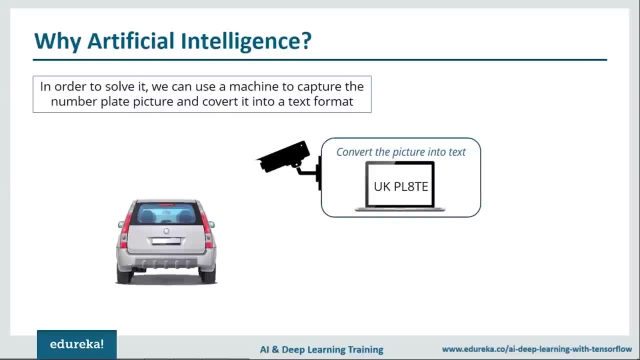 intelligence. And let me tell you, guys, you might find it very fascinating- that people in MIT are using artificial intelligence in order to predict the future. So you can imagine why we need artificial intelligence. It is even used in places where humans can't reach, For example, deep oceans. 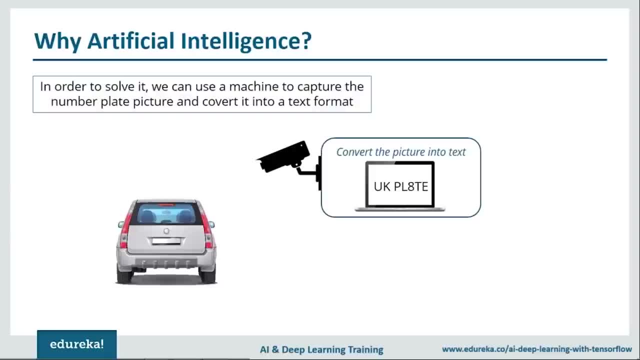 or navigation in Mars. So in those places we need machines which are smart enough to carry our tasks. So this is why we need artificial intelligence. Let us move forward and understand what exactly is artificial intelligence. Now, artificial intelligence- I know the word sounds pretty. 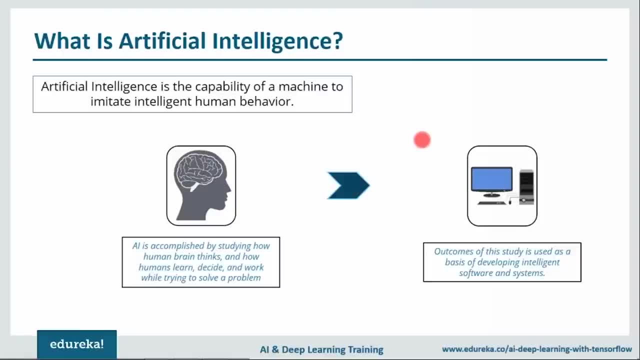 complex and there are a lot of Hollywood movies that are based on artificial intelligence. If you have seen Terminator or Matrix, all these movies are based on artificial intelligence, but you don't need to worry about it, because till now we haven't reached that level as they have. 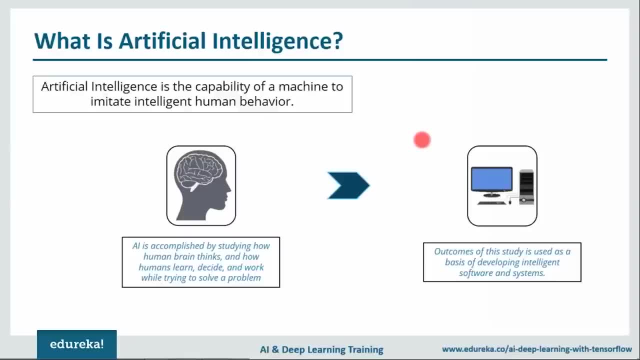 shown in movies like Terminator. But yeah, the concept is pretty similar. So basically, we want systems and softwares in such a way that they can imitate the human behavior. Now, what happens in artificial intelligence? Artificial intelligence is accomplished by studying how human brain thinks. 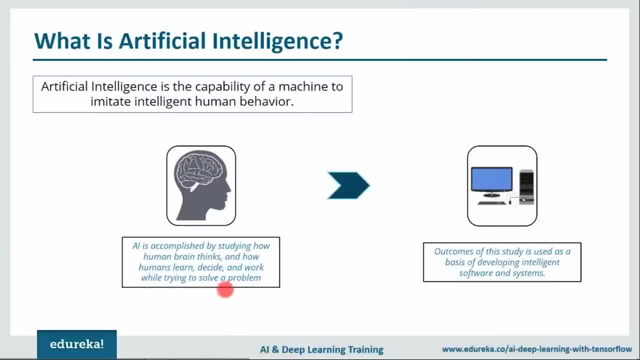 and how human brain learns, decide and work while trying to solve a problem, And then we use the outcome of this study as the basis of development of intelligent software and systems. So our major goal is to have systems or softwares that can imitate the human behavior. 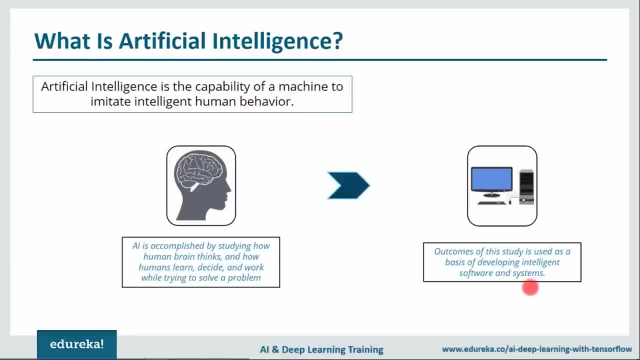 The way they think, the way they decide, the way they solve a problem. So in that similar fashion, we want our machines to do that. So this is basically artificial intelligence in a nutshell. Let us move forward and look at various applications of artificial intelligence. So this: 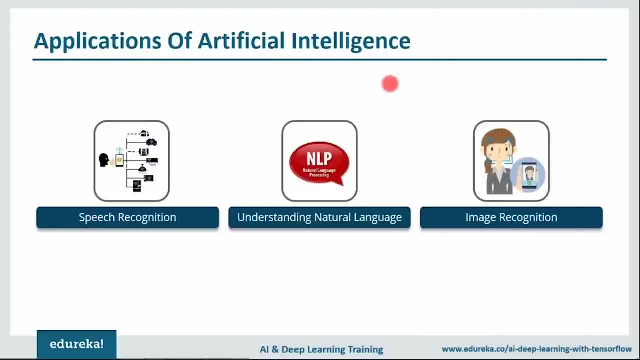 slide basically talks about artificial intelligence. So this slide basically talks about the application of artificial intelligence. Now I've listed only three of them, but there are millions of applications. For example, it is used in speech recognition. So whenever you search something on Google, so you can just tell Google and it will search it for you. Similarly, it is 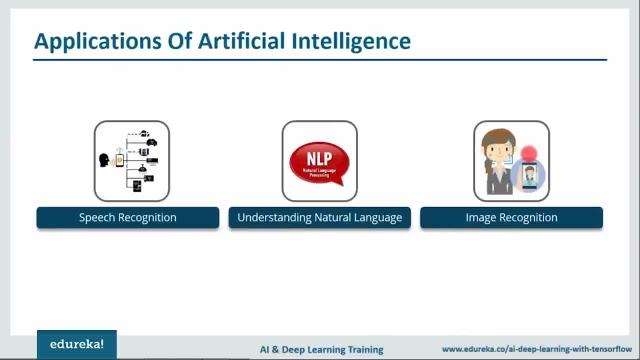 used for understanding natural language, as well as for image recognition as well. And there are many, many other applications in which artificial intelligence finds its use. For example, it can be used in self-driving cars, it can be used in Siri for recommending some products, and even when you. 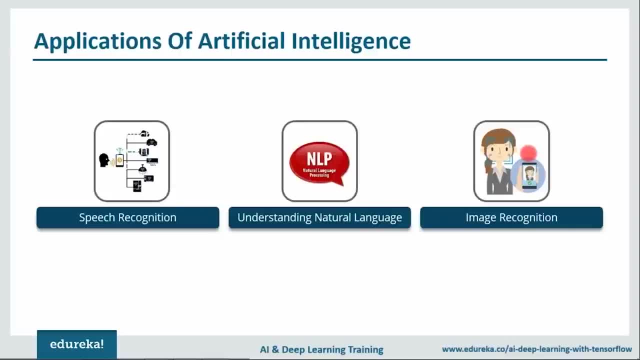 go to websites like YouTube or Pandora. YouTube can be used in self-driving cars. it can be used in audio, So anything that you can put into a video is used in self-driving cars, because there is no need for artificial intelligence in your video. Now, on the other hand, if you were to search e-books, 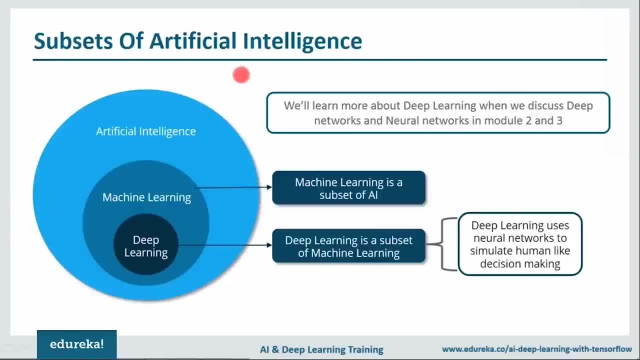 YouTube knows which video you want to mix, Pandora knows which song you want to listen to. How do you think this happens? It happens all because of artificial intelligence. So all of these are a few examples of artificial intelligence, but nowadays it is used almost everywhere. guys, Trust me on that. Now let us move forward and understand how to achieve artificial intelligence. Now, in order to achieve artificial intelligence, there are a few technologies that came. First came machine learning. Now, there were certain limitations of machine learning. In order to overcome those limitations, the machine learning has to be done by machine learning. 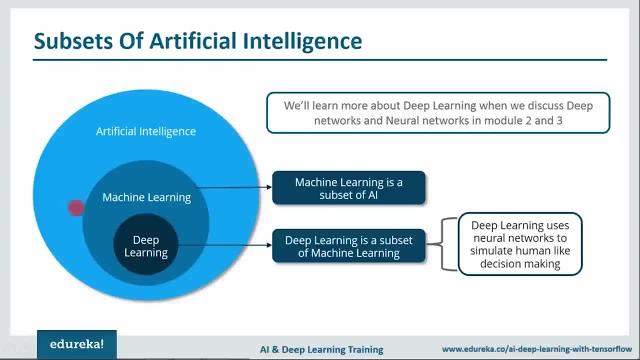 came a deep learning. Now let me tell you guys, the concept of artificial intelligence is not new. It was first coined in 1956, but it was just a theoretical concept. Then, in 80s and 90s, we were talking about neural networks. 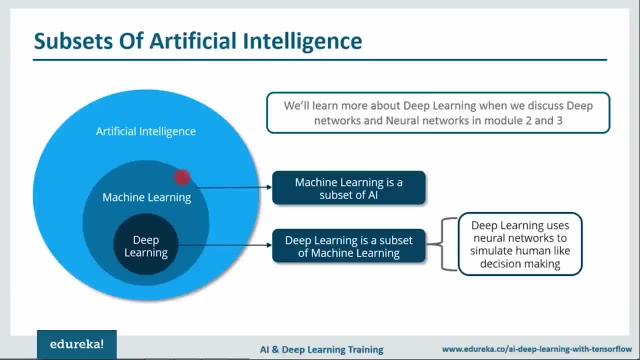 but since we didn't have enough computational power, so we couldn't utilize it properly. but in late 90s and 2000s we started using neural networks for machine learning. Then, in 2006, the term deep learning was coined for the first time. that overcame the limitations of machine learning and from 2010, deep 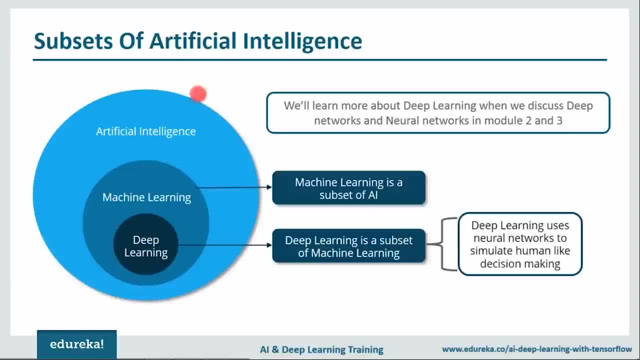 learning was used commercially as well. So this was just a small history about artificial intelligence, machine learning and deep learning. Now, in order to understand this deep learning, we need to first look at machine learning, and what were the biggest limitations of machine learning that led to the evolution of? 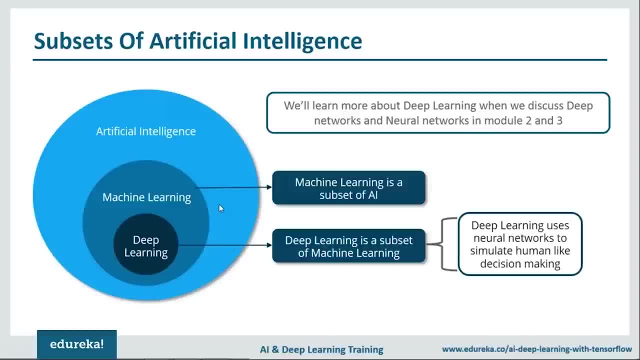 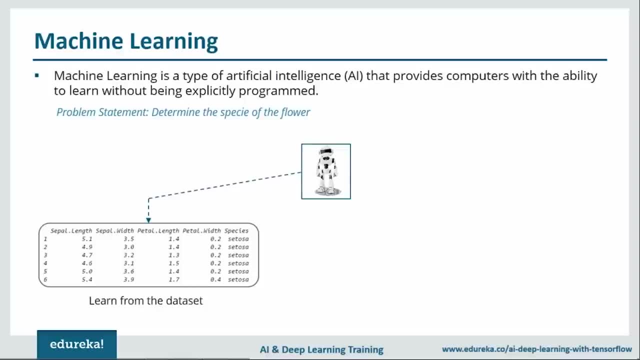 deep learning. So we'll move forward and understand what exactly is a machine learning? Now, what is machine learning? So machine learning is nothing but a type of artificial intelligence, or you can say a subset of artificial intelligence, and it provides computers with the ability to learn without being explicitly programmed. 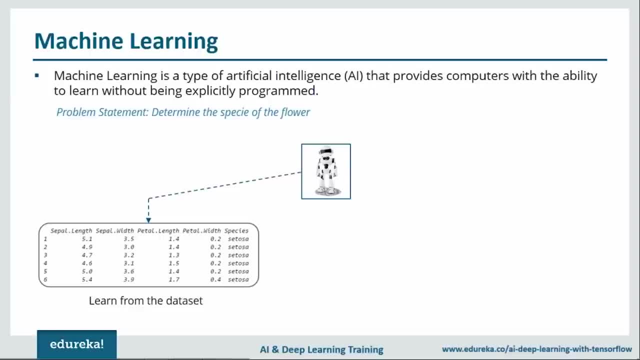 So you don't need to hard code your machine for that. Let us understand this with an example. So we have a problem statement in which, whenever you give a certain input, we need to determine the specie of the plant And what is that input. 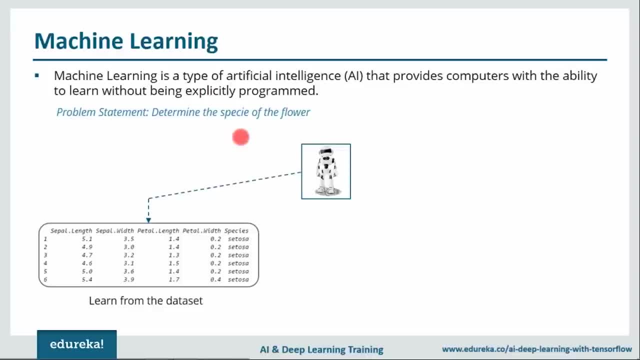 That input will be sepal length, sepal width, petal length and petal width. So whenever we get these four parameters, or these four variables, our machine should be able to predict what sort of a flower it is. Now, how do you think that will happen? 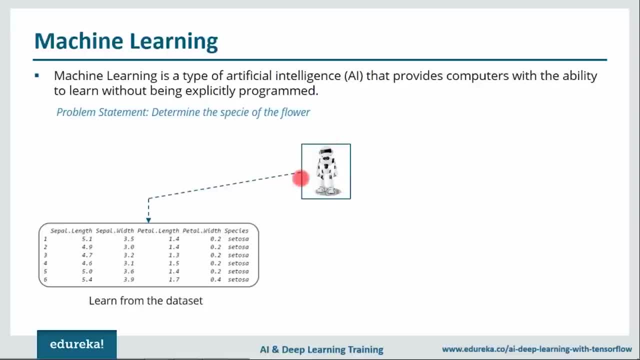 First what we need to do. we need to train our machine on the basis of the data that we have. So in this data we have sepal length, sepal width, petal length and petal width and we have species. So our machine will learn from this data. 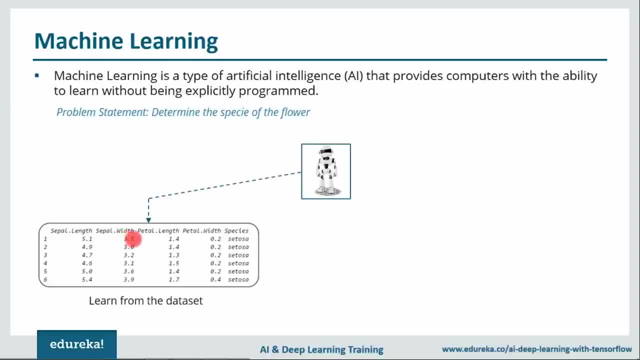 It will determine what should be the length and width of the sepal and petal, in order to classify it as setosa or versicular or other species of flowers as well. Now, what happens next? So you have trained your data, So you have trained your machine from the data set. 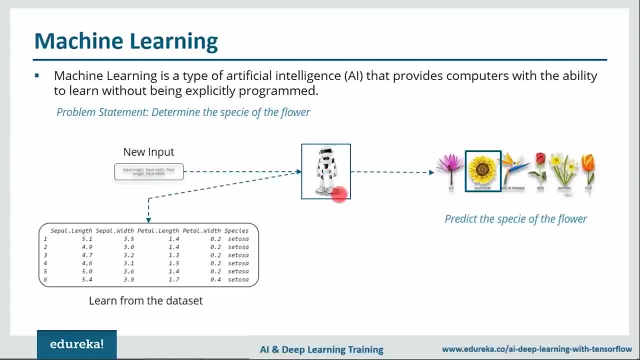 Then what happens? whenever you give a new input to this particular machine, it will predict the specie of the flower. So this is how machine learning works. It is nothing but machine learning in nutshell. So basically, I'll just revise it once more. 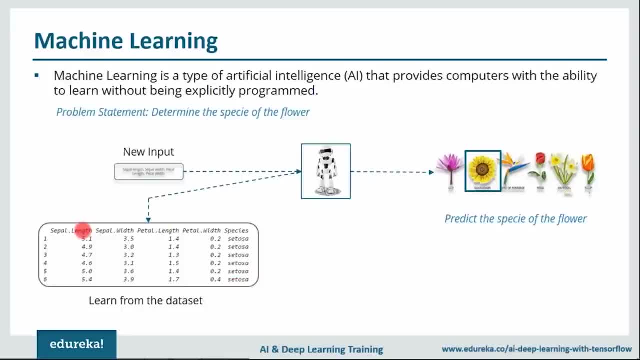 So you have a data set, So you split that data into training and testing data. So what happens? with the help of training data, you train your particular machine And after that you test it in order to determine the accuracy. And once it is done, 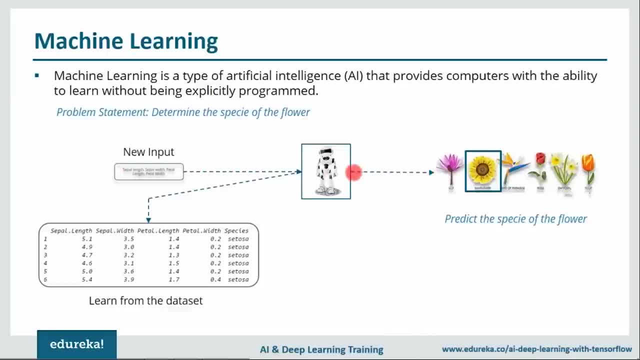 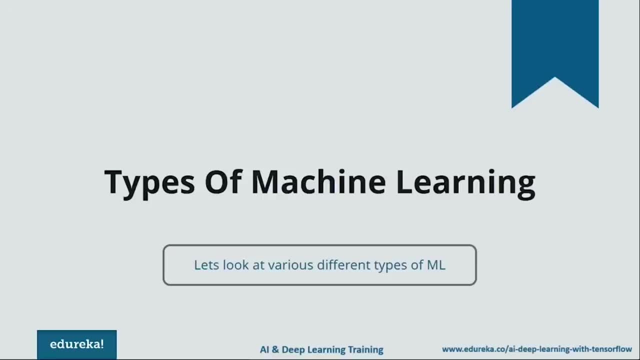 whenever you give the new input, it will predict the outcome or the desired outcome. So this is how machine learning works, guys, Let us move forward and understand various types of machine learning. So the first type is called supervised learning. Now, in supervised learning, what happens? 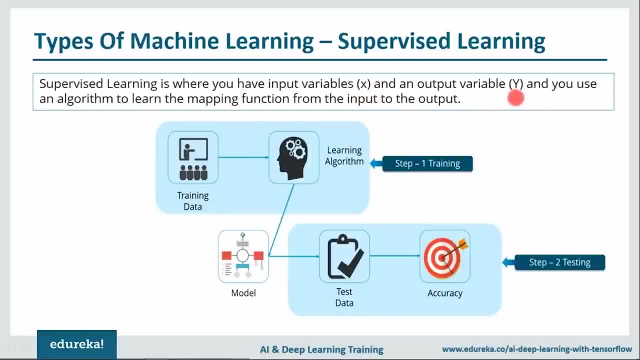 you have input variables x and an output variable y, And you can use an algorithm to learn, mapping function from the input to the output. Now let me simplify it for you. So what happens in supervised learning the data that you have? all it does is it takes the data. 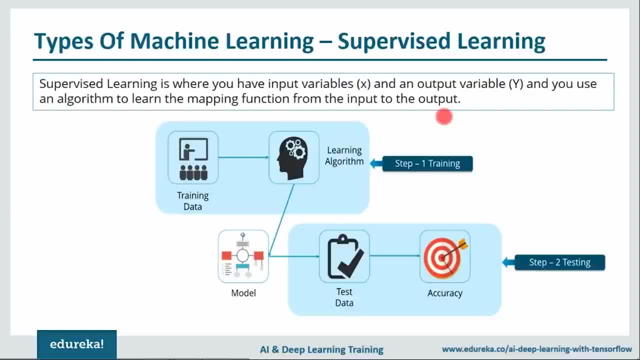 and it already contains the classification. Now let me talk about the previous example itself. So from our data set we knew that if we have this width, this length of our sepal and petal, so that will be the specie of flower. 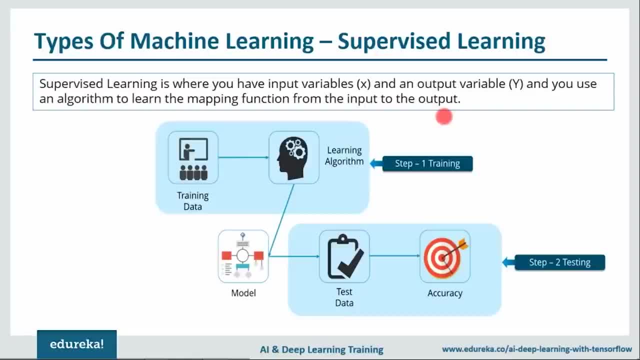 So the classifications are already defined. So that will be under supervised learning. Now let me tell you how it actually works. So you have data. you divide that data into training data as well as test data. So, on the basis of this training data, 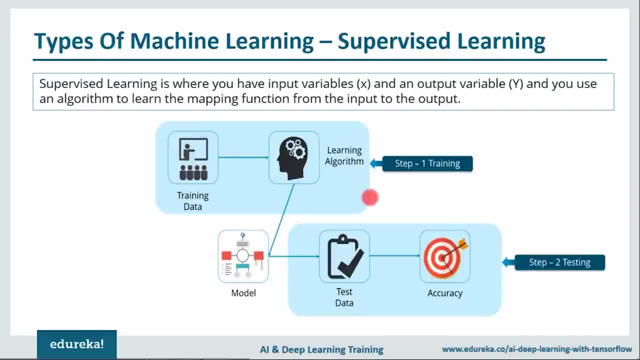 you train your machine And after that you create a model. So, as you can see that this phase is called training phase And after that you create a model. Now, in order to check this model, to get the accuracy- you have test data- 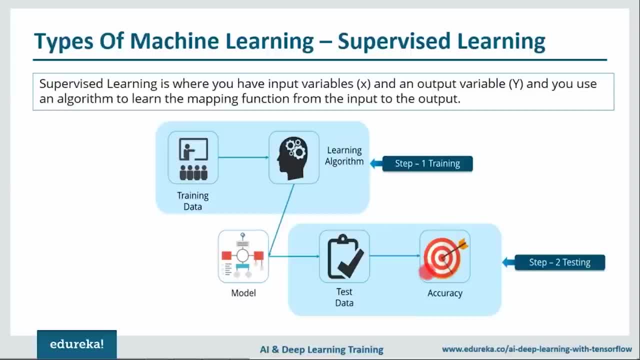 So you'll pass that test data and you'll see the accuracy. That is nothing but the actual output minus the output that is present in the test data. So with that you can get the accuracy. So this is all about supervised learning. 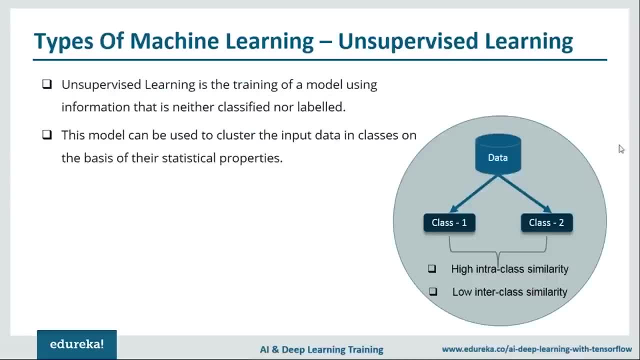 So we'll move forward and understand unsupervised learning. Now, in unsupervised learning, unlike supervised learning, you don't have any, any predefined classes. So what happens? You have data, So on the basis of that data, you try to create your own class. 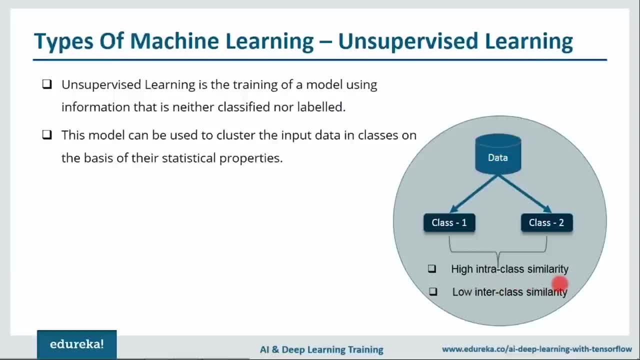 You try to make sure that whatever class you create has high intraclass similarities and have low interclass similarities. That means, if I've created two class like this, class one and class two, so the elements of this particular class should have high similarity. 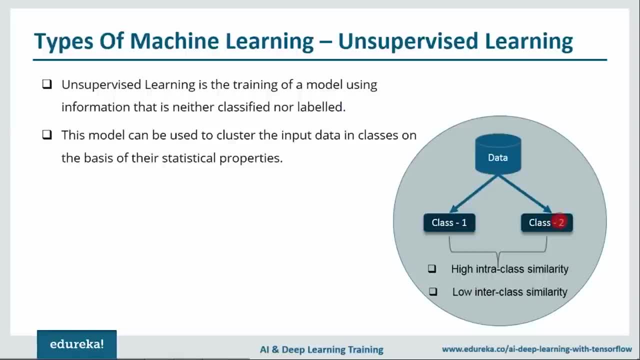 but at the same time it should have low similarity with the elements of class two. So you can think of examples as well of unsupervised learning. For example, if I have a data about my customers, So if I have a website and there are millions of visitors on my website, 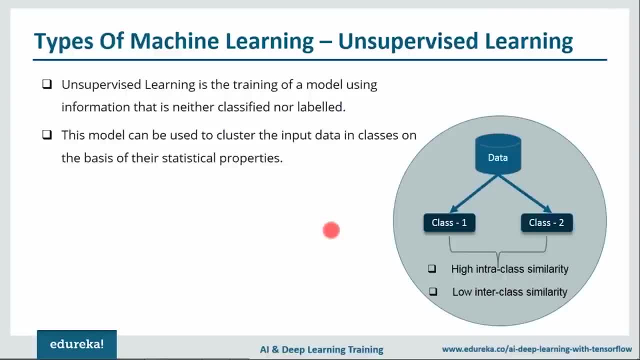 and I wanna make sure that I group people on various criteria. For example, I can group people on the basis of willingness to purchase a product that is there on my website or where they are coming from. what is the source? all those things? 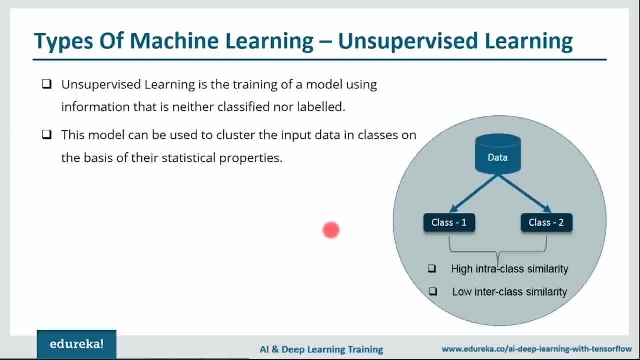 So I wanna group my customers and I wanna make sure that I have certain high priority customers and I have low priority customers and I have medium priority customers. So with the help of unsupervised learning, I can actually do that. I can make certain classes of people. 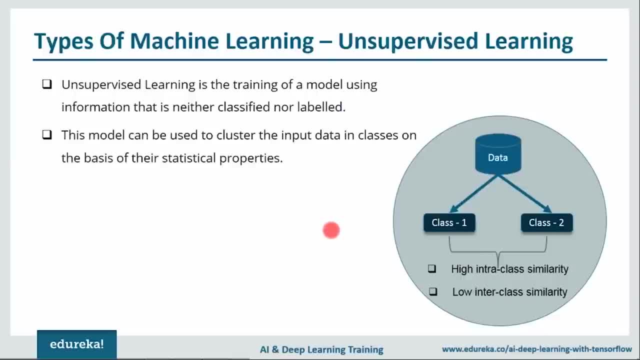 on whom I should focus more on as compared to the other class. So this was just an example, guys, You can use it in various other fields as well. So in marketing, this is how you can use unsupervised learning. So this brings us to our next type of machine learning. 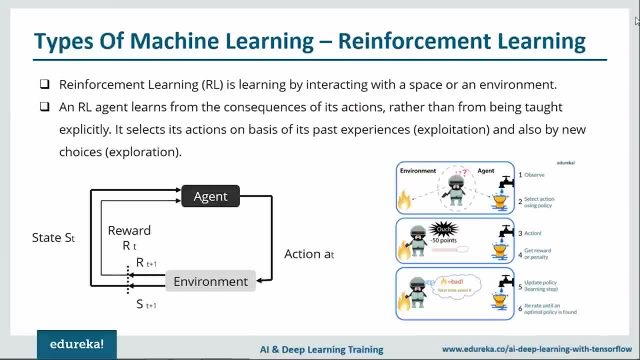 which is called reinforcement learning. Now, this is reinforcement learning, guys. Now what happens in reinforcement learning? the machine learns by interacting with space or an environment. So it learns with an experience, with its past experience and also by new choice exploration. 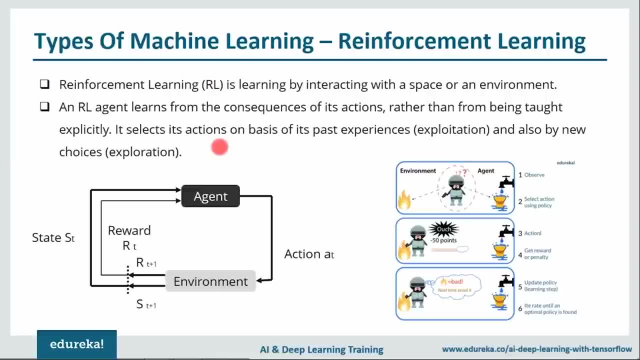 Now I'll take the analogy of dogs. So if you have any dog or a pet at your home, so if you have trained your dog in order to get the newspaper, and if it gets it, then you reward it with some chocolate or things that the dog likes, right? 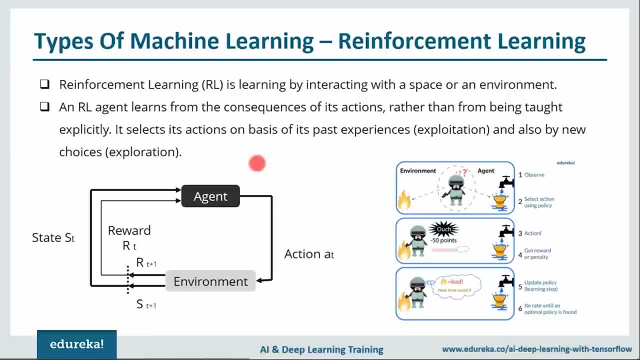 So the dog will know, whatever he has done, he's actually rewarded for that. So it'll continue doing that. But apart from that, if he does something else, if instead of the newspaper he brings something else, So what you'll do? 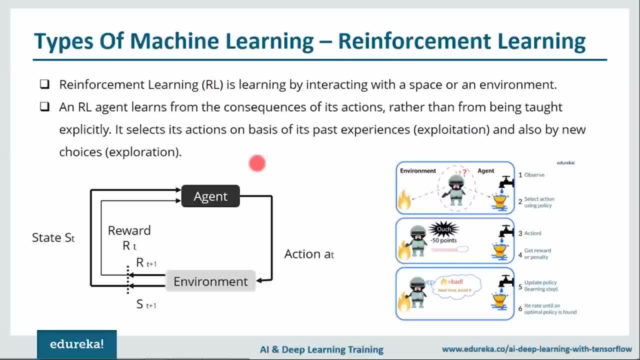 you might even punish it. So because of that, the dog will come to know that it has to get a newspaper every morning. Now the same example is there in front of your screen. So you have this machine, So it has two choices. 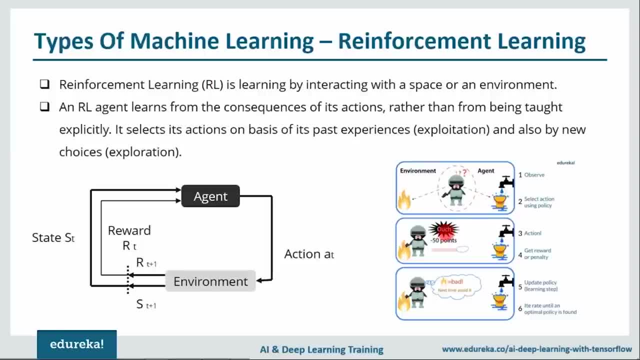 either to touch the fire or touch the water. Now, first what it does: it goes on and touch the fire, So because of that it gets some burning sensation. Now it has only other option, that is, to touch the water. So when it touched the water, 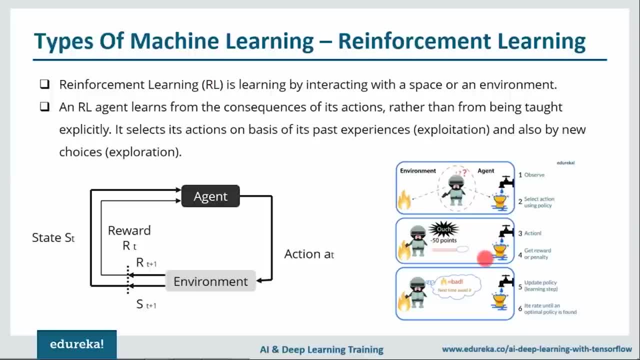 it gets some reward. So because of that, it'll understand that it does not have to touch fire ever again. Now there's a diagram that is there in front of your screen. So what happens is you have an agent. that agent performs some action. 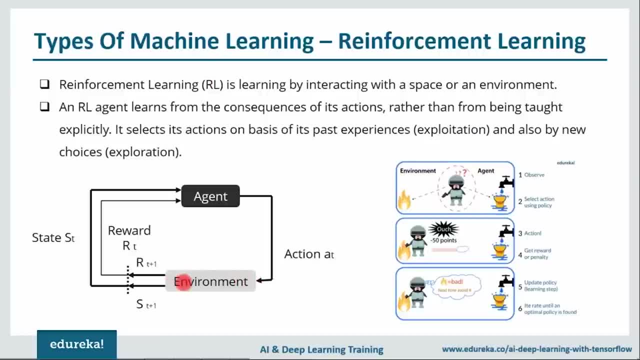 And on the basis of that action, it'll be exposed to some sort of an environment. Now, if that action is correct, then it'll be rewarded with that, But if it is not, then it'll change its choice and it'll again perform some action. 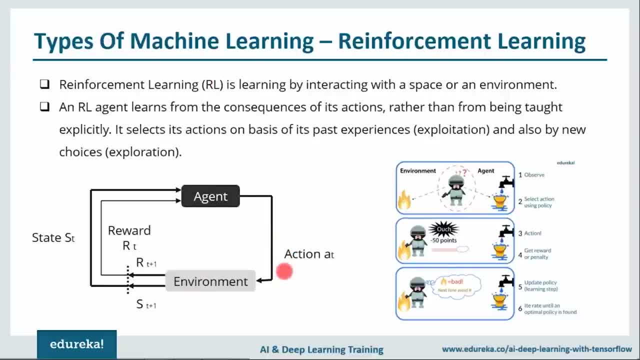 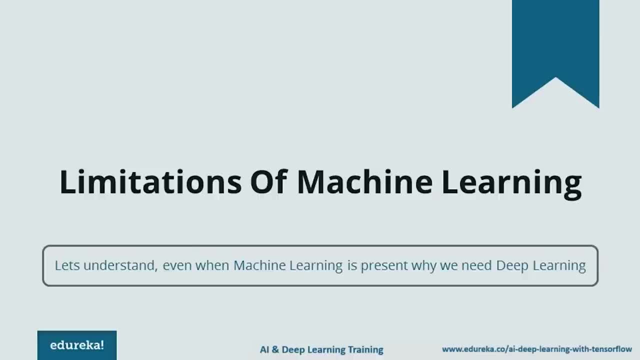 So this process will keep on repeating. So this is how reinforcement learning works. So let us move forward and understand. when we have machine learning, why do we need deep learning? That is, we'll look at various limitations of machine learning Now. the first limitation is: 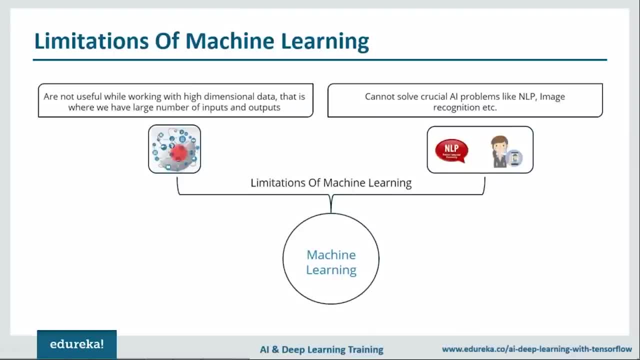 is high dimensionality of the data. Now, the data that is now generated is huge in size, So we have a very large number of inputs and outputs. So due to that, machine learning algorithms fail, So they cannot deal with high dimensionality of data. 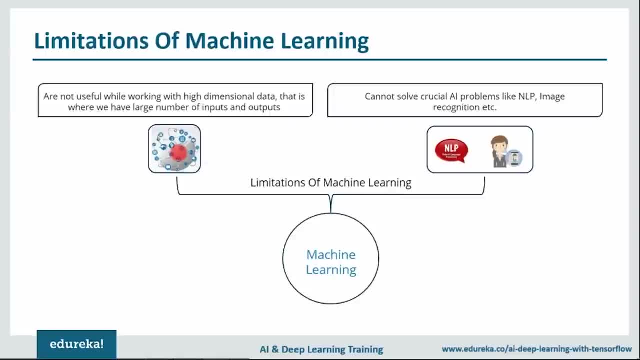 or you can say, data with large number of inputs and outputs. Now there's another problem as well, in which it is unable to solve the crucial AI problems, which can be natural language processing, image recognition and things like that. Now one of the biggest challenges. 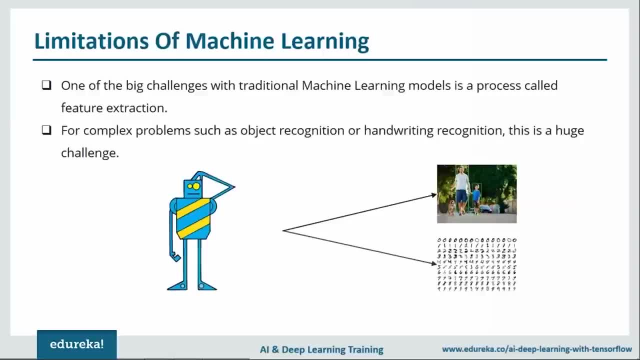 with machine learning models is feature extraction. Now let me tell you what are features. So in statistics we consider features as variables, But when we talk about artificial intelligence, these variables are nothing but the features. Now, what happens because of that? the complex problems such as object recognition. 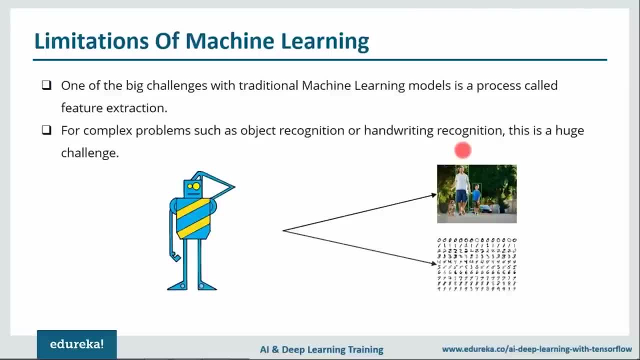 or handwriting recognition, becomes a huge challenge for machine learning algorithms to solve. Now let me give you an example of this feature extraction Suppose, if you want to predict that, whether there'll be a match today or not. So it depends on our various features. 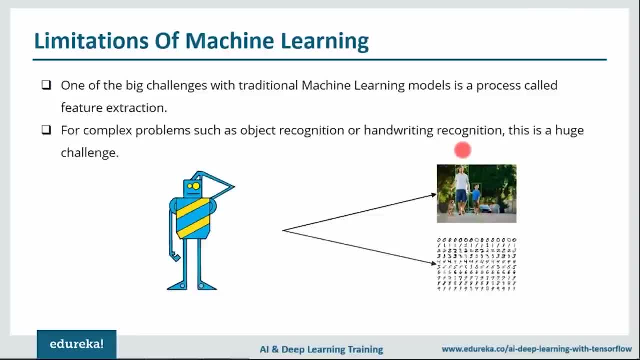 It depends on whether the weather is sunny, whether it is windy, all those things. So we have provided all those features in our dataset, But we have forgot one particular feature, that is, humidity, And our machine learning models are not that efficient that they'll automatically generate that particular feature. 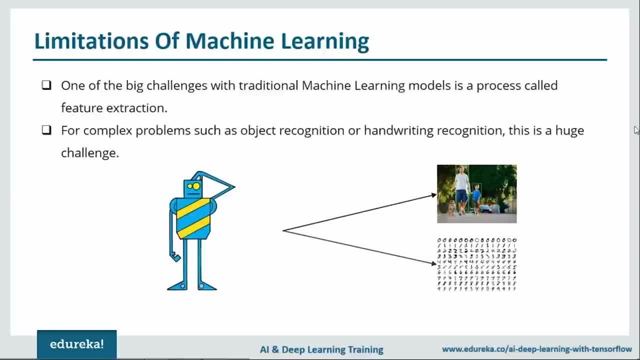 So this is one huge problem, or you can say limitation, with machine learning. Now, obviously we have limitation and it won't be fair that if I don't give you the solution to this particular problem So we'll move forward and understand how deep learning solves these kind of problems. 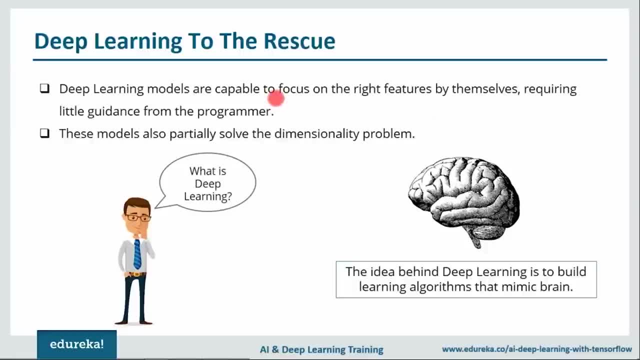 Now, as you can see, that the first line on your slide, which says that deep learning models are capable to focus on the right features by themselves, requiring little guidance from the program. So, with the help of little guidance, what these deep learning models can do. 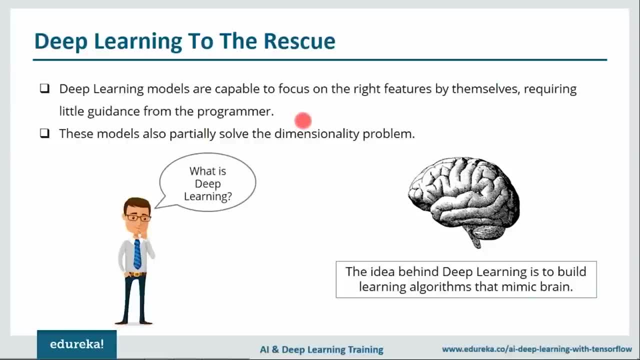 they can generate their features, on which the outcome will depend on, And, at the same time, it also solves the dimensionality problem as well. If you have very large number of inputs and outputs, you can make use of a deep learning algorithm. Now, what exactly is deep learning? 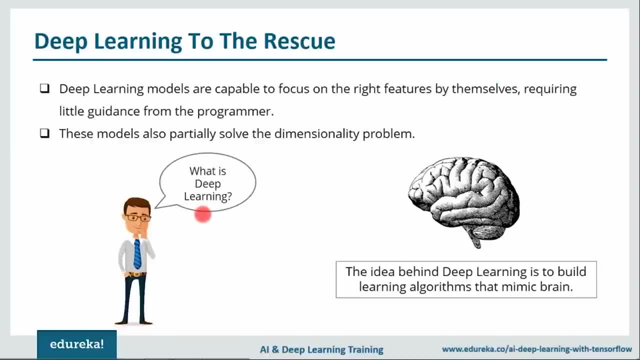 Again, since we know that it has been evolved by machine learning, and machine learning is nothing but a subset of artificial intelligence, And the idea behind artificial intelligence is to imitate the human behavior. The same idea is for the deep learning as well, is to build learning algorithms that can mimic brain. 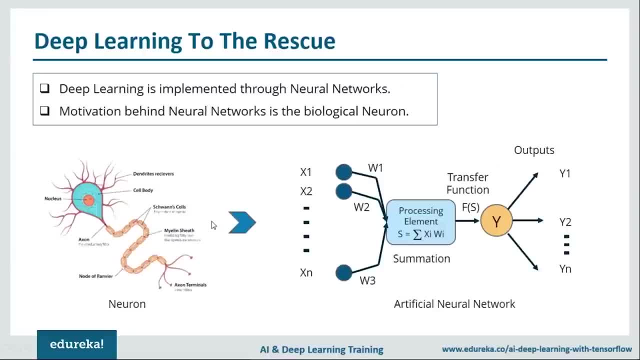 Now let us move forward and understand deep learning. what exactly it is? Now, the deep learning is implemented with the help of neural networks, And the idea or the motivation behind neural networks are nothing but neurons. What are neurons? These are nothing but your brain cells. 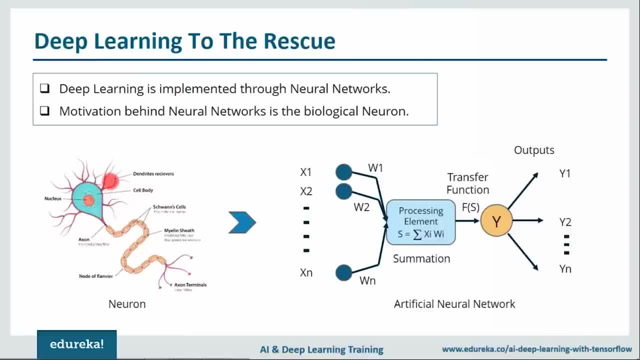 Now here's a diagram of neuron. So we have dendrites here which are used to provide input to a neuron. As you can see, we have multiple dendrites here, So these many inputs will be provided to a neuron. Now this is called cell body. 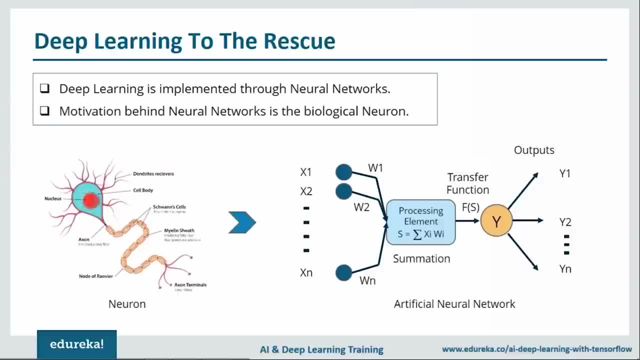 And inside the cell body we have a nucleus which performs some function. After that, that output will travel through exon and it will go towards the exon terminals, And then this neuron will fire this output towards the next neuron. Now the studies tell us that the next neuron 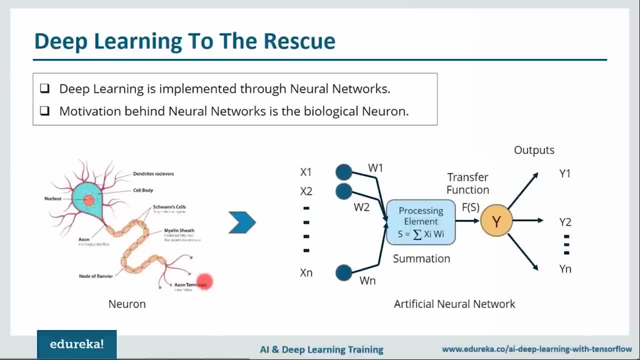 now all you can see, the two neurons are never connected to each other. There's a gap between them, So that is called a synapse. So this is how basically a neuron works like, And on the right-hand side of your slide you can see an artificial neuron. 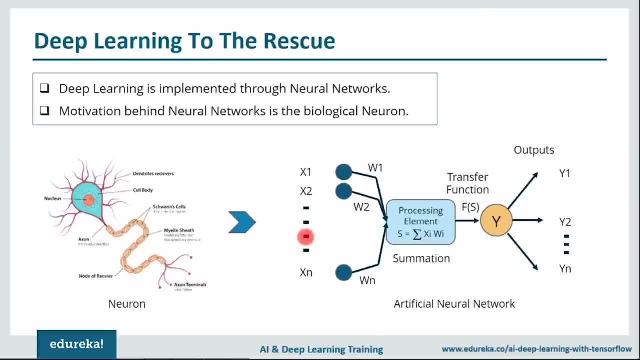 Now let me explain you that. So over here, similar to neurons, we have multiple inputs. Now these inputs will be provided to a processing element, like a cell body, And over here in the processing element, what will happen? summation of your inputs and weights. 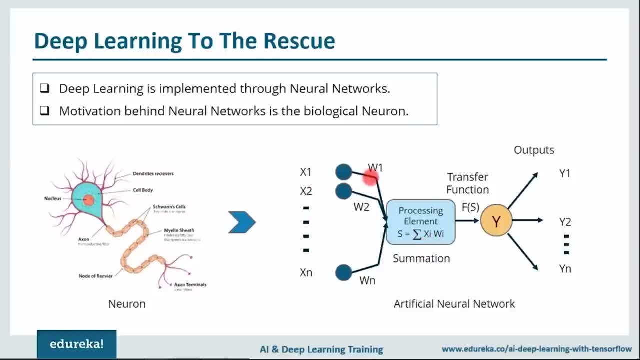 Now, when it moves on, then what will happen? this input will be multiplied with our weights. So in the beginning, what happens? these weights are randomly assigned. So what will happen if I take the example of X1?? So X1 multiplied by W1. 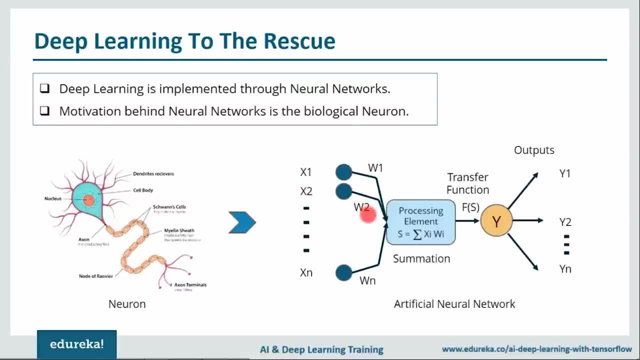 will go towards the processing element. Similarly, X2 and W2 will go towards the processing element And similarly the other inputs as well, And then summation will happen, which will generate a function of S, that is F of S. 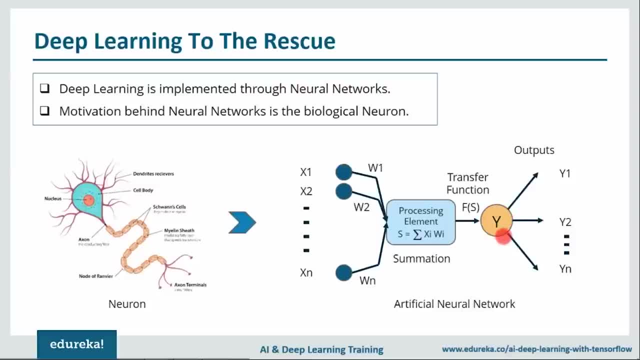 After that comes the concept of activation function. Now, what is activation function? It is nothing but in order to provide a threshold. So if your output is above the threshold, then only this neuron will fire. otherwise it won't fire. So you can use a step function as an activation function. 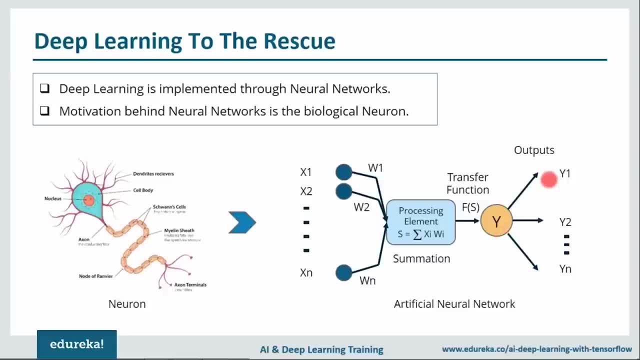 or you can even use a sigmoid function as your activation function. So this is how an artificial neuron looks like. So a network will be multiple neurons which are connected to each other will form an artificial neural network And this activation function can be a sigmoid function. 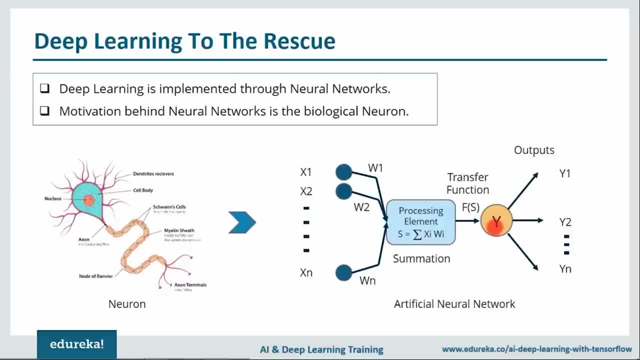 or a step function. that totally depends on your requirement. Now, once it exceeds the threshold, it'll fire. After that, what will happen? it will check the output Now if this output is not equal to the desired output. so these are the actual outputs. 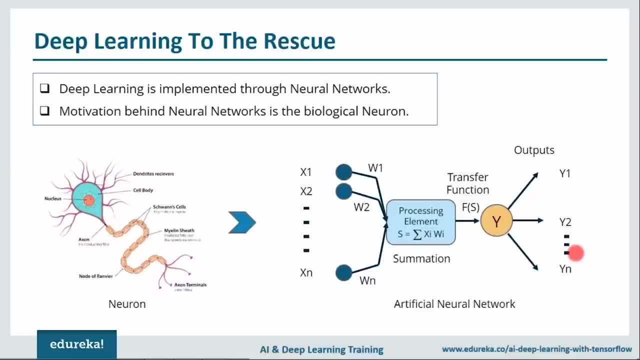 and we know the real outputs. So we'll compare both of that and we'll find the difference between the actual output and the desired output. On the basis of that difference, we are again going to update our weights And this process will keep on repeating. 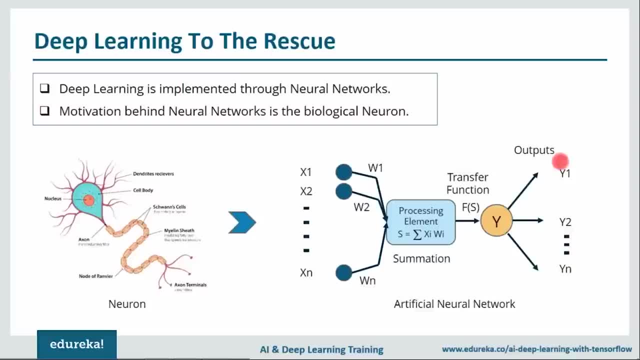 until we get the desired output as our actual output. Now, this process of updating weight is nothing but your back propagation method. So this is neural networks in a nutshell. So we'll move forward and understand what are deep networks. So, basically, deep learning is implemented. 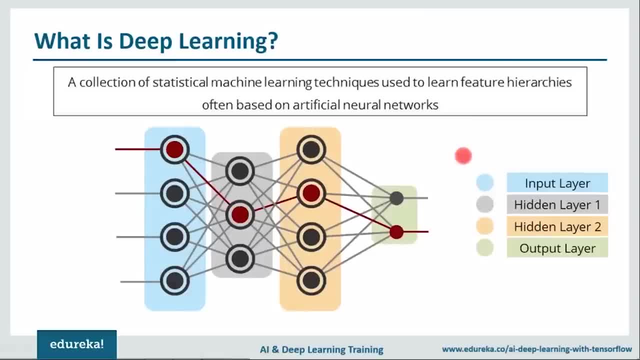 by the help of deep networks, and deep networks are nothing but neural networks with multiple hidden layers. Now, what are hidden layers? Let me explain you that. So you have inputs that come there. This will be your input layer. After that, some process happens and it'll go to the next node. 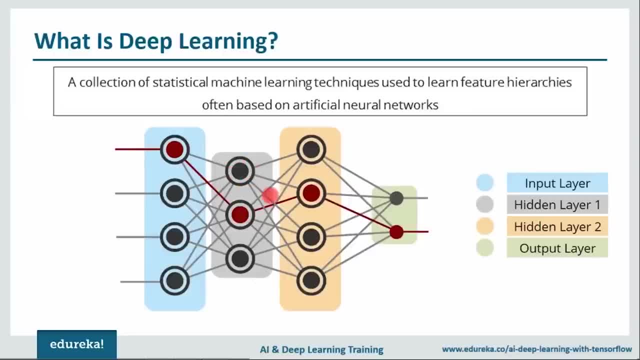 or you can say to the hidden layer nodes: So this is nothing but your hidden layer one, So every node is interconnected, if you can notice, After that you have one more hidden layer where some function will happen And, as you can see, that again 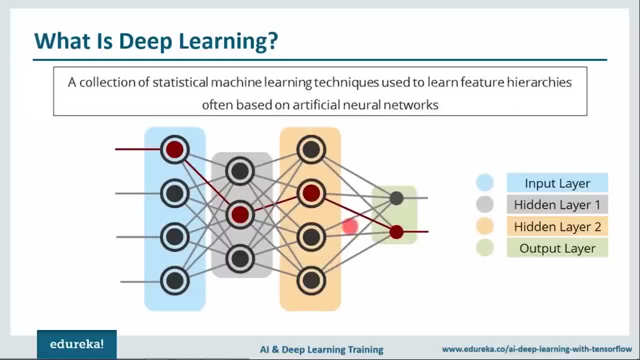 these nodes are interconnected to each other. After this hidden layer two comes the output layer. And this output layer again, we are going to check the output whether it is equal to the desired output or not. If it is not, we are again going to update the weights. 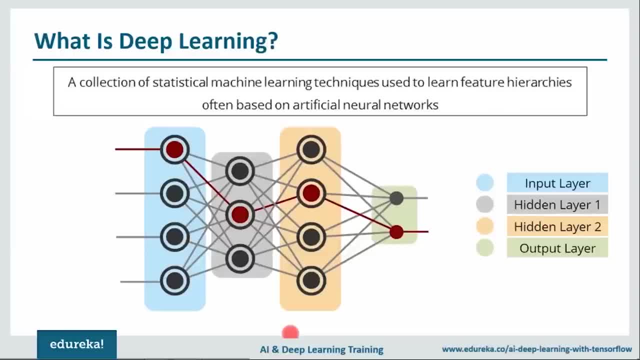 This is how a deep network looks like. Now, there can be multiple hidden layers. There can be hundreds of hidden layers as well, But when we talk about machine learning, that was not the case. We were not able to process multiple hidden layers. when we talk about machine learning, 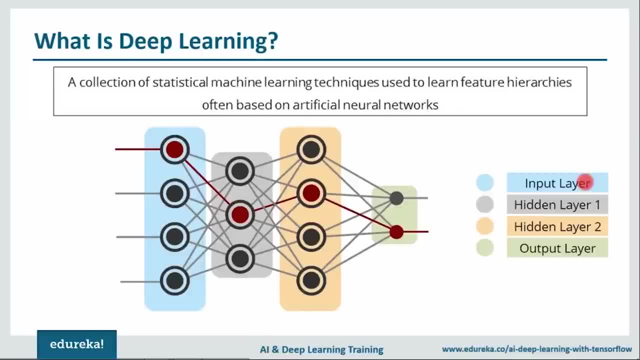 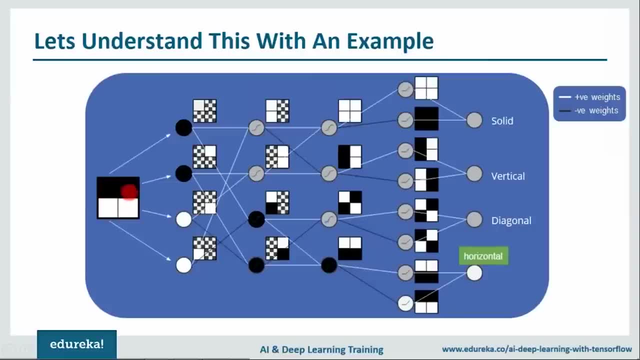 So, because of deep learning, we have multiple hidden layers at once. Now let us understand this with an example. So we'll take an image which has four pixels. So, if you can notice, we have four pixels here, among which the top two pixels are bright. 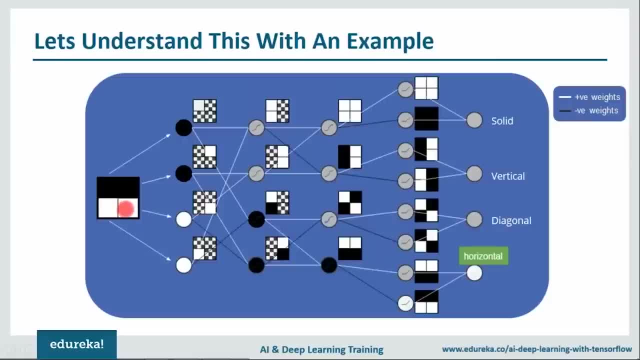 that is, they're black in color, whereas the bottom two pixels are white. Now what happens? we'll divide these pixels and we'll send these pixels to each and every node, So for that we need four nodes, So this particular pixel will go to this node. 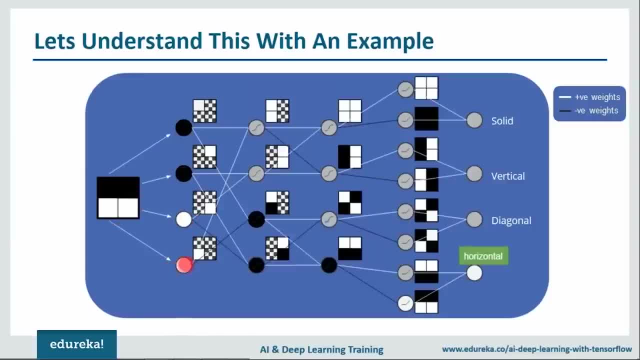 it will go to this node, this pixel will go to this node and, finally, this pixel will go to this particular node that I'm highlighting with my cursor. Now what happens? We provide them random weights, So these white lines actually represent the positive weights. 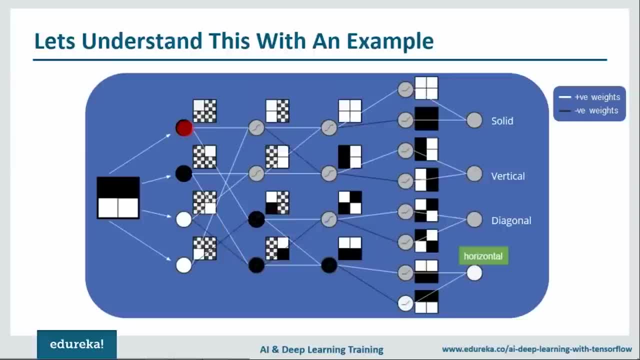 and these black lines represent the negative weights. Now, this particular brightness: when we display high brightness, we'll consider it as negative. Now what happens? When you see the next output or the next hidden layer? it'll be provided with the input, with this particular layer. 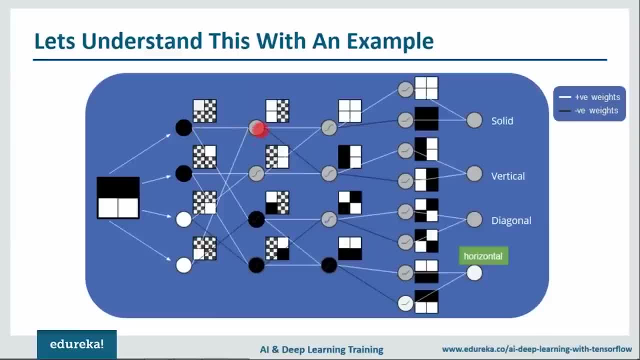 So this will provide an input with positive weight to this particular node, and the second input will come from this particular node, Since both of them are positive. so we'll get this kind of a node, Similarly this node as well. Now, when I talk about these two nodes, 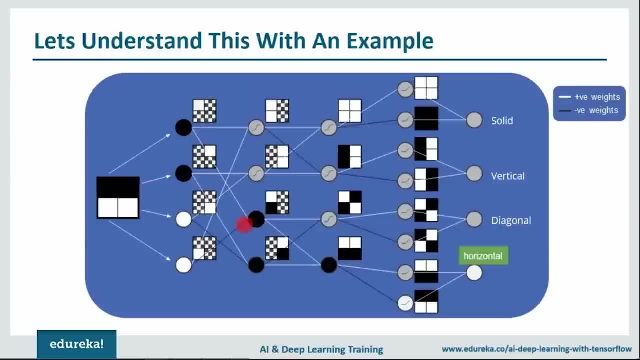 the first node over here, so this is getting input from this node as well as from this node. Now over here we have a negative weight, So because of that, the value will be negative and we have represented that with black color. 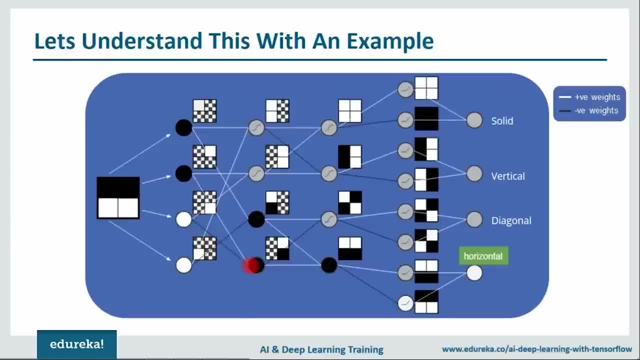 Similarly over here as well. we're getting one input from here which has a negative weight and the another input from here which again has a negative weight. So accordingly, we get again a negative value here. So these two becomes black in color. 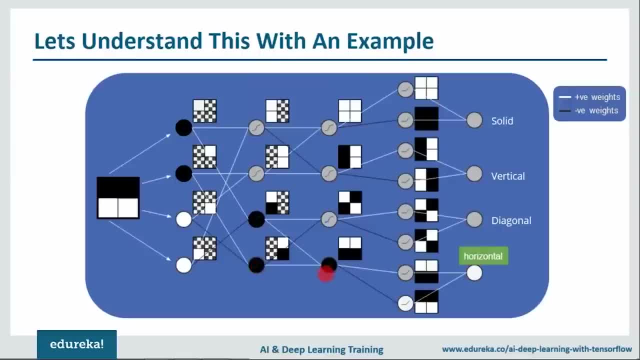 Now, if you notice what'll happen next, we'll provide one input here, which will be negative, and a positive weight, which will be again negative, and this will be also negative and a positive weight, So that'll again come out to be negative. 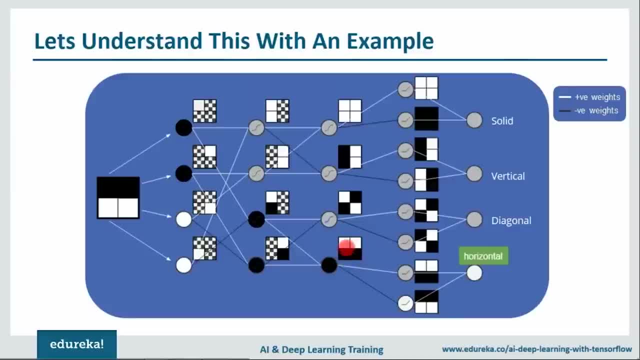 So that is why we have got this kind of a structure. If you notice this, this is nothing but the inverse of this particular image. When I talk about this node over here, we are getting the negative value with a positive weight, which is negative. 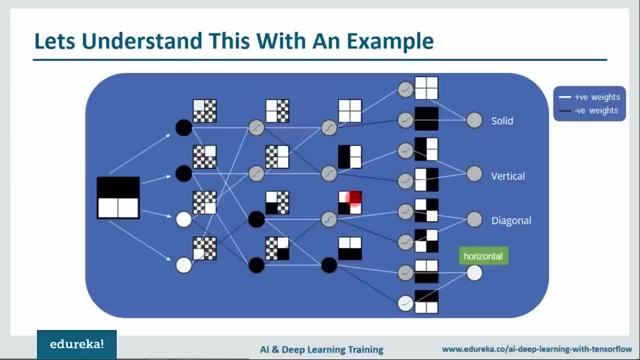 and a negative value with a negative weight which is positive. So we are getting something which is positive here. Now, obviously, I want this particular image to get inverse. I want these black strips to come up. So what I'll do? I'll actually calculate the inverse. 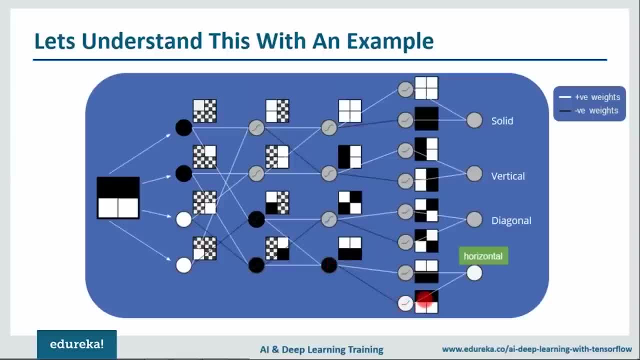 by providing a negative weight like this. So over here I've provided a negative weight, it'll come up. So when I provide a positive weight, so it'll stay wherever it is. After that it'll detect and the output you can see. 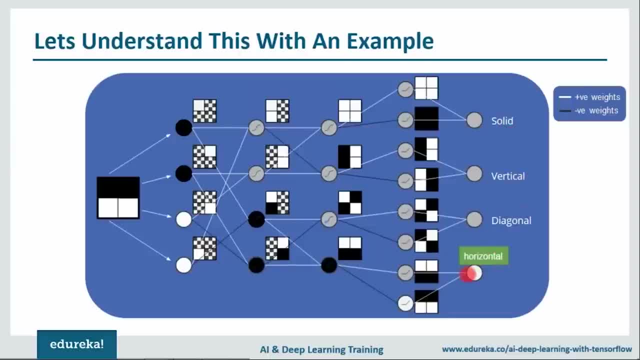 will be a horizontal image, Not a solid, not a vertical, not a diagonal, but a horizontal, And after that we are going to calculate the difference between the actual output and the desired output and we are going to update the weights accordingly. 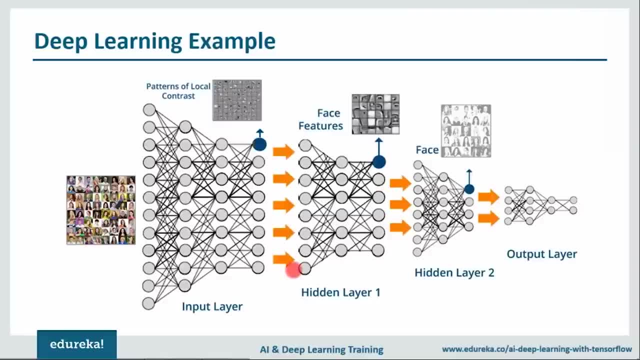 Now, this is just an example, guys. So, guys, this is one example of deep learning, where what happens? we have images here, We provide these raw data to the first layer, to the input layer. Then what happens? these input layers? 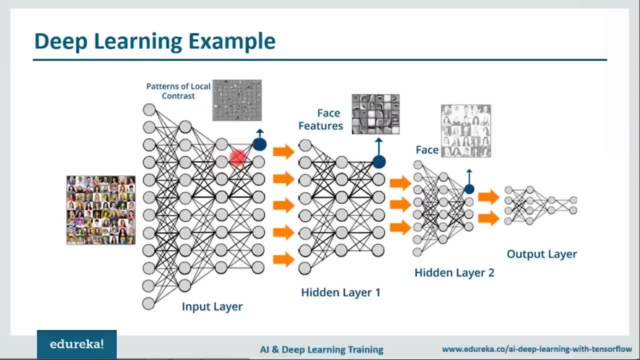 will determine the patterns of local contrast or it'll fixate those patterns of local contrast, which means that it will differentiate on the basis of of colors and luminosity and all those things. So it'll differentiate those things And after that, in the following layer, what'll happen? 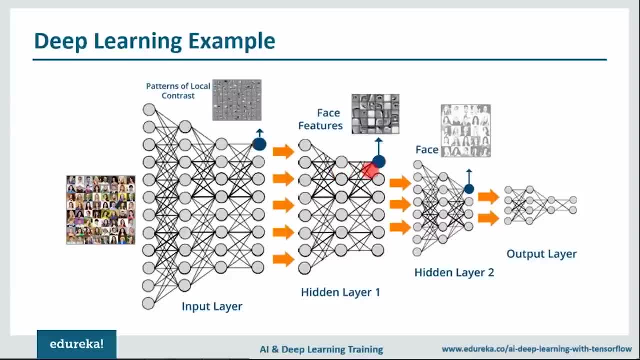 it'll determine the face features, it'll fixate those face features, So it'll form nose, eyes, ears, all those things. Then what'll happen? it'll accumulate those correct features for the correct face, or you can say that it'll fixate. 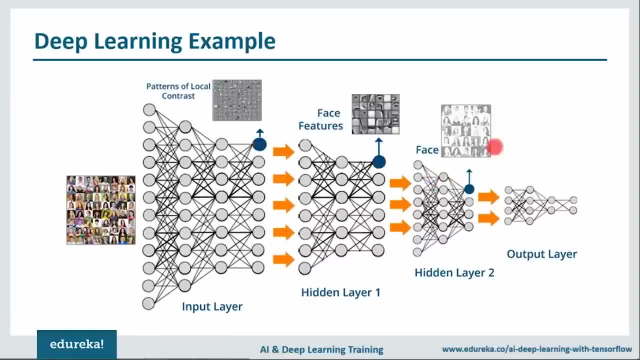 those features on the correct face template. So it'll actually determine the faces here as you can see it over here, And then it'll be sent to the output layer. Now, basically, you can add more hidden layers to solve more complex problem. 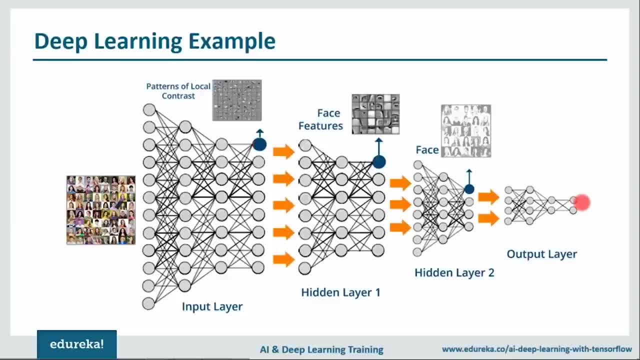 For example, if I wanna find out a particular kind of face, for example a face which has large eyes or which has light complexion, So I can do that by adding more hidden layers, And I can increase the complexity also at the same time. 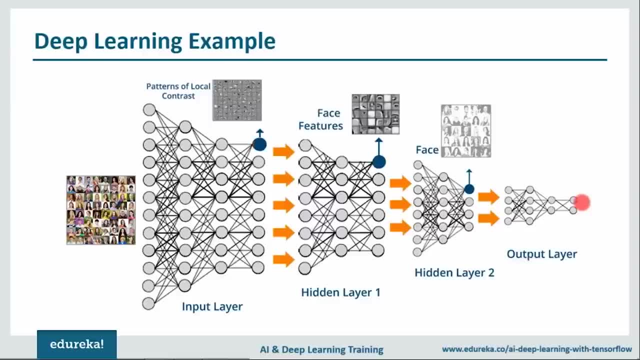 if I wanna find which image contains a dog, So for that also I can have one more hidden layer. So as and when hidden layer increases, we are able to solve more and more complex problem. So this is just a general overview of how a deep network looks like. 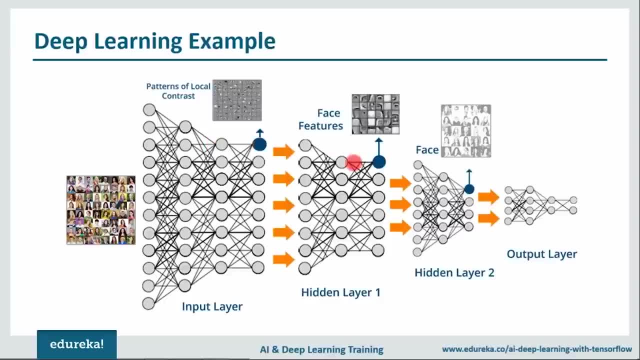 So we have first patterns of local contrast in the first layer. Then what happens? we fixate these patterns of local contrast in order to form the face features, such as eyes, nose, ears, et cetera, And then we accumulate these features for the correct face. 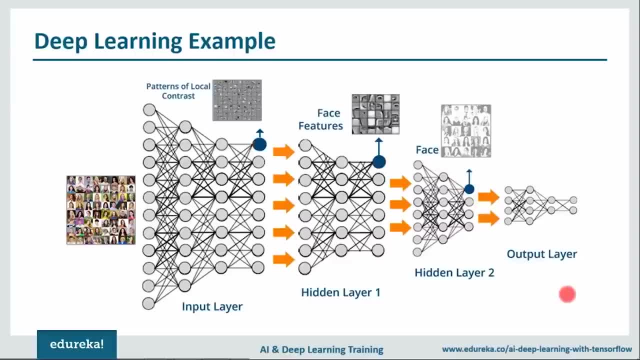 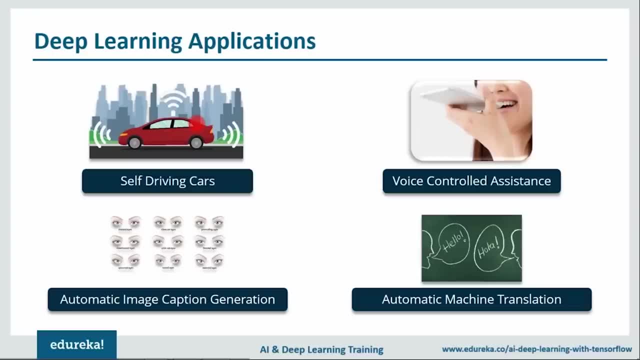 and then we determine the image. So this is how a deep learning network- or you can say deep network- looks like, And I'll give you some applications of deep learning. So here are a few applications of deep learning. It can be used in self-driving cars. 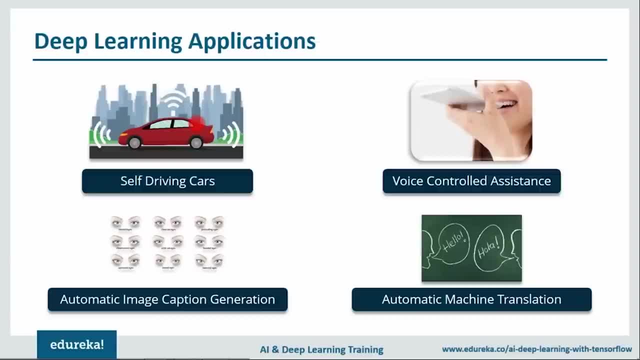 So you must have heard about self-driving cars. So what happens? it'll capture the images around it, it'll process that huge amount of data and then it'll decide what action should it take. should it take left right? should it stop? 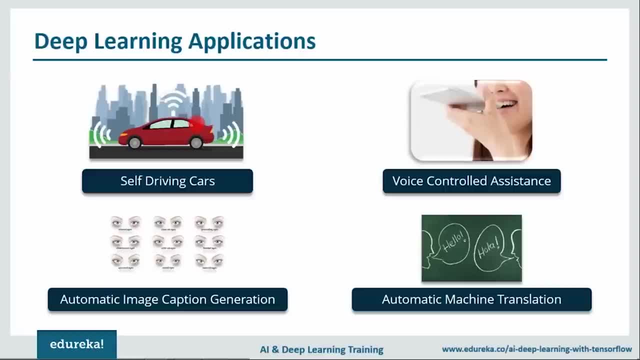 So, accordingly, it'll decide what action should it take, And that'll reduce the amount of accidents that happens every year. Then, when we talk about voice control assistance, I'm pretty sure you must have heard about Siri. All the iPhone users know about Siri, right? 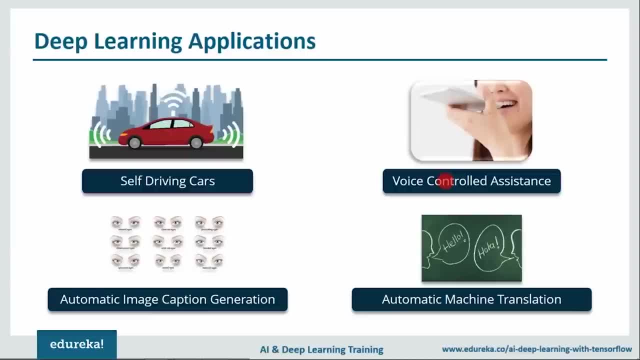 So you can tell Siri: whatever you wanna do, it'll search it for you and display for you. Then, when we talk about automatic image caption generation, so what happens in this? whatever image that you upload, the algorithm is in such a way that it'll generate the caption accordingly. 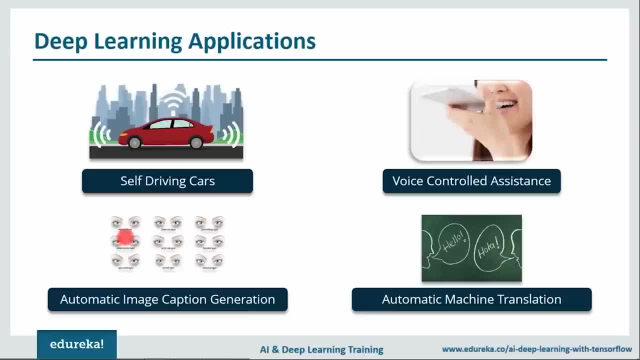 So, for example, if you have, say, blue colored eyes, so it'll display a blue colored eye caption at the bottom of the image. Now, when I talk about automatic machine translation, so we can convert English language into Spanish, similarly Spanish to French. 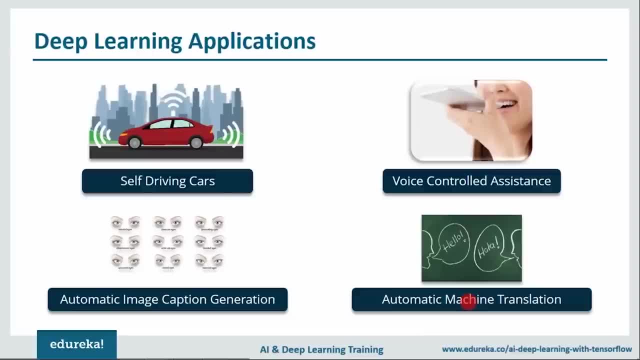 So, basically, automatic machine translation. you can convert one language to another language with the help of deep learning. And these are just a few examples, guys. There are many, many other examples of deep learning. It can be used in game playing. 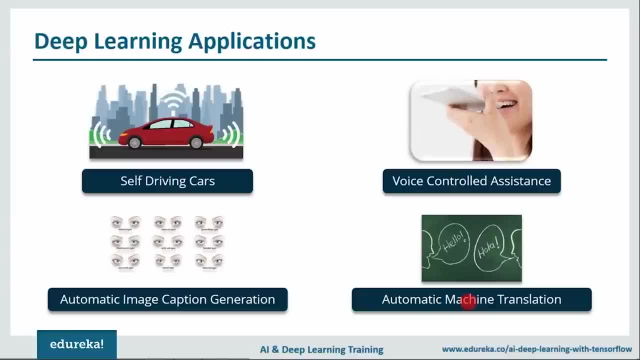 it can be used in many other things. And let me tell you one very fascinating thing that I've told you in the beginning as well: With the help of deep learning, MIT is trying to make sure that we're able to predict future. So yeah, I know it is growing exponentially right now, guys. 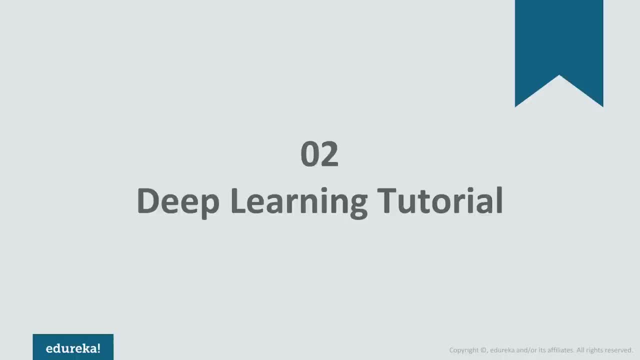 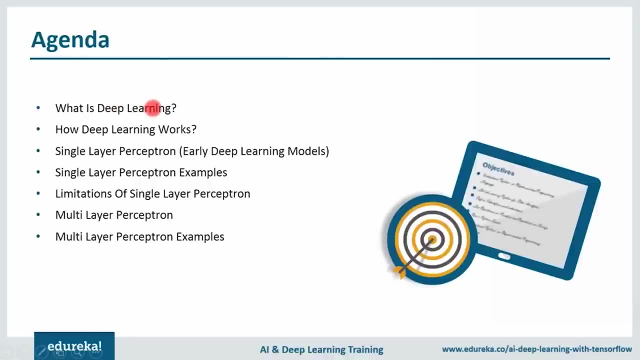 Welcome to today's session on deep learning tutorial with TensorFlow. So let us move forward and have a look at the agenda for today. So this is the agenda for today. guys, We'll understand what exactly is deep learning and how it works. So we'll look at the motivation behind deep learning. 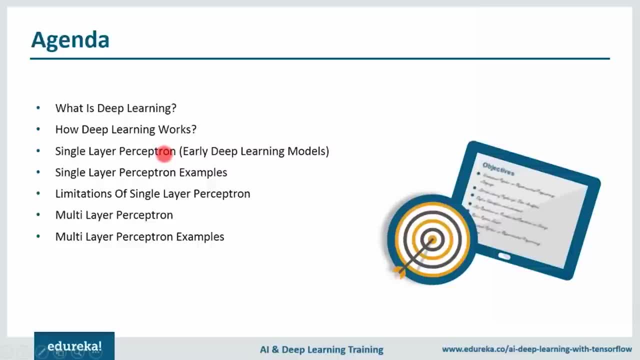 and how it actually evolved. Then we'll focus on single layer perceptron, which are nothing but the early deep learning models. We'll also look at various examples of single layer perceptron. And, guys, when I talk about perceptron, these are nothing but the artificial neurons. 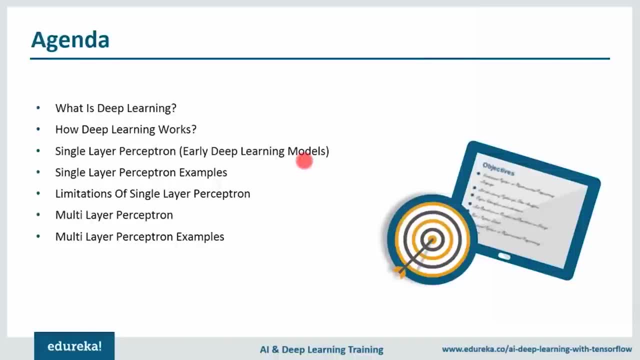 And what are neurons? Neurons are your brain cells. Then we'll also understand the limitations of single layer perceptron that led to the evolution of multi-layer perceptron. We'll understand how multi-layer perceptron overcame those limitations And we'll also look at various examples. 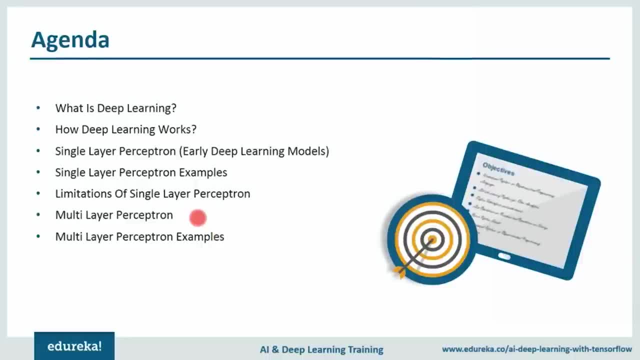 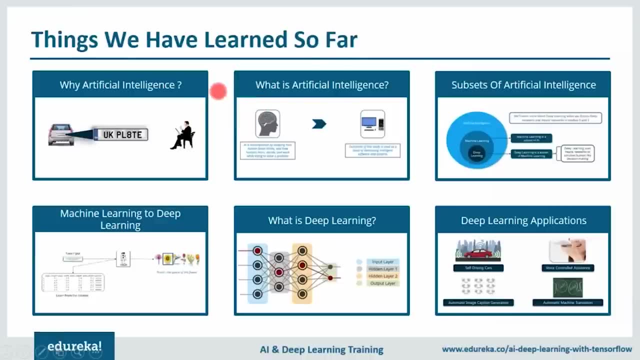 of multi-layer perceptron. Fine guys, let us move forward and understand what all things we have understood so far. So, guys, these are the things that we have studied in the previous session. We first understood why artificial intelligence, what is the need of artificial intelligence? 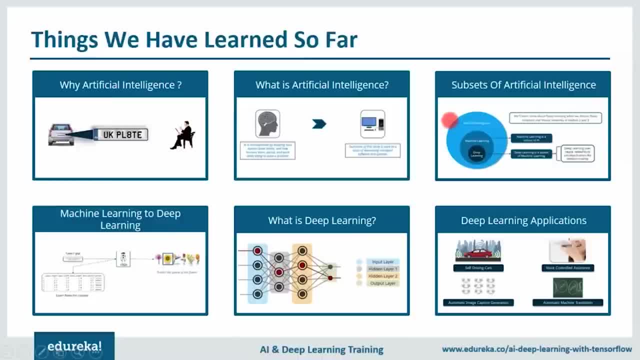 Then we saw what exactly it is and we also focused on various subsets of artificial intelligence, that is, machine learning and deep learning. Then we understood how we came from machine learning to deep learning and we saw what exactly is deep learning, along with various applications of deep learning. 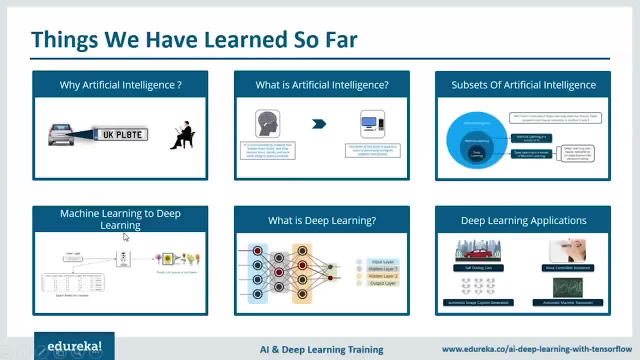 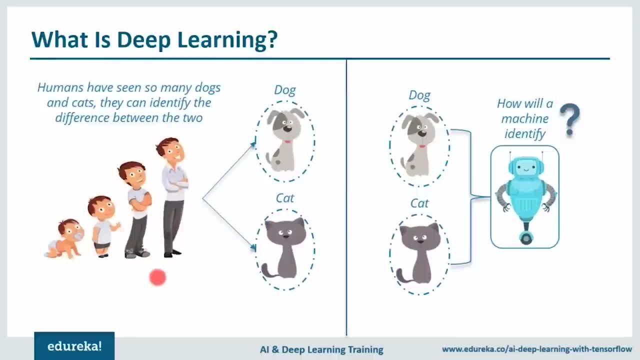 So, guys, we'll move forward now and understand what exactly is deep learning and how it works. So, guys, let us understand deep learning with an analogy. So how do you think our brain is able to identify the difference between a dog and a cat? 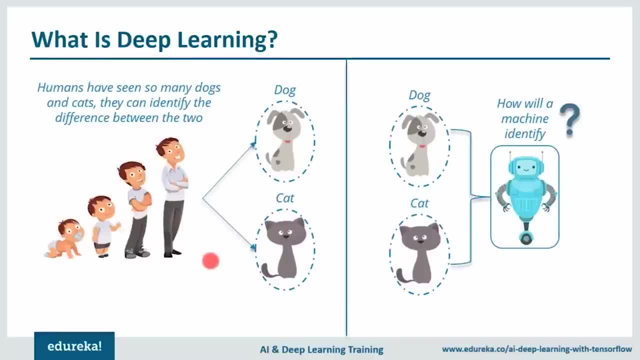 So the reason is, since the day we are born, we are actually seeing different types of cats and dogs in our day-to-day life And because of that we are able to identify the difference or spot the difference between the two, that is, dog and a cat. 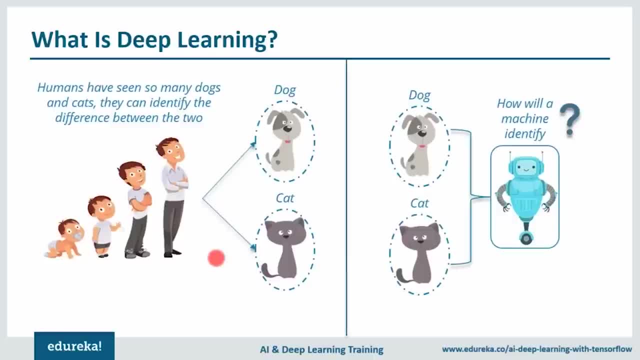 Even if we see different types of cats and dogs, we still know which is a cat and which is a dog. So this is because we have seen a lot of cats and dogs in our entire life. But what if I want a machine to do that task for me? 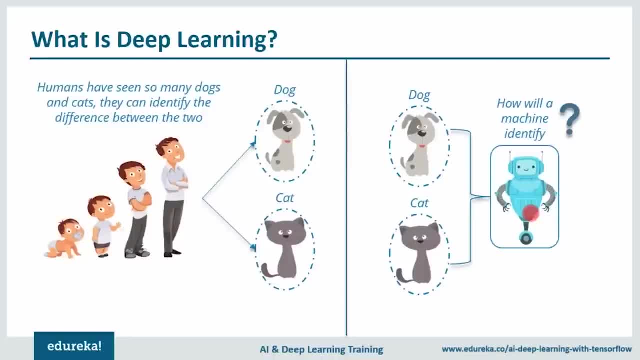 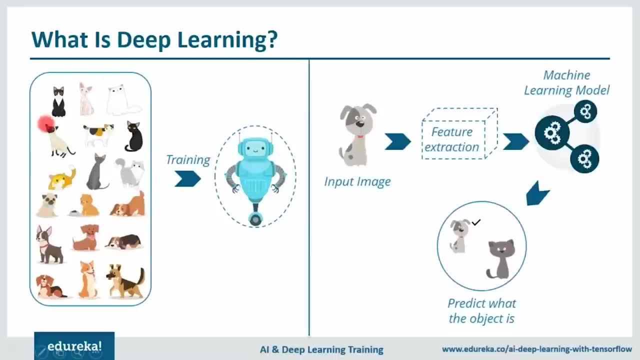 So how will a machine identify whether the given image is of a dog or a cat? So one way of doing that is we can train our machine to a lot of images, a lot of images of different cats and dogs, that is, different breeds of cats and dogs. 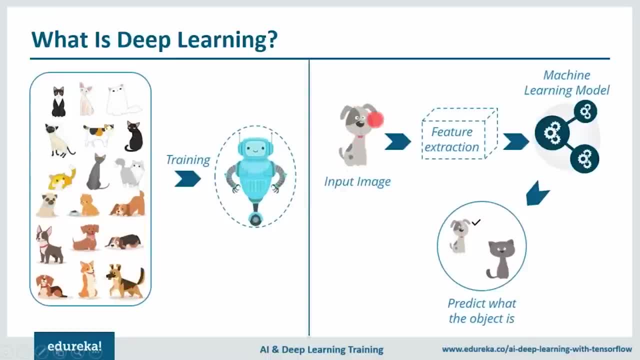 And then what'll happen once our training is done. we can provide it with an input image. then we'll manually extract certain features, Features like nose, whiskers, colors, edges, it can be anything. The important features which actually helps us. 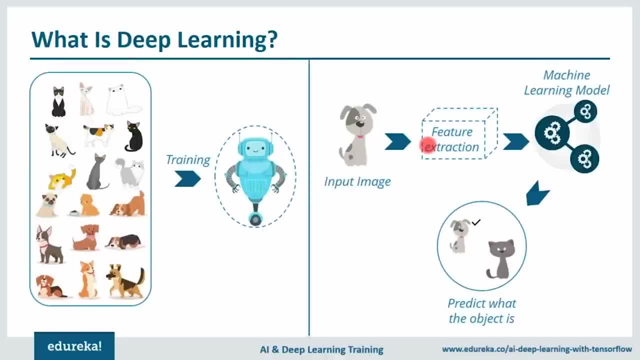 in classifying whether the input image is a cat or a dog, Then we make machine learning model with that and once it is done our machine learning model is able to predict whether the input image is of a cat or a dog. But if you notice here one very big disadvantage with this, 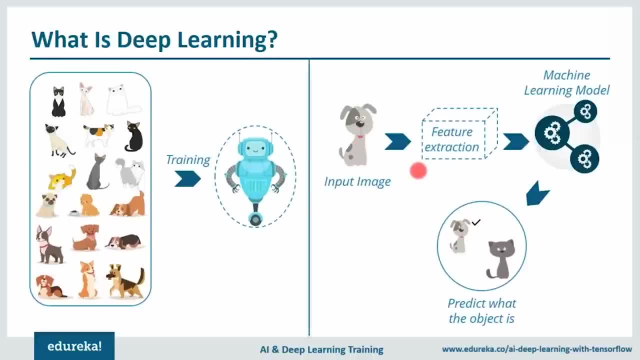 is, we have to manually extract features, features such as nose whiskers, all those features. we have to manually extract it and provide it to our machine learning model. And trust me guys, in every scenario it is not possible. If you have large number of inputs, you cannot do that. 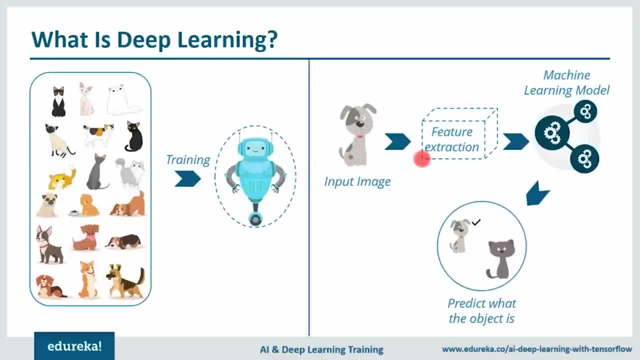 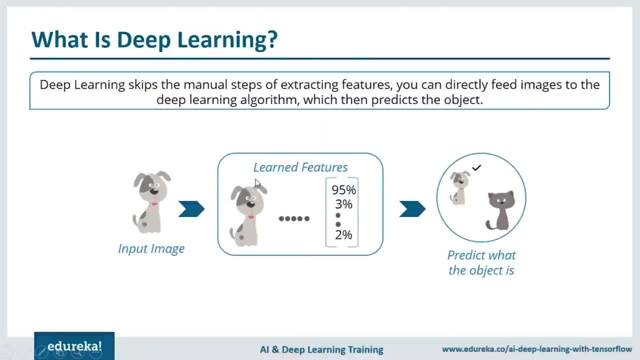 You cannot manually extract the features, or basically, you can say columns which are important for you in order to predict what the object is right, And that led to the evolution of deep learning. So what happens in deep learning? We skip the manual step of feature extraction. 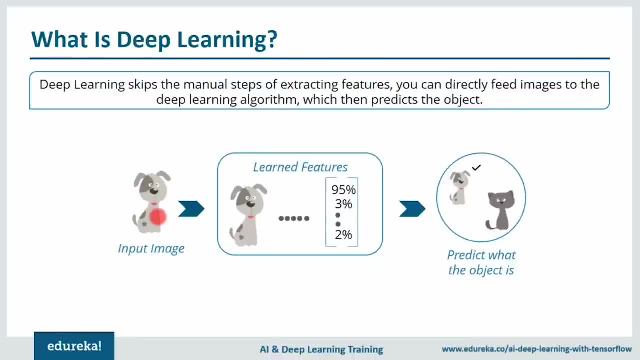 So what we do? we directly take the input image and feed it to our deep learning algorithm And because of that, what happens? whatever features are we already manually provided. apart from that, there might be many other features which are important. For example, if our features don't include: 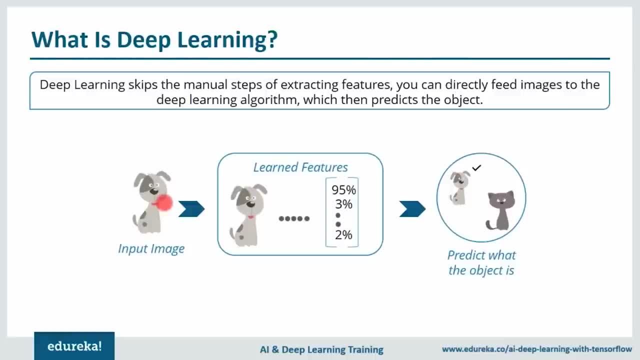 the length of the neck- and that is one of the major feature- in order to identify or classify whether it is a cat or a dog. Now what will happen? our algorithm will automatically determine that feature and will take into consideration, and then it will classify whether the input image. 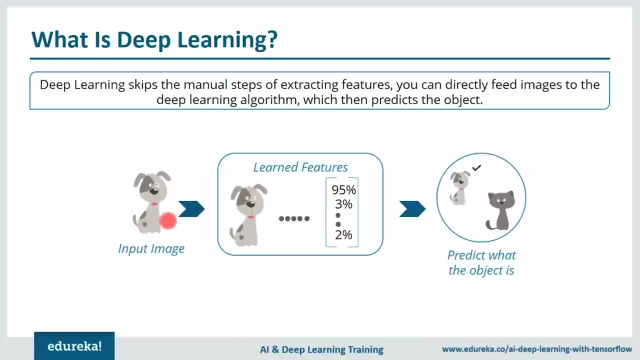 is a cat or a dog. So what happens here? we provide an input image of a dog and then it will automatically learn certain features, even if we don't provide it with those features, And after that it will give us the probability and according to this, 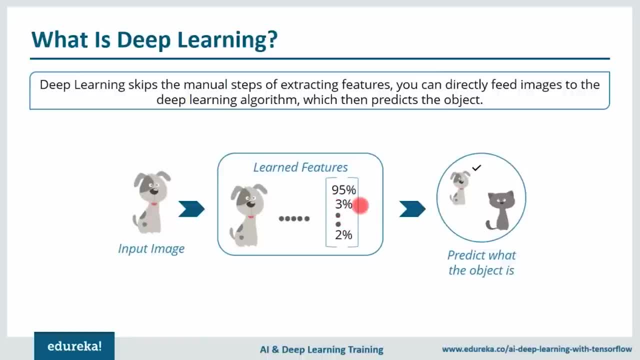 this particular scenario. it says 95% chances of being a dog, 3% chances of some other animal, similarly, 2% chances of some other animal. So since the highest probability goes with the dog, so the prediction says that the object or the input image 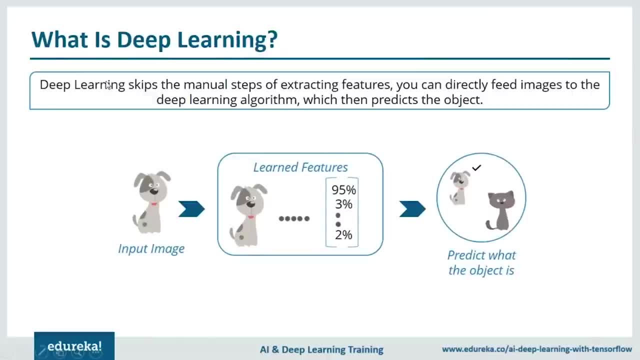 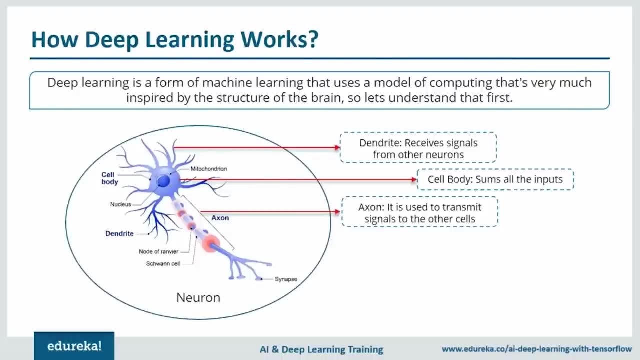 is nothing but a dog, Fine guys. so we'll move forward and we'll understand how exactly deep learning works. So the motivation behind deep learning is nothing but the human brain, As we have seen in the previous analogy as well what we are trying to do. 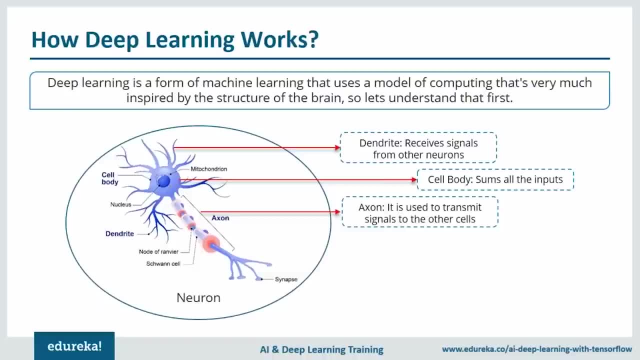 we are trying to mimic the human brain. We are trying to mimic the way we think, the way we take decisions, the way we solve problems. We are trying to make sure that we have a system that can mimic our own brain. So, obviously, the motivation for deep learning. 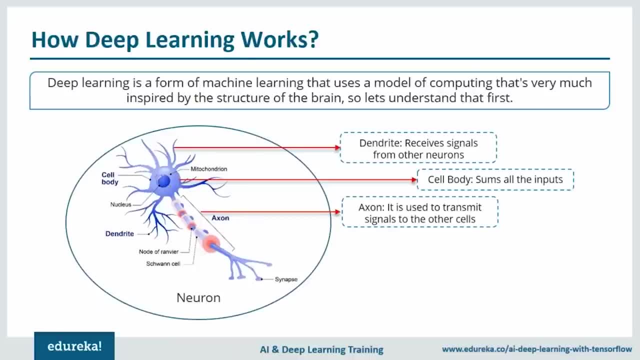 has to be our brain, And how our brain works with the help of our brain cells, which we call neuron. Now let us understand how a neuron works And let me tell you, guys, this is what we think, how a neuron works, This is what our studies tell us. 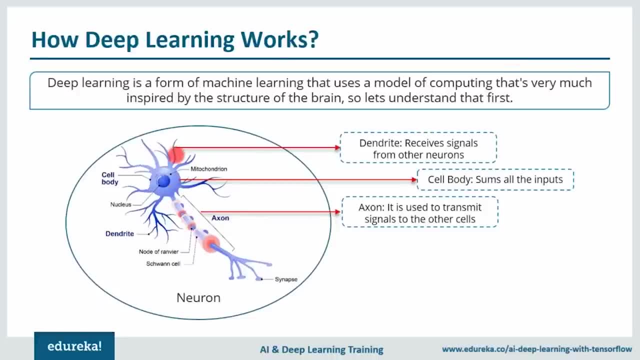 So yeah, so these are called dendrites. So dendrites receive signals from other neurons and then it passes those signals to the cell body. Now this cell body is where we it performs certain function. It can be a sigma function. That's what we believe. 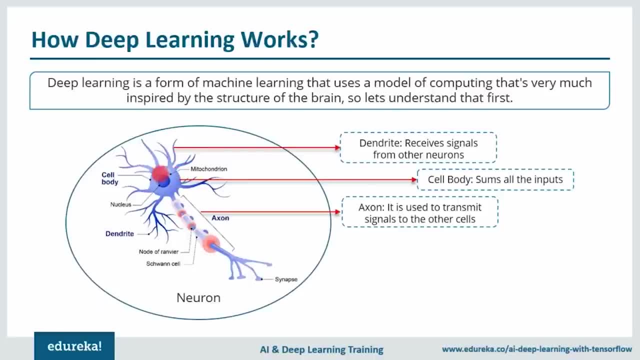 We believe it performs a sigma function that is nothing but sums all the inputs. Then, through exon, what happens? These signals are fired to the next neuron, And the next neuron is present at some distance, and that distance is nothing but synapse. So it fires only when the signals coming from the cell body. 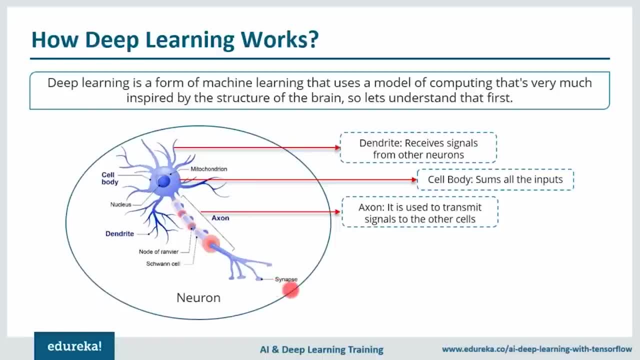 exceeds a particular limit, Then only the cell or this neuron will fire the signals to the next neuron. And this is how the neuron or the brain cell works, and we take the same process forward and we try to create artificial neurons. So let us understand why we need artificial neurons. 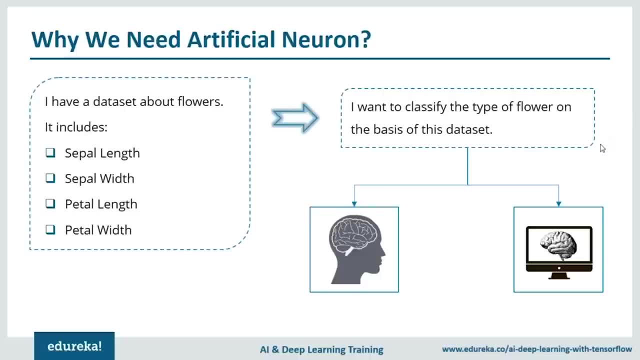 with an example. So I have a data set of flowers, say, and that data set includes sepal length, sepal width, petal length and petal width. Now what I wanna do? I wanna classify the type of flower on the basis of this data set. 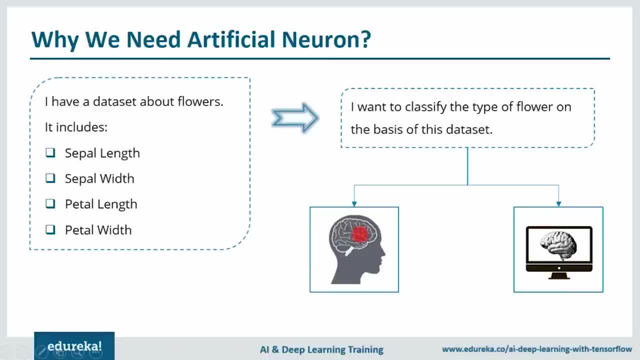 Now there are two options. Either I can do it manually- I can look at the flower manually and determine by its color or any means- and I can identify what sort of a flower it is- Or I can train a machine to do that. Now let me tell you the problem. 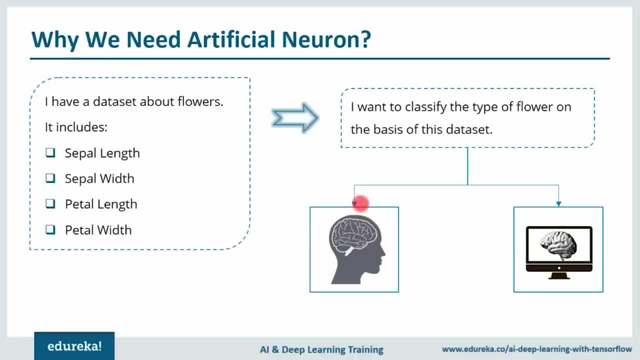 with doing this process manually. First of all, there might be millions of inputs that will be given to you, And for a human brain to perform that particular task is next to impossible. And at the same time, we always get tired at some point of time, right? 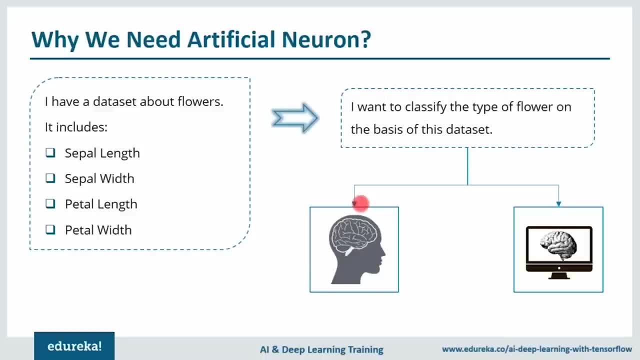 So we cannot just continue working for a long period of time in single stretch. And the third point is human error risk, which is always there. So these are a few limitations with the human brain. So what we can do, we can train a machine to do that task for us. 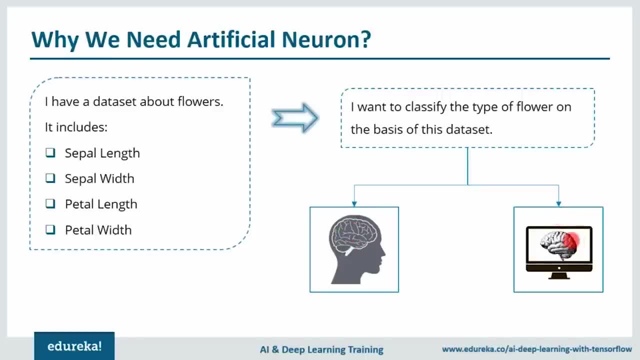 or we can put our brain inside a machine so that it can classify the flowers for us. So with this, what'll happen? the machine will never get tired and it'll make better predictions as well. So this is why we create artificial neurons, so that there's a system present that can mimic our brain. 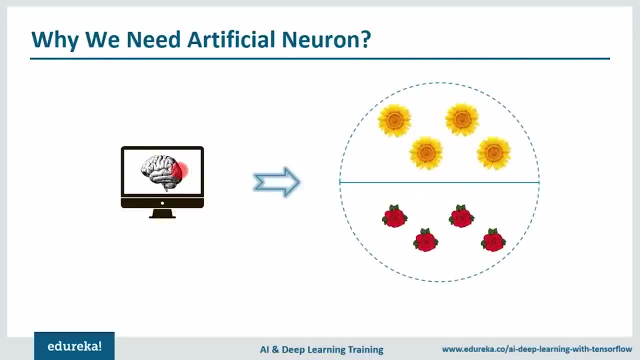 And this is how this is what exactly happens. So this particular artificial neuron can actually classify the flowers, or you can say, can divide the flowers on the basis of certain features. In our case, we have sepal length, sepal width. 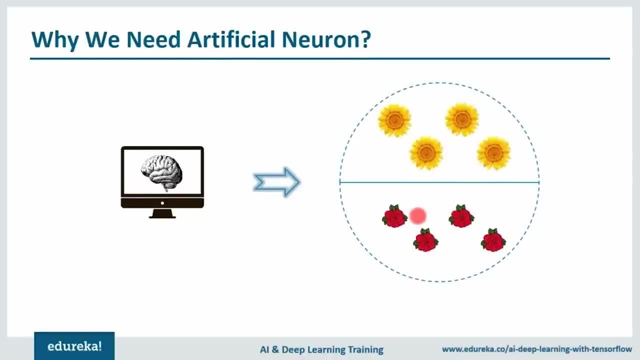 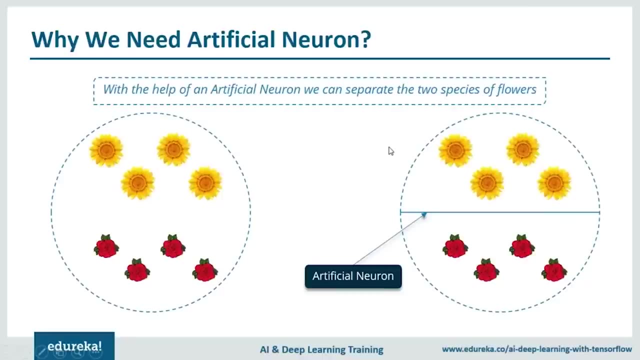 petal length and petal width. So on that basis it can classify the two flowers. So what we need here? we need some sort of a system that can actually separate the two species. And what is that system is nothing but an artificial neuron. 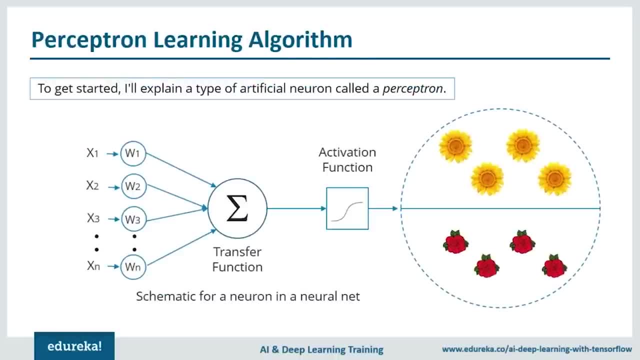 So we need artificial neuron, and one type of artificial neuron is a perceptron. Now let me explain you perceptron with a flow diagram that is there in front of your screen. Now, over here, what happens? we have set of inputs like X1, X2, dash, dash, dash till XM. 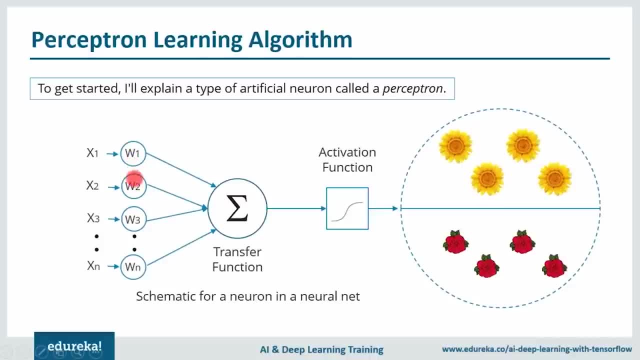 Now these inputs will be multiplied with their corresponding weights, which is W1, W2, W3 till WN in our case. Now these weights actually define how important our input is. So if the value of weight is high, we know that this particular input 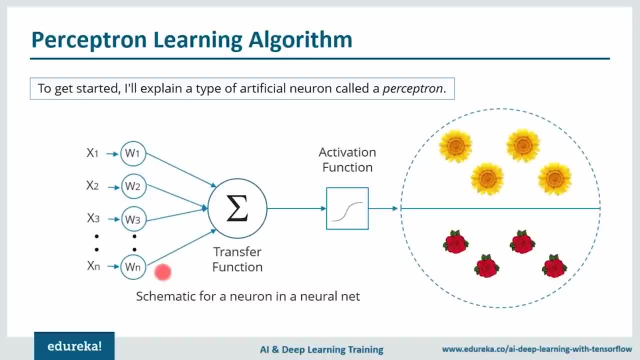 is very, very important for us. After multiplication, all of these are summed together and then it is fed to an activation function. Now the reason of using activation function is to provide a threshold value. So if our signal is above that threshold value, 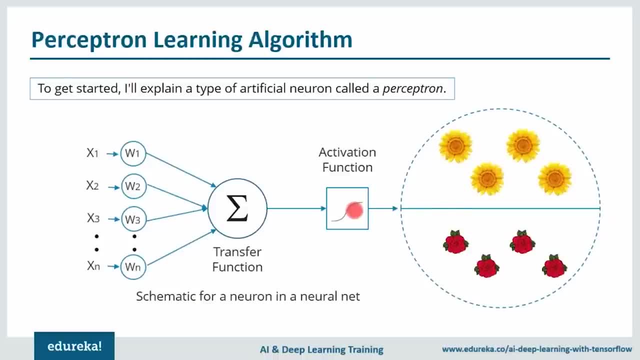 our neuron, or you can say our perceptron, will fire, Else it won't fire. So that is the reason why we use an activation function. There can be different types of activation function. There can be sigmoid, there can be step function, sine function, depending on our use case. 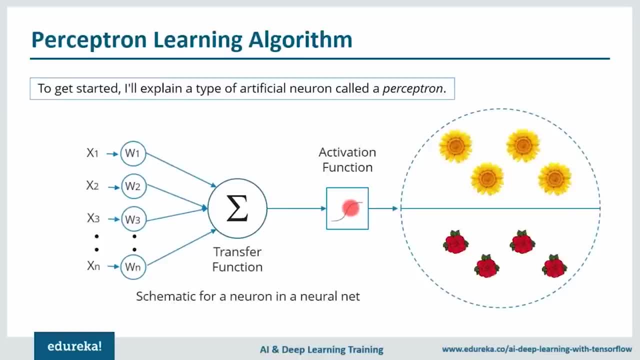 we define the activation function Now. the main idea was to define an algorithm in order to learn the values of the weights, which are W1,, W2, W3, in our case, to learn the values of the weights that are then multiplied with the input features. 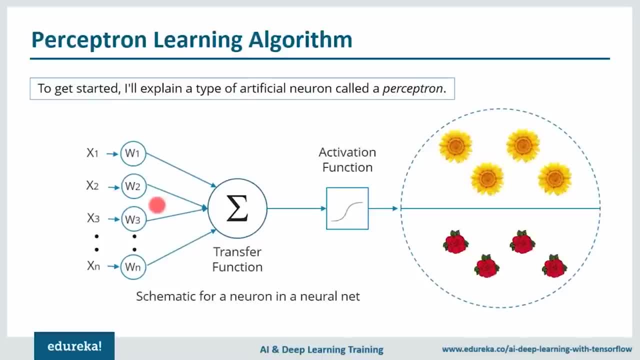 in order to make a decision whether a neuron fires or not, In context of pattern classification, which is, in our case, flowers. so we are trying to classify the two species of flowers. such an algorithm could be useful to determine if a sample belongs to one class or one type of a species. 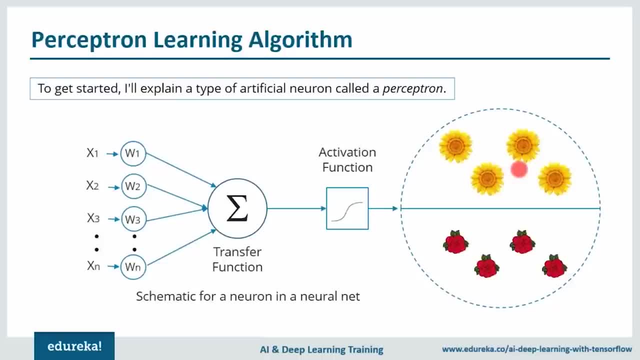 or another class or another type of the flower. We can even call perceptron as a single layer, binary linear classifier to be more specific, because it is able to classify inputs which are linearly separable, And our main task here is to predict to which of the two possible categories. 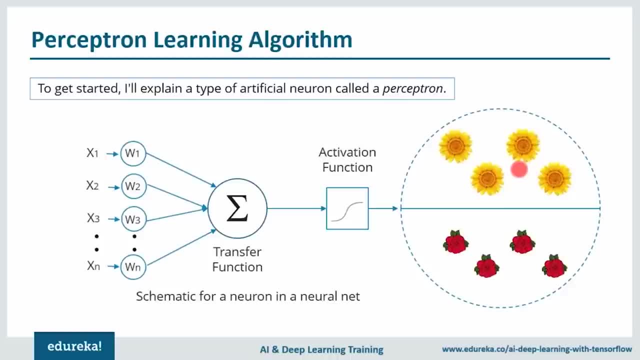 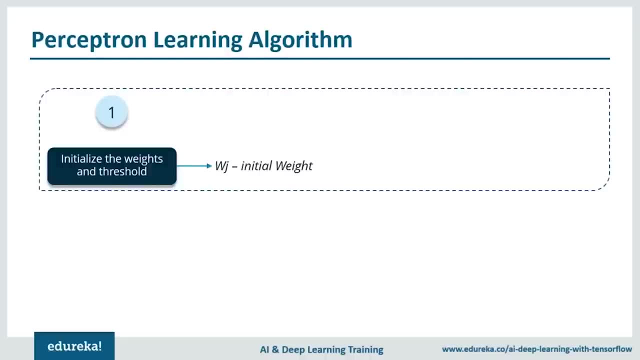 the data point belongs based on a set of input variables. Now there's an algorithm on which it works, so let me explain you that. So the first thing we do is we initialize the weights and the threshold. Now these weights can actually be a small number. 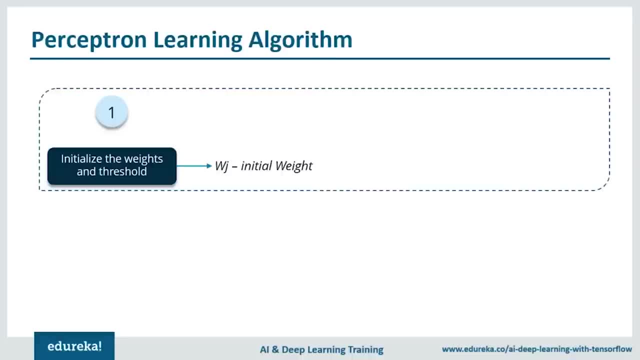 or a random number, and it can even be zero. So it depends on the use case that we have. Then what we do: we provide the input and then we calculate the output. Now, when we are training our model or we are training our artificial neuron, 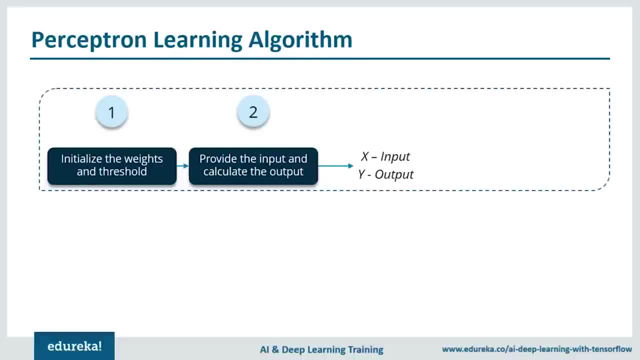 we have the output values for a particular set of inputs, So we know the output value. But what we do? we give the input and we see what will be the output of our particular neuron And accordingly we need to update the weights in order to reduce the loss. 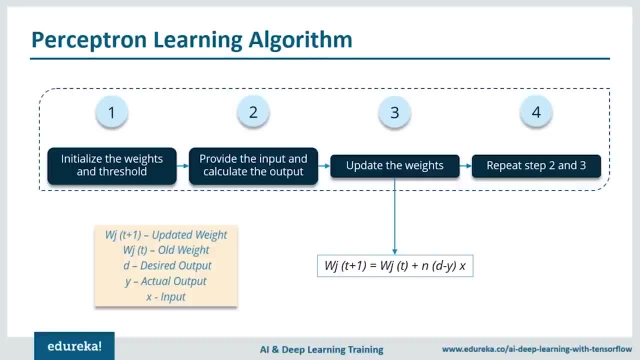 or you can say: in order to reduce the difference between the actual output and the desired output. So what happens? let me tell you that. So we need to update the weights. So how we are going to update the weights is we can say: the new weight is equal to the old weight. 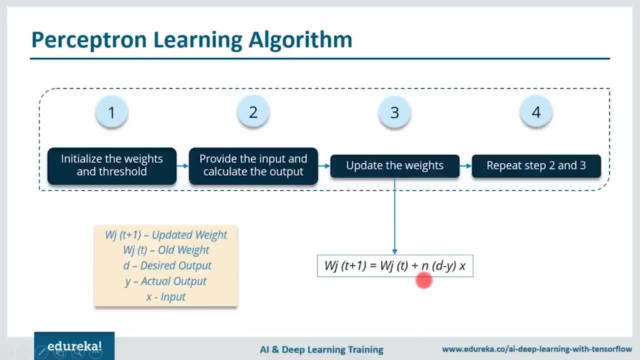 plus the learning rate. Learning rate: we'll discuss about it later in the session, But generally we choose learning rate somewhere between 0.5 to 0.01.. After that, what happens? we find the difference between the desired output and the actual output. 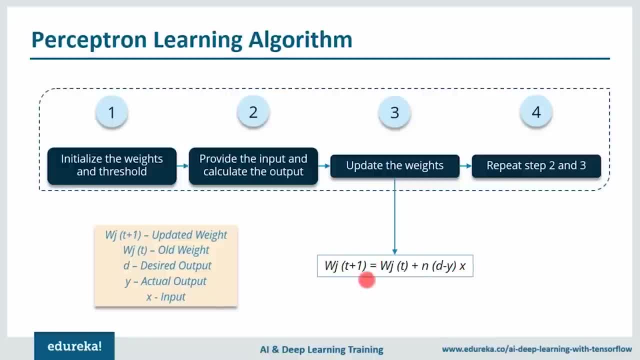 And then we multiply it with the input. So on that basis we get a new weight. So this is how we update the weights. And then what happens? we repeat the steps two and three. So we are going to repeat the steps two and three. 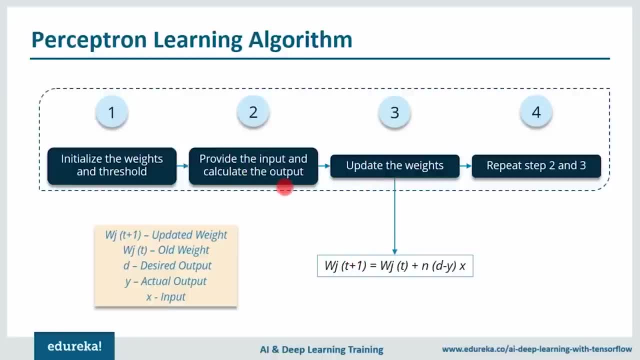 That is, we are going to apply this new weight Again, we are going to calculate the output Again, we are going to compare it with the desired output And if it matches, then it's fine. Otherwise, we are going to update it again. 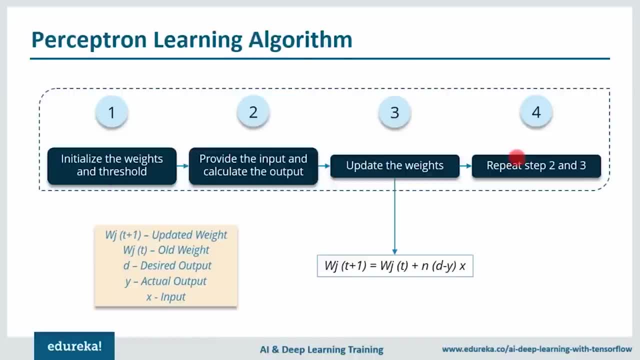 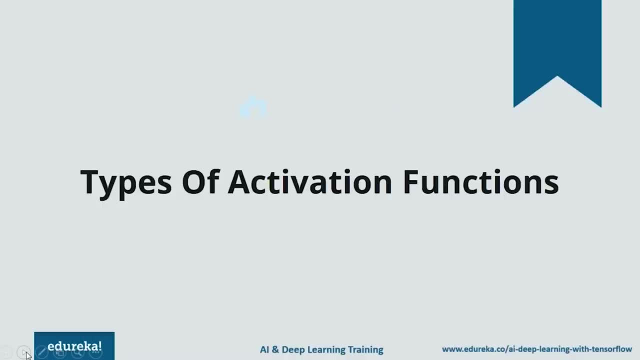 So this is how the whole perceptron learning algorithm works And don't worry, guys, I'm going to show it to you practically how it actually works in my PyCharm. Fine guys, so we'll move forward and we'll see the various types of activation functions. 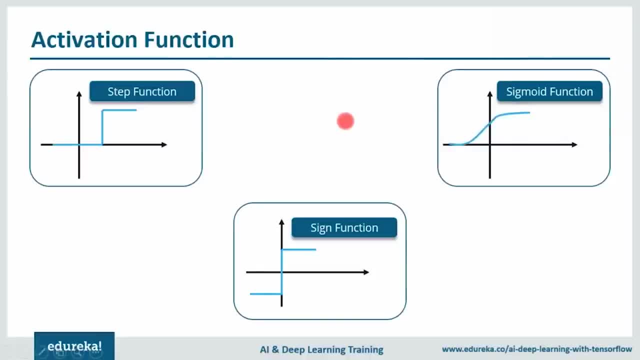 So these are the various types of activation functions that we use, although there can be many more activation functions. Again, I'm telling you, it depends on your use case. So we have a step function. So if our output is actually above this particular value, 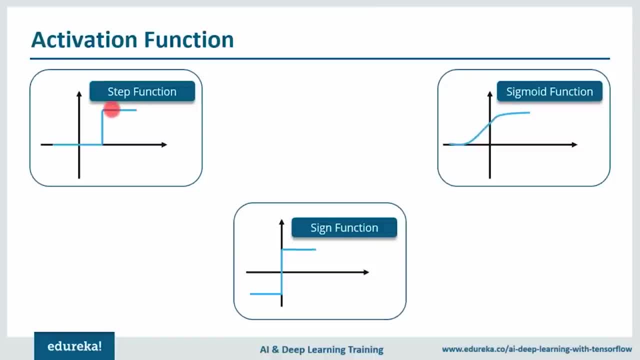 then only our neuron will fire, or you can say the output will be plus one, Or if it's less than this particular value, then we'll have no output, or we'll say zero output. Similarly for the sigmoid function as well, and same goes for sine function. 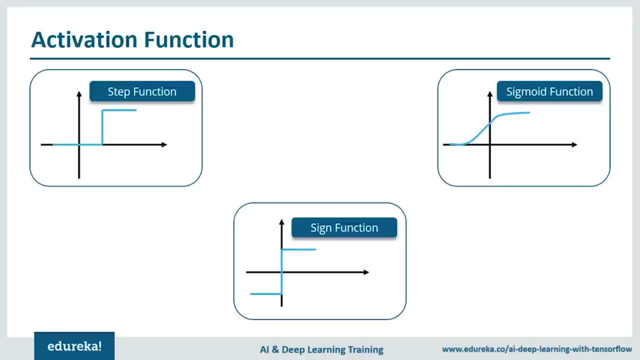 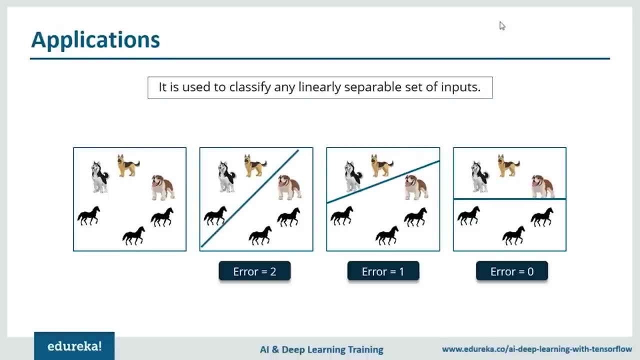 So let us move forward and we'll focus on various applications of this perceptron. Now, as I've told you earlier as well, it can be used to classify any linearly separable set of inputs. Now let me explain to you with the diagram. 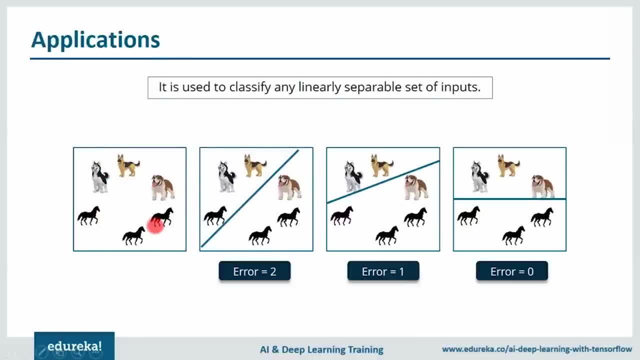 that is there in front of your screen. So we have different types of dogs and we have horses And we want a line that can separate these two. So our first iteration will produce this sort of a line, But here we can notice that we have error here. 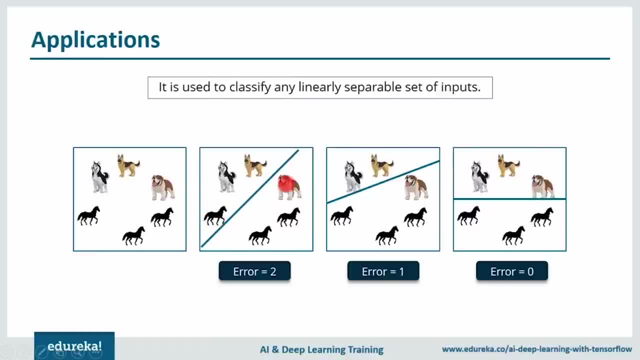 as we have classified horse- one of the horses- as a dog and a dog as a horse. So error is two here. Similarly. now, what happens? we have updated the weights. Now, after updating the weight, what happens? our error has reduced. 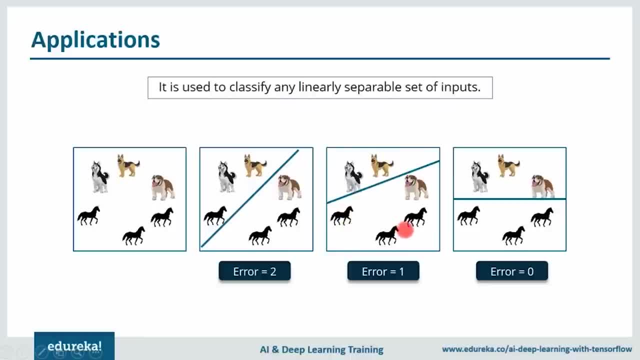 So what happens now? we have actually classified all the horses correctly, but one dog we have classified wrong and we have considered it as a horse, So our error becomes one Once again. what'll happen if you can remember the step two and three of our perceptron learning algorithm? 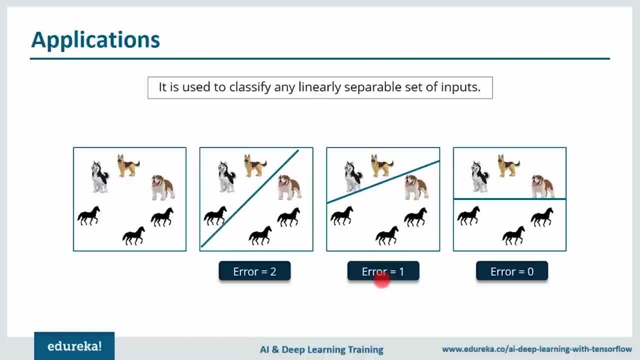 will be done, And then, after that, our weights will be updated and our desired output will become equal to our actual output, and we get a line something like this. So what we have now? we have properly classified dogs and horses, So this line separates both of them. 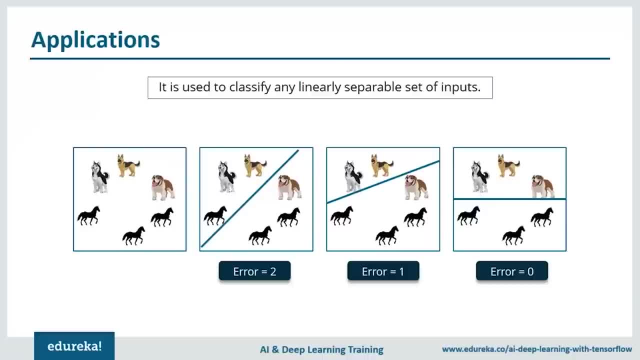 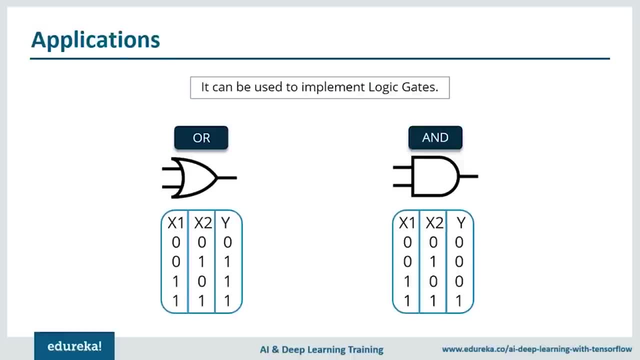 This is how we can actually use a single layer perceptron in order to classify any linearly separable set of inputs. Now we can even use it in order to implement a logic gates, That is, or, and, and. Now let me tell you how you can do that. 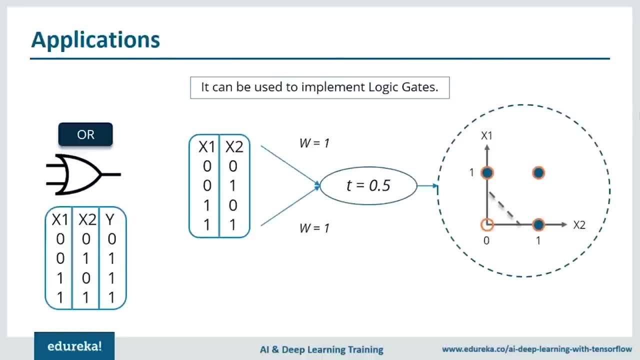 First we'll look at: or gate Now in, or gate what happens. here is the truth table. According to that, we have two inputs, X1 and X2.. So if both are zero, we get a zero. If any one of the input is high, or any one of the input is one, 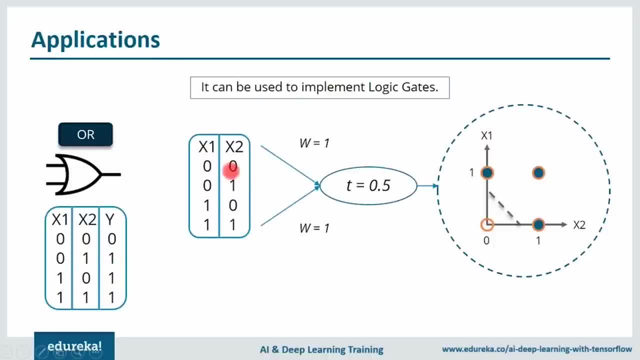 we get the output as one. So what we need to do is we need to make sure that our weights are present in such a way that we get the same output. So how we have done that when the value of weight is equal to one, and then we provide the input X1 and X2. 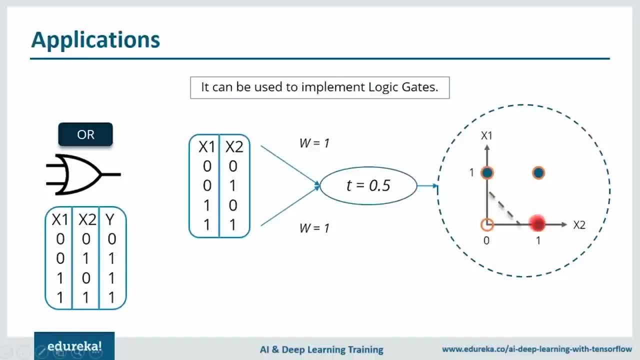 after passing through this activation function, we get this sort of a graph, which is the graph for our or gate. Now, if you want, I could use a pen and I can explain it to you. Now we have X1 and X2 as inputs. 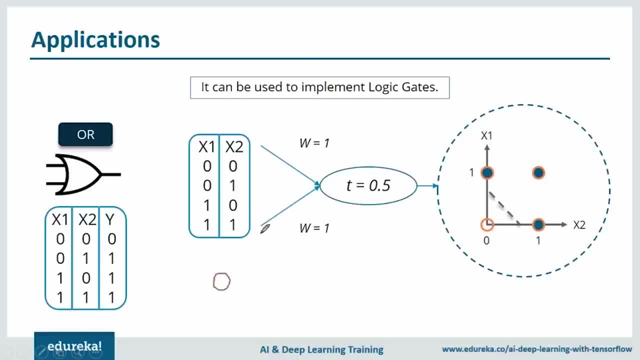 So we provide first input as zero X1, and this also as zero. So zero into zero is again zero, zero into zero is zero, And then we pass this through this activation function. Now we need to make sure that whatever value that comes here, 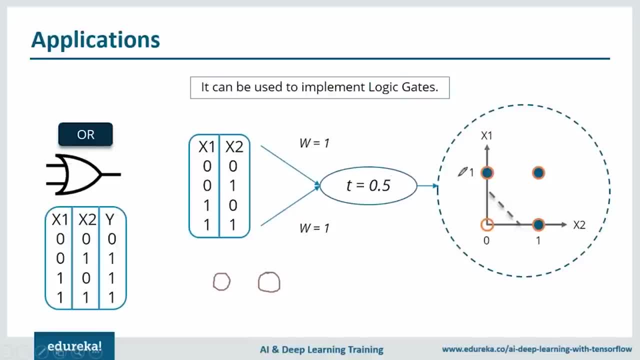 should be greater than 0.5, then only our neuron or the perceptron will fire, But since this value is actually less than 0.5, so the neuron won't fire and our output will be zero, as you can see it over here, 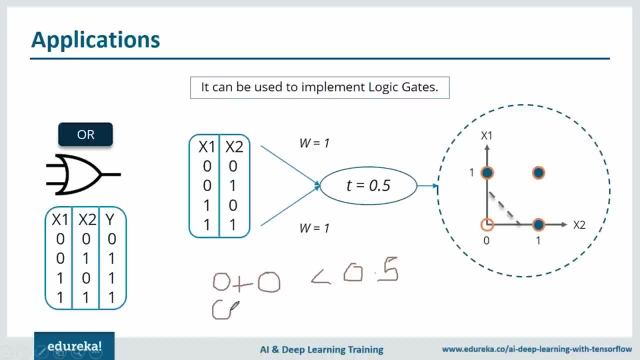 Now let's take the other set of inputs. Now our X1 is zero and our X2 is one. So one into one will be obviously one. Now in this case, our output is bigger than 0.5. Then what will happen? our neuron will fire. 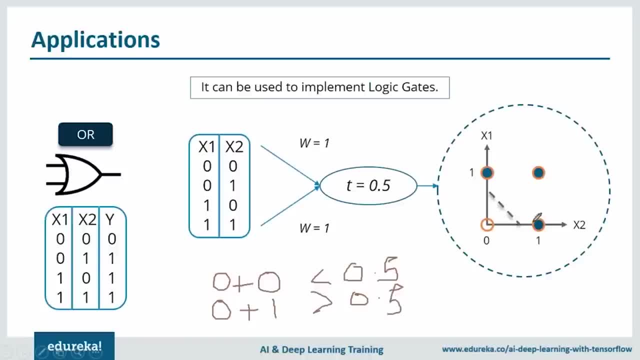 and we'll get one, the output one here, as you can see it in the graph. Similarly, when my X1 is one and X2 is zero, in that case also, our output will be 0.5.. Our output is greater than 0.5,. 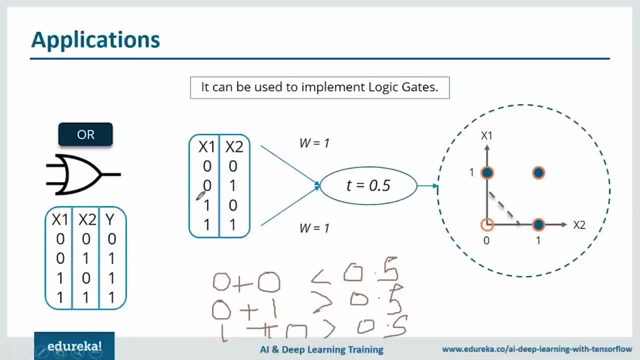 our neuron will fire and we'll get this sort of a graph. When I talk about one, one- then our output will be two, which is greater than 0.5, so we get an output that is one, And this is how we get the graph. 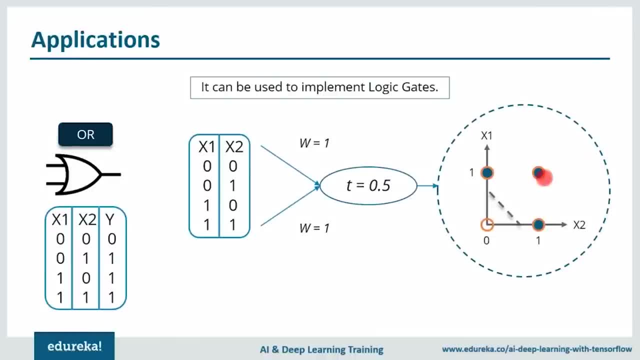 So this is how we get this graph. And now, if you notice, with the help of the single-layer perceptron, we are able to classify the ones and zeros. So this line, anything above this line, is actually one, and anything below this line, we have zeros. 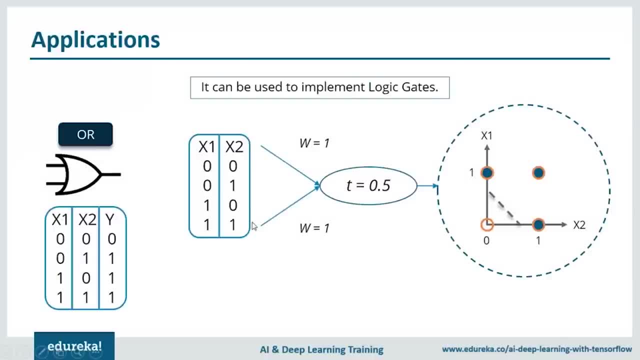 So this is how we are able to classify or able to implement OR gate Similarly when I talk about AND gate as well. so there's a difference in the truth. table of AND gate In AND gate. what happens? we need to make sure. 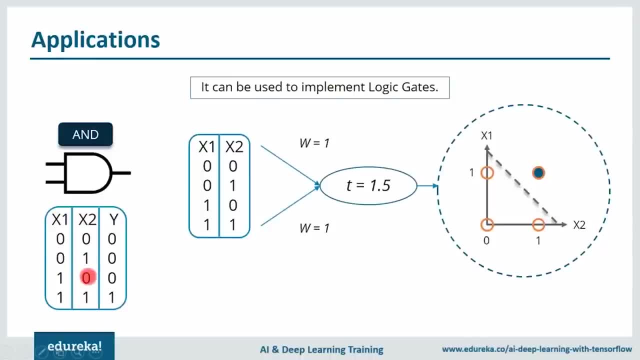 that both of our inputs are high in order to get a high output. If any of the input is low, we get a low output, And that's the reason we choose an activation function that is 1.5,, which means that if our value 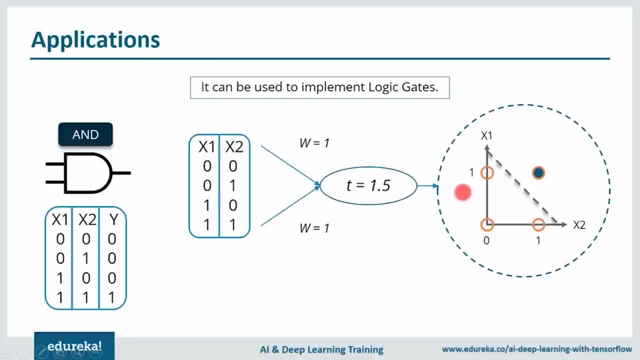 or the output is above 1.5, then only our neuron will fire and we'll get one here. And there's only one case, that is when both the inputs are high. So when both the inputs are high, I'll use my pen again and I'll explain to you. 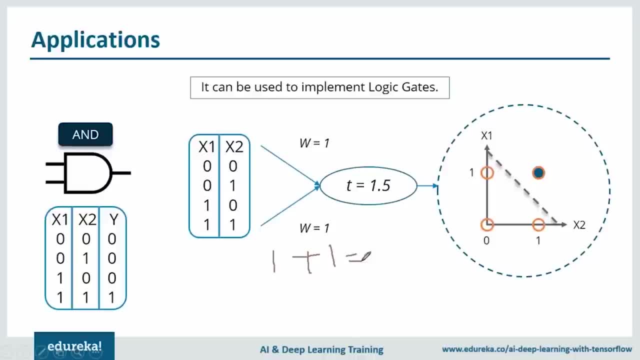 So X1 is one, X2 is one, we get something which is two, which is obviously greater than 0.5,. pardon me for my writing, but yeah, this is how it is. So one plus one, two, which is obviously greater than 0.5,. 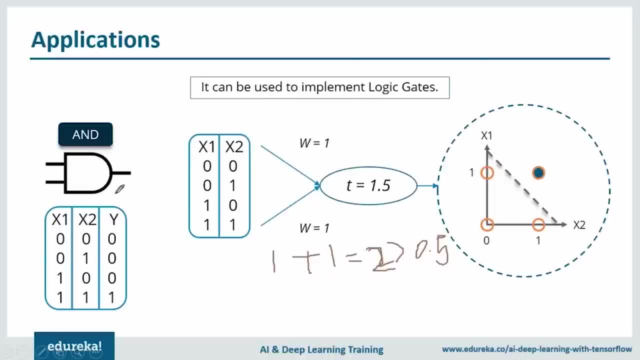 so what? we get, our neuron fires and we get one here, But for the rest of the inputs all will be less than 1.5.. So that is why our neuron doesn't fire and we get a zero output. Don't worry guys, I'll actually tell you how to implement it. 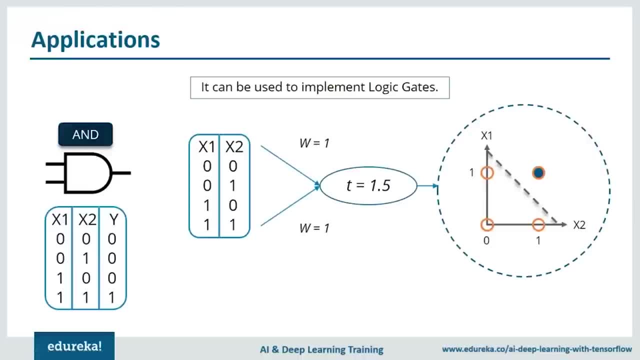 I'll open my PyCharm and I'll be showing it to you practically how to implement these gates. So for that, what I'm going to do is I'm going to first import a Python library called TensorFlow, The installation guide of this particular library. 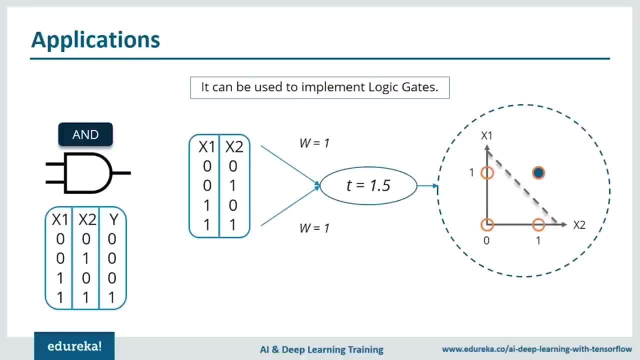 is present in an LMS for both Windows as well as for Linux, So you can just go through it and it's very easy to install that, And I'll actually execute this practically later in the session. you don't need to worry about it. 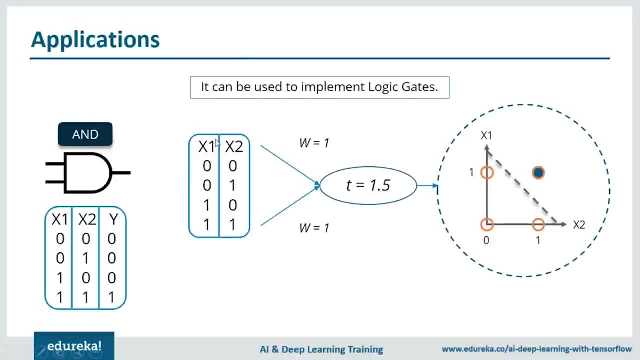 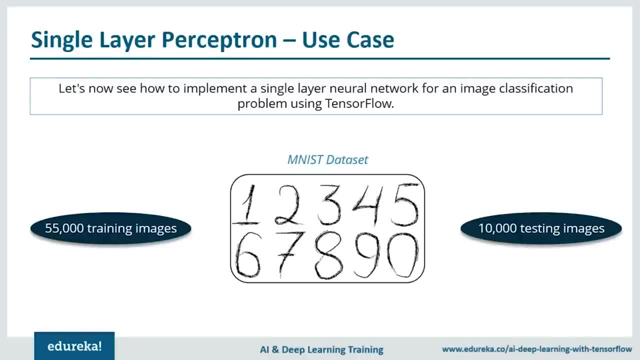 So this is how we can implement AND and OR gate. So let's move forward, guys, and we'll actually understand the use case. so let's go back to our MNIST data set. The reason for using MNIST data set is because it is already clean. 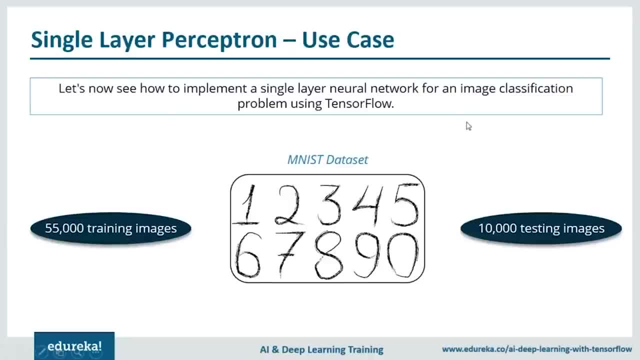 and will be a perfect example for this. Now, what this MNIST data set contains. it basically contains handwritten digits from zero to nine, And in that data set we have 50,000 training images, along with 10,000 testing images. 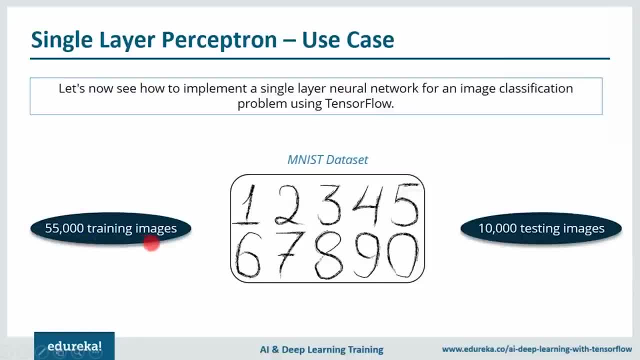 So we will train our model with those 55,000 training images, and then we are going to test the accuracy of a model with the help of those 10,000 testing images. And for all of this we need to understand first what exactly is TensorFlow? 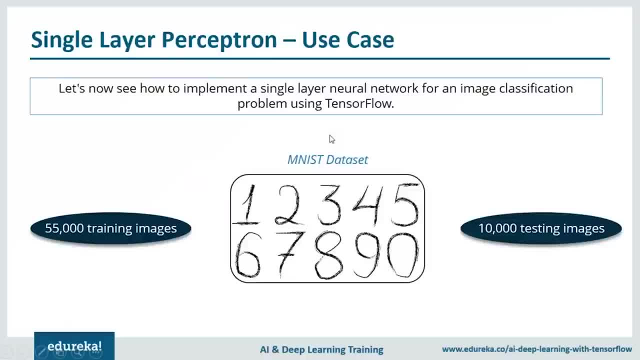 So let us move forward, guys, and we'll understand TensorFlow, and then we are going to implement all these things that we have discussed, that is, AND gate OR gate, and the MNIST data set that I'm talking about. So let's move forward, guys. 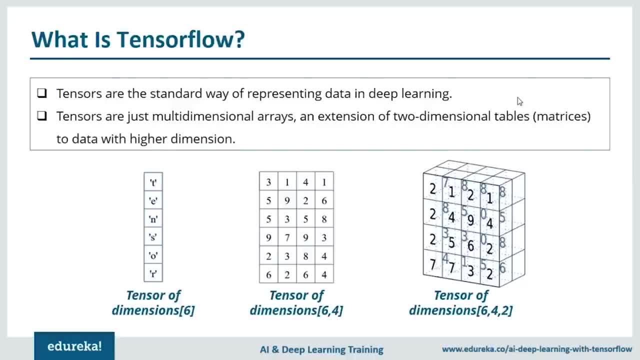 and understand what exactly is TensorFlow. Now, what is TensorFlow? As I've told you earlier as well, we use this TensorFlow library in order to implement deep learning models, And the way the data is represented in the deep learning model is called tensors. Now, what are tensors? 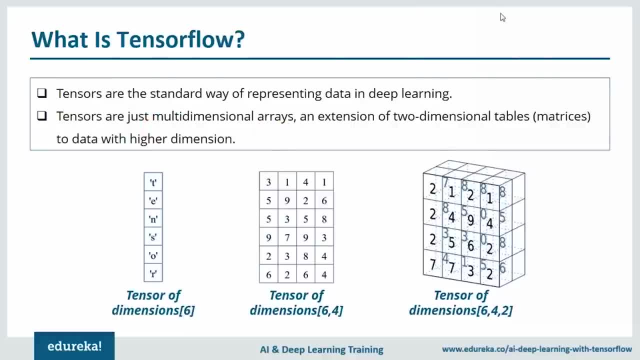 Now, tensors are just the multi-dimensional arrays, or you can say an extension of two-dimensional tables, matrices, to data with high dimension. Now let me explain to you with the examples that are there in front of your screen. So this particular data is nothing but a tensor. 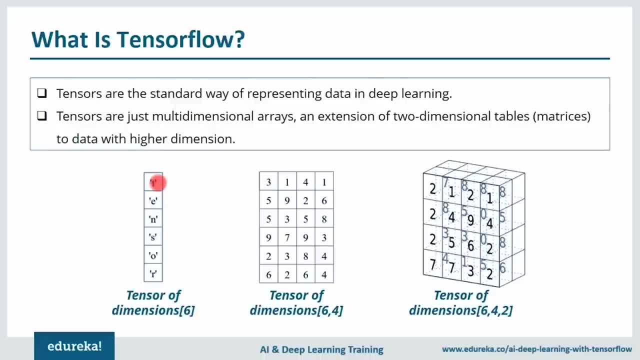 of dimension six, because we have six rows and we have only one single column. Now over here we have four columns as well as six rows, so this becomes a tensor of dimension six comma four, Similarly over here as well. so we have another dimension, that is the third dimension. 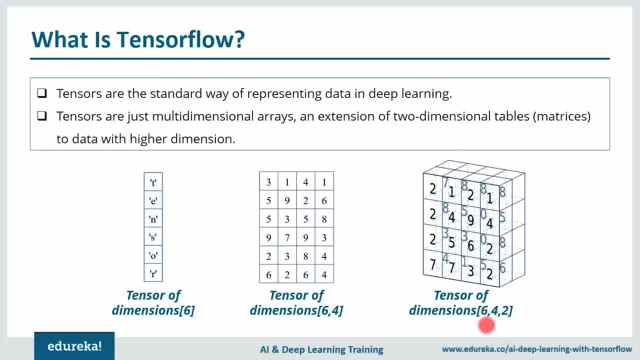 in which we have two values. so we consider this as a tensor of dimension six, four and two. So this is nothing but a way of representing data in TensorFlow. Now, if you consider the TensorFlow library at its core, it is nothing but a library. 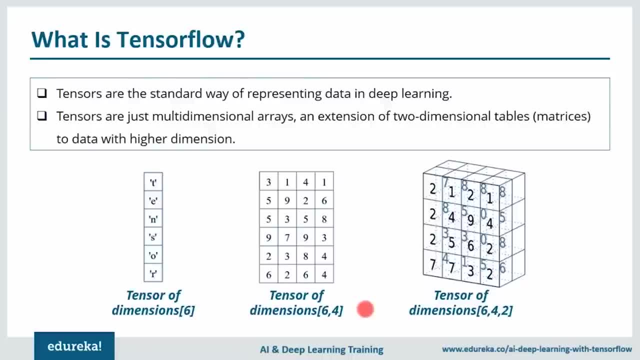 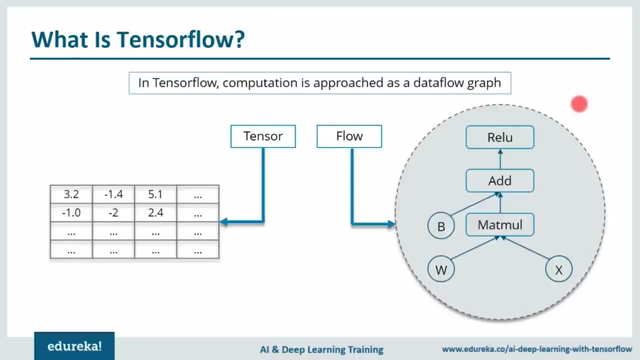 that performs matrix manipulation. That is what TensorFlow is. Now let us move forward and understand TensorFlow in a bit detail. So, as the name tells that, it consists of two words, tensor as well as flow, Now we understood what exactly tensor is. We saw it in the previous slide. 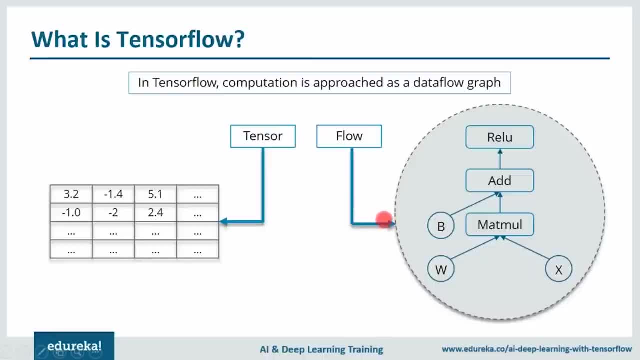 Now, when I talk about flow, it is nothing but a data flow graph. So let me just give you an example that is there in front of your screen. So we talked about weights and inputs. So we provide these weights and inputs and we perform a matrix multiplication. 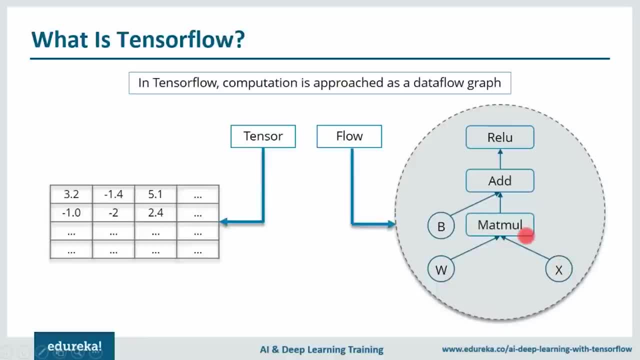 So the weight is one tensor, x input is one tensor. then we perform matrix multiplication. After that we add a bias, which we'll actually see it later in the session. You don't need to worry about this term. Then what we do? we add all of these. 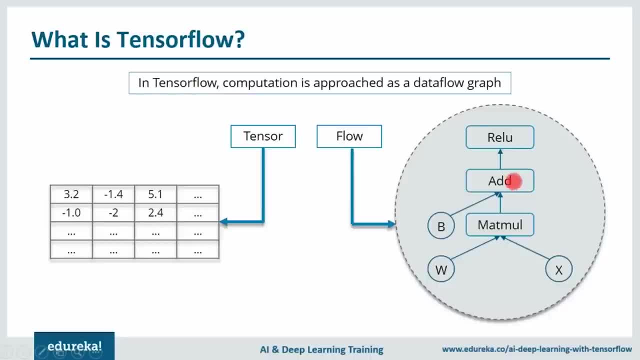 So what is this? This is nothing but the sigma function in this perceptron that we have seen. Then we pass it through an activation function and the name of that activation function is R-E-L-U or ReLU, or you can say it. 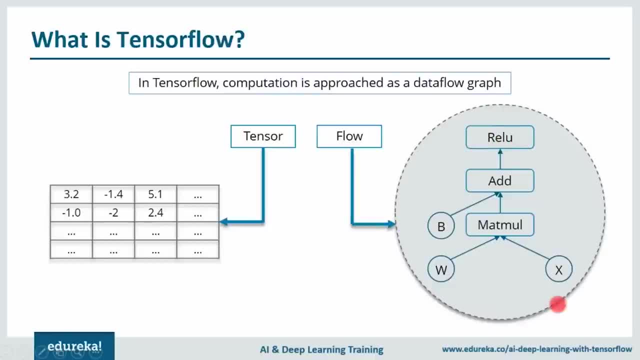 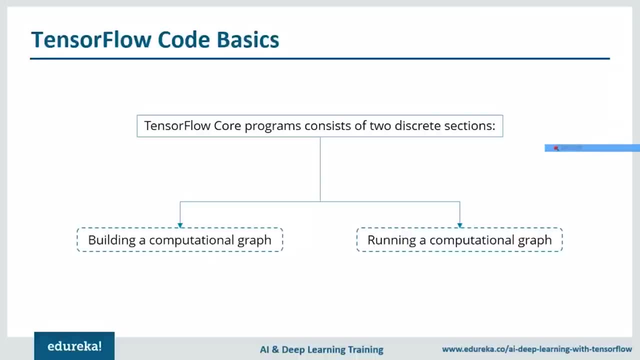 and then our neuron will fire. So this is nothing but a flow, or you can say a data flow graph. Now let us understand few code basics of TensorFlow. Now the TensorFlow programs actually consist of two parts. One is building a computational graph. 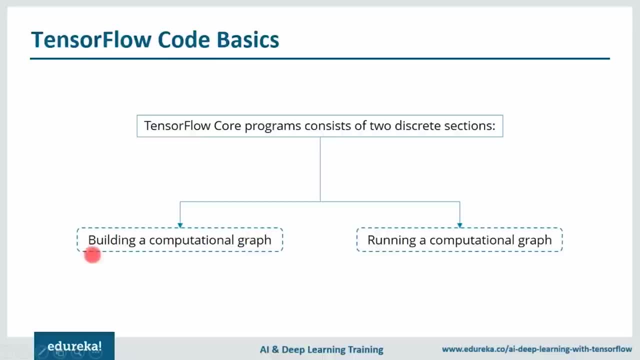 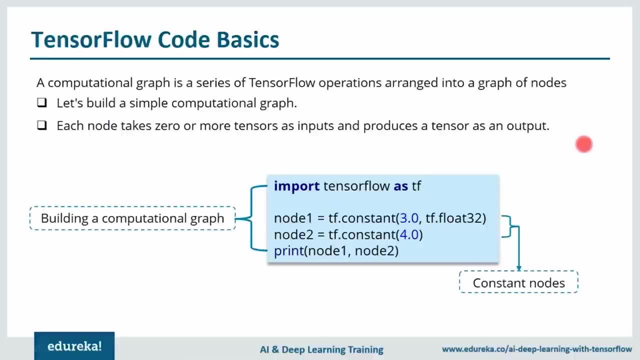 and another is running a computational graph. So we'll first understand how to build a computational graph. Now you can think of a computational graph as a network of nodes and with each node known as an operation and running some function. that can be as simple. 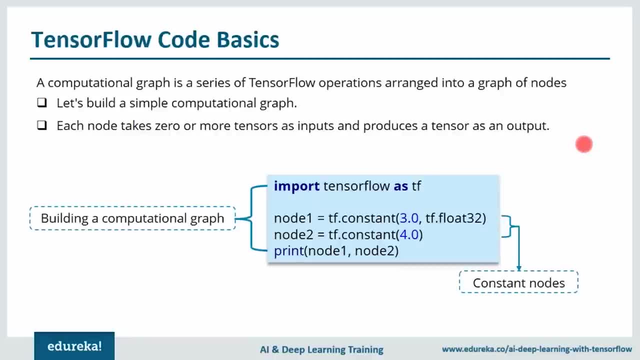 as addition or subtraction, or it can be as complex as, say, some multivariate equation. Now let me explain it to you with the code that is there in front of your screen. So the first thing you do, you import the TensorFlow library. Then what you do, you define two nodes. 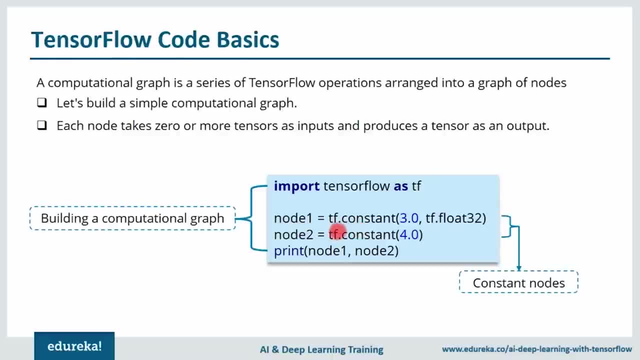 and these nodes are constants. So we'll call that function, we'll call it as tfconstant and we'll provide a value that is three, nothing but a float number of 32 bits. Similarly, we define one more node, which is a constant. 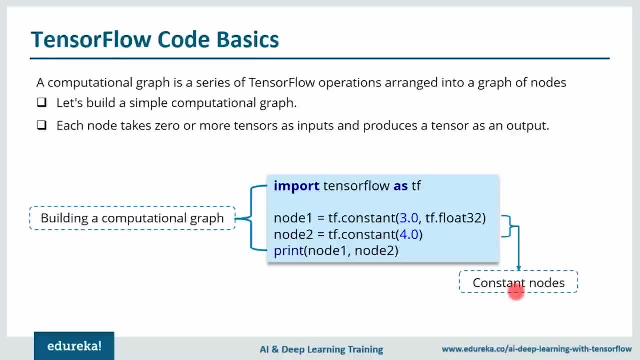 and it contains value four. So these are nothing but your constant nodes. This is basically what computational graph is. So, basically, we have built a computational graph and in this graph, each node takes zero or more tensors as inputs and produces a tensor as an output. 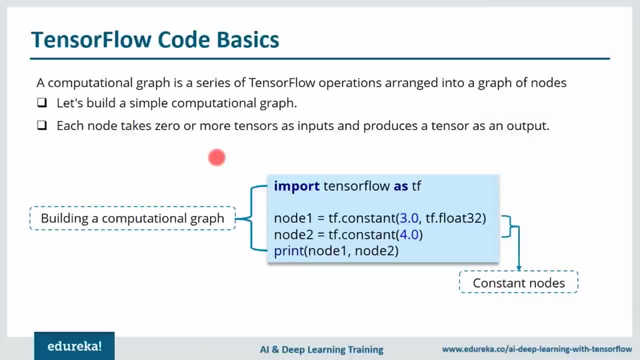 And one type of node is a constant that I've told you earlier as well, And these TensorFlow constants. it takes no inputs and it outputs a value which is stored internally. Now what I'll do? I'll actually execute this in my PyCharm. 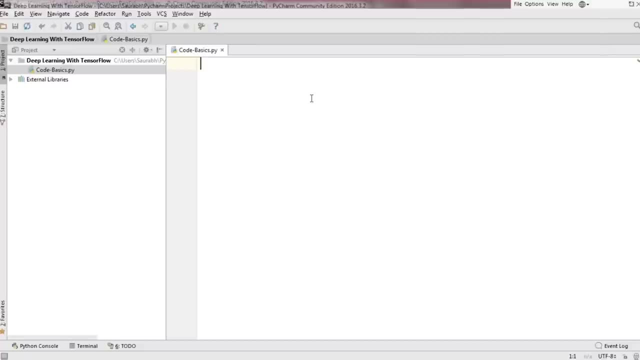 So for that I'll open it. So this is my PyCharm, guys, and I've already installed TensorFlow. So the first thing that I need to do is import the TensorFlow library. For that I'm gonna type in here: 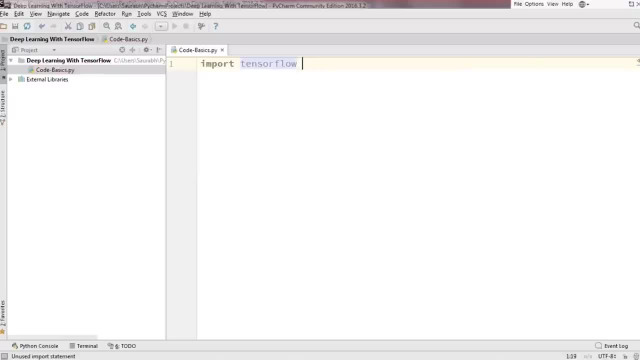 import TensorFlow as tf. So if you're familiar with the Python basics, you know what it means actually. So I'm importing TensorFlow library and in order to call that, I'm going to use the word tf. So after that, I'm going to do: 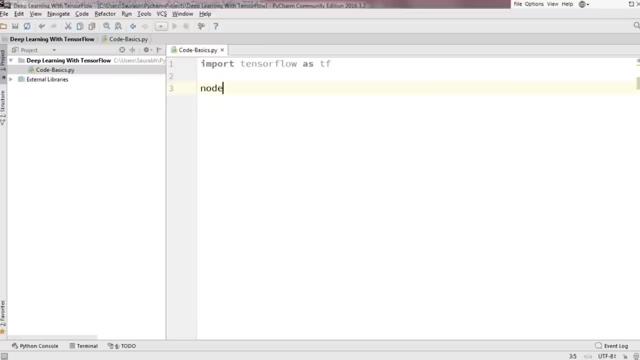 I'm gonna define my node one and node two, which are constant nodes. So for that I'm gonna type in here node one equal to tfconstant, And then I'm going to define the constant value in this. So it'll be three. 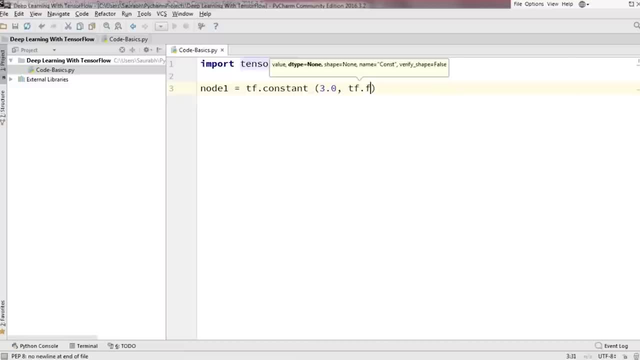 and it'll be a float value of tffloat of 32 bit. All right, And now I'm gonna define my second constant node. So I'll type in here node two: tffloat, tfconstant. I'll put four in here. 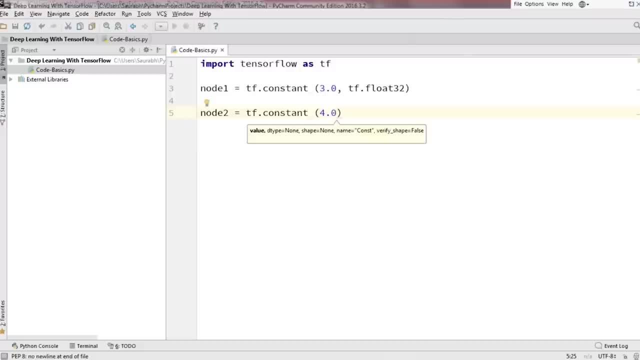 and four. that's it, And so the tffloat 32 will be present implicitly. I don't need to do that again and again. So I have created a computational graph here. So what if I print it now? So let us see what will be the output. 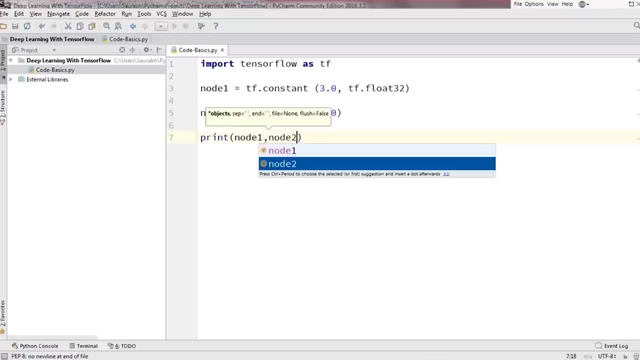 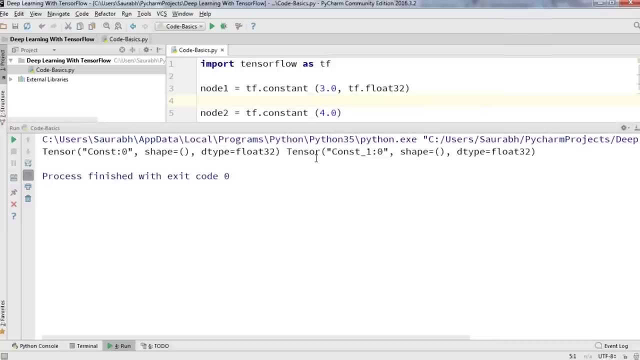 Node one. node two: Let's go ahead and run this and see what happens. If you notice here that printing the nodes does not output three and four, You might be expecting that right, That it should print three and four. But instead they are nodes that, when evaluated, 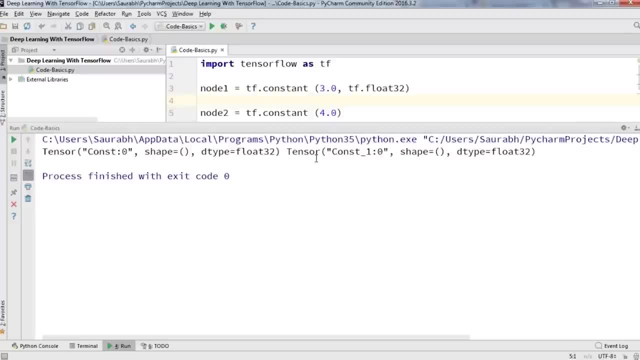 would produce three and four respectively. So to actually evaluate the nodes, what we need to do is we need to run this computational graph. So let me show you that. For that I'm again going to open the slides. So, since I've told you earlier as well, 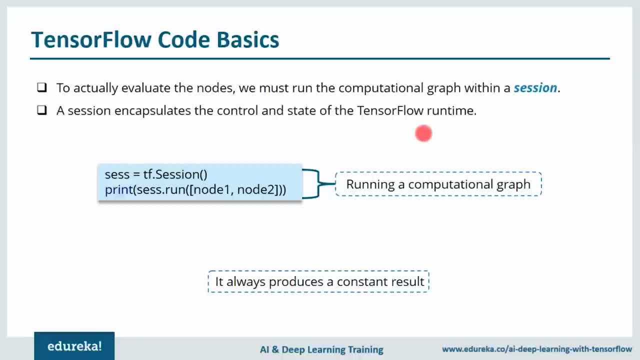 we need to actually run this computational graph within a session. And what is this session? A session actually encapsulates the control and state of the TensorFlow. run Now the code that is there in front of your screen. what it will do: it will actually create a session object. 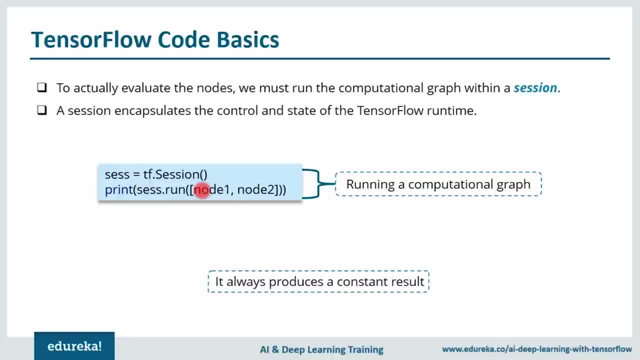 and then it invokes its run method to run enough of the computational graph in order to evaluate node one and node two. And how it does that? By running the computational graph in a session. So now let me show it to you practically how it happens. 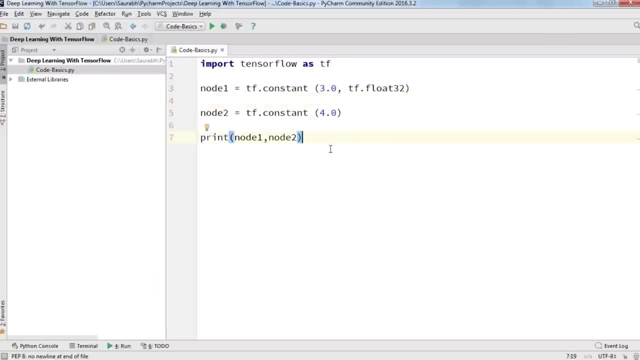 So again I'm going to open my PyCharm. This is my PyCharm guys. So let me first comment this print statement, and now I'm going to run a session, So for that I'm going to type in here: ses equal to tfsession. 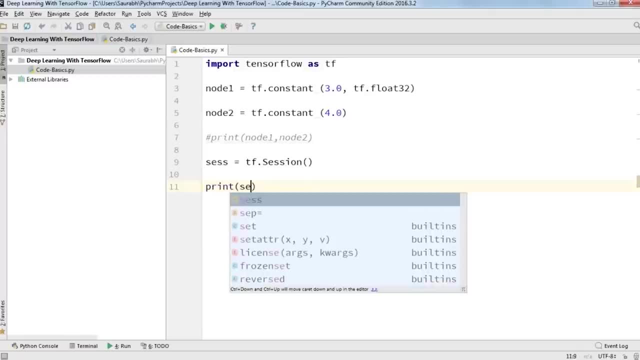 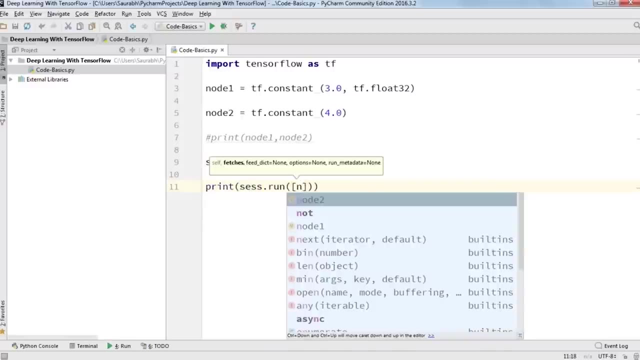 and now I'm going to print it. So for that I'm going to type in print sesrun and what I want to run. I want to run node one and node two, So I'm going to type in here: node one, comma, node two. 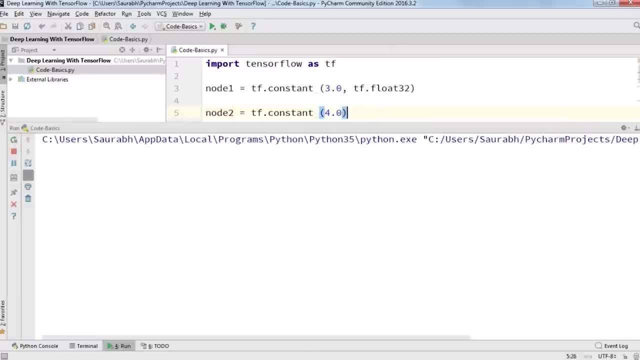 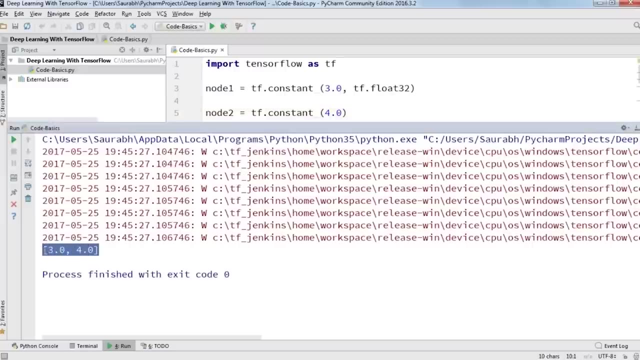 That's all. And now, when I run this, it'll actually give me the value three and four. And yup, it does, It gives me the value three and four. So what we did? we first built a computational graph. We first saw how to build, basically, a computational graph. 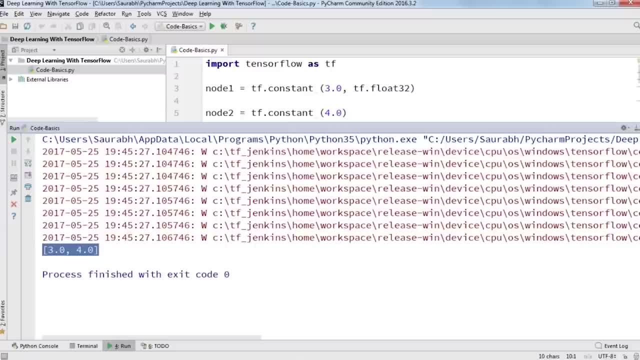 And then we understood that these all are nodes. So in order to get their value, we need to evaluate those nodes. and how we can do that? by running the computational graph inside a session And then, finally, when we run that session, we get the output three and four. 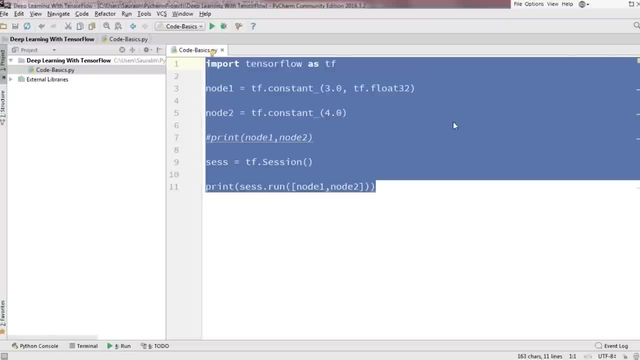 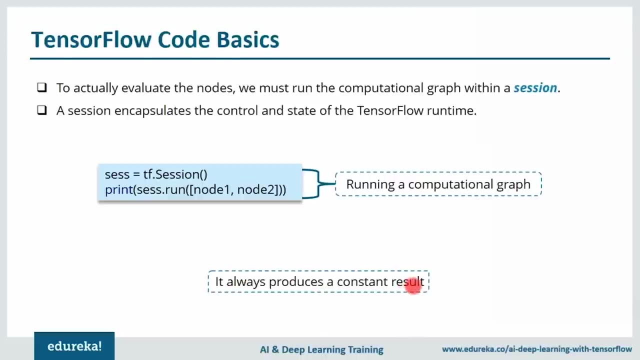 which is nothing but the values of those nodes. Fine, so I'll again open my slides, And the one thing that you must have noticed here is that it will always produce a constant result, right? So how to actually do that, So how to actually avoid that? 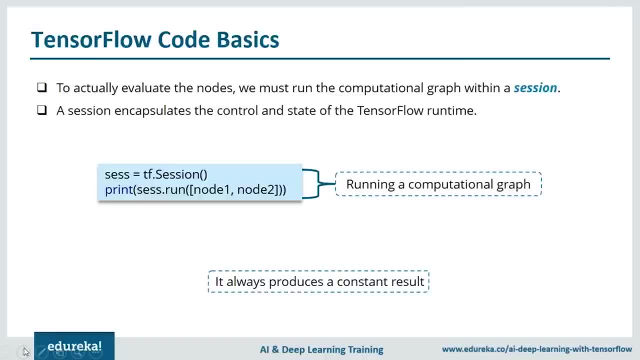 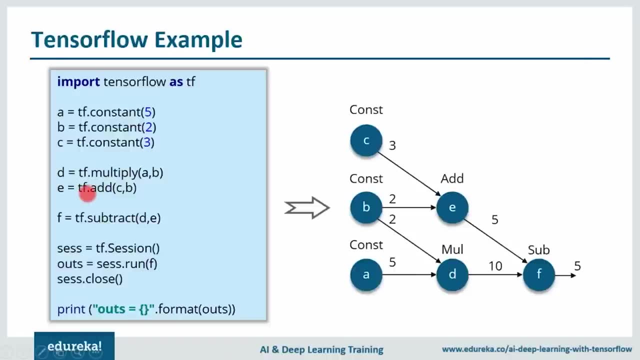 So we saw how to run a computational graph as well. Now let me explain it to you with one more example. So this is one example in which we take three constant nodes- A, B and C- and we perform certain operations like multiplication, addition and subtraction. 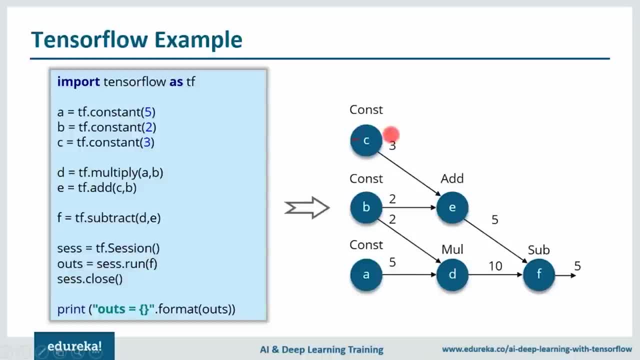 And then we run the session and then we finally close it. And this is the diagram how it looks like. So we have three constant nodes: C, B, A. A contains value five, B contains two. Similarly, C contains three. 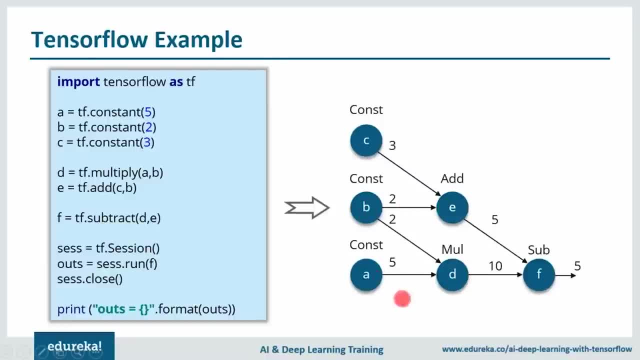 So first we add C and B, then we add B and A, Then we get two other nodes, that is, E and D, And then from that E and D, what we are going to do is we are going to subtract both of them. 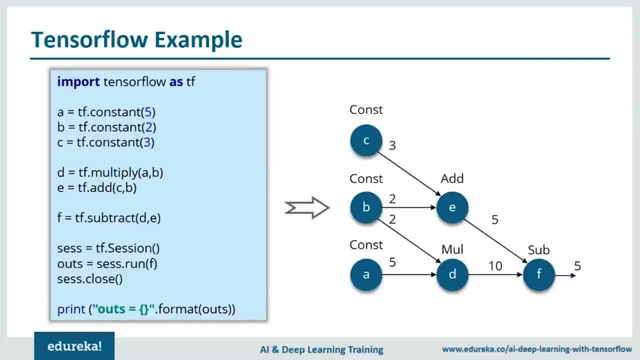 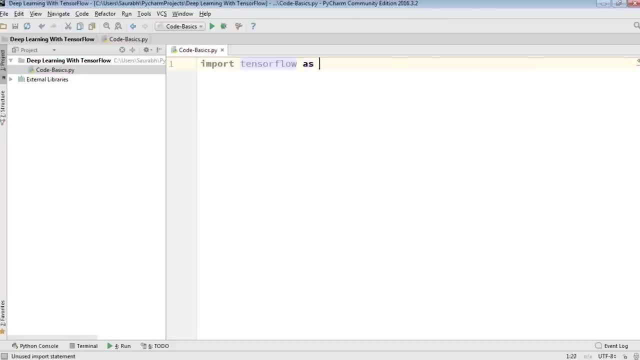 and then we get the final output. Now let me go ahead and execute this practically in my PyCharm. So this is my PyCharm again, guys. First thing I need to do is import tensorflow as tf. Then we are going to define the three constant nodes. 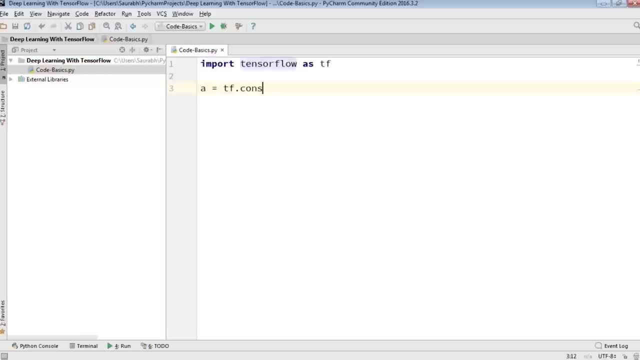 So first is A. A equals to tfconstant, And the value that will be there in A will be five. And then one more constant node that'll be B- tfconstant, And the value that'll be there in it will be two. 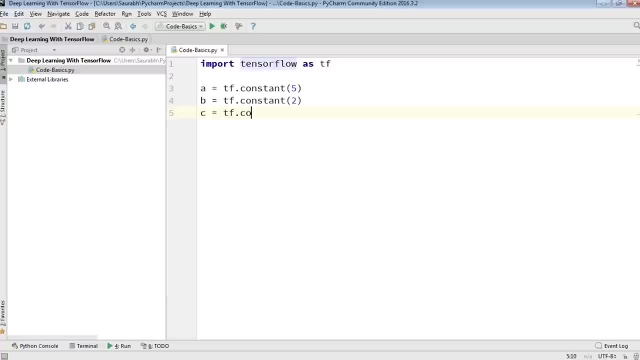 And then I'm going to define the last constant node and tfconstant, The value that'll be. there is three, All right, so we have three constant nodes And now we are going to perform certain operations in them. For that I'm going to define one node. let it be D. 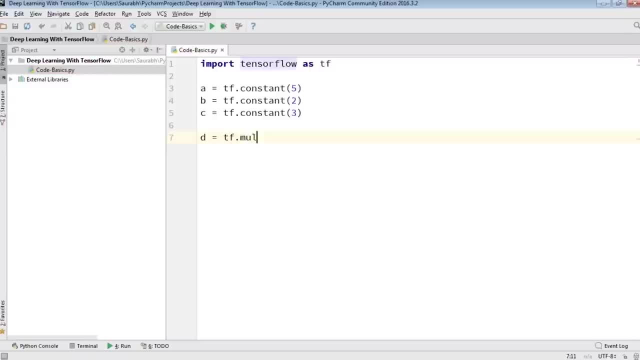 which will be equal to tfmultiplier. So the two nodes that we want to multiply, so that'll be A comma B And then there'll be one more node in order to perform some operation that is addition to tfadd. add C and B. 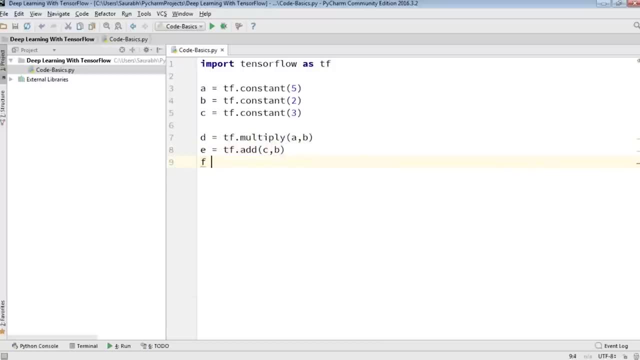 And then we're going to define one more node- let it be F- And inside that node we're going to perform the subtraction operation, tfsubtract D And E. So we have built our computational graph. Now we need to run it, and you know the process. 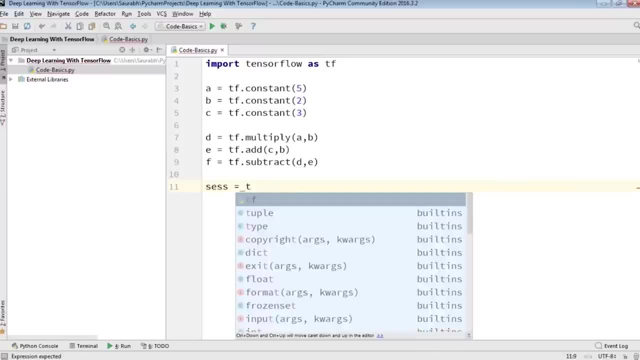 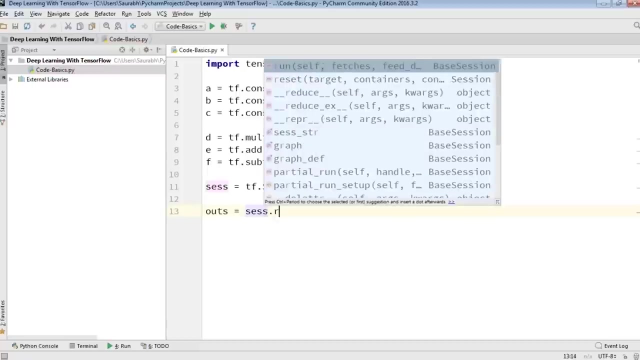 of doing that. ses is equals to tfsession And we are going to define a variable. let it be out whatever name you want to give it And just type in a sesrunf. Let's see if that happens or not. 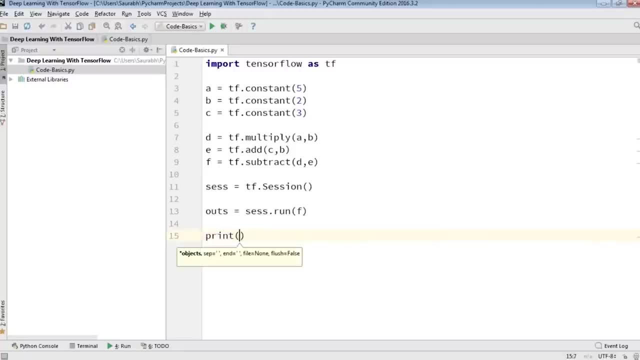 And then we're going to print it. so for that I'm going to print, And then we're going to print it. so for that I'm going to print. So for that I'm going to type in here: print out. 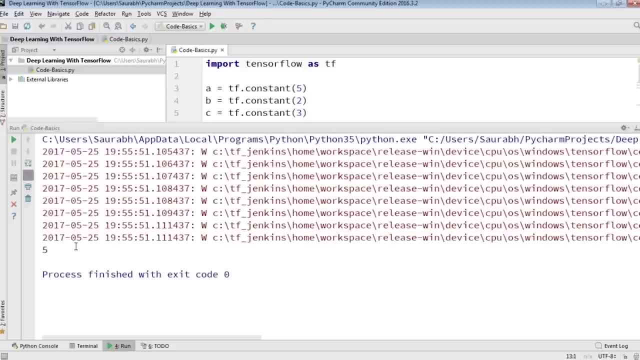 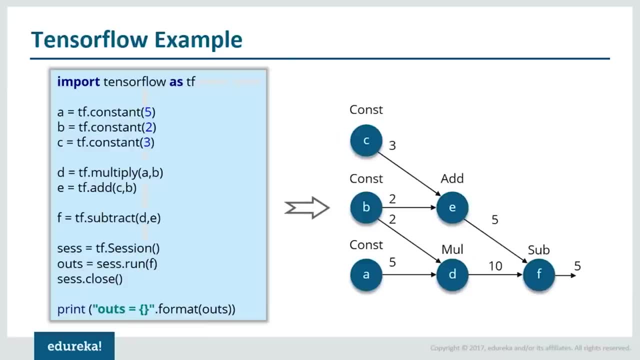 Let's go ahead and run this and see what happens. So we have got the value 5, which is correct, because if you notice our presentation as well, let me open it for you Over here. We also. we get the value 5, similar to our implementation. 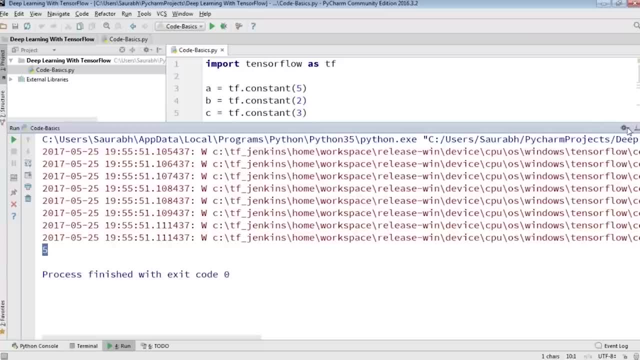 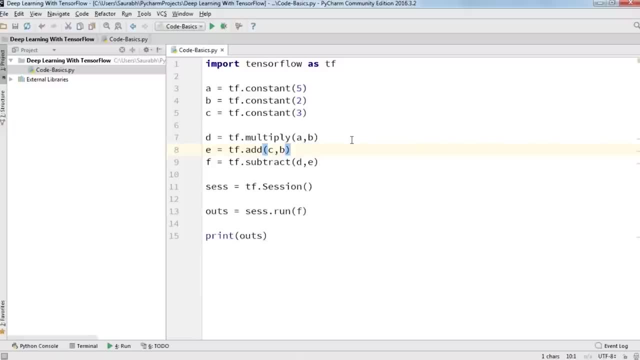 and pie charm as well. So this is how you can actually build a computational graph and run a computational graph. I've given you an example. now, guys, let us move forward, because these are all the constant nodes. What if I want to change the value that is there in the node? 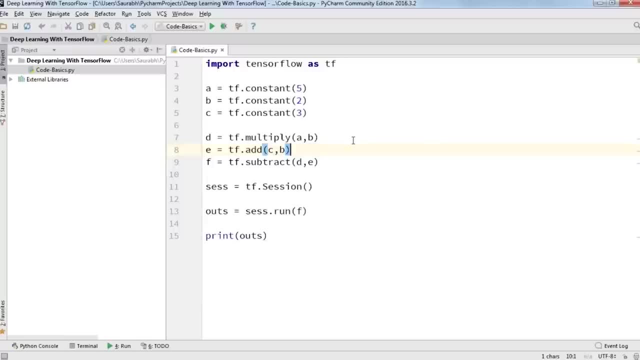 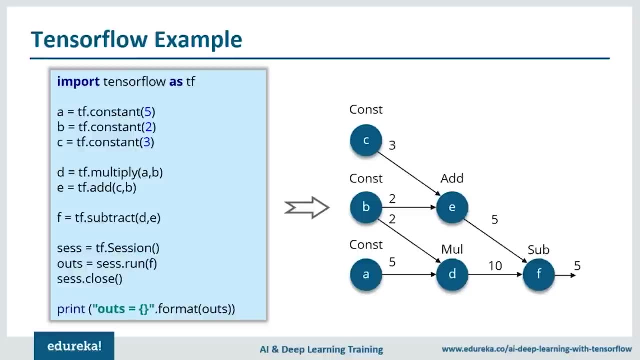 So for that we don't use a constant nodes, for that We use placeholders and variables. Let me explain it to you first. I'll open my slides. So, since these are all constant nodes, so we cannot perform any operation. Once we have provided a value, it will remain constant. 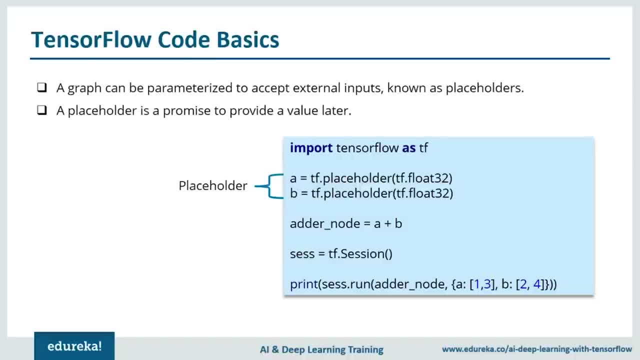 So, basically, a graph can be parameterized, except external inputs as well. And what are these? these are nothing but your placeholders, and these placeholders is basically a promise to provide values later. So there's an example that is there in front of your screen Over here. 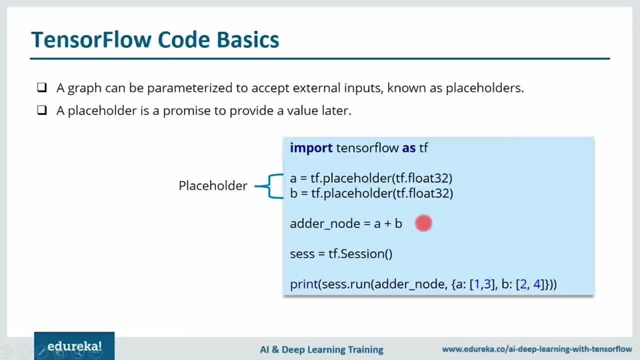 These three lines are bit like a function or a lambda, in which we define a two input parameters, a and B, and then an operation possible in them. So we have actually performing addition. so we can evaluate this graph with multiple inputs by using feed underscore dict parameter. as you can see, we are doing it here. 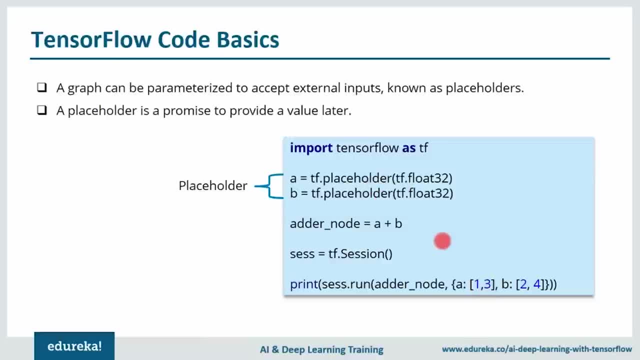 So we are actually passing all these values to our placeholders here. So these all values will be passed and accordingly will get the output. So let me show you practically how it happens. So I'm going to open My pie charm once more. I'll remove all of this, and yeah, so the first placeholder. 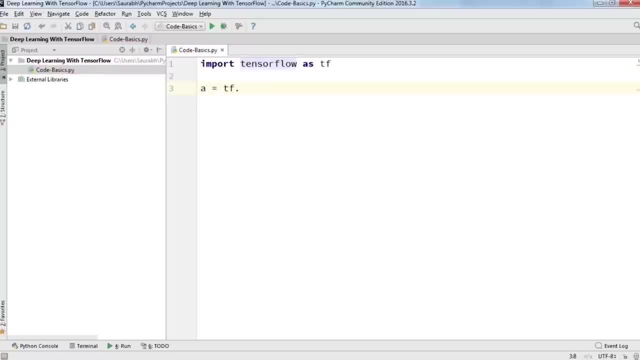 I'm going to name it as a TF, a dot Placeholder, and what sort of a placeholder it'll be. So I'll consider it as float number of 32 bits. Similarly, I'm going to define one more variable as well. I'm going to name it as B. 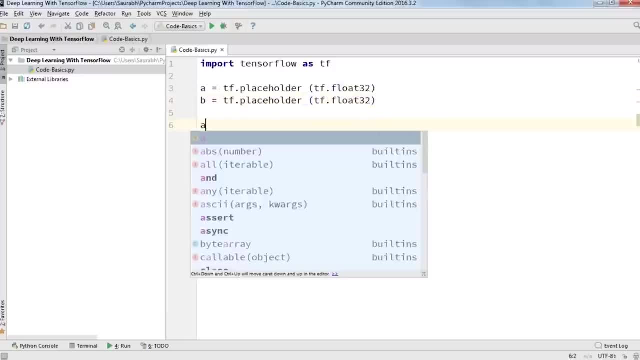 Then I'm going to define an operation that I'm going to perform them. So I'm just going to type in here: adder, underscore, node equals to a plus B, And now our placeholders are currently empty. So that, totally earlier as well, placeholders are nothing but. 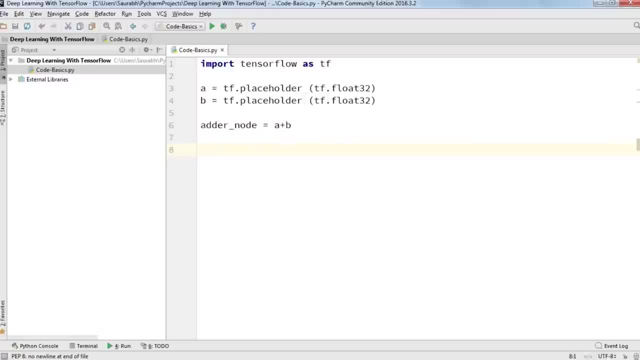 a promise in order to feed values later. So this is how we have built a computational graph. Now our next step is to start a session. So for that I'm going to type in a assess equals to TF, a dot session. Right, Since these placeholders are currently empty and we know that. 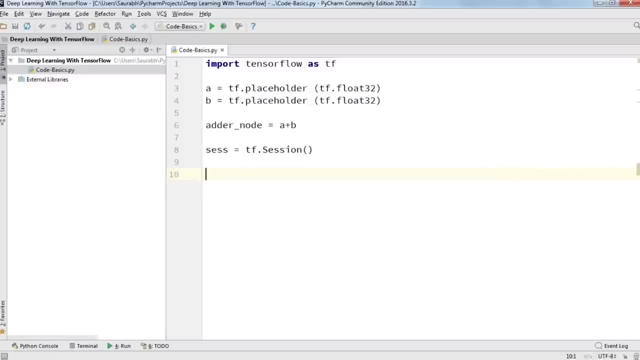 these placeholders Are nothing but a promise, in order to provide them with certain values later. So let's go ahead and provide the values, or you can say a list of values. So I'm going to type in here. print says: dot run Adder underscore node. 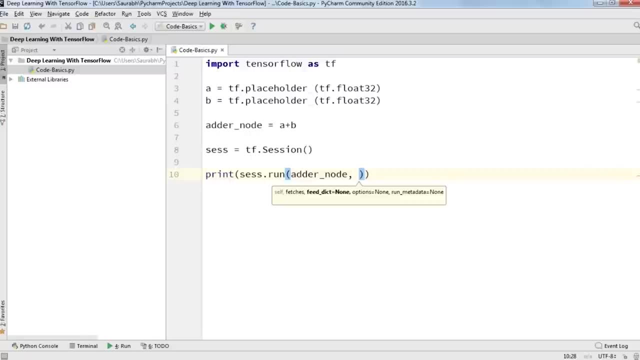 And then the values that I'm going to feed in. So, basically, I'm going to feed in a dictionary: A colon, three, a colon, a list of integer values between one to three, and one more will be B colon, a list of integer values between a two and four. 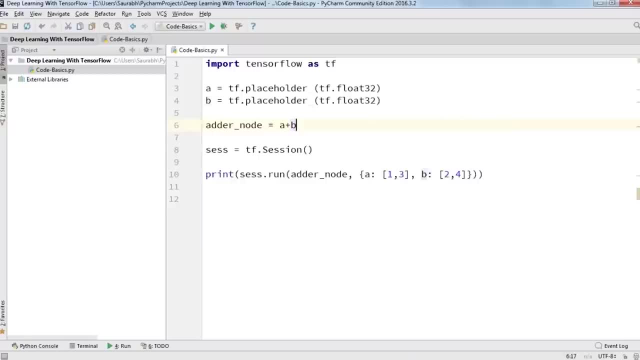 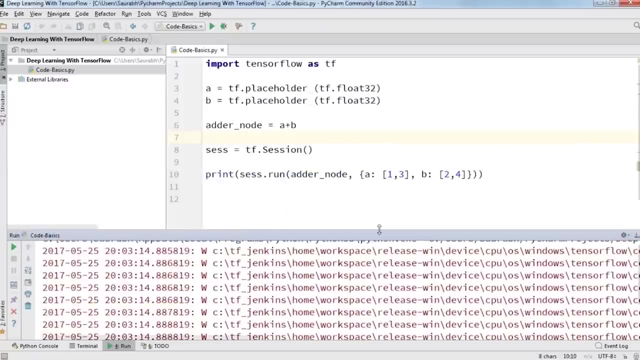 All right, So this is done. now Let us go ahead and execute this and see what happens. So we've got the output: a three and seven. So basically, if you add one into, you get three. similarly, you are three and four, you get seven. 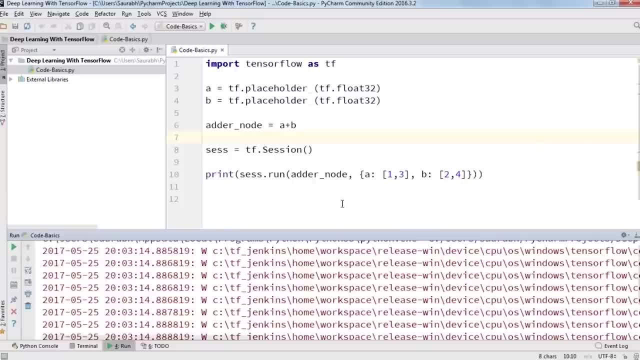 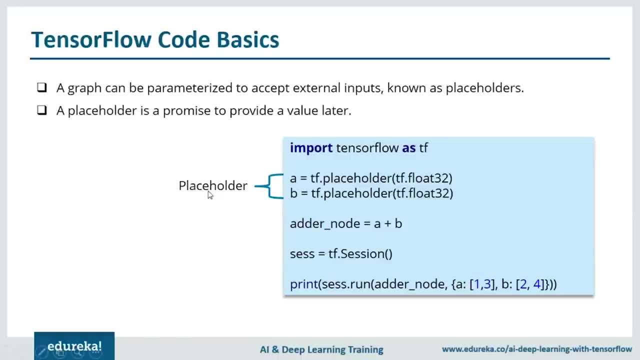 It's pretty easy mathematics, But my main focus was to make sure that you understand what our placeholders. so I'm again going to open my slides and we'll see what's up next. So we understood what exactly our placeholders. now the time to understand what our variables. 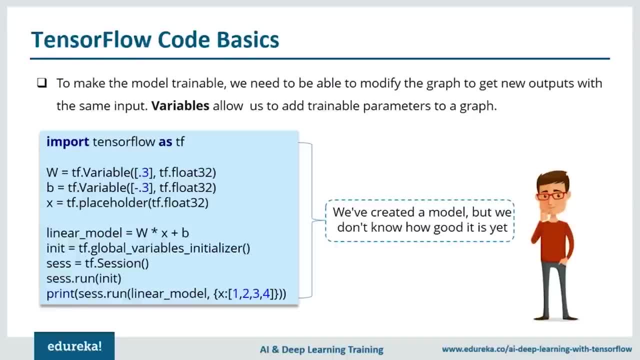 So basically, in deep learning, We typically want a model that can take arbitrary inputs. now, in order to make the model trainable, We do able to modify the graph to get new outputs with the same input, and what helps us to do that? variables basically allows us to add a trainable parameters to our graph. 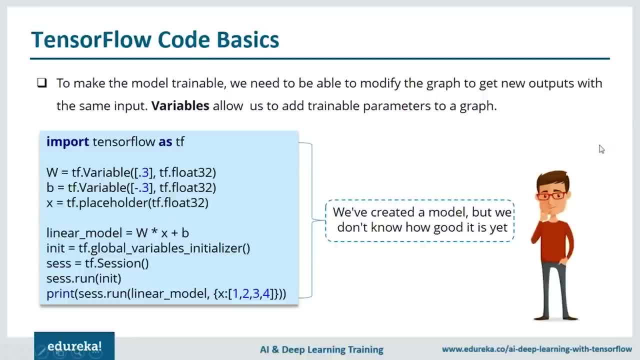 So, in order to declare variables, what we do is you can refer the code that is there in front of your screen. So we have taken two variables in one placeholder And the first variable has a value 0.3.. The other variable has minus 0.3 and the placeholder obviously. 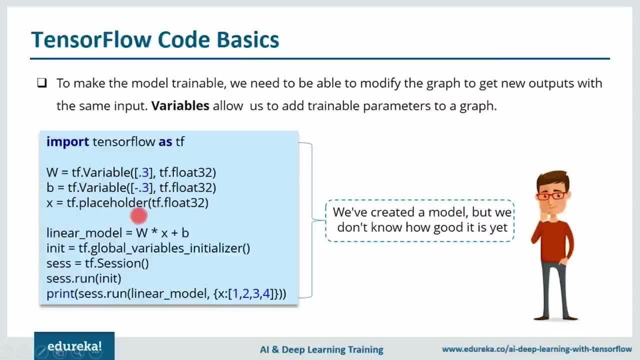 it will remain empty and then later on we feed in some values to it. Then we create a linear model, or you can say some operation, in which we are going to multiply this W with X and then we are going to add a bias or a B value to it. 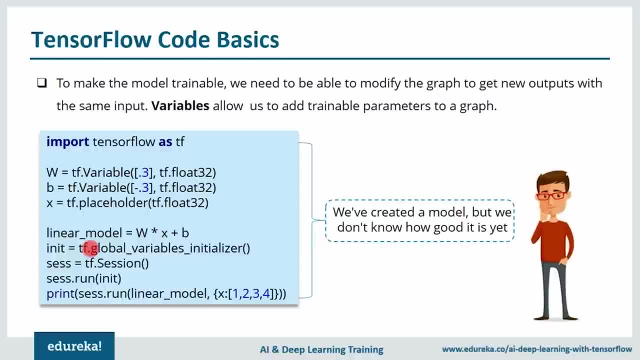 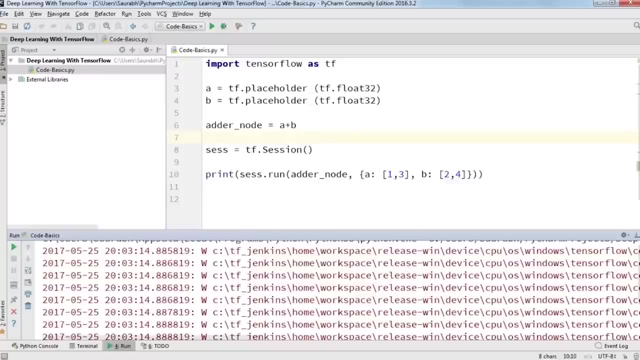 Then what we need to do is we need to initialize all the variables in the tensorflow program. So for that you must explicitly called a special operation, which is a TF dot global variable, We call it initializer, and then just directly run the session. Now let us go ahead and execute this practically guys. 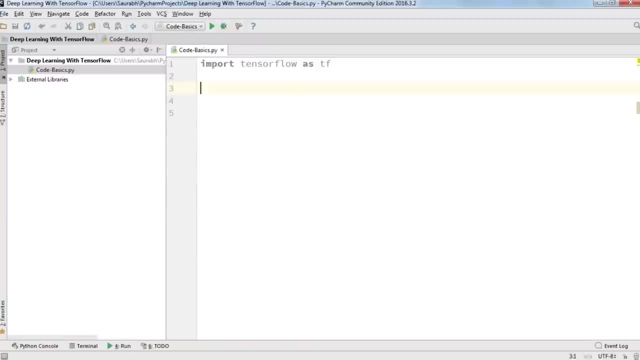 Let me remove all of this. Yeah, so our first variable will be a W and we are going to call in a TF dot variable And in that variable we are going to store a value which is 0.3.. And it is of a flow type, 32-bit. 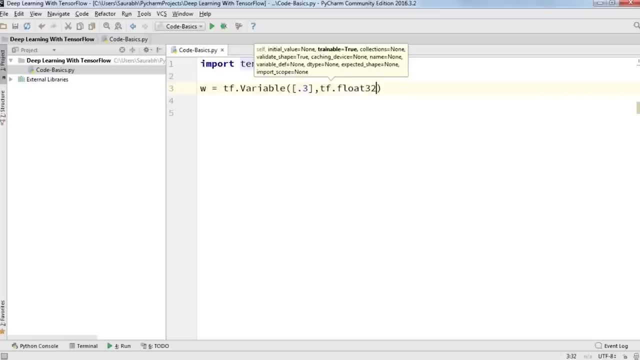 So just type in here: TF dot, float 32.. Yeah, then we're going to define one more variable. Let it be B. So I'm going to type in a TF dot variable and the value of this variable will be minus of 0.3 again. 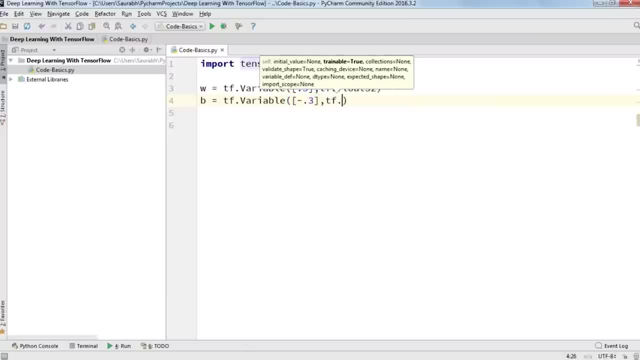 It is float type of 32-bit, So just type in that TF, dot, float 32.. Now I'm going to define a placeholder that is X. X is equals to TF, a dot Placeholder, and it is again a float type, 32-bit. 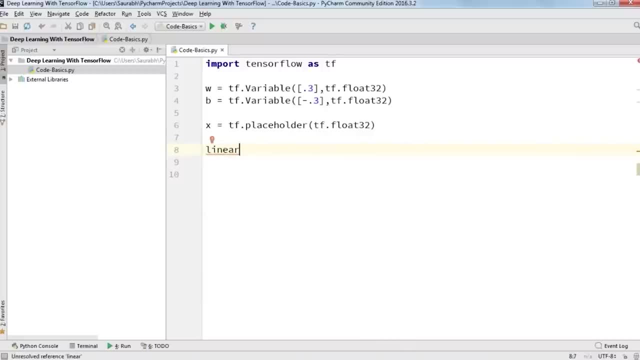 And then some operation that we are going to perform. So I'm going to type in here linear underscore model equal to W multiplied by our X value. that is a placeholder, and then we want to add a bias to it or B value to it. All right, 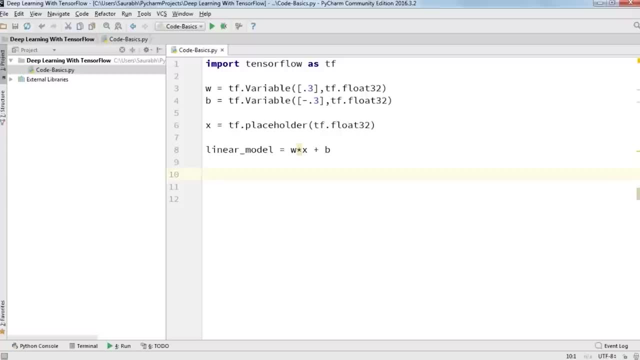 Now, as we have seen earlier as well, in order to initialize constants, We call TF dot constant And their value will never change. but, by contrast, variables are not initialized when you call TF dot variable. So to initialize all the variables in the tensorflow program, what you need to do is you need to explicitly call a special. 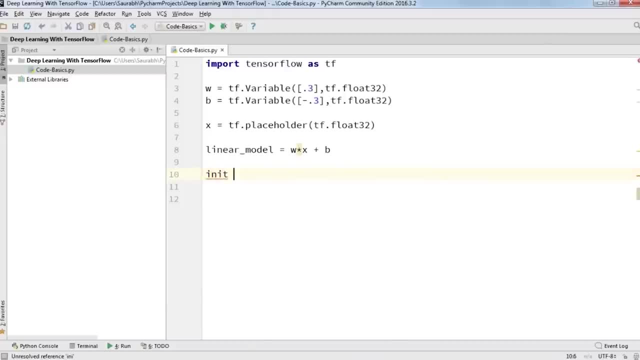 operation and how you're going to do it. Just type in here: INET equal to TF dot. global underscore variables, underscore initializer. That's all and then, and then We're going to run a session. So you know, the process says: is equals to TF dot session. 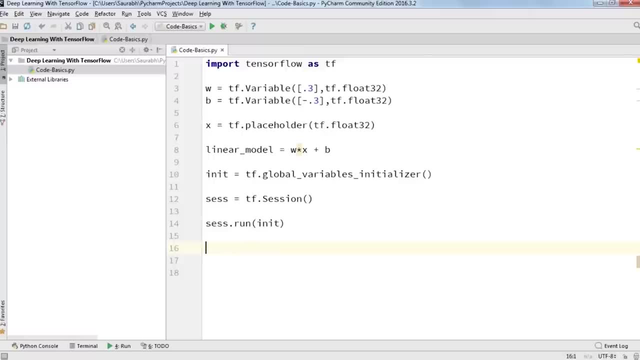 INET. Now let's print it. and before that, what we need to do is need to provide the X placeholder with some values. will actually going to do that at the print statement itself, So I'm going to type. it says dot, run, Run what run? a linear model. 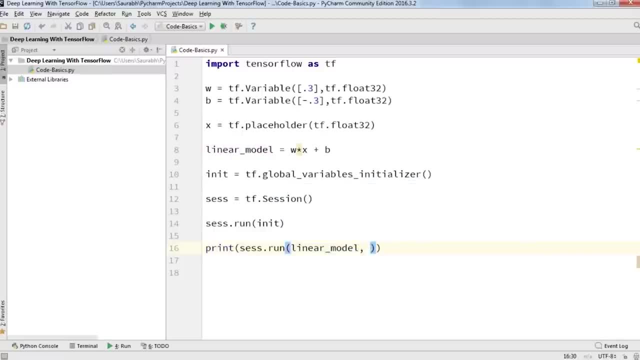 And the values are We're going to pass in. X will be a dictionary again And let me show you how you can do that. So X, a colon, and it will be a list of values from 1 comma, 2 comma, 3 comma, 4.. 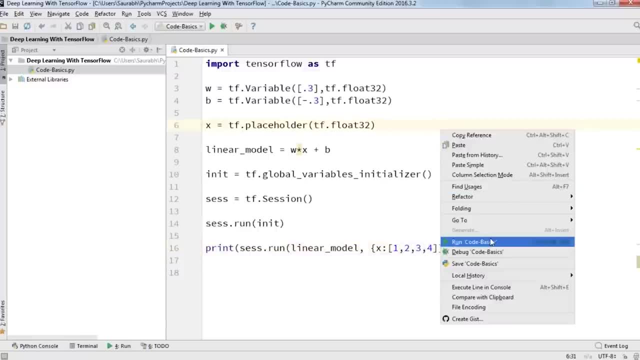 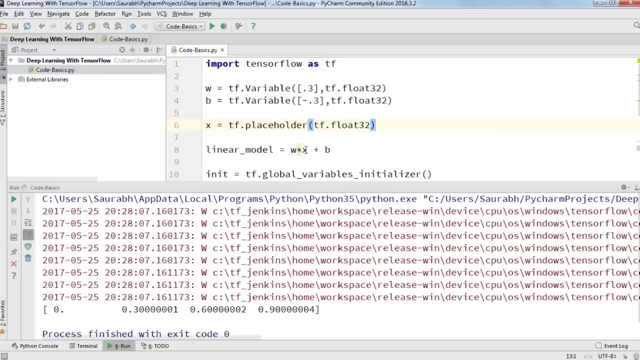 Yeah, that's all, and we are going to run it now. So this is how we get the output. It's simple mathematics, What we have. the first value of W will be 0.3, and the first value of a- B- will be a minus 0.3, and the first value of X will: 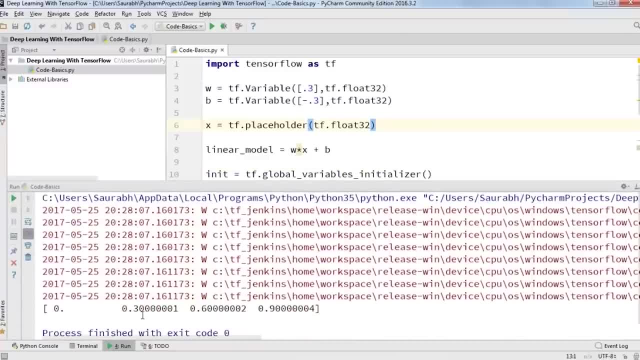 be 1.. So it will be 3 minus 3, which is again 0. similarly for other values as well. You can calculate it. It's absolutely correct. So what we have done? we have created a model, but we don't know how good it is yet. 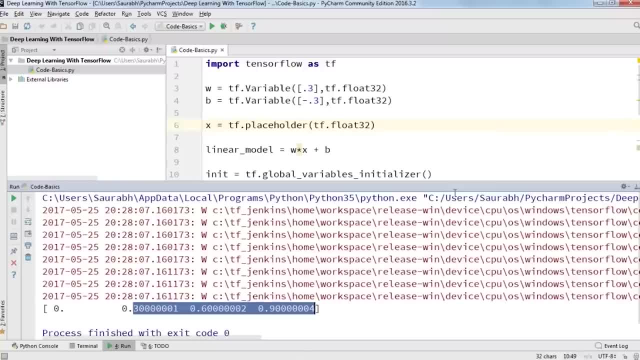 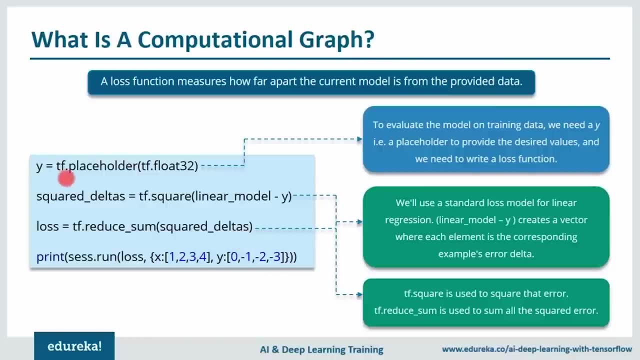 So let's see how we can actually evaluate that. for that I'm again going to open my slides. So now, in order to evaluate the model on the training data, we need a placeholder. Why, as you can see in front of your screen, to provide the desired 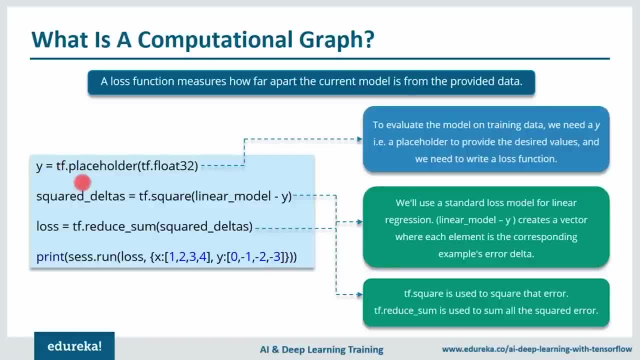 values and we need to write a loss function. So this placeholder Y will actually be provided with the desired values for each Set of inputs, and then we're going to calculate the loss function. And how are we going to do that? We're going to minus the actual output with the desired output. 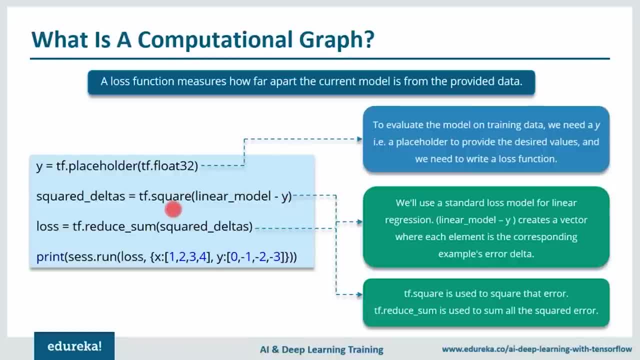 and then we are going to do the square of it. after that We're going to sum all of these square deltas and then we're going to define one single scalar as loss. So this is how we are actually going to calculate the loss, and then after that we need to provide the values to X and Y. 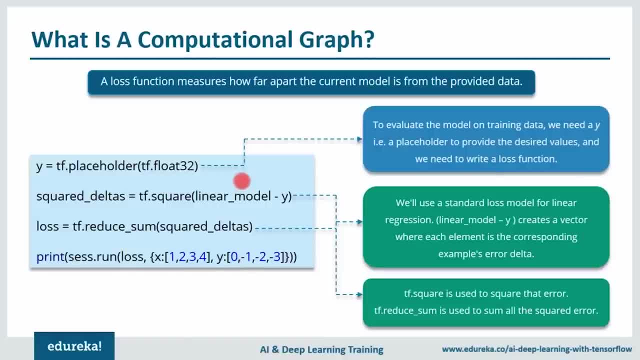 placeholders. So what I'm going to do, I'm going to open my pie charm and then I'm going to show you how correct Our model is on the basis of the values that we provide to Y placeholder. So, guys, this is my pie charm again. 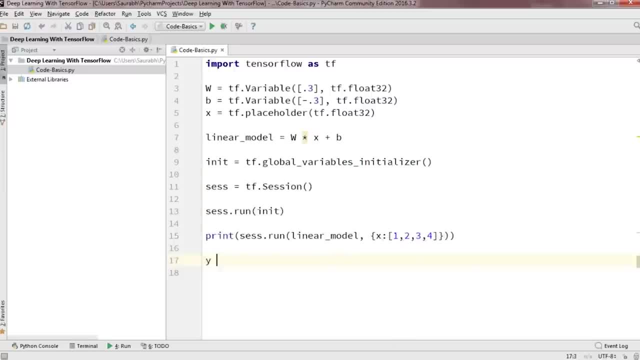 And since here I what I'm going to do is I'm going to define a placeholder first. Why is equals to TF dot, placeholder: TF dot, float 32.. So I'm going to type in a TF dot, float 32, square Delta. I've explained you all these things, but yeah, I'm going to tell. 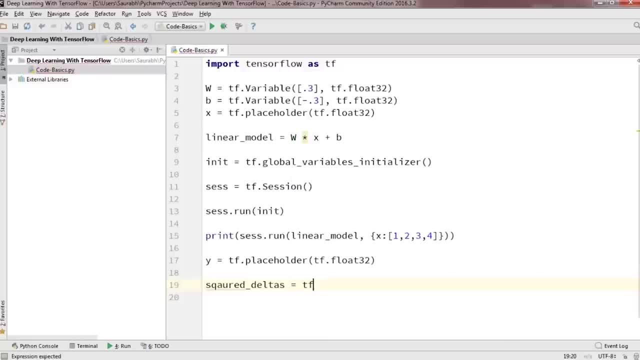 it to you again as well, Don't worry about it. TF- dot- square the actual output minus the desired output, And then I'm going to sum all those losses. or you can say: square deltas, TF dot reduce, underscore sum. So I'm going to type in here square deltas, then finally print. 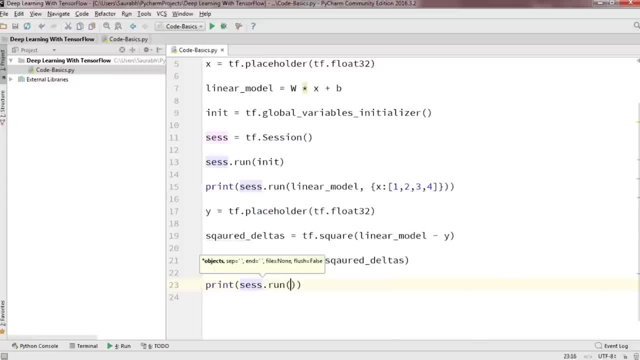 it. So I'm going to type in: says dot run loss X, colon, 1 comma, 2 comma, 3 comma 4, zero comma minus 1 comma, minus 2 comma minus 3, and that's all and we are good to go. 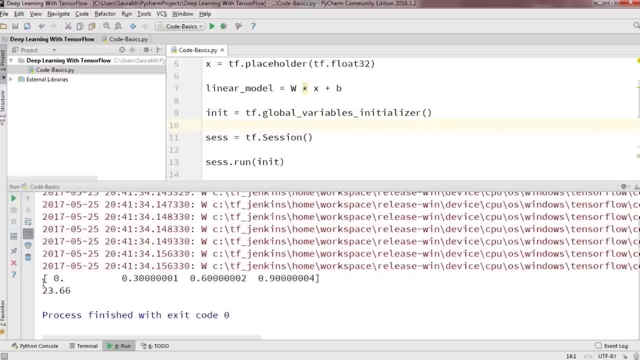 Let's run it and see what will be the loss. So the loss is 23.66, which is very, very bad. Now our next step is to realize how to actually reduce this loss. So let's go ahead with that. I'm going to open my slides. 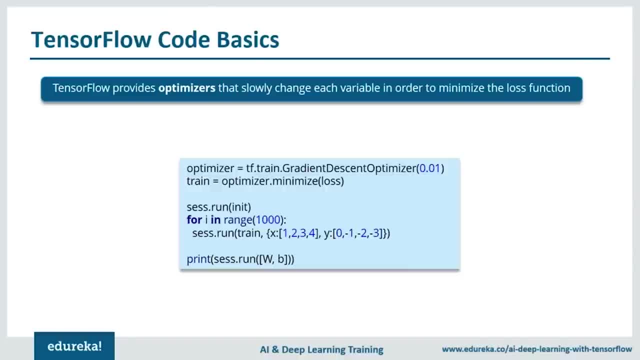 Once more. So in order to minimize the error. Now, in order to reduce this loss, TensorFlow provides optimizers that slowly change each variable in order to minimize the loss function, and the simplest optimizer is gradient descent. In order to do that, We have to call the function called TF dot gradients. 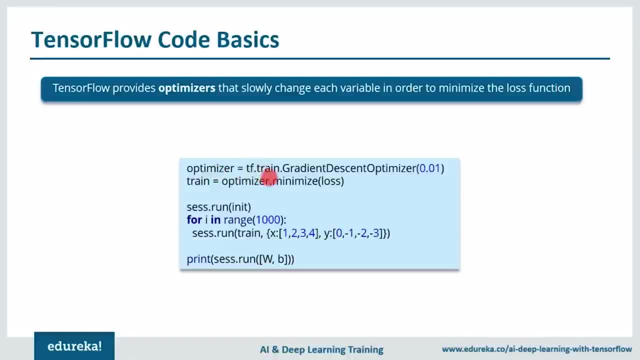 So, as you can see it in the code itself, So we have a TF, dot, train, dot, gradient descent optimizer, and this is nothing but the learning rate point zero one. then train equals to optimizer, Not minimize the loss. So we're going to call this optimizer. 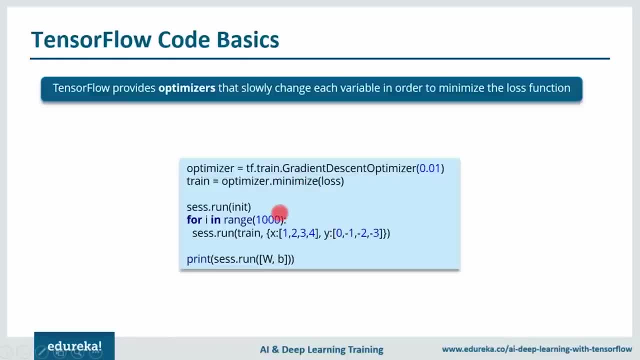 which is nothing but the gradient descent optimizer in order to minimize the loss, and then we are going to run it. So let's see if that happens or not. So for that again, I'm going to open my pie charm, And over here, 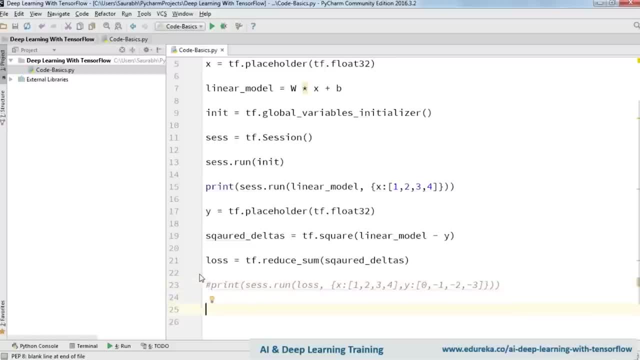 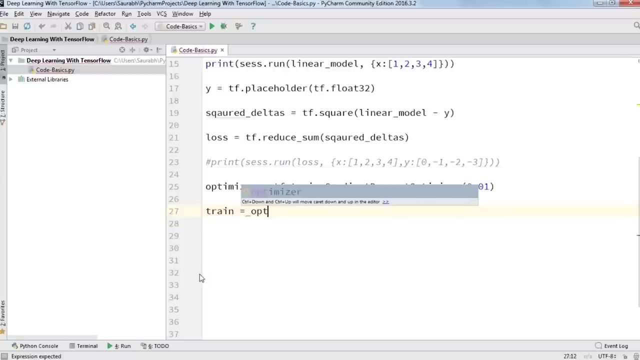 let me first comment this print statement, and now I'm going to type in here: optimizer equals to TF, dot. train Gradient descent optimizer and the learning rate will be point zero one. Now I'm going to type in here: train equal to optimizer, dot- minimize loss. 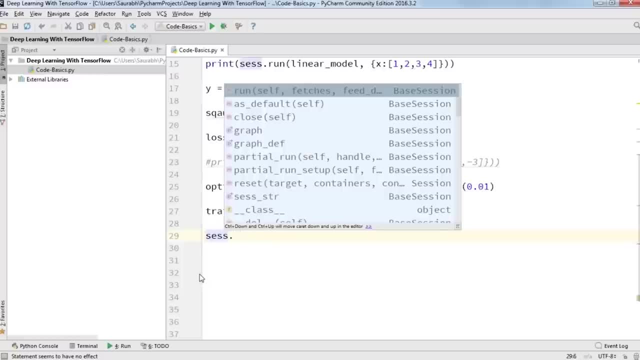 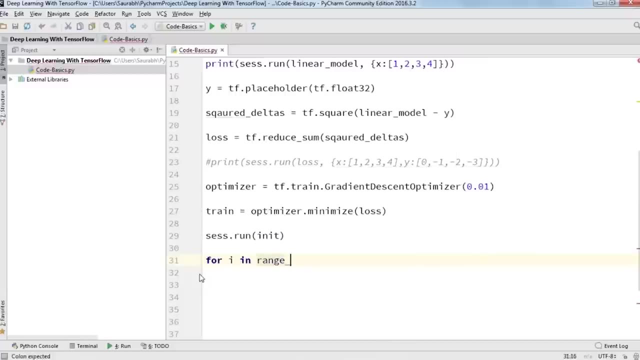 And then now let's go ahead and run. this says dot run, I in it S dot run, and we're going to feed in values to our X and Y placeholders. train comma X will have values one, two, three, four And Y will have values zero comma minus one. comma minus two comma. 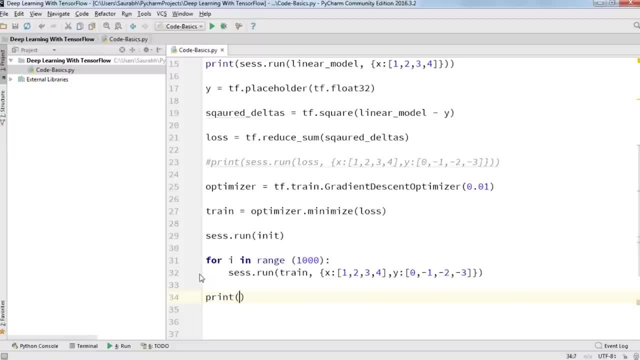 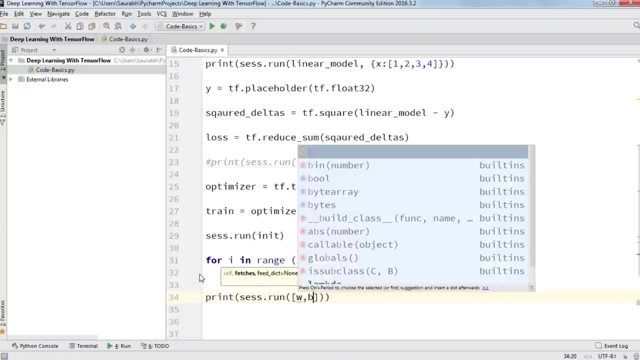 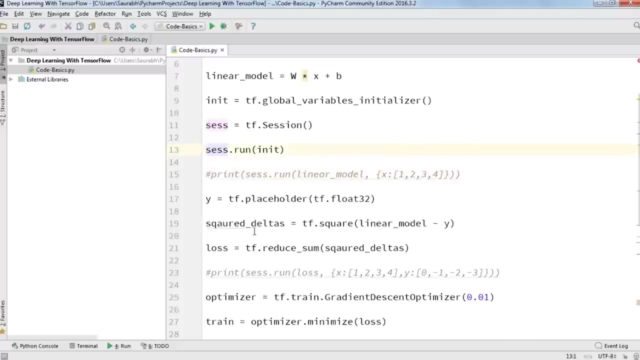 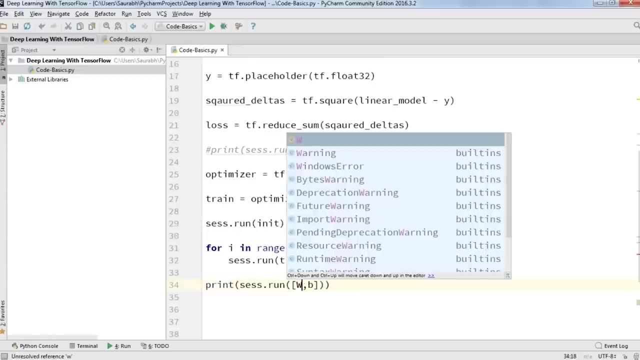 minus three. print says dot: run W comma P. Now let me first go ahead and comment these lines. All right, so I've just made a mistake here. This is in uppercase W and yeah. so now we are good to go and let's run this and see what happens. 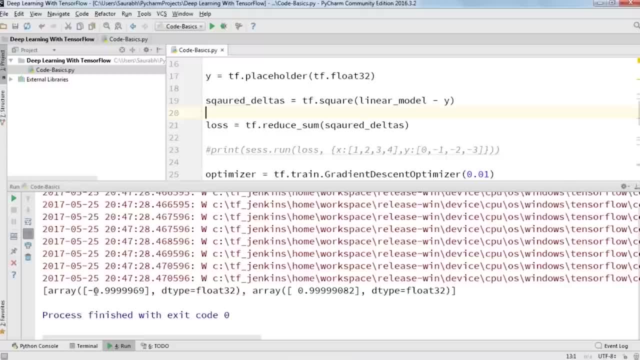 So these are our final model parameters. So the value of a W will be around The point nine, nine, nine, nine, six, nine, and the value of our B will be around a point nine, nine, nine, nine, zero, eight, two. So this is how we actually build a model and then we evaluate. 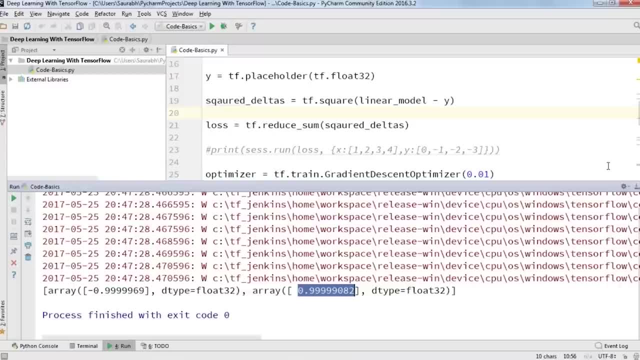 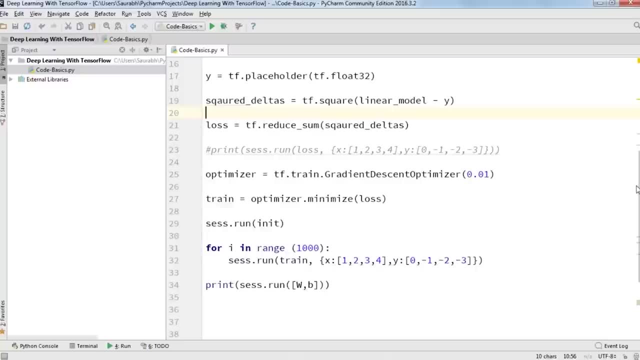 how good it is, and then we try to optimize it in the best way possible. So I've just given you a general overview of how things works in TensorFlow. So now is the time to actually implement the and and or gate that I was talking about at the beginning of the session. 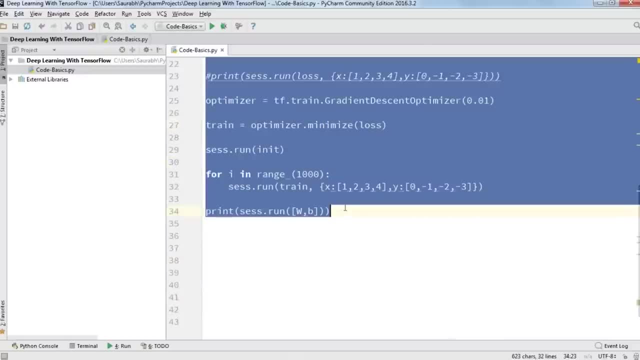 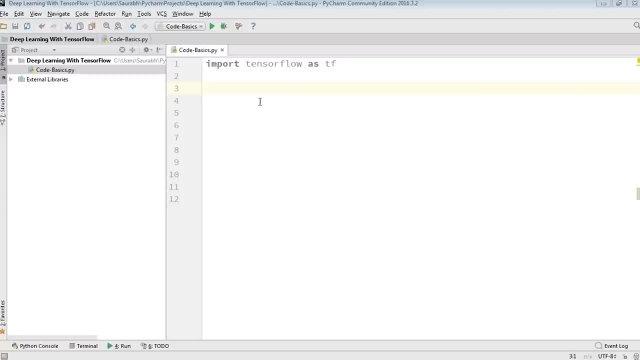 So for that, let me first remove all of this. Yeah, Now, in order to implement and gate, our training data should consist of the truth table for and gate, and we know that truth table and we know that if any of the input is low, then output. 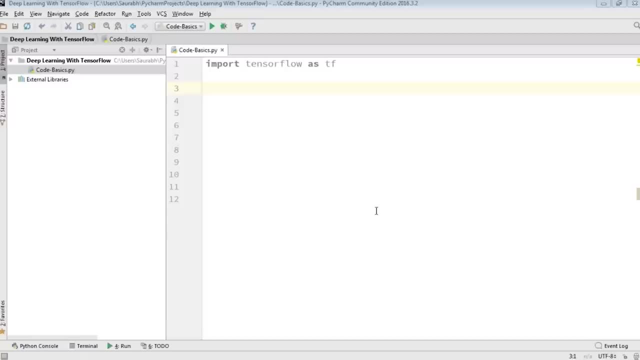 will be low, and, and if both the inputs are high, then output will be high. One thing to note here, guys, is that the bias is implemented by adding an extra value of one to all the training examples. So yeah, enough of the explanation, Let's go ahead and code it. 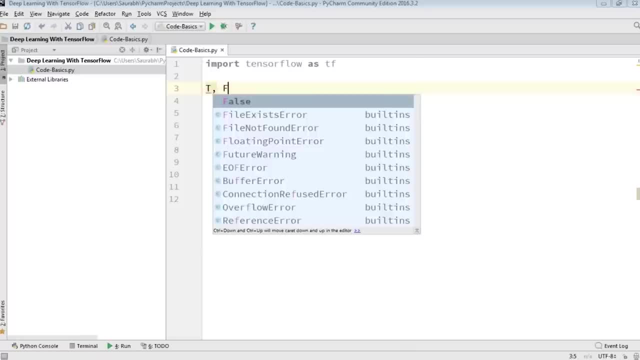 So I'm going to type in here: T comma, F equal to one point, comma minus one point and bias will always be one. So I'm going to type in here: bias is equals to 1.0. and now I'm going to provide the training data. 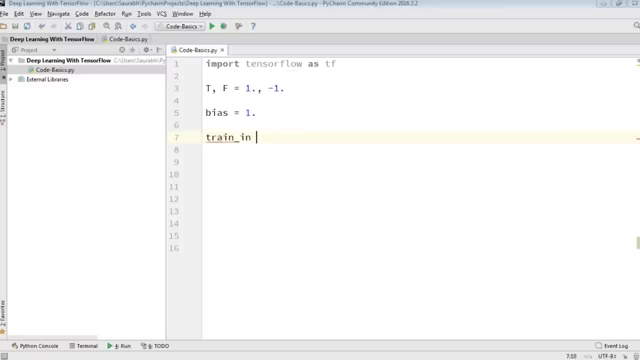 So for that I'm going to type in train underscore in equal to: if one input is true and the another input is also true, then we have bias. then again, if one input is true, the other input is false, Then also we have bias. similarly, one input is false another. 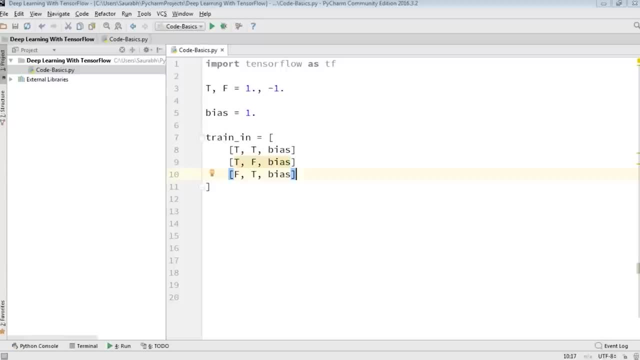 input is true, then we have bias, and then, finally, when both the inputs are false or zero, Then we have bias. right, This is our training data and the train out will type in here as the output. basically, train underscore out will be equal to: so, yeah, if both the inputs are true or both the inputs are one. 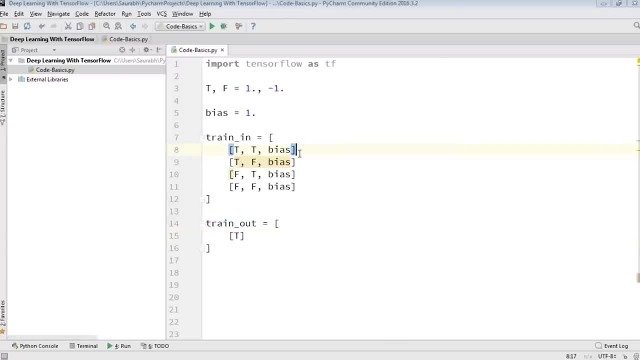 then output is true. Oops, I forgot our comma everywhere. Let me just go ahead and do that. Yeah, so if both inputs are true, the output will be true. If any of the input is for, the output will be false. I'm just going to type in here: falls everywhere, because there's. 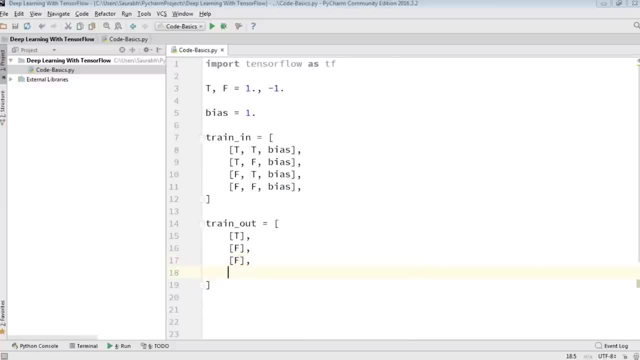 only one condition in which we have the true output. All right, so this is done now. Now, as we know that tensorflow works by building a model out of empty tensors, then plugging in known values and evaluating the model, like we have done in the previous example, since 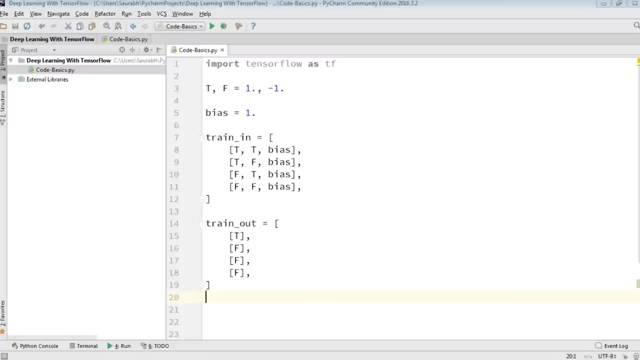 the training data that we have provided will remain constant. The only special tensorflow object we have to worry about in this case is our 3 cross 1 tensors of vectors. And now what are we going to do? We're going to define a variable and we are going to put in 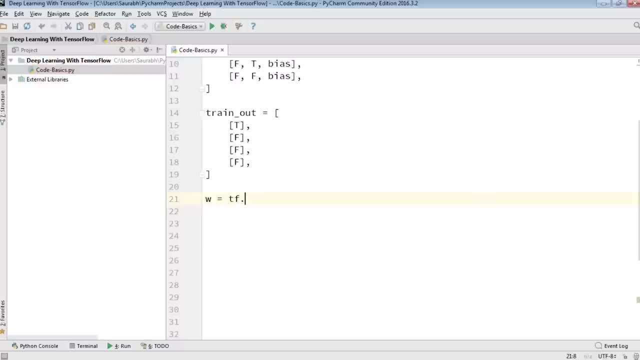 some random values in it. So I'm just going to type in TF, a dot variable, and generate the random function: TF, dot, random underscore, normal 3, comma 1.. Now what it is? it is basically a variable, so its value may be changed on each evaluation of the model as we train with all. 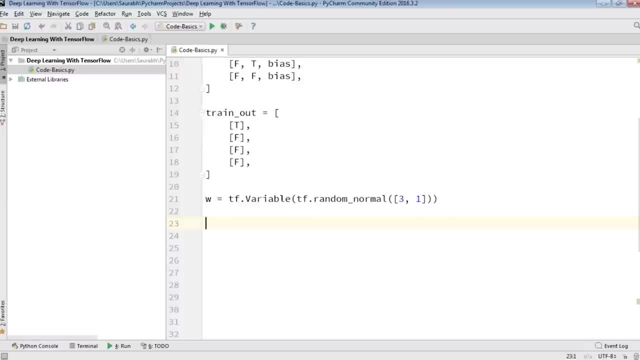 values initialized to normally distributed random numbers. Now that we have our training data and weight tensor, we have everything needed to build a model using tensorflow. So what we need to do, we need to define an activation function and we're going to define a step activation function or step. 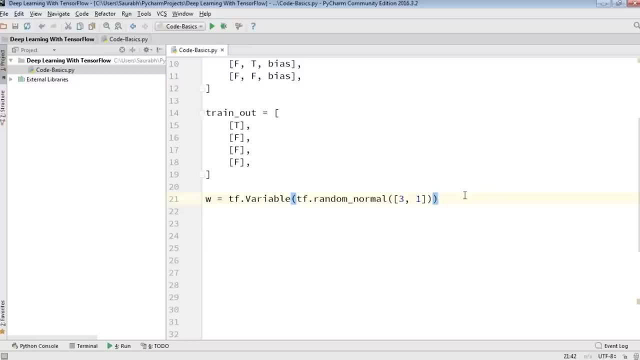 function. So for that, what I'm going to write here Is a function step. we're going to define our own step function, although you can use the predefined function as well. that totally depends on you. I'm going to type in here: is greater equal to TF, dot greater. 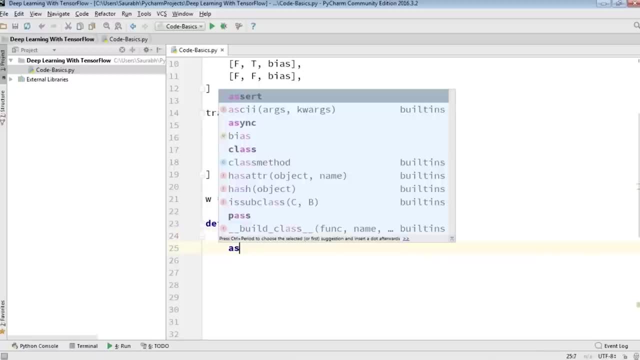 X, comma 0.. Then we're going to define one more variable as float TF: a dot T O underscore float Is underscore greater. Then we're going to define one more variable, a doubled equal to TF, a dot multiply As underscore float, comma 2.. 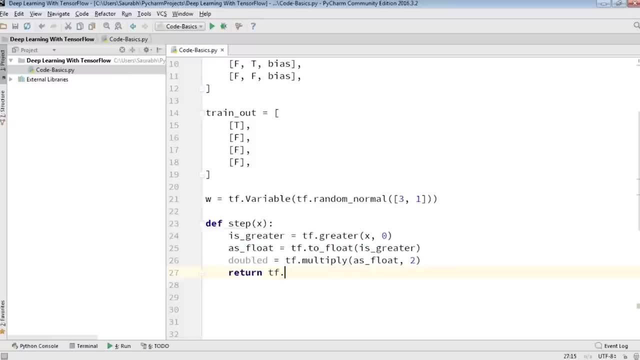 Then return TF dot Subtract doubled comma 1.. So now this is how we have defined our step function. So with the step function defined, the output error and the mean squared error of our model can be calculated in one short line each. Let me show you how you can do that. 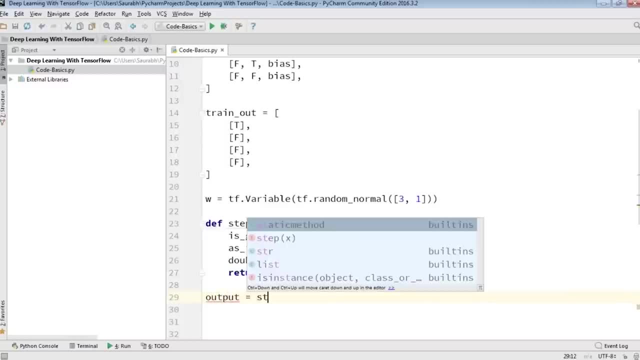 So just type in here: output equal to call that function. that is step TF: dot matrix multiplication matmul Train underscore in comma W. Now for error. We're going to type in here: error equals to TF: dot subtract Train underscore out Comma output. 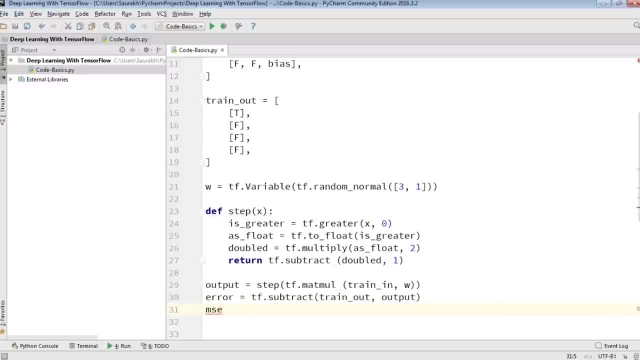 And for mean squared error, I'm going to type in here MSC equal to TF dot, reduce underscore mean TF dot Square And then error. Now the evaluation of certain tensor functions can also update the values of variables, like a tensor of weights W. 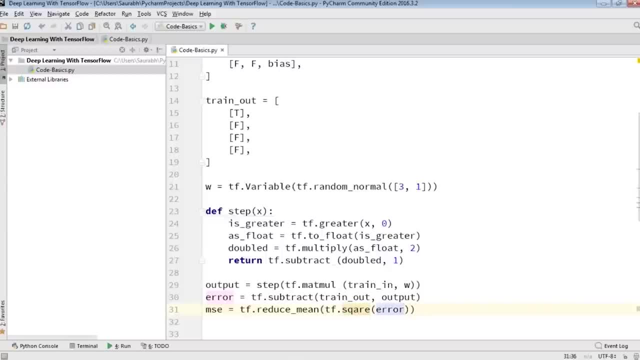 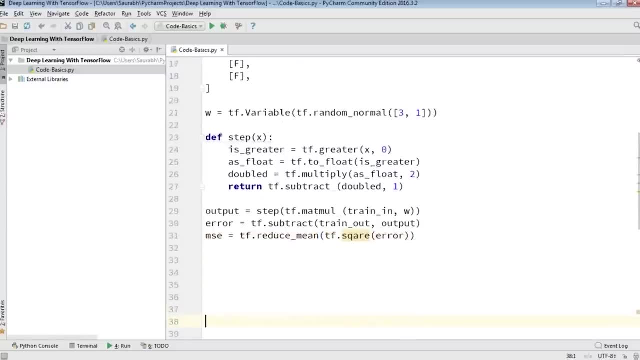 So in our case, basically, we're going to update the weights W. So first we calculate the desired adjustment based on error, Then we add it to W. Now let me show you how we'll do that. So, if you can recall, we have done that in the previous example. 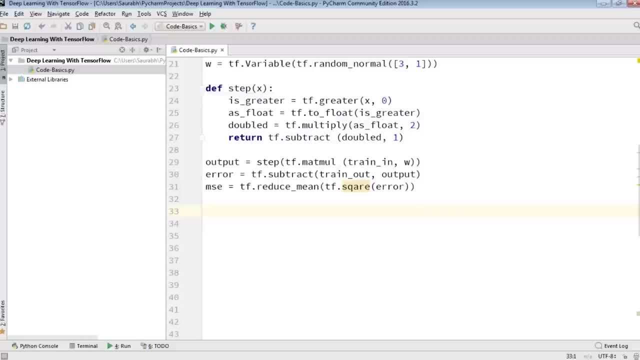 As well, where we were updating the weights and bias. So now I'm going to type in here: Delta is equals to TF dot matmul. or you can say: matrix multiplication: Train underscore in comma error comma transpose underscore a equals to true. Then we're going to type in here: train equal to TF, dot assign. 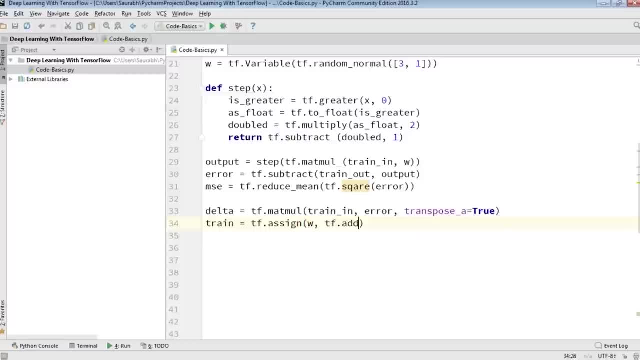 W comma TF dot, add W comma Delta, The first matrix multiplication, and then we're going to add it all. The model has to be evaluated by tensorflow session, which we have seen earlier as well, But before that we also need to initialize all the variables. 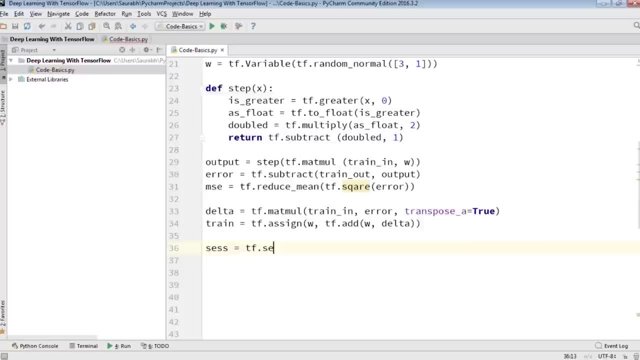 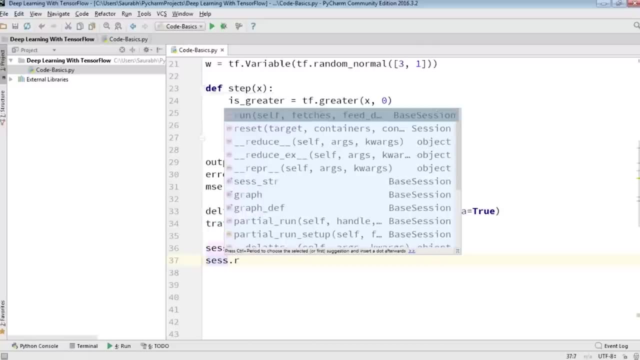 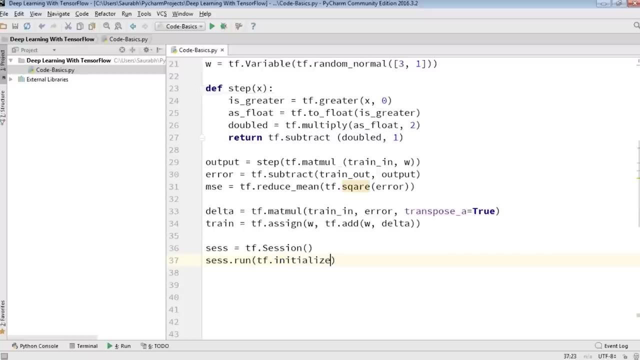 So first let me just type in here: says equals to TF, dot session. And then I'm going to type in here: says dot run, TF, dot initialize, underscore all variables. So now what our next task is in order to perform various iterations so that we get zero error. 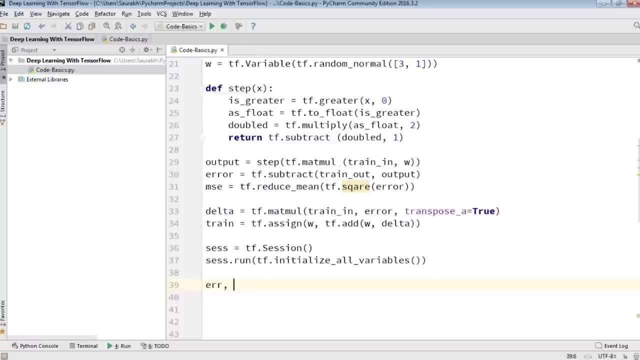 So what we're going to do, we're going to define a variable, ERR, and our target. So, basically, our ERR is nothing but an error, which can be equal to 1 or 0, because we are using binary output. So our error can be 1 and our target is to make it as 0. right now. 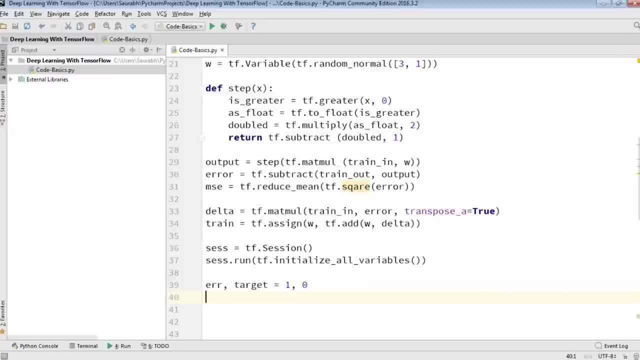 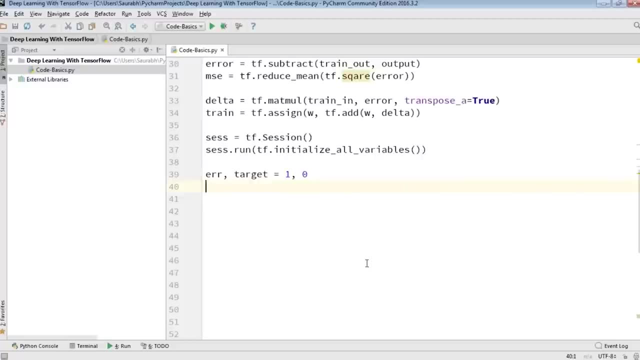 Next, what we're going to do. We're going to define a park. now. you can consider right now a park as nothing but the number of cycles, or you can say number of iterations that will be required in order to reach the desired output. or you can say, in order to reduce the error to 0.. 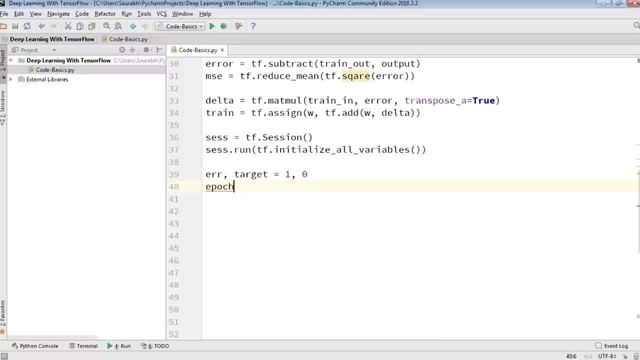 So I'm just going to define that. so I'm going to type in here a park, or you can give whatever variable name you want, and I'm going to type in here, Max underscore, a park Equal to 0 comma 10, which means that our it will start from the 0th Epoch and our maximum value of Epoch will be 10.. 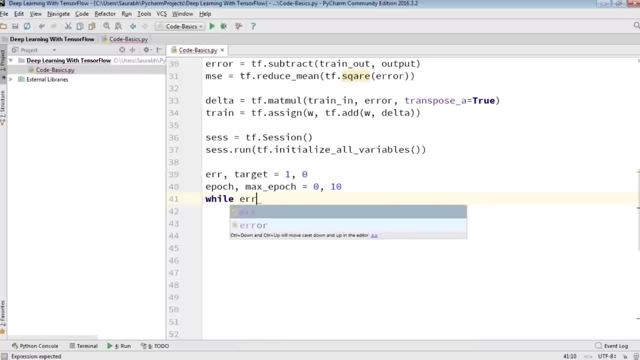 Now I'm going to define: while ERR should be is greater than target And Epoch is less than maximum, Epoch Increase the value of Epoch y1.. Then we're going to type in: ERR Says: dot run Mean squared error, comma train, And let's just finally print it and see what happens. print Epoch. 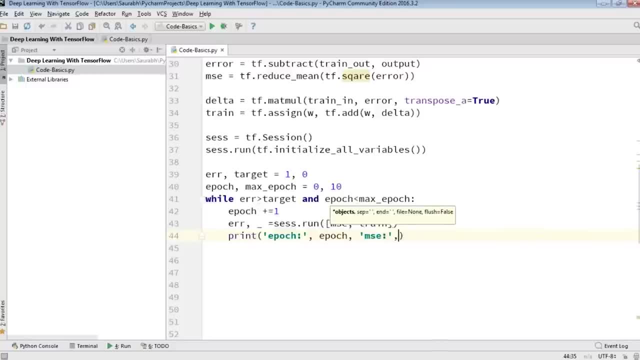 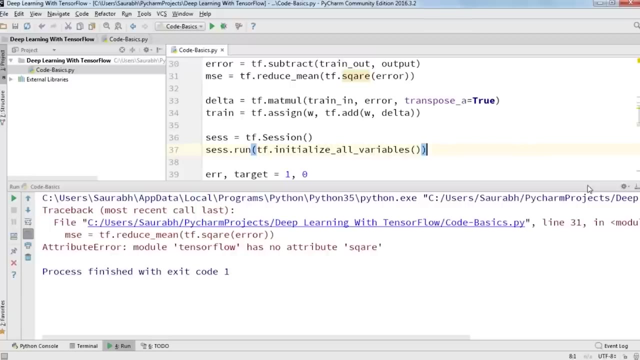 Mean squared error, Colon ERR. So, basically, what it will print? it will print the cycles, or Epoch, and the error with respect to that particular cycle. So let us go ahead and execute this and see what happens. Oops, I've typed the spelling of square wrong. 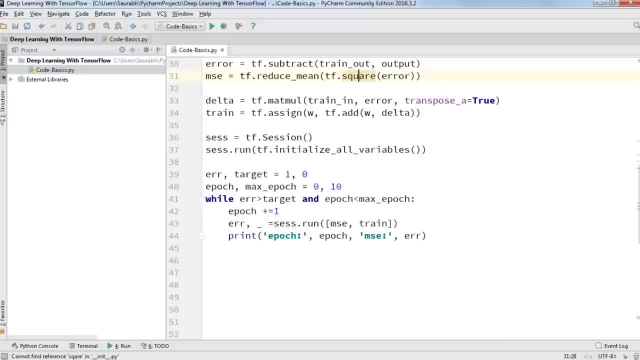 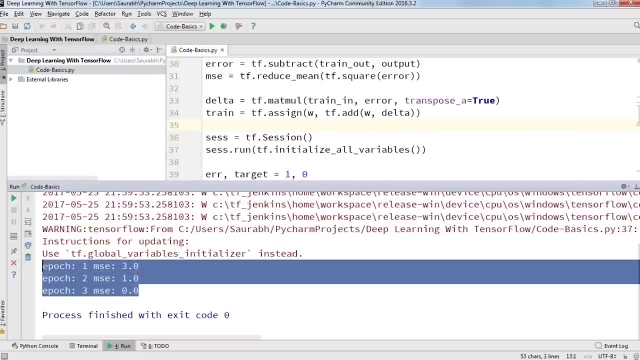 Pardon me for that, So I'm just going to make it right now. SQ, you are e? All right, let's go ahead and execute it once more. So yeah, in three Epochs we got the value of mean squared error as 0.. 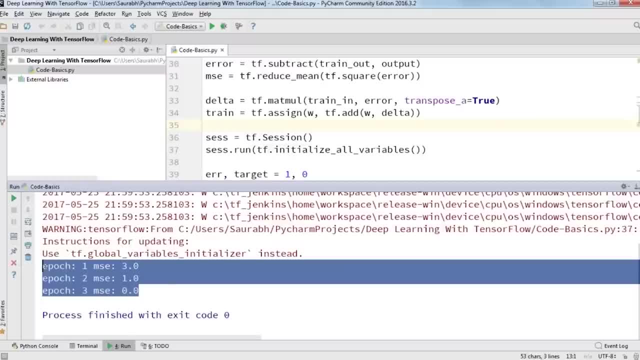 That means it took us three iterations in order to reduce the output to 0.. So this is how you can actually implement a logic gate. or you can say: this is how you can actually classify the high and low output Of a particular logic gate using single layer perception. 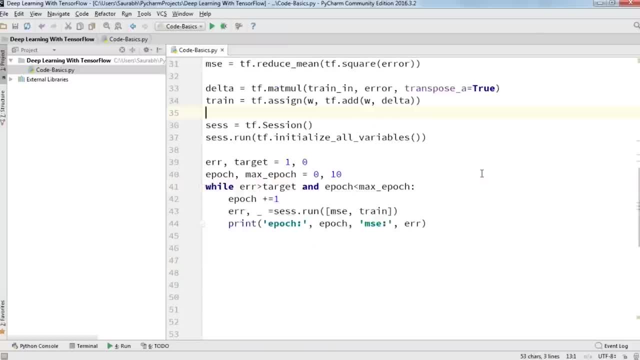 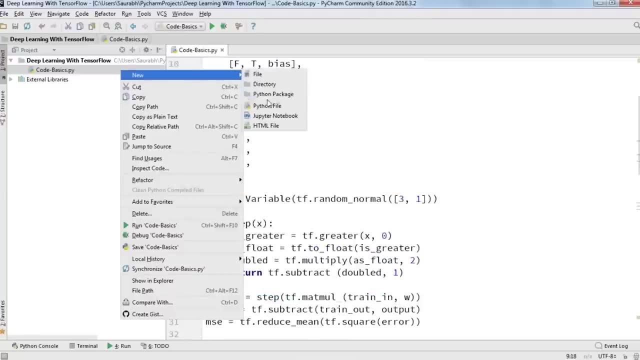 Similarly, you can do that for our gate as well. Consider this as an assignment: come up with a code that can actually classify the high and low outputs of an or gate. What I'm going to do, I'm going to create a new python file and I'm going to name it as MNIST. 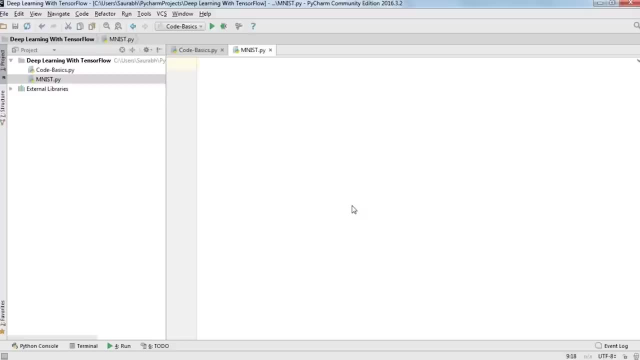 which is nothing but the data set on which we are going to perform the classification of handwritten digits. So we're going to execute a use case and we have told you earlier as well. in this MNIST data set We have handwritten digits, It's between from 0 to 9 and it has 55,000 training sets as well as 10,000 test sets. 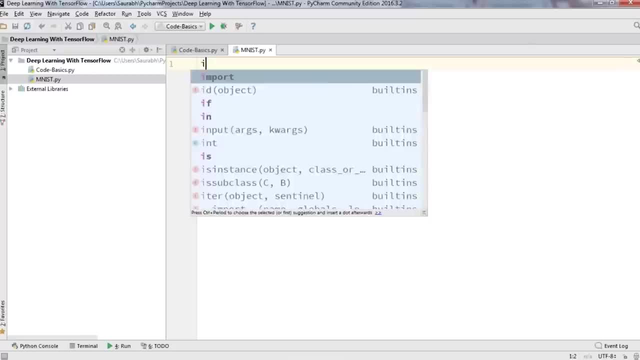 So let us go ahead with that. The first thing I'm going to do is download the data set, But before that let me just import tensorflow library as TF. and yeah, now let us download the data set. So for that I'm going to type in from tensorflow: dot examples, dot, tutorial, dot, MNIST. import input underscore data. 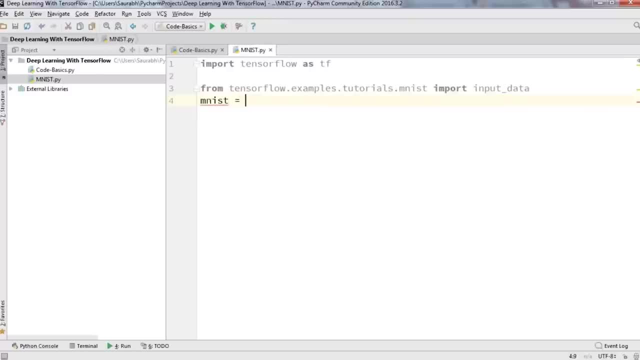 And now I'm going to type in here: MNIST is equals to input. underscore data: dot read data sets. Type in here: MNIST: underscore data: Comma 1. underscore hot equals to true. Now here, MNIST is nothing but a lightweight class which stores the training validation. 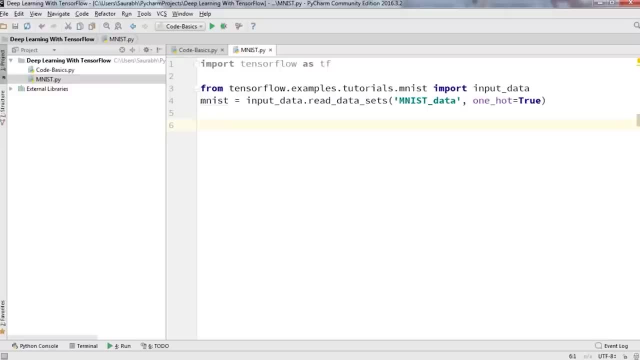 And testing sets as a numpy Y at is, and when I talk about this, one hot equals to true, is nothing but one hot encoding. Now let me tell you what one hot encoding is. So for that, let me just comment few lines. So one hot encoding means that if I'm classifying something as a seven, 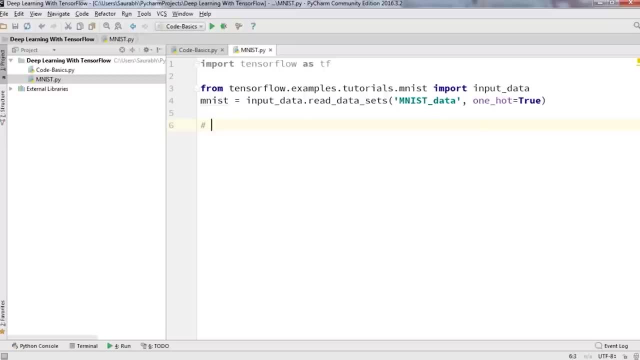 so if I classify that, my digit is seven. so how am I going to represent that? So I'm going to type in here: 0, 1, 2, 3, 4, 5, 6, 7th, a bit will be active. So I'm going to type in there one, then eight and then nine. 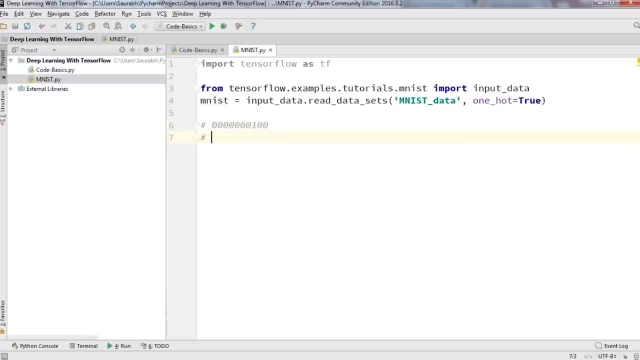 Similarly, if I want to represent, say that my digit is 2, so I'm going to type in 0, 1. on the second digit, I'm going to type in here as one and the rest all zeros. So I hope you got the concept of what exactly one hot encoding is. 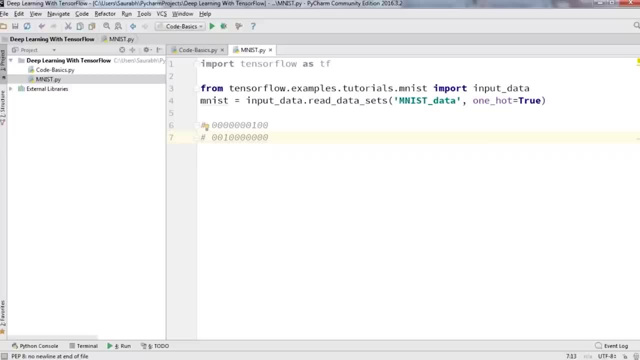 So it's like only one output is active at a time. That's all. So our next step is to start the session, like we do every time. So I'm going to type in here: sets equals to TF dot- active session. So I'm just going to type in here: interactive session. 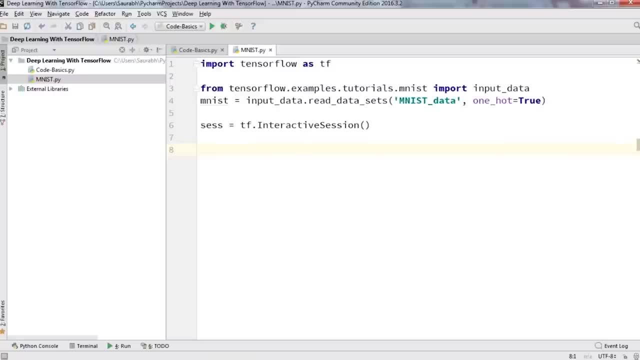 Yeah, And now we are going to do, we're going to build the computation graph by creating nodes for the input images and target output classes. So for that I'm going to define some placeholders, for that I'm going to type in: X is equals to TF dot placeholder. 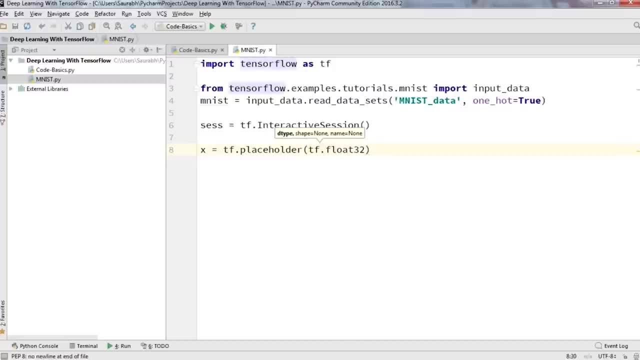 TF, dot floor 32.. And the shape will be none comma 784.. Now the input images X will consist of 2D tensors of floating point numbers. Here we assign it a shape of, say, none comma 784, as you can see. So where 784 is the dimensionality of single flattened 28 by 28 pixel. MNIST image of handwritten digits. 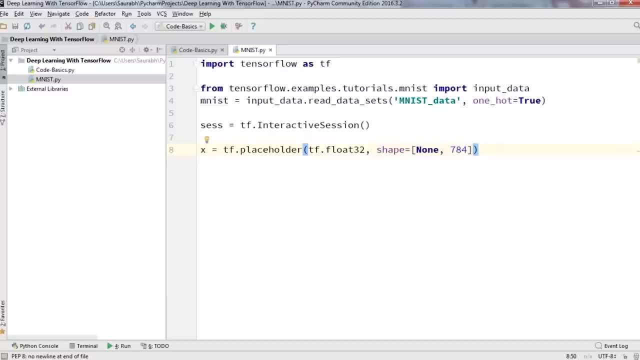 and what none indicates. it indicates that the first dimension corresponding to the batch size can be of any size, means the first dimension can be of any size. We are not putting any restrictions on that. Now I'm going to define the variable Y, which will nothing, which will be nothing but our real labels. 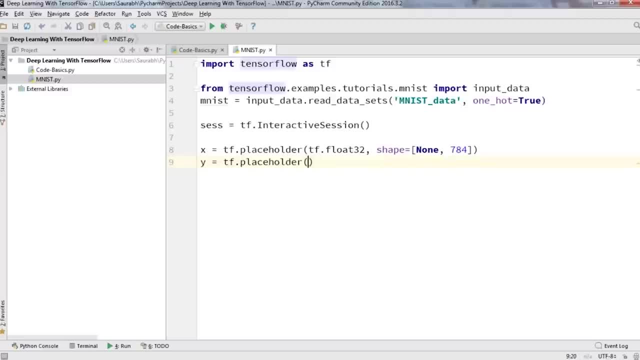 or you can say the desired output placeholder, and I'm going to type in here TF, dot, float 32, and I'm going to define the shape, which will be none comma 10, because we have 10 classes. and similarly, Y is also a 2D array where each row is one hot 10 dimensional vector indicating 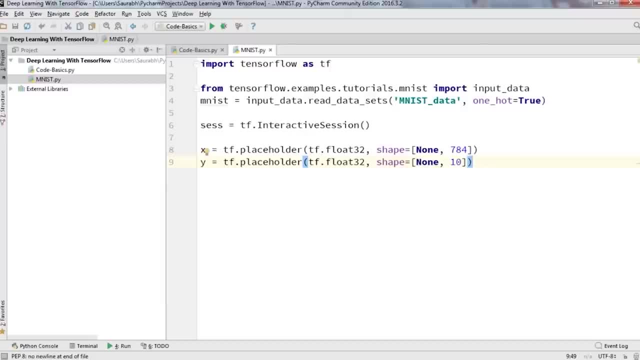 which digit class the corresponding MNIST image belongs to. and now next step is to define weight and biases for our model, like we have done in the previous example. So we could imagine treating these like additional inputs, but tensorflow has even a better way to handle them and what it is. 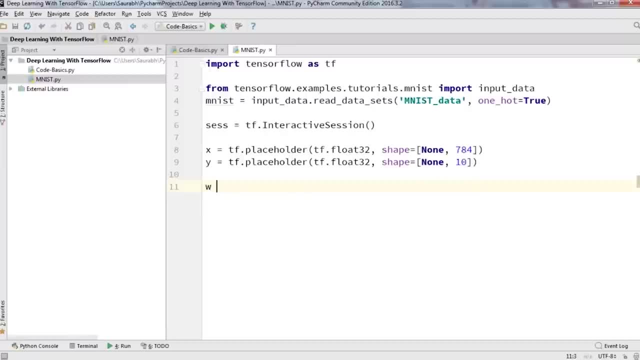 It is nothing but variables. So let us go ahead and do that. I'm going to type in here W TF, dot, variable, TF, dot zeros. I'm going to initialize it to zeros and the shape will be a 784 comma 10.. 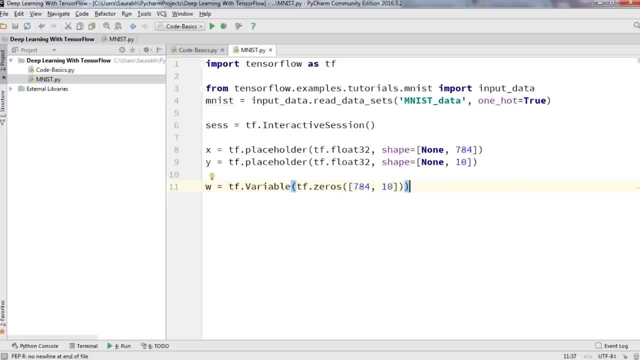 So it's like 28 cross, 28 pixels and a 10 classes. Similarly, when I talk about bias, so it will be TF dot variable, TF dot zeros. initialize it to zeros and the shape will be 10.. We pass the initial value for each parameter in the call to TF dot variable. 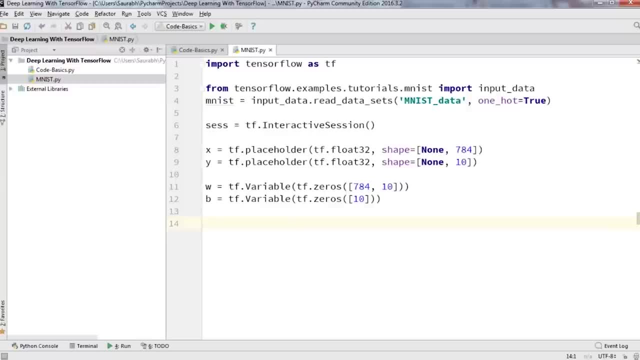 Now over here, as we can see that we initialize both W and B as tensors full of zeros, and W is a 784 cross 10 matrix because we have 784 input features and 10 outputs. and when I talk about bias B, it is a 10 dimensional vector because we have 10 classes. 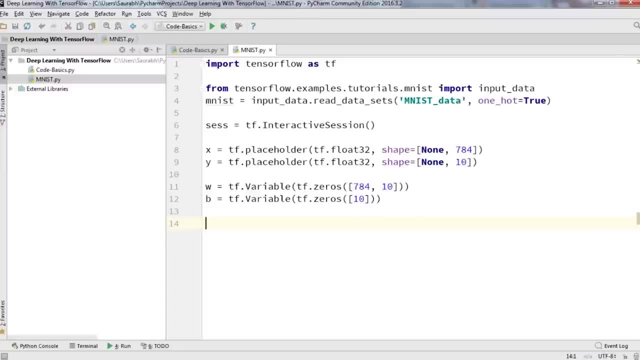 And we have learned that before we can use variables in a session, We need to first initialize it. So we're going to type it here: It says a dot run, and after that I'm going to type in TF- dot. global underscore variables. 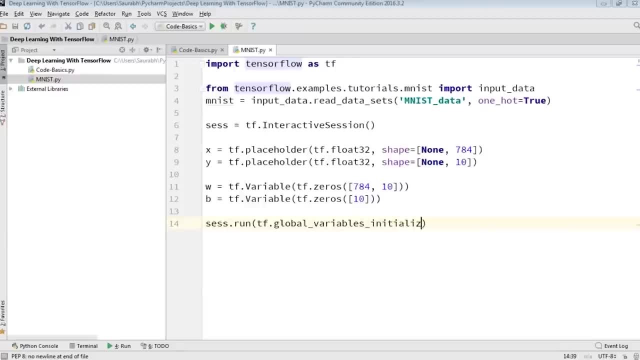 Underscore initializer. All right, so we have initialized all the variables. So our next task is to predict the class and the loss function. So we can now implement a regression model. It takes only one line. We multiply the vectorized input image X by the weight matrix W and add the bias. 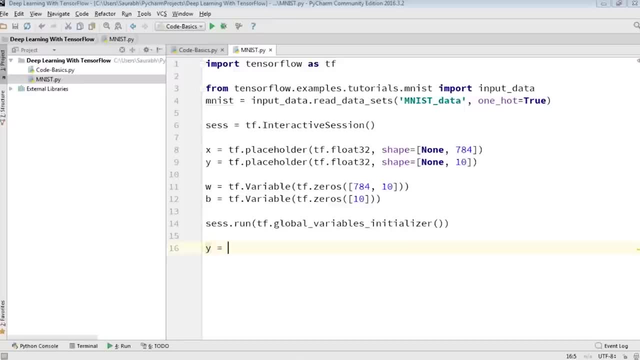 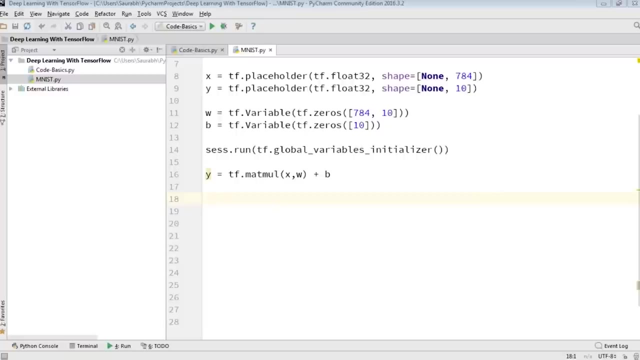 So for that I'm just going to type in here: Y equal to TF, dot matma, That is nothing but matrix multiplication X, comma, W plus B. All right, so now we can specify a loss function very easily. So the loss indicates how bad the model's prediction was. on single example. 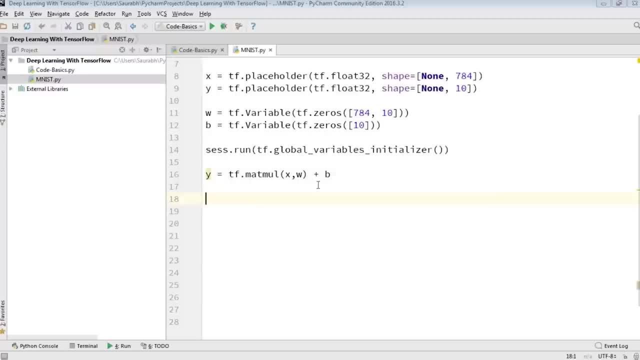 We try to minimize that while training across all the examples. So now we can specify a loss function. now, loss indicates how bad the model's prediction was on a single example And we try to minimize that while training across all the examples. Now, here our loss function will be cross entropy, or you can say the difference between the actual output and the predicted output. 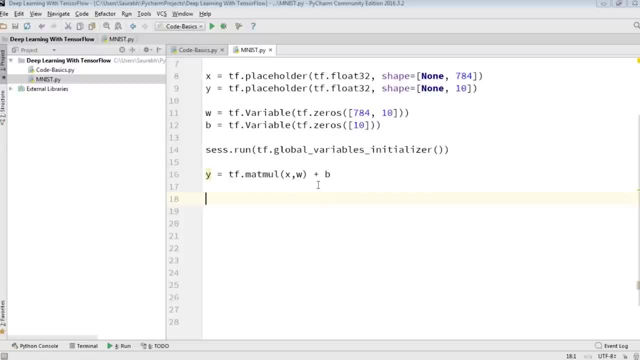 So for that, what I'm going to do, I'm going to you make use of softmax cross entropy function. So here the loss will be the difference between the target output and the actual output. So, for that, what I'm going to do is I'm just going to type in here a variable name. 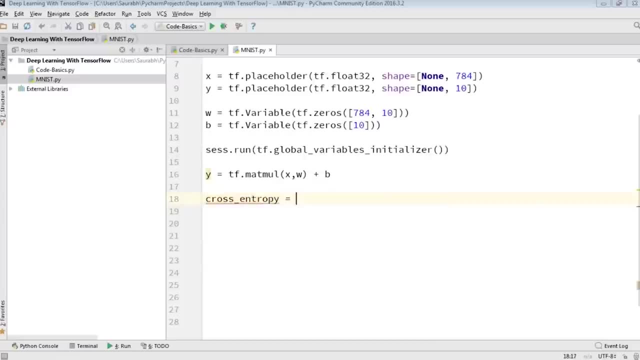 I'm going to name it as cross entropy, And, yeah, entropy equals to TF, dot, reduce, underscore, mean. And then just type in here Let me just enter the next line: TF, dot, NN, dot, softmax, underscore, cross entropy with logits. And now over here I'm going to type in first our target output, which will be labels: equals to Y comma, our actual output. 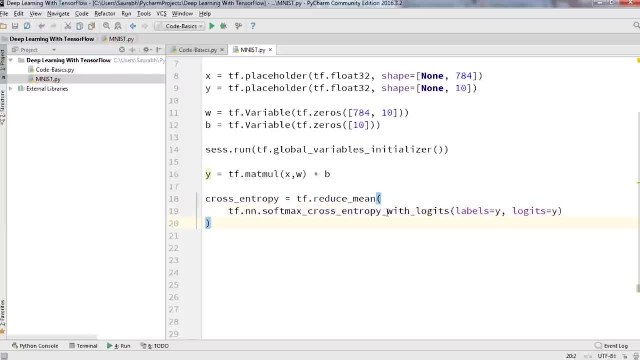 So it'll be. logits is equals to Y. That's all So over here. let me just give you a brief idea of what is happening. So labels is equals to Y means that this is our target output and this is the actual output. 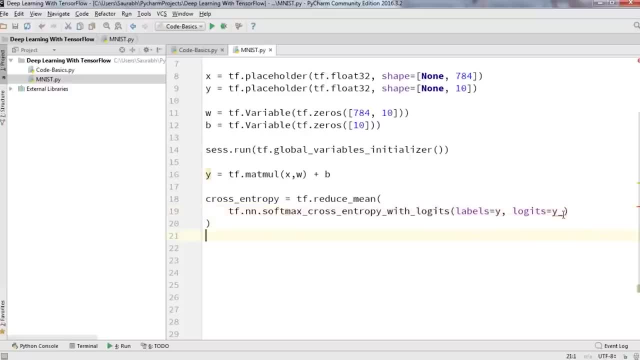 So it will be, will name it as Y underscore, And so what exactly is happening? It will calculate the difference between the target output and for the actual output. for all the examples, Then it is going to sum all of them and then find out the mean. 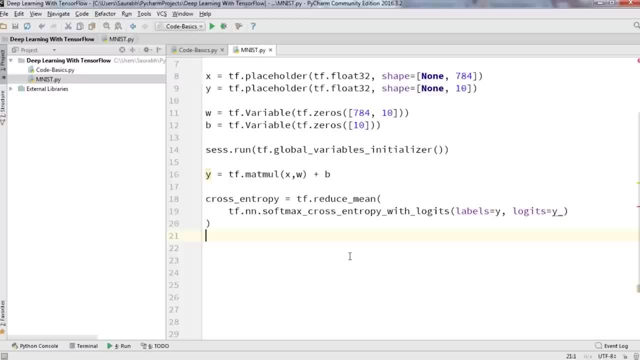 So this is what, basically, this cross entropy variable will do. Now that we have defined our model and training loss function, It is straightforward to train using TensorFlow. Now we need to train our model, So TensorFlow has a wide variety of built-in optimization algorithms, as I've told you earlier as well. 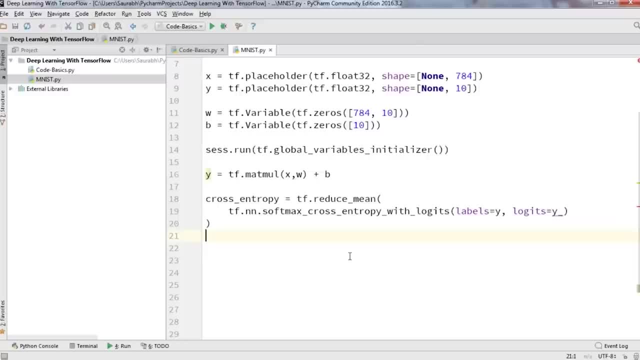 And for this example we'll use steepest gradient descent with a length of about 0.5 to descend the cross entropy. So basically we're going to use a 0.5 learning rate or you can say the step length. So for that I'm going to type in here: train underscore, step equal to TF, dot, train dot gradient descent. 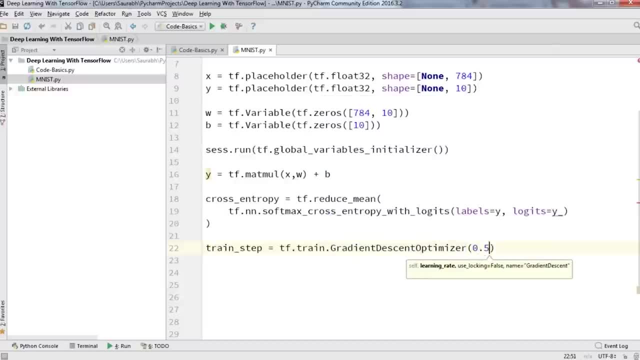 Minimizer, and the step will be 0.5, and minimize the loss, So minimize cross entropy. That's it. So what this one line basically will do: it will minimize the cross entropy, which is nothing but the loss function that we have defined. now in the next step, 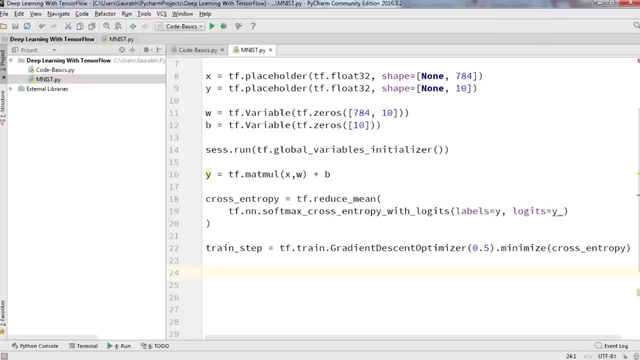 What we are going to do. We are going to load hundred training examples in each training iteration. So each time the training iteration happens, it will take hundred examples. We then run the train underscore step operation, which is nothing but to reduce The error using feed underscore dict. 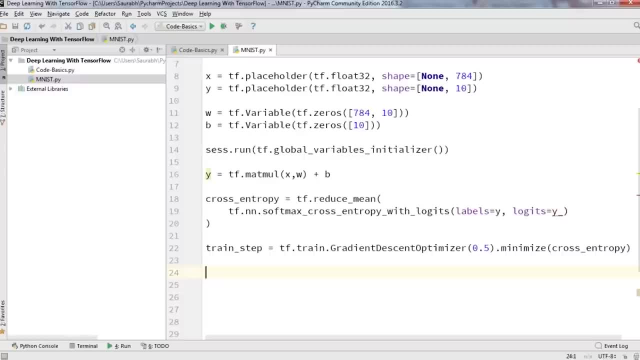 which is nothing, but we are going to feed the real values to our placeholder. Why now? next, what we are going to do? We're going to load a hundred training examples in each training iterations, which means that for each iteration will take hundred training examples. 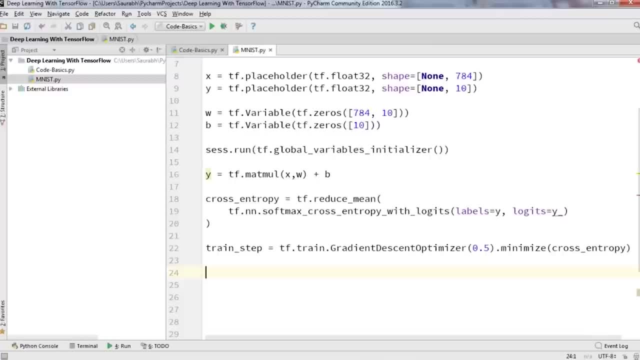 and will run the train underscore step operation, which is nothing but the optimizer. here And after that we are going to use a feed underscore dict to replace the placeholder tensors X and Y with the training examples. So basically, X will contain the input images and Y will contain the actual output. 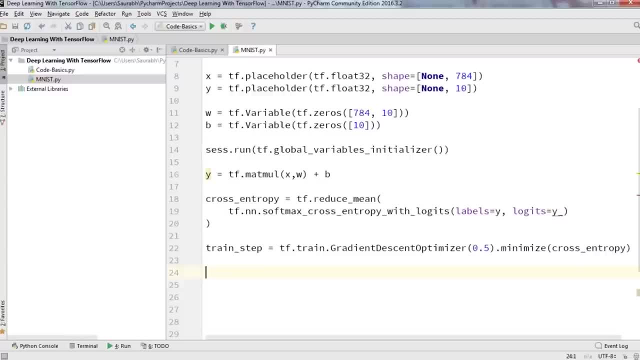 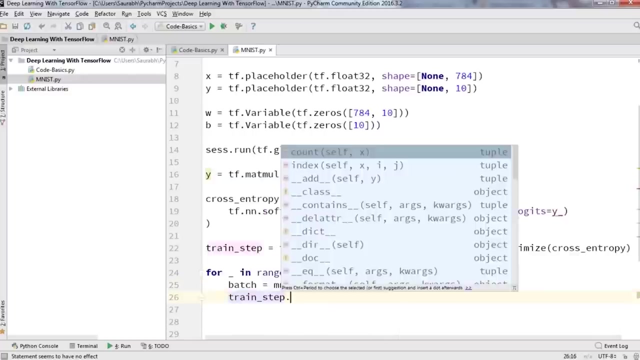 Or you can see the desired outputs for that I'm going to type in here for underscore in range: thousand Batch equals to MNIST dot train dot. next underscore: batch: Hundred train. underscore: step dot run. and I'm going to feed in the values to X and Y: variable feed. 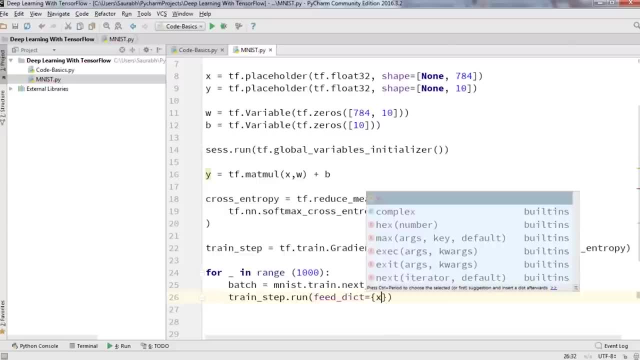 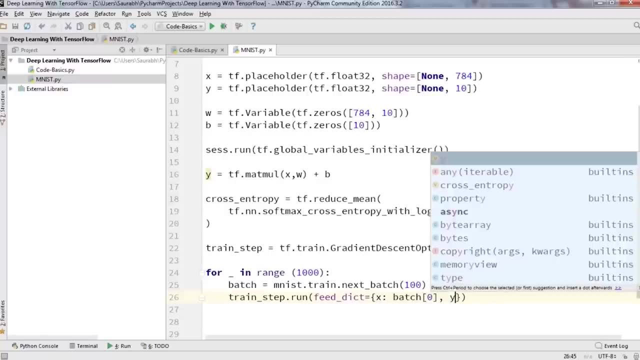 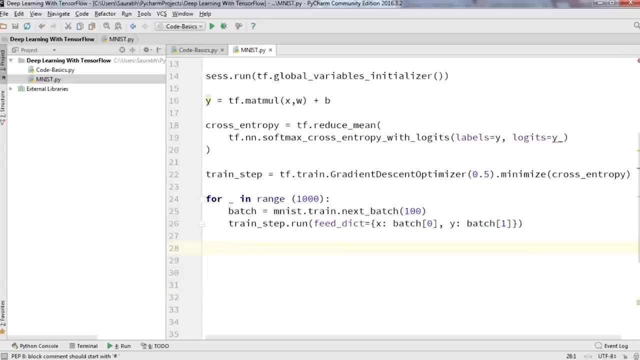 I'm going to type in here for underscore dict equal to X colon, batch zero. comma: Y colon, batch one. That's it. Now we need to evaluate our model, We need to figure out how well our model is doing, and for that I'm going to make use of TF dot argmax function. 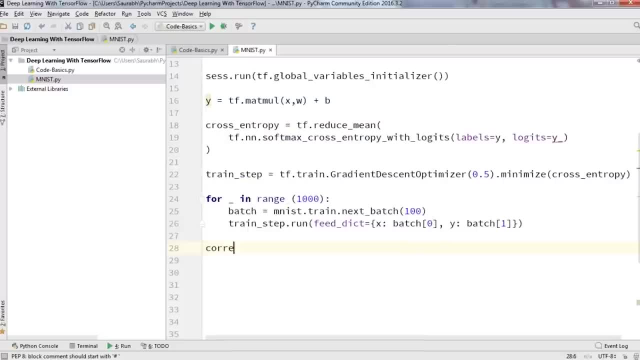 Now this TF dot argmax function. Let me tell you how it works. first I'm going to type in here correct underscore: prediction Equals to our TF dot. equal TF dot- argmax Y underscore comma 1 comma. TF dot- argmax Y, comma 1.. 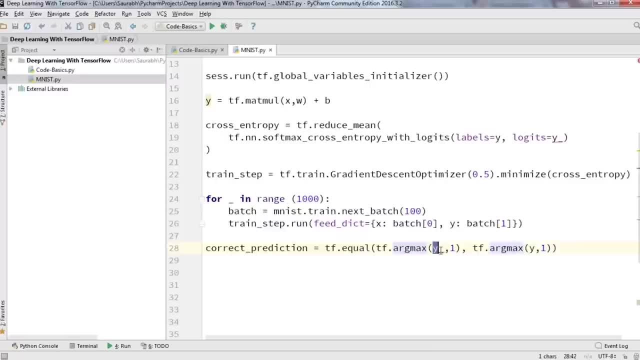 So basically, this TF dot argmax, Y underscore comma 1 is a label. our model things is most likely. for each input That means it is a predicted value, while TF dot argmax or Y comma 1 is a true label. It is there in our data set, present already and we know that it is true. 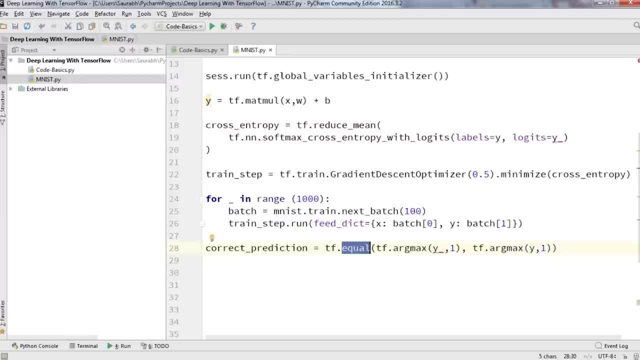 So what we are doing, we are using TF, dot equal function to check if our actual prediction matches the desired prediction. This is how it is working. So now what we're going to do: we're going to calculate the accuracy to determine what fraction are correct. 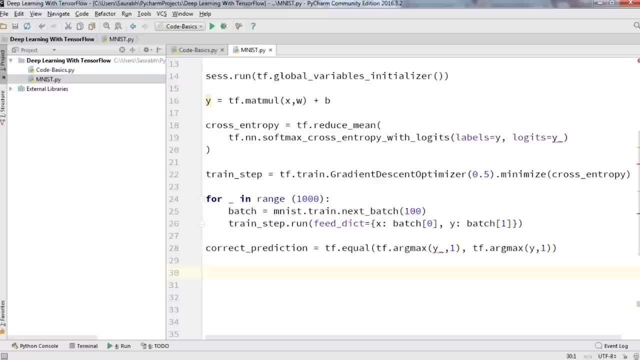 We cast a floating-point numbers and then take the mean, repeat. So now I'm going to define a variable for accuracy. So just going to type in: Accuracy equals to TF dot reduce underscore mean. TF dot cast correct underscore. prediction Cover a TF dot float 32 and what we can do. 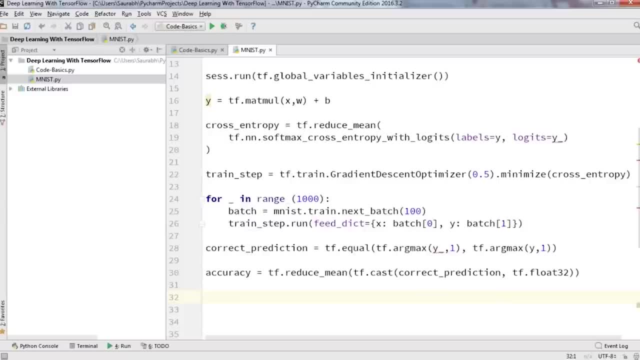 Finally, we can evaluate our accuracy on the test data, and this should give us accuracy of about 90%. So let us see if that happens. I'm going to type in here: print accuracy dot evaluate Eval feed. underscore dict Equal to X colon MNIST dot test dot images. comma Y colon: MNIST dot test dot labels. 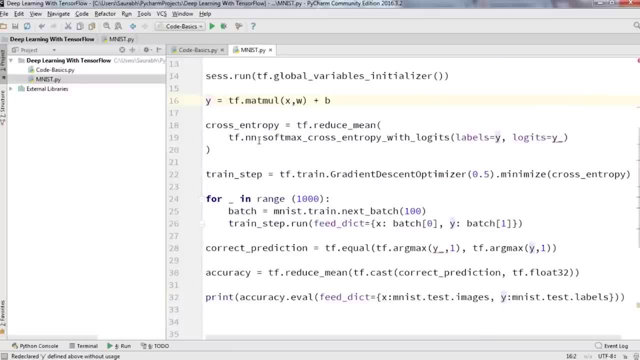 That's it, guys, and I've done a mistake here. instead of Y, it will be Y underscore, because this is our predicted value, not the actual value, And why we have considered as actual value and this Y underscore will be our predicted values. This is the mistake that I made. 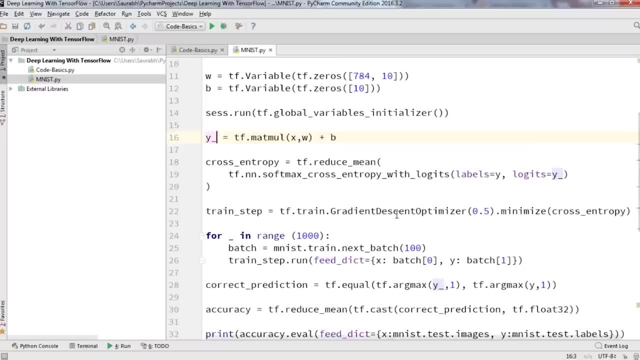 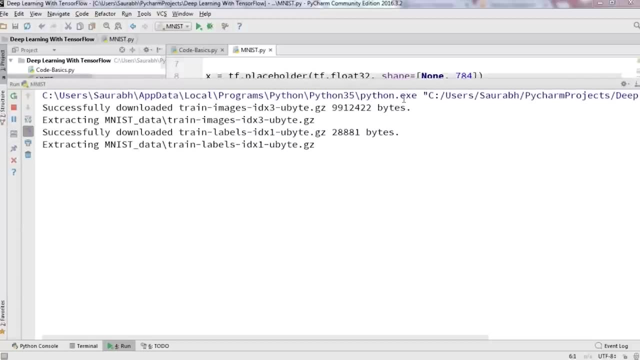 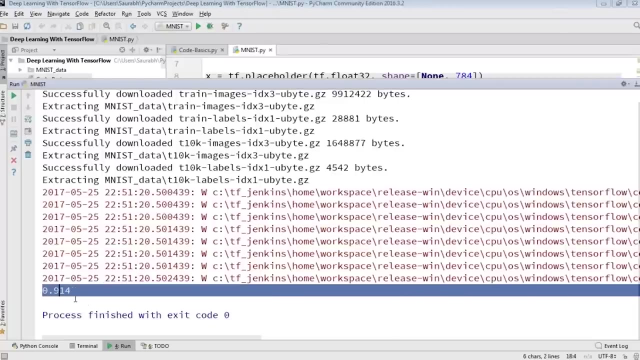 So, yeah, now I think the code looks pretty fine to me and we can go ahead and run this. Let us see what happens when we run this. So, guys, it is complete now, and this is the accuracy of a model, which is 91.4%, and which is pretty bad, though, when you talk about a data set like MNIST. 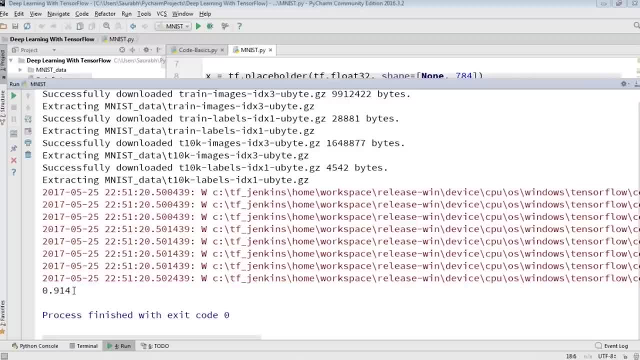 But, yeah, with a single layer, which is very, very good. So we have got an accuracy of around 92% on the MNIST data set, which means that whatever the test data sets were there, that is like 10,000 test images. So on those test images, whatever the prediction our model has made, are 91.4% correct. 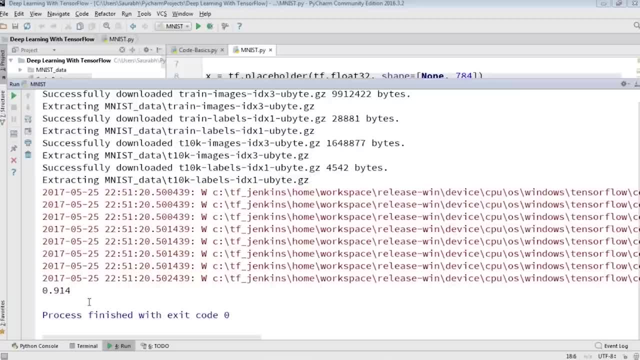 So, guys, let me just give you a quick recap of all the things we have discussed. So first we saw what exactly is deep learning and how it is different from the traditional machine learning. then we understood the motivation behind deep learning, which is nothing but your. 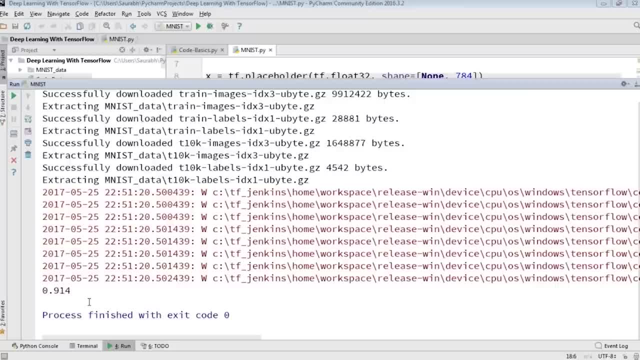 A brain cells, which are called neuron. then we understood the importance of why we need artificial neurons. and then we took the example of artificial neuron, which is called a perception, and we are looking at a couple of examples in which we implemented the and gate, we performed image classification on the MNIST data sets. 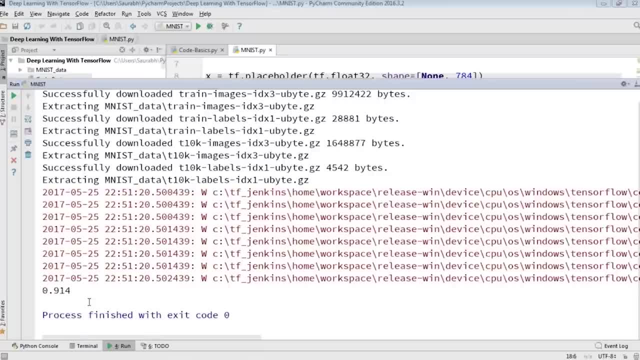 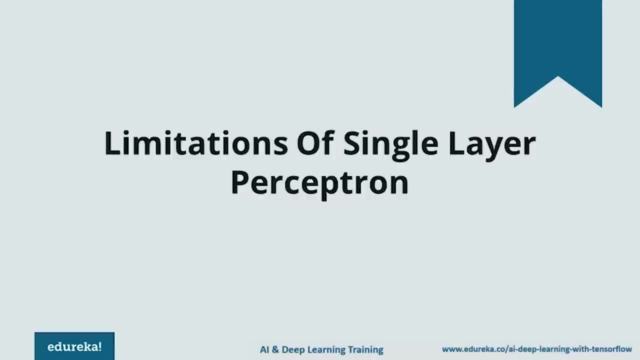 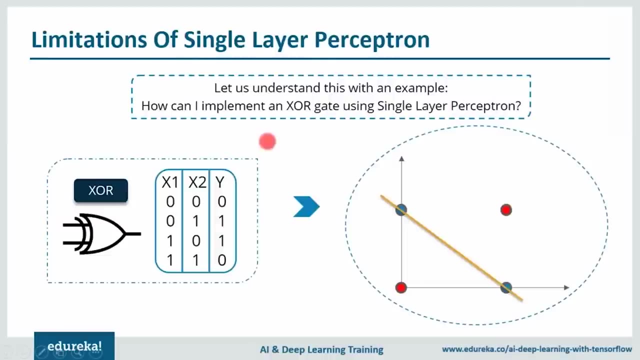 which is nothing but handwritten images between 0 to 9, and we also implemented a couple of examples in order to understand what our placeholders, variables and constants. So now there are certain limitations of single layer perception. Let us understand That. so, in order to understand that, we'll take an example. 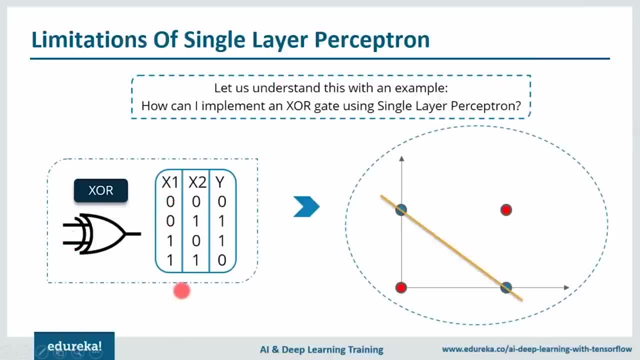 So we have an XOR gate here and this is a truth table. So, according to this truth table, if any one of the input is high, then the output is high, and if both the inputs are low, output is low, and if both the inputs are high, output is low. 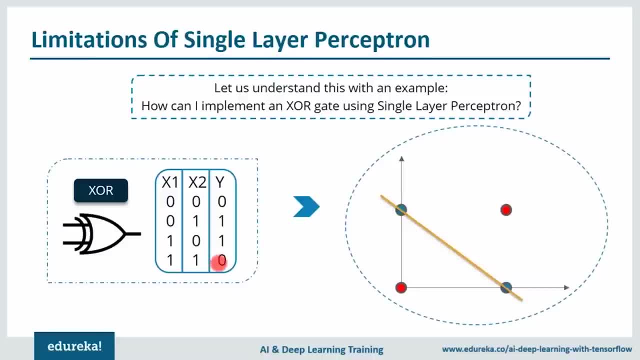 So how can you classify the high and the low outputs with a single line? Definitely you can't, if you see the points. So one point is here, one is here, here and here, and which? these two points are high outputs and these two are low. 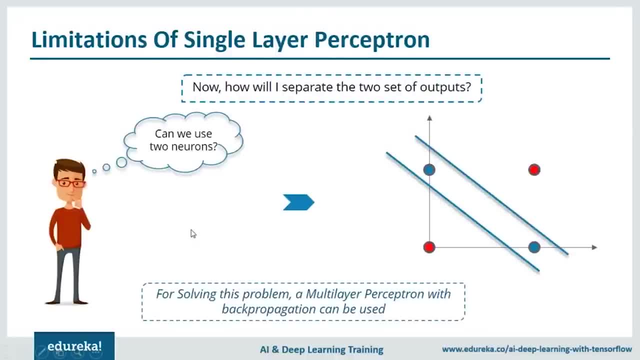 So how can you classify with a single line? Definitely you can't. So now, what's the answer to this? What if we use multiple neurons? using multiple neurons, We can have two lines that can separate it. Now we can solve this problem if we have multiple neurons. 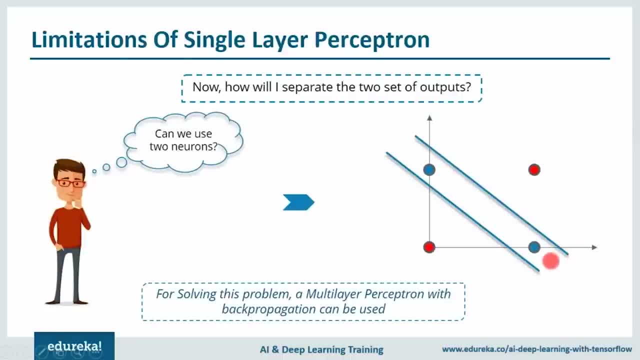 So if we use two neurons, we can have two lines and that can actually separate the high outputs as well as the low outputs. So this is where we use multi-layer perception with back propagation. So what are multi-layer perception, multi-layer perceptions? They have the same structure. 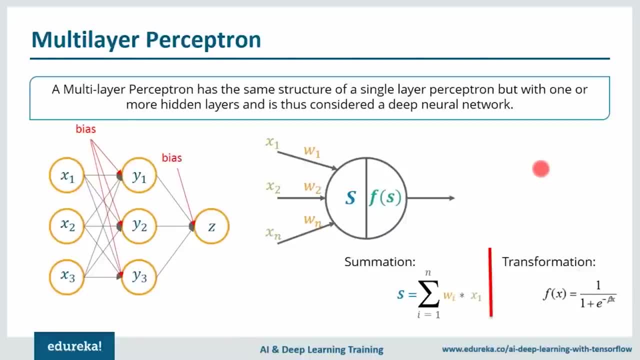 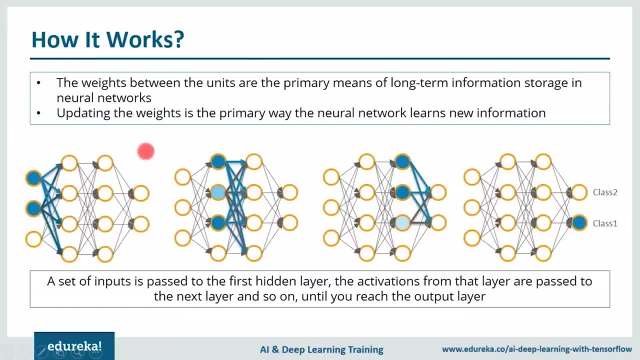 Like the single layer perception. The only difference is they have more than one hidden layer. So let me explain it to you with an example. So this is how a typical multi-layer perception looks like. So we have input layer, We have two hidden layers and we have one output layer as well. 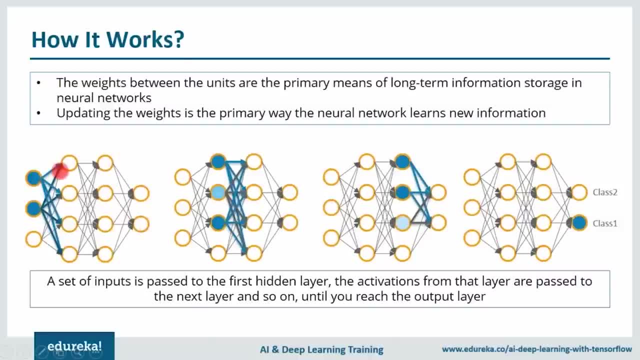 Now, typically, each of these input layers are connected to the next hidden layer. Each neuron is connected to the next neuron present at the adjacent layer, but the neurons of the same layer are not connected to each other. Now what happens? a set of inputs are passed. 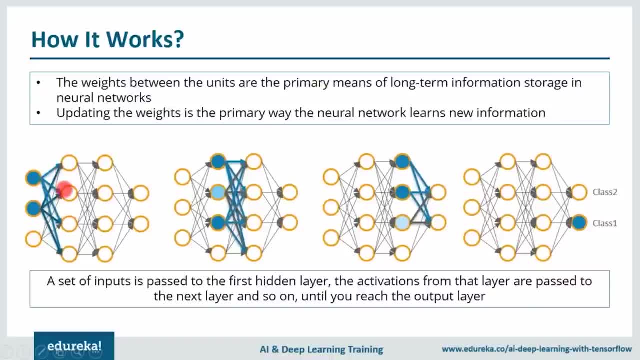 to these input layers and the output of this input layer will be passed to the first hidden layer. Then, after activation function of the first hidden layer, the output will be passed to the next hidden layer as the input and similarly. finally, we get the output. 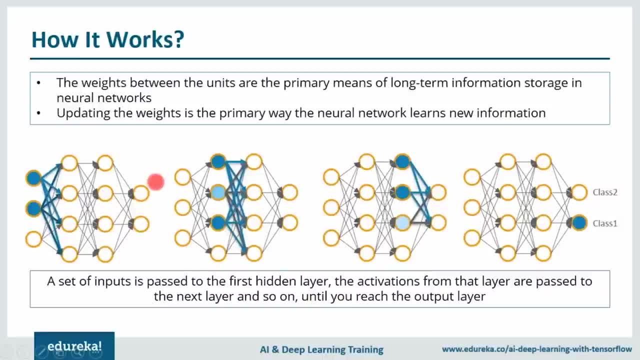 Now you must be thinking how the model learns from here. So the, basically, the model learns by updating the weights, and the algorithm that it uses is called back propagation. So the back propagation algorithm helps the model to learn and update the weights in order to increase the efficiency. 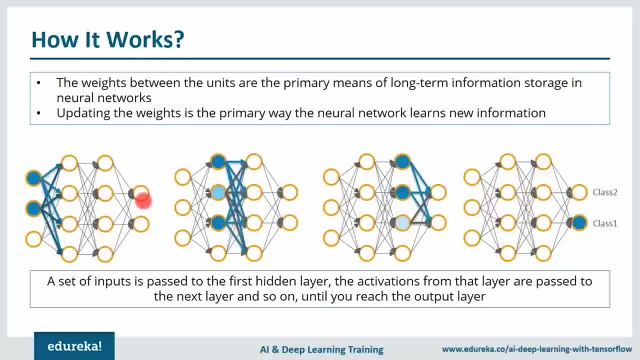 So basically, at this process of from input layer to the output layer is called a feed forward process and then, when we back propagate it in order to increase the efficiency or accuracy so that we can update the weights, that is called as a back propagation. We'll understand back propagation in more detail. 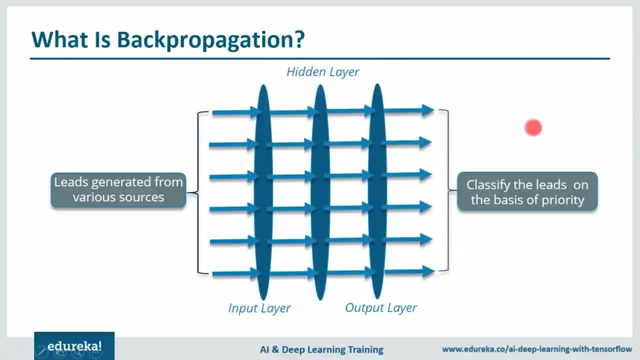 So what is back propagation? Now let us understand this with an example. So we'll take the inputs as the leads generated from various sources, and my aim is to classify the leads on the basis of the priority, So there might be certain leads which won't make it that much difference to me. 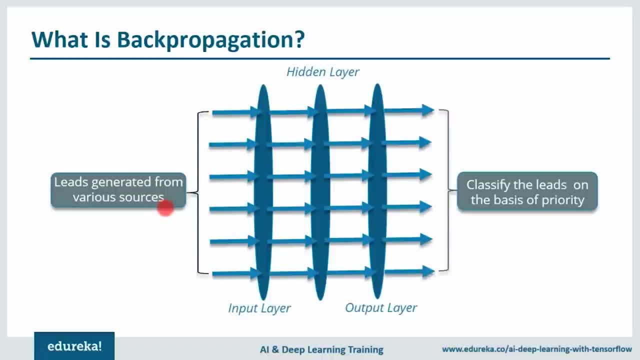 whereas compared to the other leads. So in that case, I need to make sure the leads which are important gets the highest amount of weight. How am I going to do that? first, We'll see the output that, accordingly, will calculate the error and, based on that error, 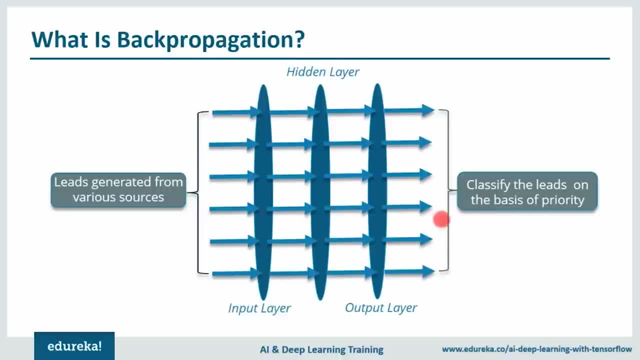 We are going to update the way, and this process is nothing but your back propagation. in a nutshell, I can say: right, although the algorithm is pretty complex, but yeah, this is basically what happens. So, in order to classify the leads in the basis of priorities, 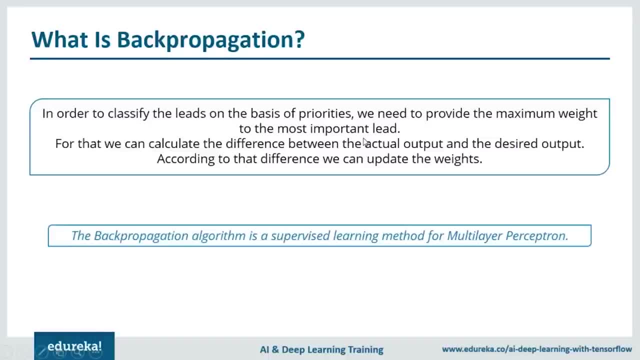 we need to provide the maximum weight to the most importantly. and how are we going to do that? We're going to compare the actual output and the desired output and according to the difference, we can update the weights. So what is back propagation? So back propagation is nothing but a supervised learning algorithm. 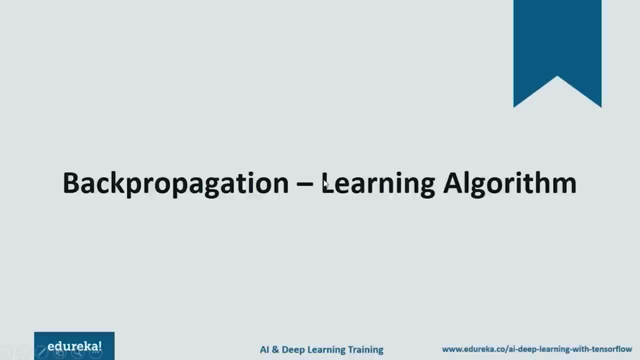 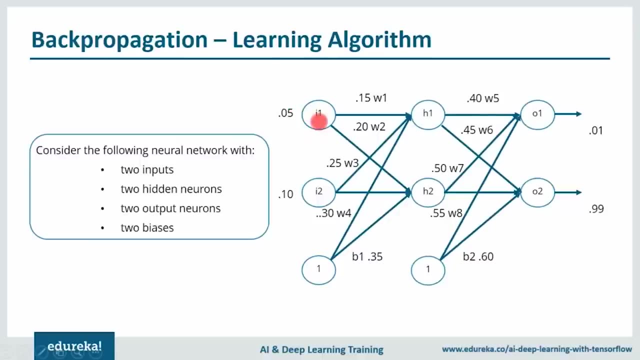 for multi-layer perceptron. Now let us understand what exactly is this algorithm. Let us understand this with an example that is there in front of your screen. So these two are our input neurons, These two are our hidden neurons and these two are our output neurons. 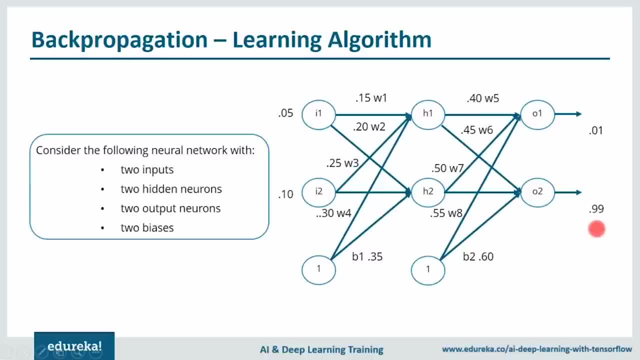 Now our aim is to get 0.01 and 0.99 as our output and at the same time we have inputs as 0.05. And 0.10. initially, we take the weights as we can see it here. 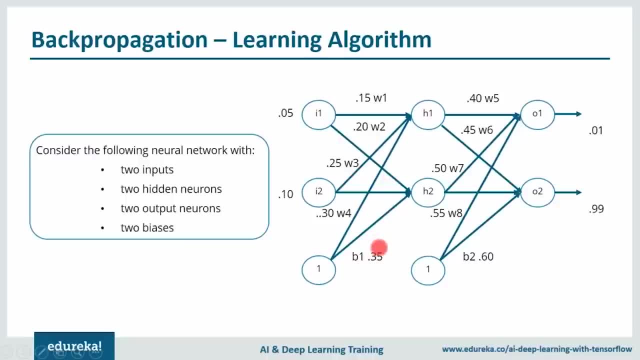 So 0.15 w1, 0.20 w2.. So these are the weights, plus we have two biases as well. Now what we need to do is we need to make sure that we have weights in such a way that we get output as 0.01 and 0.99.. 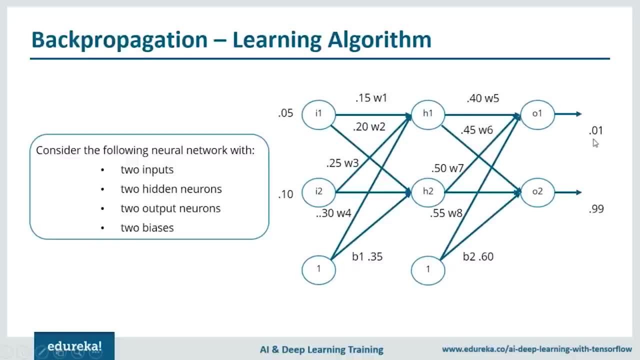 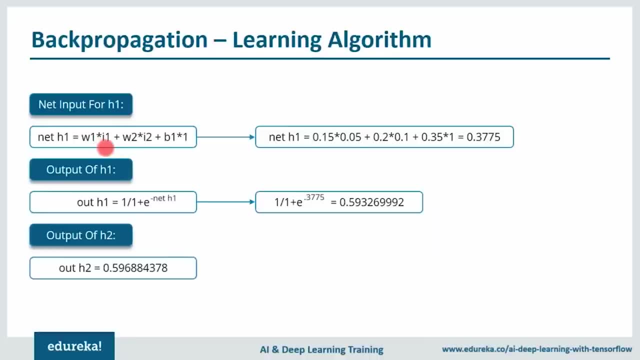 But let us see if we get that same output. when we provide these kind of weights, The net input for this particular H1 will be what it will be: w1 into I1.. That is the first input, plus w2 into I2, plus b1 into 1, which gives us the answer as 0.3775. 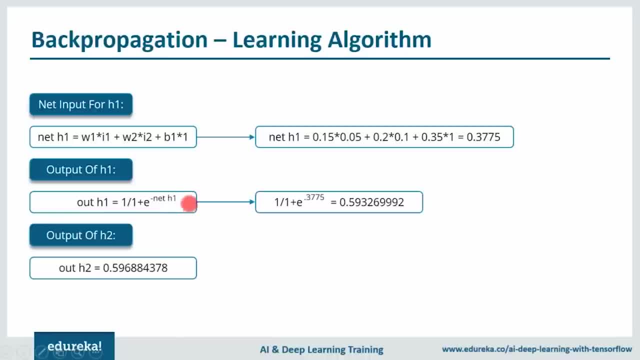 Similarly, the output for H1 will be nothing but the activation function, the output and after the activation function, and we are using her sigmoid function because our brain also uses a sigmoid functions. That's what we believe in and, at the same time, it is easily differentiable. 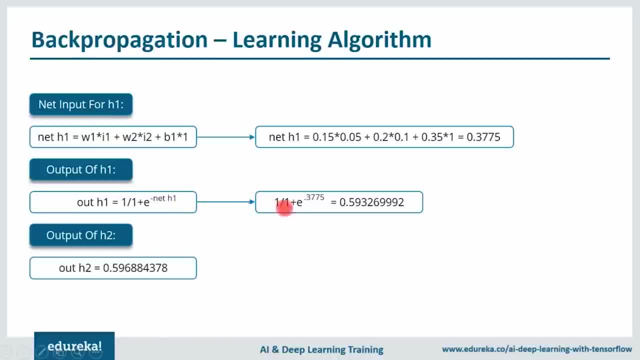 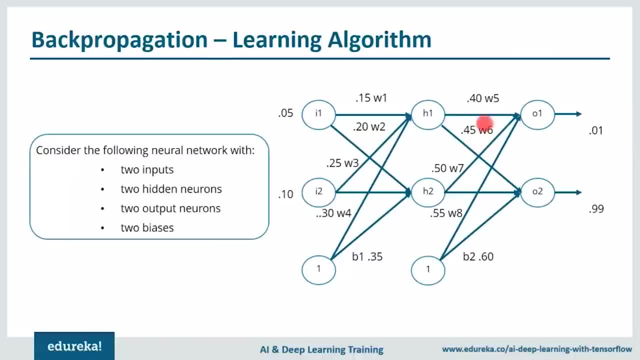 And if you differentiate it twice, you get the same number. So the output of H1 will be 0.59 something. So let me go back. So the- yeah, the output of this particular H1 will be 0.59 something. then we're going to calculate the output of H2 as well. 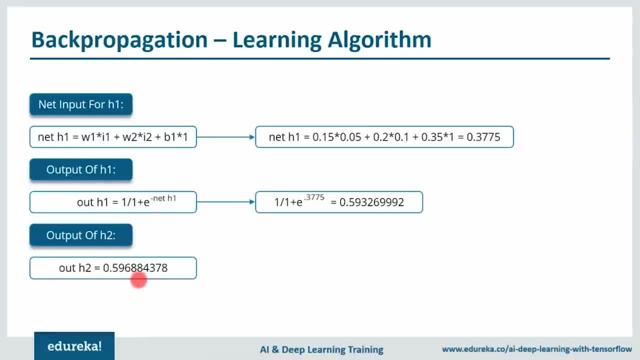 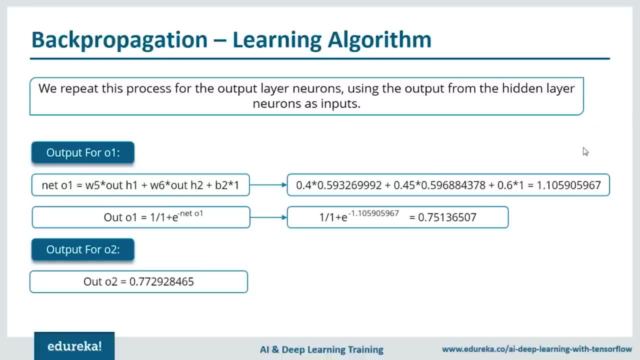 Similarly and we get the output as point five, nine, six, double eight, four, three, seven, eight. next up, We are going to repeat the process for the output layer neurons as well. So for the output layer the net input will be w5 into out of H1, w6 into out of H2 plus b2.. 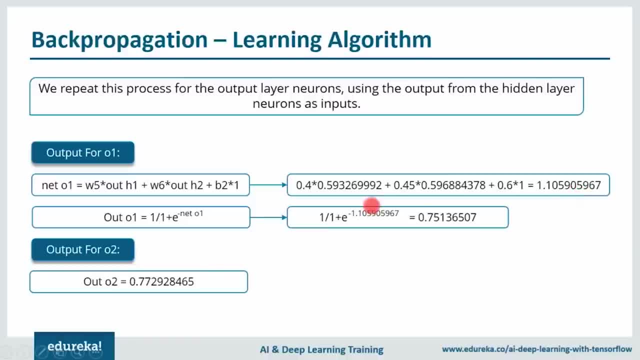 That is a bias. So we get the output somewhere like this, and then the net output for out 01 will be after the activation function, which will be 0.751.. Similarly, the output for O2 will be 0.77.. Now, if you notice that this is not the desired output, 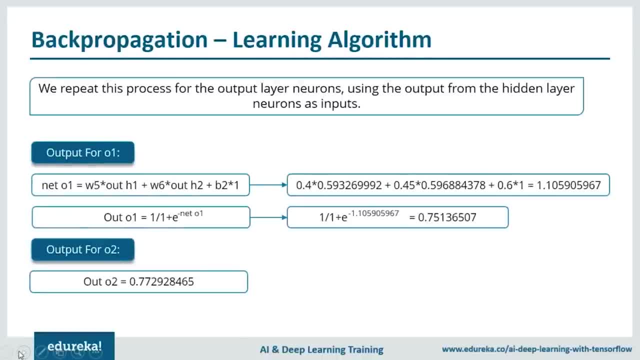 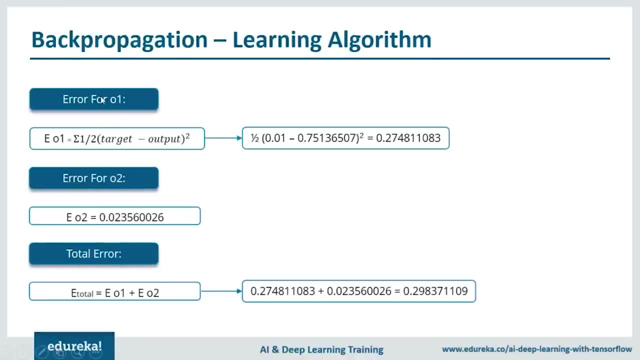 our desired output was 0.01 and 0.99.. What we got instead? we got 0.75 and 0.77.. So what we need to do, we need to update the weight. So for that, we're going to calculate the error now. error. 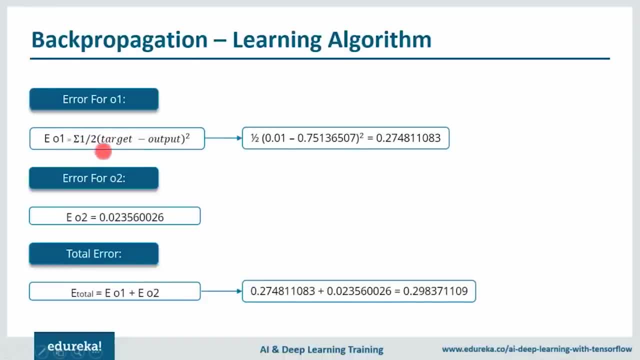 for output, O1 is nothing but the Sigma of 1 by 2 target minus output. whole square target is nothing but your desired output and output is your actual output. So your error of output for O1 neuron will be 0.278. similarly for O2 will be 0.023.. 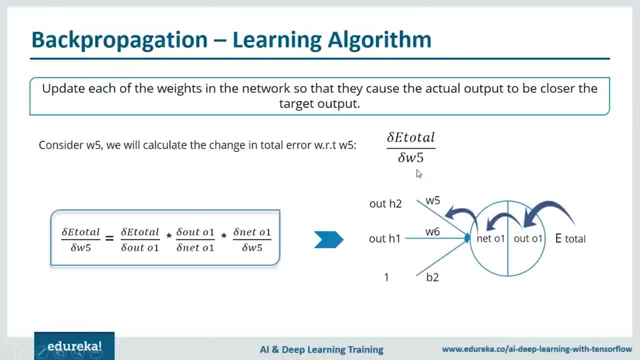 So the total error comes down to 0.29, something next up We need to update the weight so as to decrease this error. Now what we're going to do? we're going to first calculate the change in total error with respect to any of the random weight. will take w5. 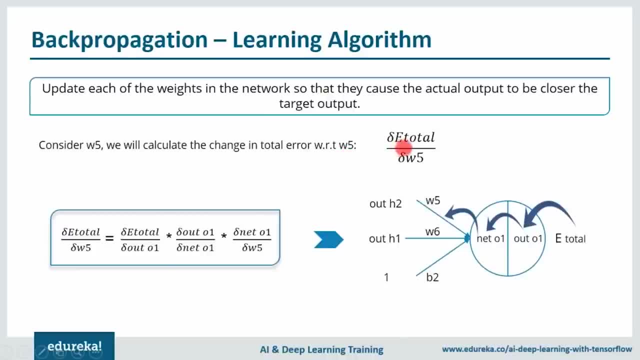 for example, just to show you. so we're going to calculate the change in the total error when we change with respect to the weight w5.. So we're going to apply a chain rule here. So using partial derivative, We're going to calculate e total by Delta of auto 1 into Delta of auto 1. 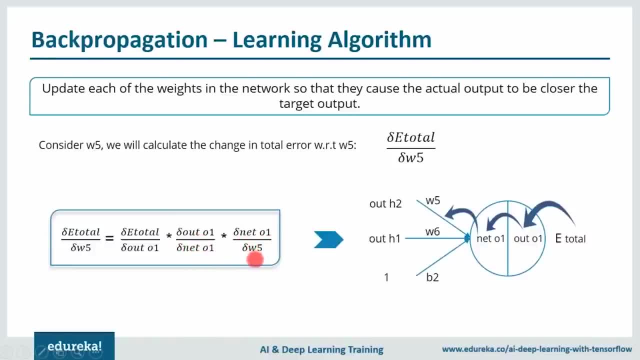 by Delta of net O1, and then Delta of net O1 by Delta of w5, as you can see it from this particular example as well. e total. change in e total with respect to auto 1. change in auto 1 with respect to net O1. 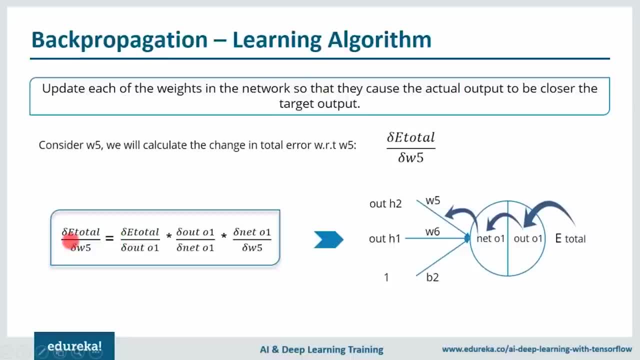 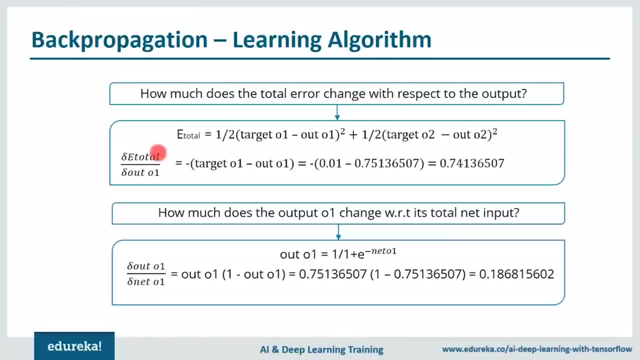 and change in net O1 with respect to w5.. We're going to multiply that and we're going to get this particular term and let us see how we do that. So how much the total error change with respect to the output e total by e out one we're going to calculate it came around 0.741.. 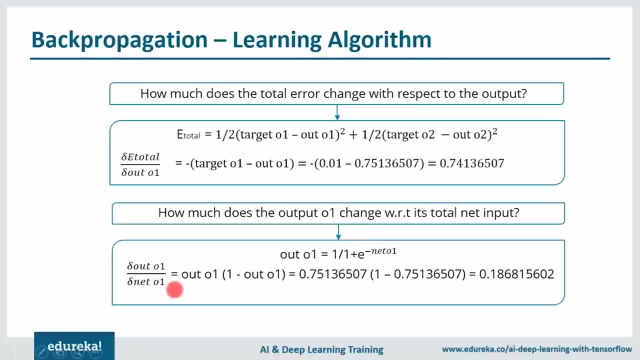 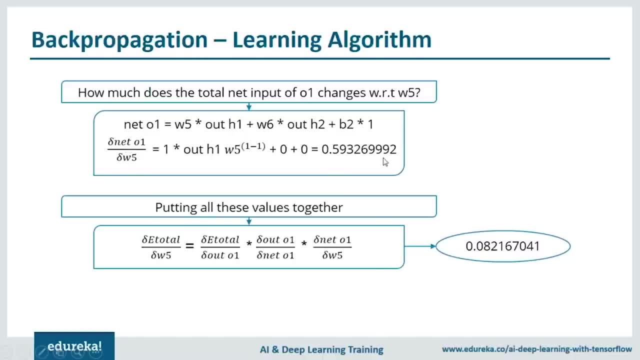 Similarly, we're going to calculate how much this output O1 change with respect to the net output, and we get this. after that We're going to calculate it for net output change with respect to w5.. Also, we got this and then, finally, what we did, we put all these values together. 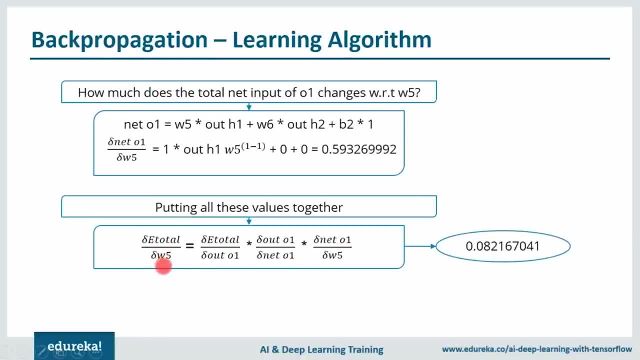 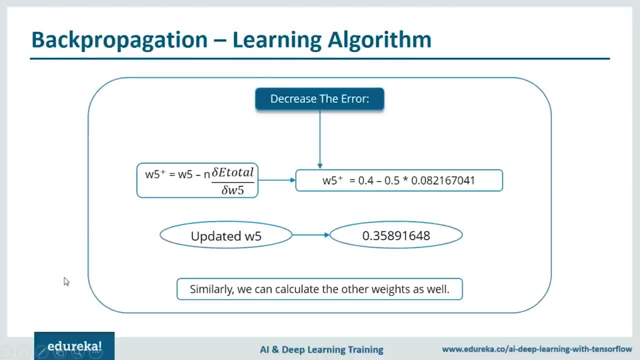 and we found out to change in the error with respect to the change in weight w5, which came to up around 0.082167041.. Now is the time to update the weight. So how we can update the weight? first thing we need to do is we need to follow this formula. 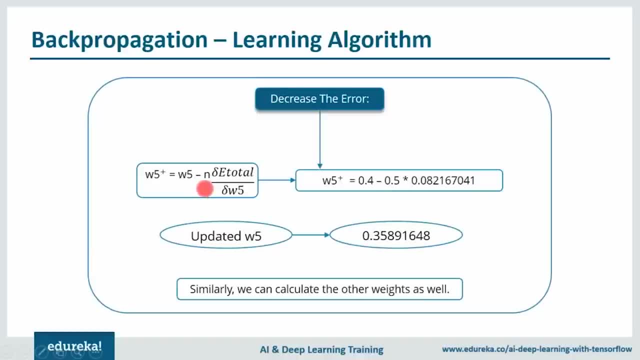 W5 plus is nothing but the updated weight, which is equal to w5 minus the learning rate into Delta of e, total by Delta of w5.. So which came to around a point three, five, eight, nine, one, six, four, eight. similarly we can calculate the other weights as well. 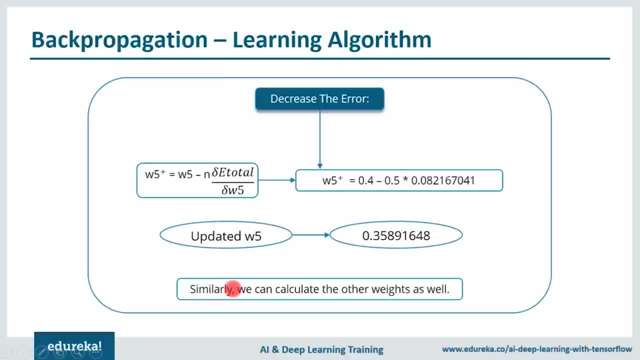 So we're going to repeat the same process and we're going to calculate the other weights as well. Then again we're going to see how much is the loss, if still the loss prevails that we're going to repeat the same back propagation learning algorithm again. 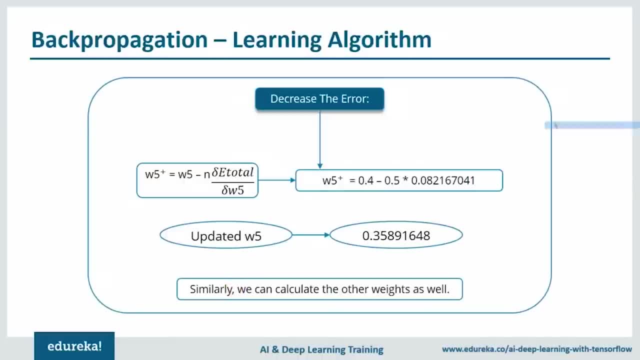 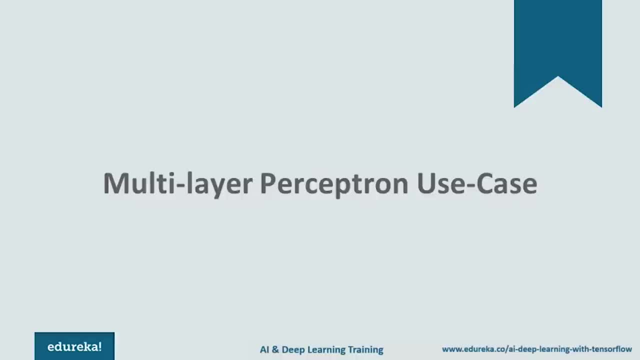 for all the ways. so this process will keep on repeating. So this is how back propagation actually works. So now what I'm going to do? I'm going to make use of the same MNIST data set and I'm going to increase the efficiency of that data set by 97 to 99%. 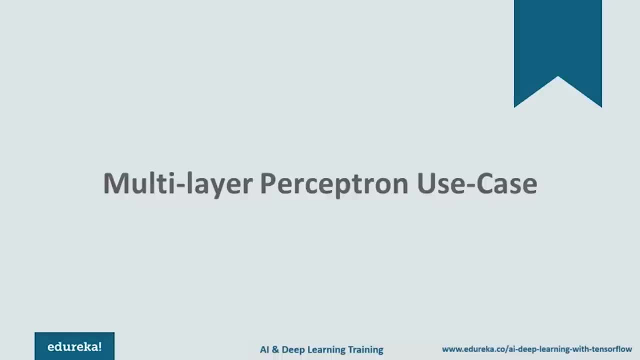 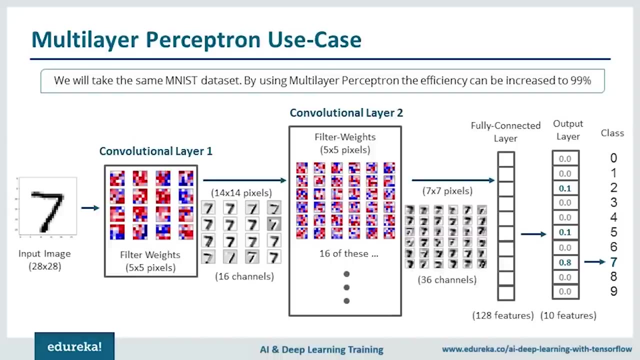 with the help of multi-layer perceptron. So, guys, let us go ahead with that. So, guys, as I've told you earlier, is where we are going to use the same MNIST data set which we have used in the single layer perceptron. 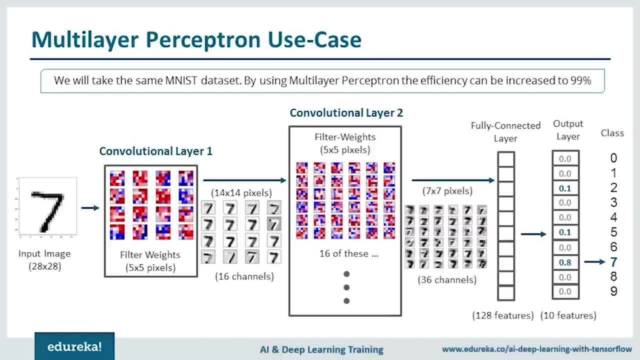 So I'm going to perform a classification using multi-layer convolutional networks. Now, what are convolutional networks? basically, these networks are used in order to classify images. So, basically, what I'm doing is I'm just trying to show you that, how we can increase the efficiency. 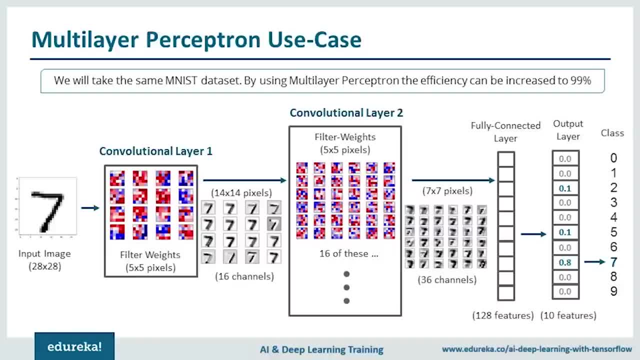 using the convolutional neural networks. I'm just giving you a general overview, or you can say a taste of how things work in convolutional neural networks. So we give an input image to this convolutional network, Then this input image is processed in the first convolutional layer using the filter weights. 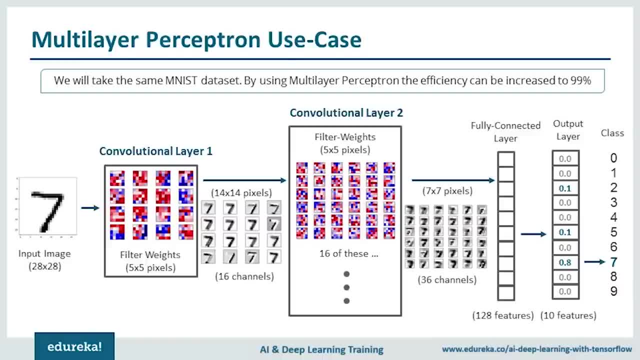 Now this result in 16 new images, one for each filter in the convolutional layer. The images are also down sampled, So the image resolution is decreased from 28 cross 28 to 14 cross 14.. Now these 16 smaller images and from the first convolutional layer are then processed. 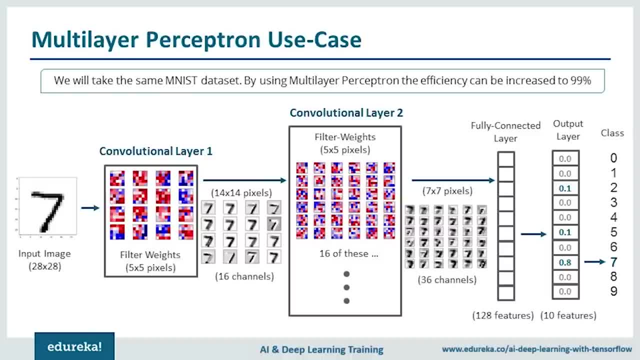 in the second convolutional layer. We need filter weights for each of these 16 channels and we need filter weights for each output channel of this layer. Now there are total 36 output channels. So there are total of 16 cross 36, equal to around 576 filters in the second convolutional layer. 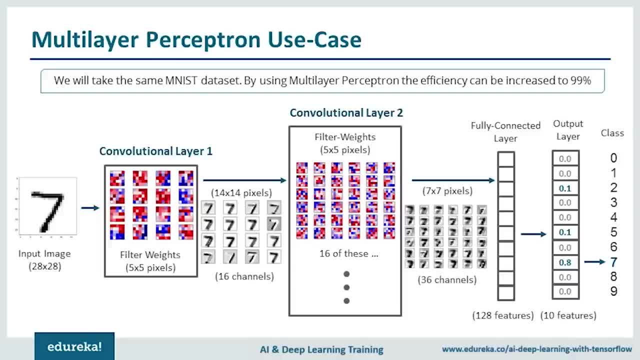 Now the resulting images are down sampled again to 7 cross 7 pixels. The output of the second convolutional layer is 36 images of 7 cross 7 pixels each. Now these are then flattened to a single vector of length: 7 cross, 7 cross 36,. 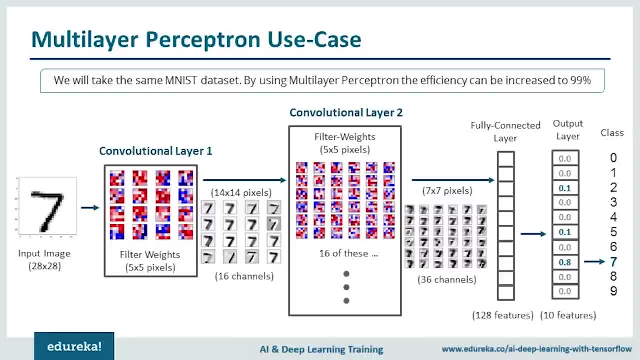 which is a 1764, which is used as the input to a fully connected layer with 128 neurons, and this feeds into another fully connected layer with 10 neurons, one for each of the classes, which is used to determine the class of the image, that is, which number is depicted in the image. 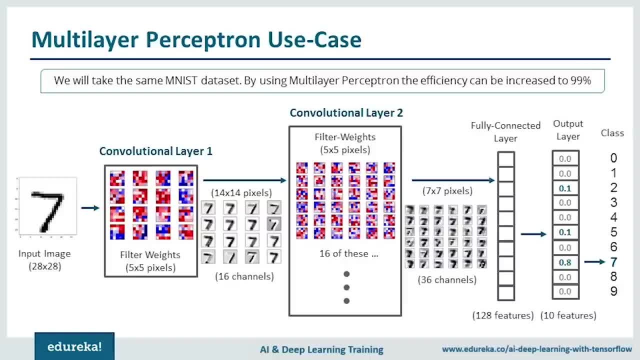 So whatever number that we provide in, so basically the output layer, or you can say the last layer, or the fully connected layer with 10 neurons, is used to determine the class or which digit is the input image of. now, the input image depicts the number 7. 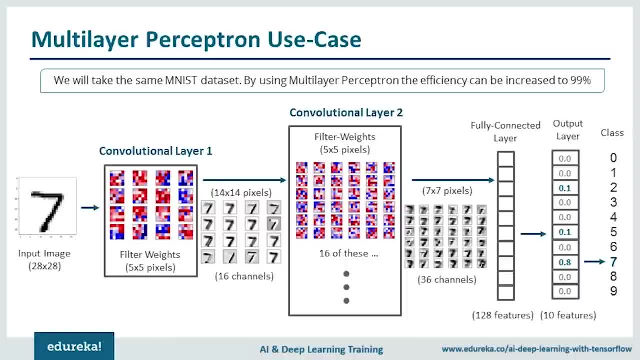 and the four copies of the images are shown here. So basically what happens? whatever filter we have in each layer, It will be present on the image pixels. So there will be a dot product of the filter and the image pixel behind that. so we'll get a dot product there. 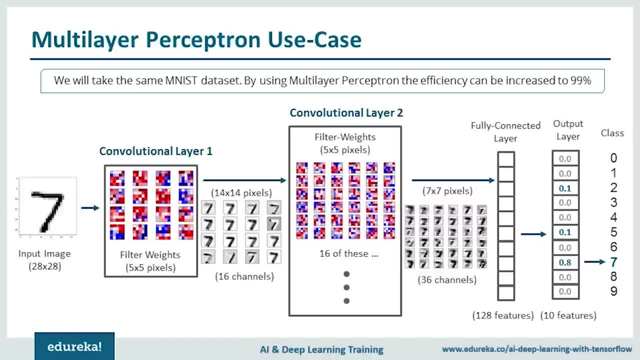 We are going to repeat that same process in each of these layers and for each of these layers and for each of these images, and we are calculating the dot product. So I hope you get the point. So let me just show you that we can increase the efficiency. 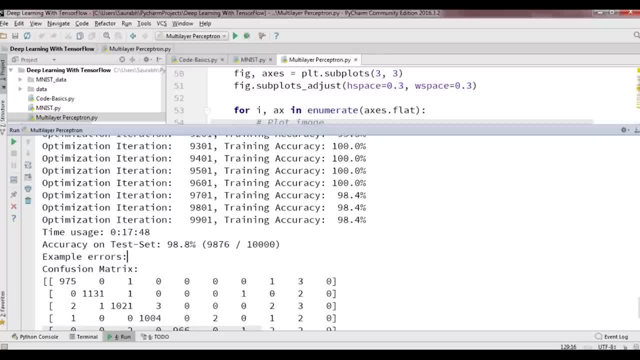 So I have already done the code and it will take time if I do it right now. So this is what the efficiency we ended up with. so it is 98.8%. So on the test sets, we had around 10,000 test samples. 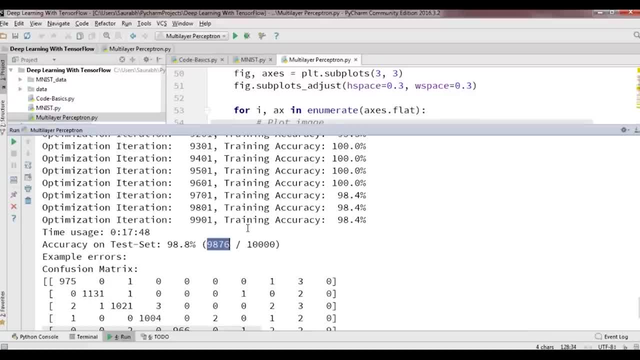 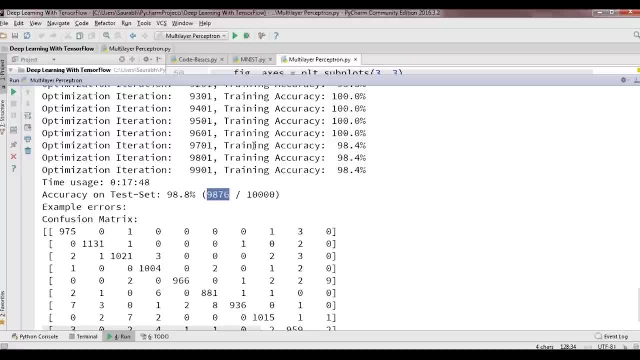 out of which we predicted 9876 correctly, So which is pretty good actually, if you see, so it because in the single layer perceptron example that we took, we were getting accuracy of around 92%, but here we are getting around 99%, which is actually very good. 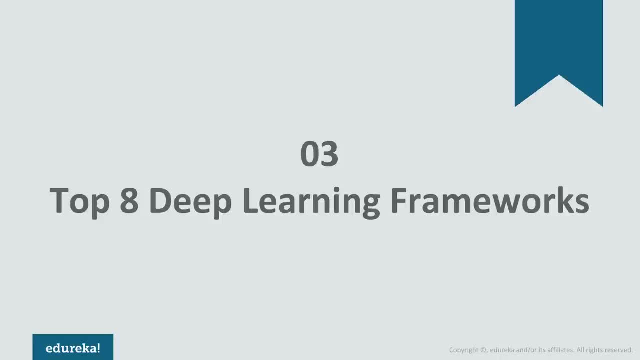 All right. In this session, let's have a look at the top 8 deep learning frameworks, which is very popular and widely used. this session is helpful for anyone who's considering to expand their knowledge about all the frameworks out there, or if you're just considering to build a career in deep learning. 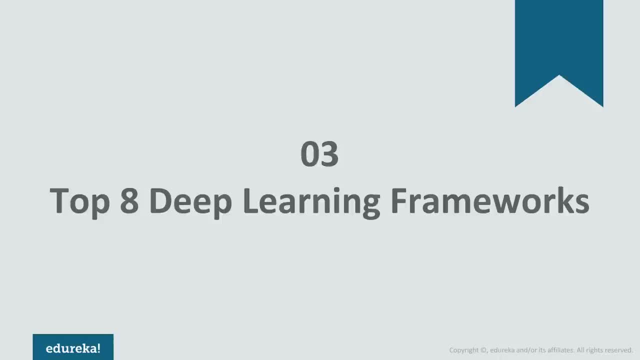 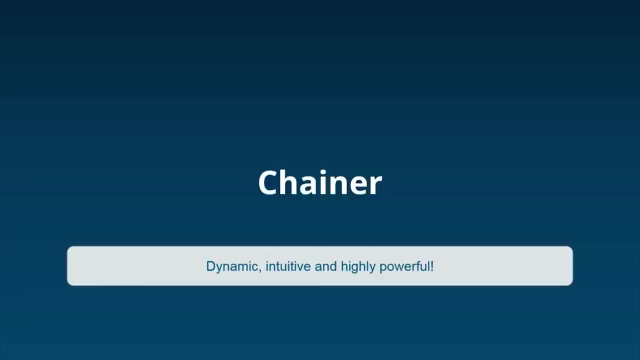 I have categorized the 8 frameworks in descending order of the rank, based on various factors such as efficiency, community and how easy it is to actually get started with each of these. without further ado, Let's dive into Chainer. It is the first one in this top 8 rundown. 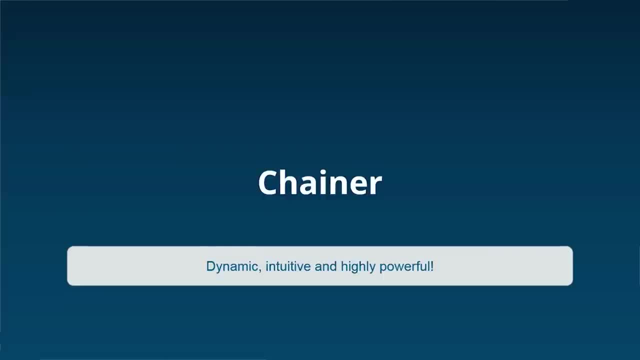 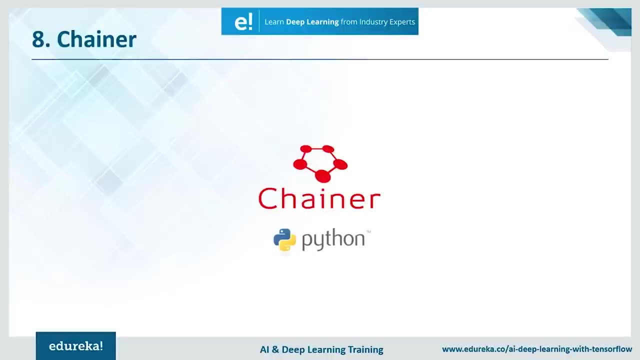 and I'm sure you guys are all curious about Chainer, right? Well, Chainer is a python-based deep learning framework defined by run strategy. The first thing we look at is performance. Well, Chainer has got that sorted. It is known for its high performance capabilities in all of the domains. 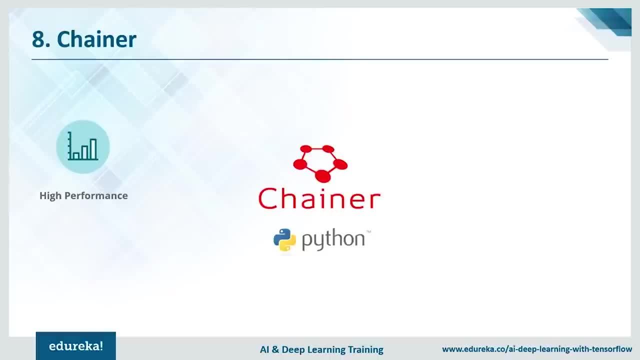 Well, with performance comes a slight prerequisite on how easy it is to actually get around and get the work done with the framework right. Again, Chainer is intuitive and coding in it is really easy, guys. I would rate it about 6 on 10 at this point, though. 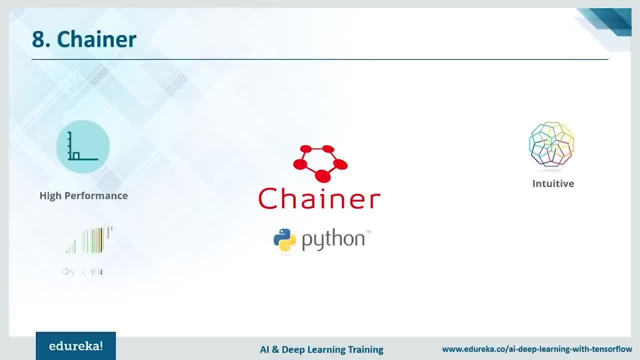 Now that you know it is intuitive. What's fancy about Chainer? Well, let me tell you, it provides really good dynamism and helps with understanding the flow of the code better, and this in turn works well because of the direct approach into good machine translation as well. 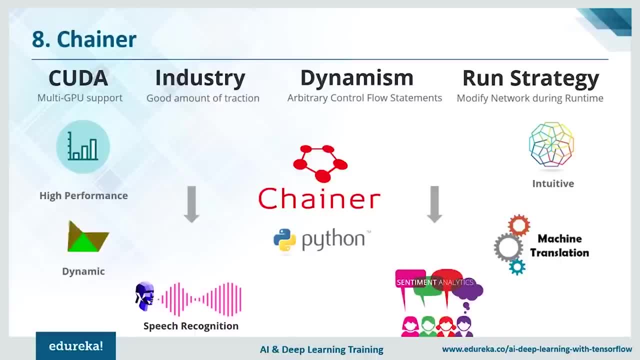 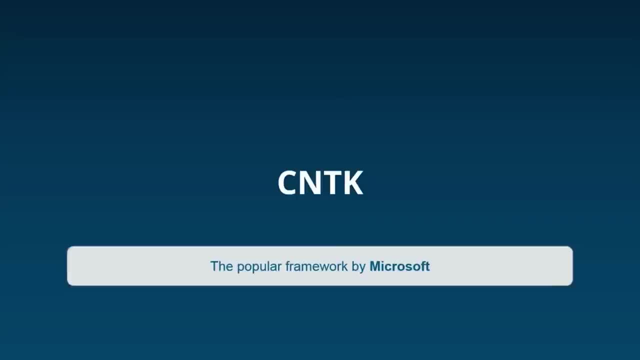 Well, Chainer is widely used, But it is mainly used for speech recognition and sentiment analysis of all sorts. Okay, So, now that Chainer is done, What do we have next on the list? Well, it's Microsoft's CNTK. 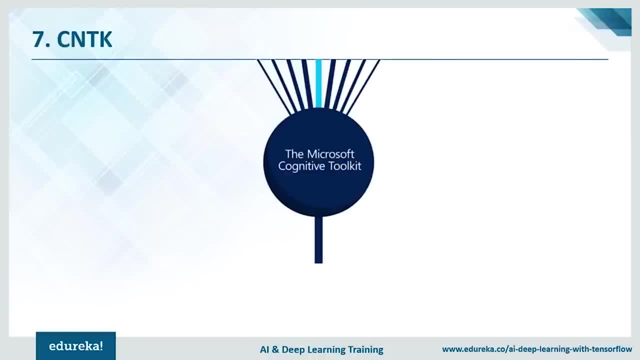 However, it has a new name now, guys. It's called Microsoft cognitive toolkit. Well, that sounds fancy, right? Well, CNTK is actually fancy as a framework. It is supported by interfaces such as command line, C++ and python. It's said to provide really high scalability in terms of training. 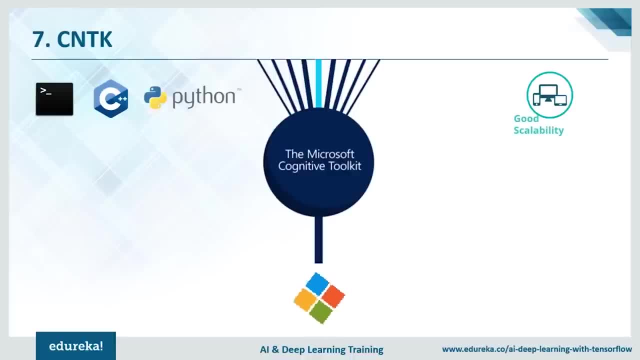 a convolutional neural network for images, speech or any textual based data. when working on multiple machines, The scalability is definitely better than Theano or, say, even TensorFlow to some extent, and when it comes to usage, it has to be handwriting recognition and speech recognition mainly. this is made easy. 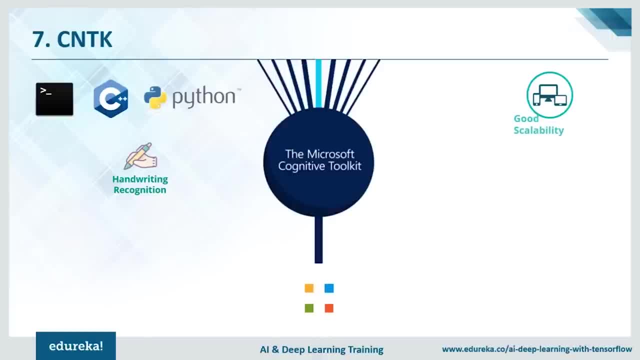 because inventing a new complex layer types in CNTK is extremely straightforward. but you might be curious at this point about how so right? Well, users will not have to implement anything In a low-level language, which is definitely worth noting. Well, now that that's done, next up we have generative. 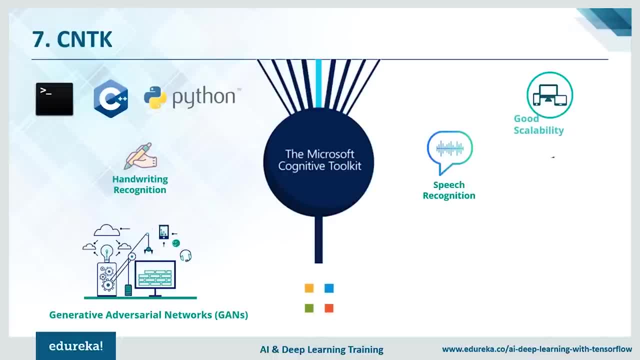 adversarial networks. Well, that's a mouthful. However, not to worry guys, It's just one of the types of reinforcement learning. and now that we've established that, how does it scale again, on a scale of 1 to 10, it ranks at about 7 on how easy it is. 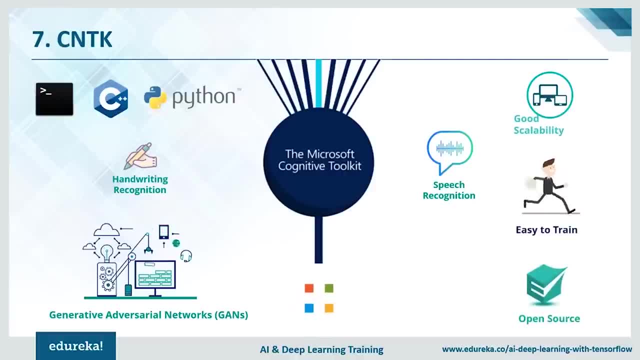 to actually train the models. and lastly, of course, Microsoft, after 2012, has been making a lot of its Technologies open-source. this definitely adds to the number of contributors that are pouring in and expanding the community. eventually, However, due to the lack of support on ARM architecture, 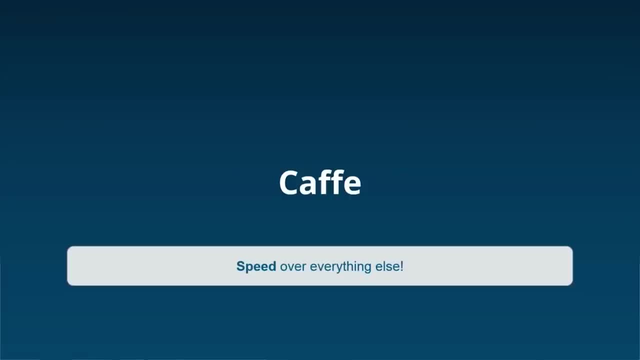 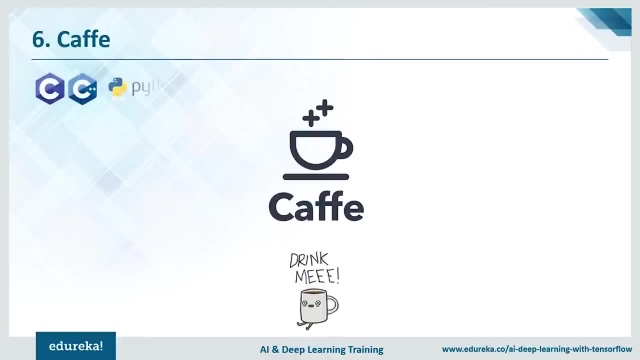 The capability on mobile is fairly limited. Well, to fix this, cafe came into the picture. Well, cafe is another deep learning framework that is supported with interfaces like C, C++, Python, matlab, as well as the command line interface. Well, that's lovely. It is popularly used for vision recognition, guys. 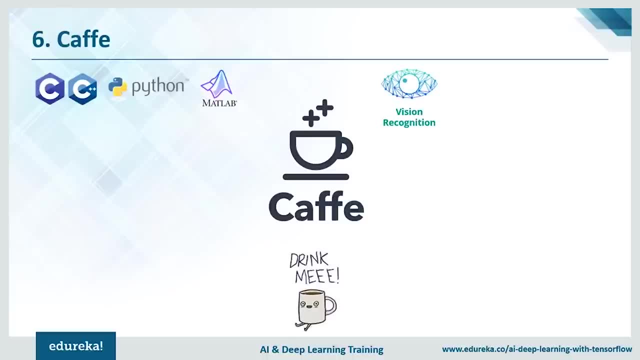 However, cafe does not support fine granularity Network layers like those found in TensorFlow or CNTK. I'm pretty sure you might be wondering why. well, we will require a bit of low-level language code, which I am sure majority of us don't like, right. 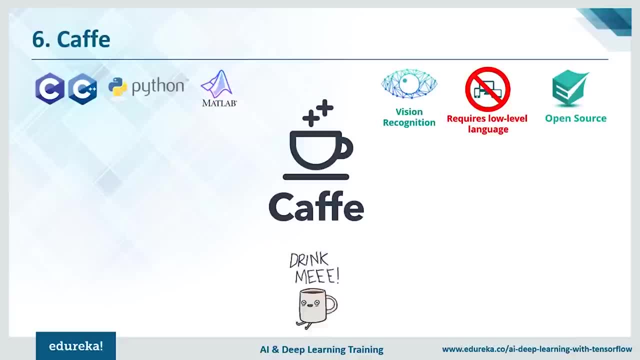 Well, again, it has to be open-source. So if it's getting all the attention for its- your speed and performance, I'm sure again You're wondering how well cafes biggest bragging right is definitely its speed. more on this in just a second. 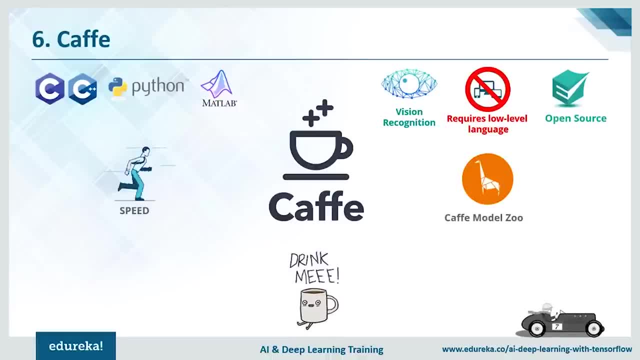 Also, the presence of something called as the cafe model Zoo was really good. It is really simple, guys. It is basically a deep net repository which is already pre-trained and it is available to use immediately. Well, now let's get back to that speed thing. 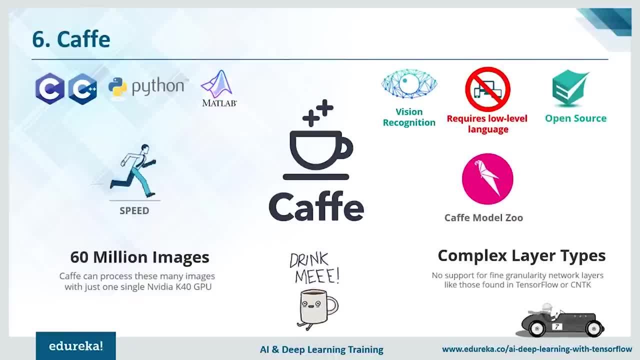 Well, we all love speed. right cafe just ups its game here, because it can process over 60 million images on a daily basis with just one single Nvidia k40 GPU. Well, that's about 1 millisecond per image for inference and 4 milliseconds per image for learning. 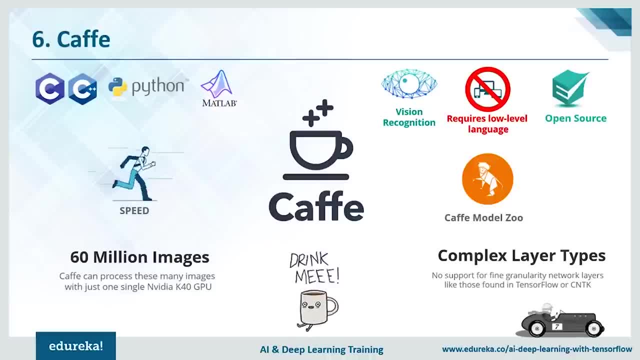 and with more recent libraries, It is getting still faster. Well, this is definitely amazing, So this is definitely like icing on a cake, and, whether it is modeling CNN's or solving image processing issues, This has to be the go-to library, in my opinion. 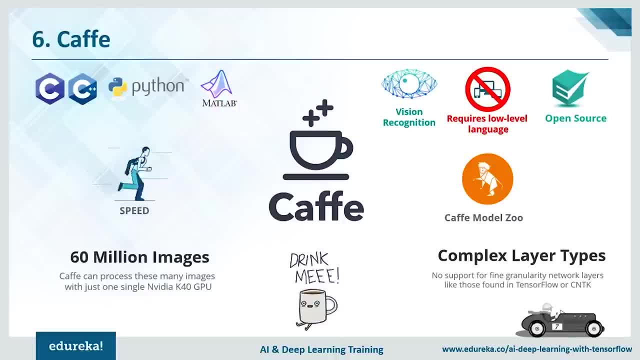 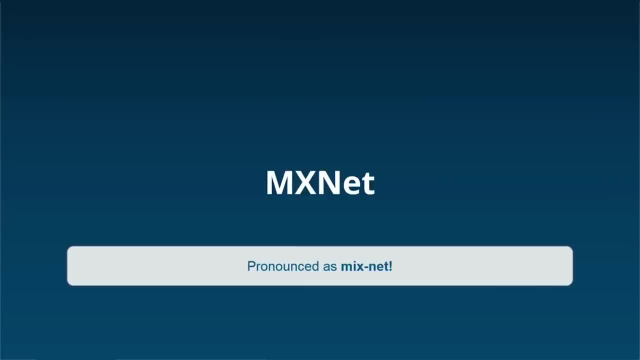 but given the architecture, the overall support and the language modeling capabilities, it lacks a little bit when compared to these other frameworks. So to fix this, what do we do? Well, let's bring in mixnet to the picture. The beauty of mixnet is that it provides the user the ability. 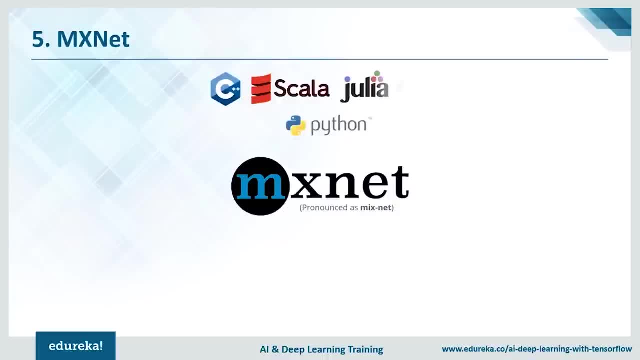 to code in a variety of programming languages, ranging from python, C++, are, Julia And scale are to name a few. Well, there are more, actually. well, this means that you can train your deep learning models with whichever language you're comfortable with, and you don't have to learn anything new from scratch. 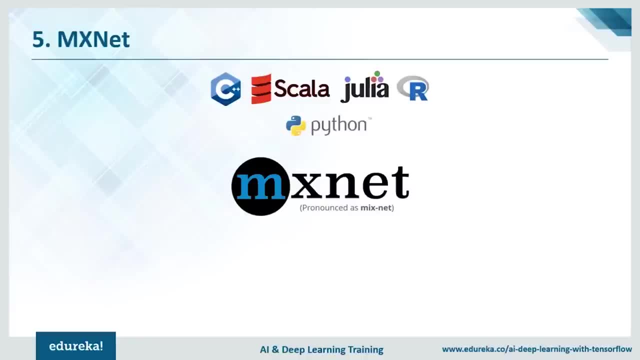 Well, that's really good right. Well, now we need to find out how mixnet actually stands out. Well, for starters, mixnet was specifically designed for high efficiency, high productivity and a lot of flexibility, guys. mixnet supports long-term, short-term memory. 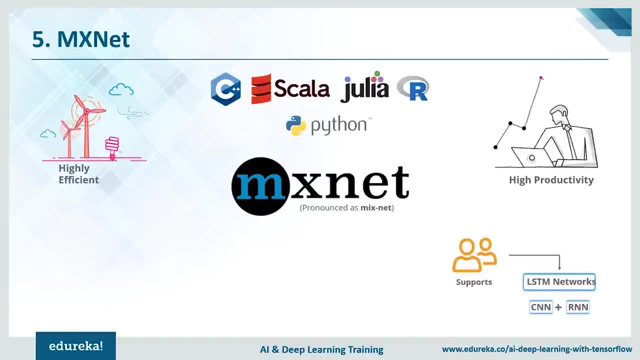 which is also called as LSTM, along with the support for both recurring neural nets and convolutional neural nets. Also, it's known for its capabilities in imaging, speech recognition, forecasting, as well as natural language processing. and, lastly, Amazon employed mixnet as its go-to reference library. 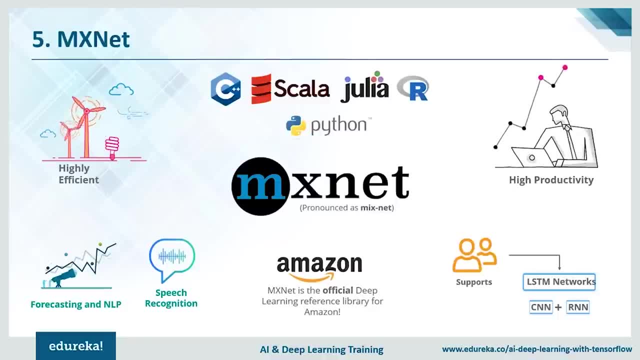 for majority of its deep learning requirements. Well, we're looking at a lot of interfaces like C, C++, python and even matlab, until missing something that makes our lives that much simpler, guys. Well, yes, you might have guessed it right: I'm talking about Java. 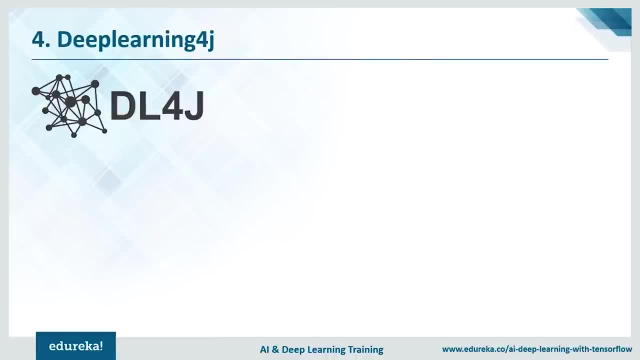 We have a framework which is exactly tail I made for this, and it's deep learning for Java guys. The biggest highlight is that it provides parallel training through iterative reduce and microservice architecture adoption, coupled with distributed CPUs and GPUs. Well, to be honest, I would be impressed by anything. 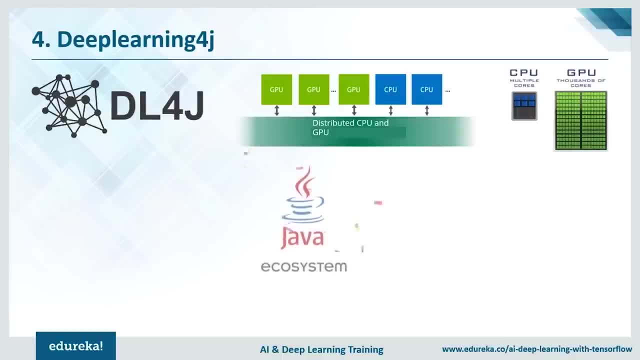 which involves a lot of CPUs and GPUs at the same time. Well, this framework is widely adopted as a commercial and industry-focused deep learning platform. Well, now that we have established that, what's the biggest advantage you ask? Well, for starters, you can bring together the entire Java. 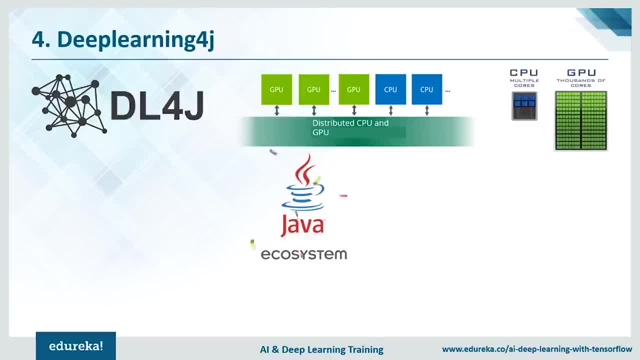 ecosystem to execute deep learning, and what makes it even better is that it can be administered on top of Hadoop and spark to orchestrate multiple host threads. The framework shows matchless potential for image recognition, fraud detection, text mining and parts of speech tagging and natural language process as well. 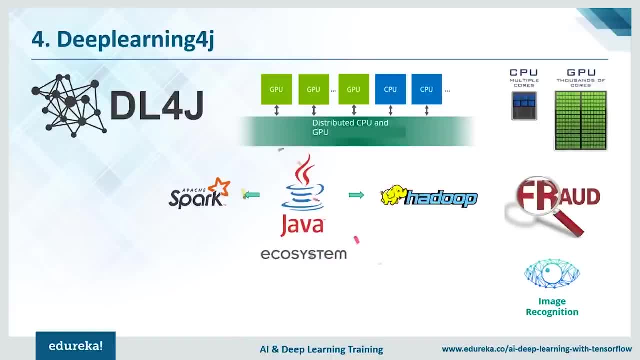 which, in my opinion, is definitely amazing. Well, deep learning for Java comes with a deep network support through RBM. RBM is nothing but restricted Boltzmann machine. also, DBN. DBN stands for deep belief networks. Well, it's nothing but a layered graphical model. in simple terms, 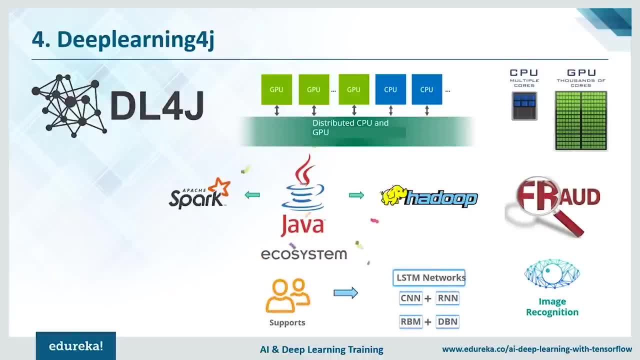 and also the added support for convolutional neural networks, recurrent neural networks and long-term short-term memory, which is also called as LSTM networks, as well. Well, guys, you need to take a note that it is much more efficient in comparison to python in multiple fields. 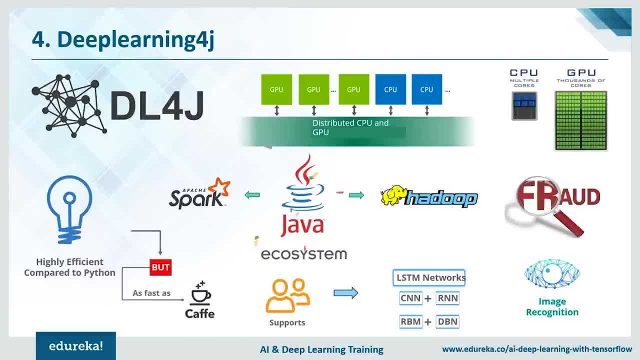 when it comes to image recognition tasks using multiple GPUs, It is actually as fast as cafe, which again impressed me a lot. also, with Java as your core programming language, You should certainly opt for this deep learning framework If you're looking for a robust and effective method. 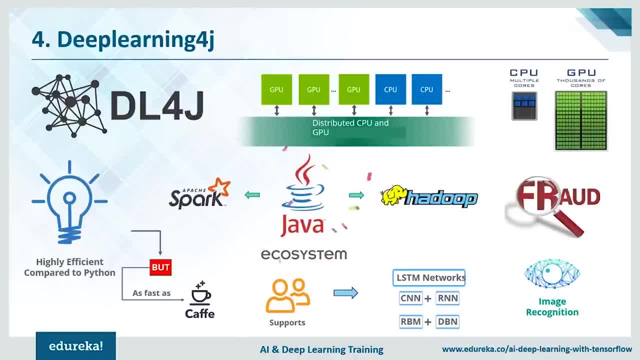 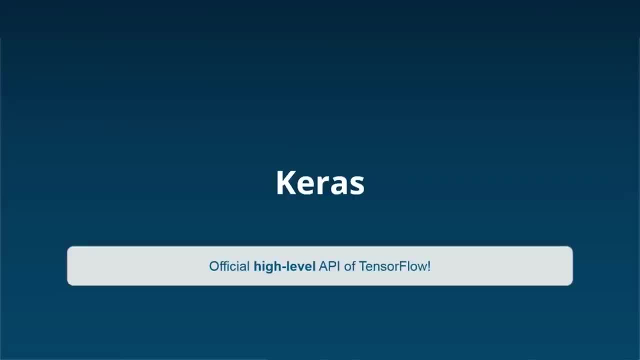 of deploying your neural network models to production. Well, now that we have sorted this out, we just left with the top three frameworks for now. Well, I have saved the best for the last. so, quickly, Let's take a look at our number three competitor. 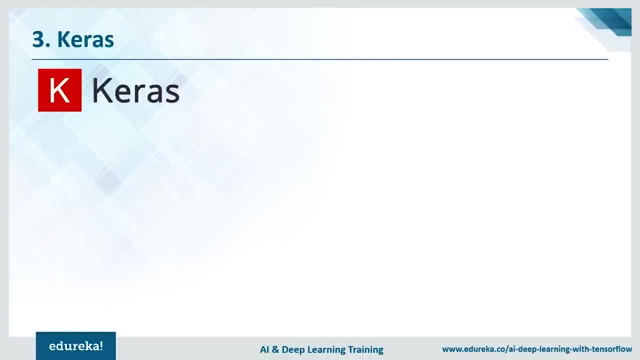 which is Kiras. Well, what I really like about Kiras is that, for starters, it is well known for being minimalistic, and you get the work done with python Well. Kara supports both convolutional and recurrent networks that are capable of running on top of either Tiano or tensorflow. 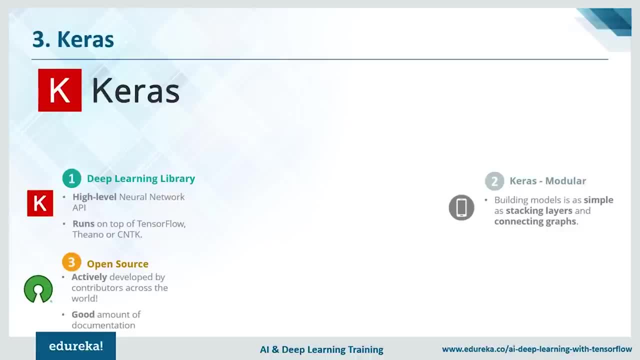 Well, due to the fact that the tensorflow interface is a tad bit challenging, coupled with the fact that it is a low-level library, that can intricate for new users, Well, it makes it a bit tough, right, But Kiras was built to provide a simplistic interface. 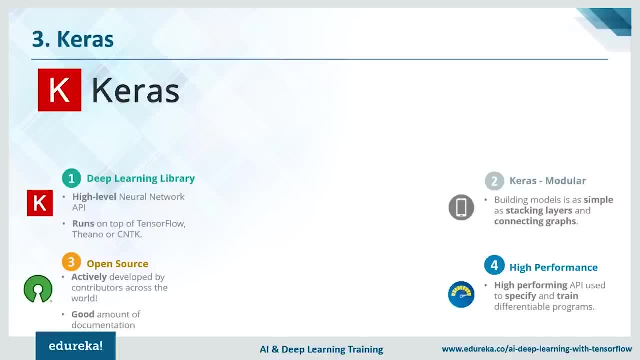 for the purpose of quick prototyping, by constructing effective neural networks that can work with tensorflow. and there we ask the question and we answered it. Also, guys, Kiras is a celebrity, to be honest. It had over 4800 contributors at launch and now it has over 250,000 active developers. 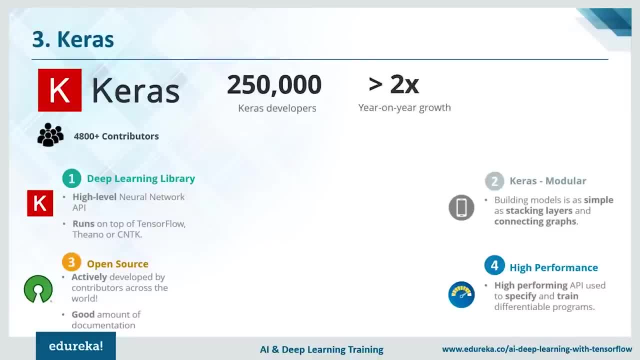 and it is still adding. well, with every year There is a two times growth on the overall development of the framework and since it's getting all this good attention, it has certainly made a really good name among the majority of the startups. Well, we have eight standout features. 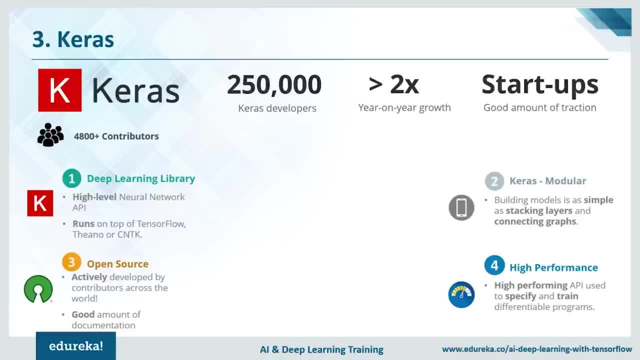 which I believe deserved a mention in the session. Well, you're curious, right? So let's start out Well, definitely starting out with the focus provided on user experience, followed by the large adoption in the industry, making everyone use the framework and build a vast community overall. 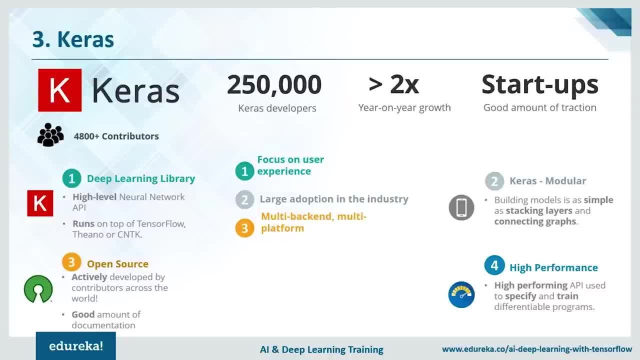 And, of course, the support to let use of multiple backends develop and deploy on multiple platforms is a plus. Well, what surprised me is that it has a real good community when it comes to research as well. And lastly, of course, all the concepts are really, really easy to grasp, guys. 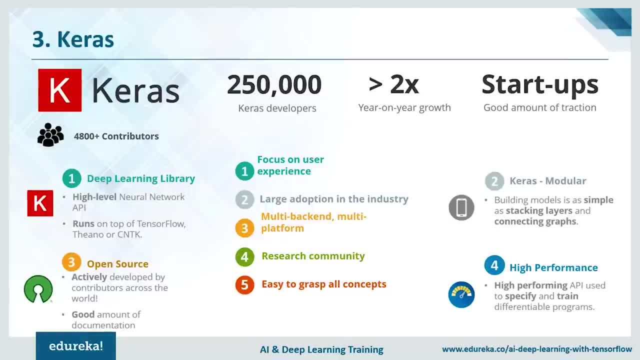 Well, guys, at this point we have established that Kiras is really good, right, But is it as good as PyTorch, which is the next framework I want you guys to check out? Well, we haven't looked at definitions for a while. 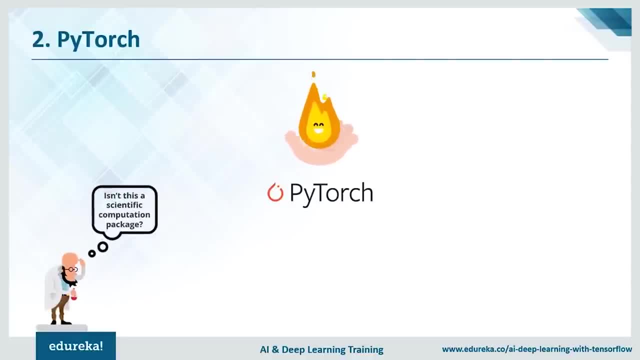 So what is PyTorch? Well, PyTorch is a scientific computation package created by all the amazing people at Facebook. It is Lua powered and works with Python, which is definitely a win already, and we haven't even begun to discuss the framework. 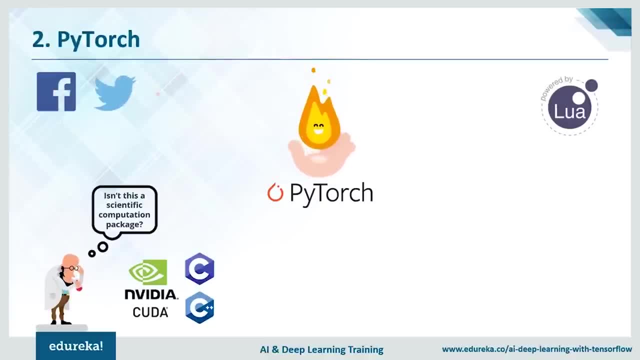 Well, guys, it's majorly used by industry Giants like Facebook, obviously, Twitter, and even Google to certain extent. Well, PyTorch is giving you a really good time when it comes to using Facebook, right? You're wondering how? well, let me tell you this consider: 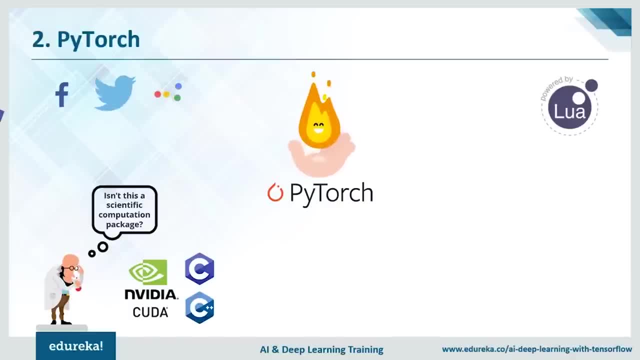 that it's a weekend and you're partying with friends. You decide to click a lot of pictures and you want to put them on Facebook. right, But tagging everyone manually. I am not a fan of this, and I'm sure you are not too well. 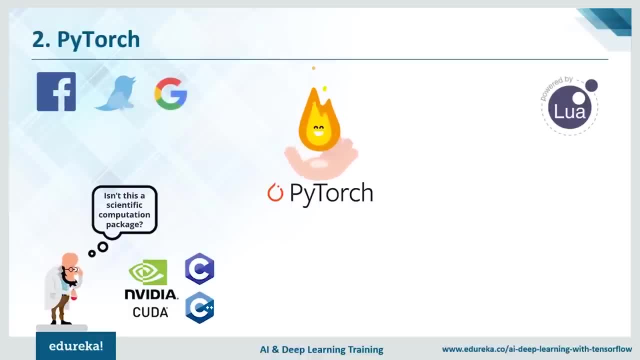 Remember those magical pop-ups which automatically detect faces? Well, thank PyTorch for that. However, as opposed to torch, which is actually the predecessor of PyTorch, PyTorch runs on python, which means that anyone with a basic understanding of python can get started. 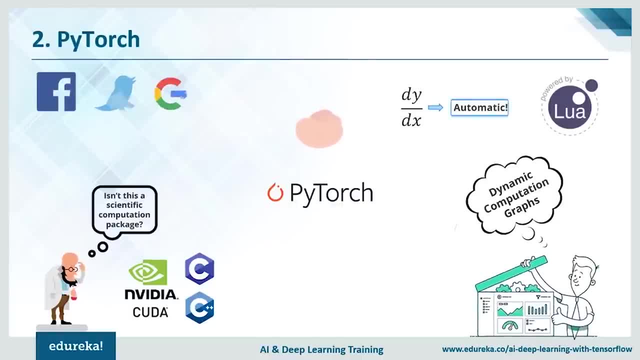 on building their own deep learning models. However, features such as automatic differentiation by the autograd module and the support for dynamic computation graphs is what makes PyTorch stand out when it compares to all the other seven frameworks. to be honest, Also off late, PyTorch has seen a high level of adoption. 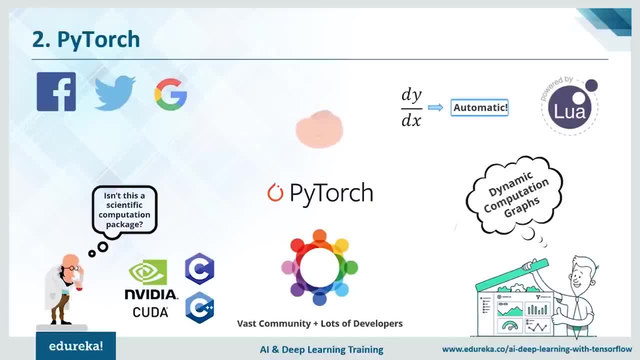 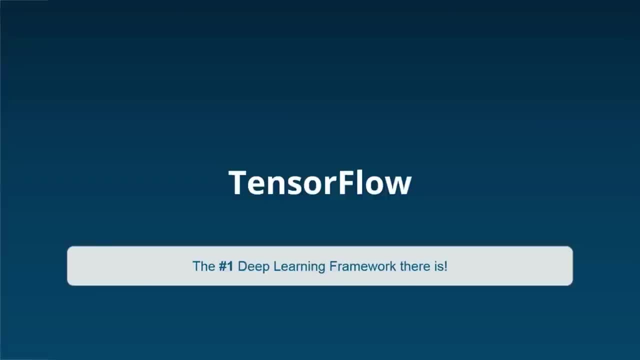 within the deep learning framework community and is considered to be quite the competitor to TensorFlow. Well, which is exactly what we are going to talk about, and TensorFlow definitely grab the number one spot and this rundown of the framework. Well, TensorFlow is the brainchild of all the amazing people at Google. 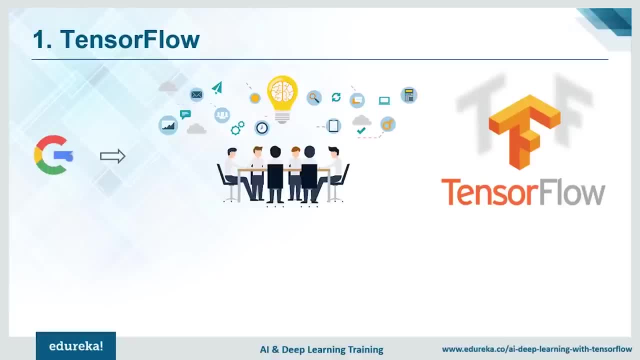 The most well-known use case of TensorFlow has definitely got to be Google Translate. right, It is coupled with the capabilities of natural language processing, text classification, speech recognition, image recognition, forecasting and tagging- well, wow, the list goes on and on. for sure. Well, it is arguably one of the best frameworks right now. 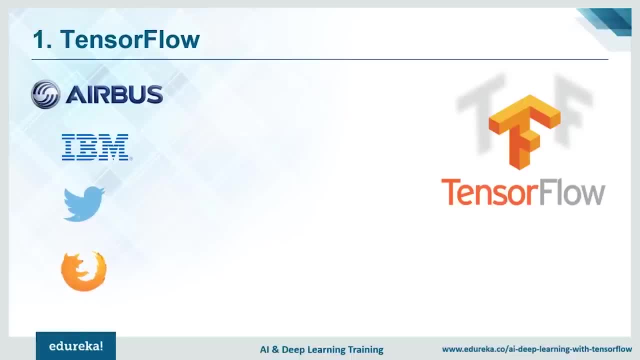 which is why it has been adopted by several Giants at scale, such as Airbus, Twitter, IBM and mainly others, due to the highly flexible system architecture. Also, guys, TensorFlow is available on both desktop and mobile and also supports language such as Python, C++ and R to create deep learning models. 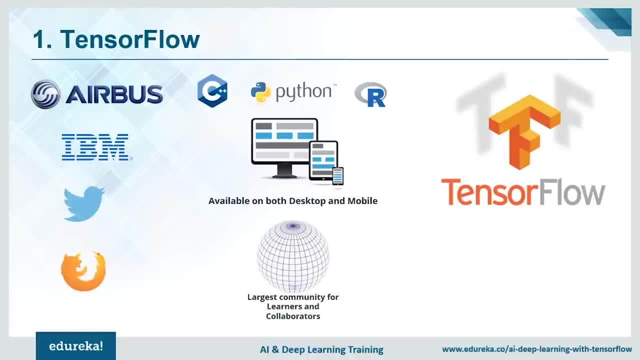 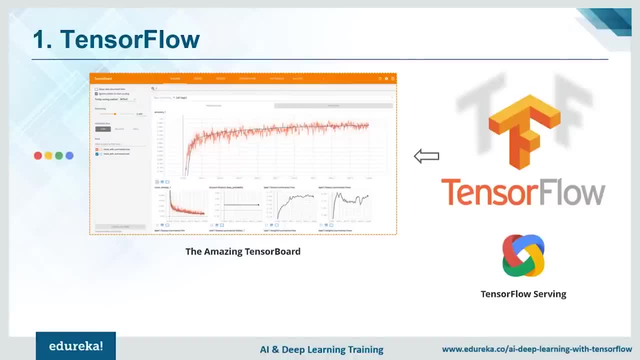 along with the wrapper libraries. Well, now we know why TensorFlow is really good, right? Well, it comes with two tools which are widely used. well, starting out with TensorBoard, it is used for effective data visualization of network modeling and performance, and secondly, TensorFlow serving 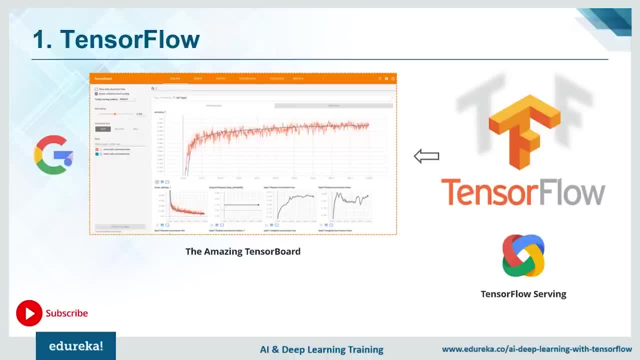 for rapid deployment of new algorithms or experiments while retaining the same server architecture and the api's. well, if you happen to be taking your first steps when it comes to deep learning, get a sort of a no-brainer that you should opt for TensorFlow, given that it is python-based. 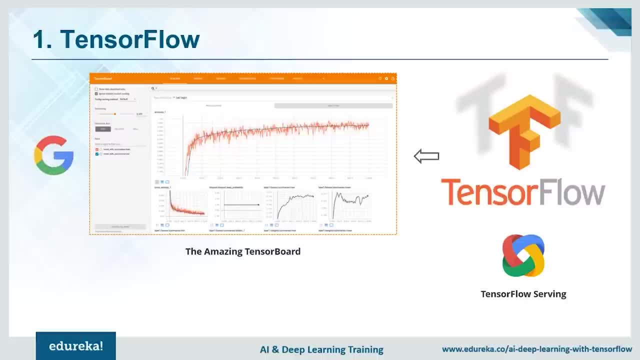 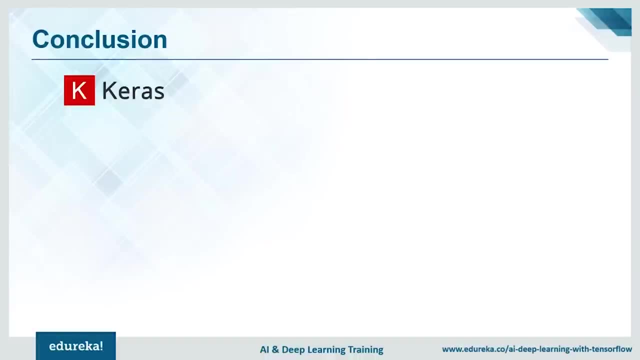 it is supported by Google and it comes loaded with documentations and walkthroughs to guide you. well, that being said, let me wind up the session by asking you this: which deep learning framework from this list would best suit your requirements? Well, the answer to that is dependent on you. 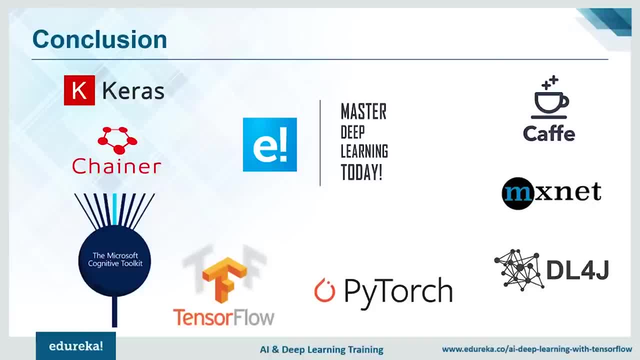 and definitely lies on a number of factors. However, if you're just looking to get started, then a python-based deep learning framework like TensorFlow or Chainer, as I previously mentioned, should be your choice. But if you happen to be seasoned, you need to consider speed. 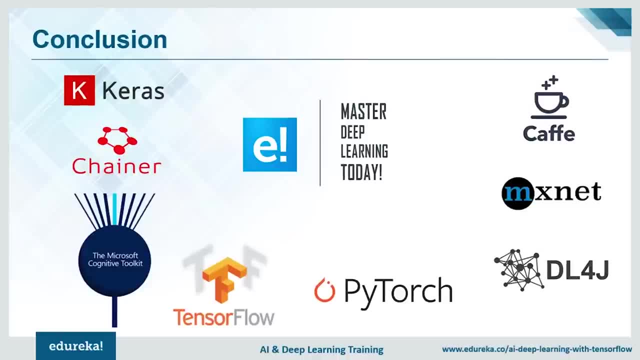 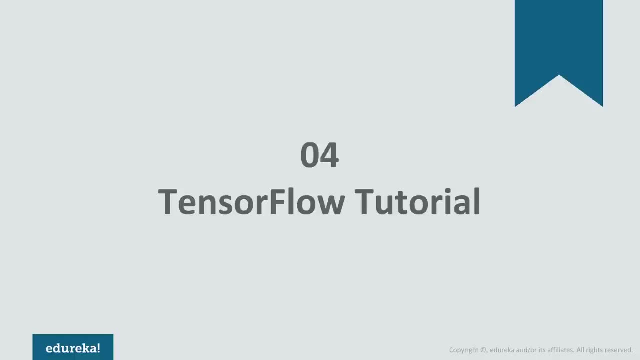 resource requirement and usage, along with the coherence of the trained model, before picking out the best deep learning framework There is. well, guys, we all love deep learning and this is one amazing community to be a part of. Welcome to this TensorFlow tutorial on deep learning. in this tutorial, 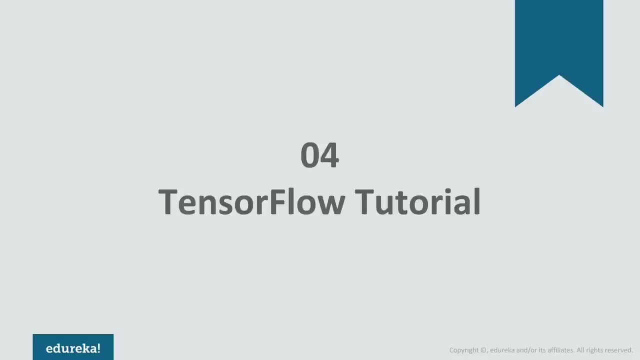 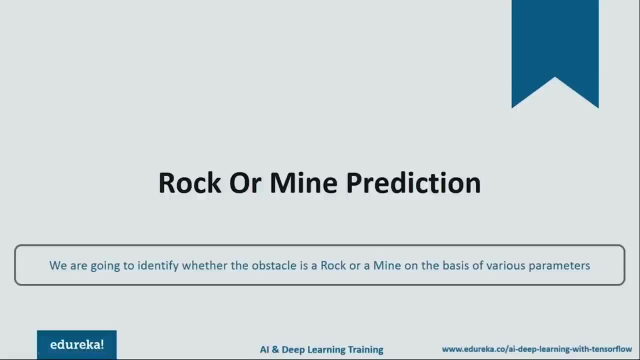 We'll be covering all the fundamentals of TensorFlow to implement a use case That is a Neville mine identifier, NMI. So let's begin, guys. Neville mine identifier is a pretty serious problem in which one needs to identify whether an obstacle is a rock or a mine on the basis of sonar signals bounced. 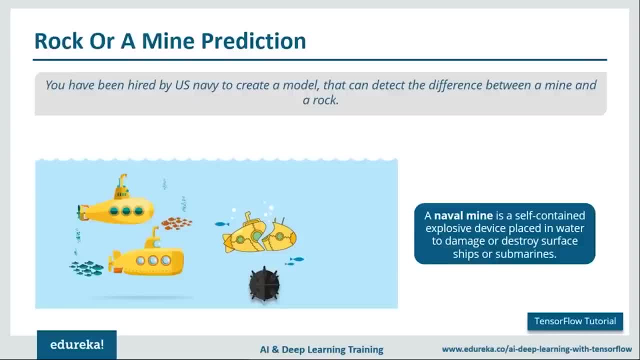 or reflected by it. So let's get into the details of this use case. Imagine you are hired by the US Navy and your task is to create a model that can differentiate between a rock and a mine. We will call this model as a Neville mine identifier- NMI. 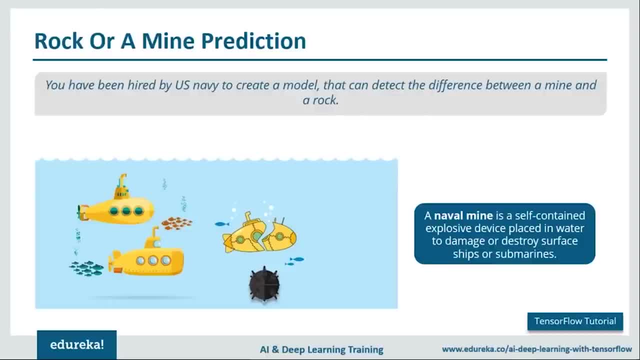 A Neville mine is a self-contained explosive device placed in water to damage or destroy surface ships or submarines. If you want a better picture, just consider the diagram that is there in front of your screen. So here we have three submarines, out of which one is broken. 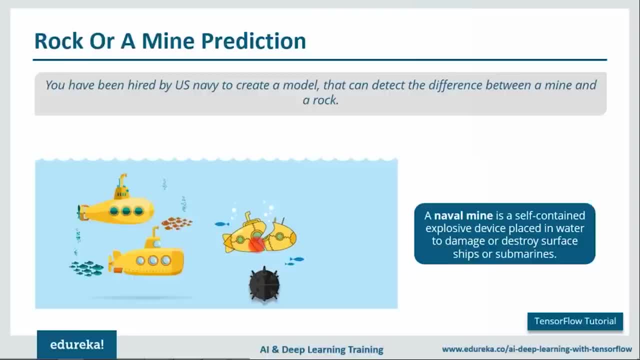 on into small pieces when it passes through a Neville mine. The major use of these underwater mines, or Neville mines, began in World War 1.. Similarly, in World War 2 nearly 700,000 Neville mines were laid, accounting for more ships sunk or damaged than any other weapon. 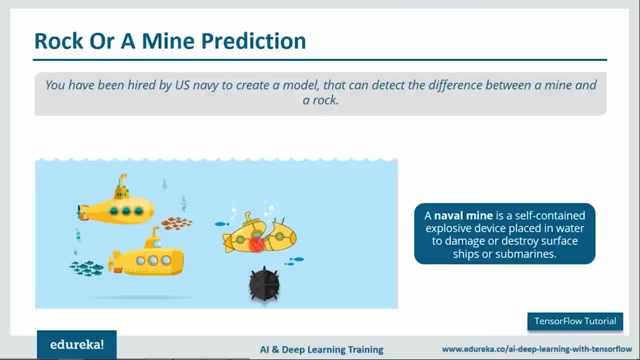 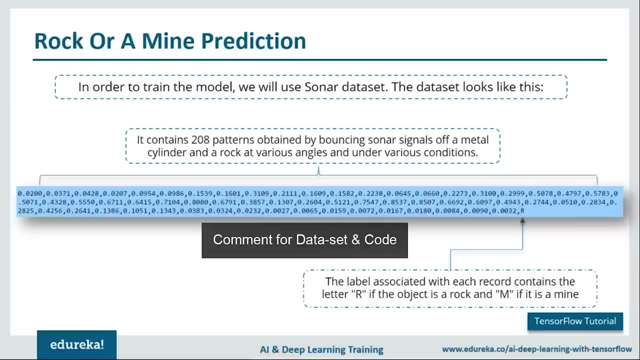 So now you must have understood the importance of this use case. This model can actually save a lot of lives. Now let's look at the data set that we'll use to create this deep learning model. Here we'll be using the sonar data set. 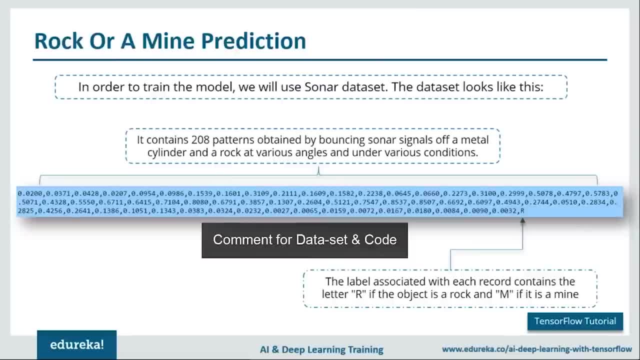 This data set contains sonar signals, which includes 111 patterns bounced off a metal cylinder and 97 patterns bounced off a rock, both at various angles and conditions. Hence, every record in the data set represents a pattern. Now let me show you the data set. 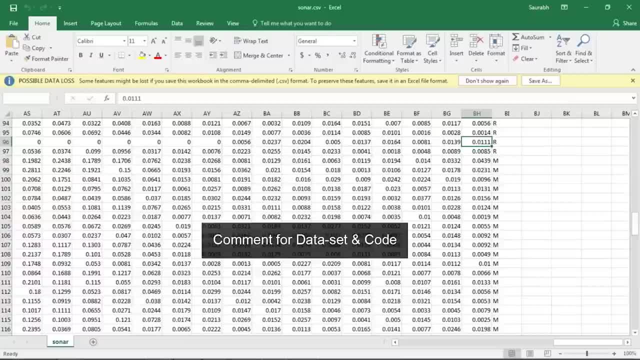 So there are total 61 columns in the data set, in which the first 60 columns is a set of 16 numbers in the range from 0.0 to 1.0, and the last column of every record is a label which represents the name of the class. that is, either a rock or a mine. 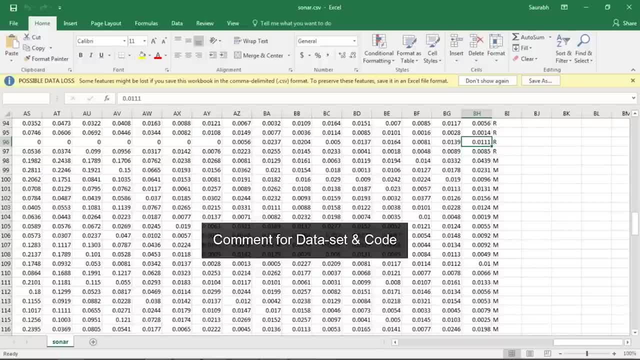 Let me explain you with an example. If the pattern is defining a rock, then the last column would contain the letter R. Similarly, the pattern represents a mine, then the last column would contain the letter M. So if you notice in the data set as well in the last column we have 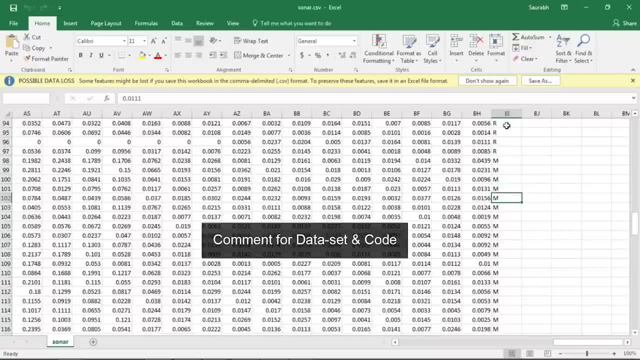 either R or M. So this is nothing but the class to which the pattern belongs to, whether it is a rock or a mine. So this data set contains both the patterns which can be analyzed for prediction and the actual outcomes, That is, whether the pattern represents a rock or a mine. 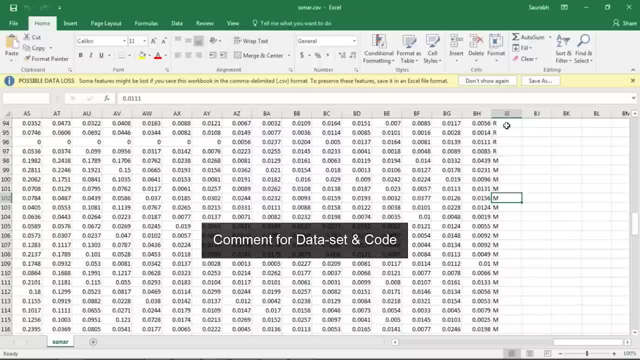 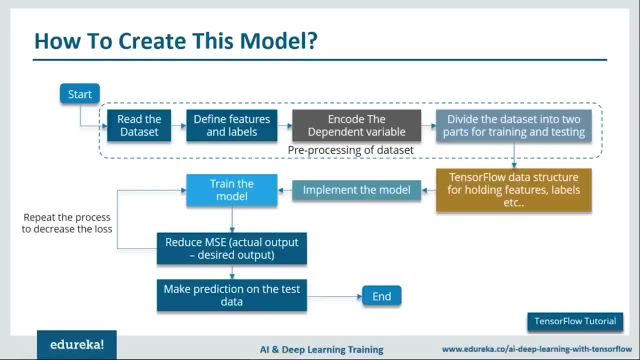 Hence it can be used for training the tensorflow model that we want to create. Now is the time to understand the flow, to implement the Neville Mine Identifier. Now, don't be scared of the fancy terms that I'll use here. You'll understand them all in the coming slides. 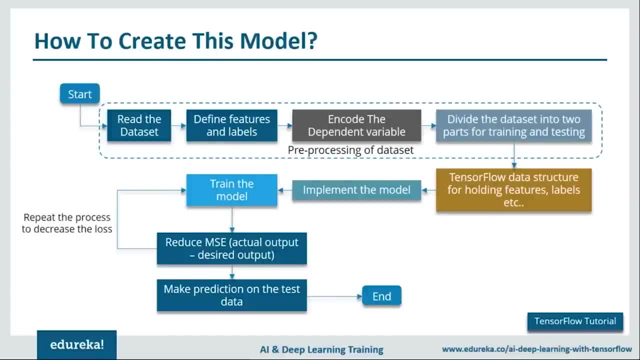 For now, we'll understand the steps that will be involved in implementing the tensorflow use case. So we'll begin by processing the data set that we have. We'll define features and labels. We'll divide the data set into two parts: training and testing. 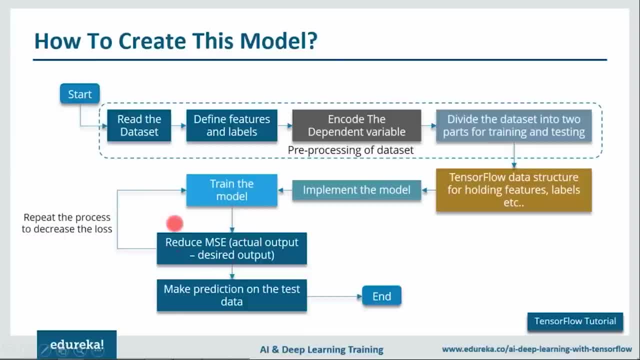 Then we'll train our model on the training data. We'll try to reduce the error. After that we'll test our model on the test data and we'll calculate the accuracy. Here our ultimate goal is to achieve the highest possible accuracy. So, guys, let me quickly execute the tensorflow model. 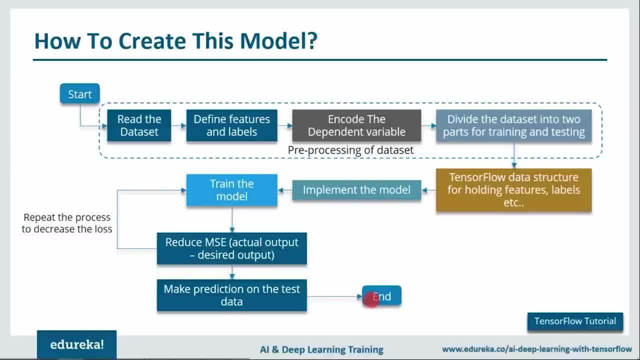 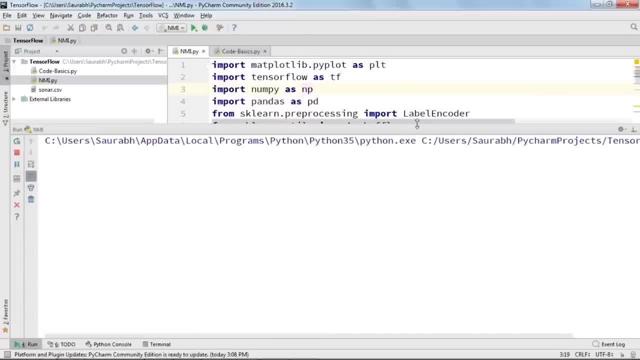 that I've already created for you. For that I'll open my PyCharm. So this is my PyCharm. guys over here, I've already written the code in order to execute the use case, So I'll just go ahead and run this. 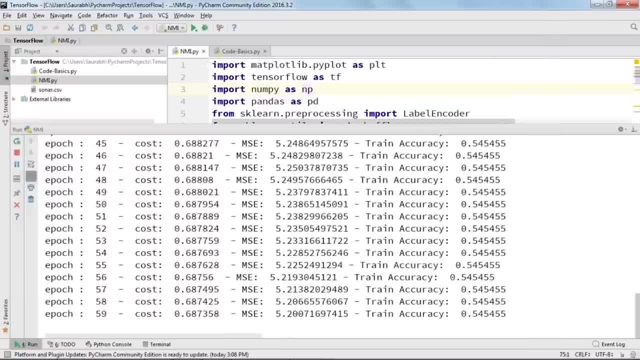 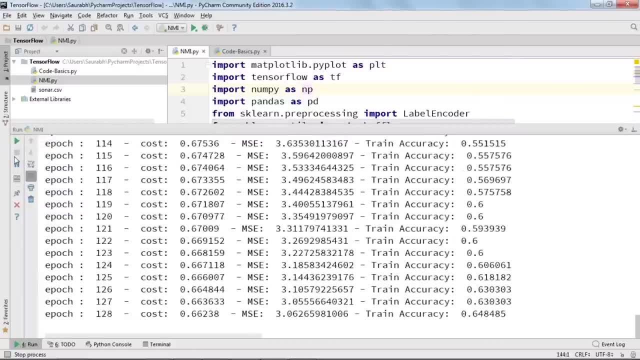 So this is how the output looks like where the deep learning model is getting trained. If you observe, with every iteration the accuracy is increasing and the error is decreasing. So we'll stop it right here. So with this, we'll get back to our slides. 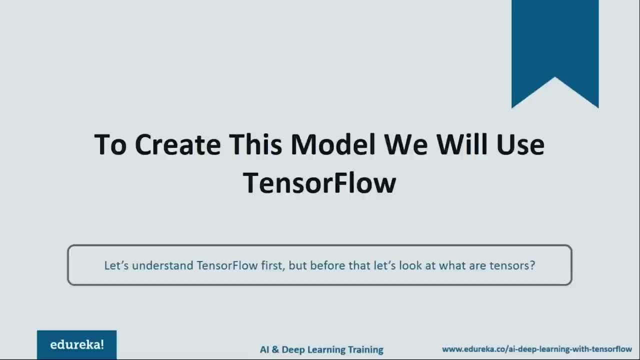 and understand the fundamentals of tensorflow first, before we get into the implementation details of this user. In order to implement this use case, we'll be using tensorflow, which is a Python library. In tensorflow, data is represented in the form of tensors, So let's understand that first. 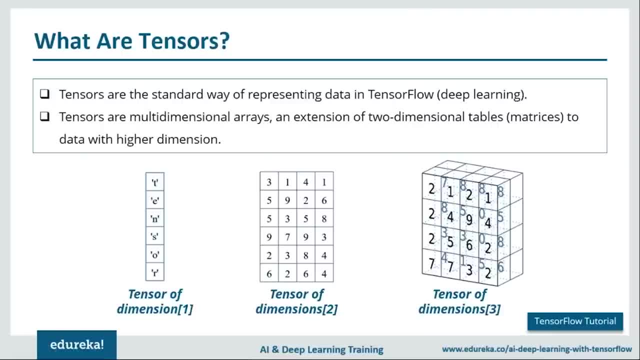 TensorFlow programs use a tensor data structure to represent all data. You can think of a tensor as an n-dimensional array or list. Now consider the example that is there in front of your screen. So the first tensor has dimension 0.. The next tensor has two dimensions. 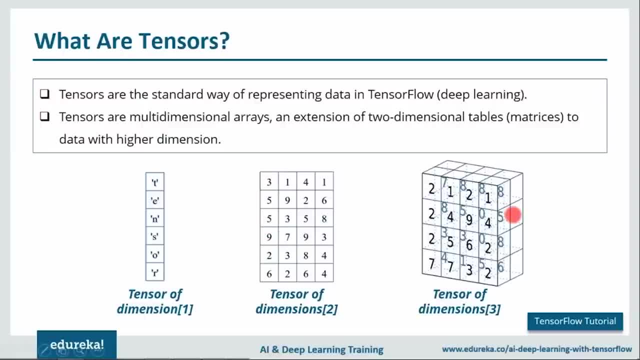 because it has rows as well as columns. And the last tensor has dimension 3 because it has one more field. Now, in tensorflow system, tensors are described by a unit of dimensionality known as rank. So let's understand that. So a rank 2 tensor is what we typically think of as a matrix. 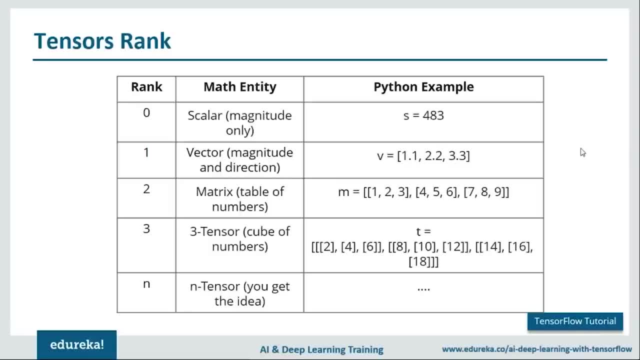 And a rank 1 tensor is a vector. Now let us focus on the table that is there in front of your screen. So rank 0 is nothing but a scalar which has magnitude only. You can think of its example as 483, 689,, numbers like that- 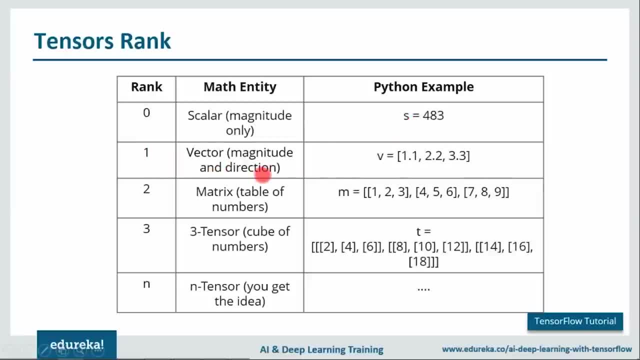 Then, when I talk about rank 1, it is a vector which has magnitude and direction, both- And you have the example in front of your screen: 1.1,, 2.2,, 3.3.. Similarly, when I talk about rank 2, 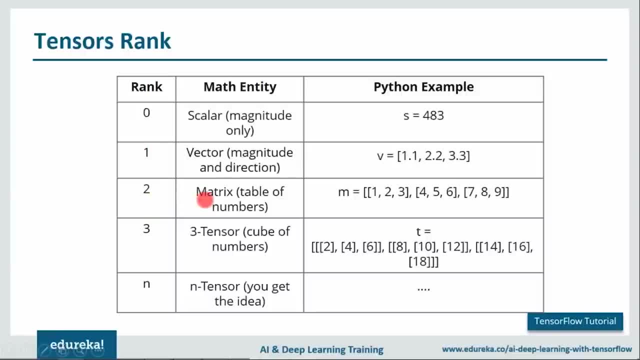 it is nothing but matrix tables of numbers. You can say rows and columns, And you have an example here as well. Similarly, when I talk about rank 3, you can see the example here. So this is how we actually define the rank of a tensor. 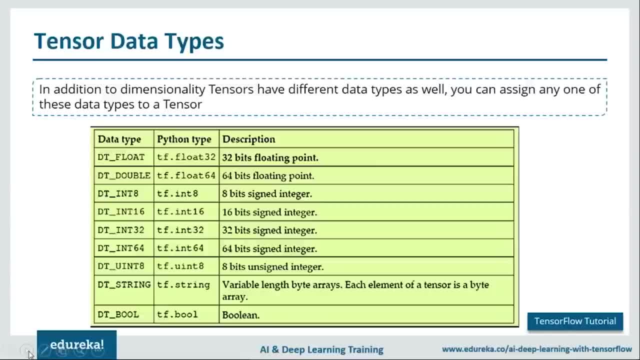 Now let us move forward and understand various tensor data types. You can see in the table that there are multiple data types. There is integer type of 8 bits, 32 bits, etc. Similarly even for float type. Then there is even string and boolean type. 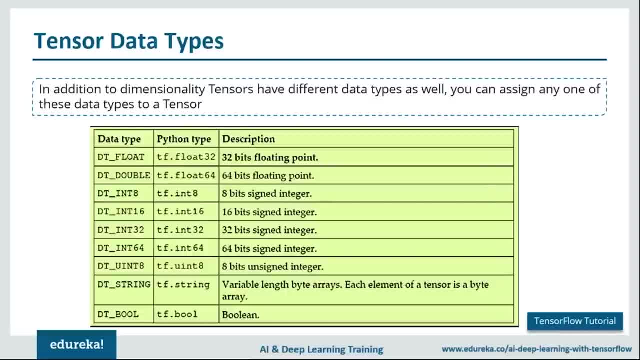 However, in TensorFlow you don't need to specify the tensor data type. It will automatically assign the correct type. But if you want to save the reserve memory, for example if you know you require only 32 bits, then there is no point in reserving 64 bits. 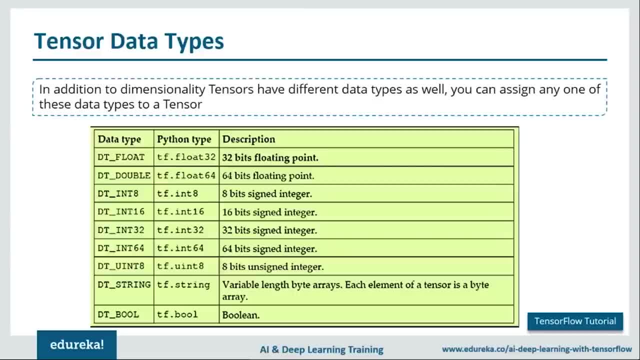 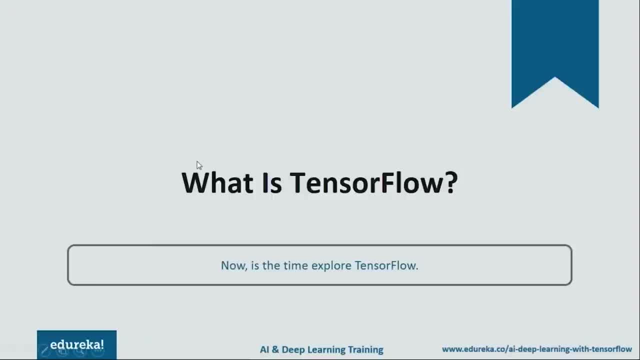 So at that time, you can specify the tensor data type to be of 32 bits. So that way, you can save some memory. So, guys, now is the time to understand what is TensorFlow. TensorFlow is an open source software library released in 2015 by Google. 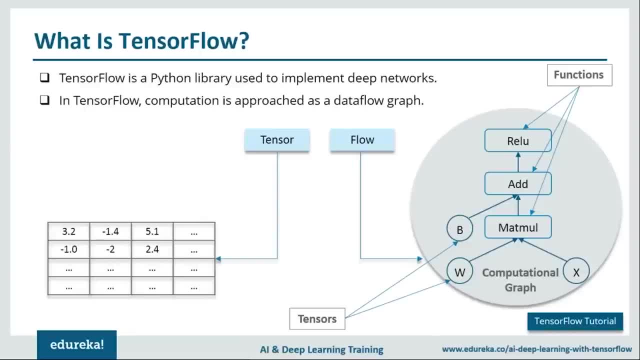 to make it easier for developers to design, develop and train deep learning models on neural networks. Now TensorFlow works by first defining and describing our model in abstract, And then we are ready, we make it a reality in a session. Now don't worry guys, in the next slide I'll explain what exactly is session. 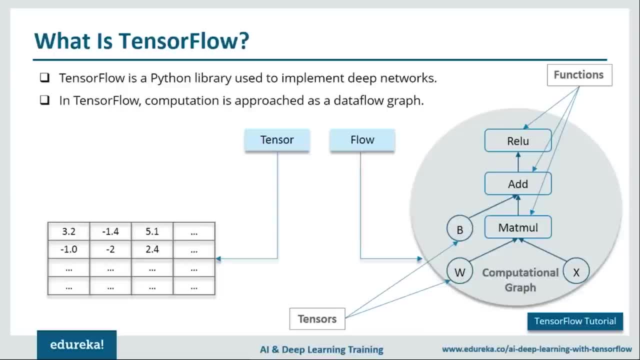 This description of the model is what is known as your computation graph in TensorFlow. And remember, guys, only tensors may be passed between the nodes in a computation graph. Now, if you notice, TensorFlow is nothing but the combination of two words: tensor, which we saw in the previous slide, and flow. 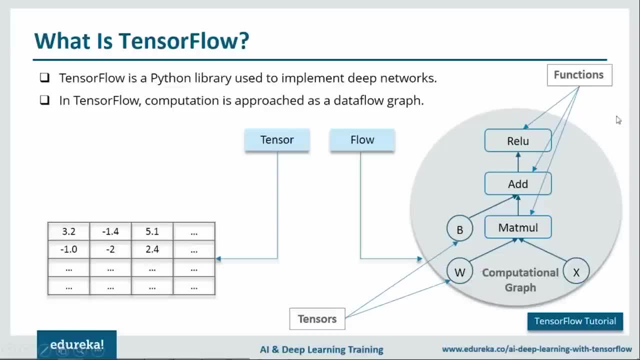 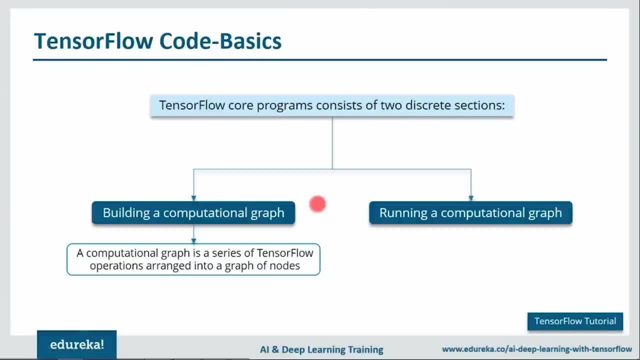 which is nothing but the tensors flowing through a computation graph. So, guys, let us dig a bit deep and understand the TensorFlow code basics. The TensorFlow programs consist of two sections. One is building the computation graph. Here we just describe the computation. It doesn't compute anything. 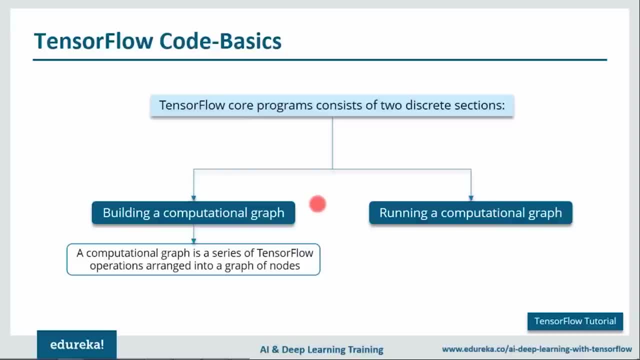 It doesn't hold any values. It just defines the operations specified in your code. When you execute it, the output will just be an abstract tensor. No actual calculations will run. Only operations will be created. To actually see the result, we need to run the session. 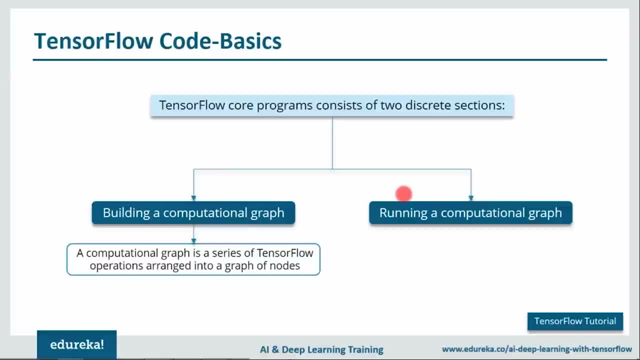 Generally, you build the graph first and then you launch the graph right. This session allow us to execute the graph or a part of the graph. Let us understand this with an example. So this is how you build a computational graph. Here we have defined two constant nodes. 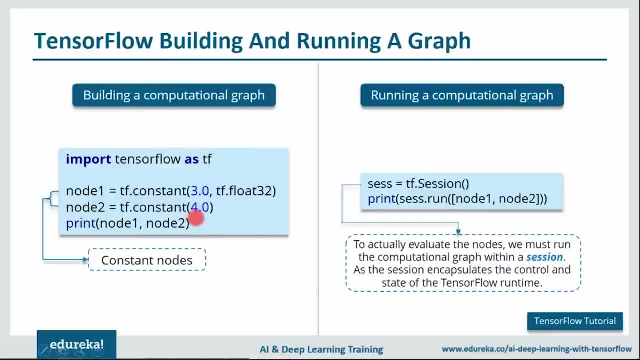 Node 1 has a value of 3 and node 2 has value 4.. Then what we do? we need to run it inside a session in order to execute the graph. Now let me go ahead and execute this practically in my PyCharm. 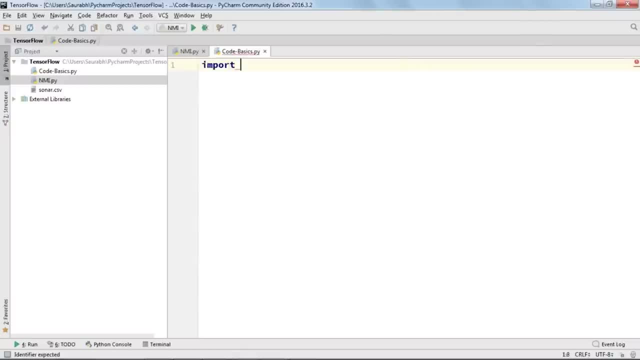 This is my PyCharm again, guys. First thing I need to do is import TensorFlow as tf. Then we will define two constant nodes, Node 1, equal to tfconstant, and the value will be stored inside. it will be 3.0. 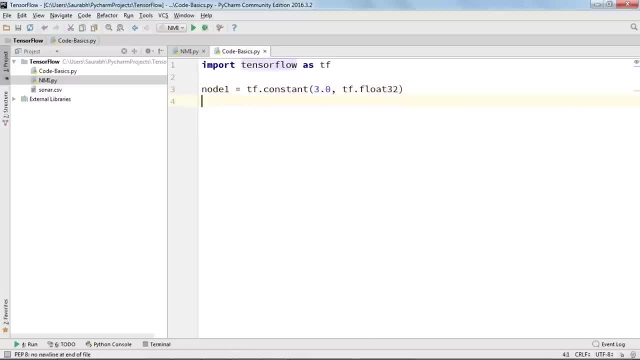 It is of tffloat 32 bits. Then we will define one more node and let it be tfconstant again and the value that will be stored will be 4.0.. Next up, when we try to print these two nodes, let us see what happens. 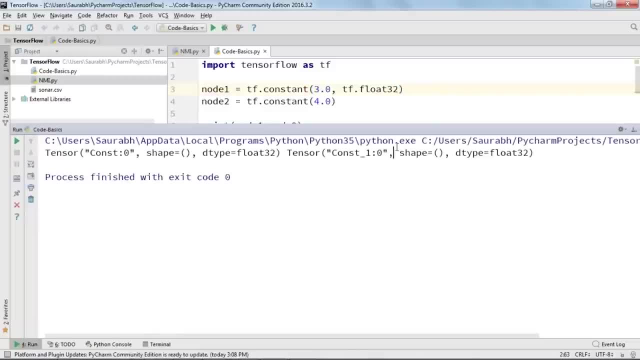 Let us go ahead and execute this Now. the output here is just an abstract tensor. No actual calculations are running, Only operations are created. Now to execute this graph, let me tell you how you can do it. First, I will comment this line. 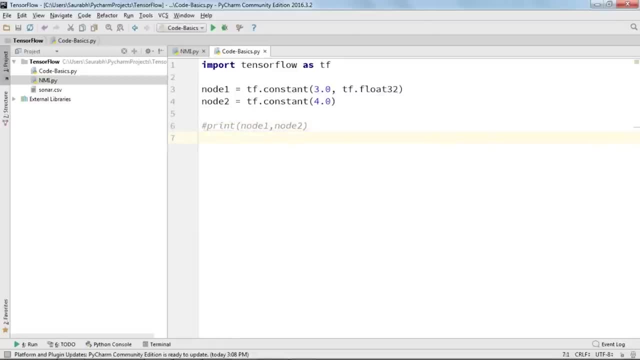 Now to execute this graph. we will run it inside a session I told you earlier as well. So session places the graph operations onto devices such as CPUs or GPUs and provides methods to execute them. So I will type in here: ses is equal to tfsession. 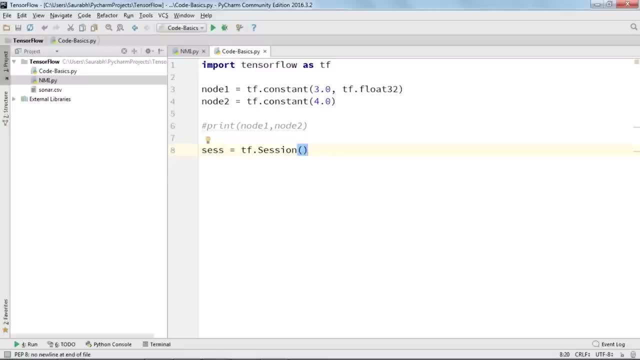 So this will basically launch the graph and create a session object. Next up we will run the results. So for that I am going to type in here: print sesrun, and we want the values of node 1 and node 2.. So let us go ahead and type that. 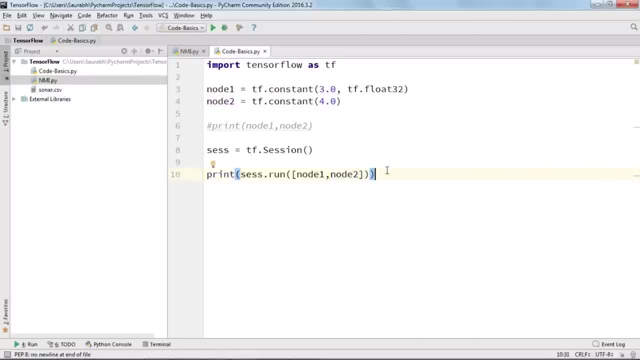 Node 2.. Yeah, this is fine now, And when we are finished with the session, we need to close it in order to free up the resources that were used. So that is also very easy. Just type in sesclose. That is all you need to do. 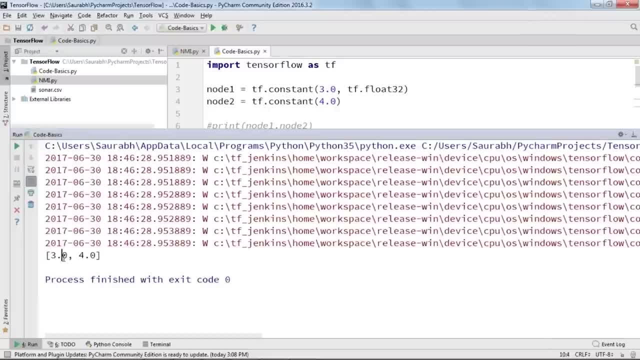 Go ahead and execute this, So we have got the output as 3 and 4, which is absolutely correct. These are the values stored in the constant nodes 1 and node 2.. There is one more way in order to launch the graph and close the graph, apart from the one that I have shown you. 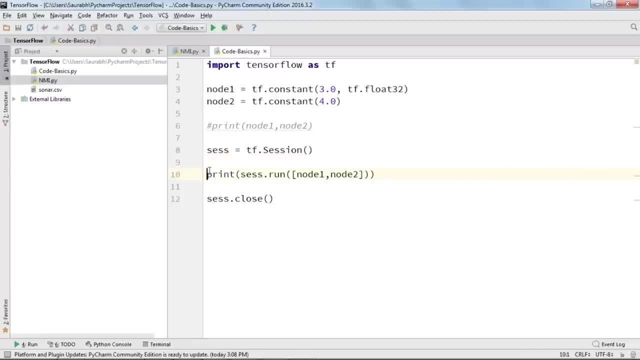 So let me show you how you can do that. For that what I am going to do, I am going to first comment this line, Even this line. So for that what I am going to use, I am going to use the with statement of python. 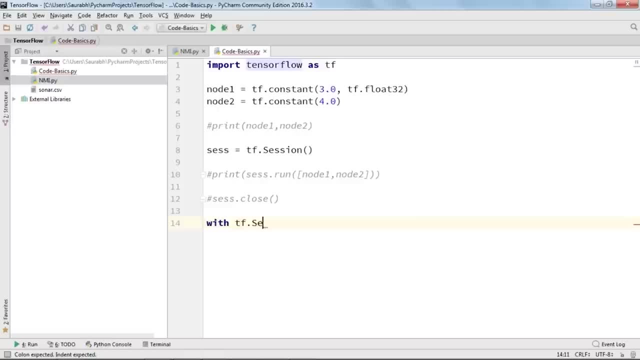 So for that I will type in here with tfsession as ses output equal to sesrun, Node 1, comma, node 2.. Go ahead and print the output. So if you are not familiar with what this does, Basically it will use the session for the block of code following the statement. 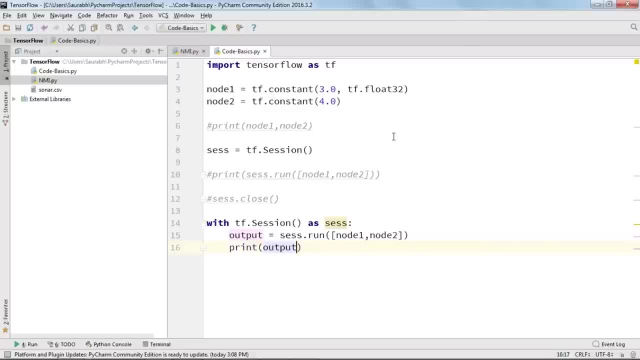 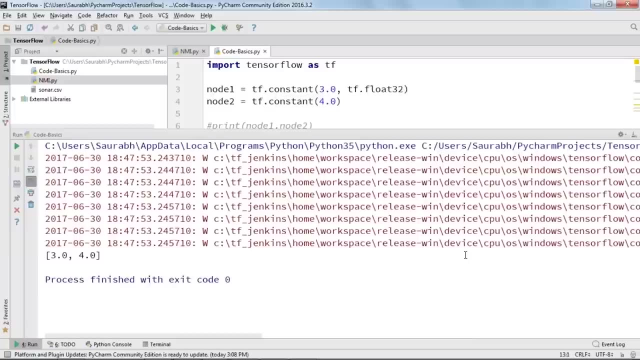 And then automatically close the session when done. The same way it works if you open a file with the with statement. So let us go ahead and execute this and we will see what happens. So again we have got the same output: 3 and 4.. 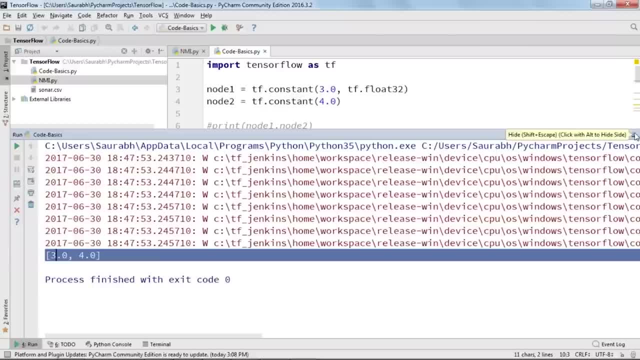 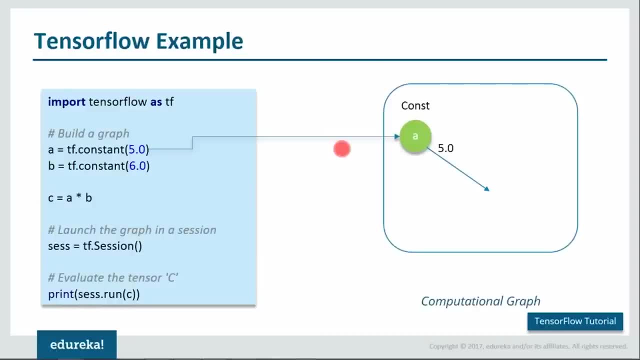 So I have explained you a couple of ways in which you can start and stop a session. So, guys, let me explain you this with one more way, So one more example, for that I will open my slides once more Here. I have first defined a constant node, A, which has a value 5 in it. 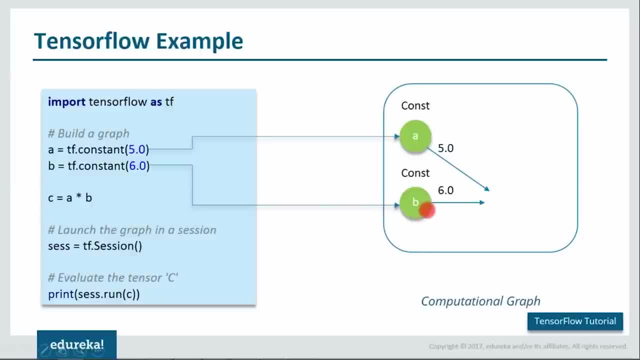 Then I have defined one more constant node, which is B, And the value stored in that node is 6.. After that, I have defined one more node, and this is nothing but the multiplication of A and B. So till now, we have built our computation graph. 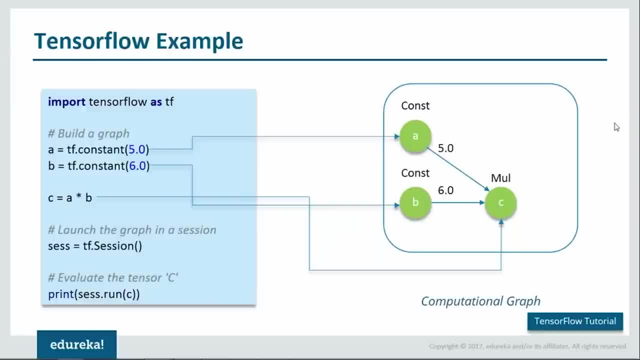 Next up, we need to run it inside a session. So when we run the session, what will happen? The values that are stored in A And B will be multiplied. Let us see if that happens. Yep, So after running the session, we got the output as 30.. 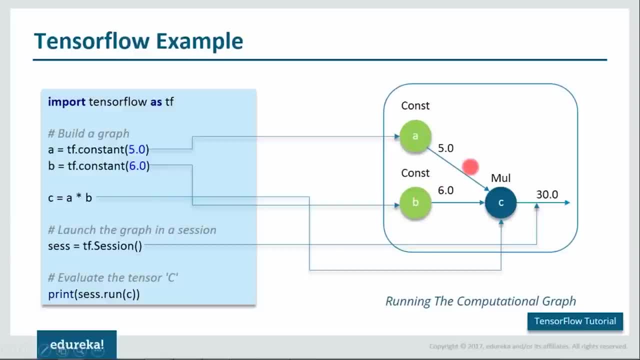 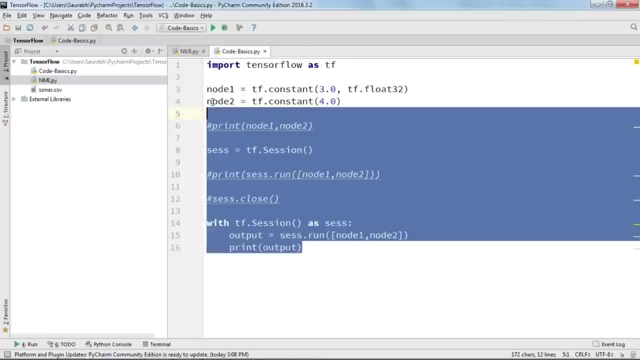 Which is nothing but the multiplication of A and B. So when you multiply 5 by 6, obviously you will get 30.. Now, guys, I will open my PyCharm and execute this practically. Let me remove all of this. So first I am going to define one constant node. 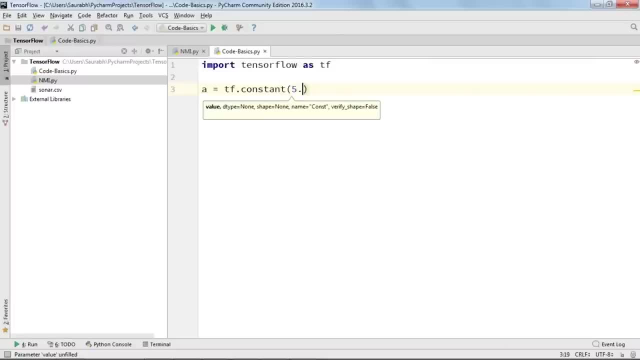 The value that will be there will be 5.0.. One more constant node. The value inside that node will be 6.0.. Then C is nothing but the multiplication of the two nodes. So we have built our computation graph. Next up we need to create the session object which will launch the graph. 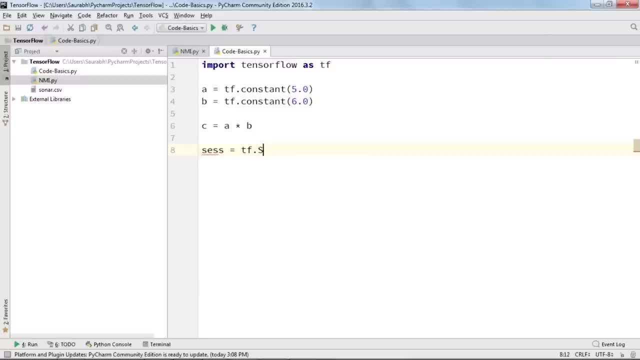 So S is equal to tf dot session. So, guys, you can even use a with statement of Python in order to do that. But yeah, I am comfortable with this, so I will continue from here, And then what I need to do is just run the session. 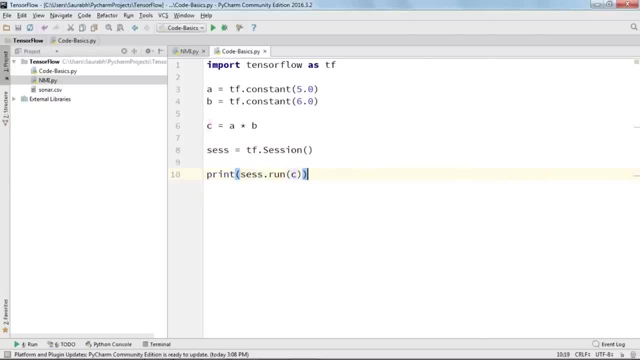 Sess dot run C. That's what I want to compute. And, yeah, finally, just close the session. Sess dot close. Go ahead and execute this. So we have got the output as 30, which is nothing but the multiplication of nodes A and B. 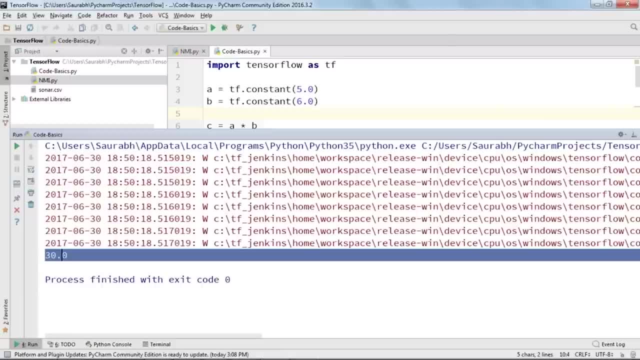 Which stores the value 5 and 6 respectively. Now I know, multiplication of two numbers is not a big deal, But it is a good example for understanding how things work in TensorFlow. Now what if I tell you that you can actually visualize a computation graph? 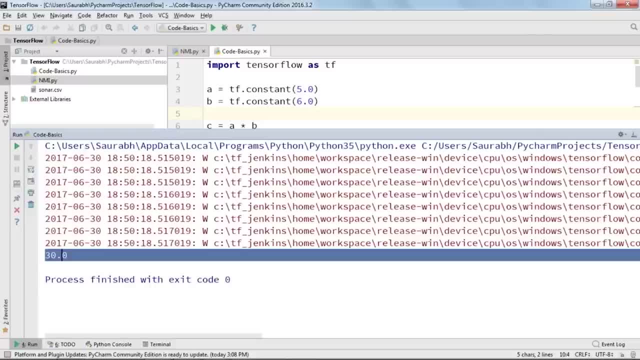 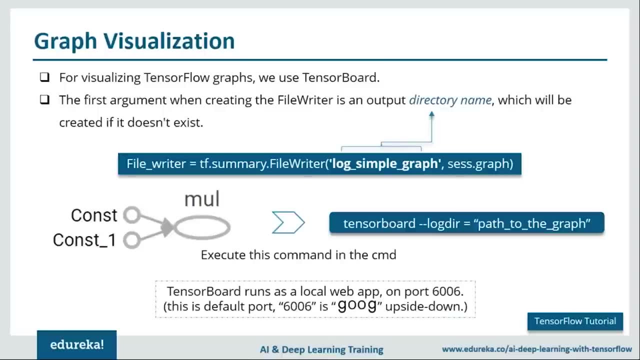 Let me tell you how. For that I'll open my slides. So for visualizing TensorFlow we use TensorBoard. TensorBoard is a suite of web applications for understanding your TensorFlow graphs. For that, what we need to do, we need to first create the object of class for writing summaries. 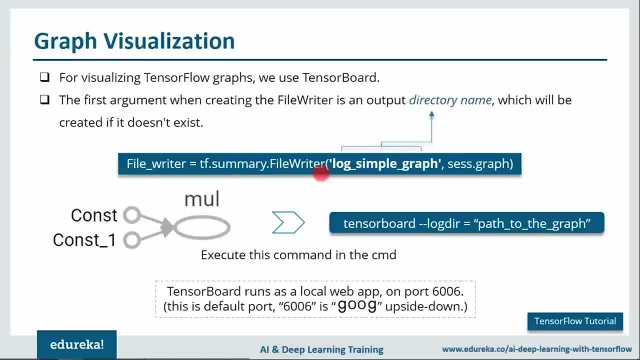 One such class is called file writer. So it has two arguments. The first argument: we need to just specify the path of the directory where we want the information to be stored That will be used by TensorBoard in order to build the graph. After that, we need to run this particular command in the command line. 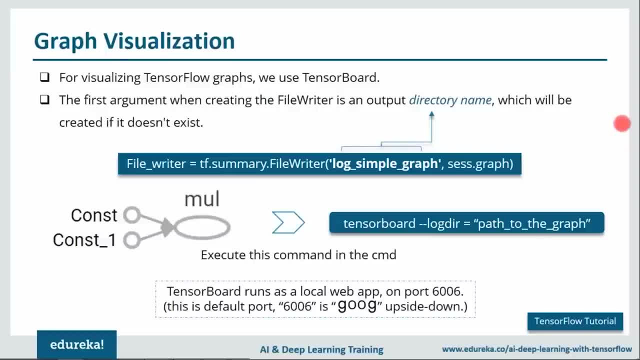 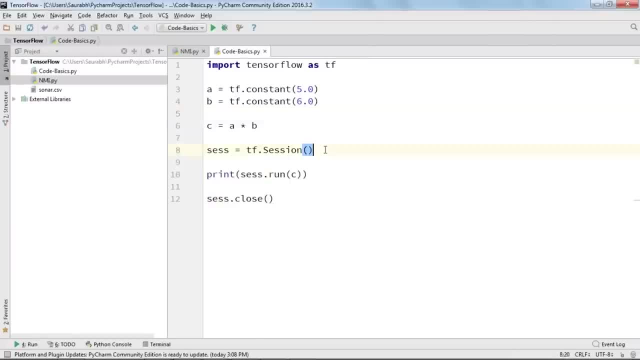 And we'll see that TensorBoard will run as a local web app on port 6006.. So I'll quickly open my PyCharm and I'll execute this practically. Let me close this. Yeah, So after that I just need to create an object. 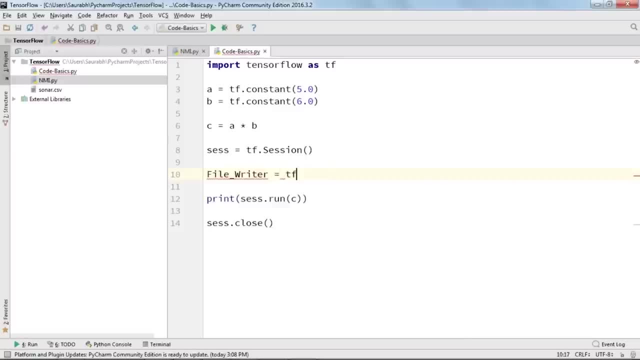 File writer. object: File writer equals to tf dot summary dot file writer And I need to provide a path here. So I've already copied the path. I'll just paste it here And once you have written the path, just type the name of the file. 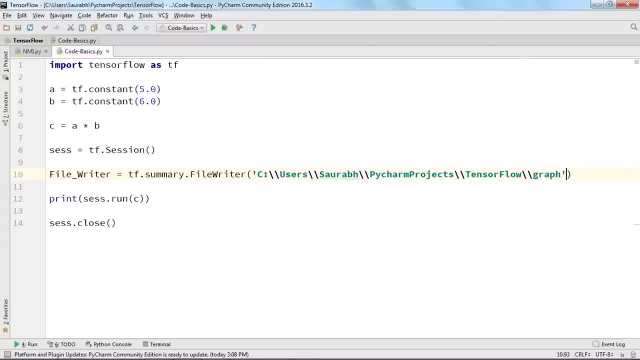 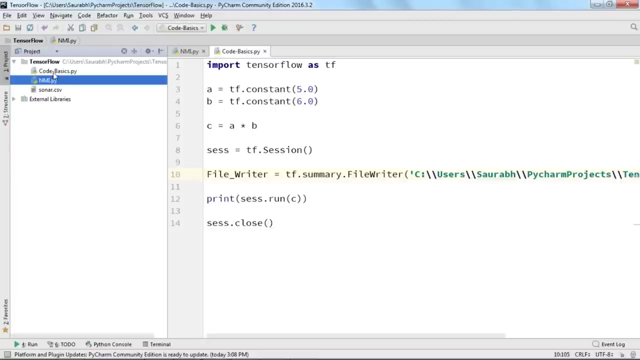 So I'll just type in here graph, And after that I need to add: says dot graph, which is used for creating a graph object. So just type in here: says dot graph. All right, So now, if I execute this, I'll see a directory here by the name of graph. 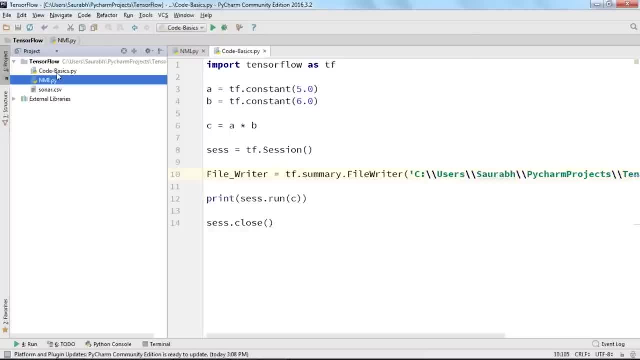 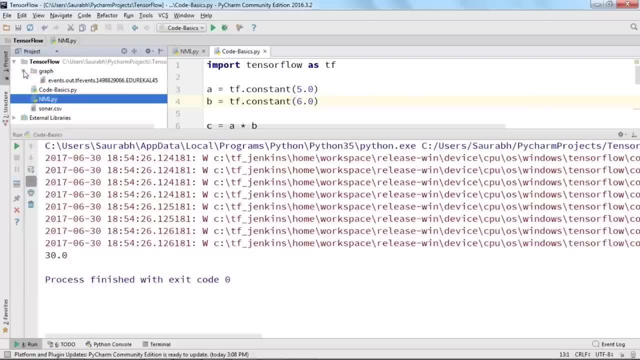 That will contain the information which will be used by TensorBoard in order to build the graph. Let us see if that happens or not. I'll run the code And, yeah, you can notice here that there is one more directory created that is called graph. 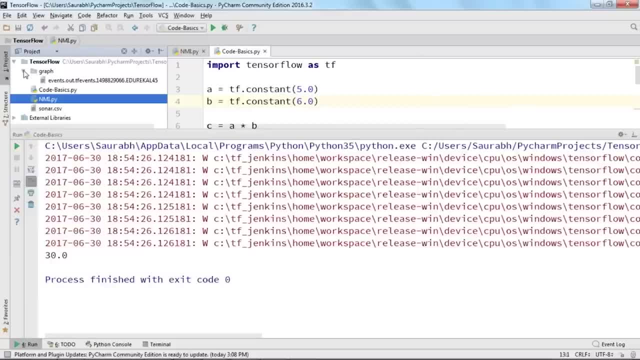 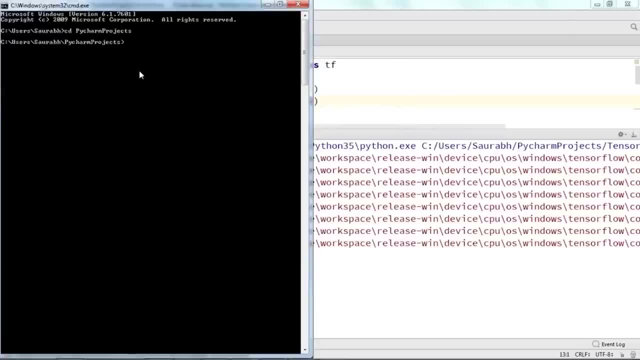 Next up, we need to open a command line and execute one command. Let me show you how you can do that. So over here, first I'll move in the PyCharm directory, Yeah, And then I'm going to type in here: TensorBoard- hyphen. hyphen- log dir equal to the path TensorFlow. 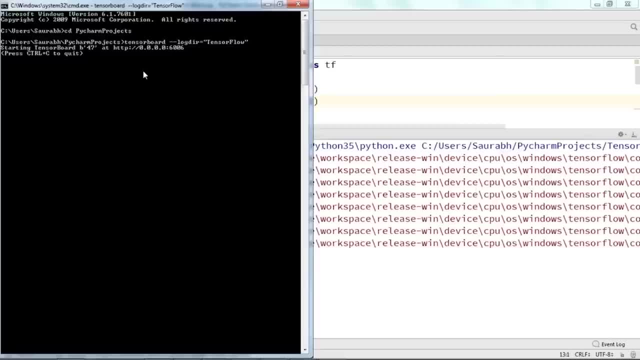 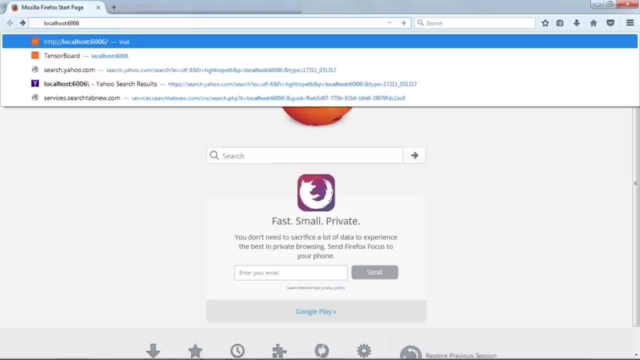 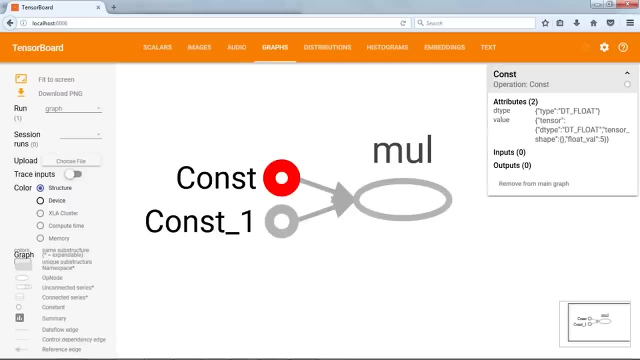 Just go ahead and execute this. So it says that TensorBoard runs as a local web app at port 6006.. Let us see how our graph looks like now. So this is how our graph looks like. It has two constant nodes here and one node for multiplication. 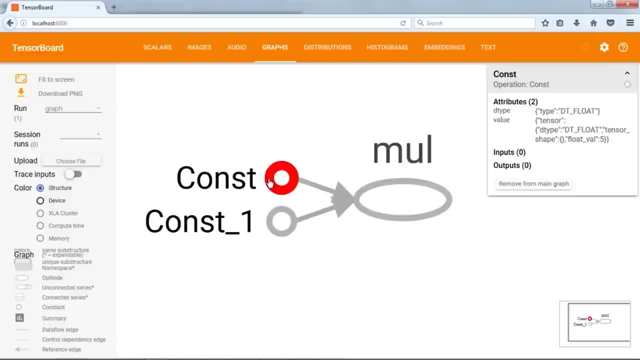 So when I click on each of these nodes, there will be some information displayed about that node. So if you notice, here it is a float type. It also contains the value that is stored inside this particular constant, Which is 5.. There are zero inputs and zero outputs. 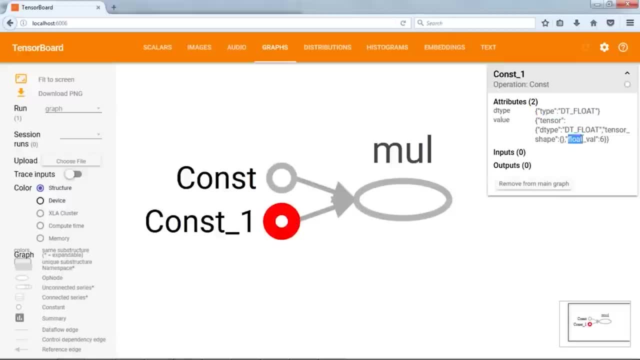 Similarly for this constant node as well. It is a float type and it holds the value 6.. Similarly, when I click on this particular node, we can see that it is again float type And it has two inputs: const and const underscore 1.. 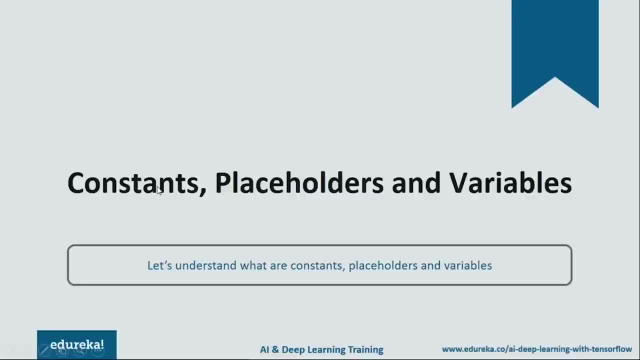 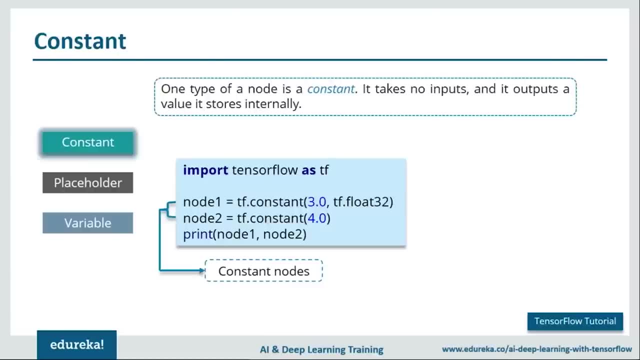 So these two inputs will be multiplied and will get the output. And now is the time to understand what are constants, placeholders and variables. So constant, as a name, tells that it will always produce a constant result. So I'll explain this as an example. 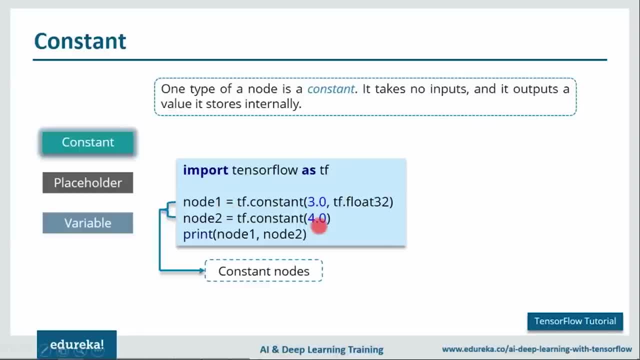 So over here we have a couple of constant nodes. First node has values 3.. Another node has value 4.. So when I execute this particular graph, I will always get the values 3 and 4.. Or you can see the values that are stored inside these two nodes. 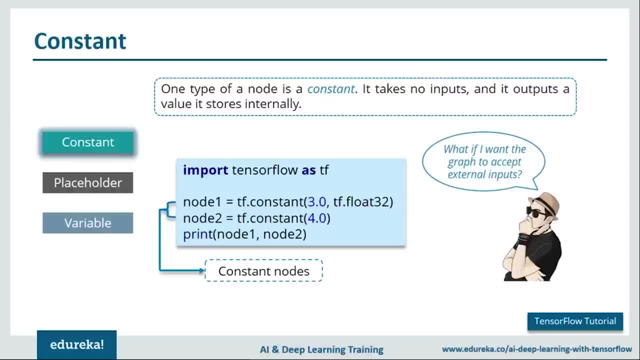 Now what if I want my graph to accept the external input? Now let me explain that with an example of our use case only. So here we want the features to be fed back to the graph That we cannot do with the help of constants. 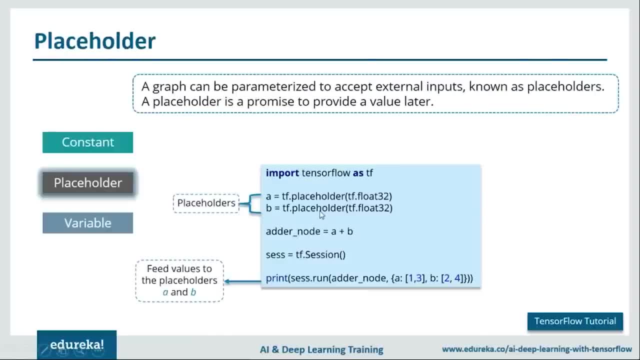 For that what we need. We need placeholders Now. a placeholder is nothing but a promise to provide a value later. Let us understand this with an example. So over here we have a couple of placeholders, A and B- of float 32 bits, And notice that we have initialized no values. 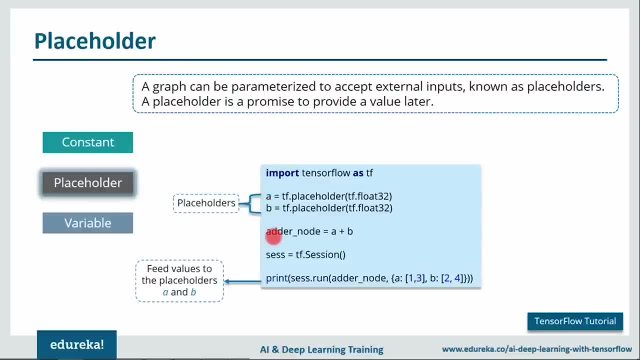 Then we have one more tensor adder underscore node, which is nothing but the addition of two placeholders. Then we have first launched the session, And when we are running the session we feed in the values of the two placeholders, as you can see here. So the value that will be fed back to the placeholder A is 1 comma 3.. 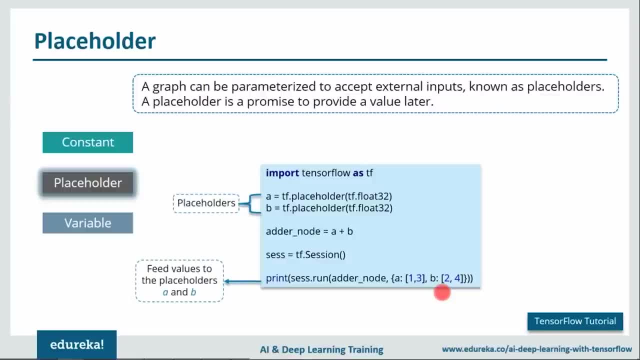 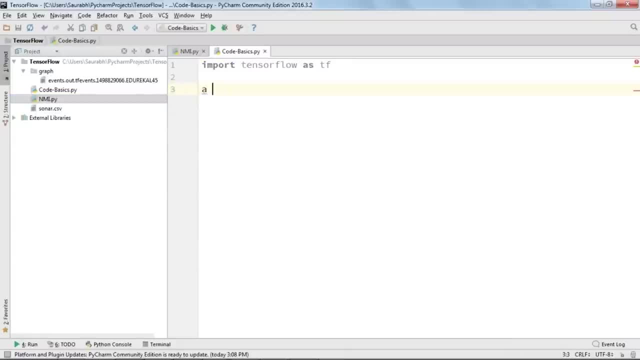 The value that will be fed back to the placeholder B will be 2 comma 4.. Now let me execute this practically in my PyCharm. Let me remove all of this, Alright. So I will define a placeholder A- tf dot placeholder, which is of float 32 bits. 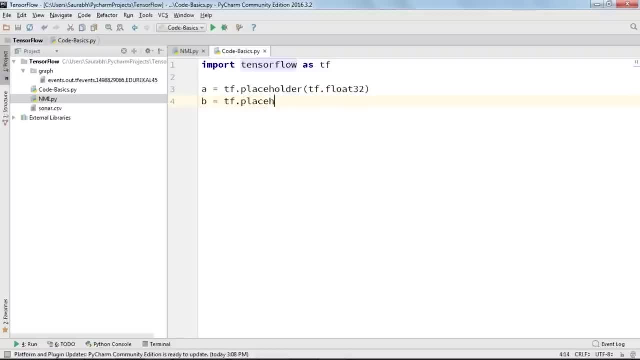 Similarly, B will be again a placeholder of tf dot float 32 bits. Then we define one more node, adder, underscore node, which is nothing but the addition of these two placeholders. Next up we need to launch the graph. For that I will type here: ses is equals to tf dot session. 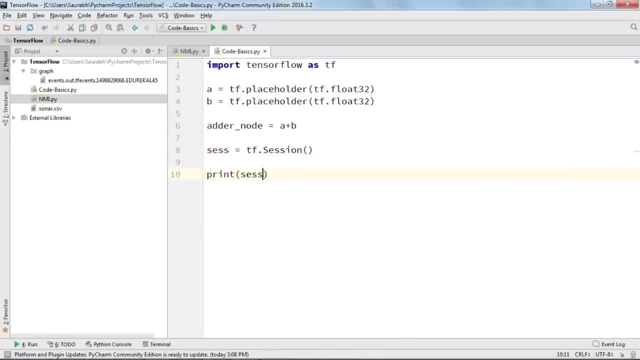 And next up we need to run the graph, Print, ses, dot, run and adder underscore node And we need to feed the values of A and B as well. So for that I will type in A 1 comma 3, B 2 comma 4.. 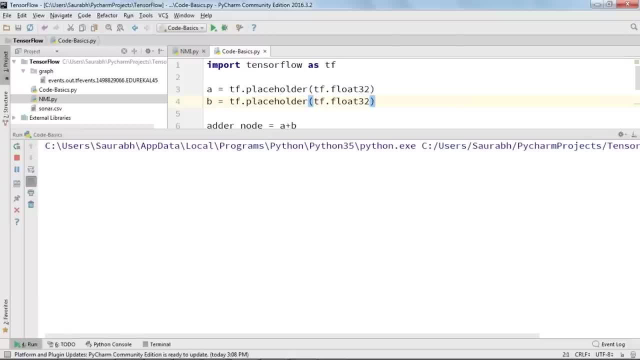 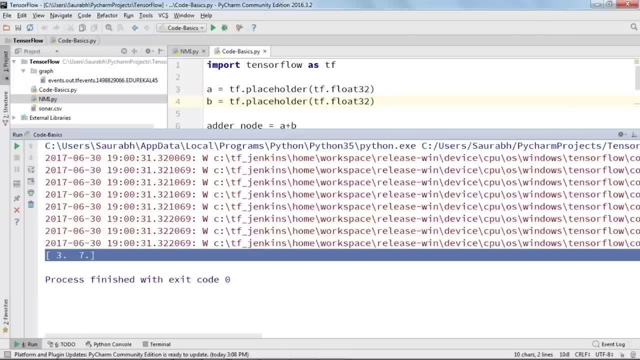 Now let us go ahead and execute this and see what happens. So here, if you notice, I get the output. as you saw earlier, I get the output as the sum of the two placeholders A and B. So the first value, 1, will be assigned to the placeholder A and value 2 will be assigned to the placeholder B. 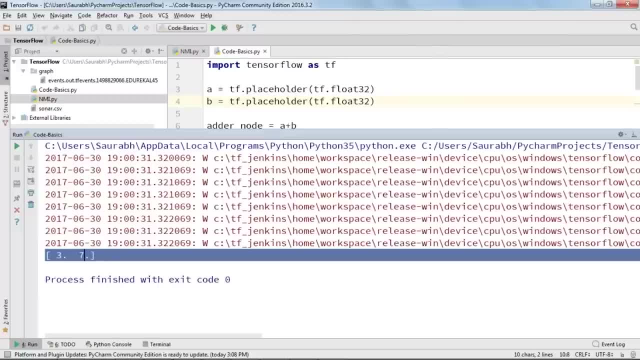 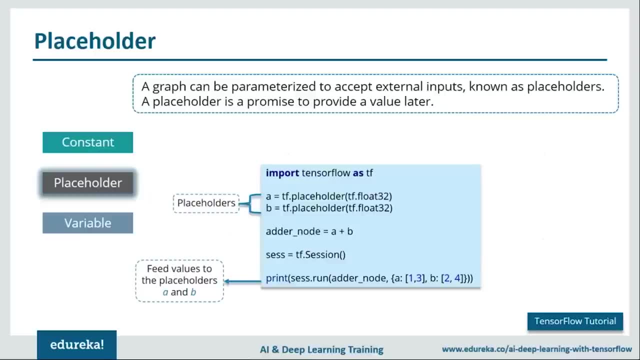 So their sum will be 3.. Similarly, A will be assigned to the value 3 and B will be assigned with value 4.. Hence, their sum will become 7.. Now let us get back to our slides once more. Now the question here is how to modify the graph if I want new output for the same input. 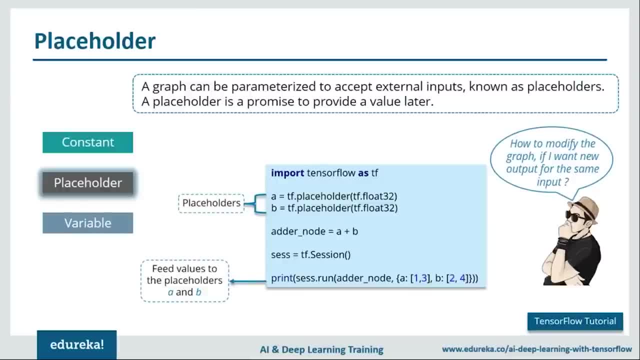 I mean, if I want my model to become trainable, I need some parameters that can change after input, So that I can change every iteration, So that the model output can be as close as possible to the actual output. For that we need variables. Now variables, as the name explains: the value of the variable will keep on changing. 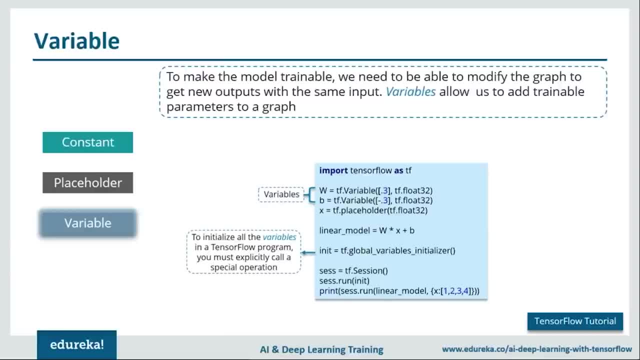 When you train a model, you use variables to hold and update parameters. Variables are in memory buffers containing tensors And remember they must be explicitly initialized, unlike constants and placeholders. So let me explain you the code that is there in front of your screen. So here we have two variables, W and B. 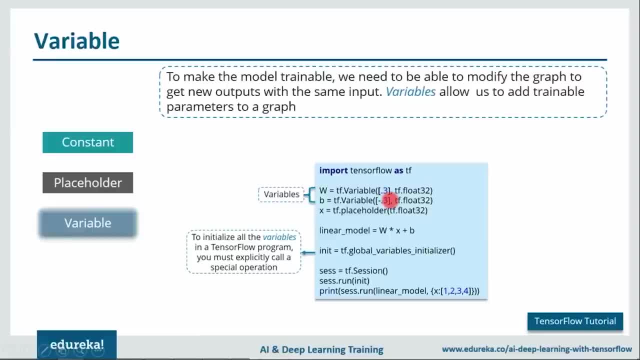 And I have initialized both of these variables with value 0.3 and minus 0.3.. So if I train my model, the values of these two variables should change in order to reduce the output. Don't worry, you will actually understand that when I explain you the loss function and optimizers. 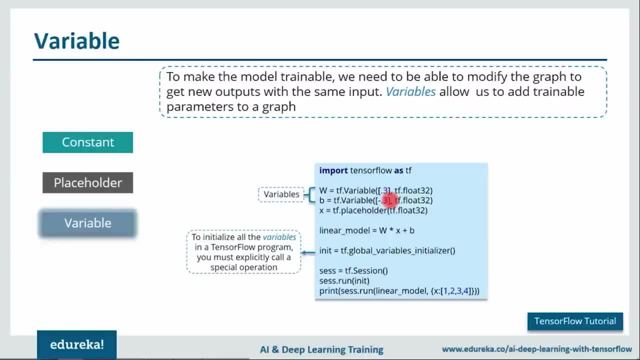 There you will understand how we actually train our model and how actually variables are updated after every iteration. In order to initialize the variables, we use tfglobal underscore variables underscore initializer. This will add an operation to initialize the variables. Then we run ses dot, run init. 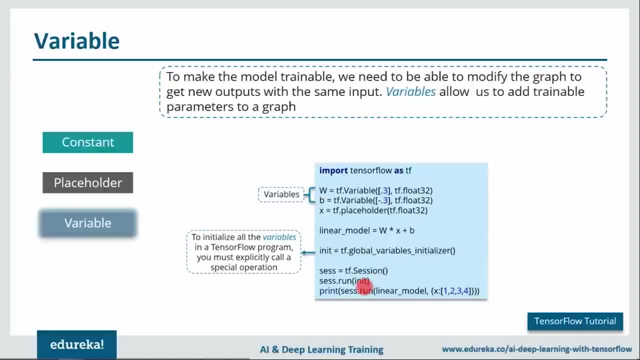 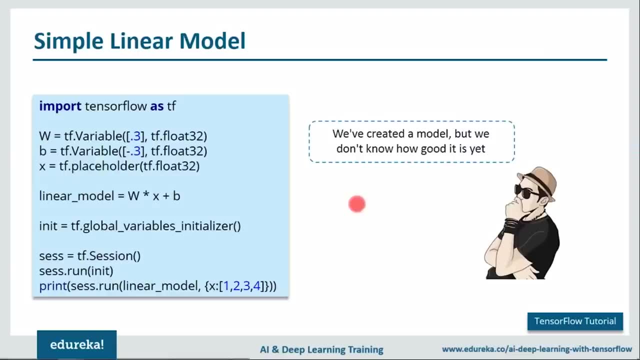 This will run that operation And remember, we only run it after launching the model. For now, let us go ahead and execute our first model. So this is our first model, guys Over here. we have imported the tensorflow as tf. Then we have defined couple of variables, W and B. 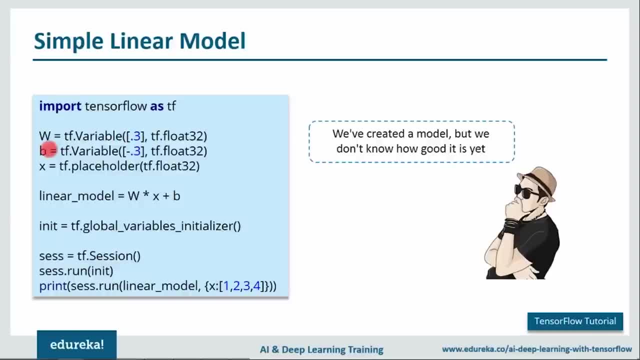 And we have initialized them with 0.3 and minus 0.3 values respectively. Then we have a placeholder X. After that we have defined one linear underscore model which is nothing but W into X plus B. Then we have initialized the variable. 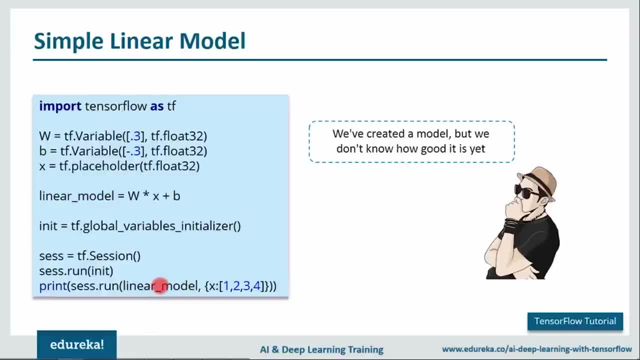 We have launched the graph and then we are running the session, And during that we are running the session and feeding the values of X. So this is basically what our model is, But we don't know how good it is yet, So obviously we cannot increase the efficiency without knowing the error. 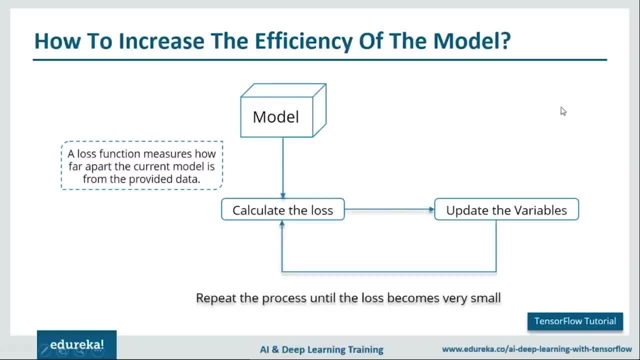 Let's understand the general flow of how we increase the efficiency. So first we create the model, as you have seen in the previous slide. Then we calculate the loss. Loss is basically how far our model's output is from the actual output. Then we try to reduce the loss by updating the variables. 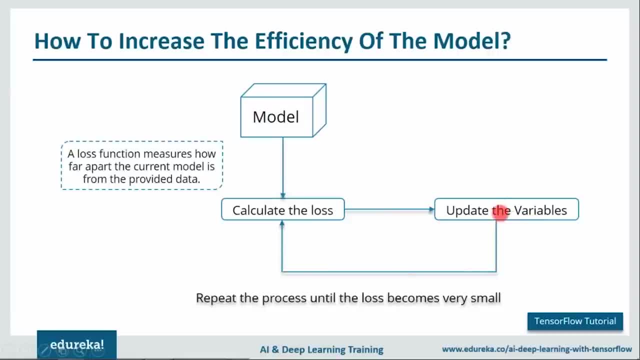 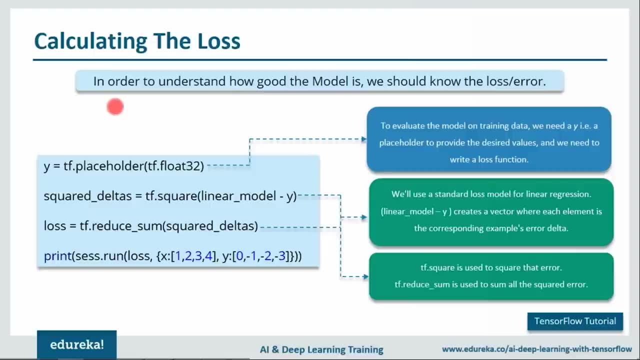 Then again we check the loss and update the variables, And this process keeps on repeating until the loss becomes minimum. And now is the time to understand how we calculate loss. So in order to find out the loss, we should first define a placeholder, And we have named it as Y. 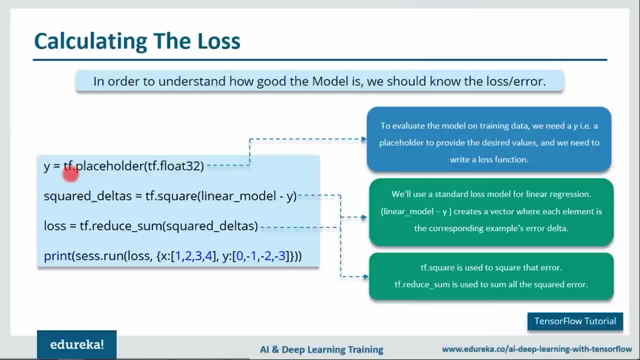 Which will hold the desired output, or you can say the output that we already know. Then we will find the difference between the linear underscore model or the output of our model with that of the output that we already know, the placeholder Y. Or you can say the difference between the model and the output of our model. 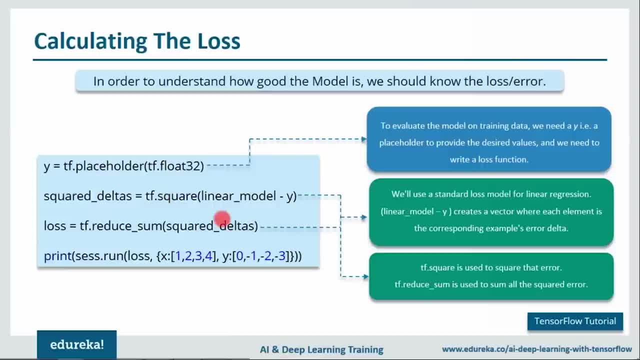 The model output and the actual output. Then we find the square of that particular difference And then, finally, we sum all the squared errors that we have calculated in the above line. So we'll sum all of these squared differences. Then what we have done, we will run the session, calculate the loss and we'll feed in the values of X and Y. 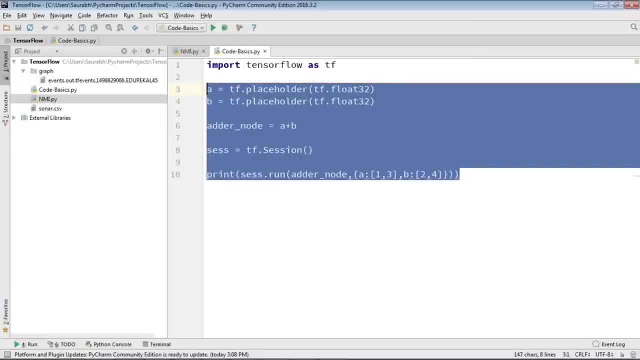 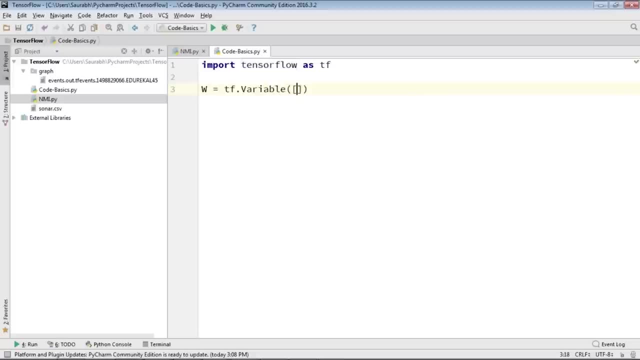 So I'll execute this practically. For that I'll open my PyCharm. Let me remove all of this. So yeah, first we'll define a variable, tfvariable, with the initial value as 0.3.. And it is tffloat- 32 bits. 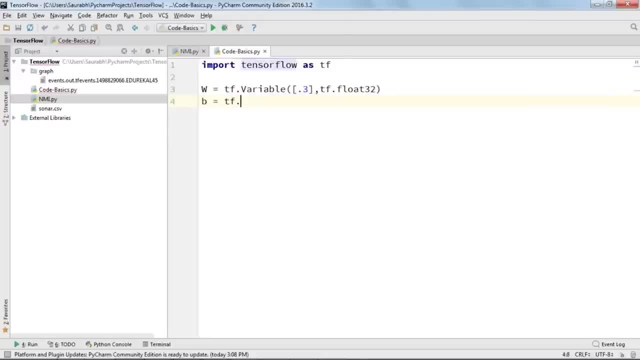 Then we will define one more variable: tfvariable minus 0.3, tffloat 32 bits. Then we'll define a placeholder that we will use in order to provide the inputs or to feed in the inputs. So let me throw in a comment here. 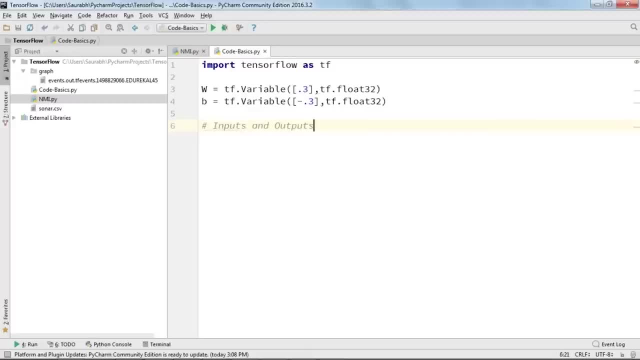 Inputs and outputs. And I can throw in one more comment here which says model parameters. Alrighty then. So now we'll define a placeholder X, which will actually hold the input values, tfplaceholder. It will be of float type 32 bits. Then we'll define one more placeholder, Y, which will actually hold the actual output of the model which we already know. 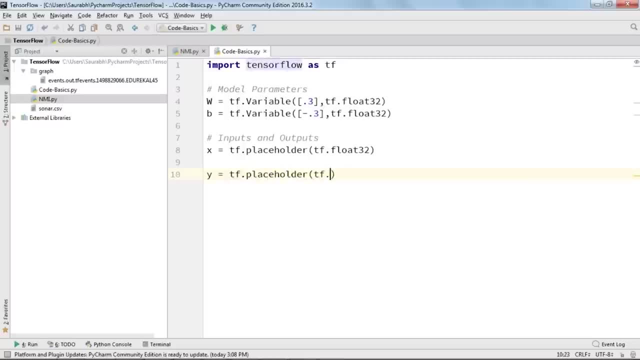 Placeholder tf float 32 bits, Alright, And just between that we'll define one more node linear underscore model which will give the output of this particular model, which we don't know. So that's the difference, guys. This Y is a placeholder and the values to this Y will feed in when we are running the session. 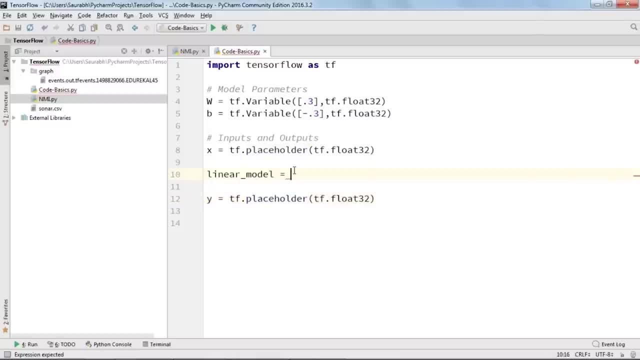 So that will be the actual output of the model, And this will be the output of the model which will come after executing the model. So this will be nothing but W into X plus B. Fine, And now we are going to define the loss function. 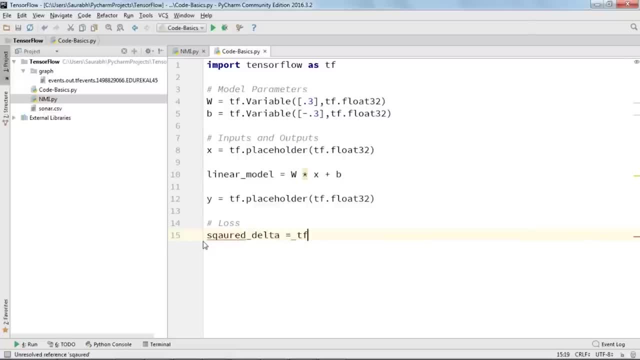 So I'll type in here: squared underscore delta is equals to tf dot square linear underscore model minus Y, which is nothing but the model output and the output that we already know. So linear underscore model is the output that we'll get through our model And Y is a placeholder which will have the output values that we will feed in. 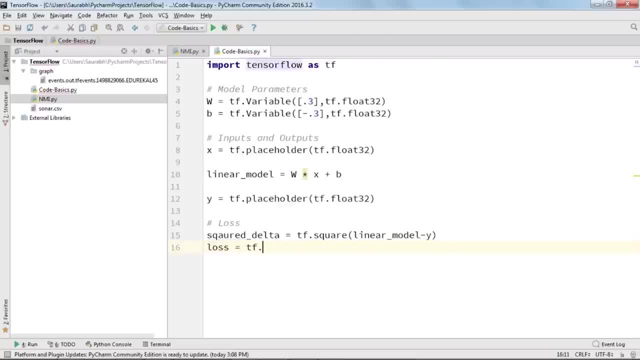 Then we are going to define a loss function. So loss is equals to tf dot reduce underscore sum of all the square delta. So we have defined a loss function here. Next up, what we need to do is initialize all the variables. For that I'm going to type in here: init is equals to tf dot. global underscore variables- underscore initializer. 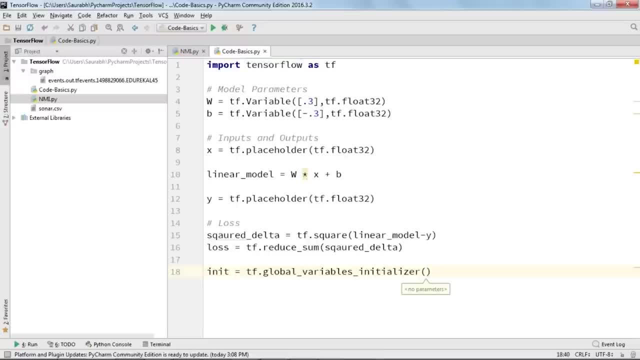 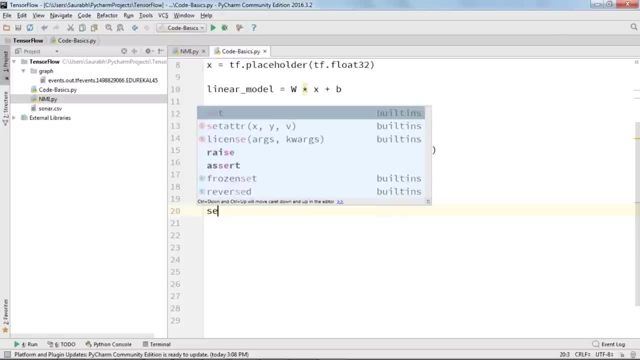 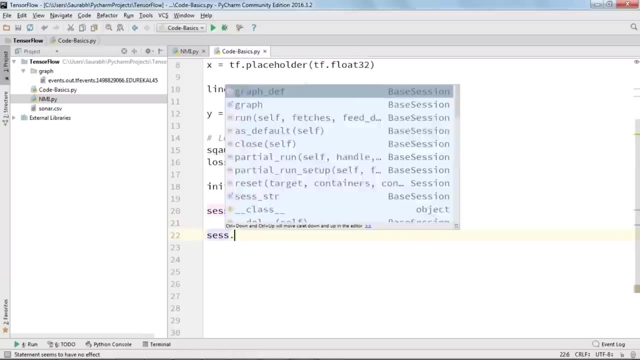 So this global variable initializer will add an operation to initialize a variable. Now we need to launch the graph For that. we need to create a session object, And we know how to do it. ses is equals to tf dot session. Yeah, And now we are going to write in here: ses dot run init. 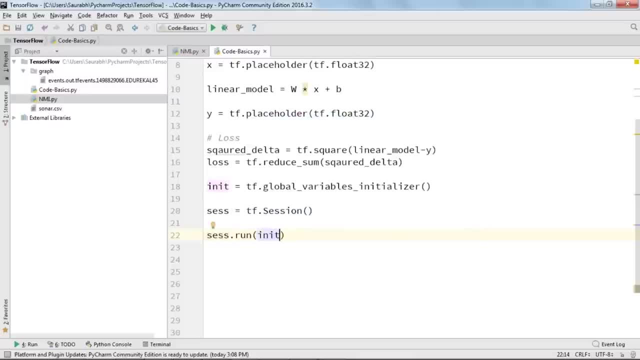 So this will run the operation that we have defined when we were talking about global variable initializer, And after this our variables are initialized. So now what we need to do is just run the session. ses dot run Calculate. Calculate the loss Feed in the values of x. 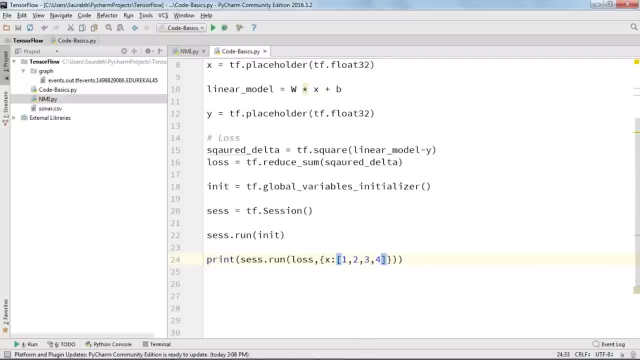 So let it be 1 comma, 2 comma, 3 comma, 4.. And now the placeholder y Feed in the value of placeholder y, So we will keep it as 0 comma minus 1 comma minus 2 comma minus 3.. 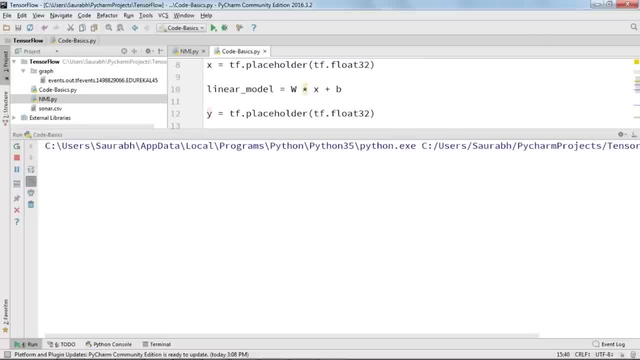 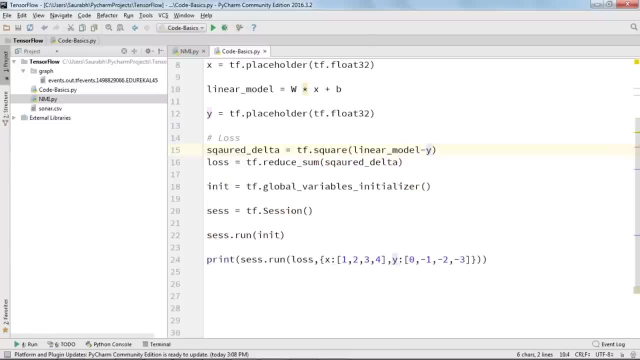 Now let us go ahead and see how much is the loss. So the loss that we have calculated is 23.66.. And let me just close this once. So over here, if you notice, if I change the value of w and b, I can actually reduce my loss. 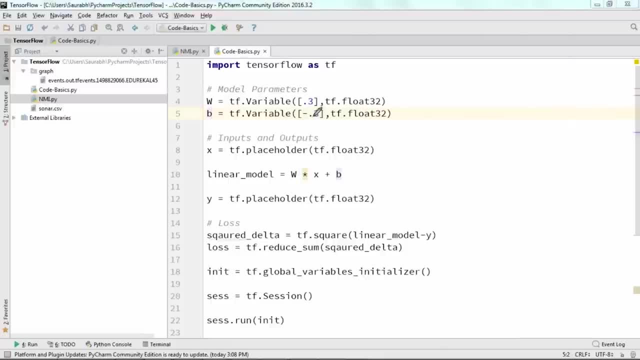 Let me show you how I can do that. I will take a pen. So instead of 0.3 and minus 0.3.. If my w becomes minus 1. And my b becomes 1. Then linear underscore model will become equal to y. 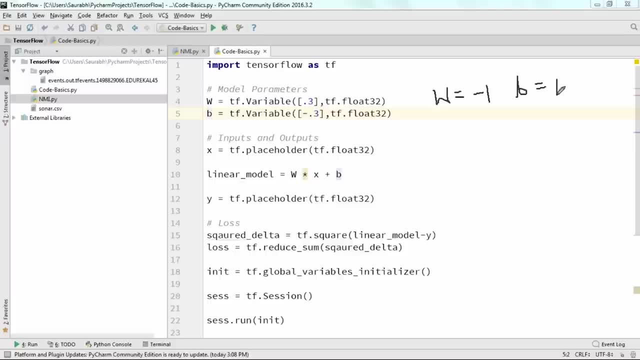 That means the output of our model will actually become equal to the actual output That we know. So let me tell you how it will happen. So our linear underscore model is w into x plus b. So we will take the values of x one by one. 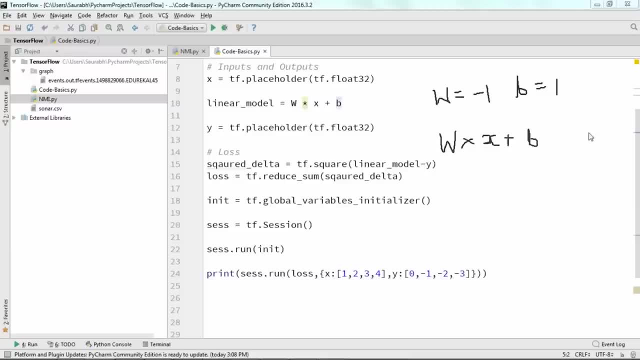 So the first value of x is 1.. So let me take that first. And the value of b is minus 1.. So minus 1 into 1, plus 1 is equal to 0. So the value of our linear underscore model. 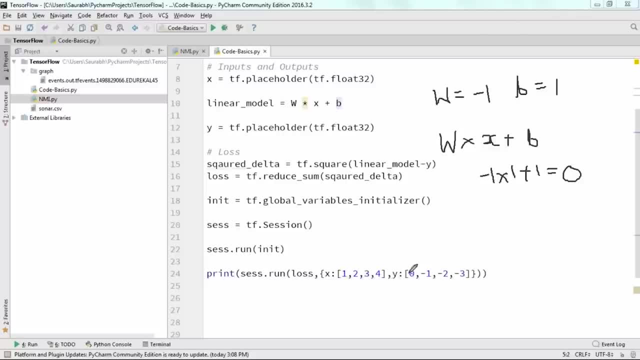 Is 0.. And over here also the value of y, That is our placeholder, or the actual output, is also 0.. Let us take the next value of x, Which is nothing but 2.. 1 minus 1 into 2 plus 1 is equal to what? 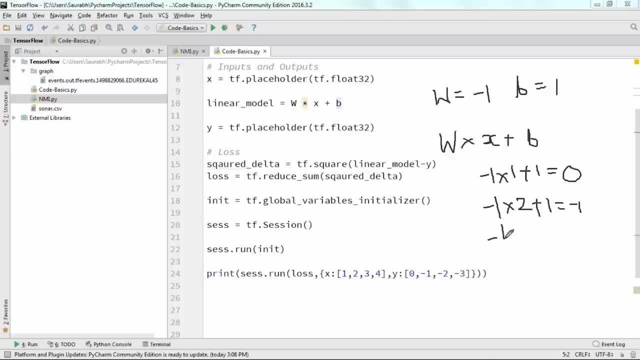 Minus 1. Which is again equal to y. Similarly, minus 1 into 3 plus 1 is equal to minus 2., Which is also equal to our placeholder 1. Y. Finally, if I take the last value of x, 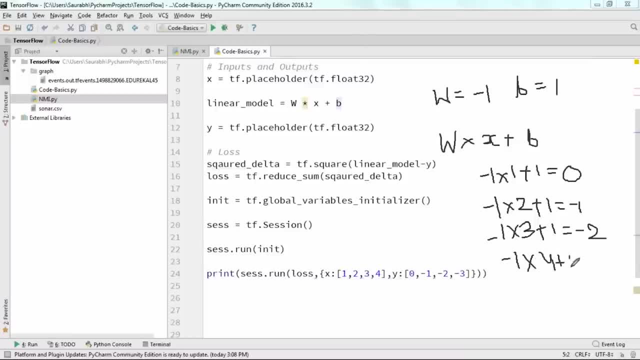 Which is 4 plus 1. It will be equal to minus 3.. So this is how, when we update the variables, We can actually reduce the loss. So here, if I keep the values of w and b as minus 1 and 1 respectively, 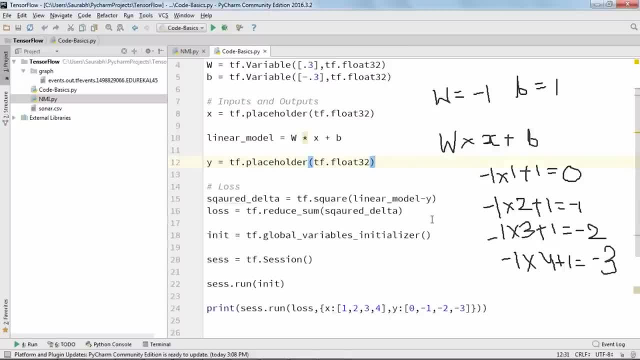 The loss that I will get will be 0.. So this is how you can actually reduce the loss: By updating the variables. So when I was explaining variables, Where I told you That in order to make the model trainable, We need to update the values of variables, 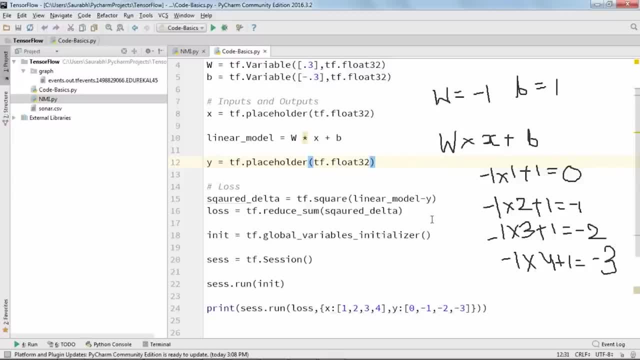 This is what I was talking about. So by changing the value of variables We can actually reduce the loss. We can make the model output as close as possible to the actual output. Now, if I make this as minus 1.0.. And this as 1.0.. 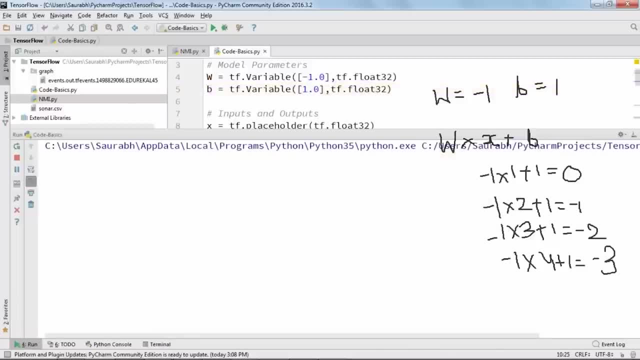 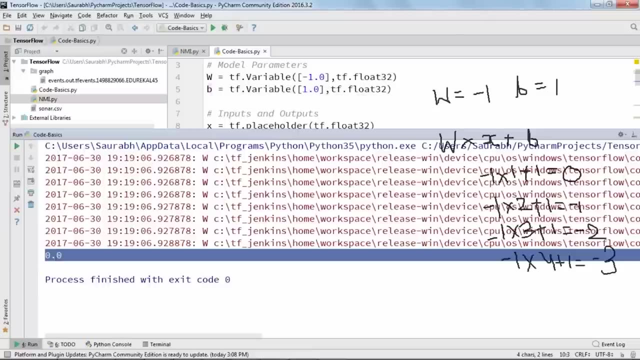 We should get 0 error. Let us see if that happens or not. So we have 0 loss. But over here I have manually done it. I have manually updated the variables So we can actually reduce the loss of w and b. 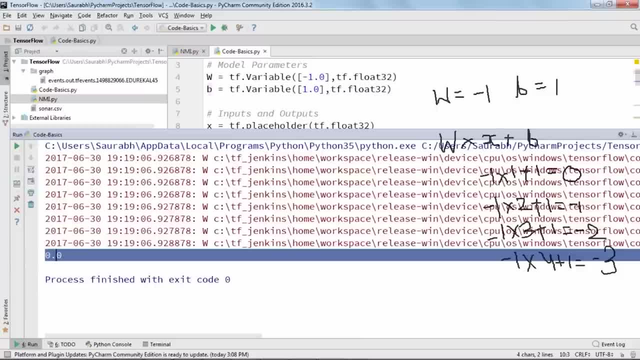 What if I want my model to do it on its own? What if I want the machine to learn the new values of w and b? That will minimize the loss. So at that time we need optimizers. So for that I will open my slides once more. 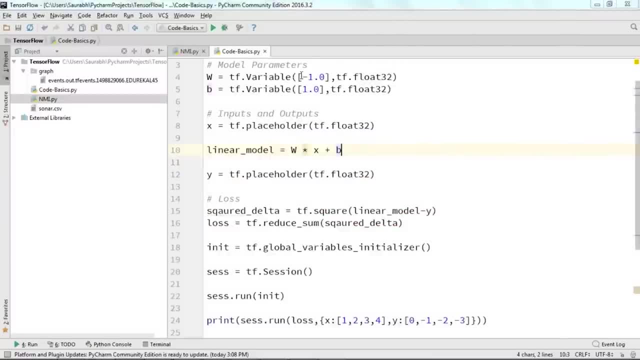 Let me remove all of this, Yeah, and keep this to its normal value, 0.3.. It was plus 0.3.. Yeah, and this will be minus 0.3.. Now I will open my slides. So, in order to increase the efficiency, 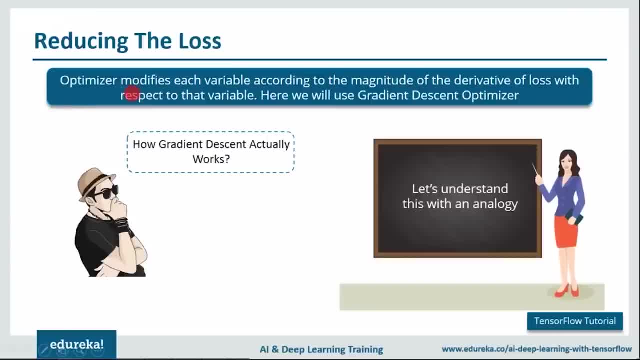 And minimize the loss And update the variables, We use optimizers. These optimizers modifies each variable according to the magnitude of the derivative of loss with respect to that variable. Now, what does that mean? It means, basically, that an optimizer will check the magnitude of the derivative of loss. 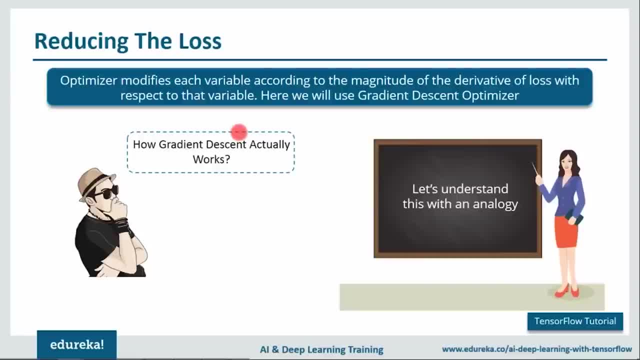 That means an optimizer will check the change in the loss with respect to the change in the variable, And if the loss is decreasing, Then it will keep on changing the variable in that particular direction. So here we will use gradient descent optimization. Let us understand this with an analogy. 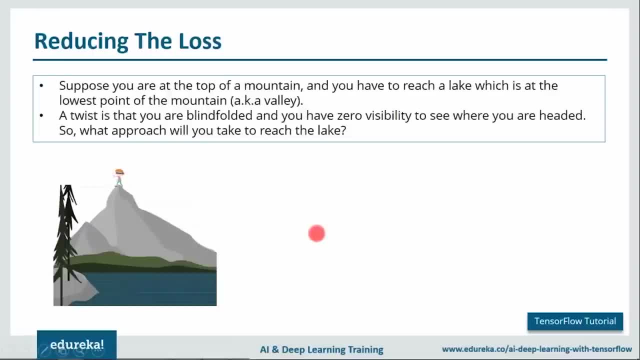 Suppose you are at the top of the mountain and your task is to reach the lake Which is present near the valley, And the catch here is that you are blindfolded. So how will you approach this task? One way of doing this is to observe the ground near you. 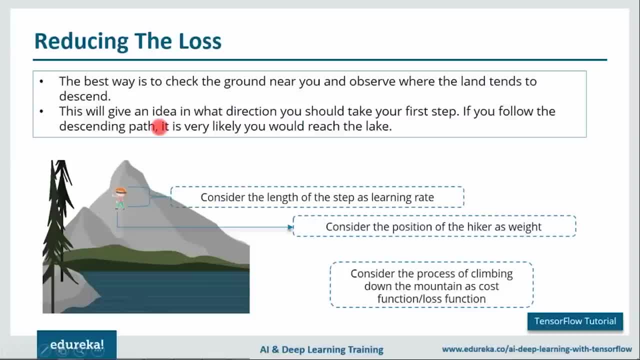 And move in the direction where the land tends to descend. Consider every step that you take as learning rate And the position as weight. The whole process is called as loss function. When you reach the lake, Consider that point as global loss minimum. 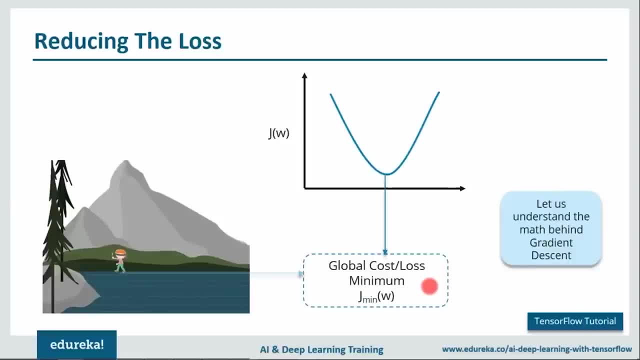 Now you can apply the same concept on our model as well, Where the ground tends to descend. Similarly, the optimizer checks in which direction should the variables be updated So as to decrease the loss And will keep on updating the variables in that particular direction. 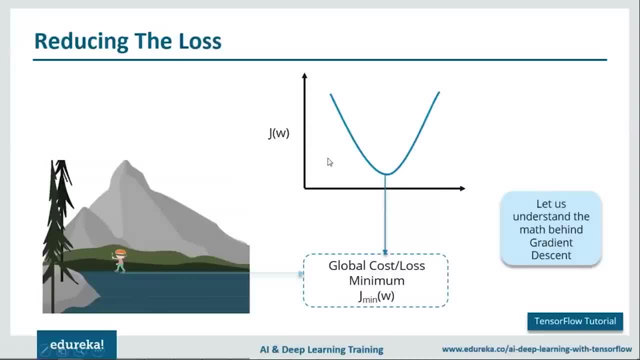 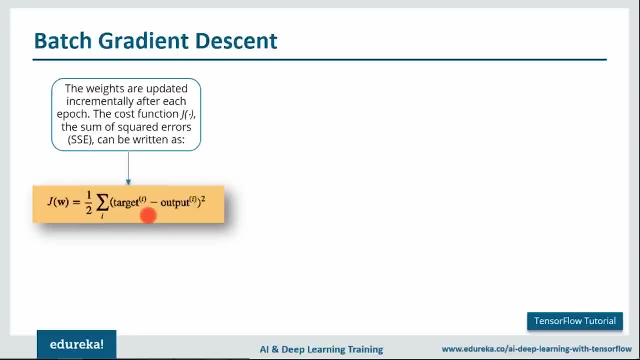 So let us understand the math behind gradient descent optimizer. First we calculate the loss. How we do that? By summing all the square differences between the model output and the actual output And then dividing it by 2. So here our target output is nothing but the output that we know. 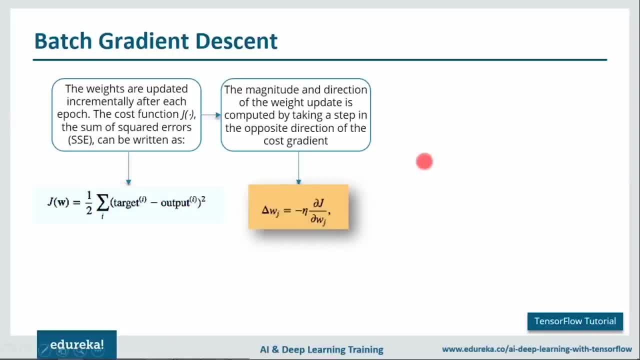 And output is nothing but the model output. After that we calculate the change in the variable delta w. This is equal to the learning rate multiplied by the rate of change of loss with respect to that variable. After that, the new variable or the updated variable is equal to the sum of the change in the variable. 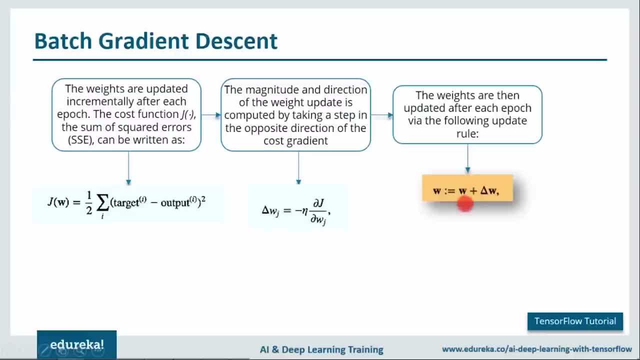 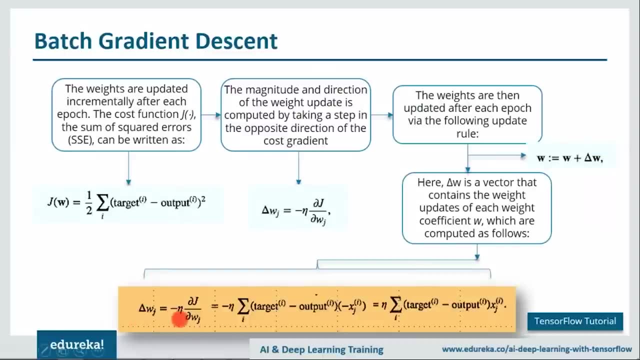 Plus the old value of that particular variable. So it will be w plus delta w. Now let me simplify this Equation for you. So over here, when we are calculating delta wj, Which is equal to minus of learning rate, into delta j by delta wj, 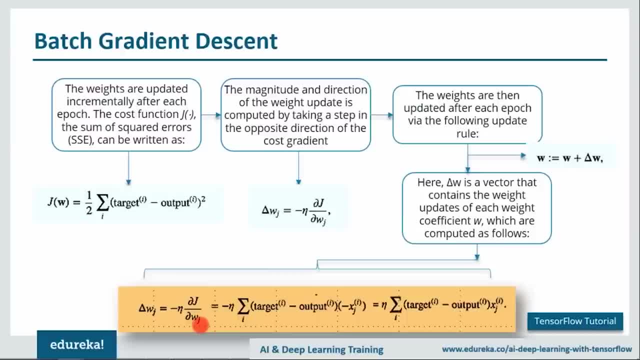 Or you can say the rate of change of error with respect to that particular variable. We put in the values of j, Then we find out the derivative And we get the equation as learning rate into summation of target i minus output. i That means the actual output minus the model output into xj of i. 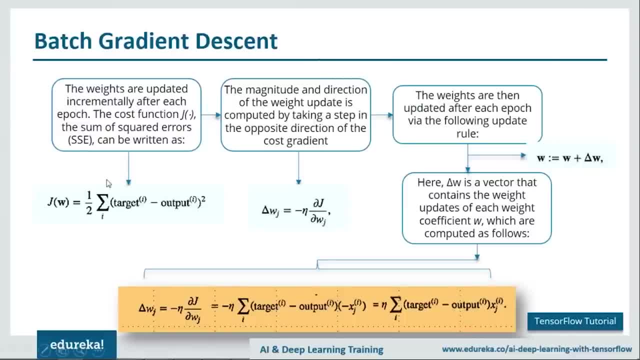 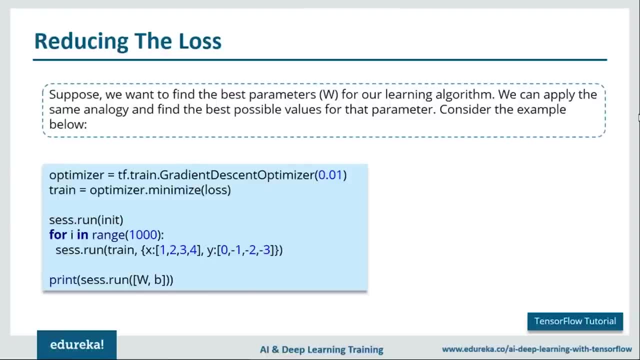 Which is nothing but your input. Fine guys. So we'll move forward and see how we can apply gradient descent In our model. Now, in order to modify the variables in our model, We'll use the code that is there in front of your screen. 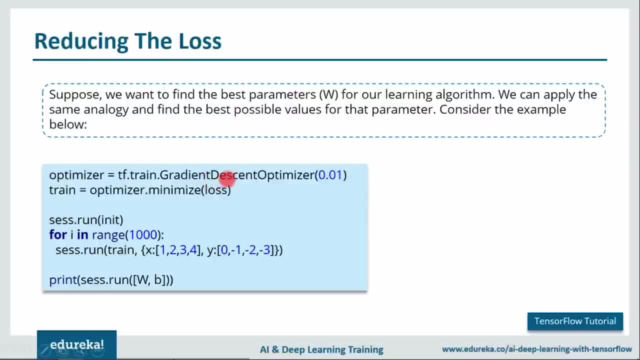 Here we will first create an object of class tf, dot, train dot- gradient descent optimizer And it will implement the gradient descent algorithm. It takes one argument as the learning rate. The second part: this minimize Returns an operation that applies gradients. It will reduce the loss by updating the variables. 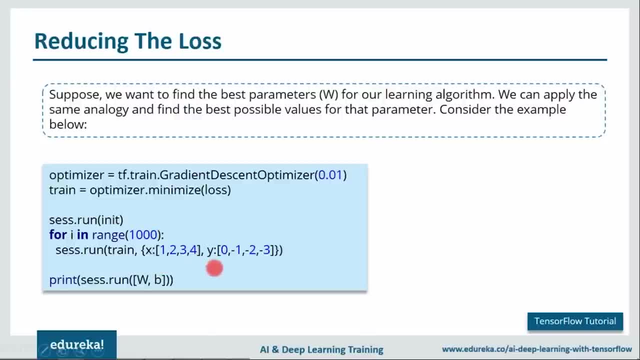 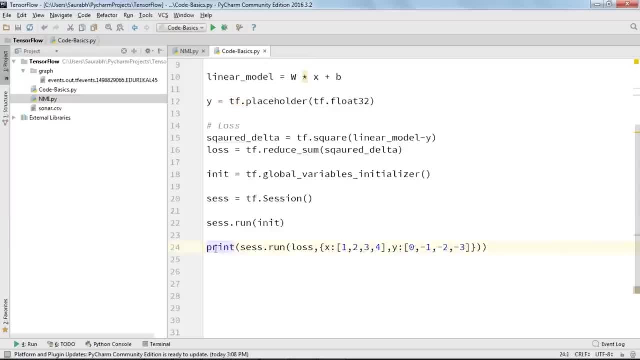 Finally, just run the session and feed in the values of x and y And then evaluate the variables w and j. So let me go to my PyCharm and execute this. Let me comment this line first. So after defining loss, We will optimize our model. 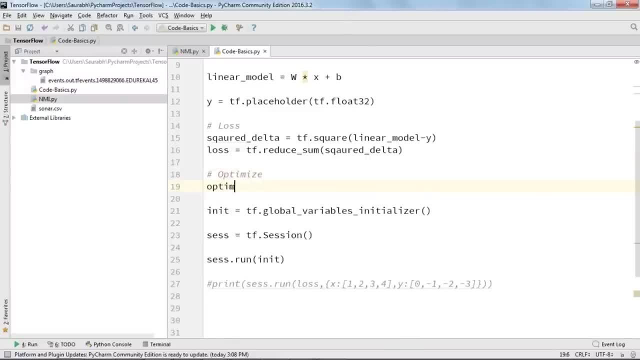 We'll write in here: optimizer equal to tf, dot, train dot, gradient, descent optimizer with a learning rate of 0.01.. Learning rate is nothing but the steps, Steps in which you change your variable. Then, on the other hand, Then what we do. 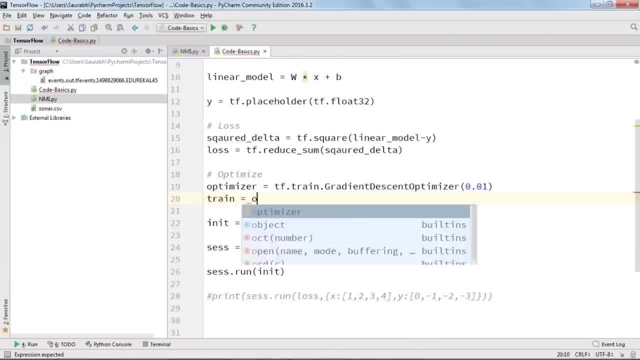 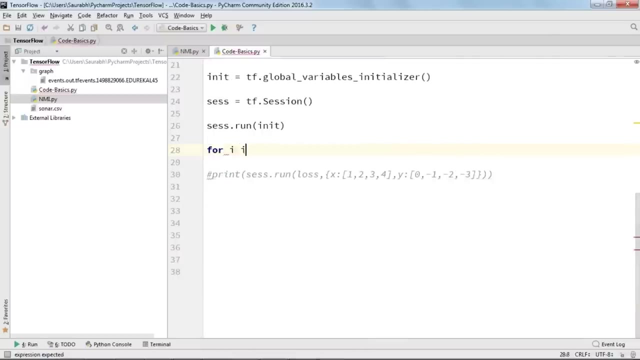 We will write in here: train is equal to optimizer dot. minimize loss, All right. And after initializing the variable We need to run the session. So for that I will use a for loop. So I'll type in here, for i in range thousand ses dot run train comma. 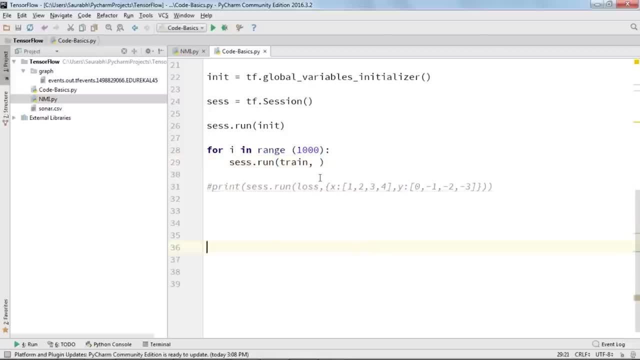 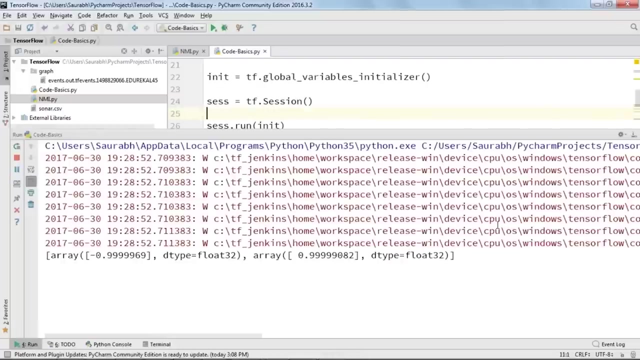 Feed in the values of x and y. So I'll just copy it from here And I'll paste it there. All right, Then go ahead and evaluate the variables w and b. So we have got the new value of w as minus point nine. nine, nine, nine, nine, six, nine. 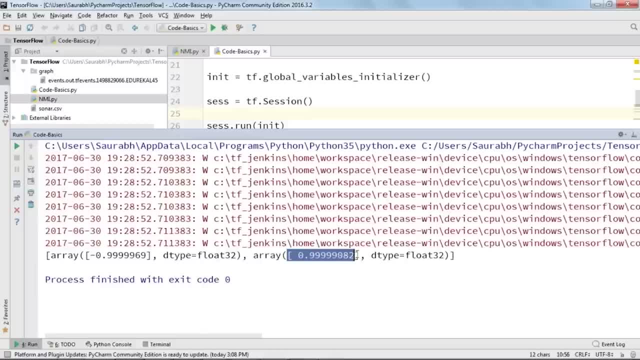 And the new value of b as point nine, nine, nine, nine, nine zero eight two. Now, if you can recall, When we were calculating it manually, We got the output for w as minus one And for b we got it as plus one, And these two values are almost the same. 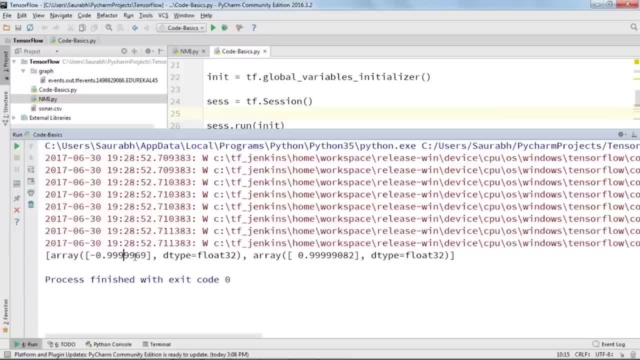 So minus point nine, nine, nine, nine can be rounded off to minus one, And point nine, nine, nine, nine, zero eight, two Can be rounded off to plus one. So this is how you actually build a model. Then you calculate the loss And then you train the model. 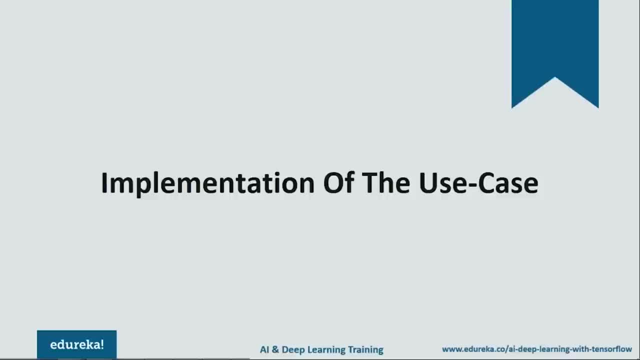 So, guys, this brings us to the most Awaited topic of today's session, Which is the implementation of NMI. That is our use case, Which is Neville mine identifier. So, guys, let me first tell you the steps that are involved in order to implement this use case. 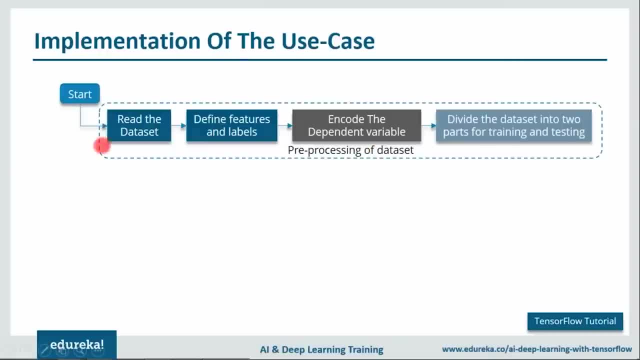 First we need to process the data set that we have. We'll first read the data set, Then we are going to define the features and labels. So what are labels? Labels are nothing but the class to which the pattern represents. In our case, 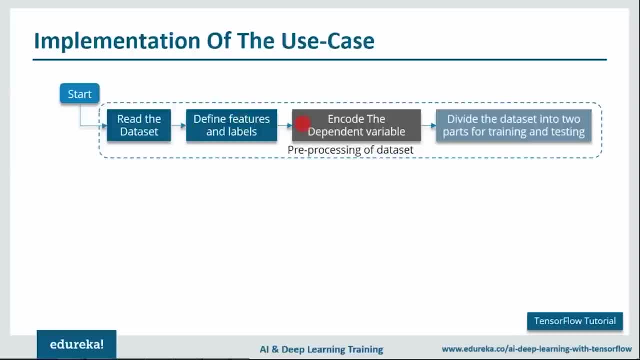 it can be a rock or a mine. Then we need to encode the dependent variable, And here the dependent variable is nothing but your label. So we are going to encode those dependent variables. After that, we are going to divide the data set into two parts. 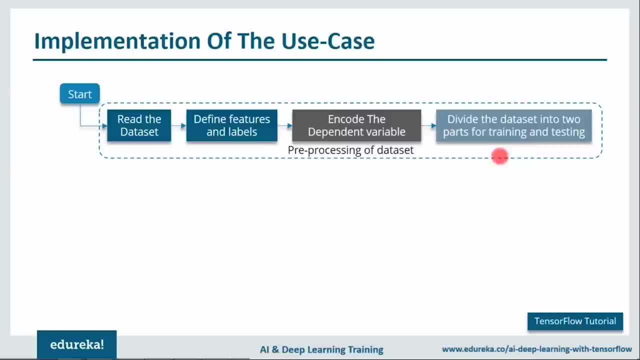 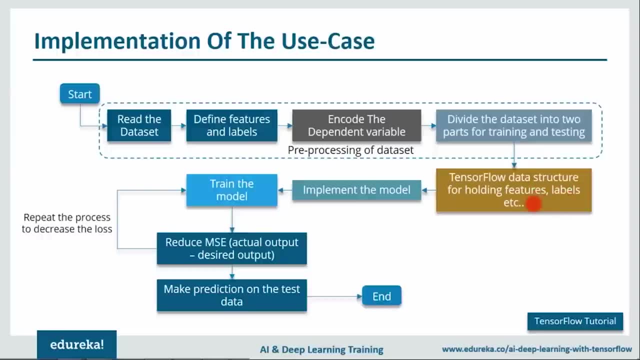 One for training, another for testing. And by the end of this step, our data set is now ready. Next, we are going to use TensorFlow data structures for holding features, labels, etc. So here we'll be defining weights, biases. 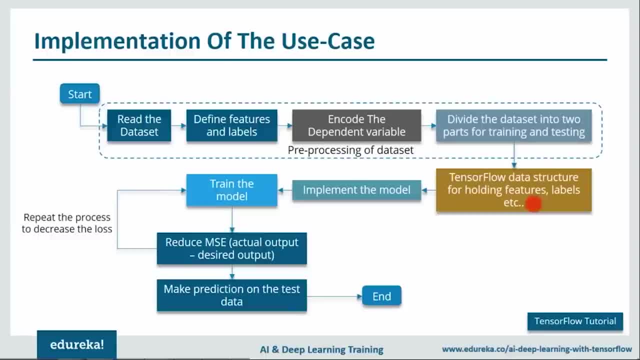 We'll have a couple of placeholders for inputs as well as for the desired output that we already know, And we'll also define one tensor that will be our model output. Then we are going to implement the model. We are going to write the project in order to implement the model. 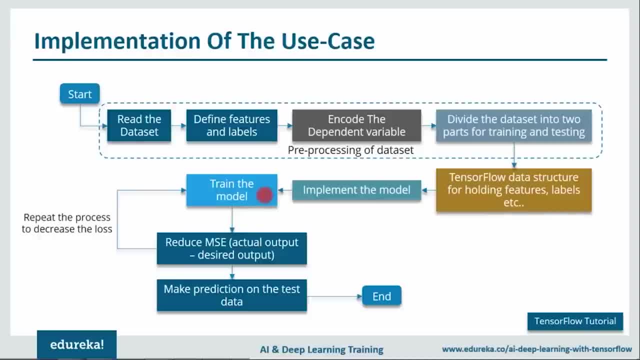 Then, what we are going to do. we are going to train the model on the training data that we have. So, in this particular step, we have divided the data set into two parts: training and testing. We'll use that training data to train our model. 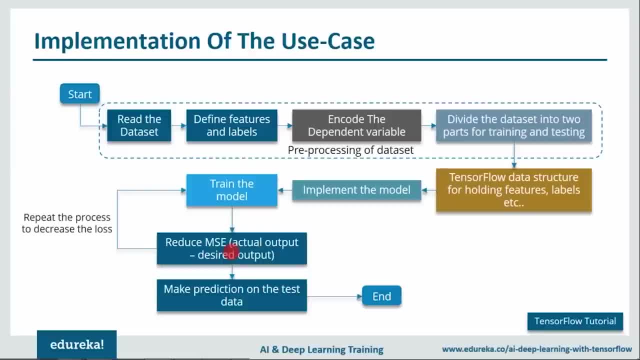 Then we are going to calculate the error, That is, how far your model output is from the actual output- And then we'll try to reduce this error, And when we reach to a point where the error becomes minimum, we are going to test our model on the test data. 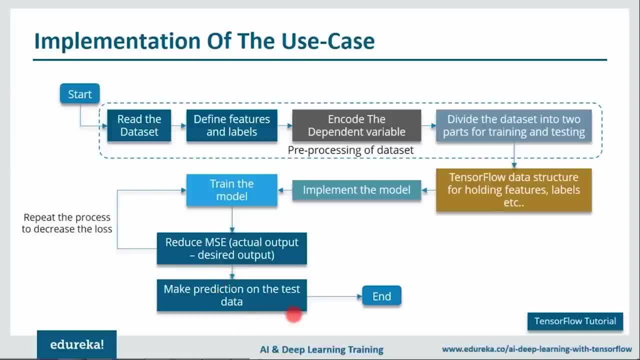 Or you can say: we are going to make prediction on the test data And that will give us the accuracy of our model. So this is how we are going to implement the use case. Now I'll open my PyCharm and execute this practically, guys. 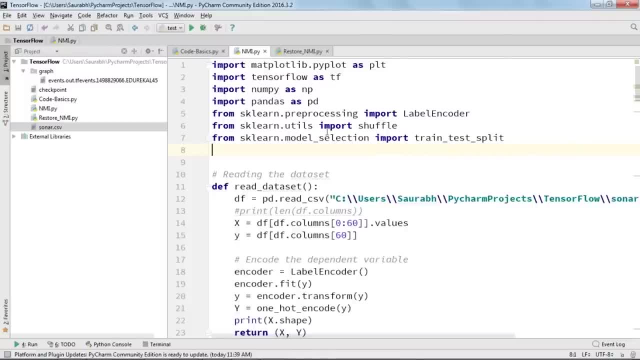 So, guys, we'll first start with importing the necessary libraries. First we'll import matplotlib, which is used for visualization, the tensorflow, the numpy pandas and sklearn as well. So these are the libraries that we are going to use. 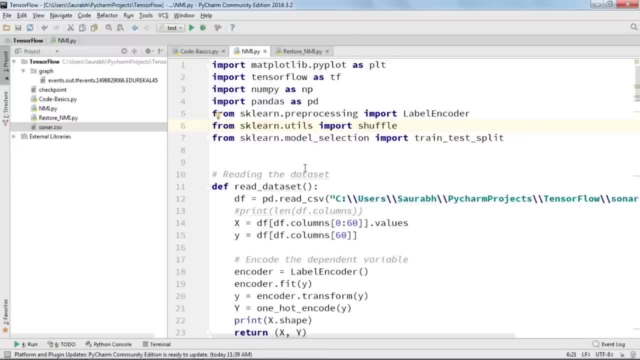 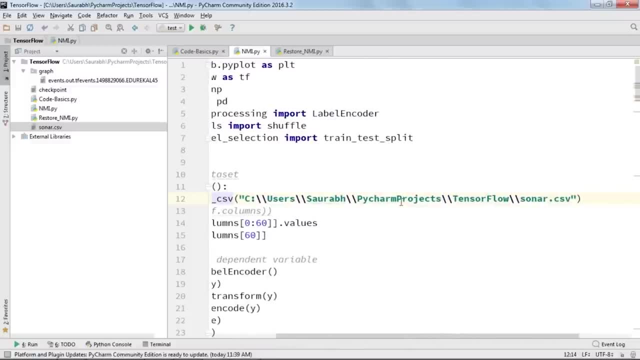 So we need to import these libraries. Then we are going to read the data set. For that we are going to use pandas, So we are going to convert this data set into a data frame, a pandas data frame, and we are going to give the path. 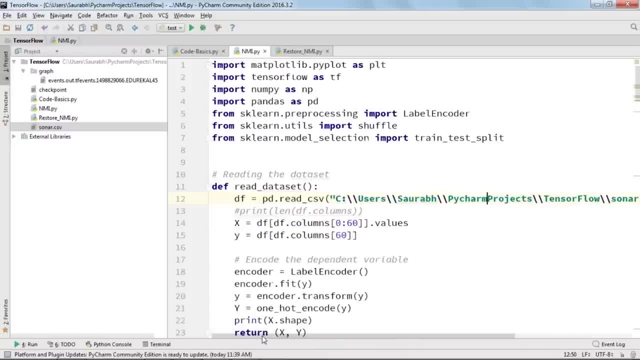 to where our file is stored or our data set is stored. Then we are going to define features and labels. So here x will be our feature. So basically the first column till the 60th column will be our features, and the last column represents the label, as I've told you earlier as well. 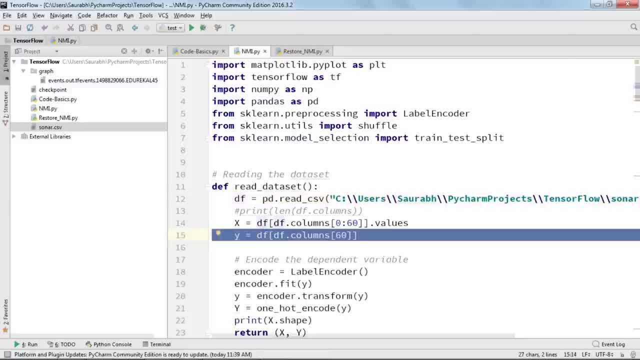 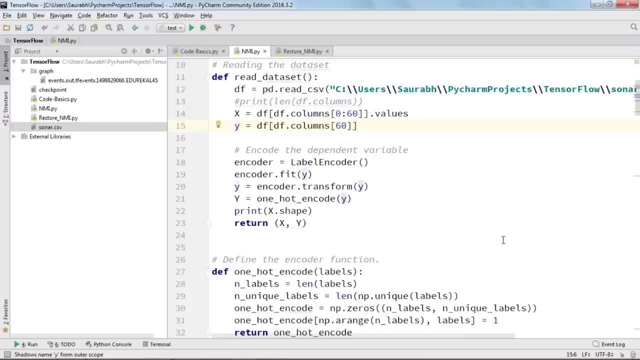 So the last column will be our label, and it will be stored in y. After that we need to encode the dependent variable, which is nothing but our label. Now we'll perform label encoding first, and then we're going to perform one-hot encoding. 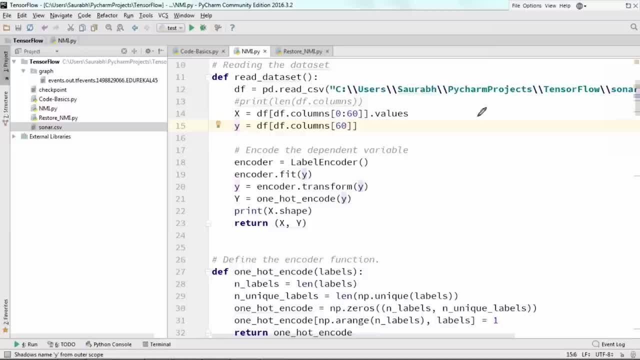 So, guys, I'll explain you one-hot encoding and label encoding with a pen. So suppose, if I have labels like rock, then mine, then again rock, then one more mine. First we'll perform label encoding in which I'll assign values to it. 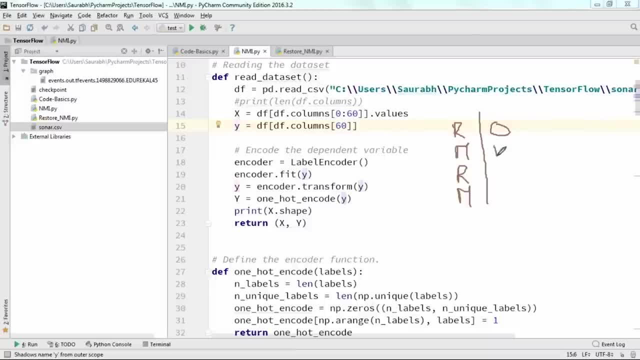 So suppose, if I assign zero to a rock and one to a mine, so I'll keep it that way for the rest of the rows as well. All right, So now we'll perform one-hot encoding in which we'll have two columns, one for mine and another for rock. 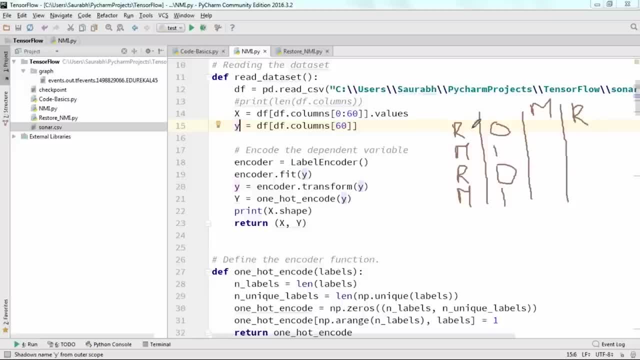 So wherever the data represents a mine, it'll be one. So this basically represents a rock, so it'll be zero. This row represents a mine, so it'll be one. This represents a rock, so it'll be zero. Similarly, 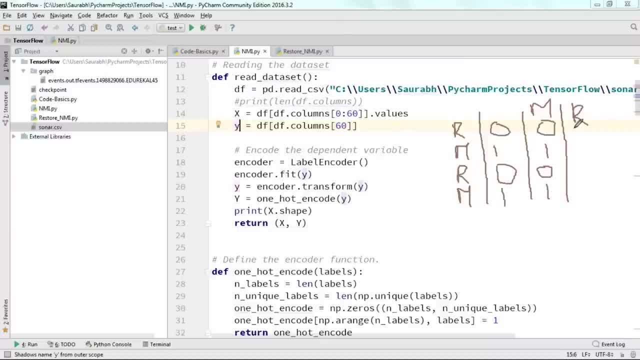 this represents a mine, so it'll be one. Now the second column: wherever the data represents a rock, we'll keep it as one. So this represents a rock, we'll keep it as one. This represents a mine, so let it be zero. 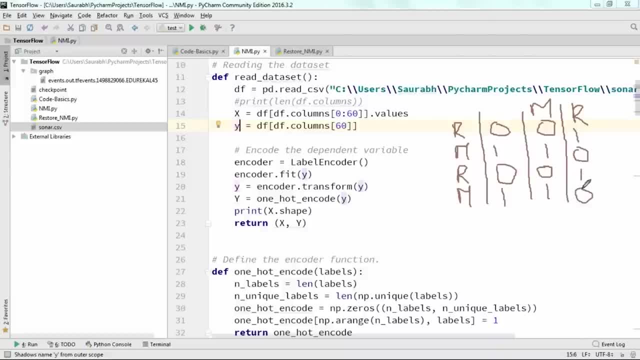 This will again be one, because it represents a rock. This represents a mine, so we'll keep it as zero. So this is how you perform one-hot encoding. So what is one-hot encoding? Basically, only one input will be active at one time. 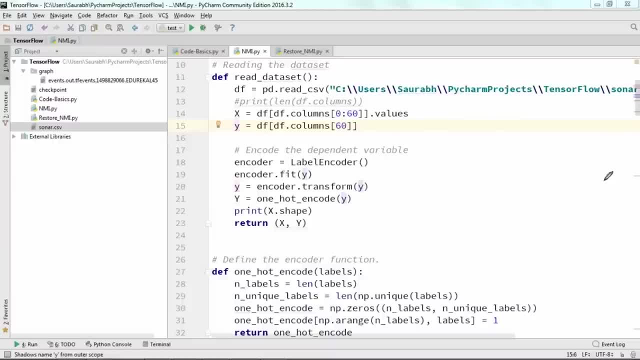 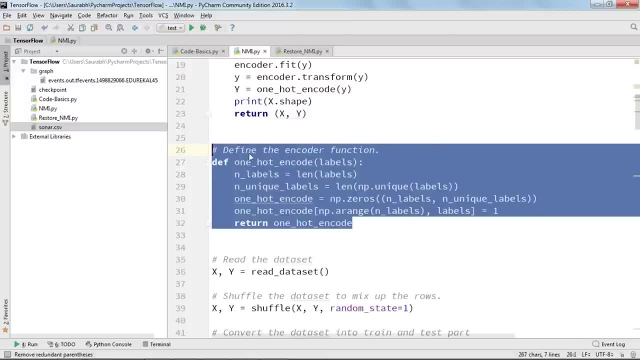 So, basically, what is one-hot encoding? Only one input will be active, So let us move forward now. So this is the function that actually defines one-hot encoding. So this is where we have performed the one-hot encoding. Then what we are gonna do, 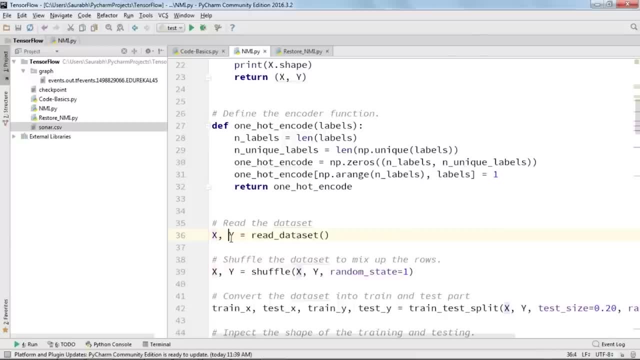 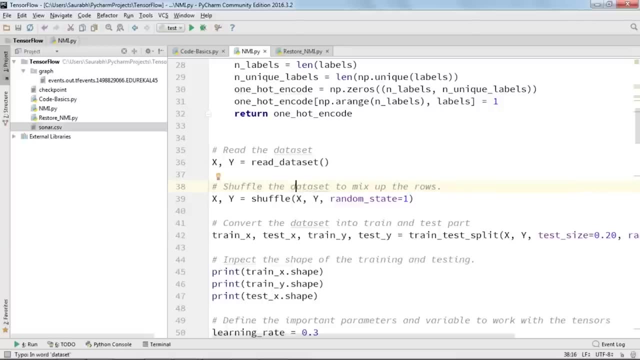 we are gonna read the data set. So X is basically a feature and Y is one-hot encoded label. Then we are gonna shuffle the data set. We need to shuffle the data set because the whole data set that we have it is present in an order. 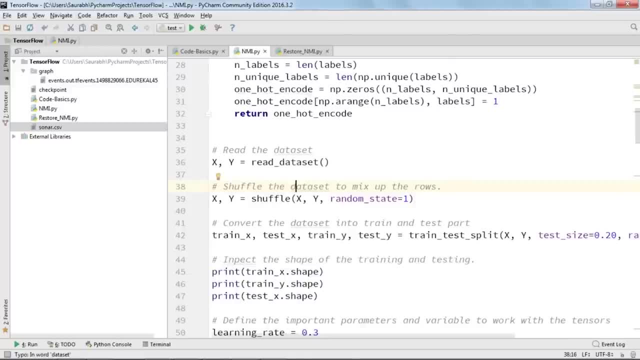 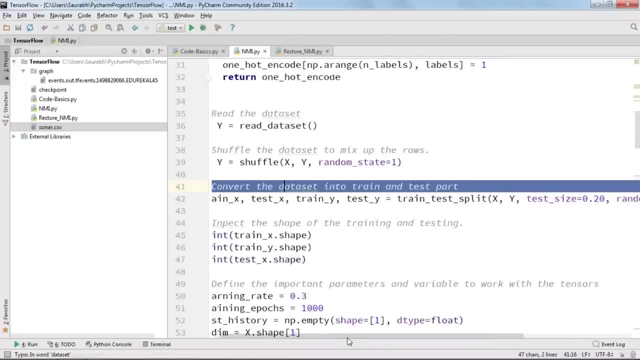 For example, in the beginning we have mines and then we have rocks, So we need to shuffle it. So after doing that, we are gonna split the data set into two parts: training and testing. How are we gonna do that? You can see it over here. 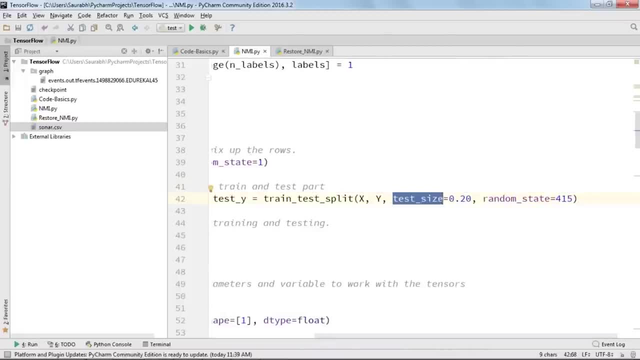 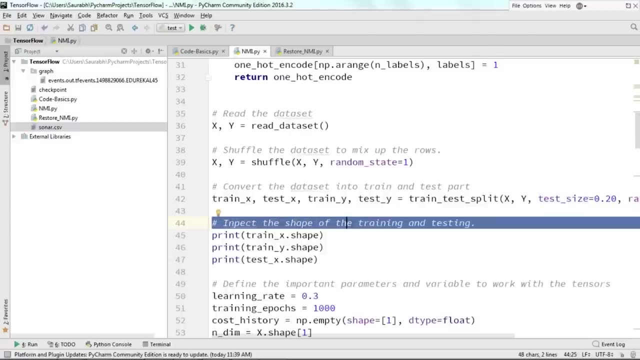 So we have defined the test size as 0.20,, which means the 20% of the data set will be your testing data set. Now you can go ahead and inspect the shape of the training and the testing data, although it is not necessary. 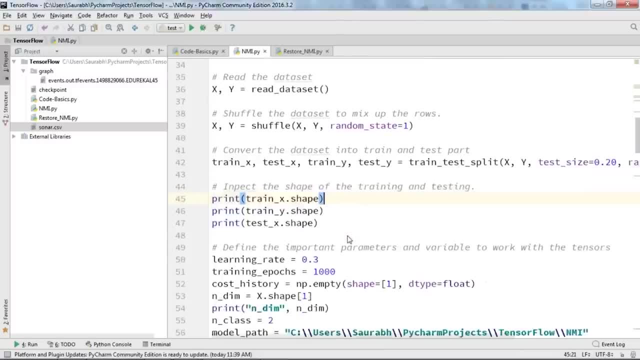 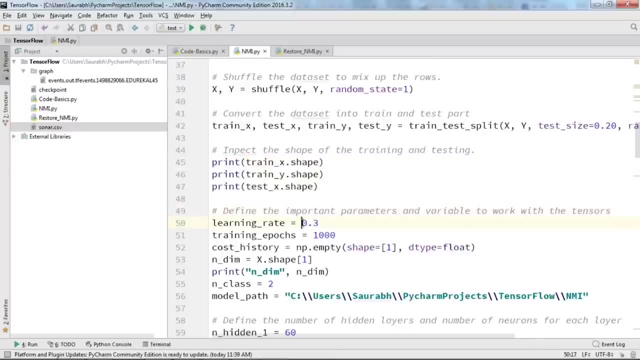 but still, if you wanna go ahead and do it, you can do that as well. Then we are going to define the important parameters and variables to work with tensors. So first we are gonna define learning rate. So we have seen what exactly learning rate is. 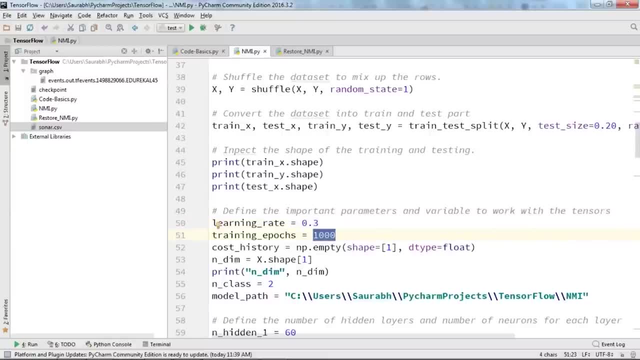 Then we are gonna define the epoch. Epoch basically means the total number of iterations that will be done in order to minimize the error. Then we are gonna define a loss function cost history. Then we have n underscore dim. So what is n dim? 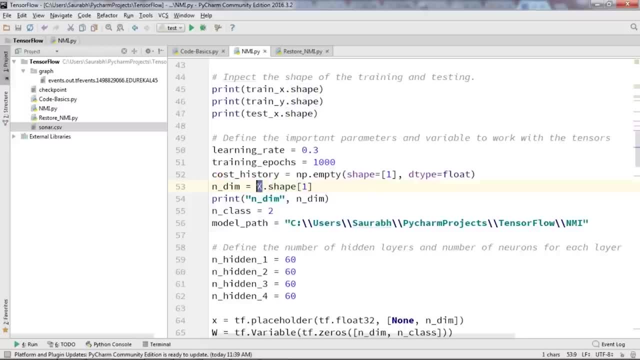 So basically, n dim is nothing but the shape of your features, which is stored in X, And that too it will only include the columns, the number of columns. So then we'll print it, and you can still avoid this step if you don't wanna print it. 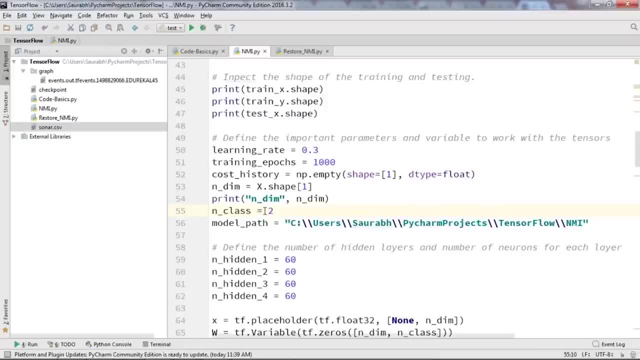 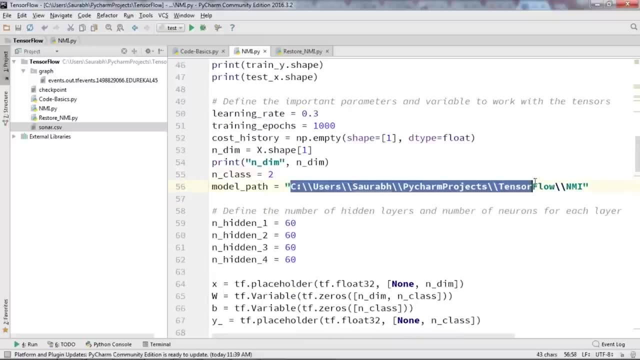 it's all fine. Then you define the number of columns. So, since we have only two classes- that is, mine and rock- we're gonna keep it as two. Then we're gonna provide the model path, which will be nothing but the place where we want to store our model. 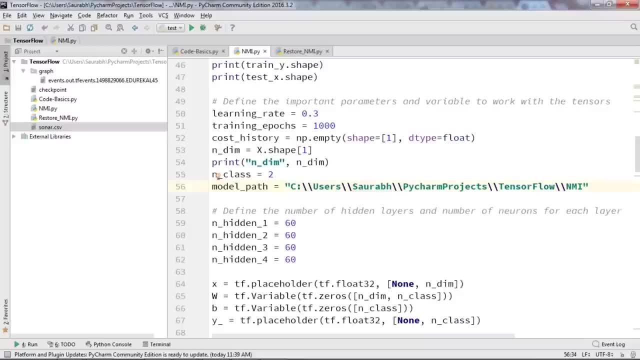 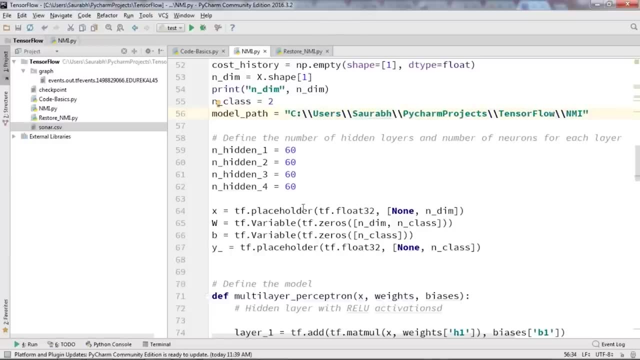 So I've given the same path in which I'm currently working, So you will see a couple of files created. when we execute this model, Then we need to define the number of hidden layers and number of neurons for each layer. So, basically, I've talked about hidden layers. 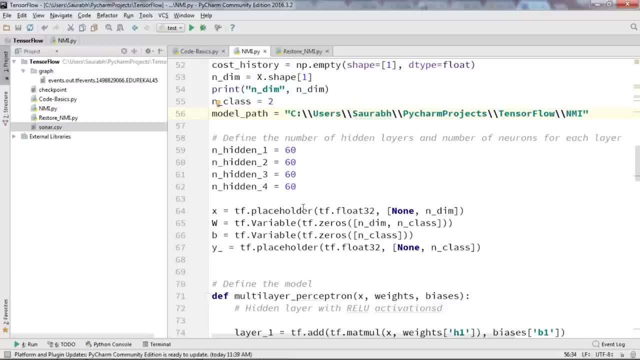 neurons, multi-layer perceptron, perceptron- everything in detail in the previous tutorial. Then we have the number of neurons for hidden layer one, two, three and four. So we're gonna take four hidden layers. So this is nothing but an example. 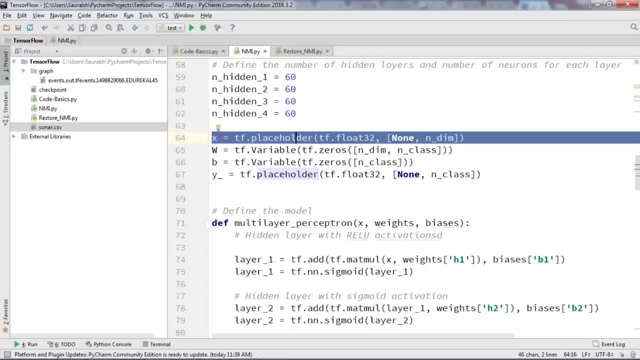 of multi-layer perceptron. So X is our placeholder in which we're gonna feed in the input values or you can say the data set. It is: offload 32 bits, and then the shape of this particular tensor is none, comma, endim. 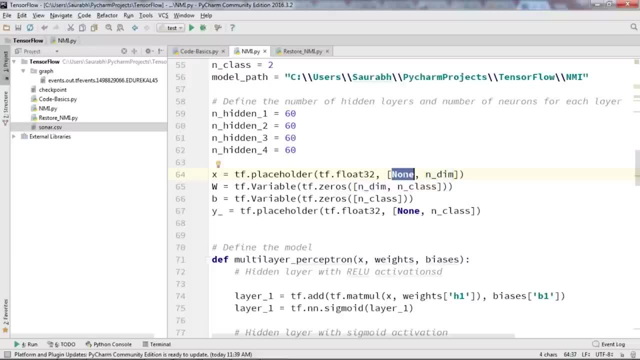 So endim is what we have seen earlier. So if I write here none, which means it can be any value, Then we'll define a variable W, which will be initialized with zeros and it'll have shape N, underscore dim, which we know what it is. 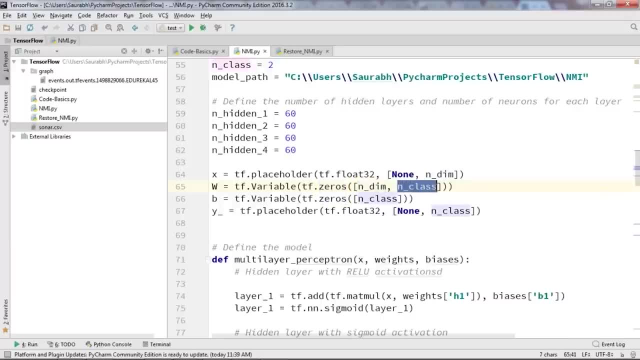 and N underscore dim is N underscore class, which is nothing but the class to which a pattern represents. So we have two classes here. So it'll be N underscore dim, comma two. Then we have one more variable. B will fill it with zeros. 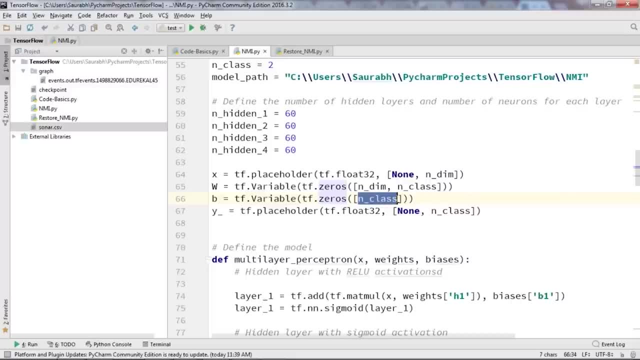 or we'll initialize it with zeros and it'll have a shape of N underscore class, that is, two. Then we're gonna define a placeholder, Y dash, which will be nothing but the output of our model that we already know, and its shape will be none. 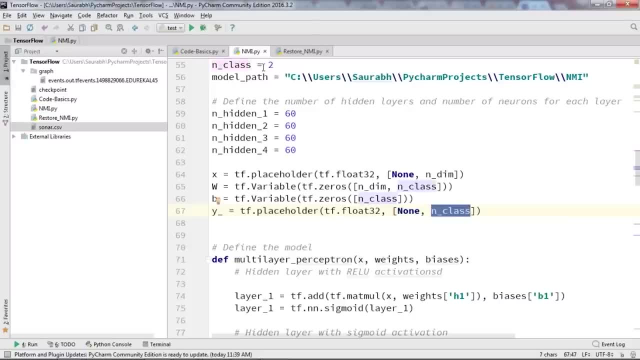 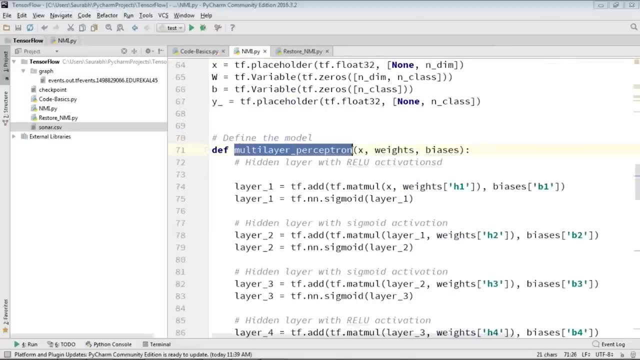 comma. N underscore class None can be any value and we know N underscore class is equal to two because we have only two classes. so now we are going to define a model. We're gonna name it as multi-layer perceptron because it is an example. 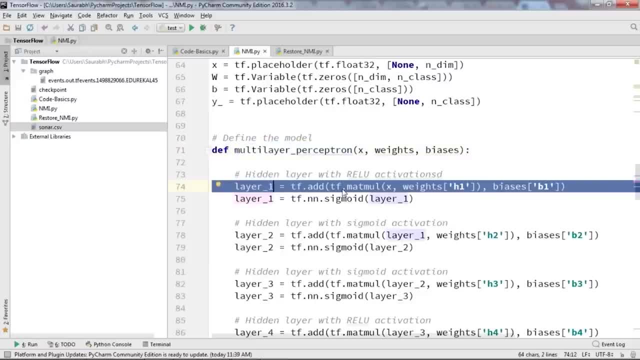 of multi-layer perceptron. So first we'll define the first hidden layer, in which it'll be nothing but the matrix multiplication of your input and the weight, and then we're gonna add it to the bias, Then we're gonna pass it through a sigmoid. 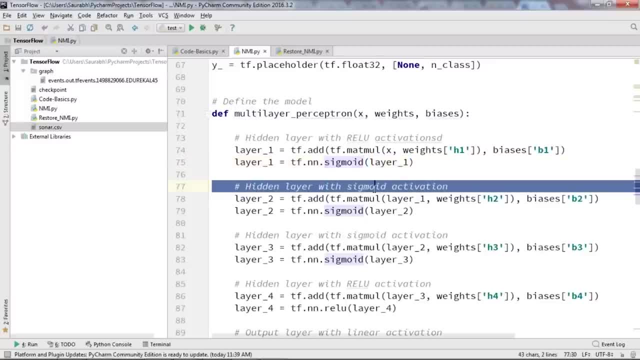 activation function, Then the second hidden layer. also the same thing will happen, and the input for the second hidden layer will be the output of the first hidden layer. So we're gonna type in here, layer underscore one, and then we're gonna define the weight, which will be H2.. 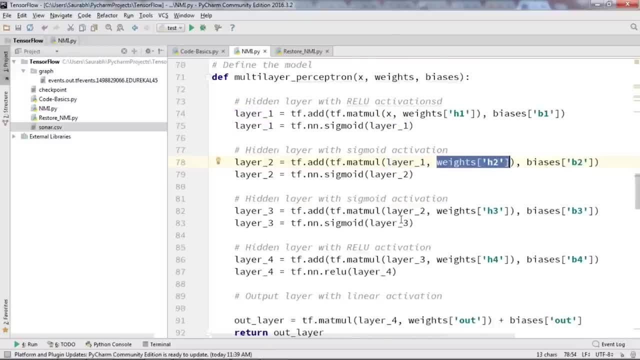 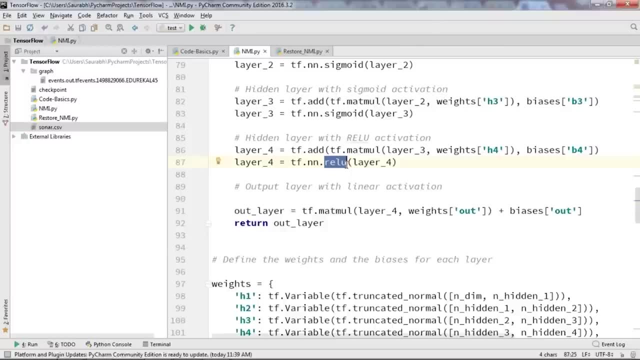 So matrix multiplication of that and then add it to the bias. Similarly for hidden layer three as well, and in hidden layer four, instead of using sigmoid activation function we'll use ReLU activation function. and then finally comes the output layer in which we're gonna perform. 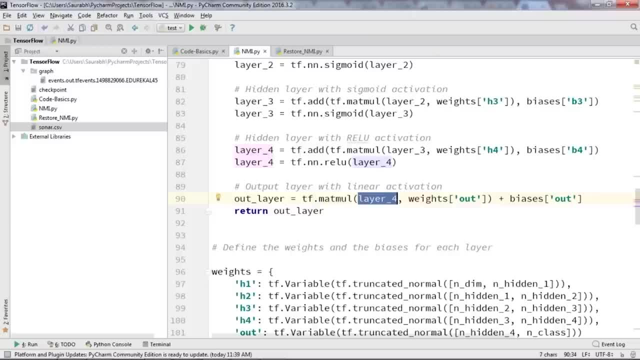 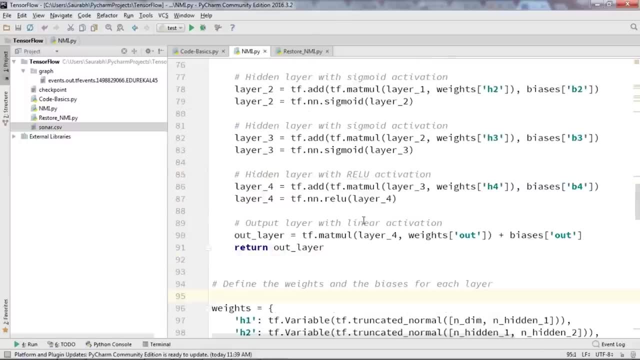 matrix multiplication output of the previous hidden layer and the weights, and then we're gonna add biases to it. So now we need to define weights and biases for each layer. So H1 is the weight for the first hidden layer. So we're gonna define that. 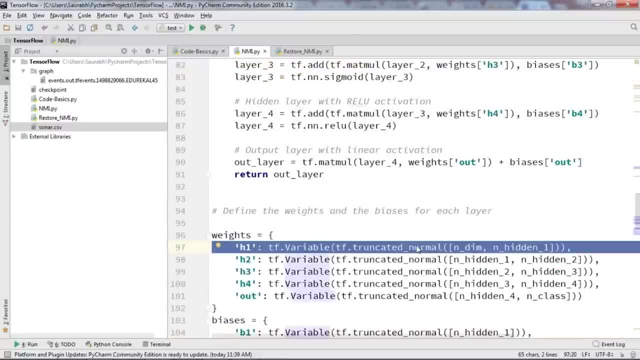 It'll be a variable and it'll be a truncated normal of N underscore DRIM and N underscore, hidden underscore one, which is nothing but the shape of this particular tensor or this particular variable: N underscore DIM, we know, and N underscore, hidden underscore one, is nothing but 60.. 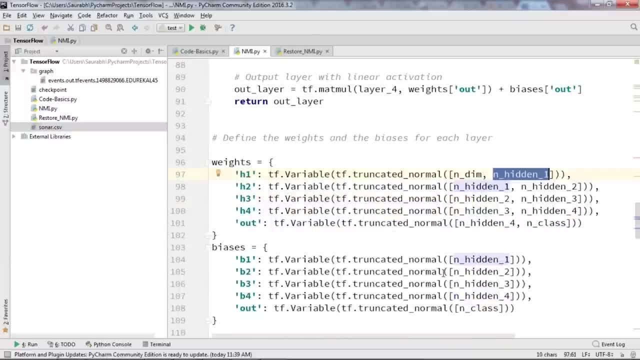 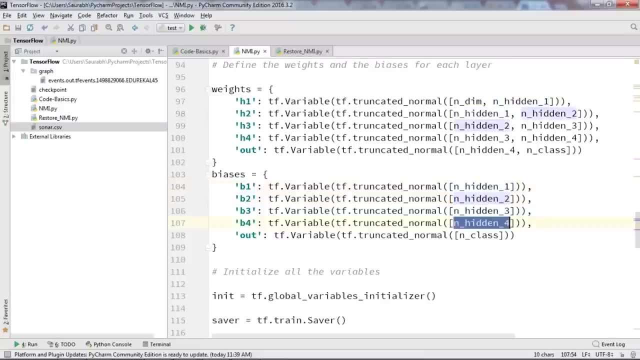 Similarly for other weights as well, and the same goes for biases as well. Here we'll have shape which is equal to N underscore, hidden underscore one, hidden underscore two, three and four, and then, finally, the output bias will be equal to N underscore class, which will be 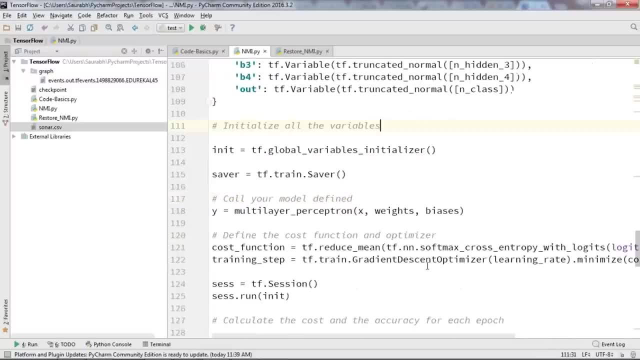 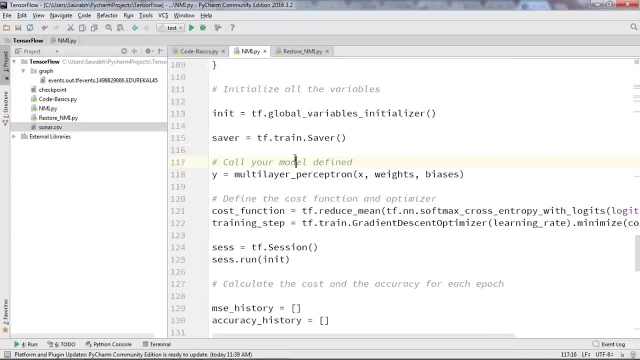 nothing but two, Because we have only two classes. Then we need to initialize all the variables, which we have seen how to do that. After that, we're gonna create a saver object in order to save our model. Then we're gonna call the model that we have. 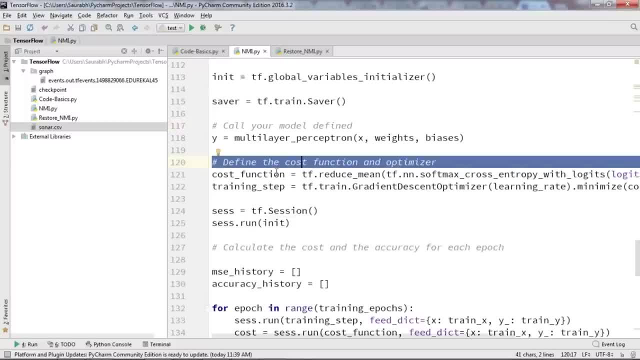 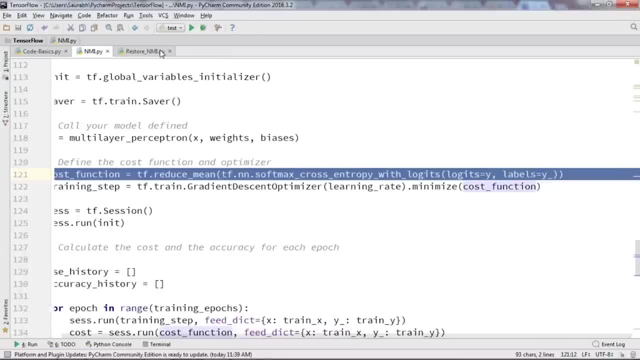 defined above. Then we're gonna define the cost function and optimize it. Cost function is nothing but the loss function. This is our loss function that we have defined here. So over here, if you notice, let me just show it to you, Yeah. 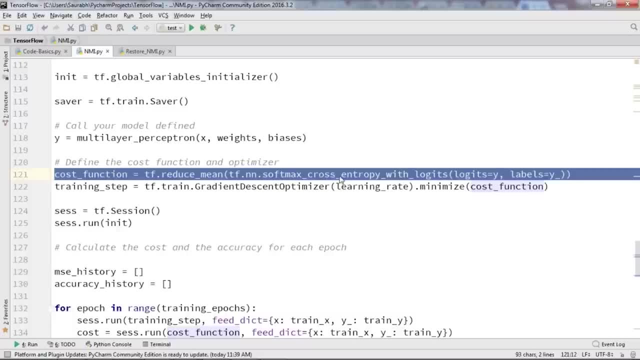 So this is how we have defined a cost function. So we're gonna use a softmax cross entropy and logic and this y is nothing but your output and labels y dash is nothing but your actual output. or you can say the output that we already know and this is the model output. 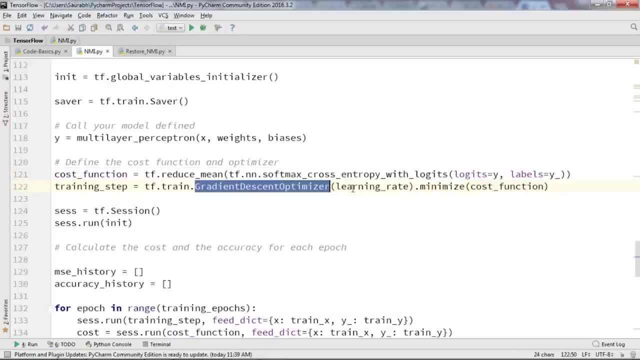 Then we're gonna perform optimization, We're gonna use gradient descent optimizer, and then this is will be: the learning rate will be 0.03, which we have defined above, and then it will be minimizing the cost function or the loss. So this is how. 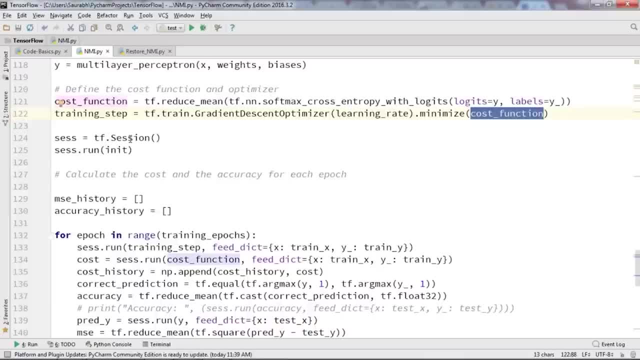 we'll optimize it. Then, what we need to do? we need to create a session object that will launch the graph and this will initialize all the variables. Then we need to calculate the cost and the accuracy for each epoch. How are we gonna do that? 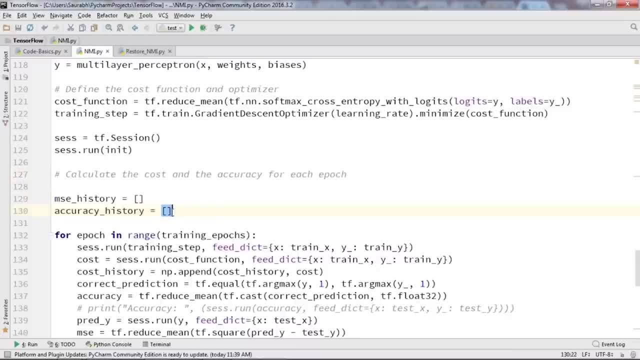 We're gonna use for loop for that. So first we'll define mse, underscore history and accurate history. we'll keep it empty. Then we're gonna define for epoch in range training, underscore epochs Over here. first we'll run the training step, We're gonna feed. 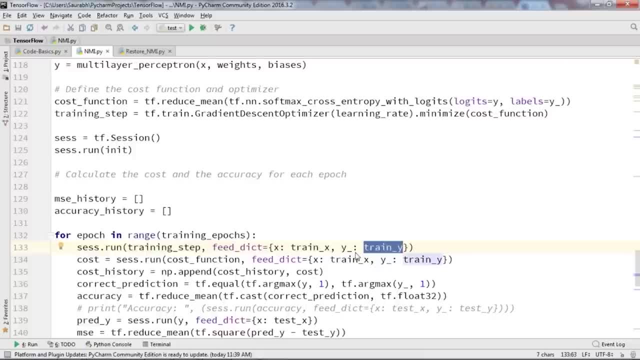 in the values of train underscore x and train underscore y, which is nothing but the training data. Then we're gonna run the cost function or you can say the loss and again feed in the values of train underscore x, and then what we're gonna do, we're gonna define. 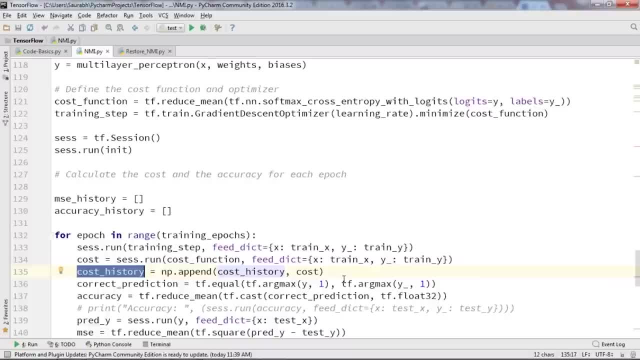 cost history, which will be append, the cost history comma cost. So whatever cost history we have, whatever cost, we'll get it here, it'll be appended and it'll be here cost history, So we can see that for every epoch. that's why we're doing it. 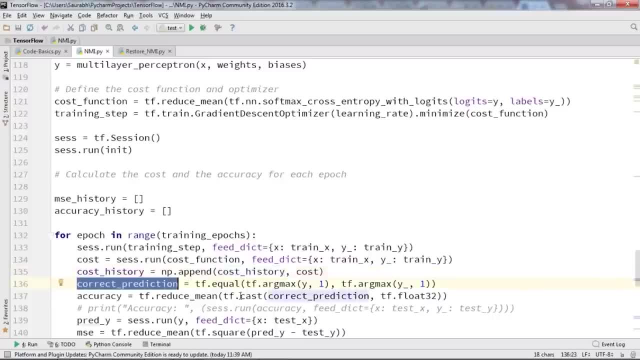 So it'll be appending one by one, Then we're gonna find out the correct prediction, which will be equal to tf dot, argmax y, comma one, and argmax y dash, comma one, which is nothing but the difference between the actual output and the model output. 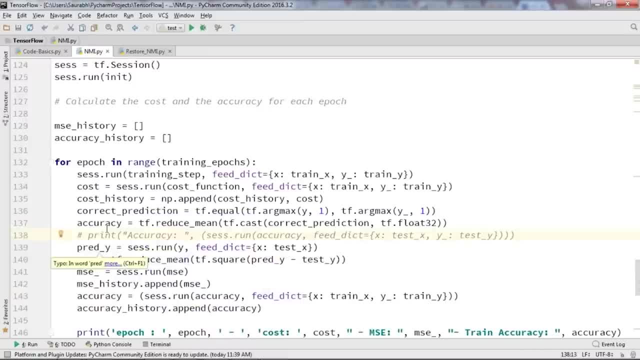 and after that we're gonna calculate the accuracy here and then what we need to do. we'll define a parameter, print underscore y, which will be nothing but says dot, run and the actual output, and feed in the test data in order to see how accurate our model is. 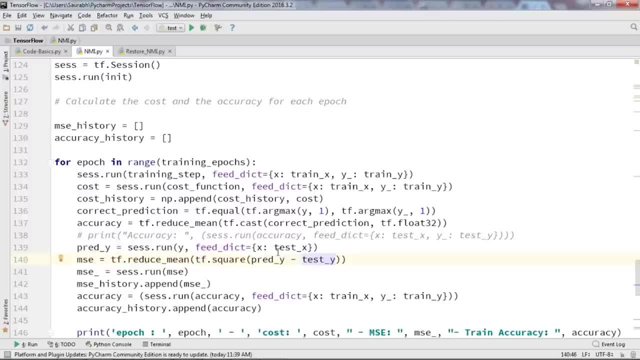 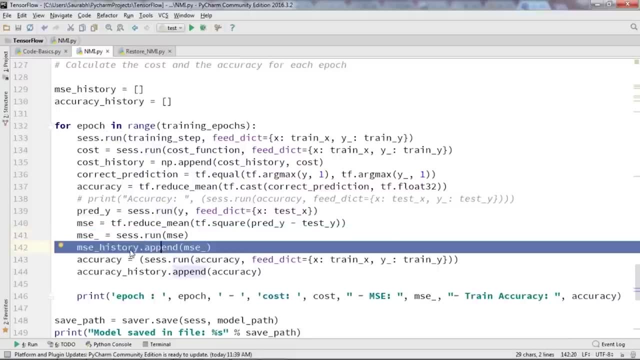 Similarly, we're gonna define mse mean squared error, which will be nothing but the difference between the predicted value and the test value. Then we're gonna launch the graph here and we're gonna find the mse history dot append. so this will actually keep on updating the mse value. 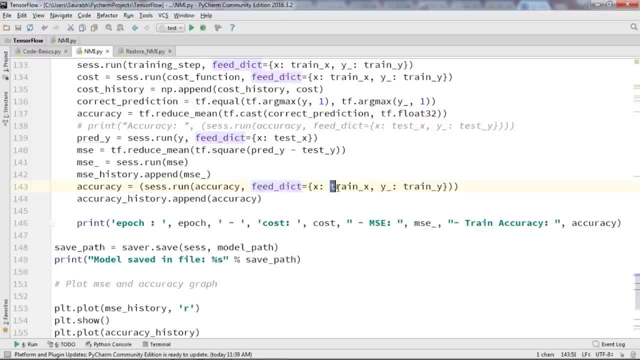 for every epoch, Then we're gonna find out the training data. so basically we'll be finding here the accuracy on the training data, not on the test data, and we'll keep on appending so that for every epoch we can see that. Then we're gonna print. 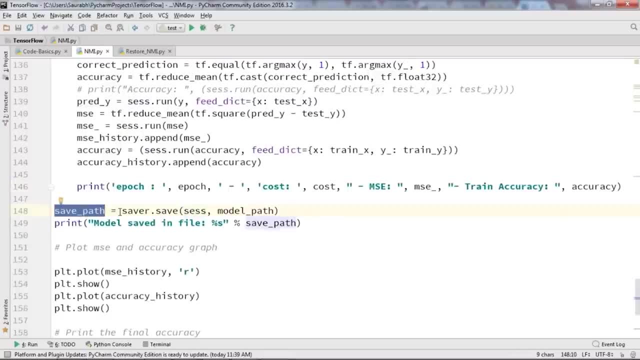 that value for every epoch. After that we're gonna define one more parameter: save underscore path, which will be saver dot save says comma model, so this will actually save the model in the model path. Now we're gonna plot the graph of mse and accuracy. mse is nothing. 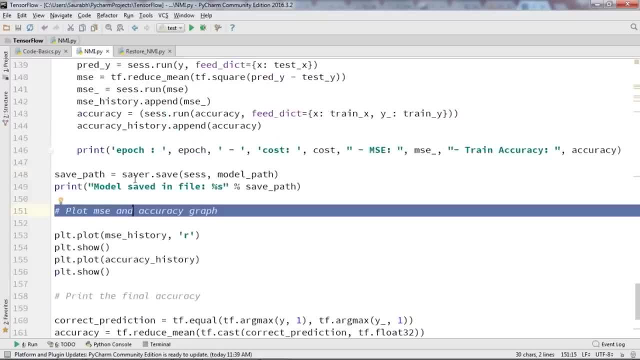 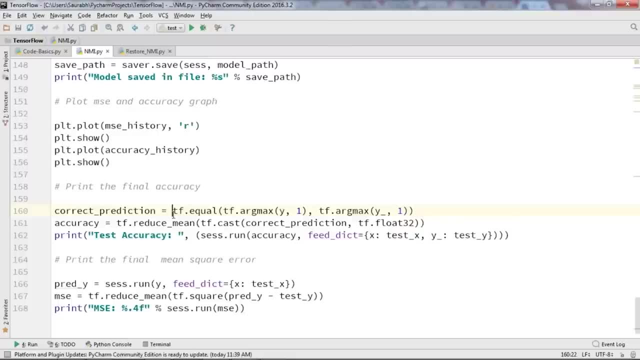 but the mean squared error and accuracy will be there on your test data and mean squared error. so we're gonna print that mse here. if you can notice Then what we need to do, we need to print the final accuracy for that we'll first find out. 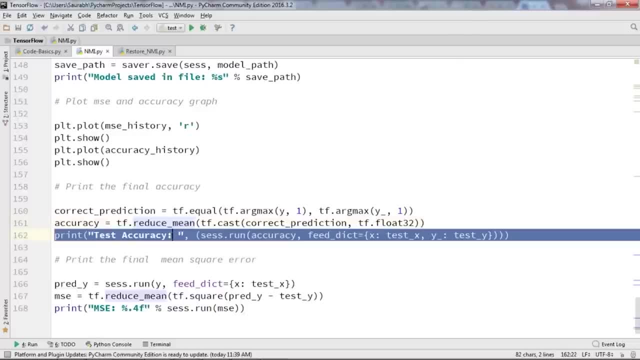 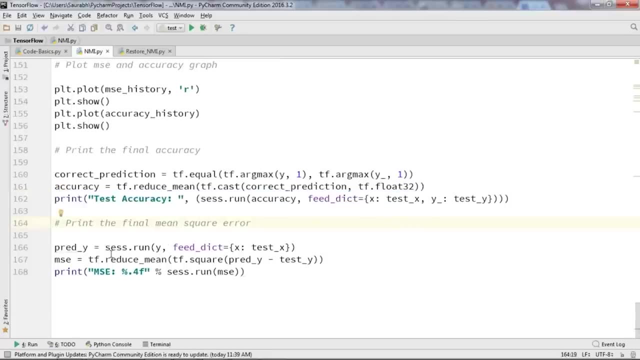 the correct predictions made by our model, and then we're gonna find out the accuracy and finally we're gonna print it by running the session and feeding the values of test data in x and y. Finally, we need to print in the final mean squared error, which will be nothing. 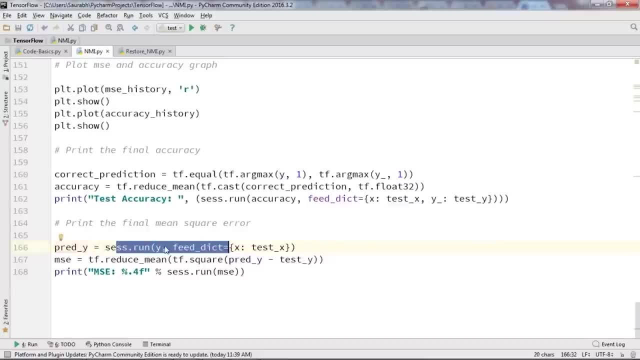 but pred underscore y says dot run y, comma, feed dict. so y is our actual output and feed underscore dict is just we're feeding the test input. Then we're gonna calculate mse, mean squared error, which is nothing but the difference between the predicted value and the actual value. 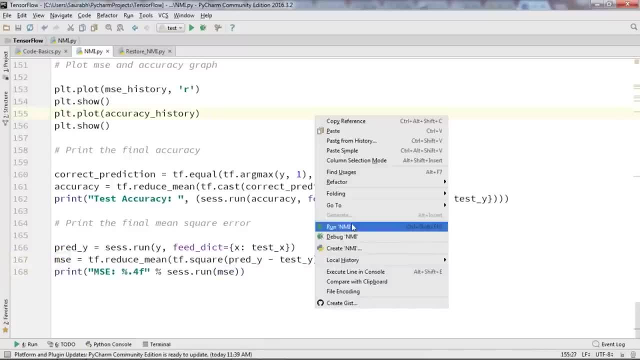 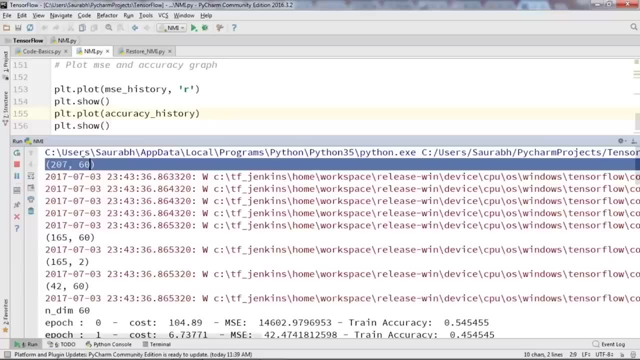 which is there in the test data, and then just go ahead and print this. So we'll now start training our model. so let us go ahead and run this. So in the beginning, if you noted, it has printed the shape and then it is printing the test. 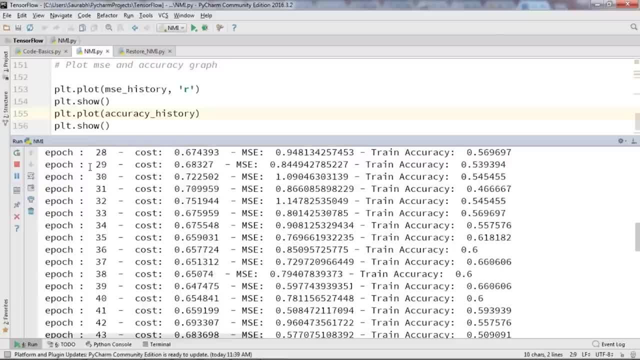 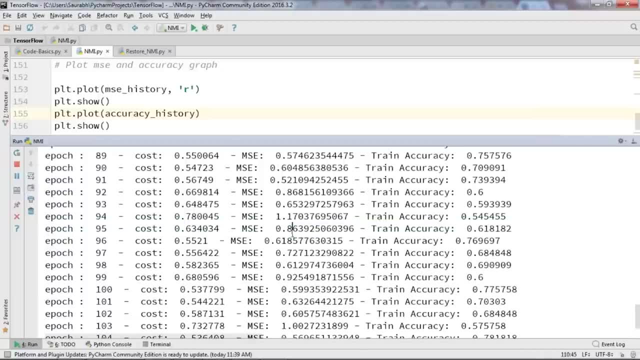 and the training data shape as well. and now it has started training our model. so you can notice the training accuracy that we are getting here. so it will keep on repeating this process for thousand times, for thousand epochs, basically For thousand iterations. after that, our model will be trained. 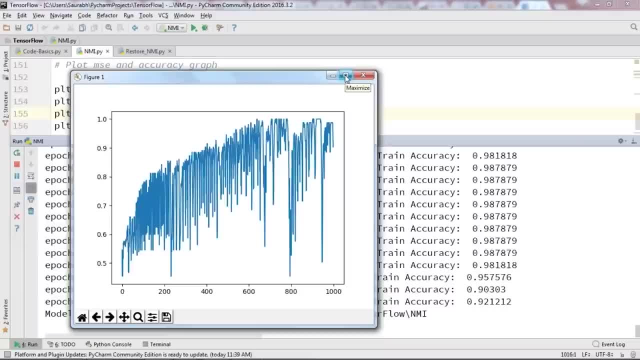 So, guys, this is the accuracy that we have got on our test data. So this y axis represents the accuracy and the x axis represents the number of epochs. So we have thousand epochs here. that means it's gonna train it thousand times. So let me just close it now. 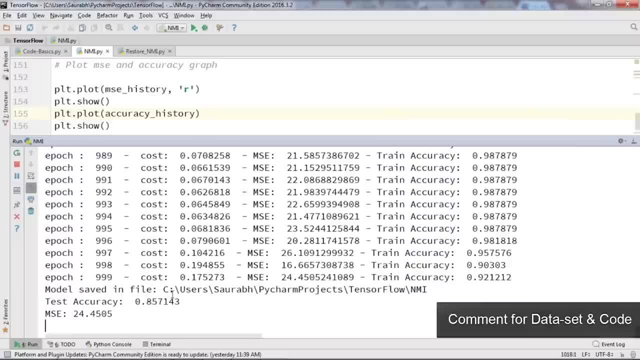 and yeah, so we have got the test accuracy. that's 85%, and the average mean squared error is 24.4505. and our model is saved in this particular directory, which is my current working directory. guys, Now let me close this and open the project structure. 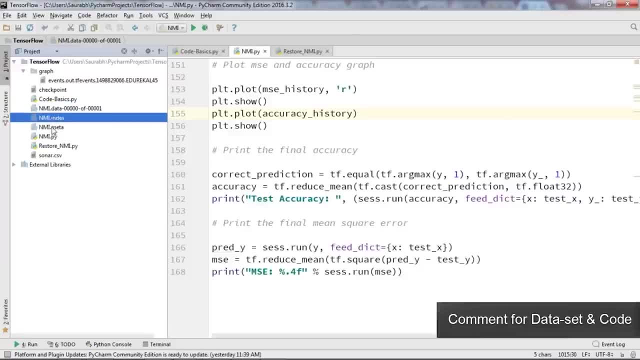 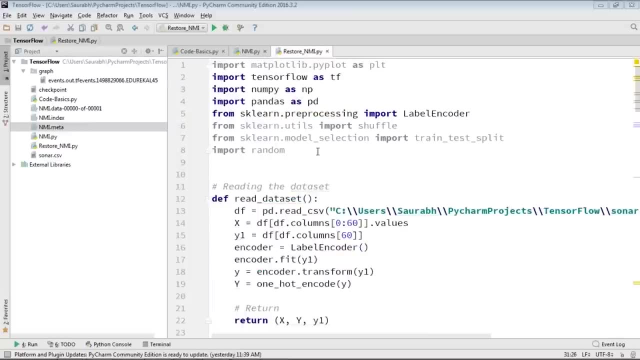 and you can see a couple of files that have been created here. So, guys, we have successfully trained our model and we have saved it as well. Now what we are going to do? we are going to restore this model. So, basically, we will be providing some input. 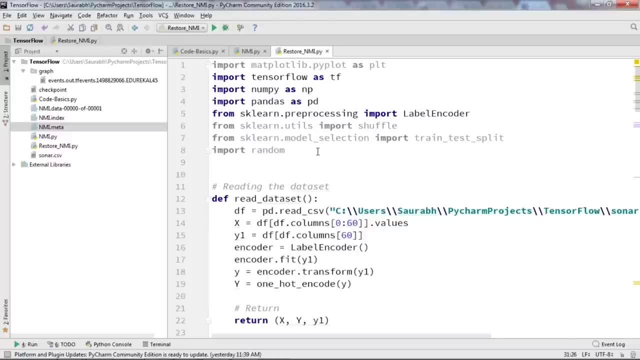 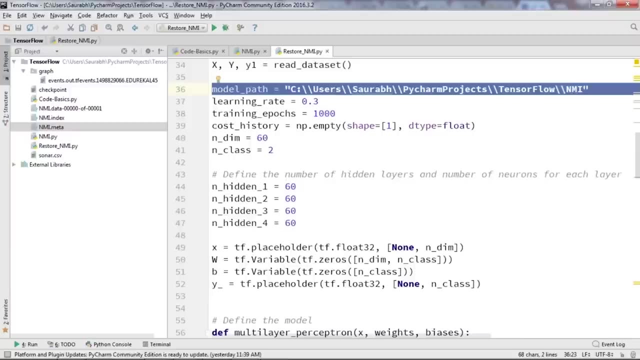 to this particular model and it will predict the outcome for us. So it will predict whether it is a rock or a mine. So the whole code remains the same. It's just that you need to provide the model path, which you have done when you were actually defining. 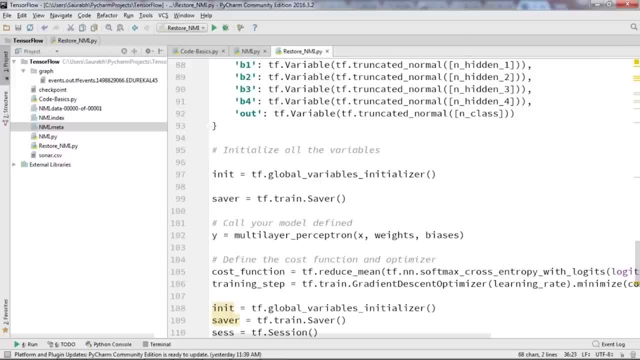 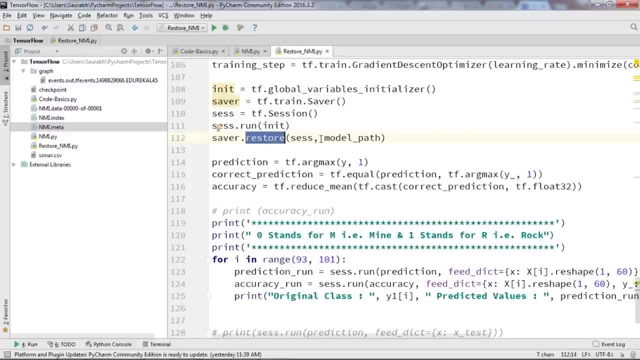 the model and training it, and then what you need to do is you need to again create one saver object and after that, finally, you need to call this restore function in order to restore the model that we have Over here. you are going to provide two arguments. 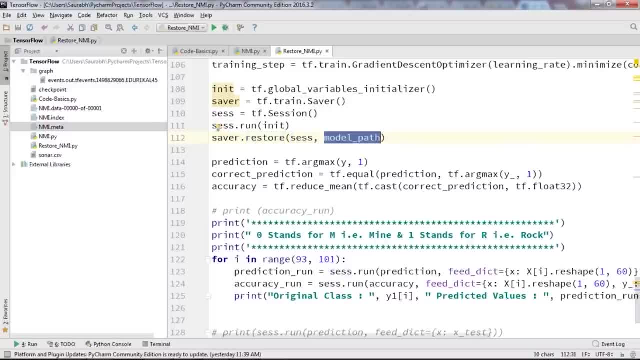 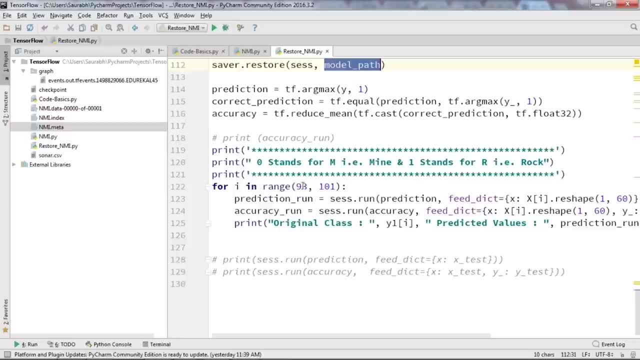 one is says and another is nothing but your model underscore path, which we have given in the previous step. So, guys, this is how it is, and we are going to provide the input from the data set only, which will be from row 93 till 101. 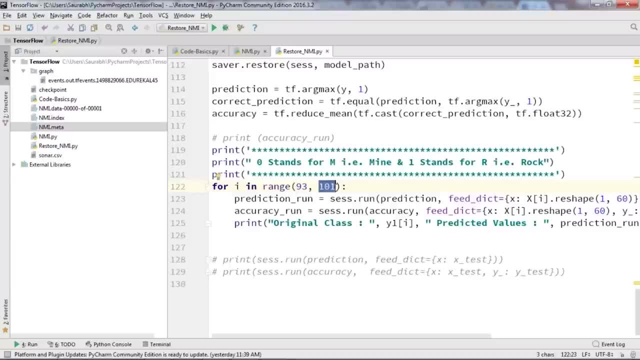 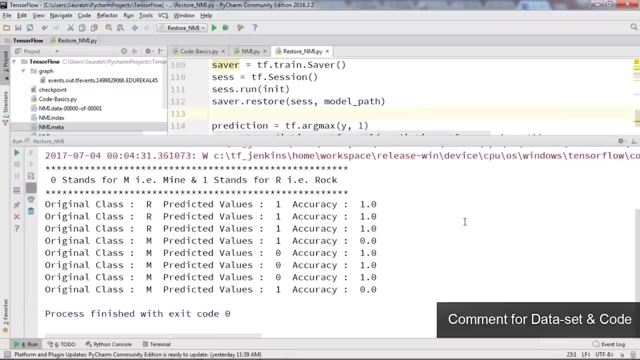 but it won't include the 101th row. It will only be there till 100th row, Fine guys, So let us go ahead and run this. So, guys, this is how the predicted values looks like Over here. the original class was R. 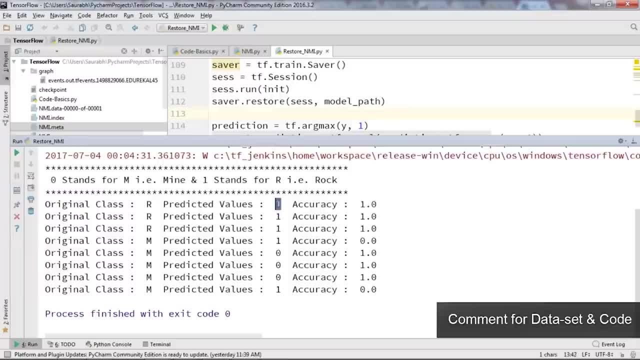 we predicted a value is one which means we have correctly predicted this particular class and we have got the accuracy of 100%. Similarly for other values as well. But if you notice over here, we have got the accuracy as zero because we have predicted the wrong value of the class. 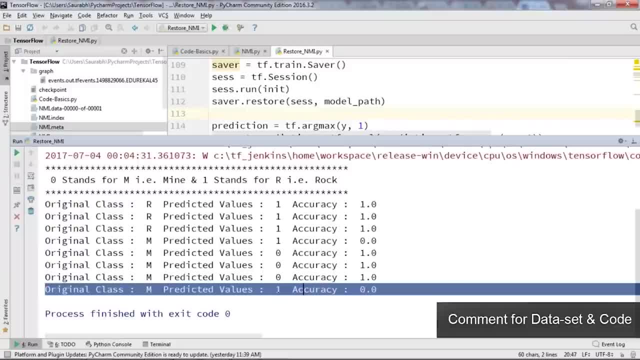 Similarly here as well. it is a mine, but we have predicted it as a rock, So that's why we have got accuracy as zero. So, guys, this is how we actually train a model and we restore it. So this is all about Neville mine identifier. 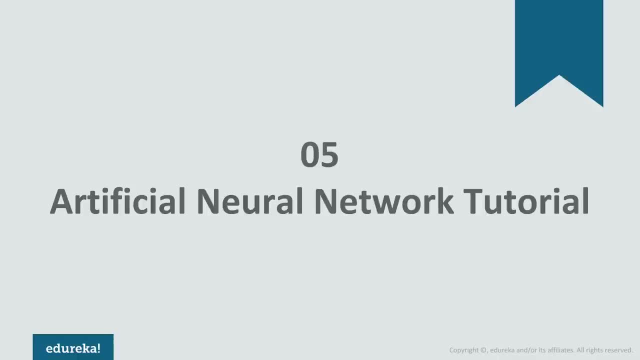 Today, I'll be covering all the fundamentals of neural networks. After that, we'll be using that knowledge in order to solve a real-life problem. So let's take a look at what we are going to implement in this session, and after that we'll be discussing the agenda. 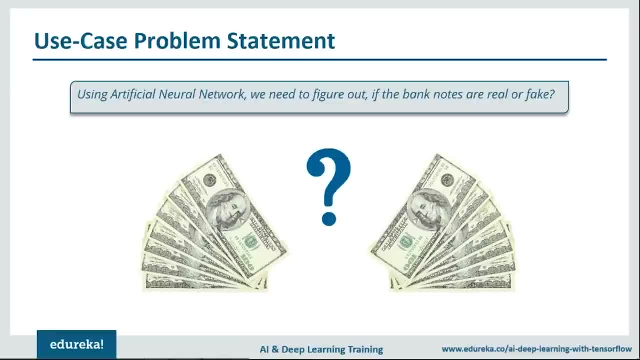 So this is the problem statement. guys, We need to figure out if the banknotes are real or fake, and for that we'll be using artificial neural networks, and obviously we need some sort of data in order to train our network. So let us see how the data set looks like. 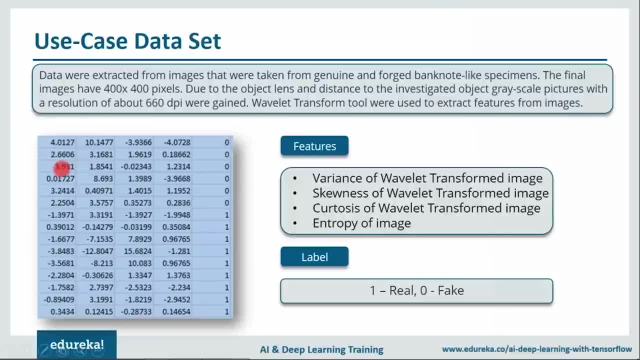 So over here I've taken a screenshot of the data set, with few of the rows and it data were extracted from images that were taken from genuine banknote like specimens. After that, wavelet transform tools were used to extract features from those images and these are few features. 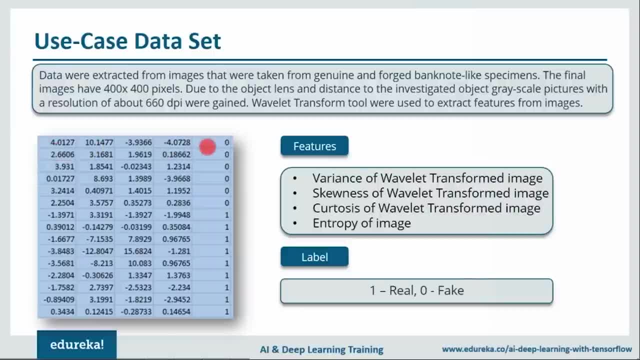 that I'm highlighting with my cursor and the final column, or the last column, actually represents the label. So basically, label tells us to which class that pattern represents, whether that pattern represents a fake note or it represents a real note. Let us discuss these features and labels. 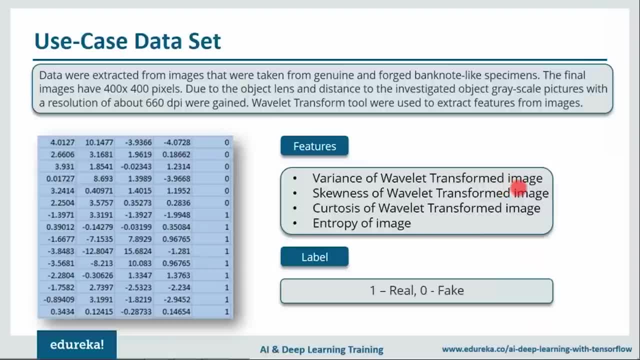 one by one. So the first feature, or the first column, is nothing but variants of a wavelet transformed image. The second column is newness, The third is courtesies of wavelet transformed image and finally, fourth one is entropy of the image. 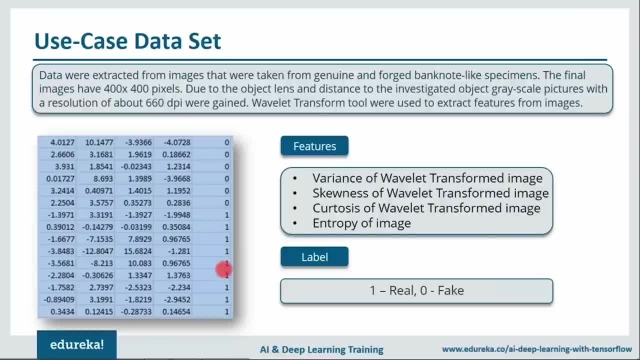 After that, when I talk about label- which is nothing but my last column over here- if the value is one, that means the pattern represents a real note, whereas when value is zero, that means it represents a fake note. So, guys, let's move forward and we'll see. 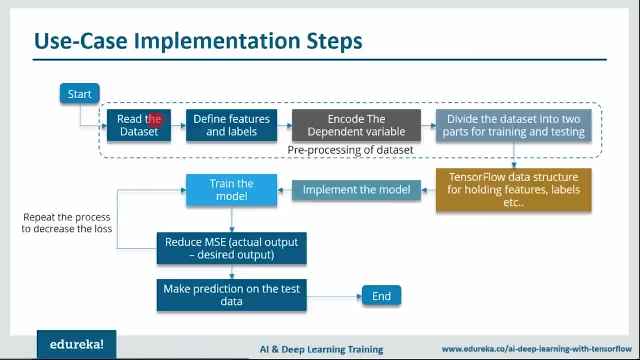 what are the various steps involved in order to implement this use case? So over here, we'll first begin by reading the data set that we have will define features and labels. after that we are going to encode the data set as a dependent variable. it is nothing. 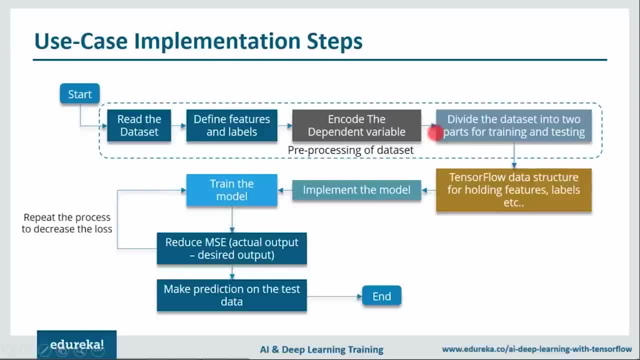 but your label. then we are going to divide the data set into two parts, one for training, another for testing. after that, we'll use TensorFlow data structures for holding features, labels, etc. and TensorFlow is nothing but a Python library that is used in order to implement deep learning models. 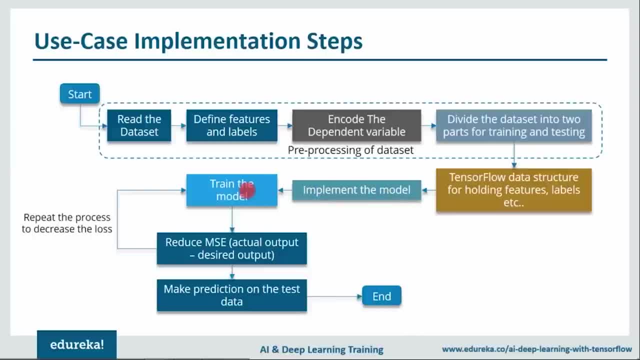 or you can say neural networks. then we'll write the code in order to implement the model and, once this is done, we will train our model. on the training data, we'll calculate the error. error is nothing but your difference between the model output and the actual output. 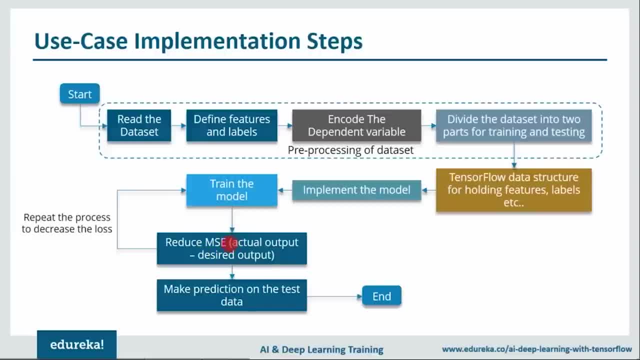 and we'll try to reduce this error and once this error becomes minimum, we'll make prediction on the test data and we'll calculate the final accuracy. So, guys, let me quickly open my PyCharm and show you how the output looks like. So this is my PyCharm, guys. 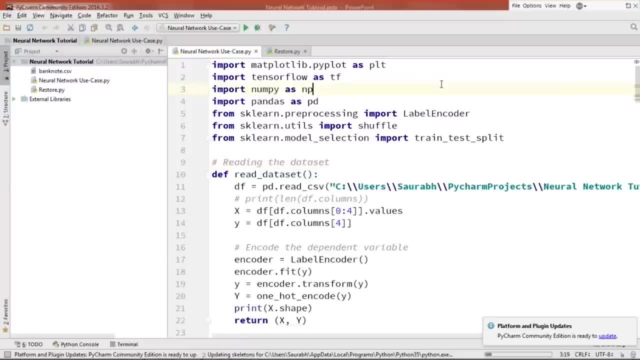 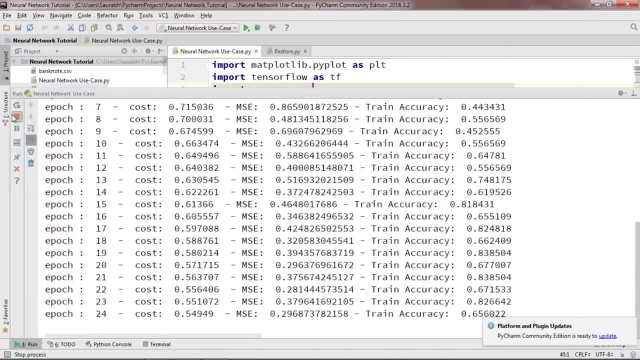 over here, I've already written the code in order to execute the use case. I'll go ahead and run this and I'll show you the output. So over here, as you can see, with every iteration the accuracy is increasing. so let me just stop it right here. 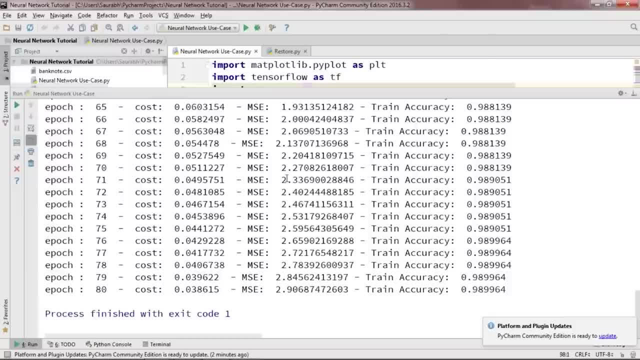 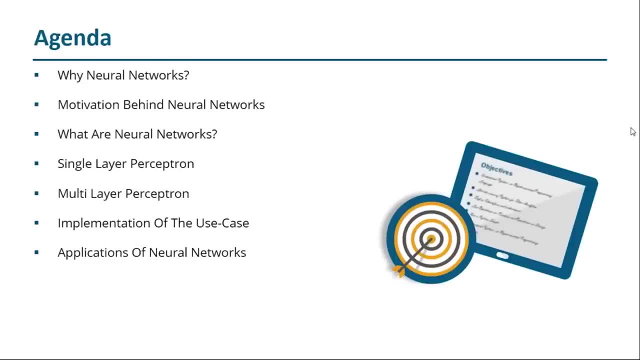 so over here. so what I'll do? I'll open my slides once more and we'll discuss the fundamentals of neural networks that are required in order to implement this use case. so we'll look at the agenda. what are the things we need to discuss? so this is the agenda. 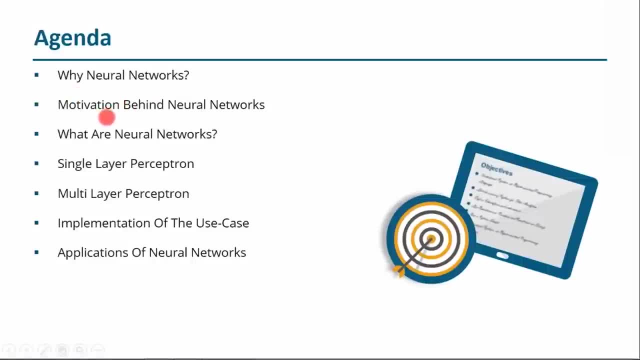 here, guys. we'll start by first understanding why we need neural networks. then we'll focus on what is the motivation behind neural networks and what exactly are neural networks. after that we'll understand what is single layer perceptron and multi layer perceptron, and then I'll tell you. 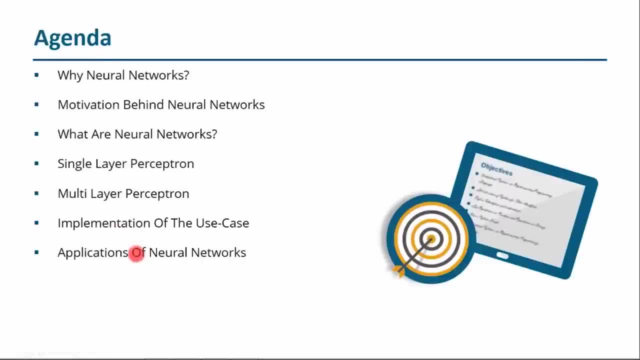 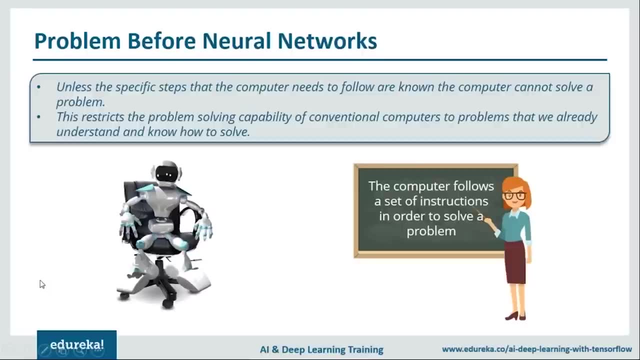 how to implement the use case that I was talking about in the beginning, about the various applications of neural networks. so we'll move forward and we'll understand why we need neural networks. so, in order to understand why we need neural networks, we are going to compare the approach. 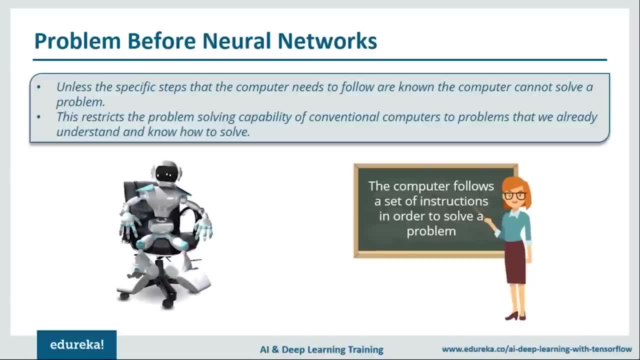 before and after neural networks and we'll see what were the various problems that were there before neural networks, so earlier conventional computers use an algorithmic approach, that is, the computer follows a set of instructions in order to solve a problem and unless the specific steps that the computer 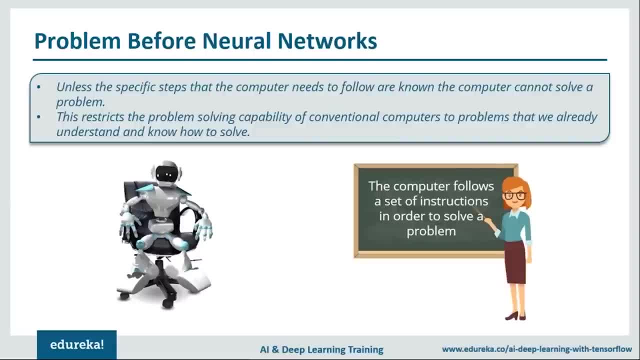 needs to follow are known. the computer solves the problem, so obviously we need a person who actually knows how to solve that problem and he or she can provide the instructions to the computer as to how to solve that particular problem, right? so we first should know the answer to that problem. 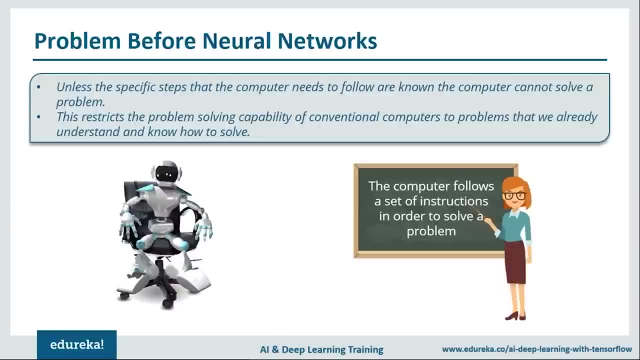 or we should know how to overcome that challenge or problem which is there in front of us. then only we can provide instructions to the computer. so this restricts the problem solving capability of conventional computers to problems that we already understand and know how to solve. but what about? 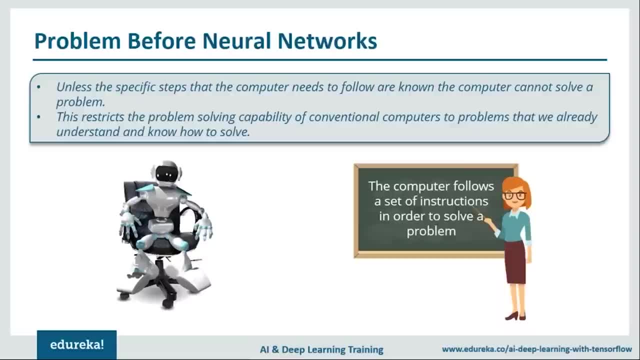 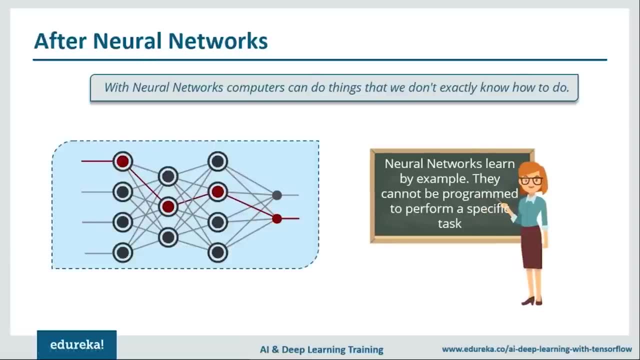 those problems whose answer was not solved by the computer. so that's where our traditional approach was a failure. so that's why neural networks were introduced. now let us see what was the scenario after neural networks. so neural networks basically process information in a similar way the human brain does. 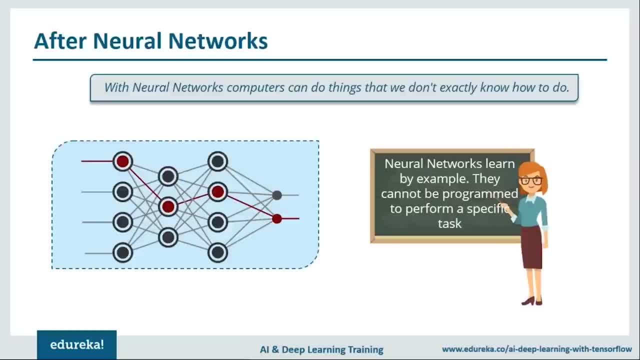 and these networks? they actually learn from examples. you cannot program them to perform a specific task. they will learn from their examples, from their experience, so you don't need to provide all the instructions, right? so this is what basically neural network does. so, even if you don't know, 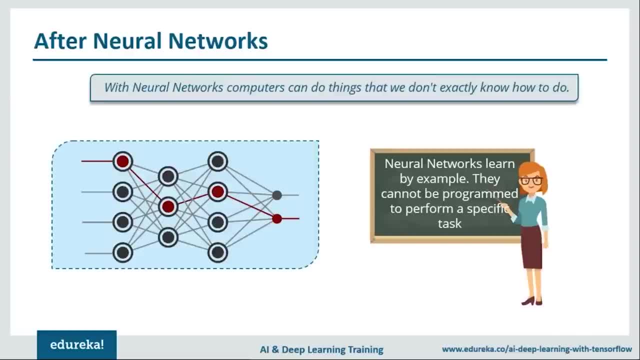 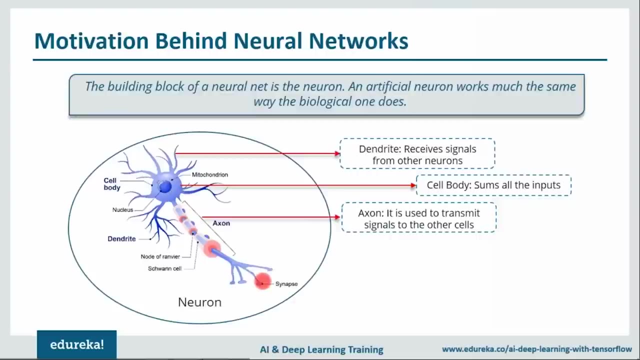 how to solve a problem. you can train your network in such a way that, with experience, it can actually learn how to solve the problem. so that was a major reason why neural networks came into existence. so we will move forward and we will understand what is the motivation. 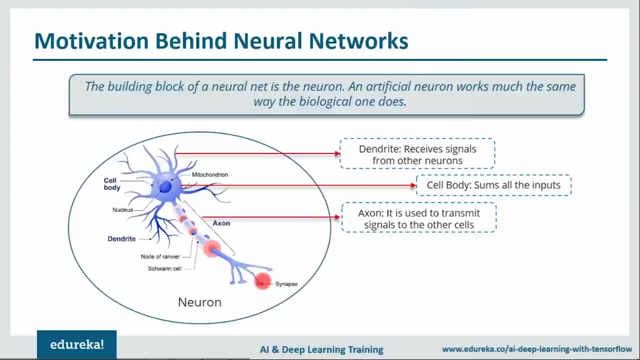 behind neural networks. so these neural networks are basically inspired by neurons, which are nothing but your brain cells. as I've told you earlier as well that neural networks work like human brain, and so the name and similar to a newborn human baby, as he or she learns from his or her. 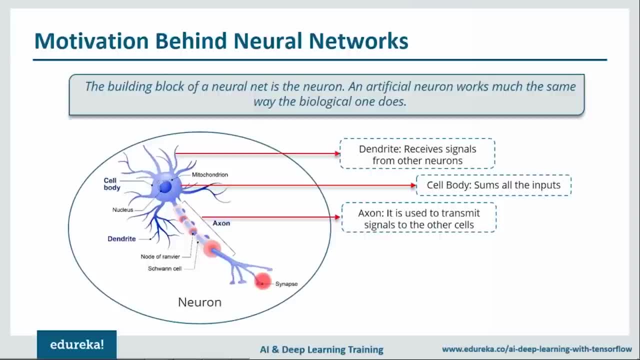 experience. we want a network to do that as well, but we want it to do very quickly. so here's a diagram of a neuron. basically, a biological neuron receives input from other sources, combines them in some way, perform a generally non-linear operation on the result and then outputs. 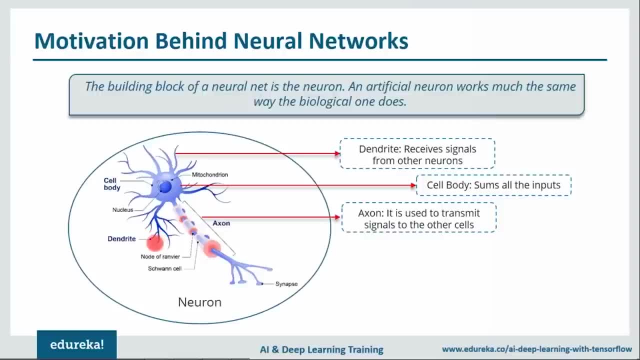 the final result. so here, if you notice these dendrites, these dendrites will receive signals from the other neurons. then what will happen? it will transfer it to the cell body. the cell body will perform some function. it can be summation, can be multiplication. so, after performing, 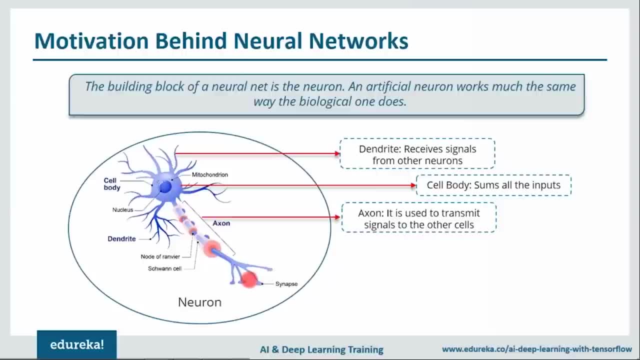 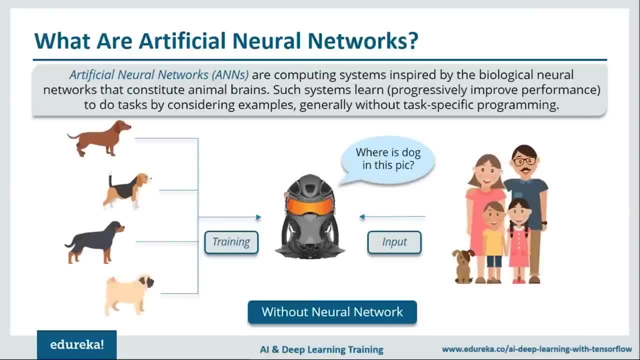 that summation on the set of inputs. via exon it is transferred to the next neuron. now let's understand what exactly are artificial neural networks. it is basically a computing system that is designed to simulate the way the human brain analyzes and process the information. artificial neural networks- 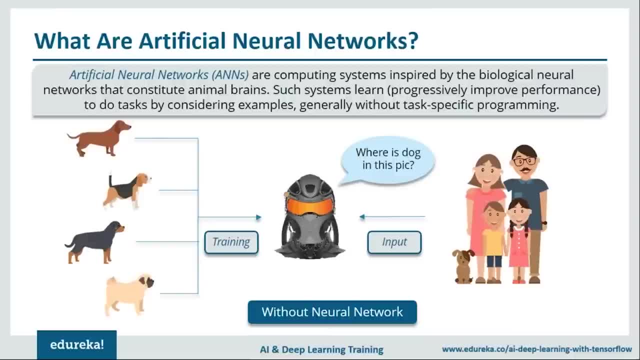 has self-learning capabilities that enable it to produce better results as more data becomes available. so if you train your network on more data, it will be more accurate. so these neural networks: they actually learn by example and you can configure your neural network for specific applications. it can be pattern recognition. 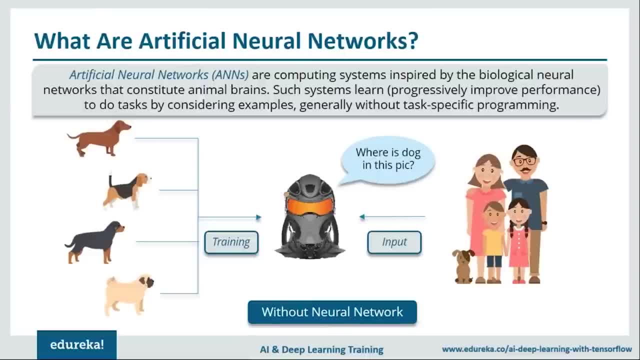 or it can be data classification, anything like that. alright, so because of neural networks, we see a lot of new technology has evolved, from translating web pages to other languages, to having a virtual assistant to order groceries, to using chat bots. all of these things are possible because of 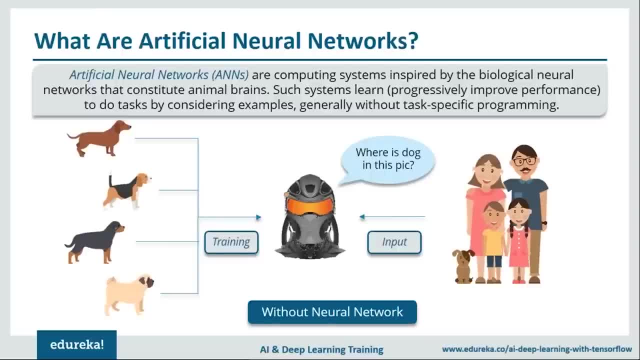 neural networks. so, in a nutshell, if I need to tell you, artificial neural network is nothing but a network of various artificial neurons, alright, so let me show you the importance of neural network with two scenarios, before and after neural network. so over here we have a machine and we have trained 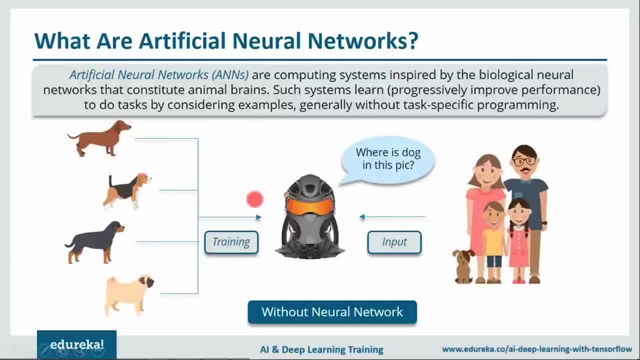 this machine on four types of dogs, as you can see where I am highlighting with my cursor, and once the training is done, we provide a random image of this dog. but this dog is not like the other dogs on which we have trained our system on, so without neural networks. 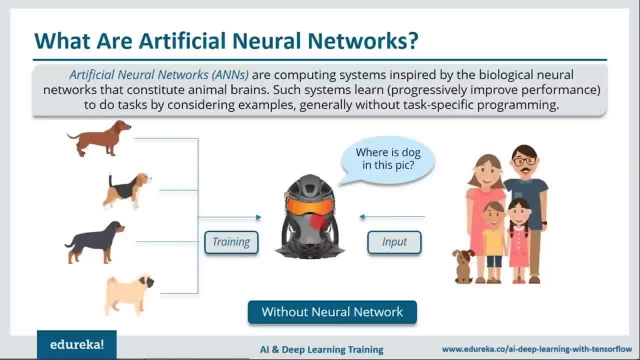 our machine cannot identify that dog in the picture as you can see it over here. basically, our machine will be confused. it cannot figure out where the dog is now. when I talk about neural networks, even if we have not trained our machine on this specific dog, but still. 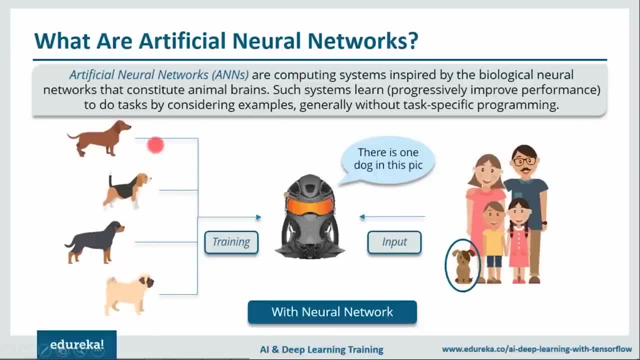 it can identify certain features of the dogs that we have trained on and it can match those features with the dog that is there in this particular image of the dog. so this happens all because of neural networks. so this is just an example to show you how important 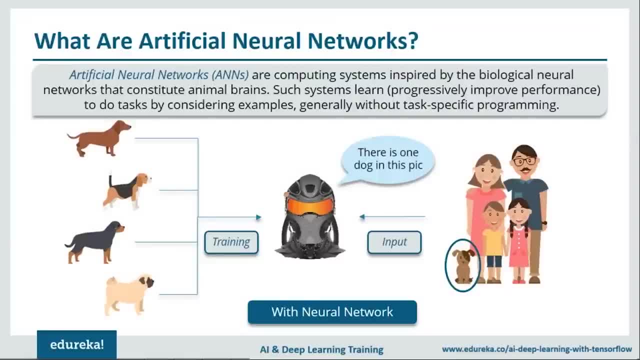 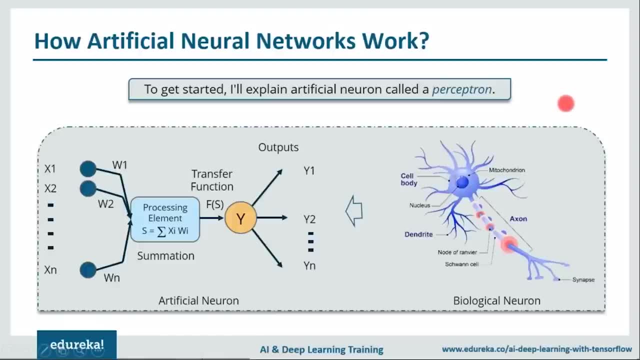 our neural networks. now I know you all must be thinking how neural networks work. so for that we'll move forward and understand how it actually works. so over here I'll begin by first explaining a single artificial neuron that is called as perceptron. so this is an example. 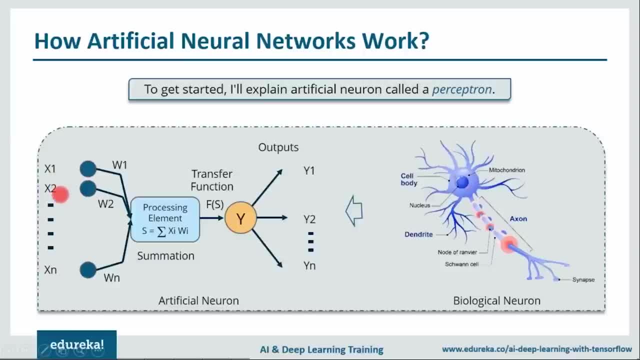 of a perceptron over here. we have multiple inputs: x1, x2, dash, dash, dash till xn, and we have corresponding weights as well: x1, w2 for x2, similarly wn for xn. then what happens? we calculated the weighted sum of these inputs and after doing that, 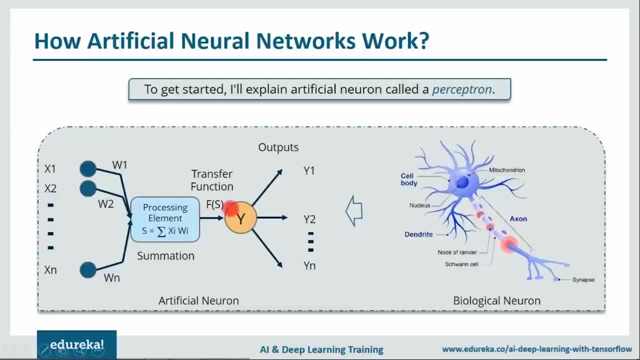 we pass it through an activation function. this activation function is nothing, but it provides a threshold value. so above that value my neuron will fire, else it won't fire. so this is basically an artificial neuron. so when I talk about a neural network it involves a lot of these. 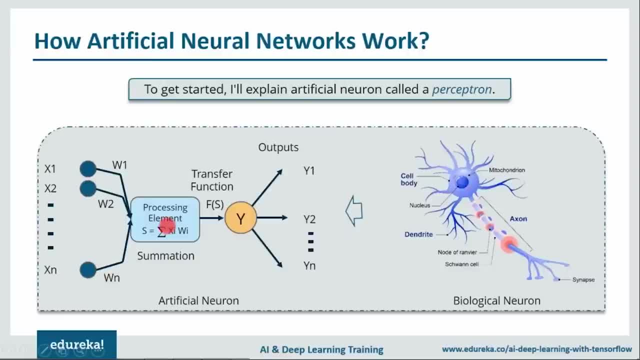 artificial neurons with their own activation function and their processing element. now we'll move on to the next step. we'll move forward and we'll actually understand various modes of this perceptron or single artificial neuron. so there are two modes in a perceptron. one is training. 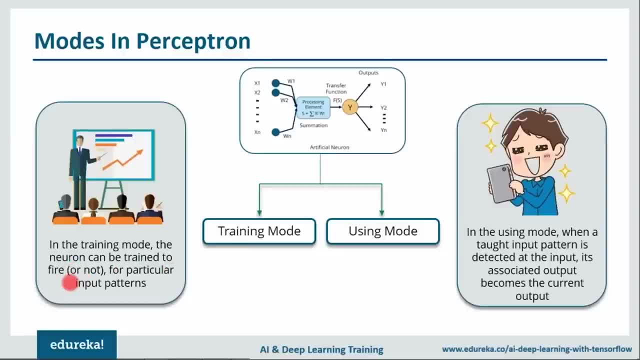 another is using mode. in training mode, the neuron can be trained to fire for particular input patterns, which means that we'll actually train our neuron to fire on certain set of inputs and to not fire on the other set of inputs. that's what basically training mode is. 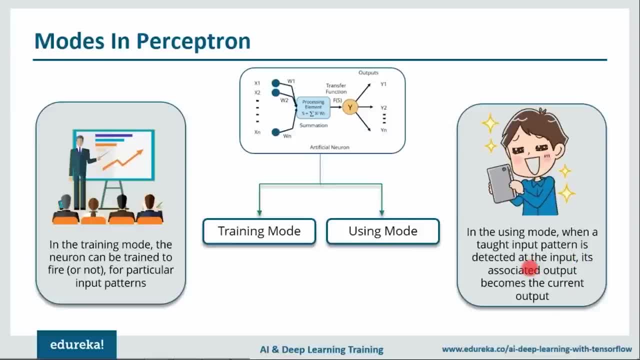 when I talk about using mode, it means that when a taut input pattern is detected at the input, its associated output becomes the current output, which means that once the training is done and we provide an input on which the neuron has been trained on, so it'll detect. 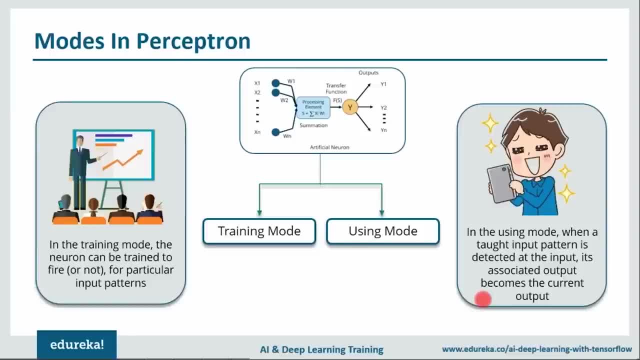 the input and will provide the associated output. so that's what basically using mode is. so first you need to train it, then only you can use your perceptron or your network. so these are the two modes, guys. next up we'll understand what are the various activation functions. 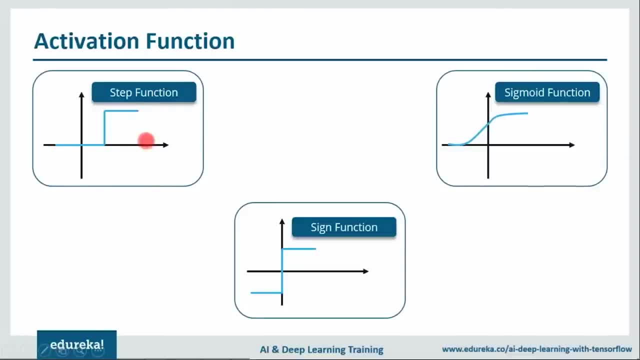 available. so these are the three activation functions, although there are many more, but I've listed down three step function, so over here. similarly for sigmoid and sine function as well. so these are three activation functions. there are many more, that I've told you earlier as well, so these are the three. 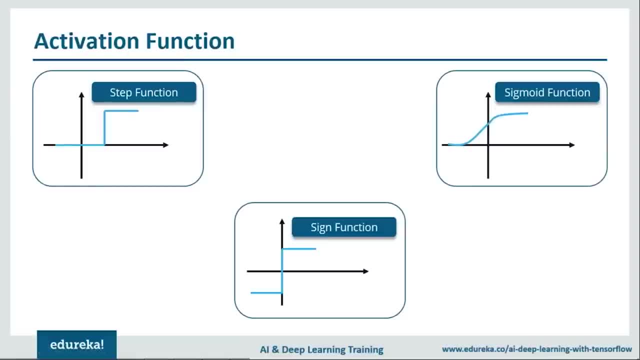 majorly used activation functions. next up, what we are going to do, we are going to understand how a neuron learns from its experience. so I'll give you a very good analogy in order to understand that and later on when we talk about the neural networks. or you can say: 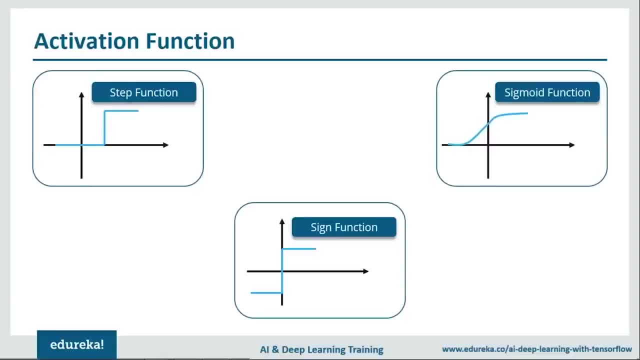 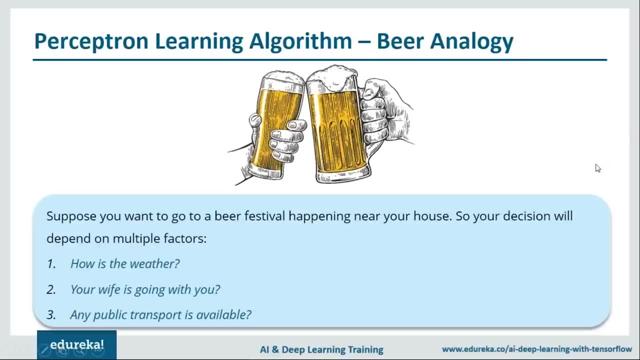 multiple neurons in a network. I'll explain you the math behind it. I'll explain you the math behind learning. so, guys, trust me, that analogy is pretty interesting. so I know all of you must have guessed it. so these are two beer mugs and all of you. 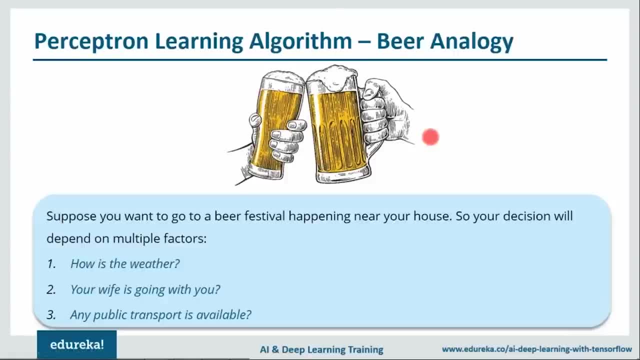 who love beer can actually relate to this analogy a lot, and I know most of you actually love beer, so that's why I've chosen this particular analogy, so that all of you can relate to it, all right, jokes apart. so fine guys, so there's a beer festival. 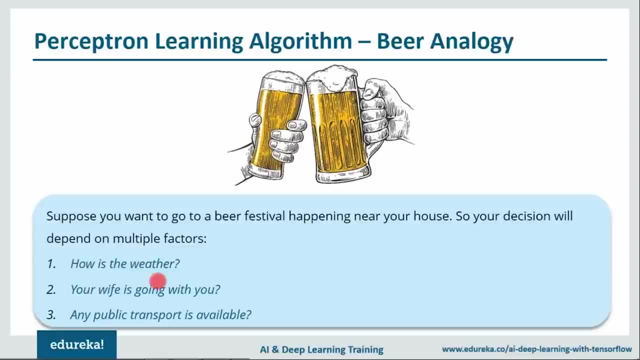 happening near your house and you want to badly go there, but your decision actually depends on whether you go or not. second is, your wife or husband is going with you or not? and the third one is: any public transport is available. so, on these three factors, your decision. 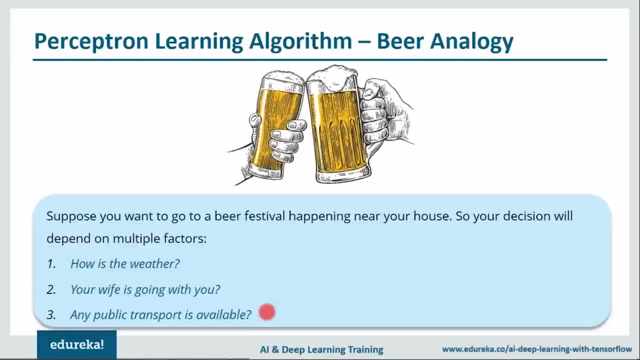 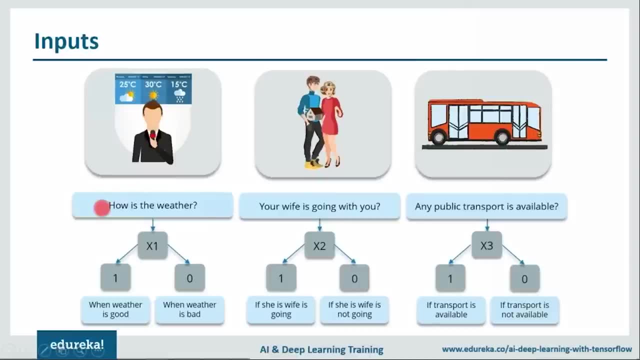 will depend whether you'll go or not. so we'll consider these three factors as inputs to our perceptron and we'll consider our decision of going or not going to the beer festival as our output. so let us move forward with that and we'll see if it's going. 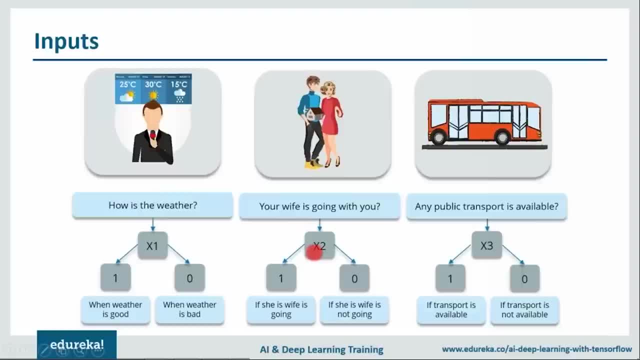 or not. if it's going, then it's one, if it's not going, then it's zero. similarly, for public transport, if it is available, then it is one, else it is zero. so these are the three inputs that I'm talking about. let's see the output. 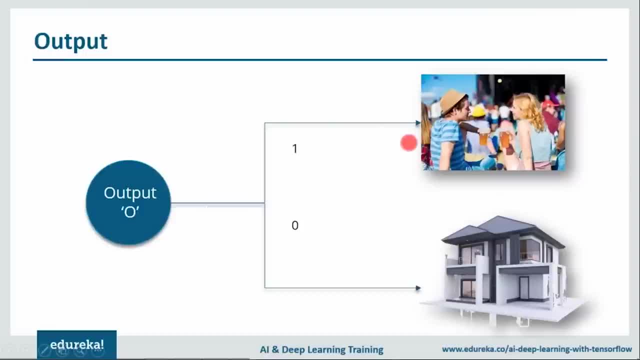 so output will be one when you're going to the beer festival and output will be zero when you want to relax at home. you want to have beer at home, only you don't want to go outside. so these are the two outputs, whether you're going or you're not going. 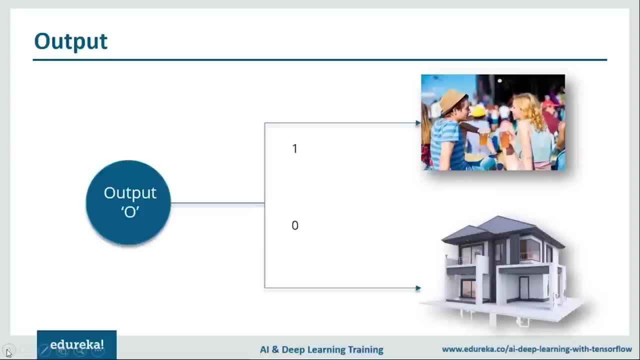 now what a human brain does over here, over here. okay, fine, I need to go to the beer festival, but there are three things that I need to consider. but will I give importance to all these factors equally? definitely not. there will be certain factors which will be of higher priority for me. 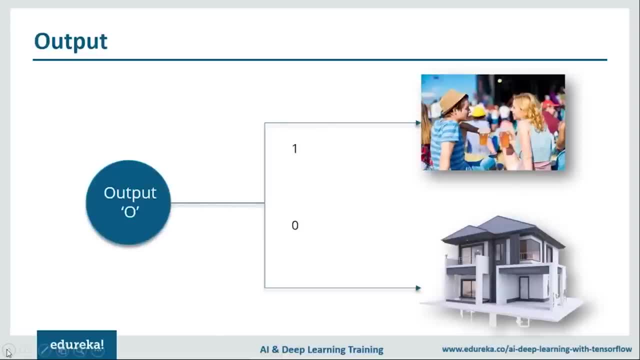 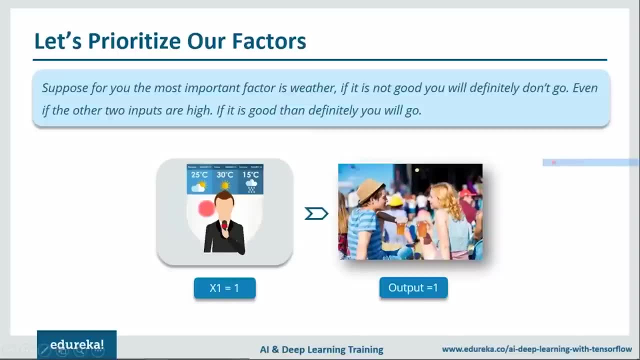 I'll focus on those factors more, whereas few factors won't affect that much to me. alright, so let's prioritize our inputs or factors. so here, our most important factor is weather. so if weather is good, I love beer so much that I don't care, even if my wife is going. 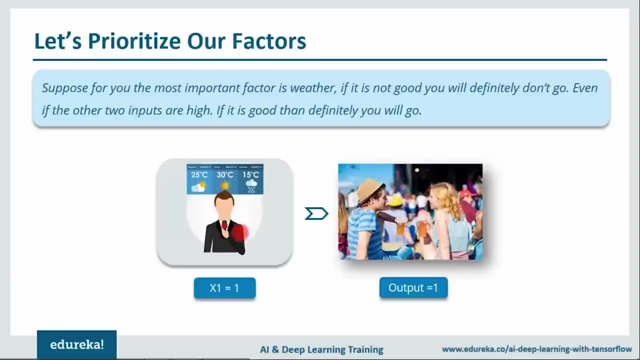 with me or not, or if there is a public neighborhood available. so I love beer that much that if weather is good, that definitely I'm going there. that means when x1 is high, output will be definitely high. so how we do that, how we actually prioritize our factors, 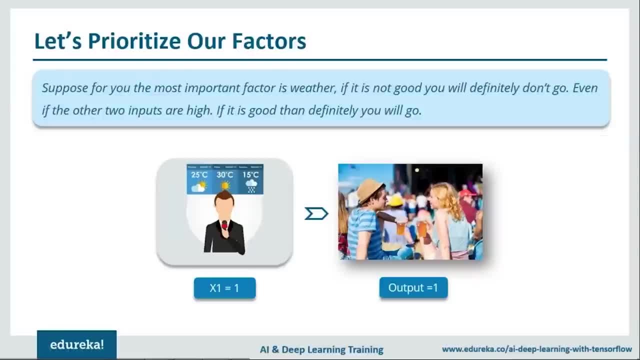 or how we actually give importance more to a particular input and less to another input in a perceptron or in a neuron. so we do that by using weights. so we assign high weights to the more important factors or more important inputs and we assign low weights to those particular inputs. 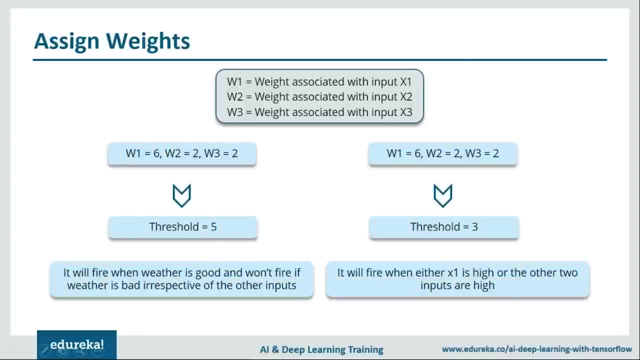 which are not that important for us. so let's assign weights, guys. so weight w1 is associated with input x1, w2 with x2 and similarly w3 with x3. now, as I've told you earlier as well, that weather is a very important factor. 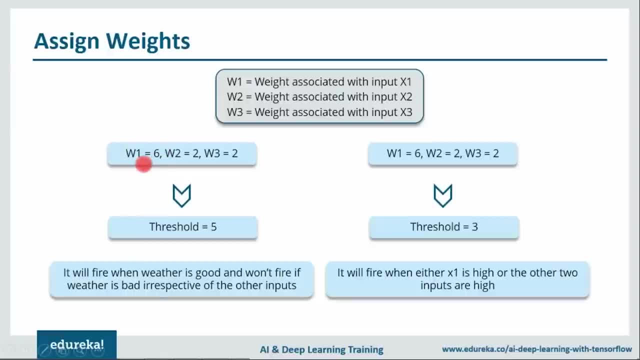 so I'll assign a pretty high weight to weather and I'll keep it as 6. similarly, w2 and w3 are not that important, so I'll keep it as 2 too. after that, I've defined a threshold value as 5, which means that 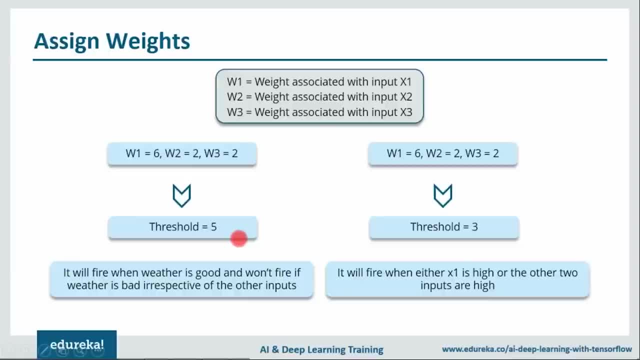 when the weighted sum of my input is greater than 5, then only my neuron will fire. or you can say: then only I'll be going to the beer festival, alright, so I'll use my pen and we'll see what happens when weather is good. so when weather is good. 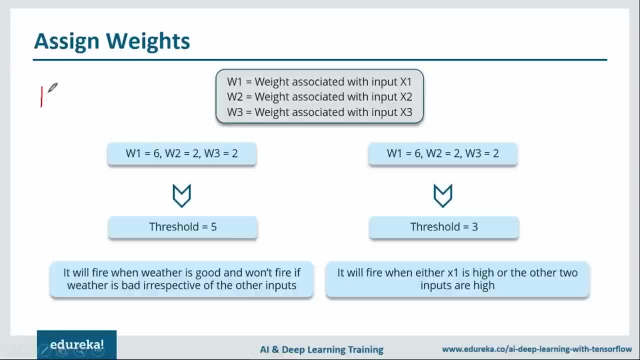 our x1 is 1, our weight is 6. we'll multiply it with 6. then if my wife decides that she is going to stay at home and she will probably be busy with cooking and she doesn't want to drink beer with me, so she's not coming. 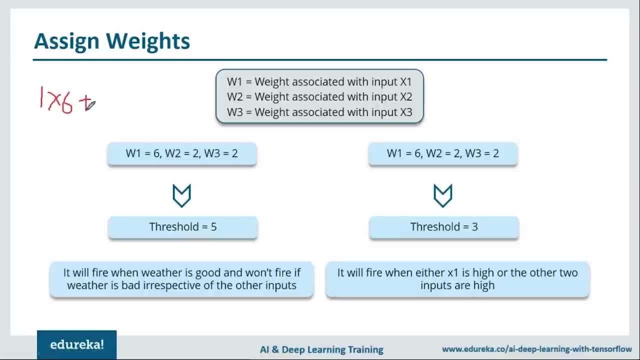 so that input becomes 0. 0 into 2 will actually make no difference, because it will be 0. then again there is no public transport available. also then also there is no public transport available, so that input becomes 0 available. also then also this will be 0. 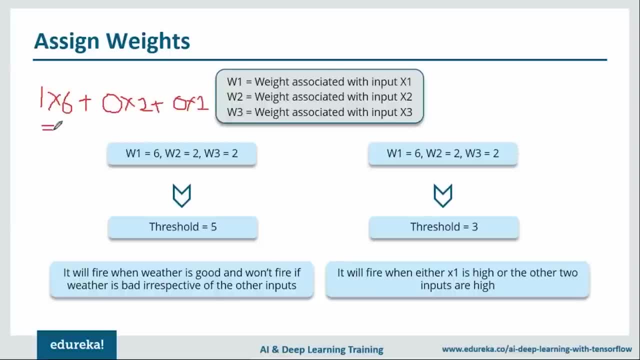 into 2. so what output I get here? I get here as 6 and notice the threshold value: it is 5. so definitely 6 is greater than 5. that means my output will be 1, or you can say my neuron will fire or I'll actually. 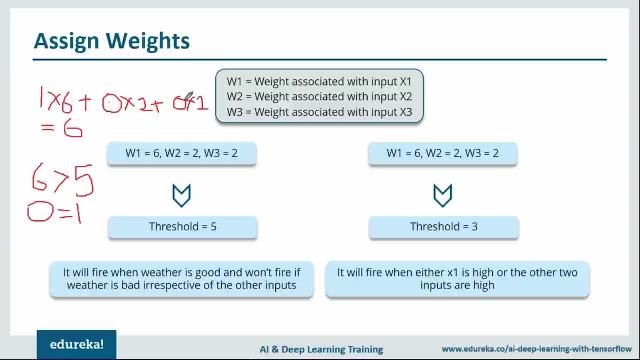 go to the beer festival. so even if these two inputs are 0, for me that means my wife is not willing to go with me, there is no public transport available, but weather is good, which has very high weight value and it actually matters a lot to me. 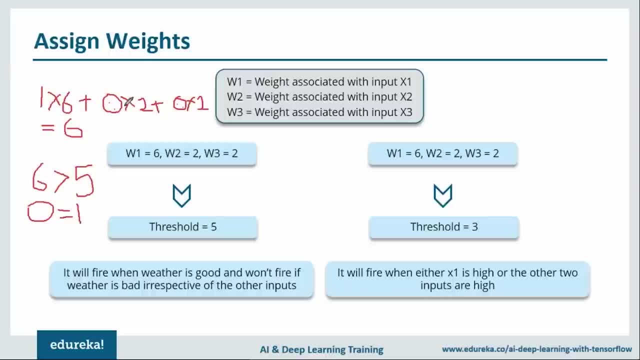 so if that is high, it doesn't really matter whether the two inputs are high or not. I will definitely go to the beer festival. all right, now I'll explain you a different scenario. so over here our threshold was 5. but what if I change this threshold? 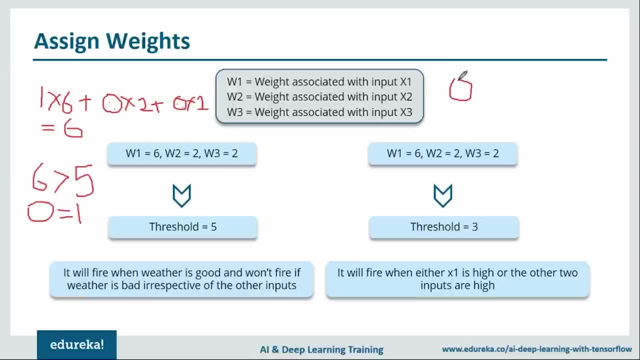 to 3. so in that scenario, even if my weather is not good, I'll give it a 0, so 0 into 6. but my wife and public transport both are available all right. so 1 into 2 plus 1 into 2, which is equal. 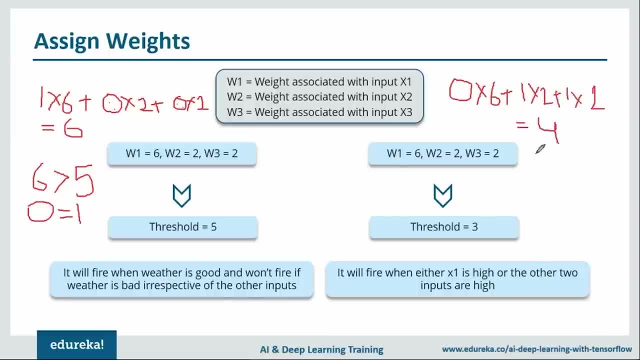 to 4, and it is definitely greater than 3. then also, my output will be 1. that means I will definitely go to the beer festival, even if weather is bad and my neuron will fire. so these are the two scenarios that I have discussed with you. 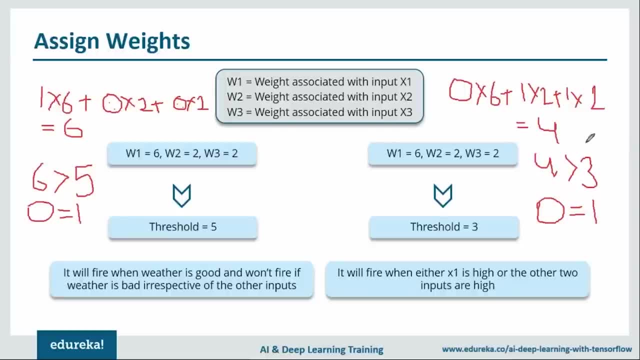 all right. so there can be many other scenarios in which you can actually assign weight to your problem or to your learning algorithm. so these are the two ways in which you can assign weights and prioritize your inputs or factors on which your output will depend, so obviously in real life. 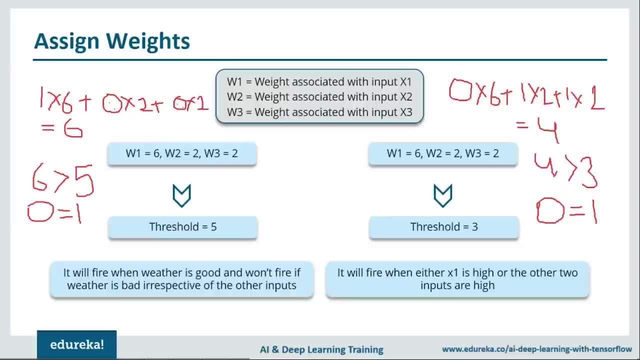 all the inputs or all the factors are not as important for you, so you actually prioritize them. and how you do that in perceptron, you provide high weight to it. this is just an analogy, so that you can relate to a perceptron to a real life we'll actually discuss. 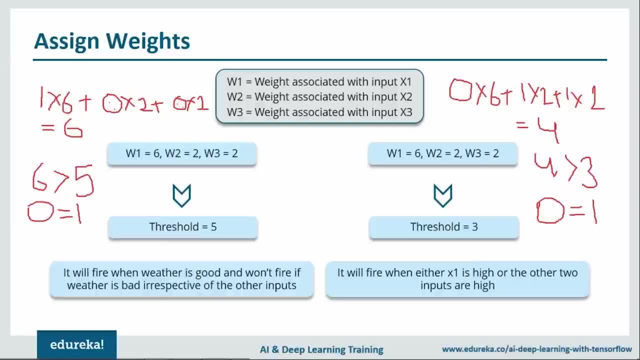 how a network or a neuron learns all right, so how the weights are actually updated and how the output is changing, that all those things will be discussing later in the session. but my aim is to make you understand that you can actually relate to a real life problem. 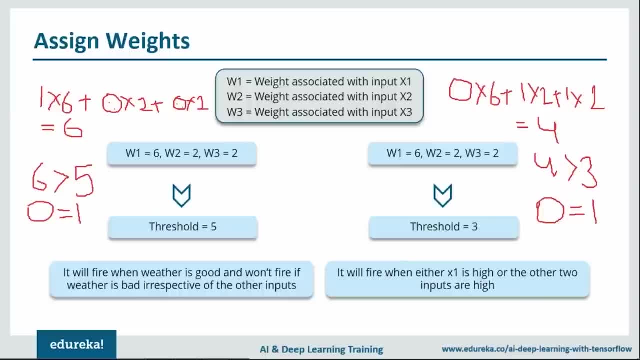 with that of a perceptron, all right. and in real life, problems are not that easy. they are very, very complex problems that we actually face. so in order to solve those problems, a single neuron is definitely not enough. so we need networks of neuron, and that's where 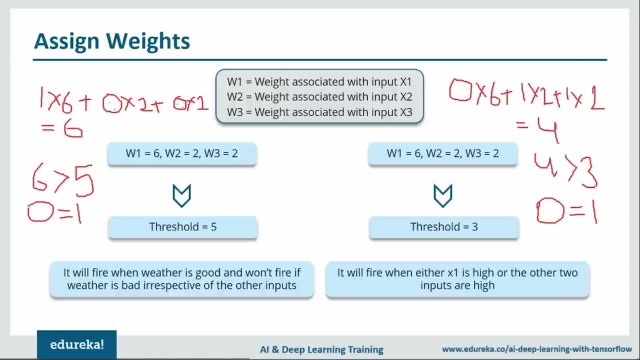 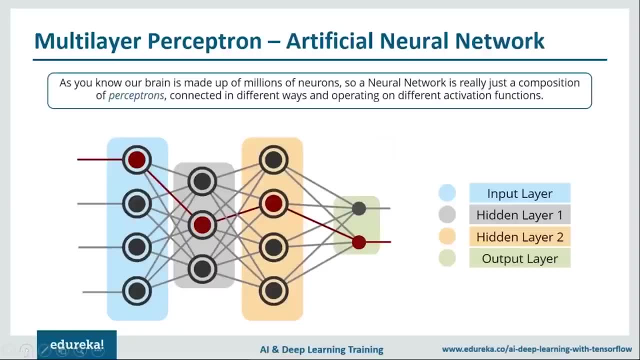 artificial neural network, or you can say multi-layer perceptron, comes into the picture. now let us discuss that multi-layer perceptron or artificial neural network. so this is how an artificial neural network actually looks like. so over here we have multiple neurons in present in different layers. 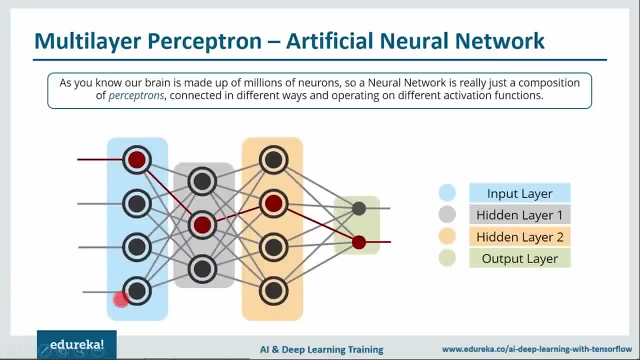 the first layer is always your input layer. this is where you actually feed in all of your inputs. then we have the first hidden layer, then we have second hidden layer and then we have the output layer, although the number of hidden layers depends on what are you working. 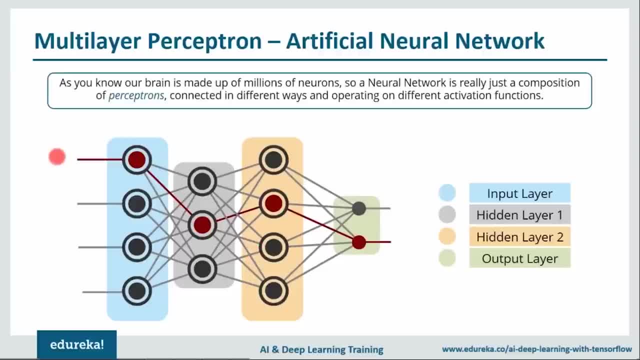 what is your problem? so that actually determines how many hidden layers you'll have. so let me explain you what is actually happening here. so you provide in some input to the first layer, which is nothing but your input layer. you provide inputs to these neurons, alright, and after some function, 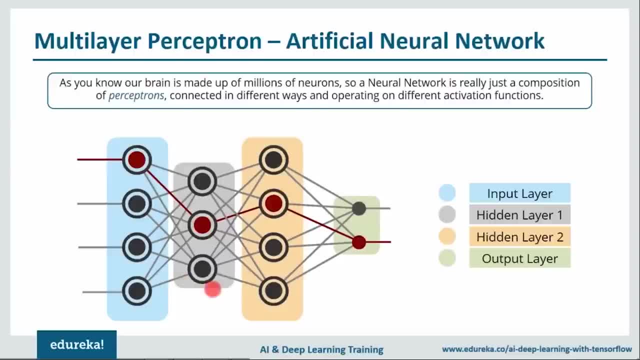 the output of these neurons will become the input to the next layer, which is nothing but your hidden layer one. then these hidden layers also have various neurons. these neurons will have different activation functions, so they'll perform their own function on the inputs that it receives. so the output. 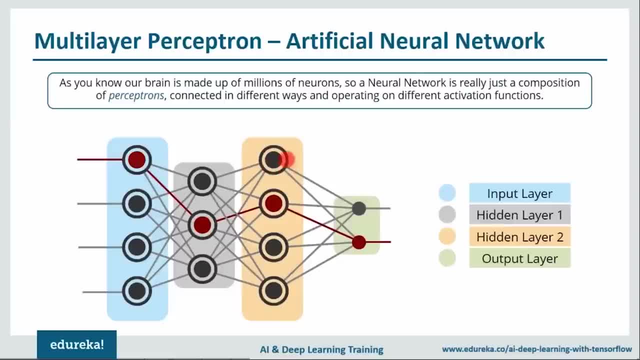 of this layer will be the input to the next hidden layer, which is hidden layer two. similarly, the output of this hidden layer will be the input to the output layer and finally we get the output. so this is how, basically, an artificial neural network looks like. now let me explain you. 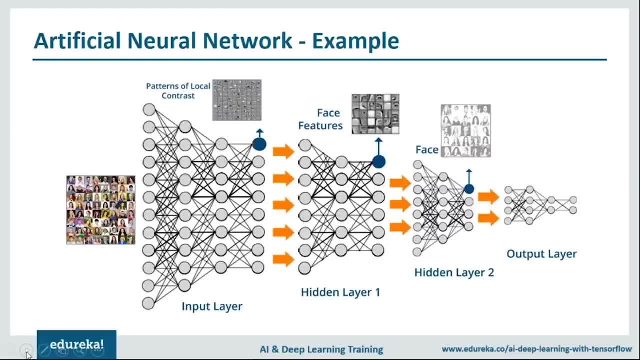 this with an example. so over here I'll take an example of image recognition using neural networks. so over here, what happens? we feed in a lot of images to our input layer. now this input layer will actually detect the patterns of local contrast, and then we'll feed. 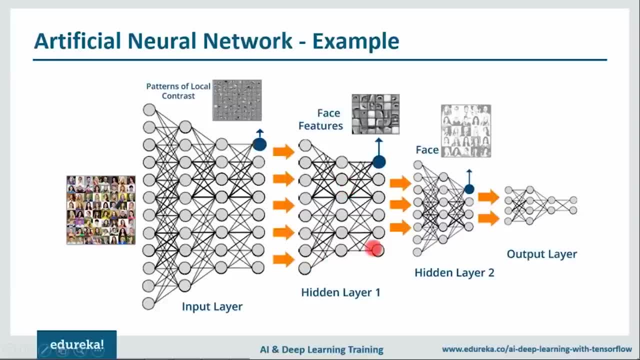 that to the next layer, which is hidden layer one. so in this hidden layer one the face features will be recognized. we recognize eyes, nose, ears, things like that- and then that will be again fed as input to the next hidden layer, and in this hidden layer we'll assemble. 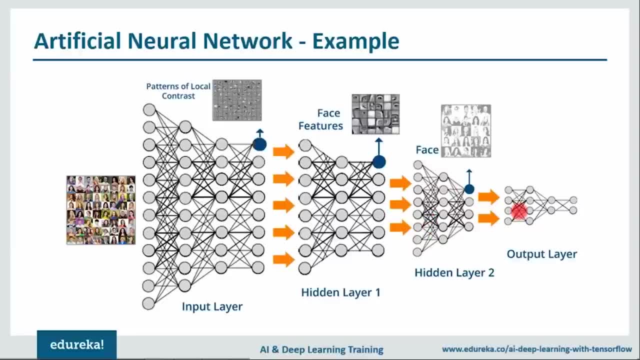 those features and we'll try to make a face and then we'll get the output, that is, the face will be recognized properly. so, if you notice, here, with every layer we are trying to get a more abstract version or the generalized version of the input. so this is basically. 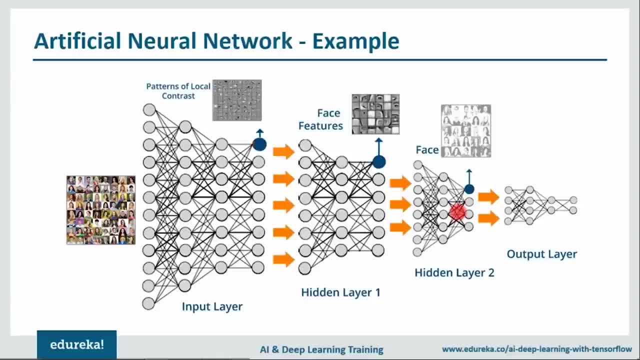 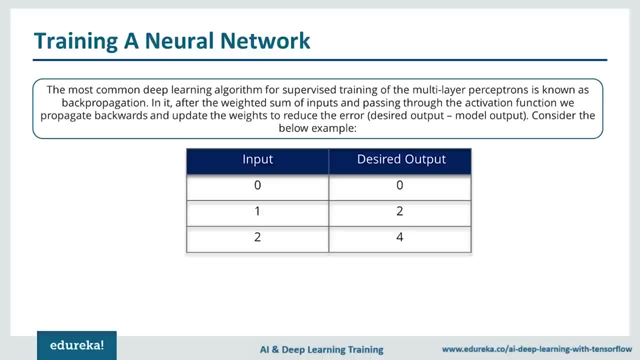 an artificial neural network, how it works, all right, and there's a lot of training and learning which is involved that I'll show you now: training a neural network, so how we actually train a neural network. so, basically, the most common algorithm for training a network is called. 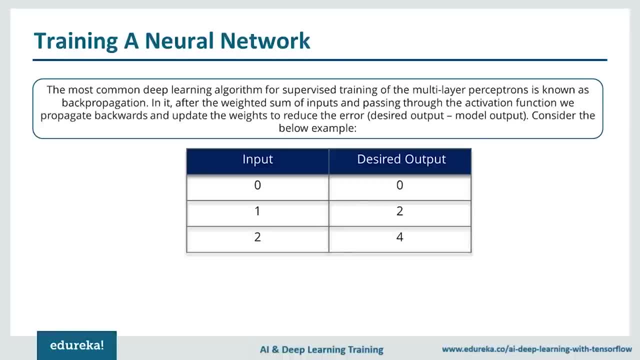 back propagation. so what happens in back propagation? after the weighted sum of inputs and passing through an activation function and getting the output, we compare that output to the actual output that we already know, we figure out how much is the difference, we calculate the error and, based on that error, 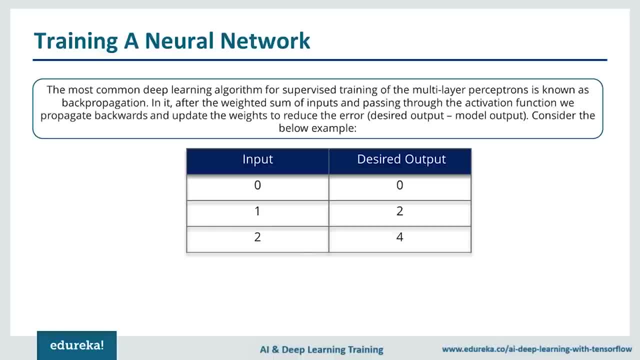 what we do, we propagate backwards and we'll see what happens when we change the weight. will the error decrease or will it increase? and if it increases, when it increases, by increasing the value of the variables or by decreasing the value of variables. so we kind of calculate. 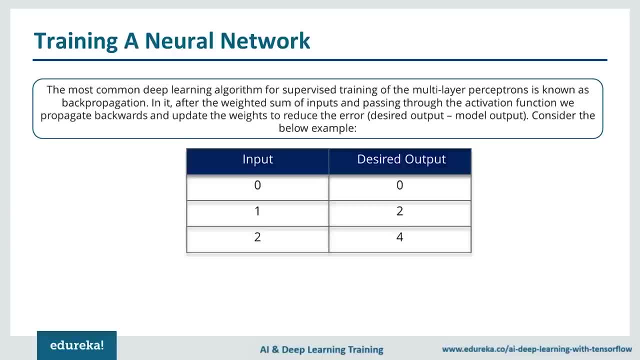 all those things and we update our variables in such a way that our error becomes minimum. and it takes a lot of iterations. trust me guys, it takes a lot of iterations. we get output a lot of times and then we compare it with the model, with the actual output. 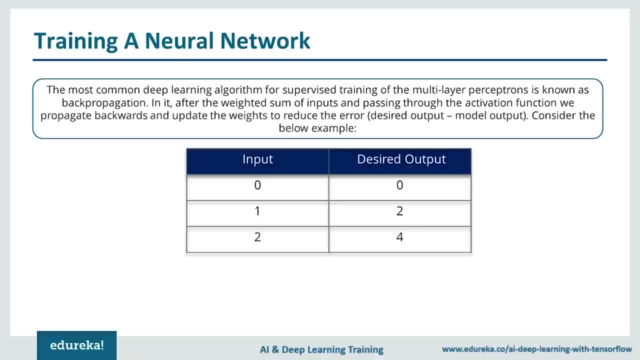 we propagate backwards. we change the variables and again we calculate the output, we compare it again with the desired output of the actual output. then again we propagate backwards. so this process keeps on repeating until we get the minimum value. All right. So there's an example. 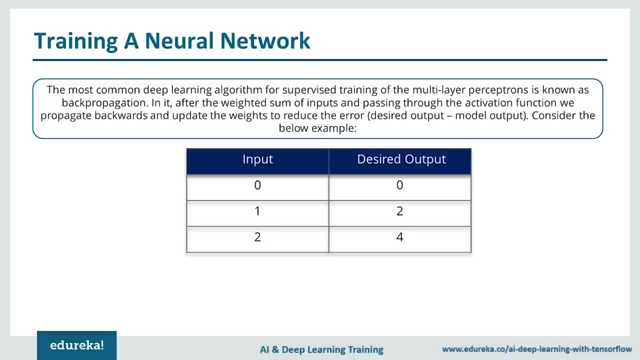 that is there in front of your screen. don't be scared of the terms that I use. I'll actually explaining with an example. So this is the example over here. we have 0, 1 and 2 as inputs and our desired output or the output. 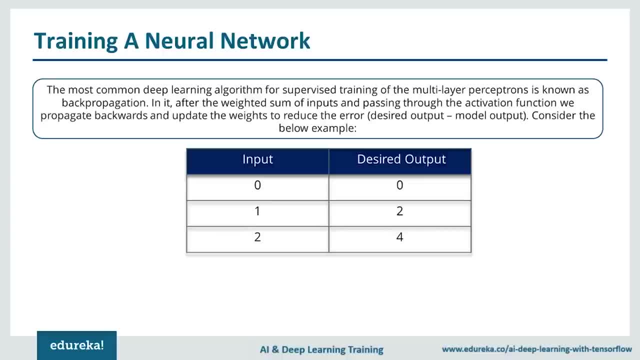 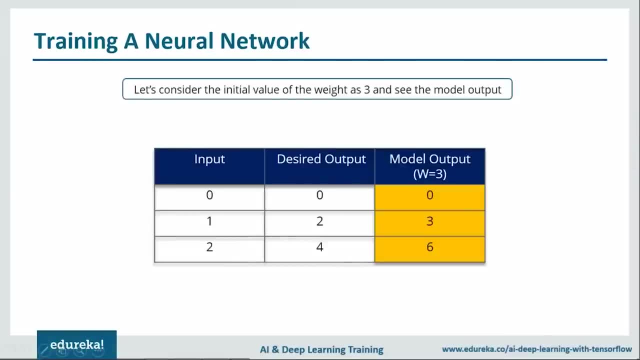 that we already know is 0, 1 and 4. all right, So over here. but I'm training a computer to do that right. The computer is not a human. So what happens? I actually initialize my weight. I keep the value as 3. 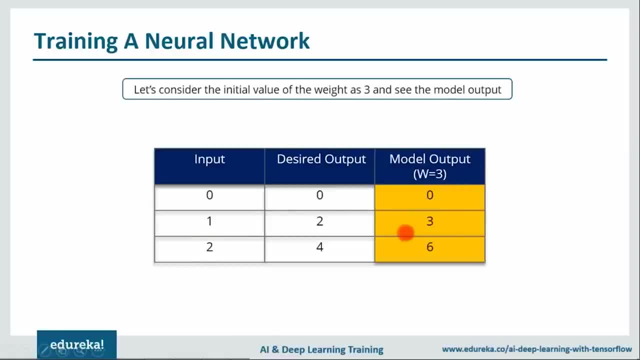 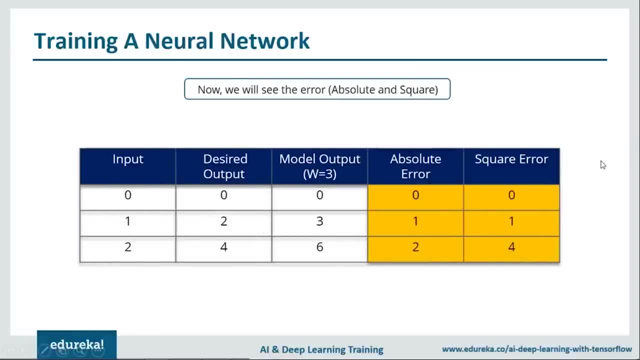 so the model output will be: 3 into 0 is 0, 3 into 1 is 3, 3 into 2 is 6. now, obviously it is not equal to your desired output. So we check the error now, the error that we have got here. 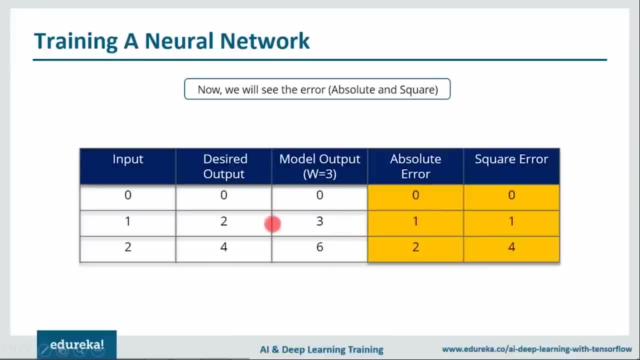 is 0, 1 and 2, which is nothing but your difference. So 0 minus 0 is 0, 3 minus 2 is 1, 6 minus 4 is 2. now this is called an absolute error. after squaring this error. 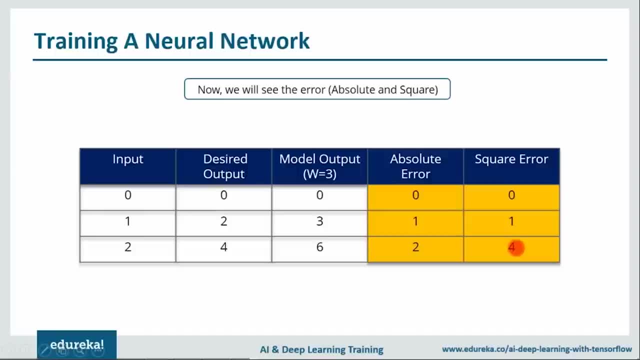 we get square error, which is nothing but 0, 1 and 4. all right, So now what we need to do? we need to update the variables. We have seen that the output that we got is actually different from the desired output, So we need to update. 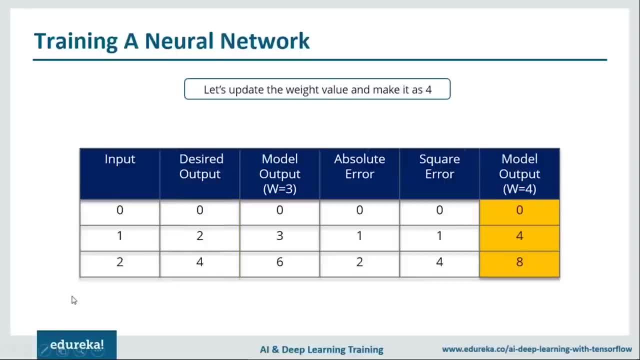 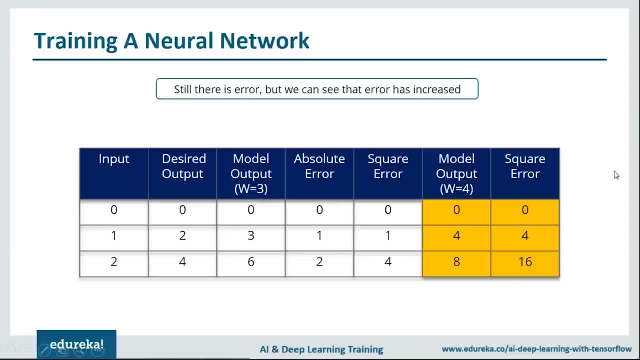 the value of the weight. So instead of 3, our computer makes it as 4. after making the value as 4, we get the model output as 0, 4 and 8, and then we saw that the error has actually increased instead of decreasing. 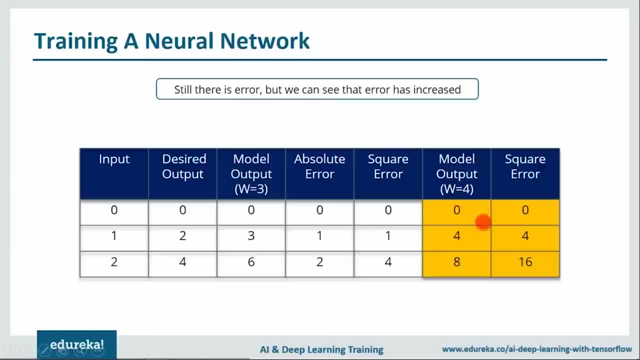 the error has increased. So after updating the variable, the error has increased. So you can see that square error is 0, 4 and 16, and earlier it was 0, 1 and 4. that means we cannot increase the weight value right now. 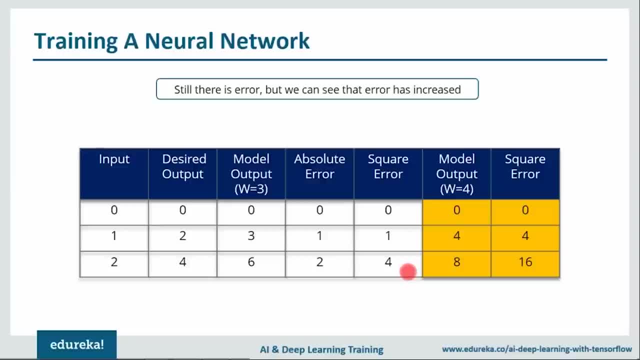 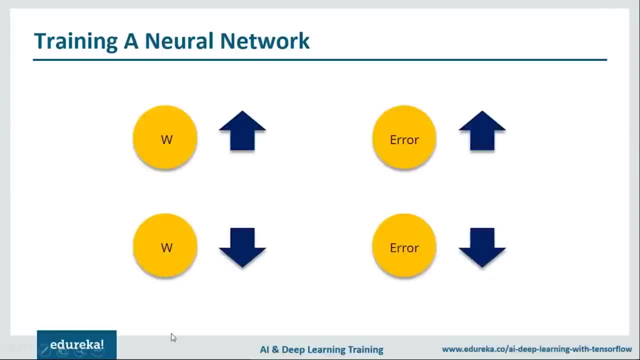 But if we decrease that, make it as 2, we get the output which is actually equal to desired out. but is it always the case that we need to only decrease the weight? definitely not, So in this particular scenario. whenever I'm increasing the weight, error is increasing. 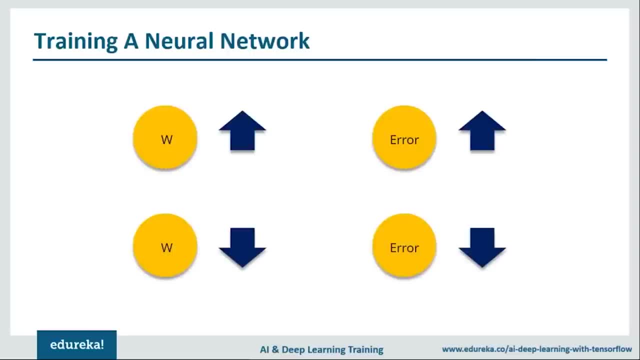 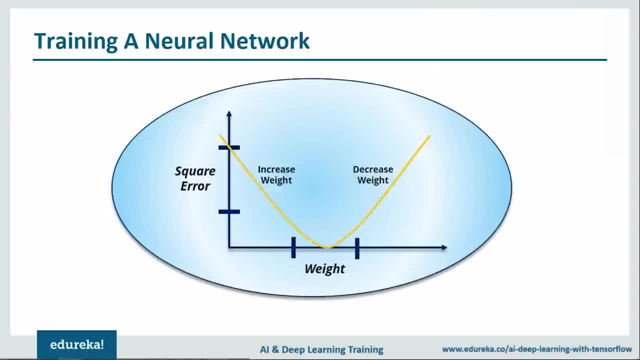 and when I'm decreasing the weight, error is decreasing. but, as I've told you earlier as well, this is not the case every time. sometimes you need to increase the weight as well. So I said: fine guys, This is how, basically, a computer decide whether it has to increase. 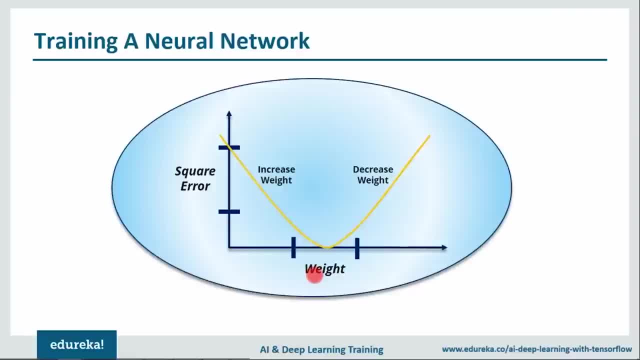 the weight or decrease away. So what happens here? This is a graph of square error versus weight. So over here, what happens? suppose your square error is somewhere here and your computer: it starts increasing the weight in order to reduce the square error and it notices: 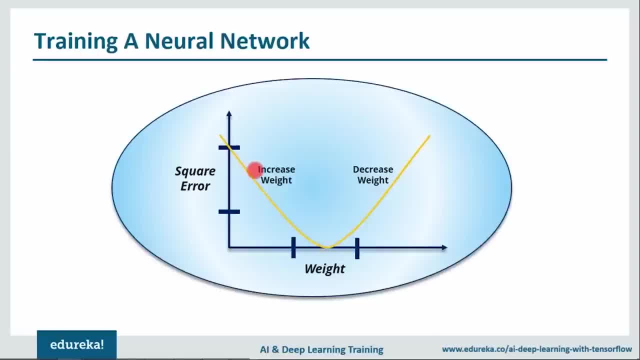 that whenever it increases the weight, square error is actually decreasing. So we'll keep on increasing until the square error reaches a minimum value and after that, when it tries to still increase the weight, the square error will increase. So that time our network will recognize that whenever it is increasing. 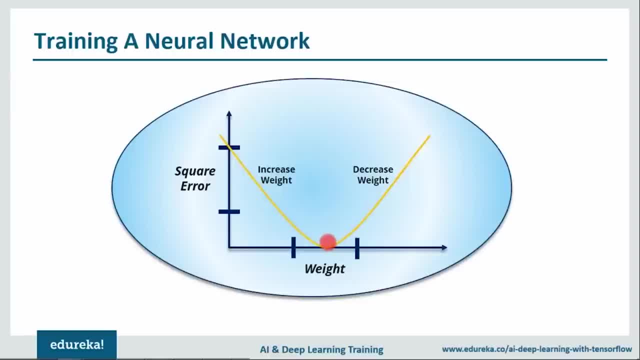 the weight after this point, error is increasing. So therefore it will stop right there and that will be our weight value. Similarly, there can be one more scenario. Suppose if we increase the weight, but then also the square error is increasing. So at that time 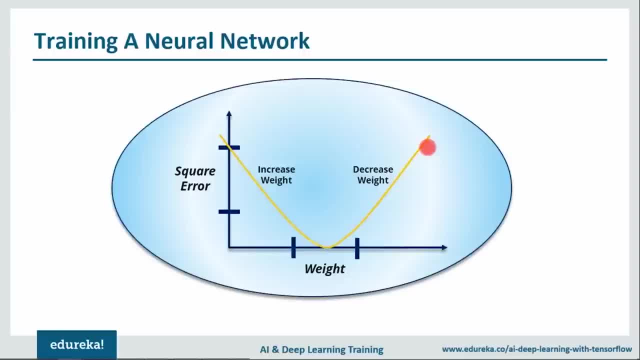 we cannot increase the weight. at that time computer will realize: okay, fine, whenever I'm increasing the weight, the square error is increasing. So it will go in the opposite direction. So we'll start decreasing the weight and the moment it decreases more, the square error again increases. 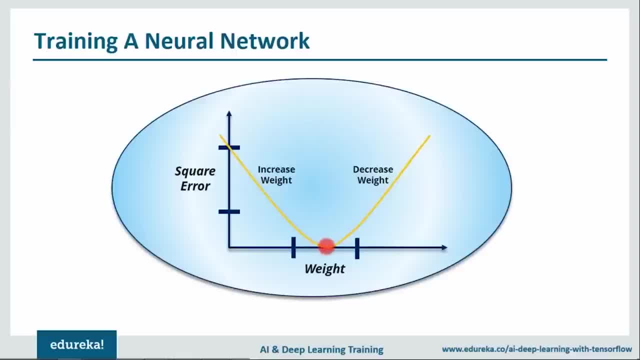 So our network will know that whenever it decreases the weight value, the square error is increasing, So that point will be our final weight value. So, guys, this is what basically back propagation, in a nutshell, is Fine, so we'll move forward, and now is the correct time. 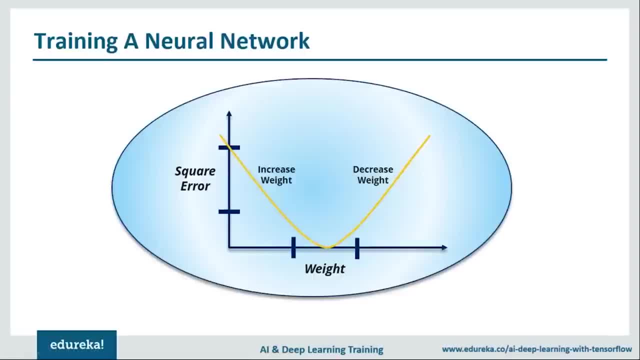 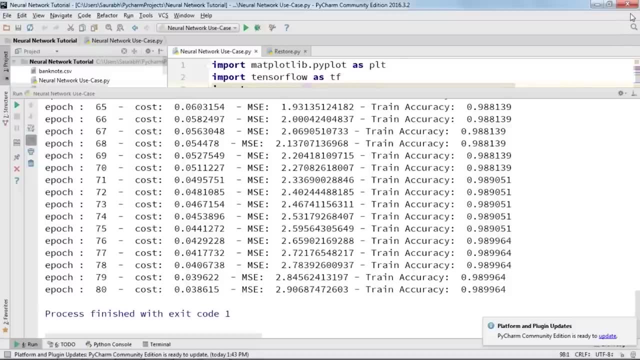 to understand how to implement the use case that I was talking about at the beginning, That is, how to determine whether a node is fake or real. So for that I'll open my PyCharm. This is my PyCharm. let me just close this. 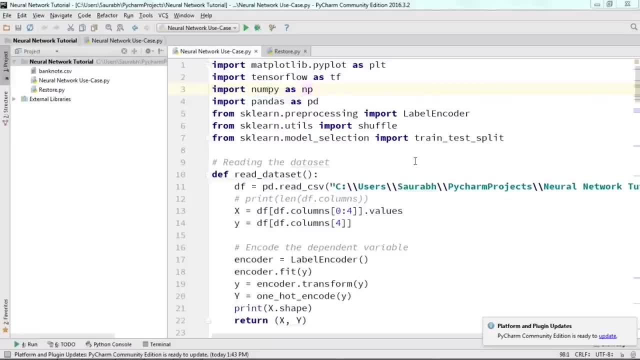 All right, So this is the code that I've written in order to implement the use case. So over here what we do: we import the first important libraries which are required. Matplotlib is used for visualization, TensorFlow, we know, in order to implement the neural networks. 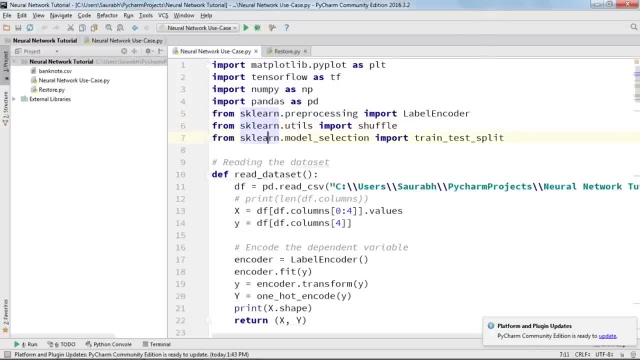 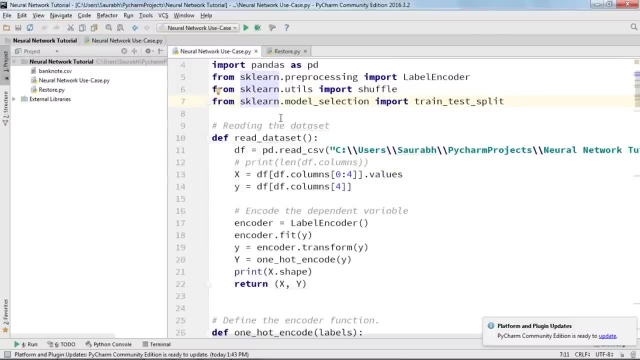 NumPy for arrays, Pandas for reading the data set, Similarly sklearn for label encoding as well as for shuffling and also to split the data set into training and testing paths. So we'll begin by first reading the data set in Pandas in order to read. 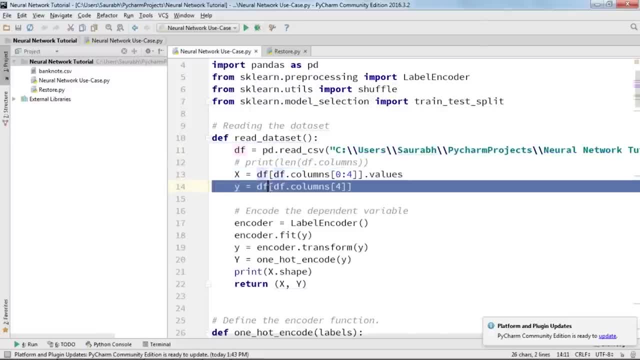 the CSV file which has the data set. After that I'll define features and labels. So X will be my feature and Y will contain my label. So basically, X includes all the columns apart from the last column, which is the fifth one. and because the indexing starts, 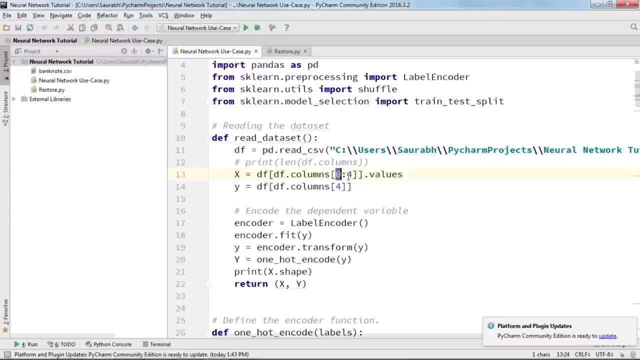 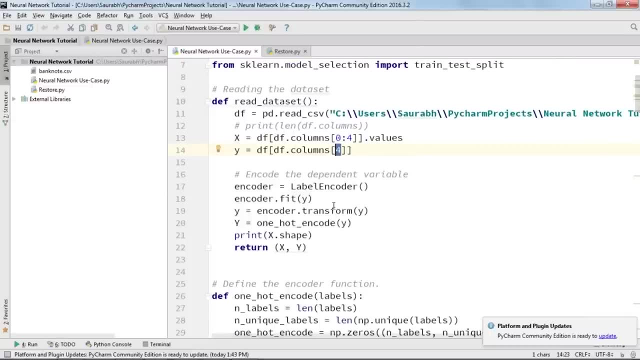 from zero. that's why we have written zero till fourth, So it won't include the fourth column. All right, And so our last column will actually be our label. Then what we need to do? we need to encode the dependent variable. So the dependent variable. 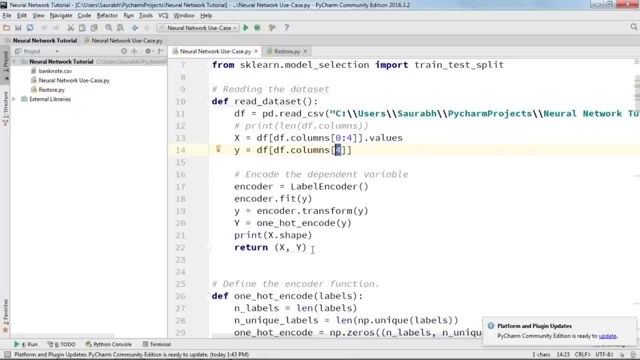 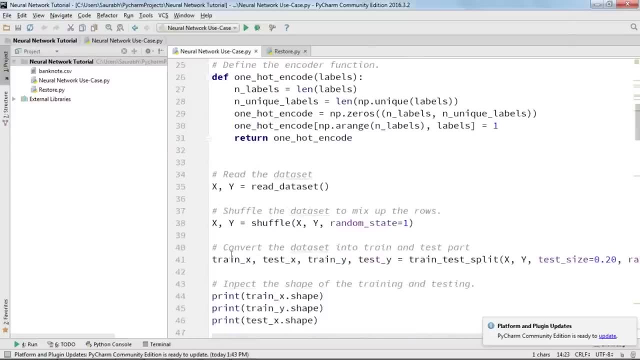 as I've told you earlier as well, is not your label, but your label. So I've discussed encoding in TensorFlow tutorial. you can go through it and you can actually get to know why and how we do that. Then what we have done, we have read the data set. 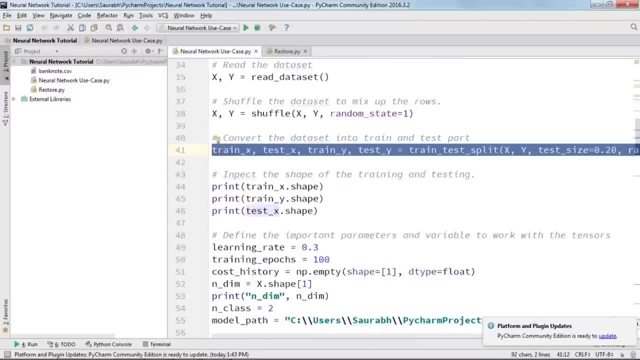 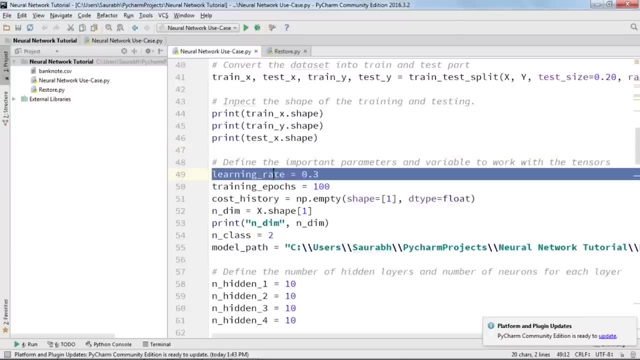 then what we need to do is to split our data set into training and testing, and these are all optional steps. You can print the shape of your training and test data. if you don't want to do it, it's still fine. Then we have defined. 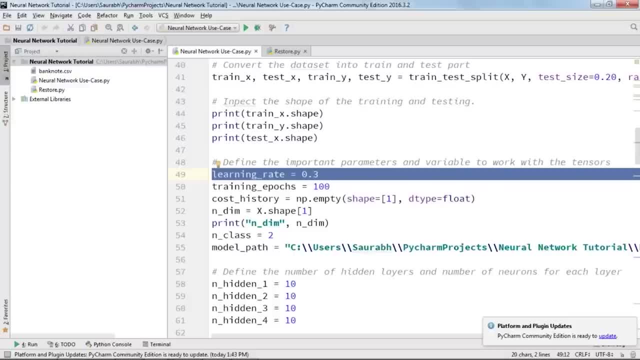 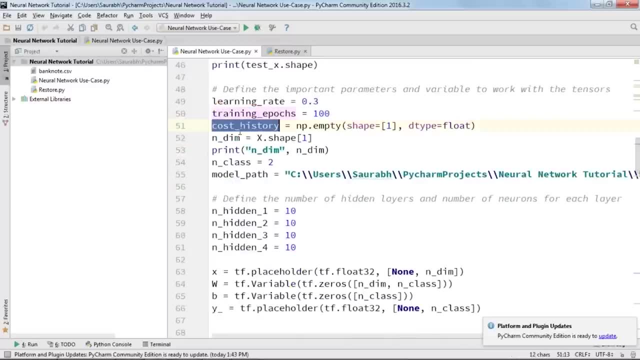 learning rate. So learning rate is actually the steps in which the weights will be updated. All right, So that is what basically learning rate is. So that's all the iterations. Then we have defined course history. that will be an empty numpy array and its shape will be one. 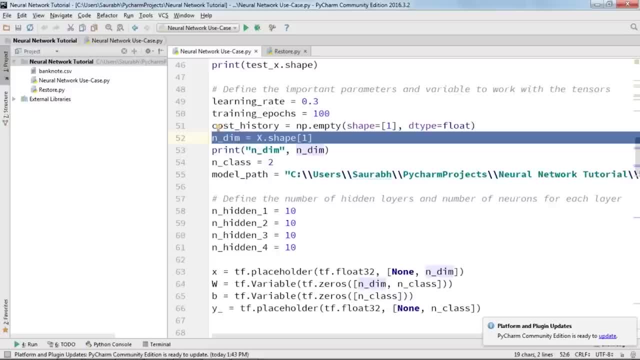 and it will include the flow type objects. Then we have defined end dim, which is nothing but your x shape of axis, one which means your column. Then we'll print that. After that we have defined the number of classes, So there can be only two classes. 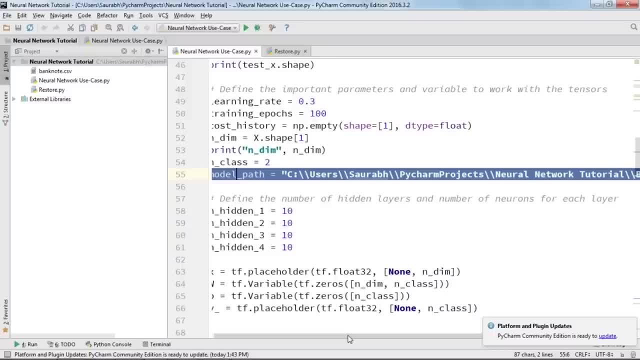 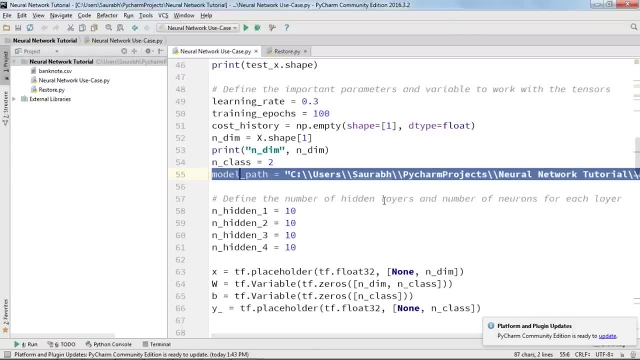 whether the node can be fake or it can be real. And this model path I've given in order to save my model. So I've just given a path where I need to save it. Now is the time to actually define our neural network. 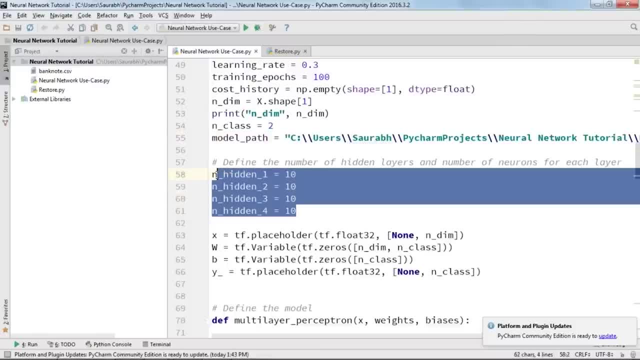 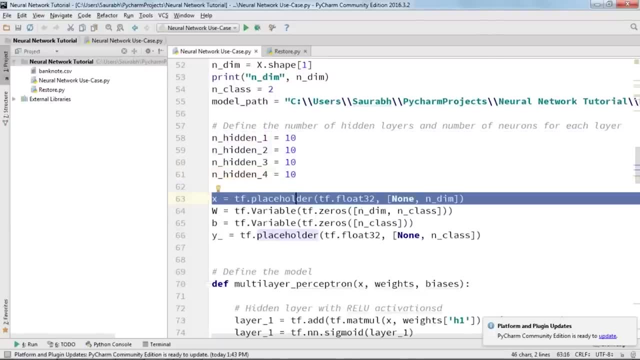 So we'll first make sure that we have defined the important parameters like hidden layers, number of neurons in hidden layers. So I'll take ten neurons in every hidden layer and I'm taking four layers like that. Then x will be my placeholder and the shape. 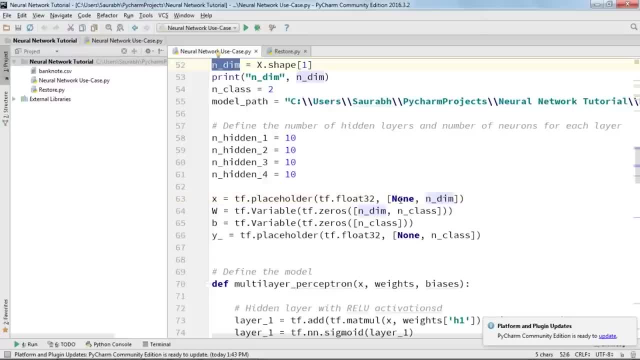 of this particular placeholder is none, n underscore, dim, n underscore, dim value. I'll get it from here- and none can be any value. I'll define one variable, w, and I'll initialize it with zeros, and this will be the shape. similarly for bias as well. 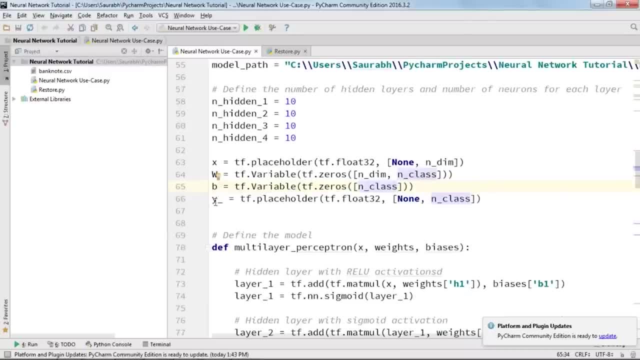 This will be the particular shape and there will be one more placeholder, y dash, which will actually be used in order to provide us with the actual output of the model. There'll be one model output and there'll be one actual output which we use in order to calculate. 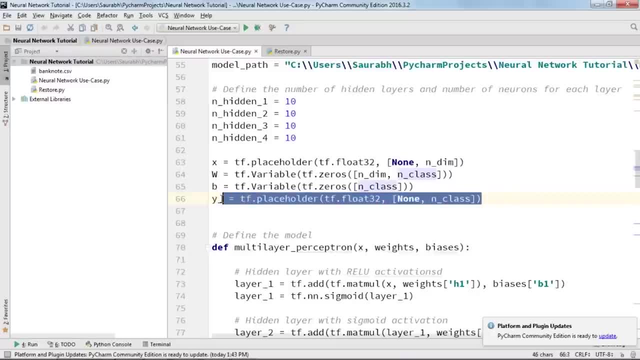 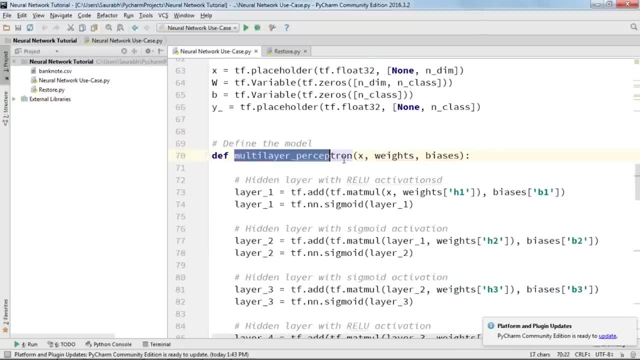 the difference right. So we'll feed in the actual values of the labels in this particular placeholder, y, dash, And now we'll define the model. So over here we have named the function as multi-layer perceptron, and in it we'll first define. 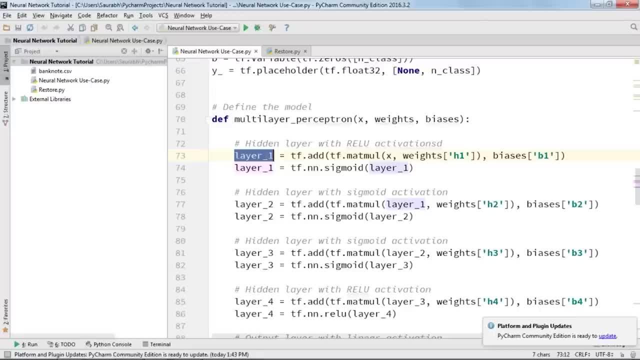 the first layer, So the first hidden layer, and then we are going to name it as layer underscore, one, which will be nothing but the matrix multiplication of x and weights of h1. that is the hidden layer one, and that'll be added to your biases b1.. 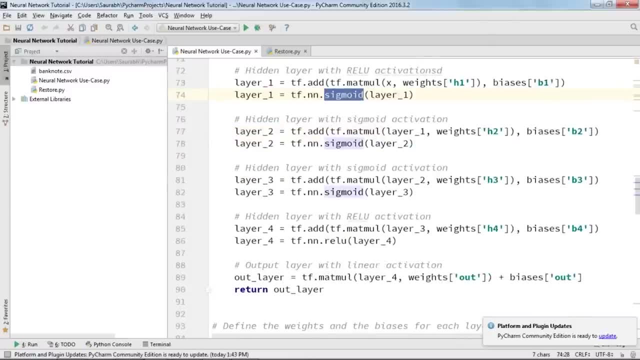 After that we'll pass it through a sigmoid activation function. Similarly in layer two as well: matrix multiplication of layer one and weights of h2.. So, if you can notice, layer one was the network layer just before the layer two, right? So the output. 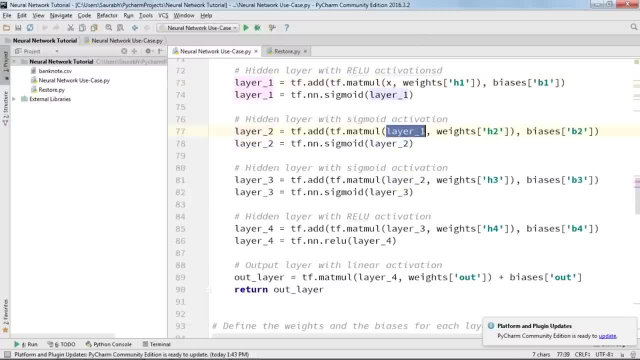 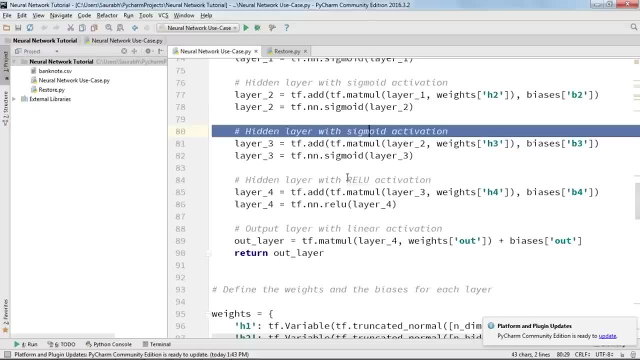 of this layer one will become input to the layer two, and that's why it's called hidden underscore one. It'll be multiplied by weights h2, and then we'll add it with the bias. Similarly for this particular hidden layer as well, and this particular layer. 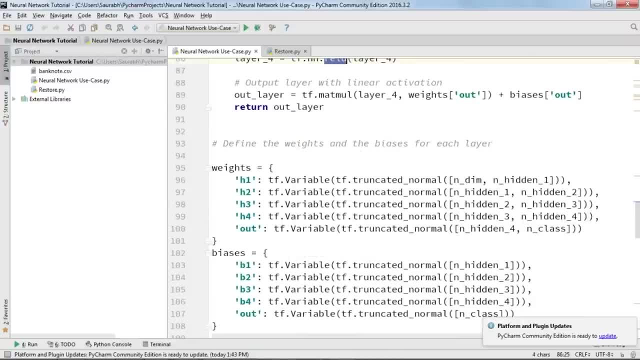 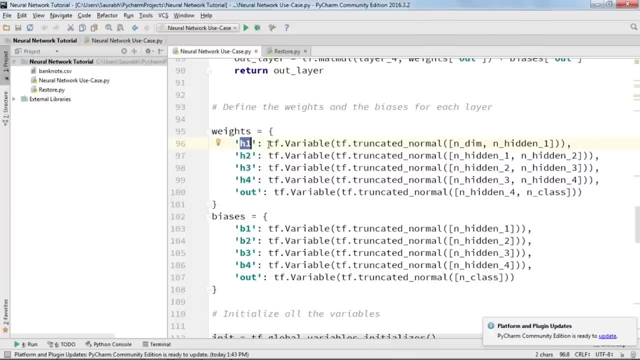 as well, But over here we are going to use the ReLU activation function instead of sigmoid. Then we are going to define the weights and biases. So this is how we basically define weights. This is how we basically define weights. So weights h1. 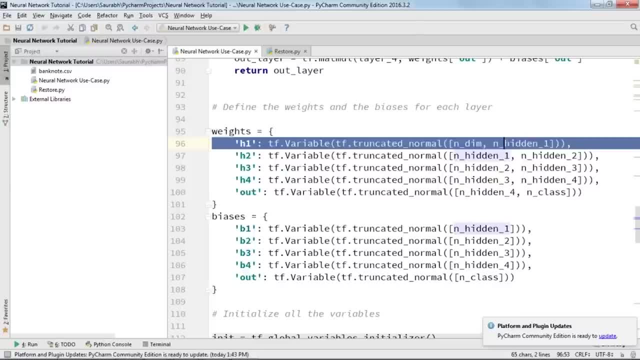 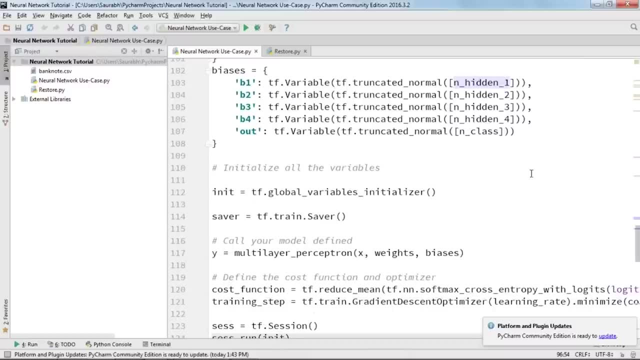 will be a variable which will be a truncated normal with the shape of n underscore dim and n underscore hidden underscore one. And after that, what we have done, we have defined biases as well. Then we need to initialize all the variables. So all these things. 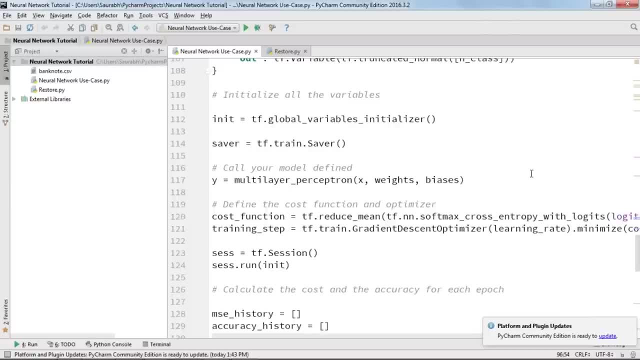 actually have discussed in brief when I was talking about TensorFlow, So you can go through TensorFlow tutorial at any point of time if you have any question. We have discussed everything there, Since in TensorFlow we need to initialize the variables before we use it. So that's how we do it. 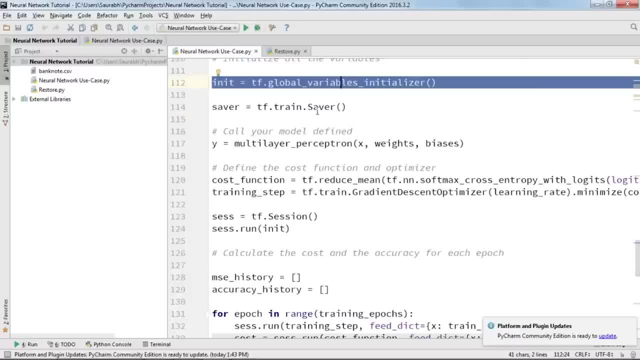 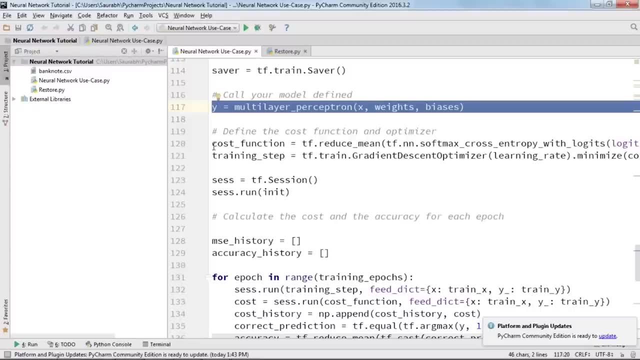 We first initialize it and then we need to run it. That's when your variables will be initialized. After that, we are going to create a saver object and then, finally, we are going to run the session. And then comes that part where the training happens. 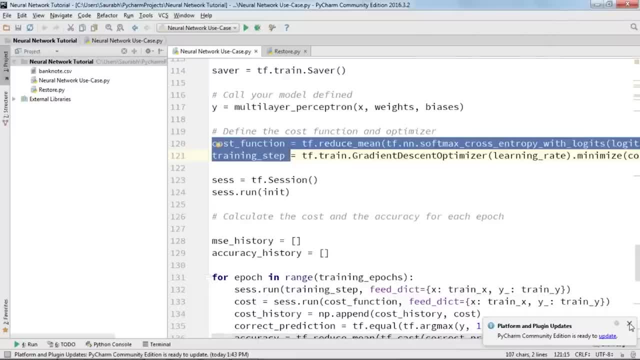 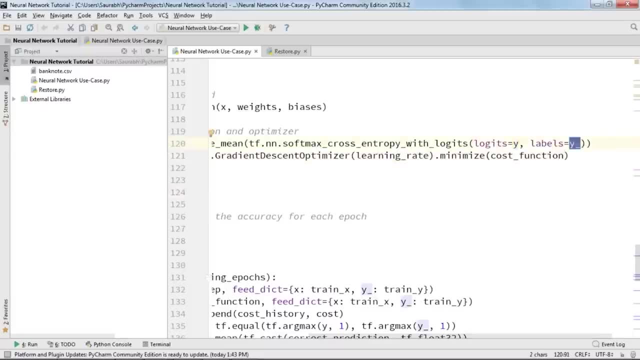 Cause function. Cause function is nothing, but you can say an error. that will be calculated between the actual output and the model output. All right, So y is nothing but our model output and y dash is nothing but actual output or the output that we already know. 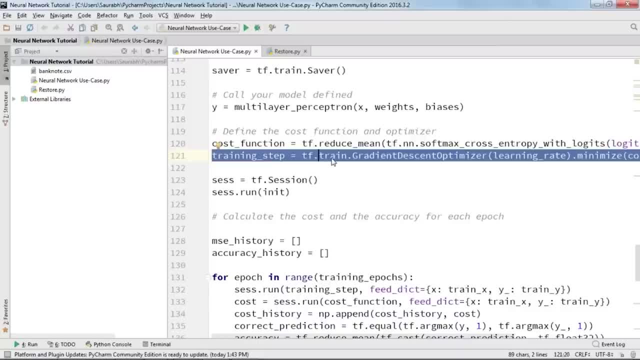 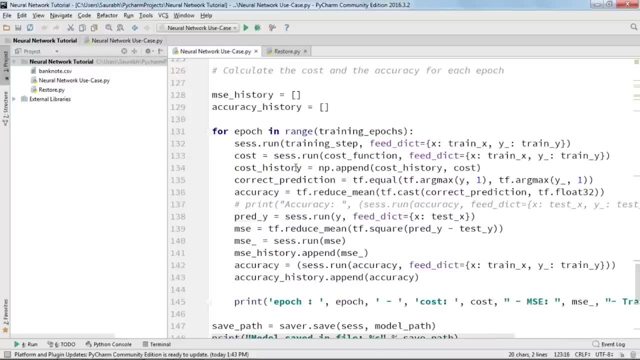 All right. And then we are going to use a gradient descent optimizer to reduce error, Then we are going to create a session object as well, And, finally, what we are going to do, we are going to run the session. So this is how, for every epoch. 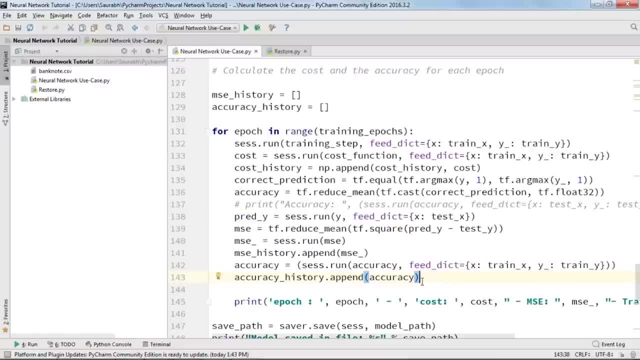 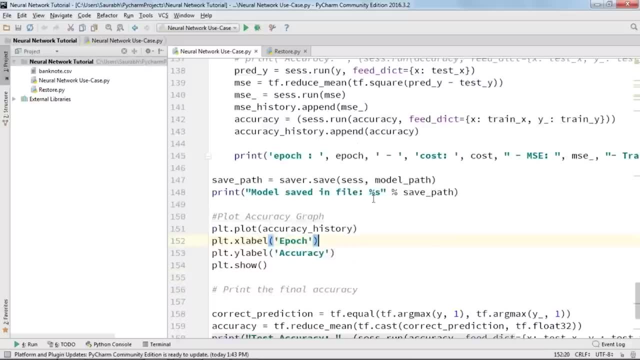 we will be calculating the change in the error as well as the accuracy that comes after every epoch on the training data. After we have calculated the accuracy on the training data, we are going to plot it for every epoch how the accuracy is And after plotting that. 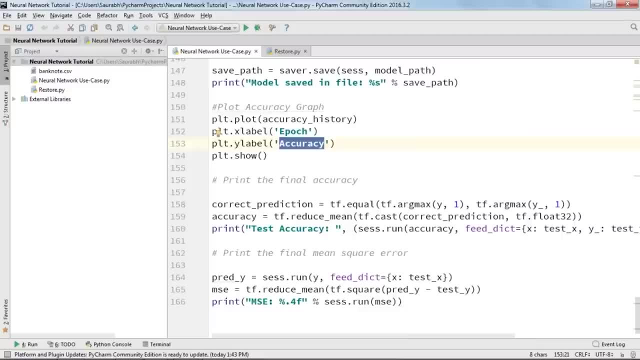 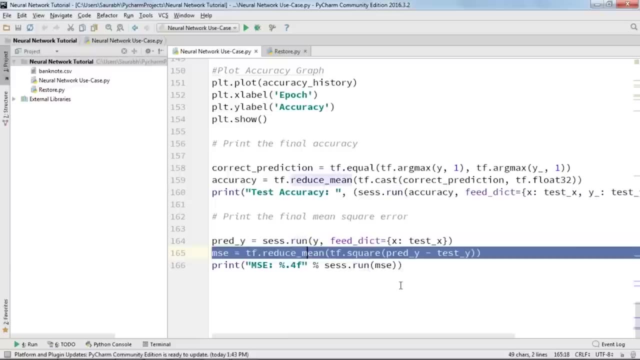 we are going to print the final accuracy, which will be on our test data. So using the same model will make prediction on the test data And after that we are going to print the final accuracy and the mean squared error. So let's go ahead. 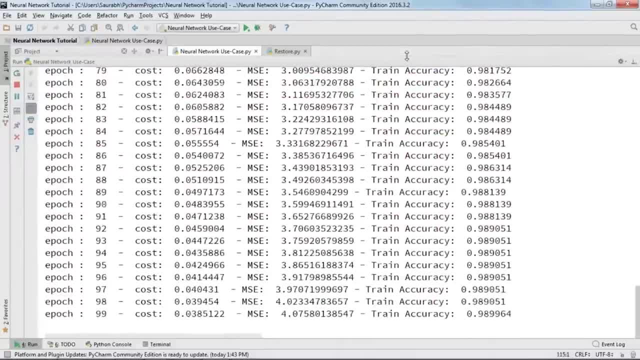 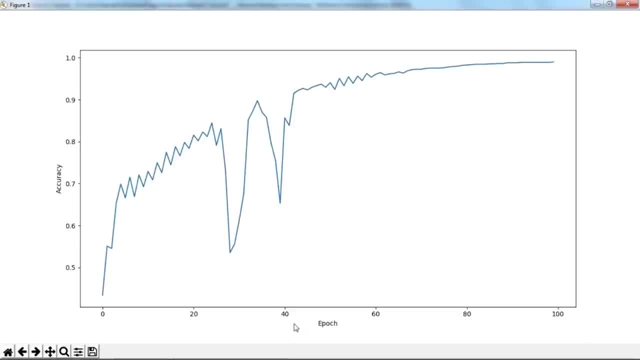 and execute this, guys. All right, the training is done and this is the graph we have got for accuracy versus epoch. This is accuracy. y-axis represents accuracy, whereas this is epochs. We have taken 100 epochs and our accuracy has reached somewhere around 99%. 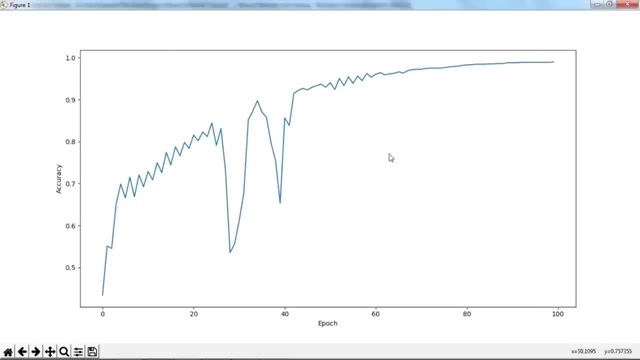 So with every epoch it is actually increasing. apart from a couple of instances It is actually keep on increasing. So the more data you train your model on, it will be more accurate. Let me just close it. So now the model has also been saved. 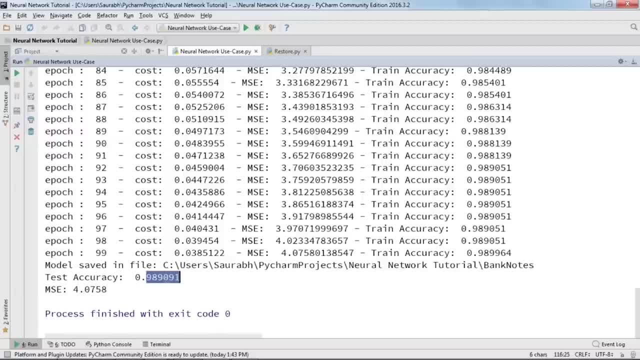 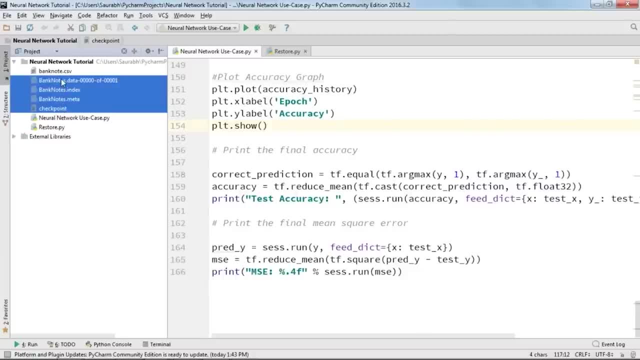 where I wanted it to be. This is my final change in test accuracy and this is the mean squared error. All right, So these are the files that will appear once you save your model. These are the four files that I've highlighted Now what we need to do. 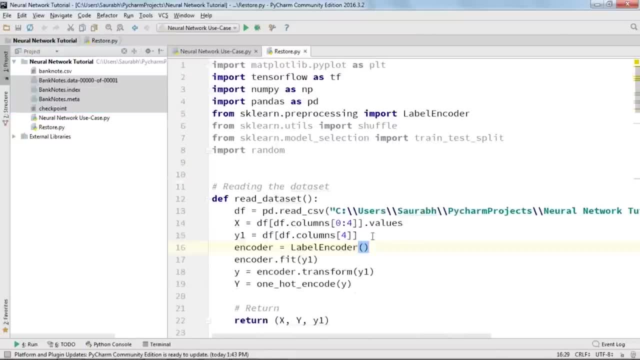 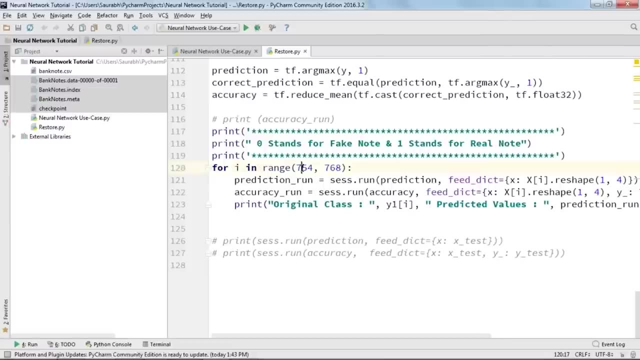 is restore this particular model, and I've explained this in detail: how to restore a model that you have already saved. So over here, what I'll do: I'll take some random range. I've taken it actually from 754 to 768.. So all the values. 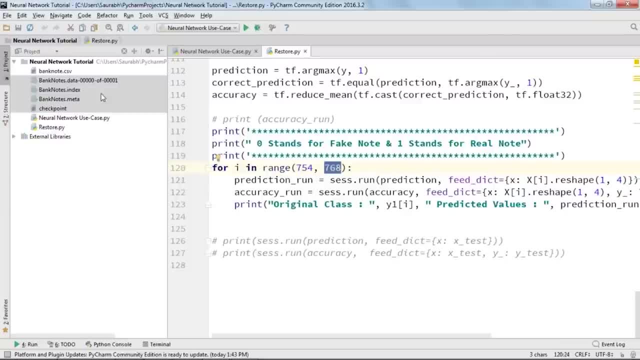 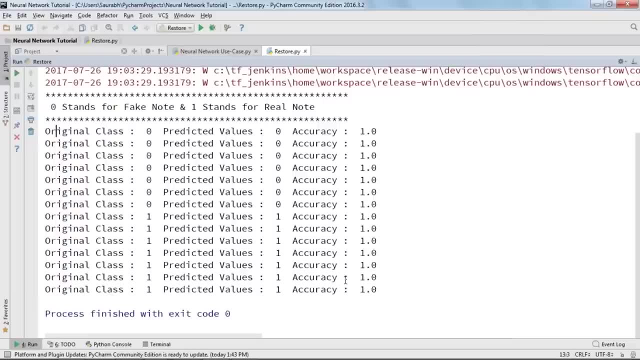 in the row of 754 and 768 will be fed to our model and our model will make prediction on that. So let us go ahead and run this. So when I'm restoring my model, it seems that my model is 100% accurate for the values. 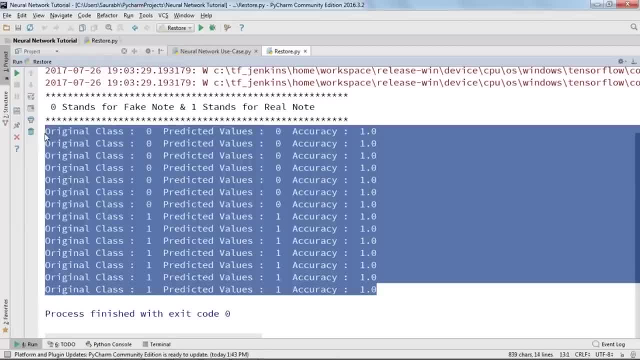 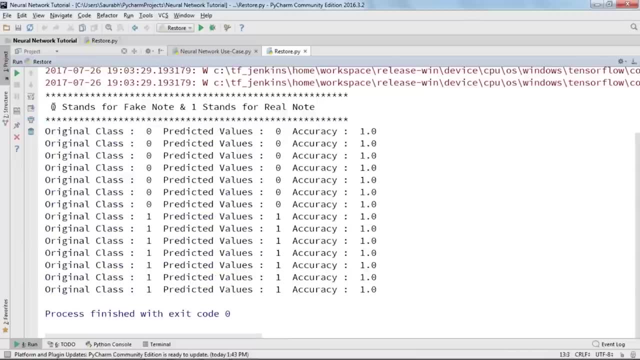 that I've fed in. So, whatever values that I have actually given as input to my model, it has correctly identified its class, whether it's a fake node or a real node, because 0 stands for fake node and 1 stands for real node. Okay, 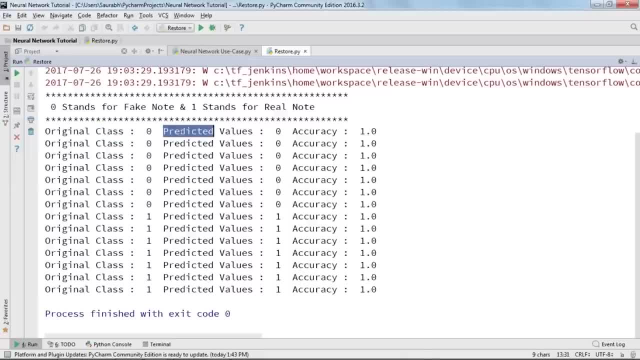 So original class is nothing but which is there in my data set. So it is 0 already, and what prediction my model has made is 0. That means it is fake, So accuracy becomes 100%. Similarly for other values as well. 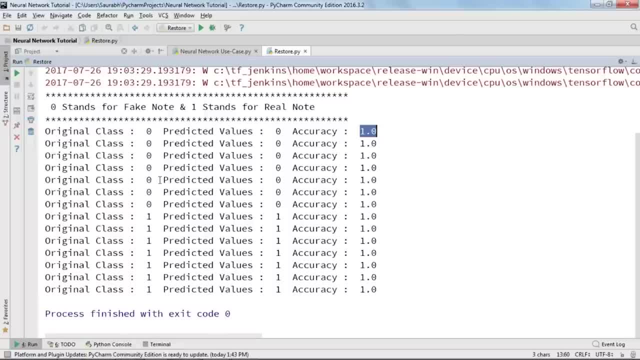 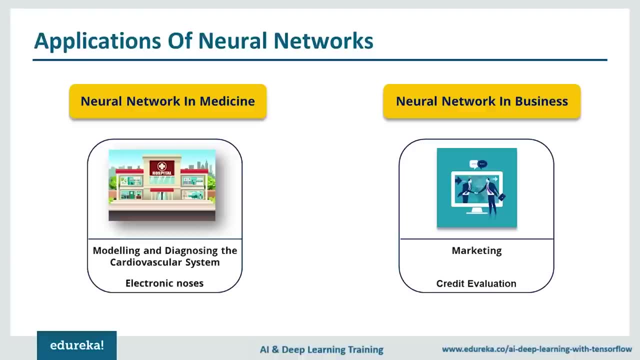 Fine guys, this is how we basically implement the use case that we saw in the beginning, So I'll quickly discuss few applications of neural networks. So in the slide you can notice that I've listed down only two applications, although there are many more. 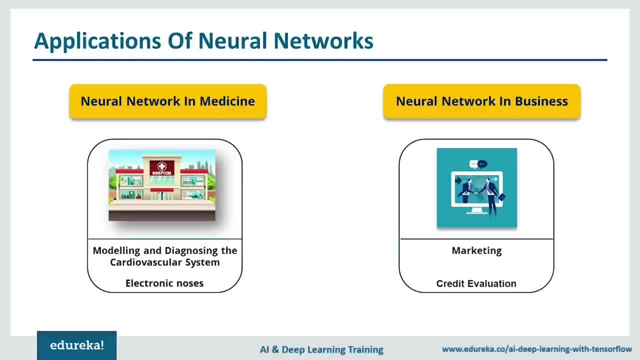 So neural networks in medicine. Artificial neural networks are currently a very hot research area in medicine and it is believed that they will receive extensive application to biomedical systems in the next few years. And currently the research is mostly on modeling parts of human body And recognizing diseases. 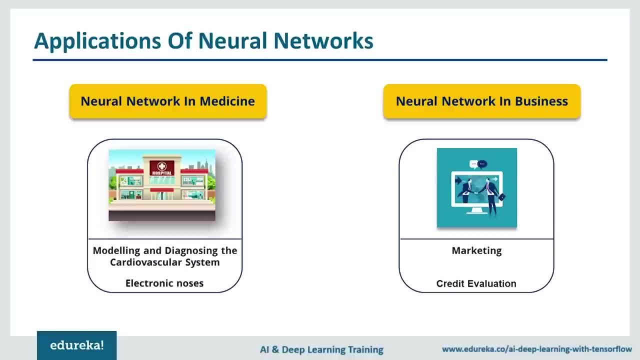 from various scans. For example, it can be cardiograms, CAT scans, ultrasonic scans, etc. And currently the research is going mostly on two major areas. First is modeling and diagnosing the cardiovascular system, So neural networks are used experimentally. 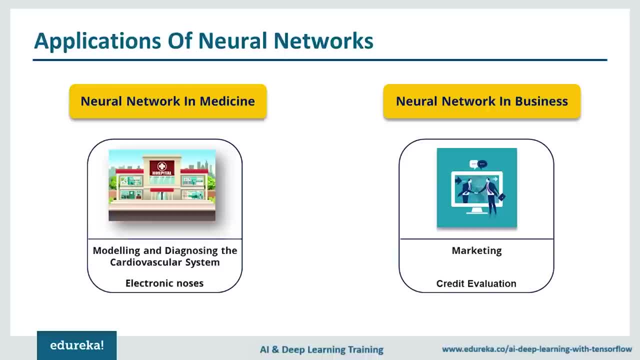 to model the human cardiovascular system. Diagnosis can be achieved by building a model of the cardiovascular system of an individual and comparing it with the real time physiological measurements taken from the patient. And, trust me guys, if this routine is carried out regularly, potential harmful. 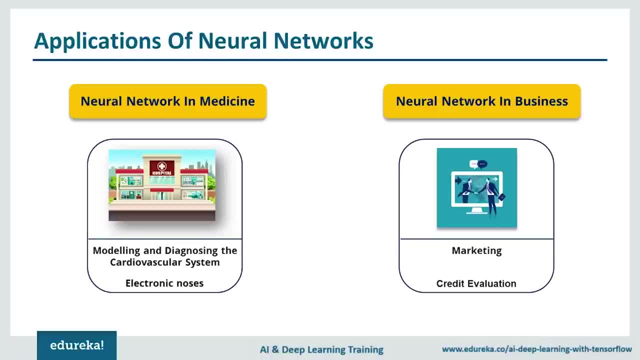 medical conditions can be detected at an early stage And thus make the process of combating disease much easier. Apart from that, it is currently being used in electronic noses as well. Electronic noses have several potential applications in telemedicine. Now let me just give you. 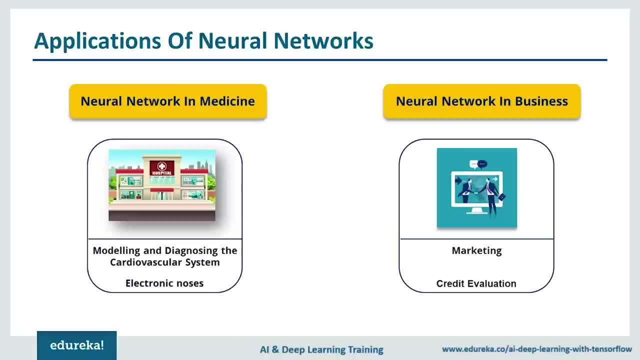 an introduction to telemedicine. Telemedicine is a practice of medicine over long distance via a communication link. So what the electronic noses will do? they would identify odors in the remote surgical environment. These identified odors would then be electronically transmitted to another site. 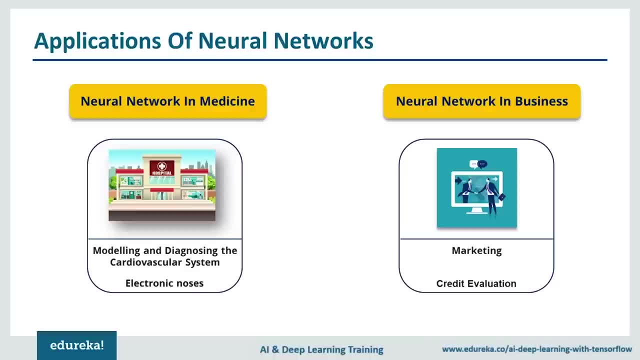 where an door generation system would recreate them, Because the sense of the smell can be an important sense to the surgeon. telesmell would enhance telepresent surgery. So these are the two ways in which you can use it. in medicine You can use it. 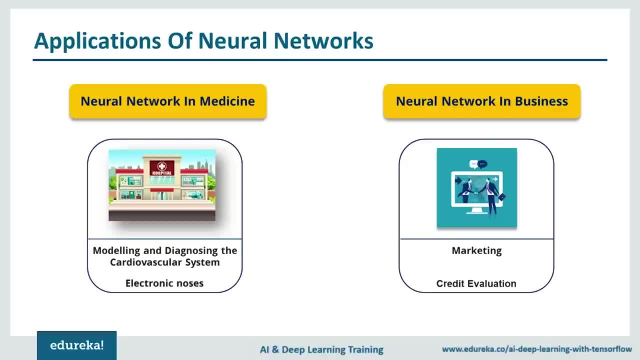 in business as well, guys. So business is basically a diverted field with several general areas of specialization, such as accounting or financial analysis. Almost any neural network application would fit into one business area, or financial analysis. Now there is some potential for using neural networks for business purposes. 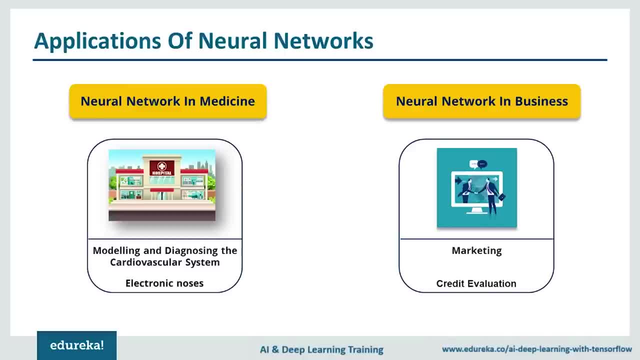 including resource allocation and scheduling. I have listed down two major areas where it can be used. One is marketing. So there is a marketing application which has been integrated with a neural network system. The airline marketing tactician is a computer system made of various 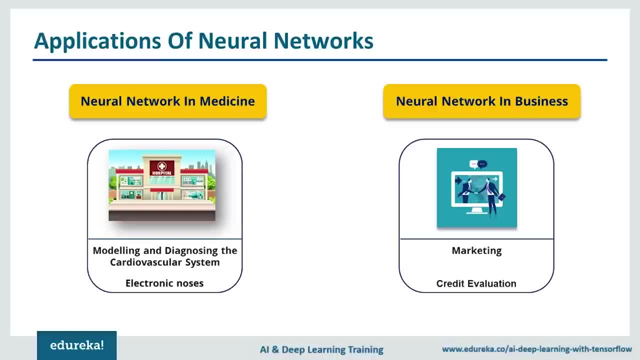 intelligent technologies, including expert systems. A feed forward neural network is integrated with the neural network system. The airline marketing tactician is integrated with the AMT, which is nothing but airline marketing tactician and was trained using back propagation to assist the marketing control of airline seat. 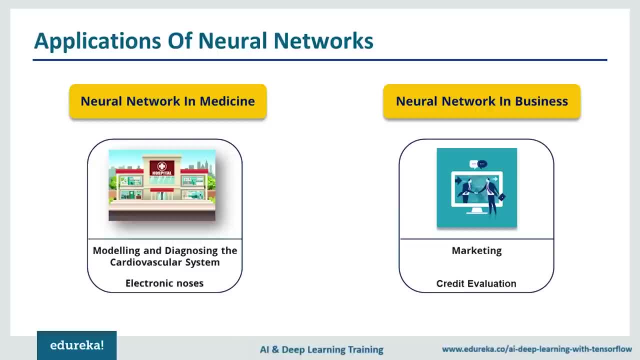 or location. So it has wide applications and marketing as well. Now the second area is credit evaluation. Now I'll give you an example here. The HNC company has developed several neural network applications, and one of them is a credit scoring system which increases. 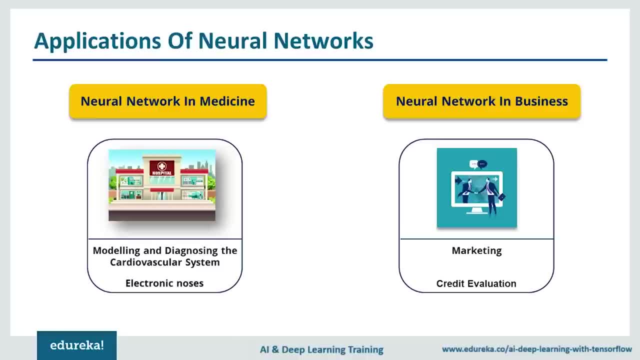 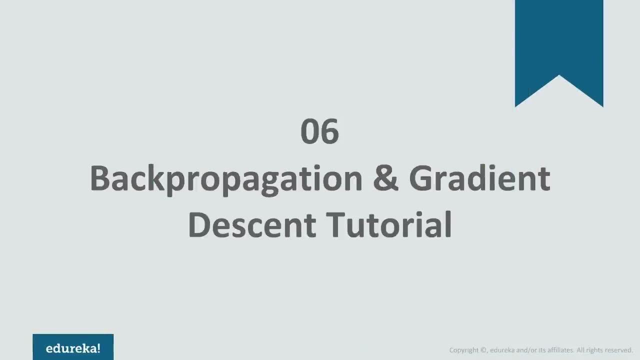 the profitability of existing model. you guys, neural network is actually the future. People are talking about neural networks everywhere, and especially after the introduction of GPUs and the amount of data that we have now. neural network is actually spreading like play right now In this video. 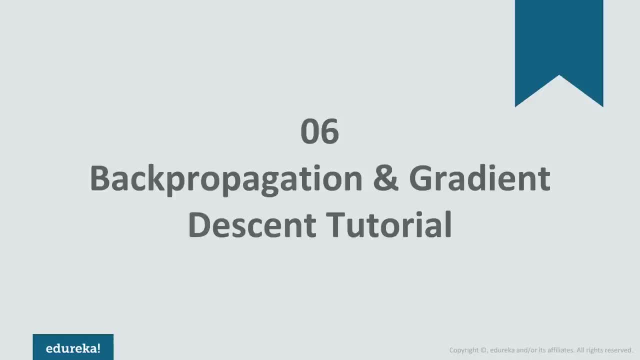 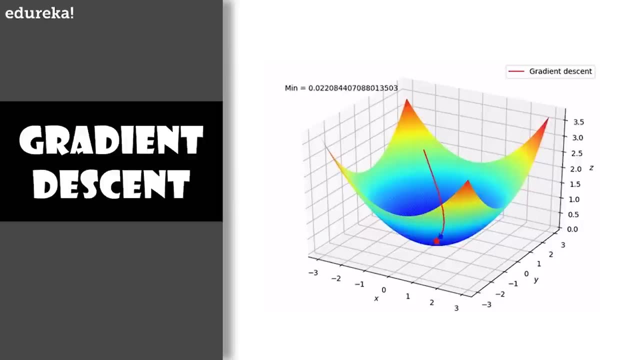 I'll introduce you the idea of gradient descent, which underlies not only how neural network works and learn, but how a lot of other machine learning works as well and what those hidden layers of neurons end up actually looking for. So just to remind you guys that our goal 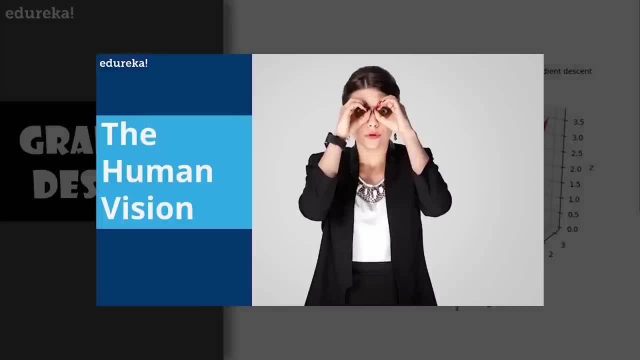 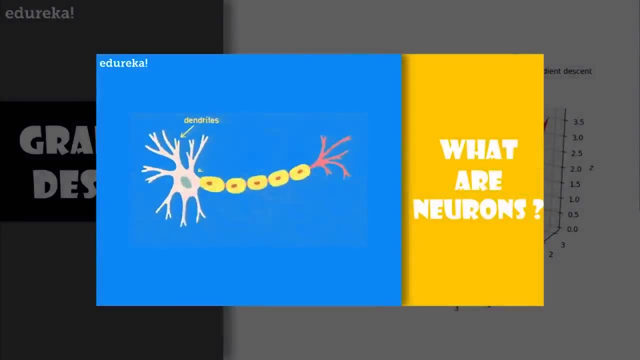 here is the recognition of the handwritten digits, and these digits are rendered on a 28 by 28 pixel grid, Each pixel with some grayscale value between 0 and 1.. Those are what determine the activations of the 784 neurons in the input layer. 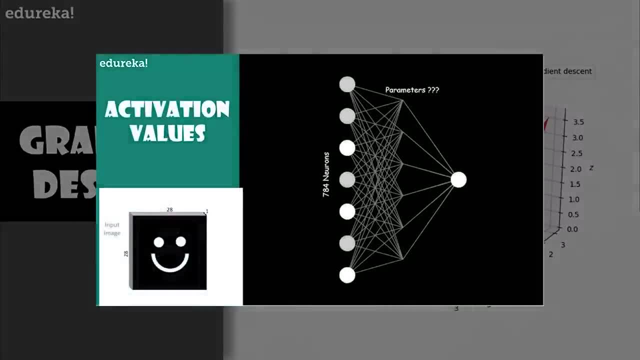 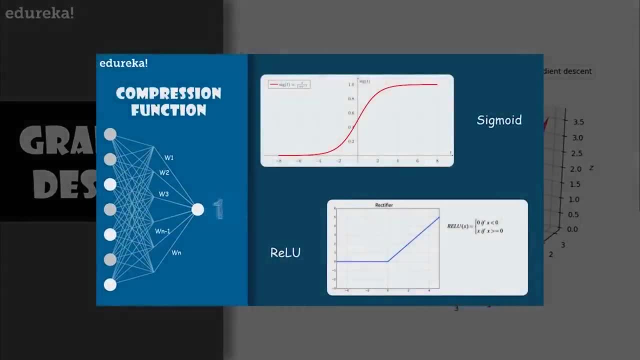 and these activation for each neuron is in the following layers: is based on a weighted sum of the activations in the previous layer with a special number called the bias. Then you compute that sum with some other function like the sigmoid or a ReLU function. and we also discussed 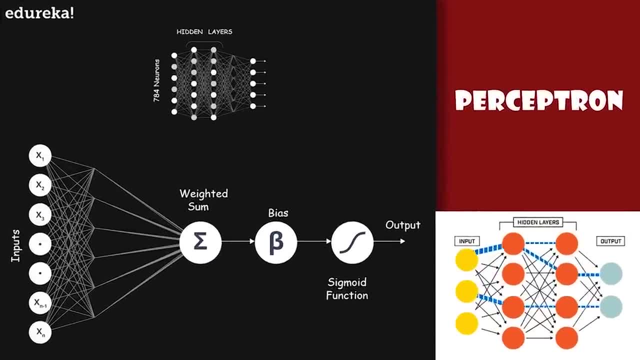 how a perceptron works and behaves like a function. Obviously, the perceptron isn't a complete model of human decision making, but what the example illustrates is how a perceptron can weigh up different kinds of evidence in order to make decisions, and it should seem plausible. 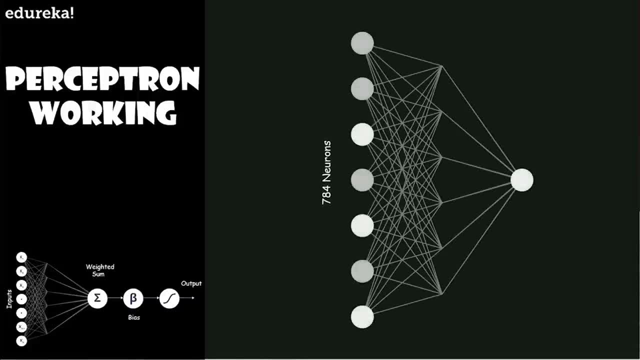 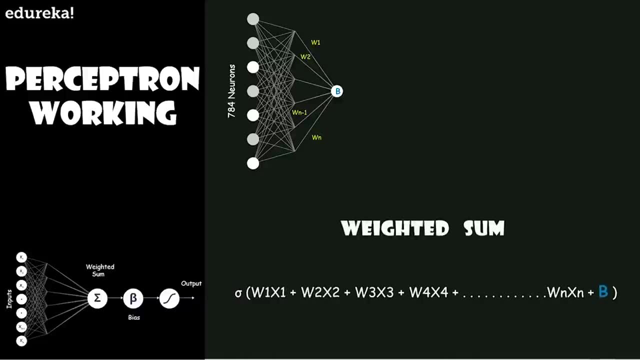 that a complex network of perceptron could make quite subtle decisions In this network. the first column is made by weighing the input evidence. What about the perceptrons in the second layer? Each of those perceptron is making a decision by weighing up. 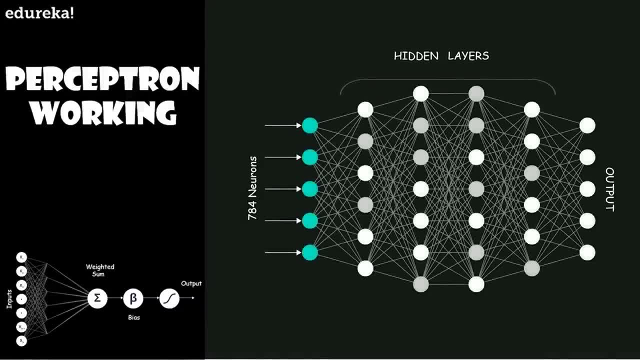 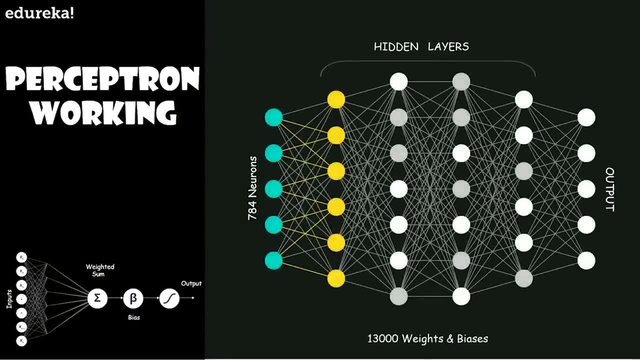 the results from the first layer of the decision making. In this way, a perceptron in the second layer can make a decision at a more complex and more abstract level than the perceptron in the first layer. In total, given that somewhat arbitrary choice, 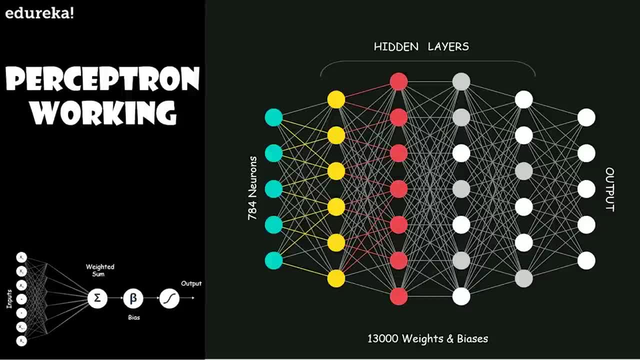 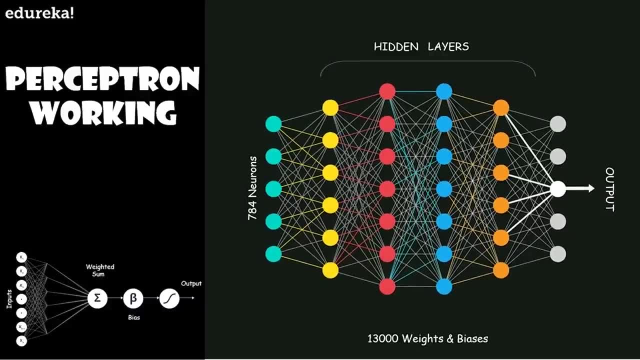 of the two hidden layers. with 16 neurons, the network has about 13,000 weights and biases that we can adjust based on the network you know actually does. So here we are going to learn how the network learns. What we want is an algorithm. 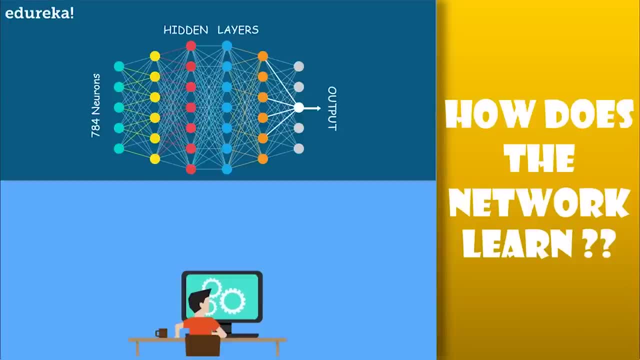 where you can show this network a series of training data which comes in the form of different images of handwritten digits along with labels for what they are supposed to be, and it will adjust those 13,000 weights and biases so as to improve its performance on the training data. 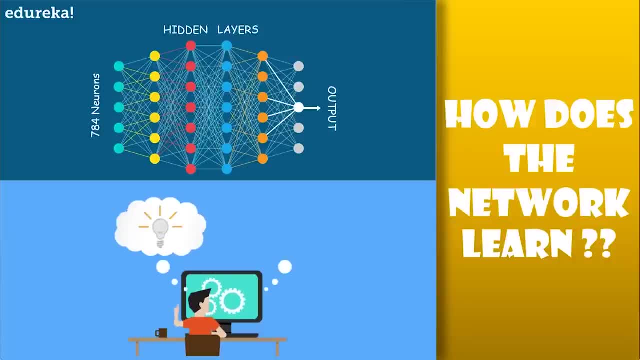 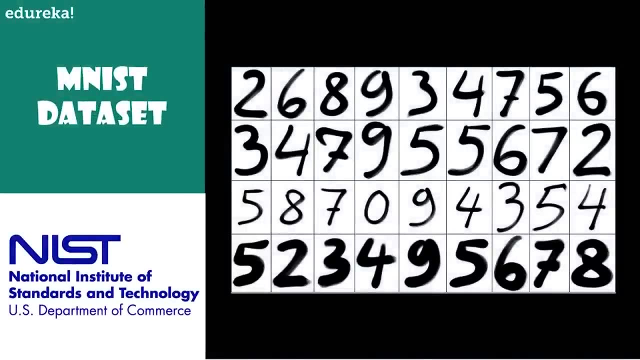 Hopefully, this layer structure will mean that what it learns generalizes to images beyond that of the training data that we are going to use. We will use the MNIST dataset here, which contains tens of thousands of scanned images of handwritten digits, together with their correct classification. 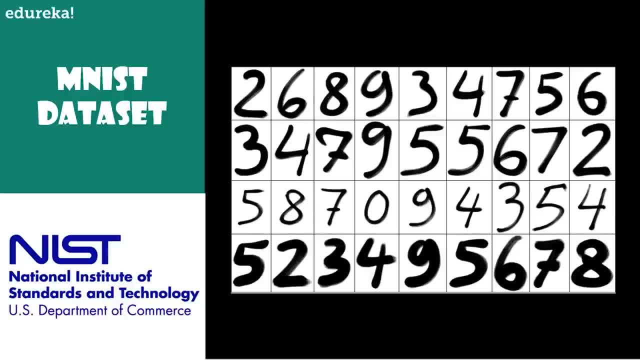 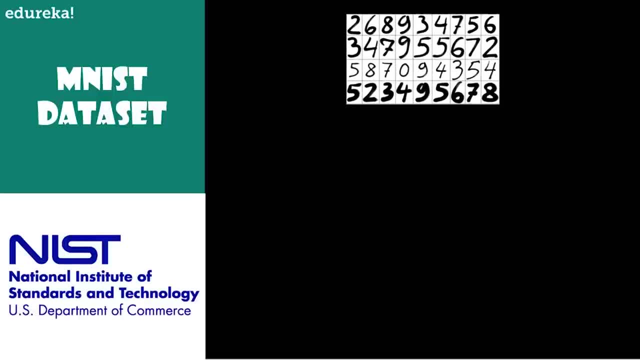 The MNIST names comes from the fact that it is a modified subset of two datasets collected by NIST, which is the United States National Institute of Standards and Technology. The data comes in two parts. The first part contains 60,000 images to be used. 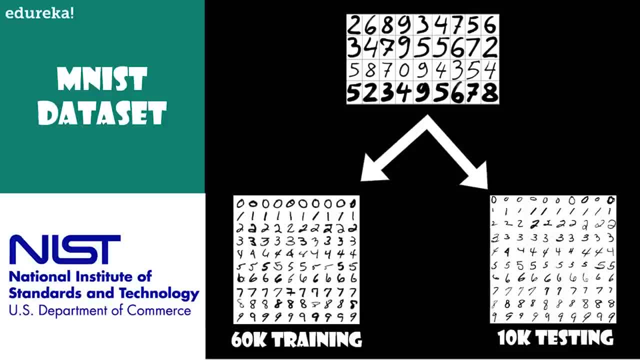 as training data. These images are scanned, handwritten samples from 250 years ago. The MNIST dataset is 10,000 images to be used as the test data. Again, these are 28x28 grayscale images. What we would like is an algorithm. 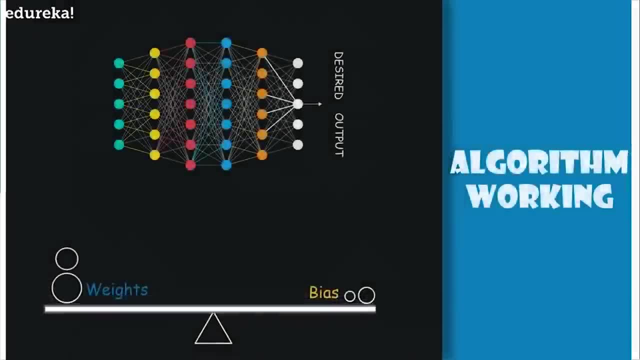 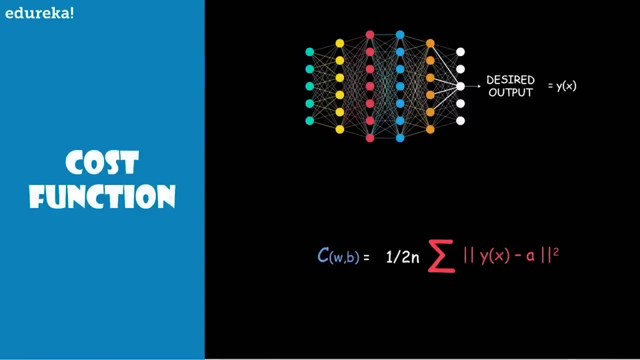 which lets us find weights and biases so that the output from the network approximates to the desired output of all the training inputs. Now, to quantify how we will be achieving this goal, we define here a cost function, which is sometimes referred to as a loss. 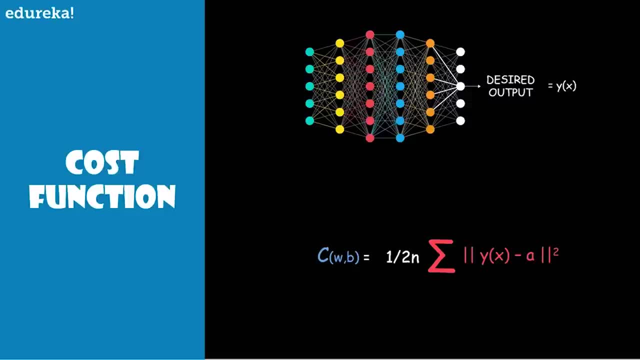 or an objective function. B denotes all the biases and is the total number of training inputs. For us it is 60K and A is the vector of outputs from the network when X is the input and the sum is over all the training inputs. 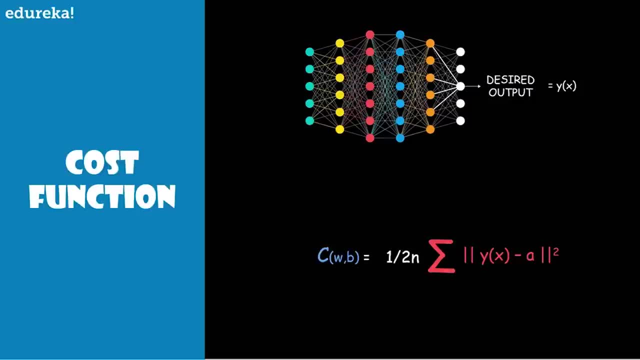 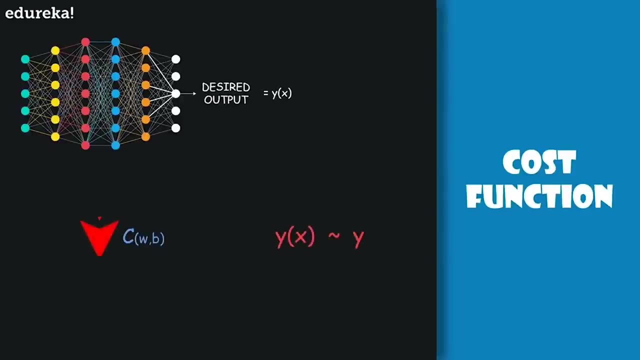 which is the X. Of course, the output depends on the values of X, W and B, which are the inputs, weights and biases. Now the cost becomes small. that is the output for all the training inputs: X. So 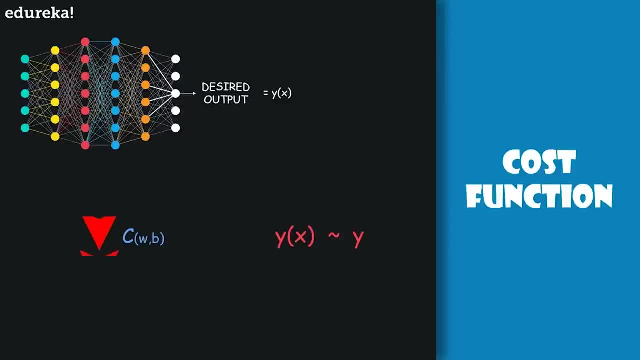 our training algorithm has done a good job if it can find the weights and biases so that the cost is equal to 0. By contrast, it's not doing so well when we say that the cost is large. So the aim of our training algorithm 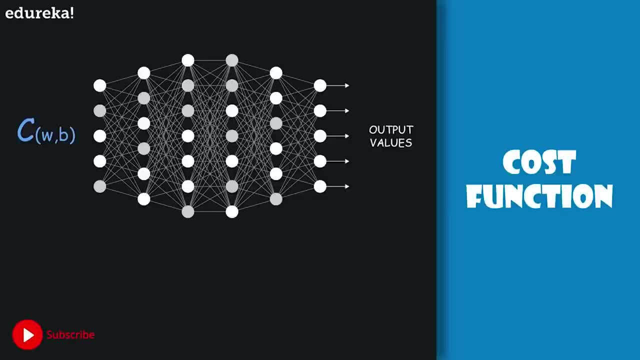 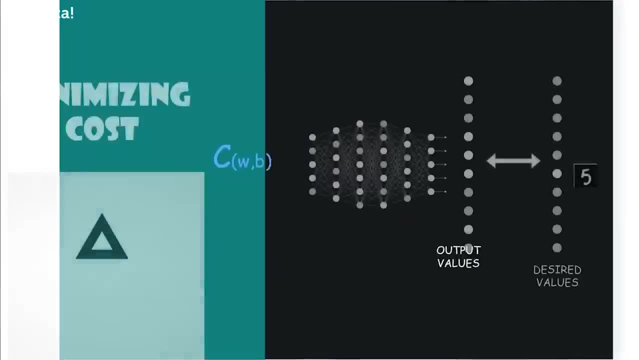 will be to minimize the cost as a function of the weights and biases, and in other words, we want to find a set of weights and biases as the gradient descent. We are just going to initialize all those weights and bias totally randomly. What we do is: 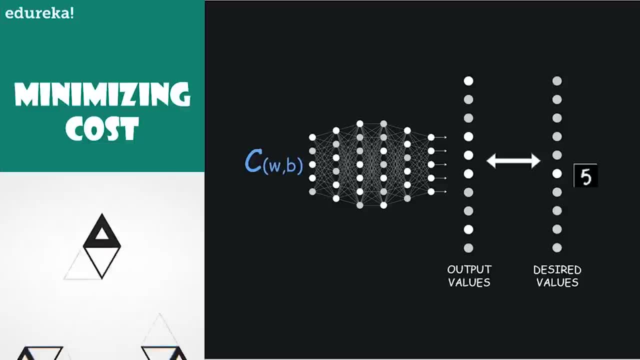 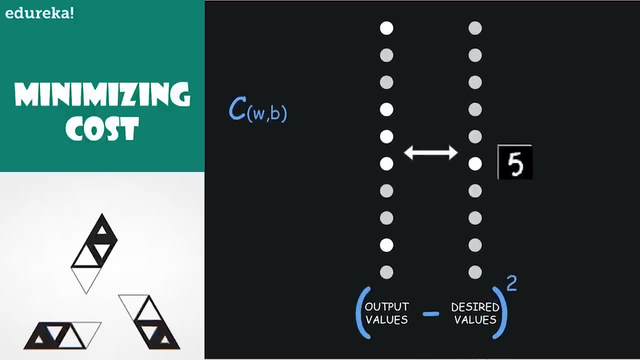 we define a cost function as a way of telling the computer what is good and what is bad. To do this, we need to add up the squares of the differences between each of the given outputs, which are the given activations, and the value you want them to have. 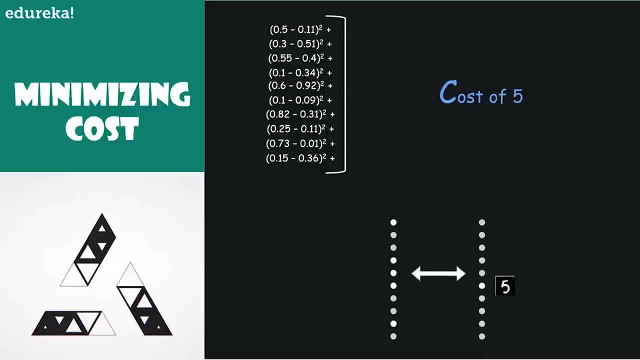 and this is what we call the cost of a single training example. This sum is small when the network and the training algorithm will be to minimize the cost as a function of weights and biases. so then, what we do is consider the average cost of all these tens. 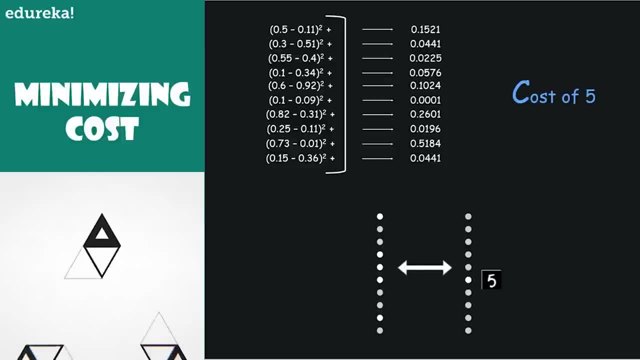 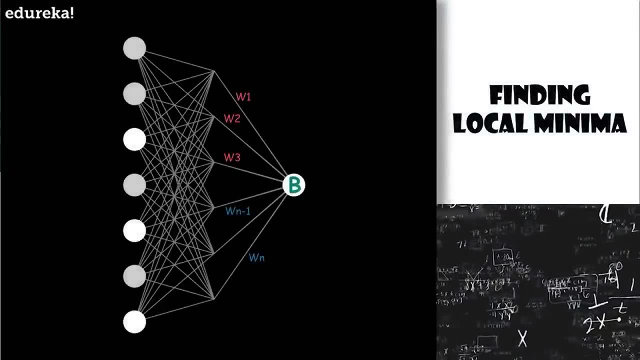 and thousands of training examples. The way it's defined depends upon the network's behavior over all the tens of thousands of the pieces of the training data. That's a lot to think about. How do you find an input that minimizes the value of this function? 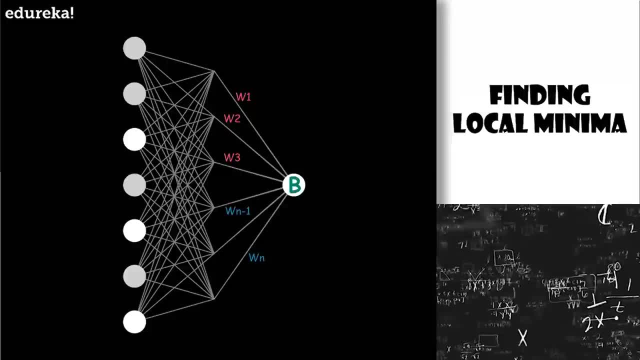 For the most part, making changes makes it difficult to figure out how to change the weights and biases to get improved performance. If we instead use a smooth cost function like the quadratic cost, it turns out to be easy to figure out how to make small changes. 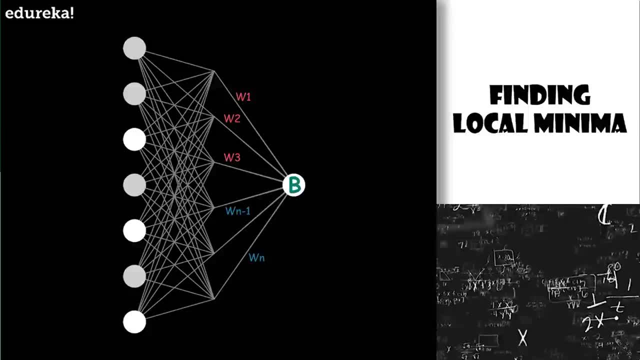 in weights and biases so as to get an improvement in the cost. So for now, we are going to imagine that we have been simply given a function of many variables and what we want is to minimize that function. Those of you from the calculus background will be able. 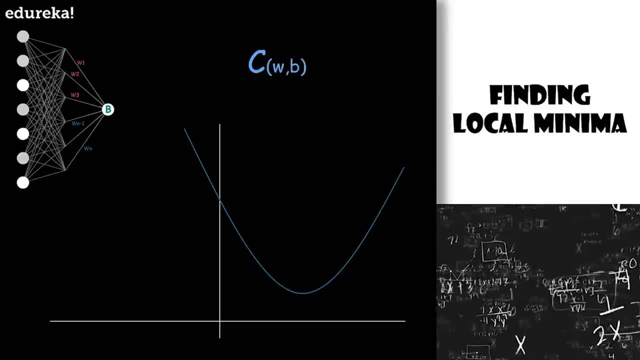 to understand that minimum explicitly. A more flexible tactics is to start from any old input and figure out in which direction you should step out to make the output low. Specifically, if you can figure out the slope of a function, where you are, then if you are. 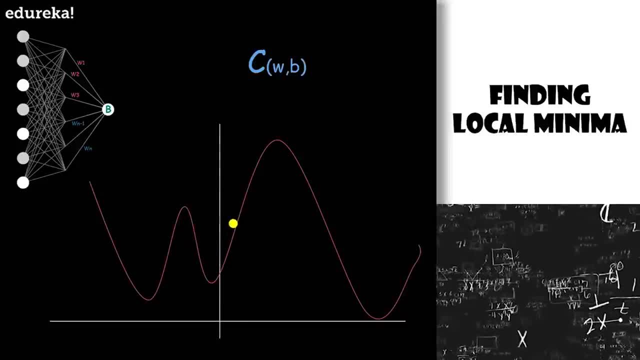 shifting towards left, then the slope is positive, and if you are shifting towards right, the slope can be negative. it will be the reverse. So if we do this repeatedly, at each point checking the next slope, that's not always feasible for really complicated functions- Now, really complicated. 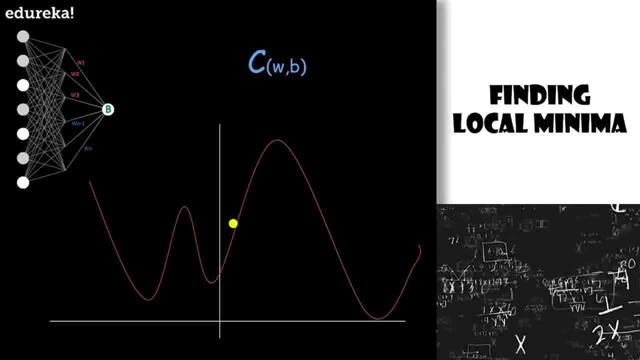 functions can have a lot of minimas. There is a beautiful analogy which suggests an algorithm which works pretty well. We start by thinking of our function as a kind of a valley. What we do is we imagine a ball rolling down the slope of the valley. 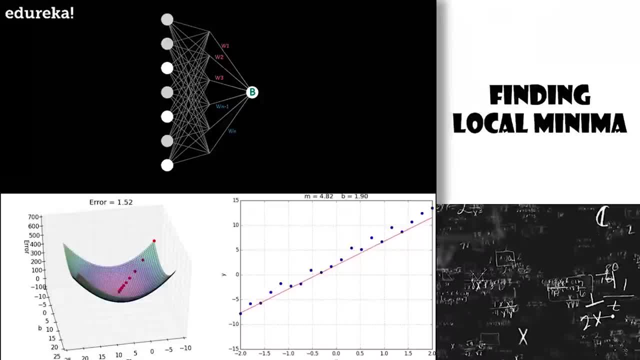 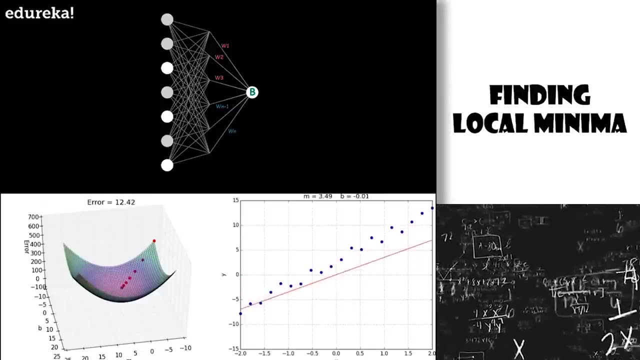 and our everyday experience tells us that the ball will eventually roll to the bottom of the valley. Perhaps we can use this idea as a way to find out where the ball is. Similarly, with multi-variable calculus, we'll know that the gradient of a function gives you the 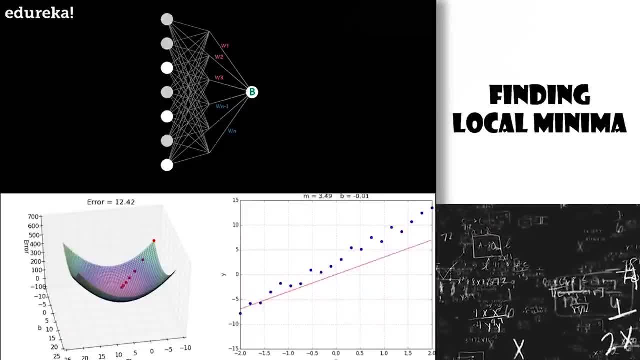 direction of the steepest axis. Basically, which direction should you step to increase the function most quickly? naturally enough, taking the negative of that gradient gives you the direction to step. that decreases the function by some. multiple of the negative gradient is known as the gradient descent. 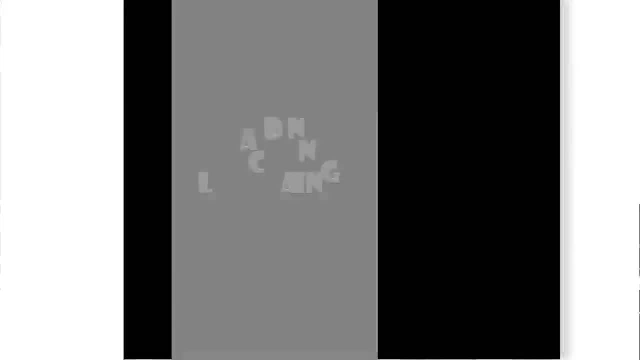 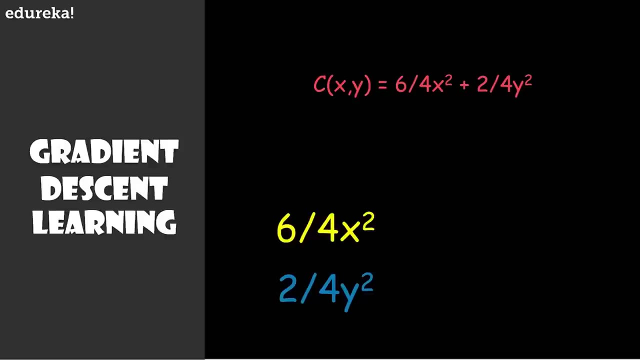 You'll see in our network an adjustment to one of the weights might have a much greater impact on the cost function than the adjustment to other weights. So if we take a particular cost function, suppose 6 by 4 x squared plus 2 by 4- 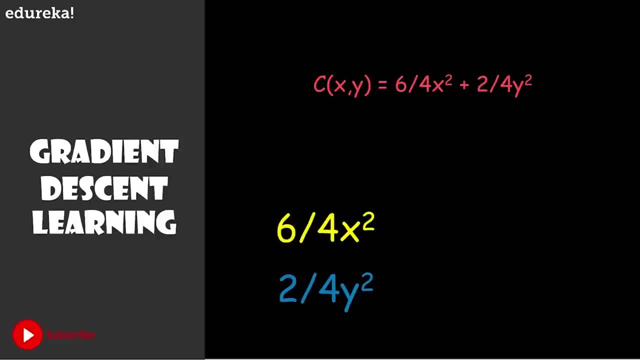 y squared. So this is just a simple example. Now what we do is compute its gradient at some particular point. The first variable, which is 6 by 4 x squared, has three times the importance as it changes to the second variable, The gradient. 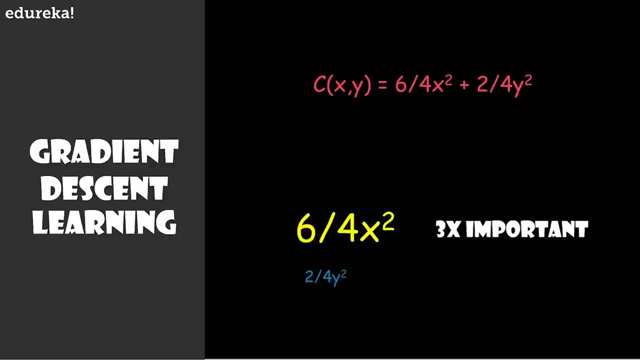 of the cost function is one more layer of complexity that still tells us what nudges to all these weights and biases cause the fastest change to the value of the cost function. So when you initialize the network with random weights and biases and adjust it to the 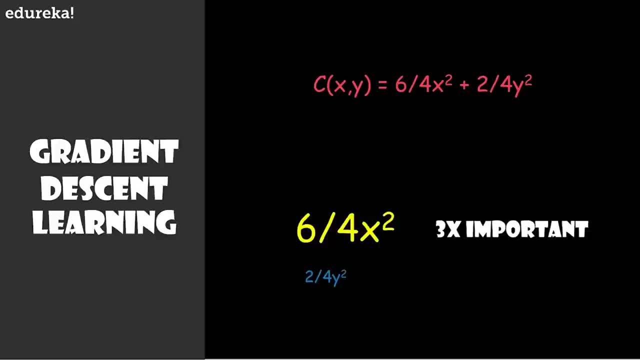 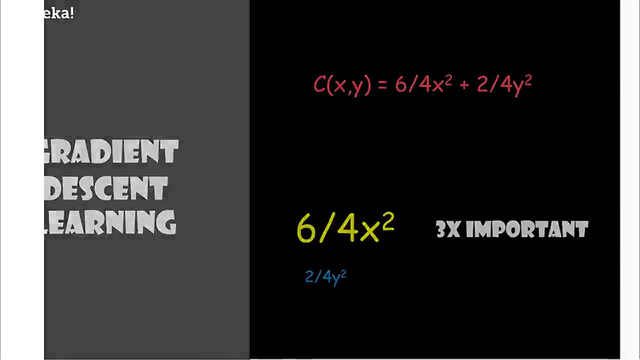 value of the cost function, you can get the accuracy up Now. I just think there's something incredible about any network doing this well on images that it's never seen before, given that we never specifically told it what patterns to look for. Now here we tackle back. 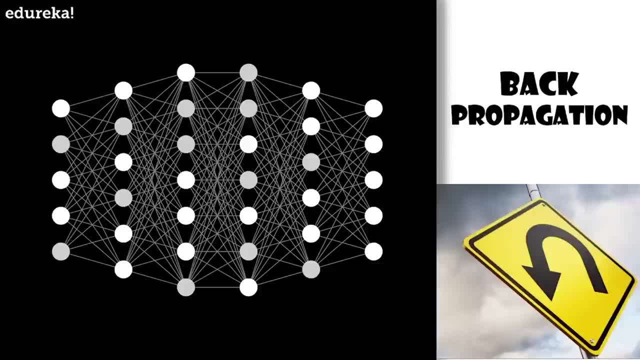 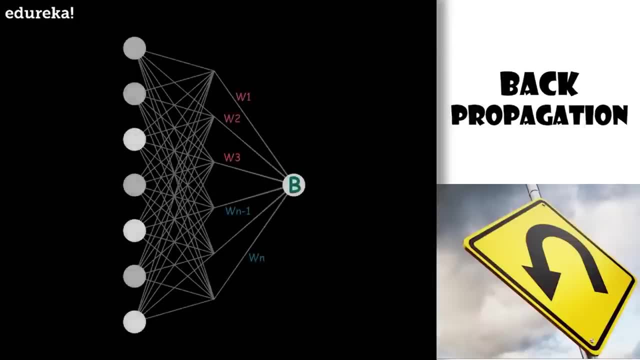 propagation, which is the core algorithm behind how a neural network learns. Now, what is a neural network? basically, it's an algorithm for computing the complicated gradient. The magnitude of each component here is telling us how sensitive the cost function is to the weights and bias. 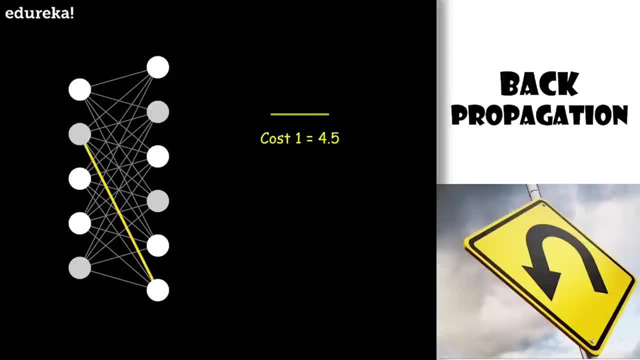 Now, let's say you compute a negative gradient and the component associated with the weight on this edge here comes out to be 4.5, while the component associated with the other edge comes out to be 0.1.. The way you will do changes. 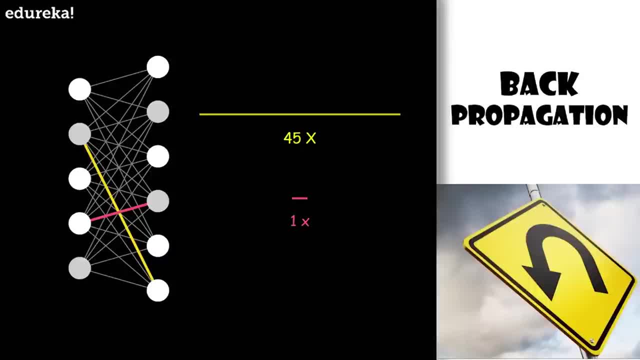 in that of the first weight. so if you do a change in the first connection that would have an effect on the cost which is 45 times the change you made on the second connection. The cost involves arranging a certain cost, for example over all the tens and thousands. 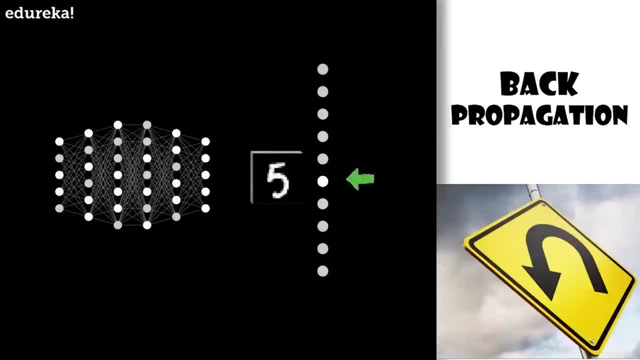 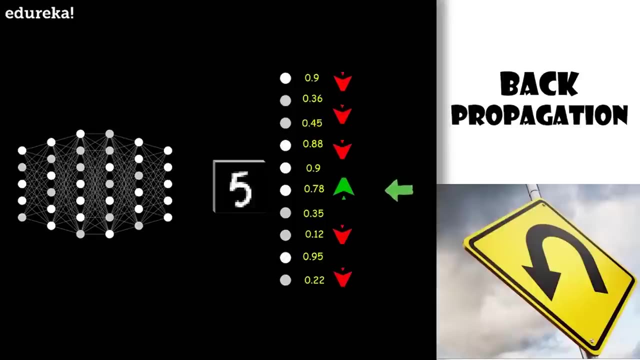 of training examples. For now we're going to focus our attention on one single example. So let's take an example of the digit network, which is not well trained, so the activations in the output are going to be pretty random. Now we can't directly change. 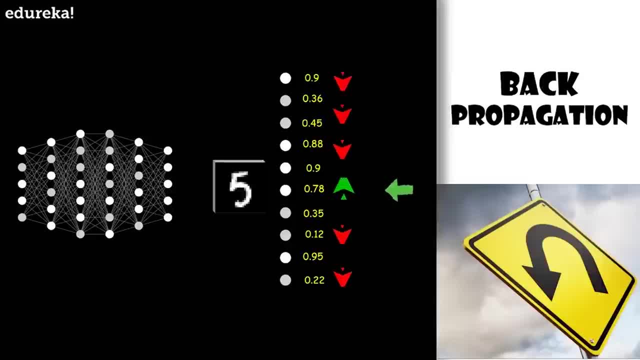 those activations. we only have the influence on the weights and biases, but it is helpful to keep a track of which adjustment we wish should take place to that output layer. and since we want it to classify the image as a 5, we want the sixth value to get nudged. 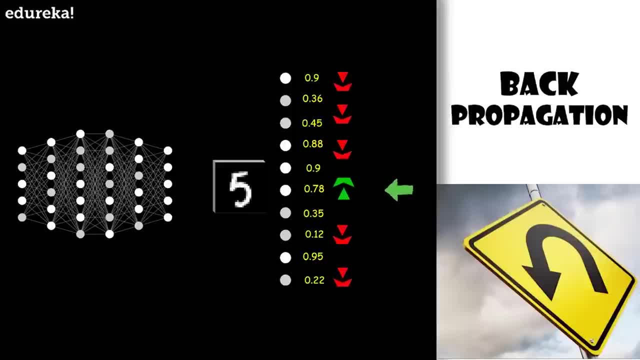 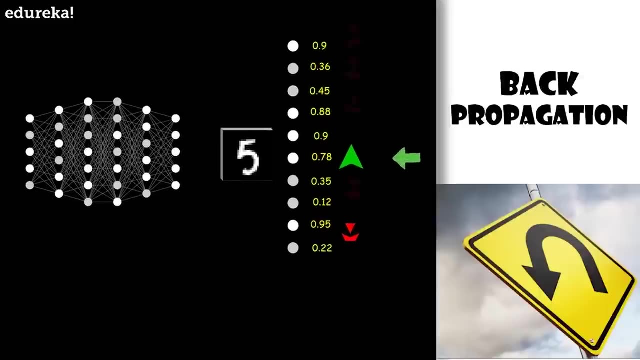 up while all the activations are active. For example, the increase to that number 5 neuron activation is in a sense more important than the decrease to the number 7 neuron, which is already pretty close to the zero mark. So there are three different parameters that can team. 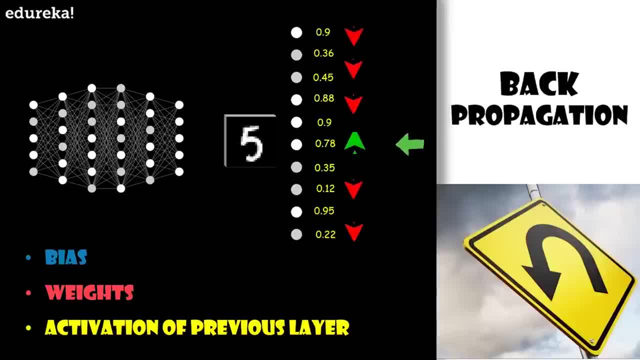 up together to help increase the activation. You can increase the bias, you can increase the weights and you can change the activation. as with the last layer, it is helpful to keep a note of what those desired changes are. Now, these changes are being made only for the digit. 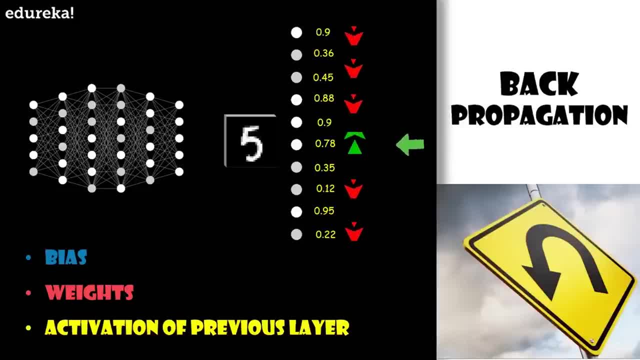 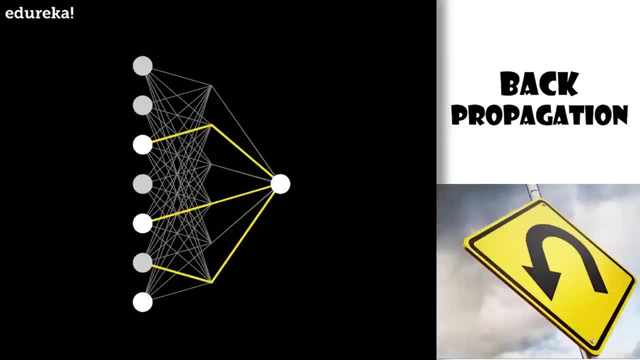 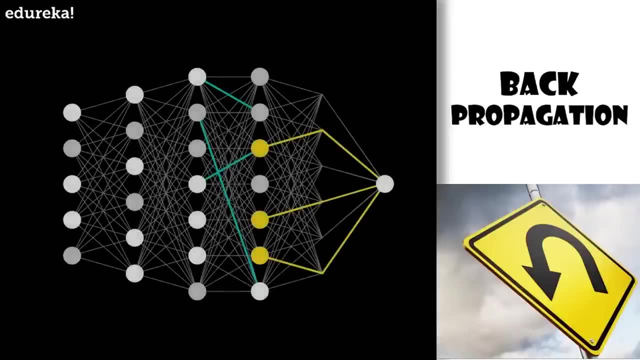 5. We also want all the other neurons in the last layer to become less active, and each of those other output neurons has its own thoughts about what should happen to the second to last layer. So the desire of this digit 5 neuron is added together. 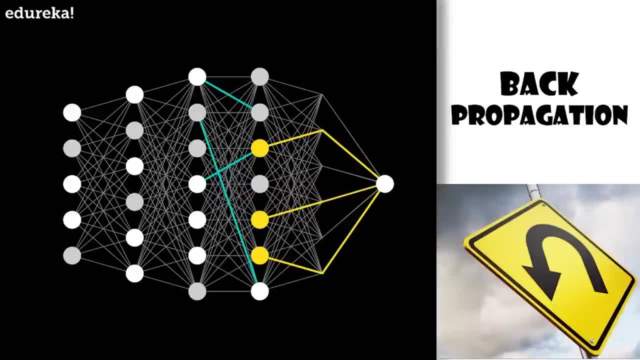 with the desires of all the other neurons, Again in proportion to the corresponding weights and in proportion to how much each of those neurons needs to change This right here is where the idea of propagating backwards comes in. Now, once you have the idea of all the nudges, 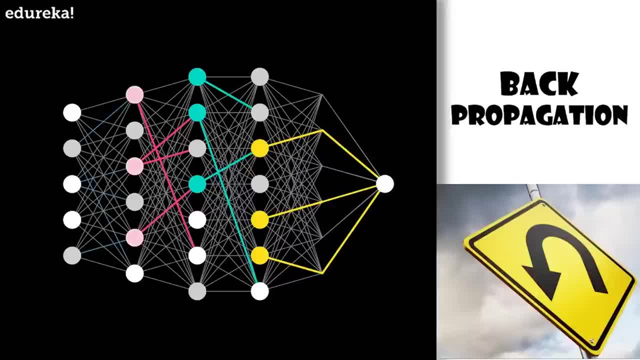 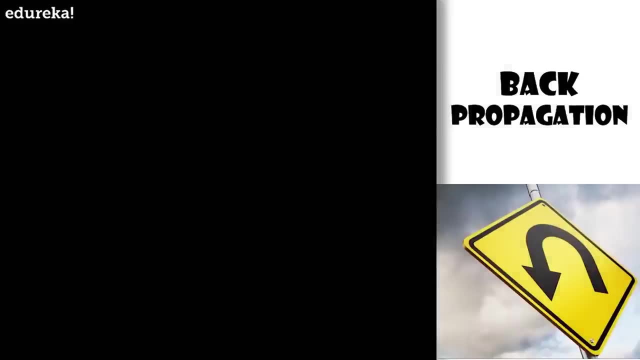 you want to make to the second to last layer, you can recursively apply the same process to the relevant weights and biases that determine those values, repeating the same process through and changing the weights and biases. This network can only classify a 5 as it is changing. 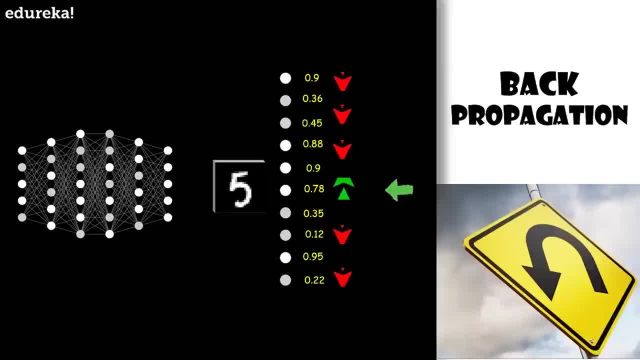 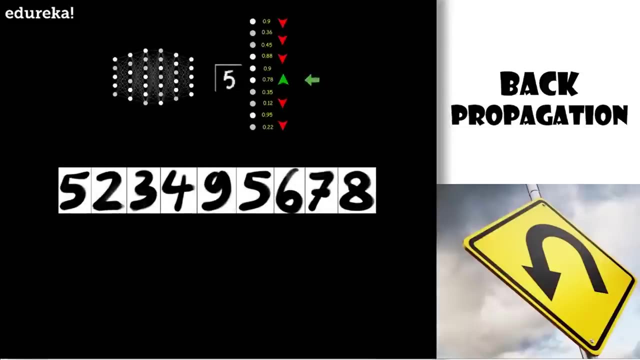 its value to classify 5 better. So what you do now is go through the same back propagation routine for every other training example, recording how each one of them would change the weights and biases, and you average together those weights and the desired changes. Now this collection. 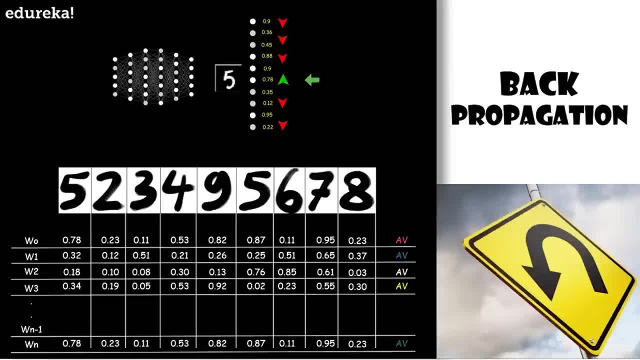 here of the weights and biases is proportional to the negative gradient of the cause function. It takes the computer an extremely long time to add up the influence of every single training example, every single gradient descent step. So, guys, I hope you got an idea of what. 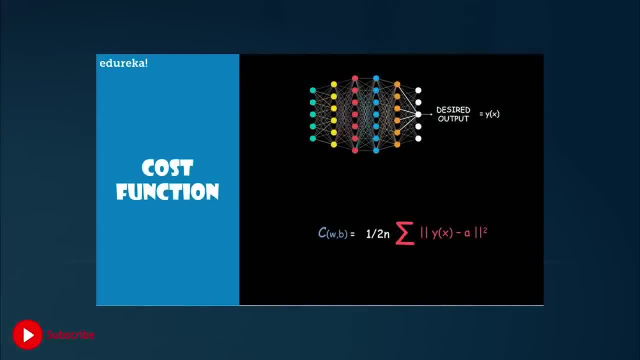 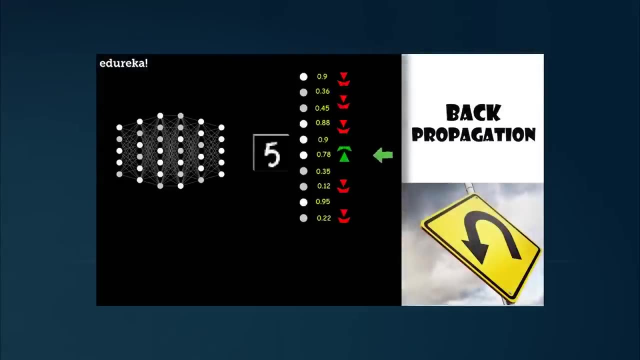 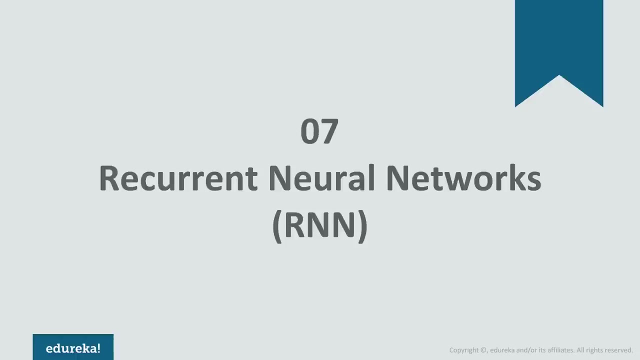 exactly a gradient descent is how it works, the various parameters involved in the working of the gradient descent, and how back the neural network is learning and modifying itself to have a better accuracy. Today we'll be focusing on recurrent neural networks, So, without any further ado, let us 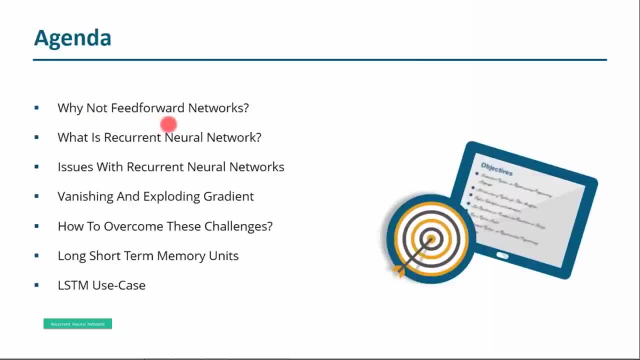 move forward and have a look at the agenda for today. So we'll begin by understanding why can't we use feed forward networks for various problems. will focus on various issues with feed forward networks. after that we'll understand how recurrent neural network solve this problem and 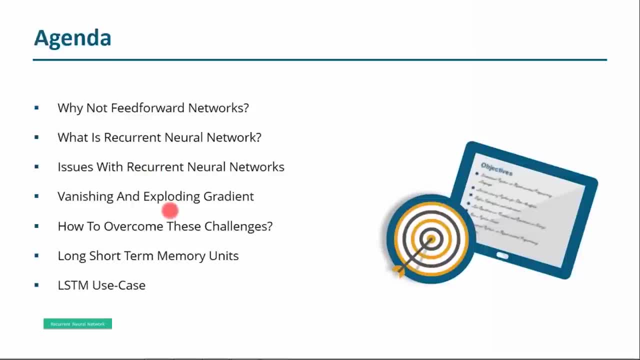 finally, we'll be looking at an LSTM use case. So, guys, let's begin. we'll understand why can't we use feed forward networks. Now let us take an example of a feed forward network that is used for image classification. So we have trained this. 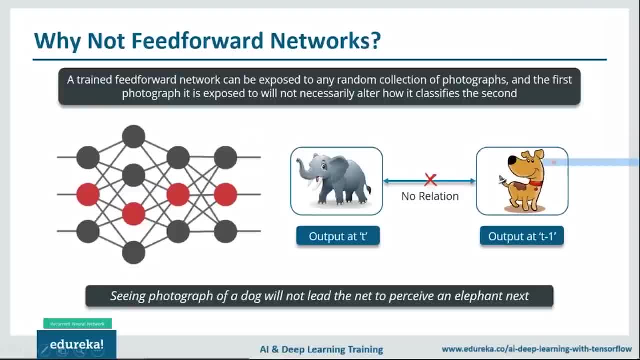 particular network for classifying various images of animals. Now, if you feed in an image of a dog, it will identify that image and it will identify the image and will provide a relevant label to that particular image. Similarly, if we feed in an image of an elephant, it 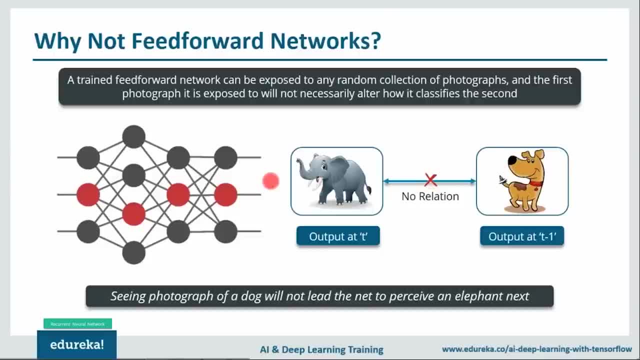 will provide a relevant label to that particular image as well. Now, if you notice, the new output that we have got that is, classifying an elephant has no relation with the previous output that is of a dog, or you can say that the output at time t is: 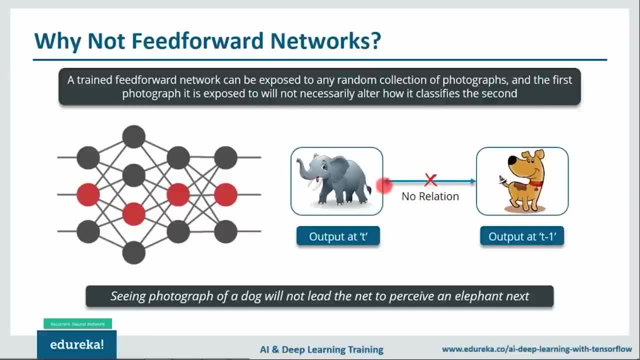 independent of output at time t minus 1, as we can see that there is no relation between the new output and the previous output, Outputs are independent to each other. Now there are few scenarios where we actually need the previous output to get the new output. 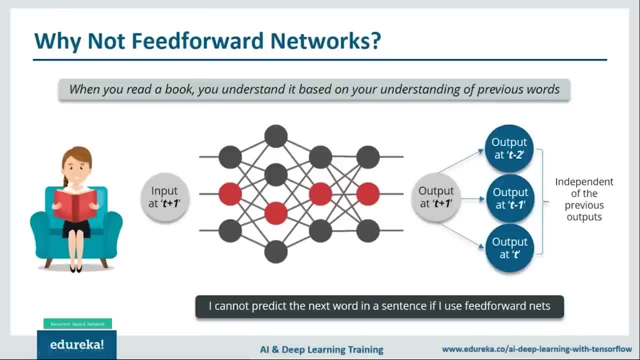 Let us discuss one such scenario Now. what happens when you read a book? You will understand that book only on the understanding of your previous words. Alright, so if I use a feed forward network and try to predict the next word in a sentence, I can't do. 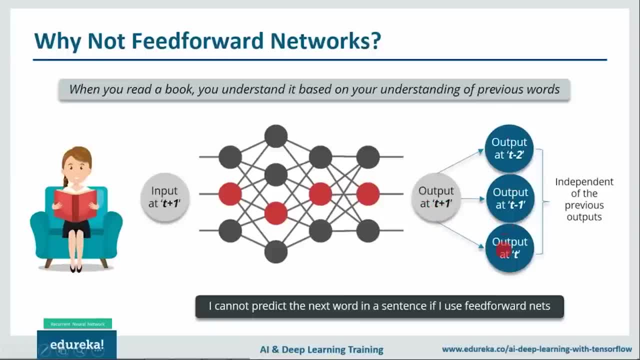 that. Why can't I do that? Because my output will actually depend on the previous outputs, But in the feed forward network my output at t plus 1 has no relation with output at t minus 2, t minus 1 and at t. 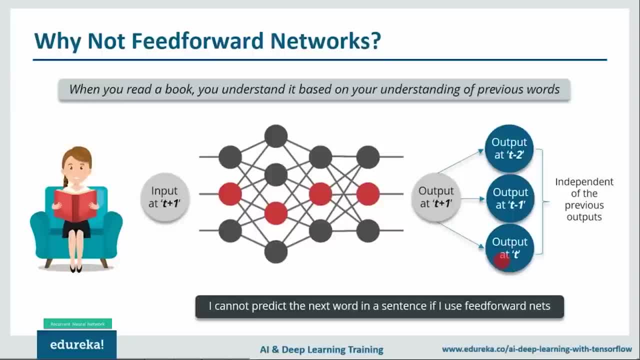 So, basically, we cannot use feed forward networks for predicting the next word in a sentence. Similarly, you can think of many other examples where we need the previous output, some information from the previous output, so as to infer the new output. This is just one small example. 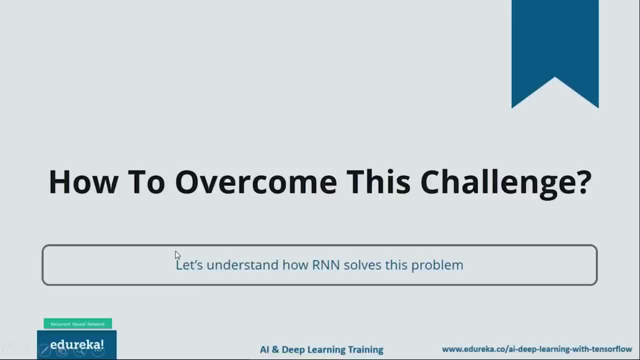 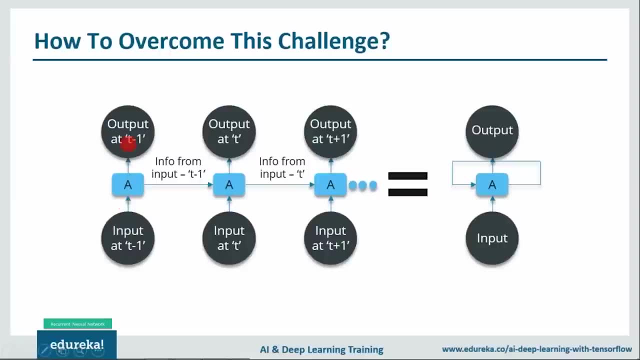 There are many other examples that you can think of. So we will move forward and understand how we can solve this particular problem. So over here what we have done: we have taken the input from our network. then we will get the output at t minus 1.. 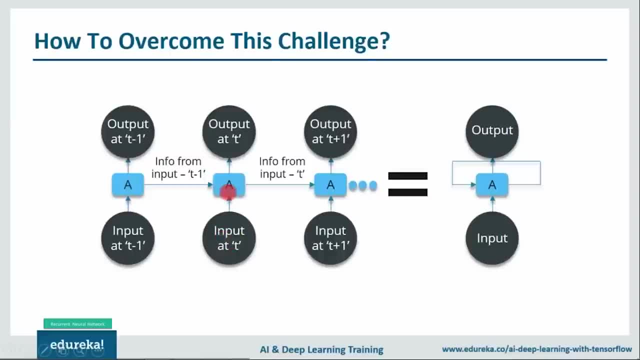 Then at the next time stamp, that is, at time t, we have input at time t that will be given to our network along with the information from the previous time stamp, that is, t minus 1, and that will help us to get the output at t. 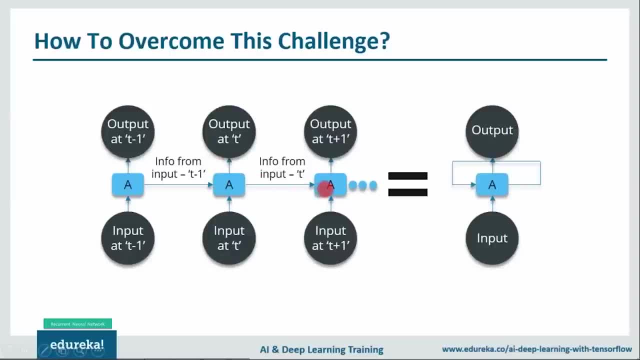 Similarly, at output for t plus 1, we have two inputs. One is a new input that we give, another is the information coming from the previous time stamp, that is t, in order to get the output at time t plus 1.. Similarly it can go. 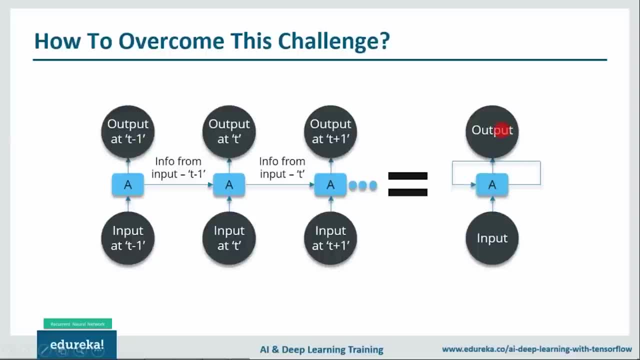 on. So here we have two inputs. So over here I have just written a generalized way to represent it. There is a loop where the information from the previous time stamp is flowing, and this is how we can solve this particular challenge. Now let us understand. 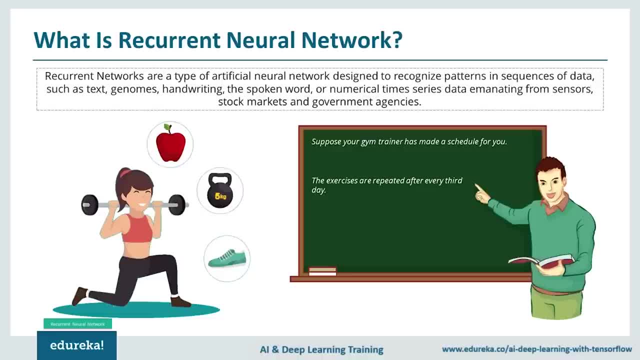 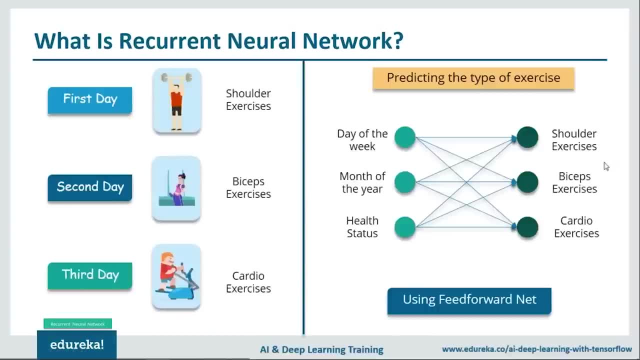 what exactly are recurrent neural networks? So for understanding recurrent neural network, I will take an analogy. Suppose your gym trainer has made a schedule for you. The exercises are repeated after every third day. Now this is the order of your exercises. First day you will be: 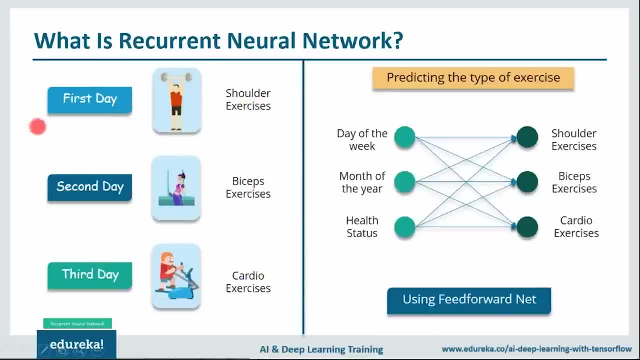 doing shoulders. second day you will be doing biceps. third day, you will be doing cardio. These exercises are repeated in a proper order. Now what happens when we use a feed forward network for predicting the exercise today? So we will provide in the input, such as day of. 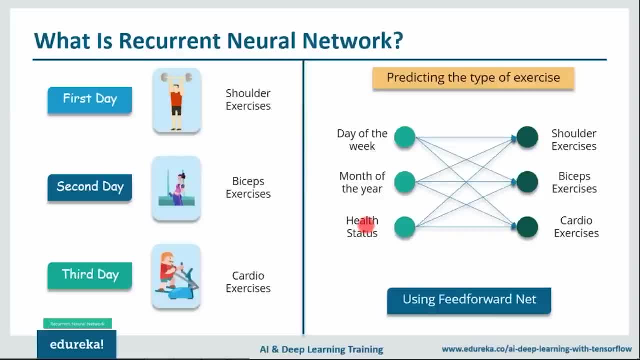 the week, month of the year and health status Alright, and we need to train our model or our network on the exercises that we have done in the past. After that, there will be a complex voting procedure involved that will predict the exercise for us. 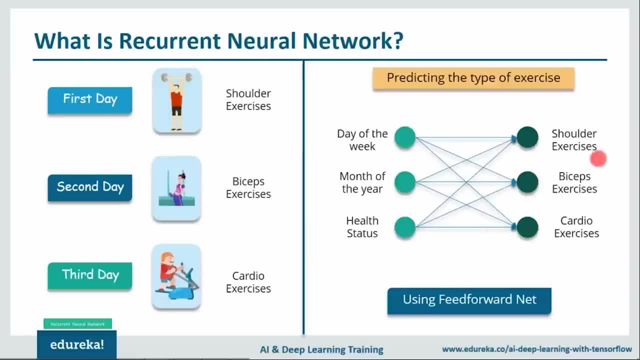 And that procedure won't be that accurate. So whatever output we will get won't be as accurate as we want it to be. Now, what if I change my inputs and I make my inputs as what I have done yesterday? So if I have done, 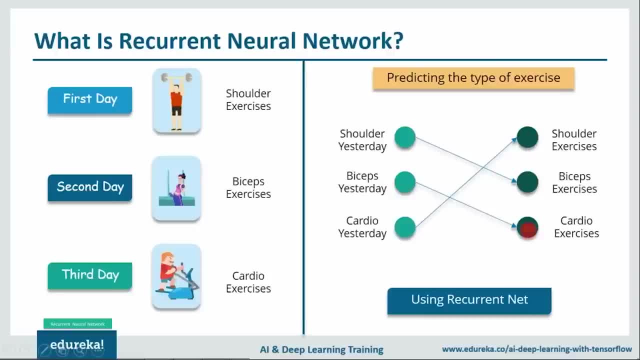 shoulder, then definitely today, I will be doing biceps. Similarly, if I have done biceps yesterday, today I will be doing cardio. Similarly, if I have done cardio yesterday, today I will be doing shoulder Now. there can be one scenario where you are unable to go to gym for 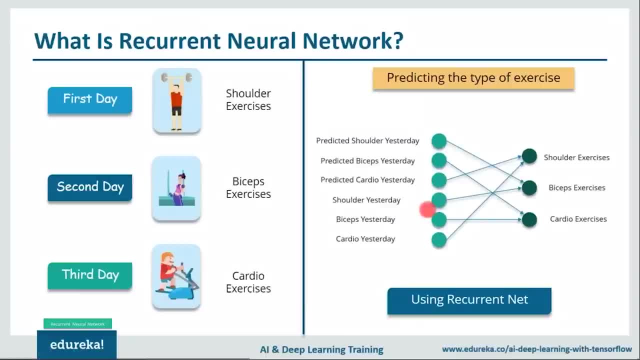 one day, due to some personal reasons, you could not go to the gym. Now what will happen at that time? We will go one time stamp back and we will feed in what exercise that happened day before yesterday. So if the exercise that happened day before 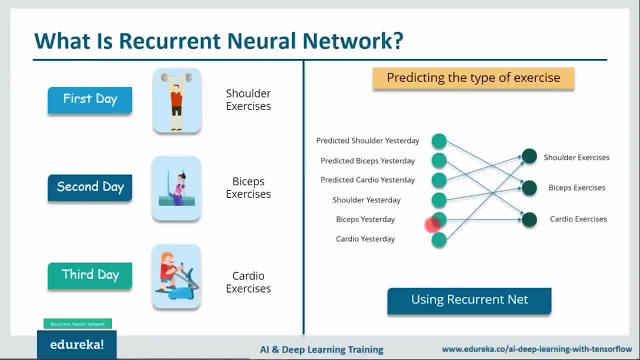 yesterday was shoulder, then yesterday there were biceps. Similarly, if biceps happened day before yesterday, then yesterday would have been cardio exercises. Similarly, if cardio would have happened day before yesterday, yesterday would have been shoulder exercises. And this prediction, the prediction for the 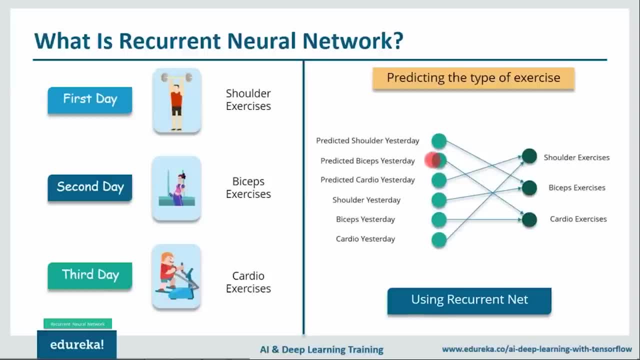 exercise that happened yesterday will be fed back to our network and these predictions will be used as inputs in order to predict what exercise will happen today. Similarly, if you have missed your gym, say for two days, three days or one week, so you need to. 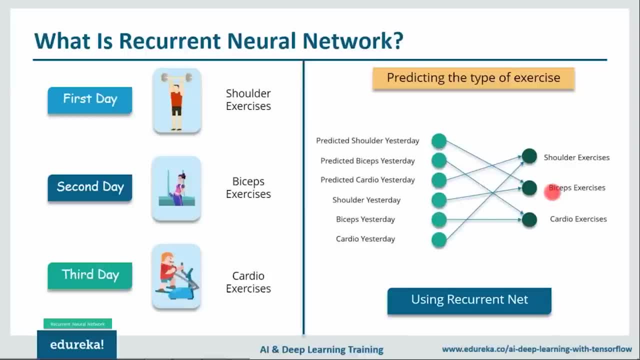 roll back. You need to go to the last day when you went to the gym. you need to go back to the last day when you went to the gym. you need to figure out what exercise you did on that day. Feed that as an input. 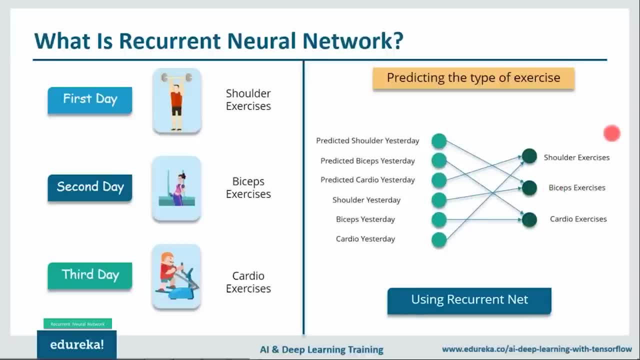 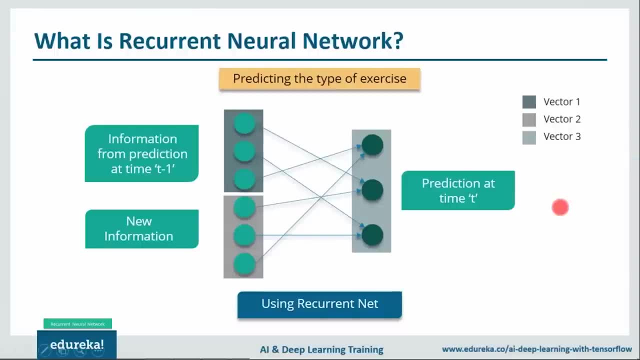 and then only you'll be getting the relevant output as to what exercise will happen today. Now, what I'll do? I'll convert these things into a vector. Now, what is a vector? Vector is nothing but a list of numbers. Alright, So this is the new. 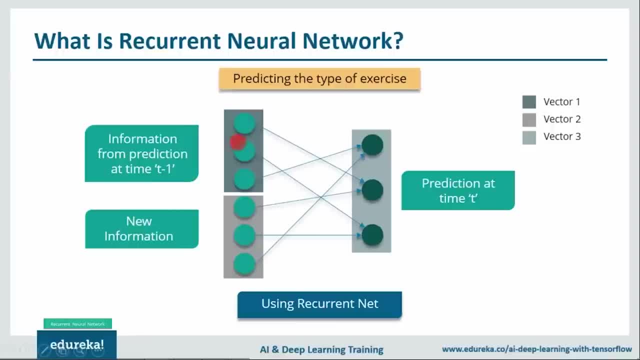 information, guys, along with the information from the prediction at the previous time step. So we need both of these in order to get the prediction at time. t Imagine if I have done shoulder exercises yesterday, So this will be one. this will be zero, and 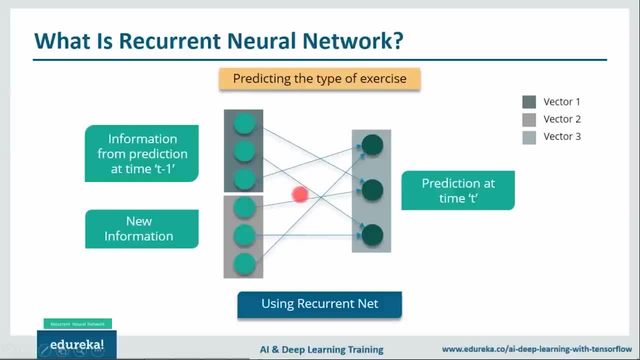 this will be zero. So what will happen will be biceps exercise, because if I have done shoulder yesterday, it will be biceps. So my output will be zero. one and zero. And this is how vectors work, guys. So I hope you have. 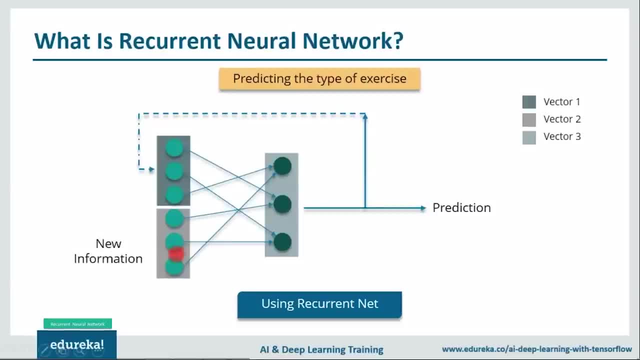 understood this, guys. Now this is how a neural network looks like, guys. We have new information along with the information from the previous time step. The output that we have got in the previous time step will use. certain information from that will feed into our network. 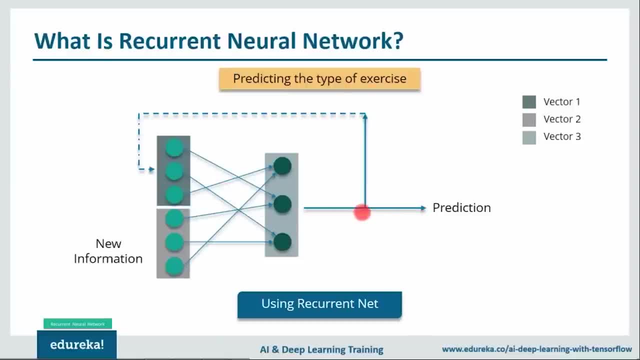 as inputs and then that will help us to get the new output. Similarly, this new output that we have got will feed into our network as inputs and then that will take some information from that feed in as an input to our network along with the new information to. 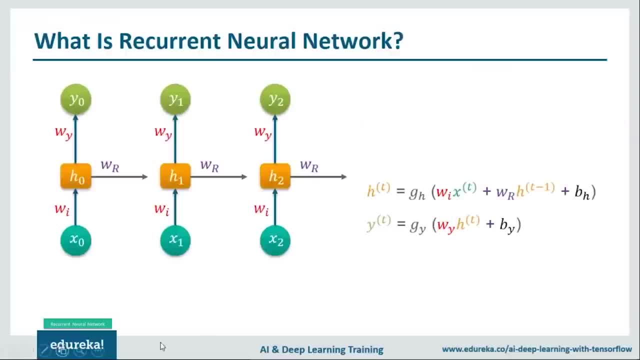 get the new prediction, and this process keeps on repeating. Now let me show you the math behind the recurrent neural networks. So this is the structure of a recurrent neural network. guys, Let me explain you what happens here. Now consider a time. t equals to zero. 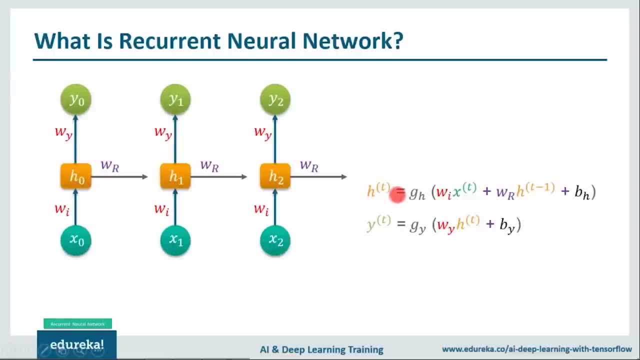 We have input x naught and we need to figure out what is h naught. So according to this equation, h of zero is equal to wi weight matrix multiplied by our input x of zero plus wr of zero. So that's going to be. 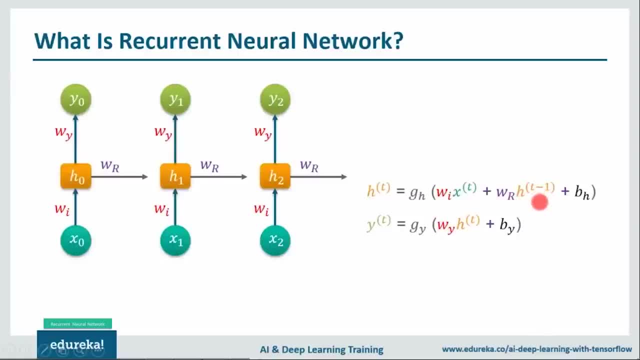 h of zero minus one, which is h of minus one, and time can never be negative, so this particular equation cannot be applied here. plus a bias, So wi into x of zero, plus bh passes through a function, g of h to get h of zero over here. 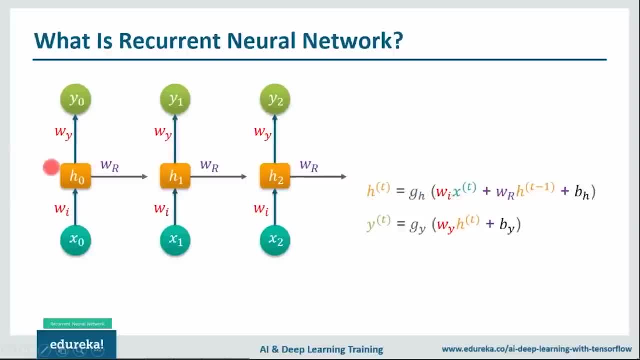 After that I want to calculate y naught. So for y naught I will multiply h of zero with the weight matrix wi and I will add a bias to it and pass it through a function g of y to get y naught Now, in the next time. 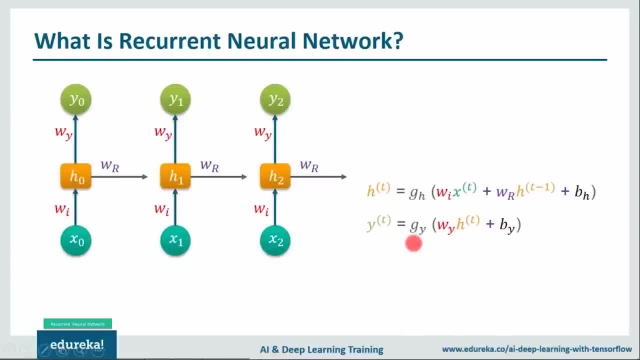 stamp, that is, at time, t equals to one. things become more and more complicated. So let me show you how to do this. So let me show you how to do this. So let me show you how to do this. This becomes a bit tricky. 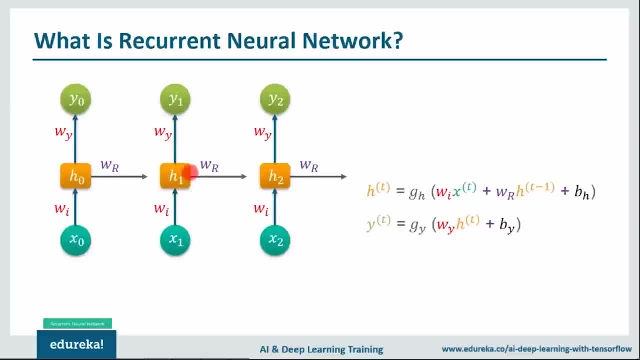 Now let me explain you what happens here. So at time t equals to one, I have input x one. I need to figure out what is h one. So for that I'll use this equation. So I'll multiply wi. that is the weight matrix. 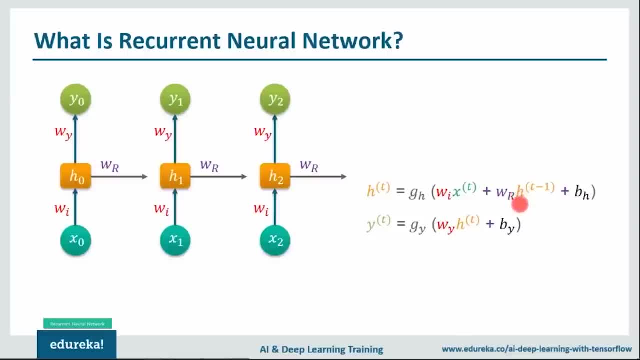 by the input x one plus wr, into h of one minus one, which is zero, h of zero. we know what we got from here. So wr into h of zero plus the bias. pass it through a function g of h to get the output as: 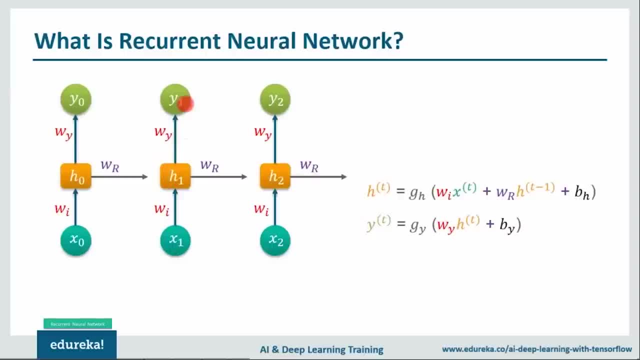 h one. Now this h one we'll use to get y one. We'll use this to get y one. We'll multiply h one with wi plus a bias and we'll pass it through a function g of y to get y one. Similarly, the next. 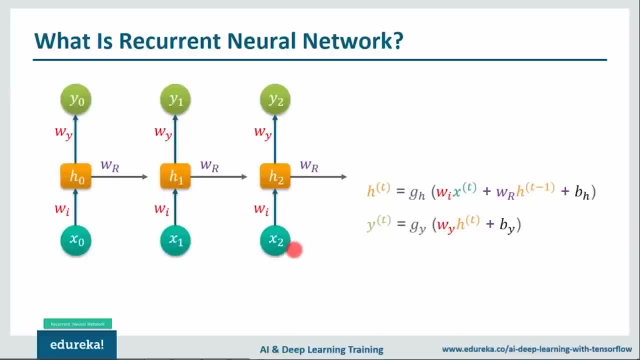 time stamp, that is, at time, t equals to two. we have input x two. We need to figure out what will be h two. So we'll multiply the weight matrix wi with x of two plus wr into h of one that we have got here, plus b of h. 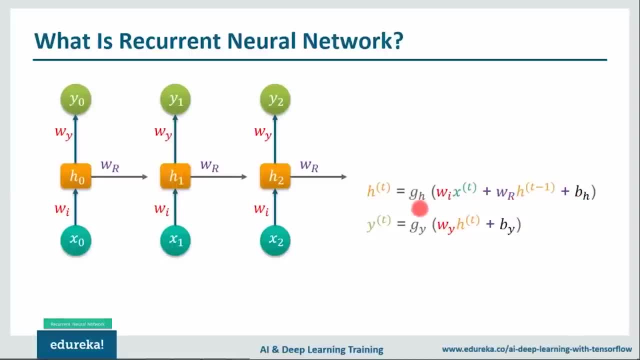 and pass it through a function g of h to get h of two. From h of two we'll calculate y of two, wi into h of two plus by that is the bias. pass it through a function g of y to get y two. 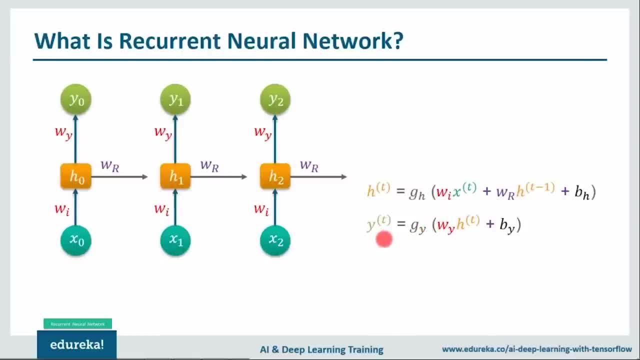 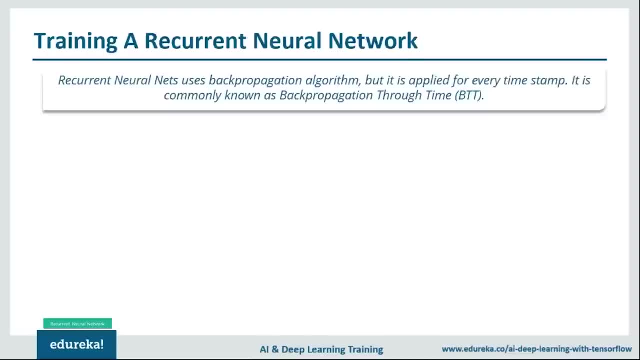 So now we know what we need to do to get y two. So we need to get y two, And this is how recurrent neural network works. guys, Now you must be thinking how to train a recurrent neural network. So a recurrent neural network uses back. 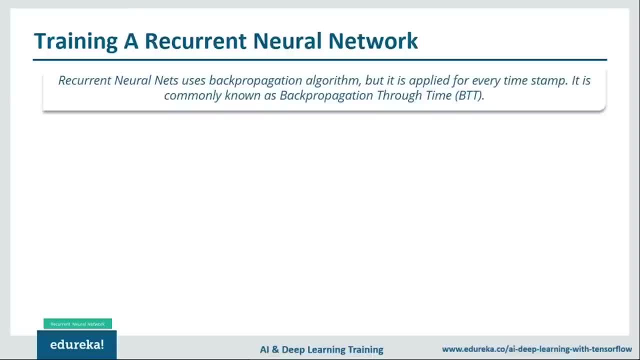 propagation algorithm for training, But back propagation happens for every time stamp. That is why it is commonly called as back propagation through type, And I've discussed back propagation in detail in artificial neural network tutorials so you can go through that Over here. I won't be. 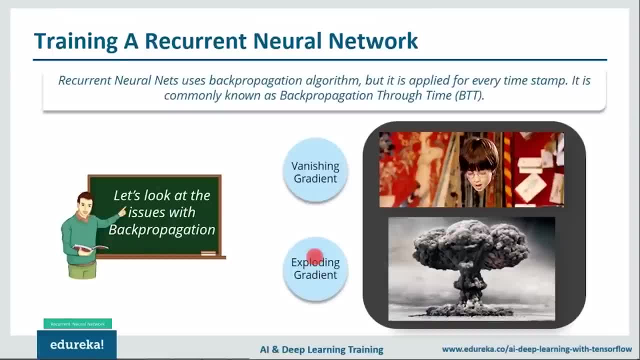 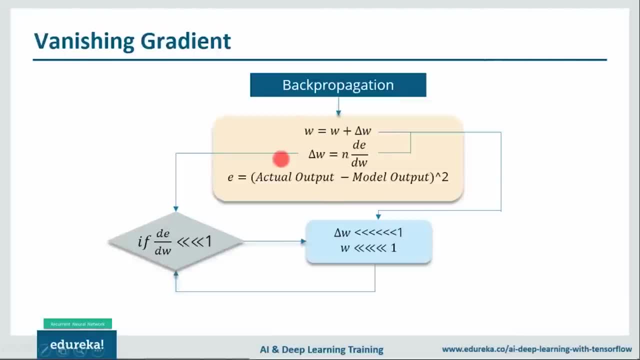 discussing back propagation in detail. I'll just give you a brief introduction of back propagation so that you can start exploring gradients. Let us see those one by one. So in vanishing gradient, what happens when you use back propagation? you tend to calculate the error. 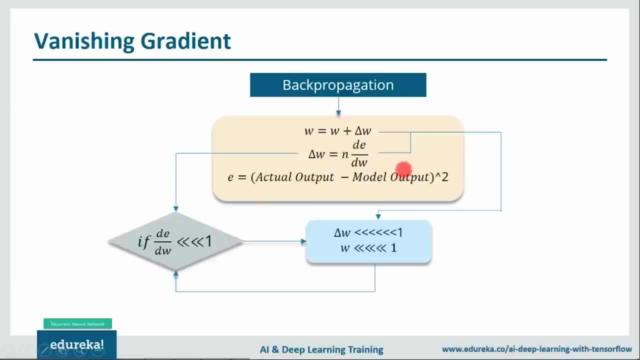 which is nothing but the actual output that you already know, minus the model output, the output that you got through your model and the square of that. So you figure out the error With that error. what do you do? You tend to find out the change in error. 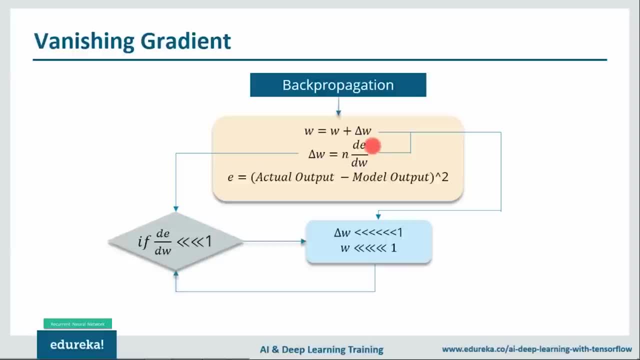 with respect to change in weight or any variable, So we'll call it weight here. So the change in weight multiplied by learning rate will give you the change in weight. Then you need to add that change in weight to the old weight to get the new weight. 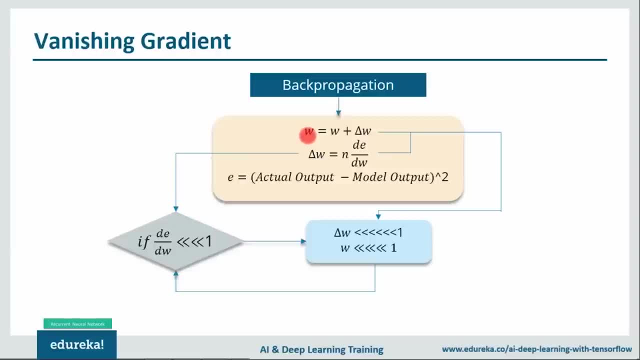 Alright. So obviously what we're trying to do, we're trying to reduce the error. So for that we need to figure out what will be the change in error if my variables are changed Right, So that way we can get the change in the variable. 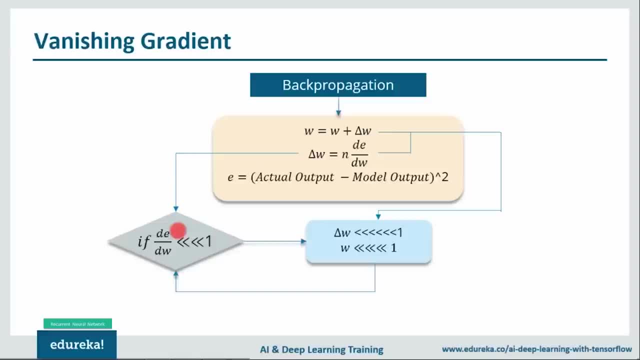 and add it to our old variable to get the new variable Now over here. what can happen if the value DE by DW- that is a gradient, or you can say the rate of change of error with respect to our variable weight, becomes very small than one? 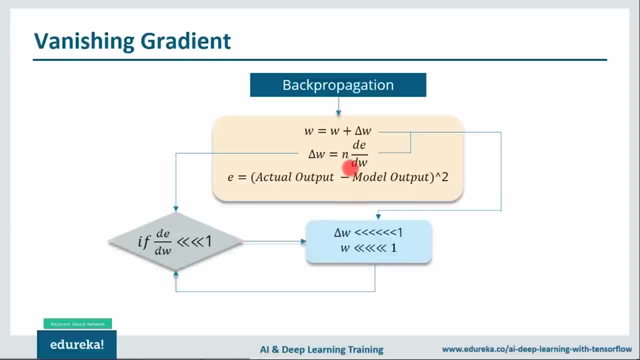 Like it is point zero, zero, something. So if you multiply that with the learning rate, which is definitely smaller than one, then you get the change of weight, which is negligible. Alright, So there might be certain examples where you know you are trying to predict, say a next. 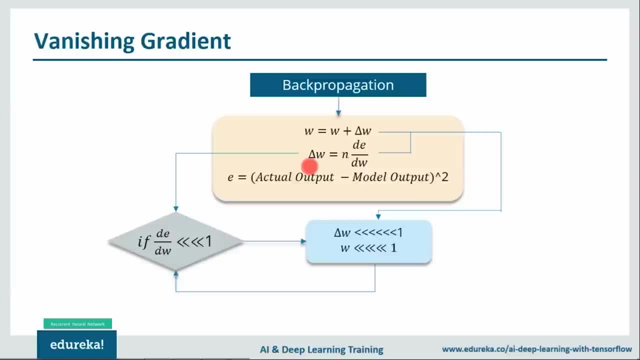 word in a sentence and that sentence is pretty long. For example, if I say I went to France, dash, dash, dash, I went to France, Then there are certain words. Then I say few of them, speak dash. Now I need to predict speak what will. 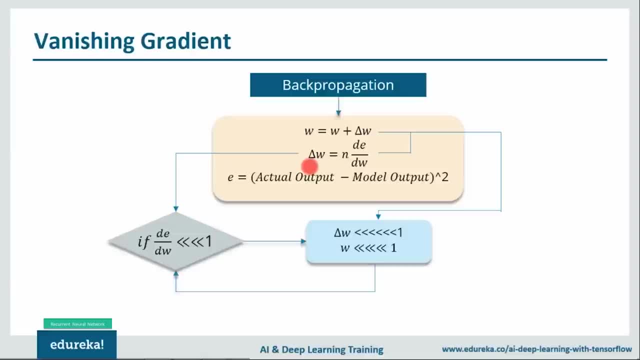 come after speak. So for that I need to go back in time and check what was the context, which will be very complex, And due to that, there will be a lot of iterations And because of that, this error, this change in weight, will become very small, very small. 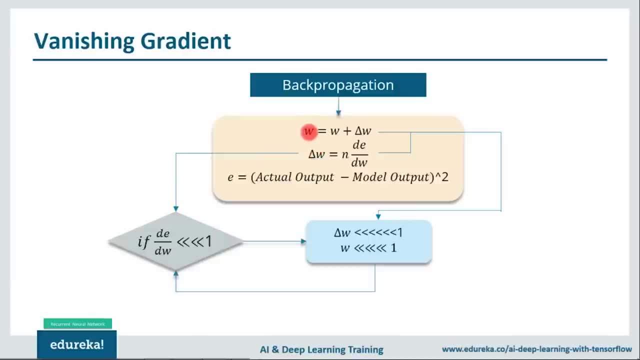 So the new weight that we'll get will be actually almost equal to your old weight, So there won't be any updation of weight. that will be happening, And that is nothing but your vanishing gradient. Alright, I'll repeat it once more. 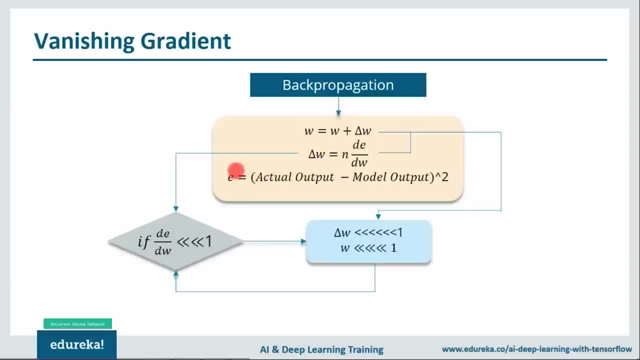 So what happens in back propagation? you find that there is no change in weight. So we first calculate the error. This error is nothing but the difference between the actual output or model output and the square of that. With that error we figure out what will. 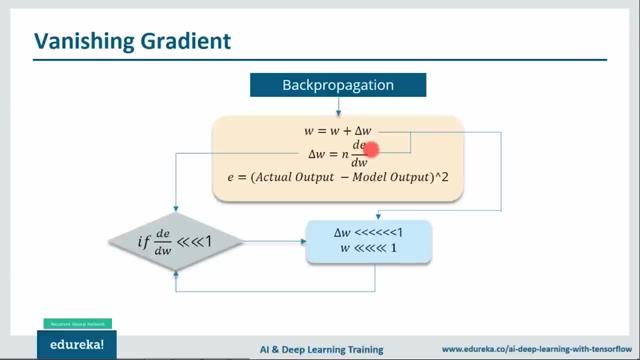 be the change in error when we change a particular variable, say weight. So DE by DW multiplied with learning rate to get the change in the variable or change in the weight. Now we'll add that change in the weight to our old weight to get the new weight. 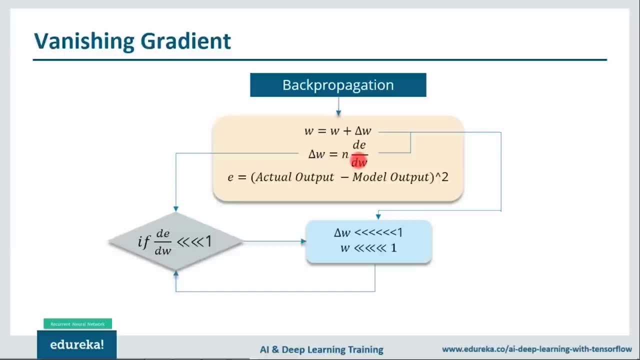 This is what back propagation is, guys. Alright, I'm just giving you a small introduction to back propagation. Now consider a scenario where you need to predict what comes after speak And your sentence is something like this: I have been to France. then there are a lot of. 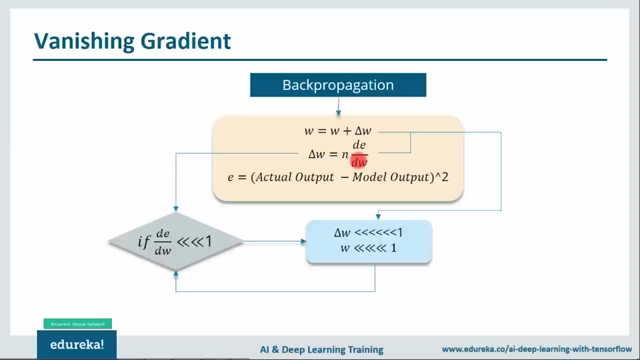 words. After that, few people speak, and then you need to predict what comes after speak. Now, if I need to do that, I need to go back and understand the context. What is it talking about? And that is nothing but your long term dependencies. 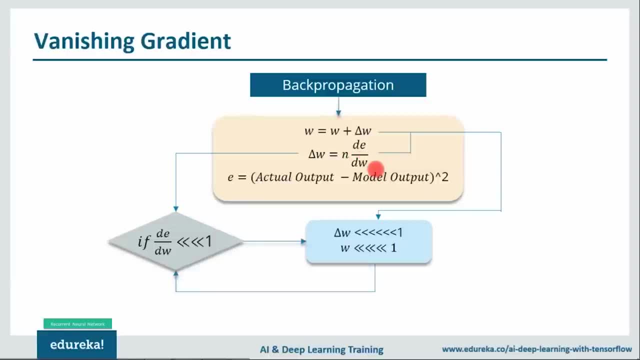 So what happens during long term dependencies? if this DE by DW becomes very small, then when you multiply it with N, which is again smaller than 1, you get delta W, which will be very small. That will be negligible. So the new weight that you will get here 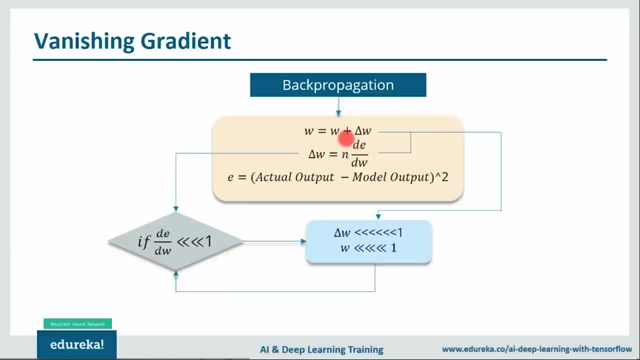 will be almost equal to your old weight. So I hope you are getting my point. So this new weight- so there will be no updation of weights guys- This new weight will definitely be, will always be almost equal to our old weight. There won't be any. 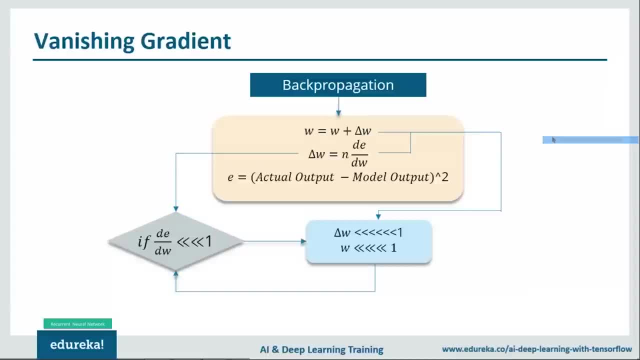 learning here. So that is nothing but your vanishing gradient problem. Similarly, when I talk about exploding gradient, it is just the opposite of vanishing gradient. So what happens when your gradient, or DE by DW, becomes very large, becomes greater than greater than 1.. 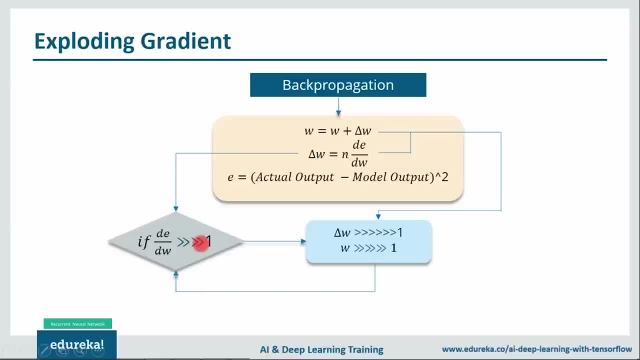 Alright And you have some long term dependencies. So at that time your DE by DW will keep on increasing, delta W will become large and because of that your weights, the new weight that will come, will be very different from your old weight. So these two are the. 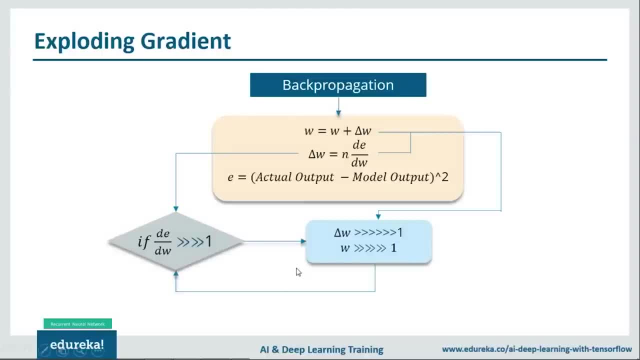 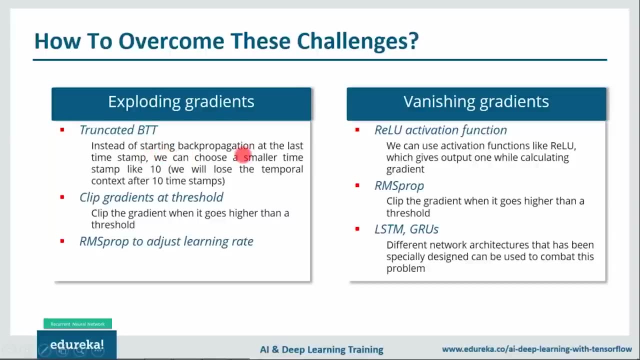 problems with back propagation. Now let us see how to solve these problems Now. exploding gradients can be solved with the help of truncated BTT back propagation through time. So instead of starting back propagation at the last time stamp, we can use a smaller time stamp like 10. 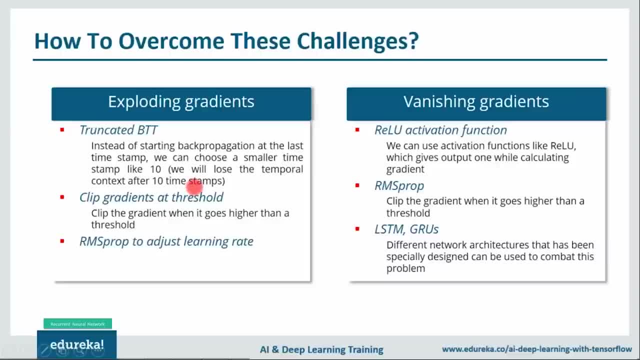 or we can clip the gradients at a threshold, so there can be a threshold value where we can, you know, clip the gradients and we can adjust the learning rate as well. Now for vanishing gradient, we can use a ReLU activation function We have discussed. 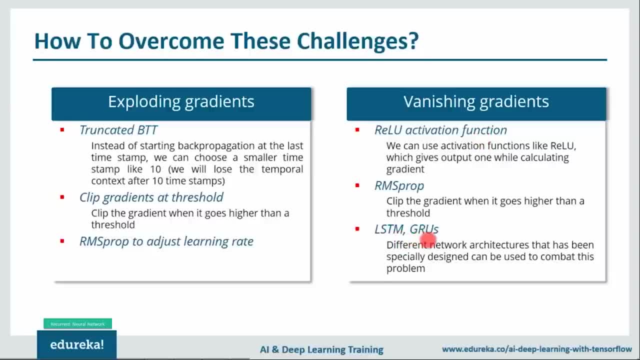 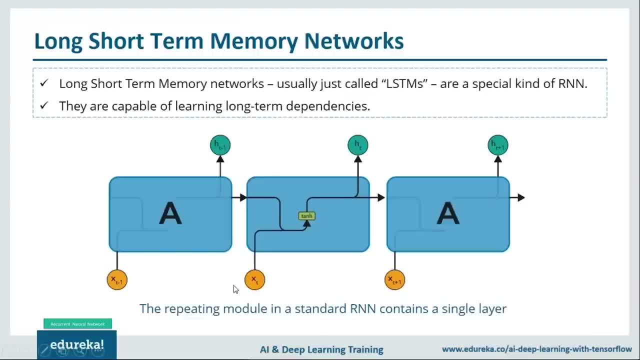 ReLU activation function in artificial neural network. tutorial, guys. Similarly, we can also use LSTM and GRUs. In this tutorial, we will be discussing LSTMs, that are long short term memory units. Now let us understand what exactly are LSTMs. So, guys, we saw. 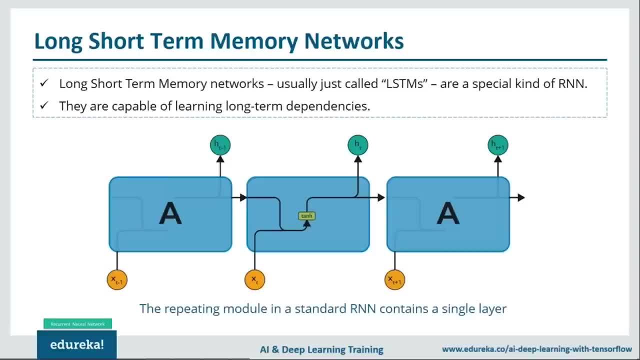 what are the two recurrent neural networks. Now we will understand how we can solve that with the help of LSTMs. Now what are LSTMs? Long, short term memory networks, usually called as LSTMs, are nothing but a special kind of recurrent neural. 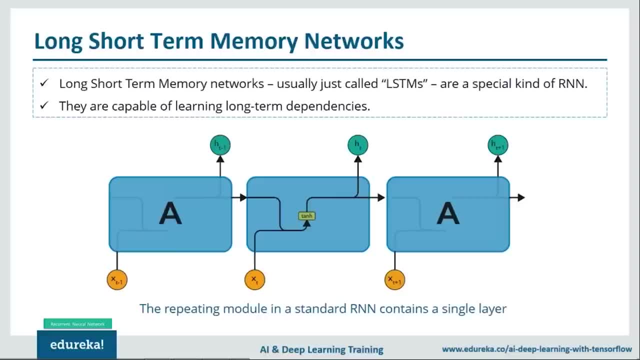 network and these recurrent neural networks are capable of learning long term dependencies. Now, what are long term dependencies? I have discussed that in the previous slide, but I will just explain it to you here as well. Now what happens sometimes? we only need to look at the recent. 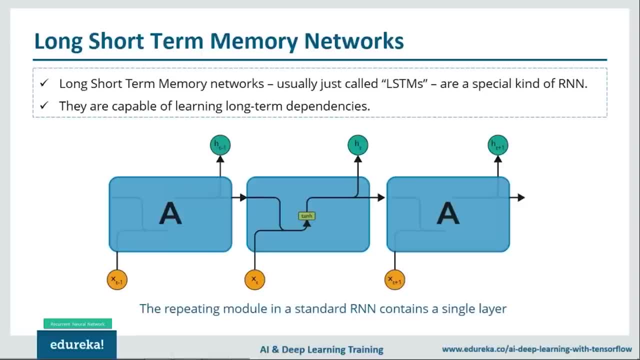 information to perform the present task. Now let me give you a language model trying to predict the next word based on the previous ones. If we are trying to predict the last word in the sentence, say: the clouds are in the sky, So we don't need 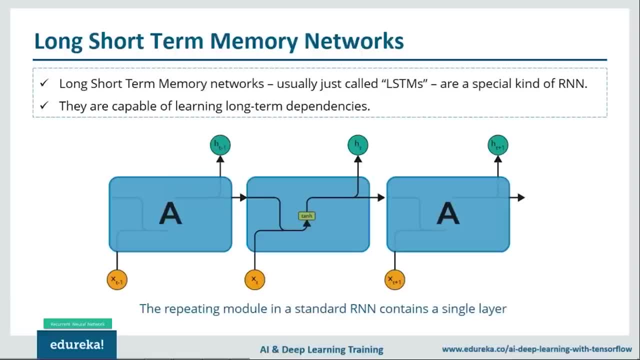 any further context, It's pretty obvious that the next word is going to be sky. Now, in such cases where the gap between the relevant information and the place that it's needed is small, RNNs can learn to use the past information, and at that time, there won't. 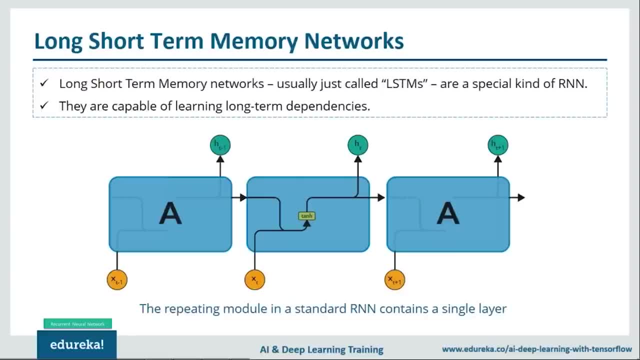 be such problems like vanishing and exploring gradient, But there are few cases where we need more context. Consider trying to predict the last word in the text. I grew up in France. Then there are some words after that comes. I speak fluent French. 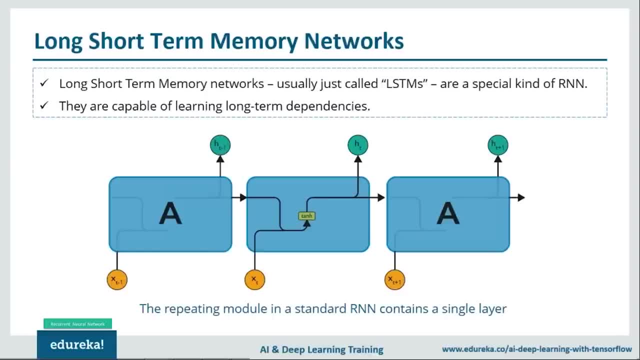 Now, recent information suggests that the next word is probably the name of a language, But if you want to narrow down which language, we need the context of France from further back, and it's entirely possible for the gap between the relevant information and the point where it is. 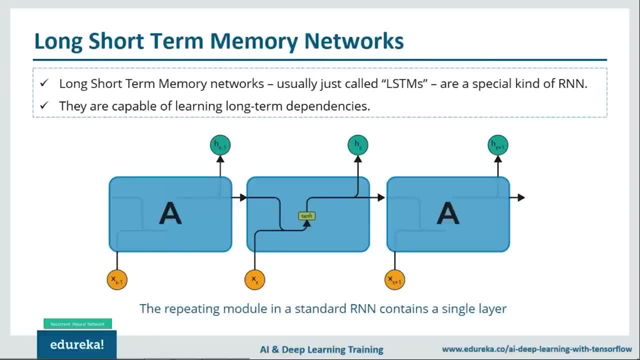 needed to become very large, And this is nothing but long-term dependencies. So let's look at the context of France, So let's start with France, and the LSTMs are capable of handling such long-term dependencies. Now LSTMs also have 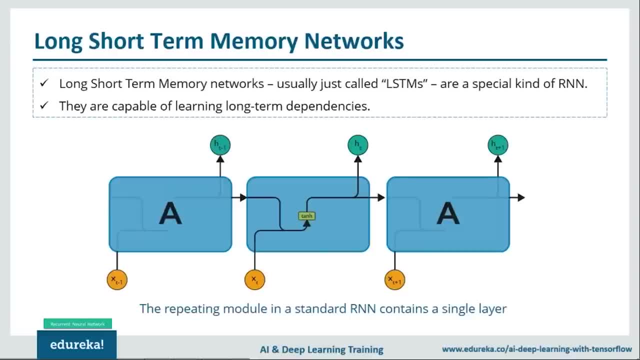 a chain like structure, like recurrent neural networks. Now, all the recurrent neural networks have the form of a chain of repeating modules of neural networks. Now, in standard RNNs, the repeating module will have a very simple structure, such as a single tanh layer that you can see. 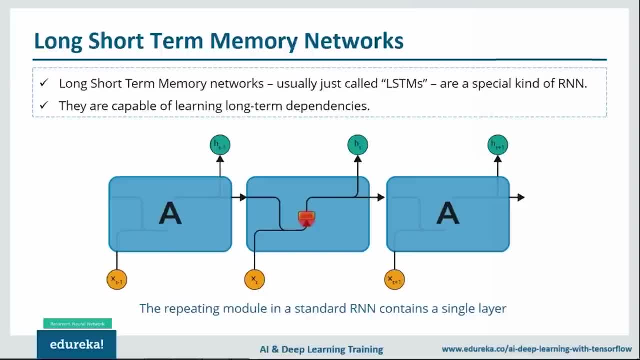 Now, this tanh layer is nothing but a squashing function. Now, what I mean by squashing function is to convert my values between minus one and one. Alright, that's why we use tanh, And this is an example of an RNN. 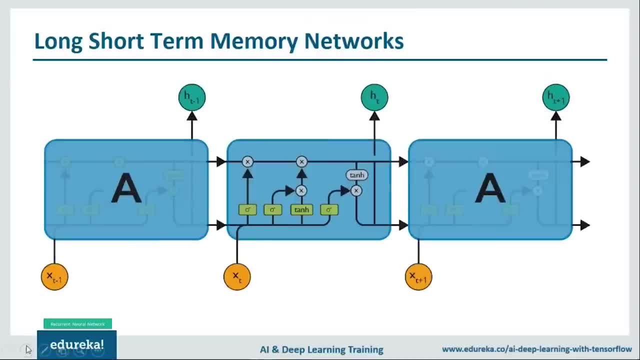 Now we'll understand what exactly are LSTMs. Now this is a structure of an LSTM. If you notice, LSTM also have a chain like structure, but the repeating module has different structures. Instead of having a single neural network layer, there are four interacting in a very 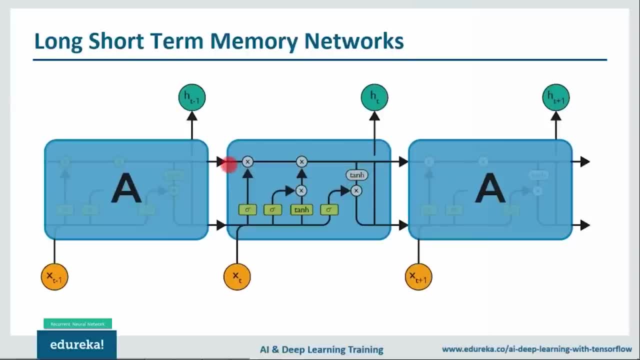 special way. Now, the key to LSTM is the cell state, Now this particular line that I'm highlighting. this is what is called the cell state, The horizontal line running through the top of the diagram. So this is nothing but your cell state. 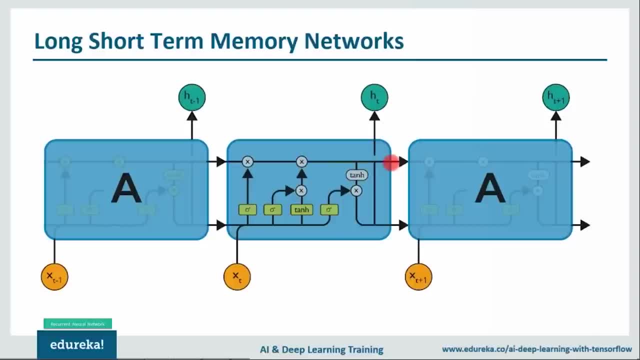 Now you can consider the cell state as a kind of a conveyor belt. It runs straight down the entire chain with only some minor linear interactions. Now, what I'll do? I'll give you a walkthrough of LSTM step by step. Alright, so we'll start. 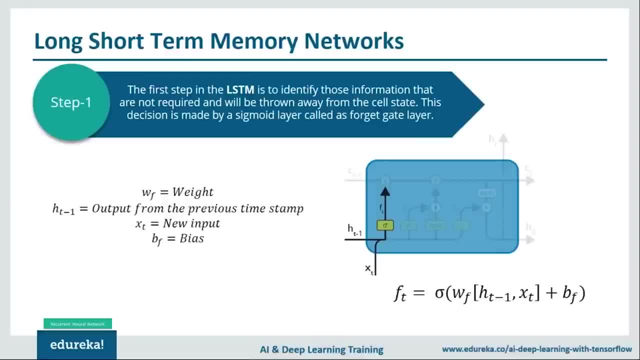 with the first step. Alright, guys. so the first step in our LSTM is to decide what information we are going to throw away from the cell state. And you know what is the cell state? right, I've discussed in the previous slide. Now this decision. 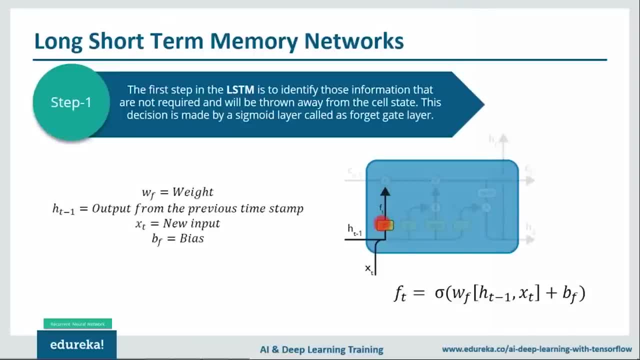 is made by the sigmoid layer, So the layer that I'm highlighting with my cursor, it is a sigmoid layer called the forget gate layer. It looks at HT minus one, that is, the information from the previous time stamp, and XT, which is the new input, and outputs a number. 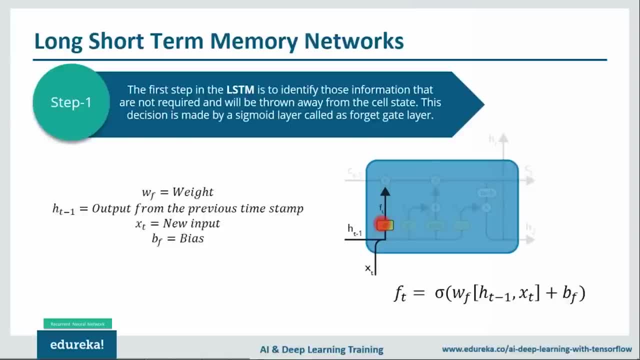 between zeros and one for each number in the cell state, CT minus one, which is coming from the previous time stamp. One represents completely- keep this, while a zero represents completely, get rid of this. Now, if we go back to our example of a language model trying to predict, 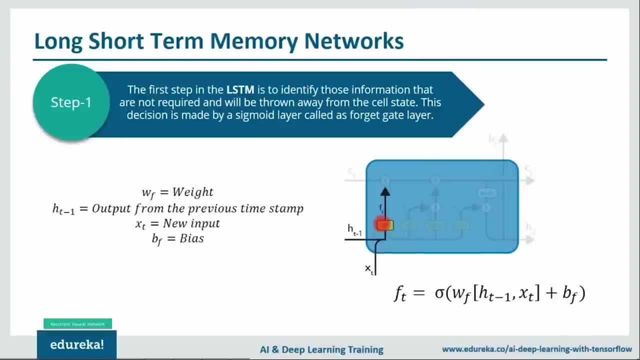 the next word based on all the previous ones. in such a problem the cell state might include the gender of the new subject, So the subject pronouns can be used when we see a new subject. we want to forget the gender of the old subject, right? 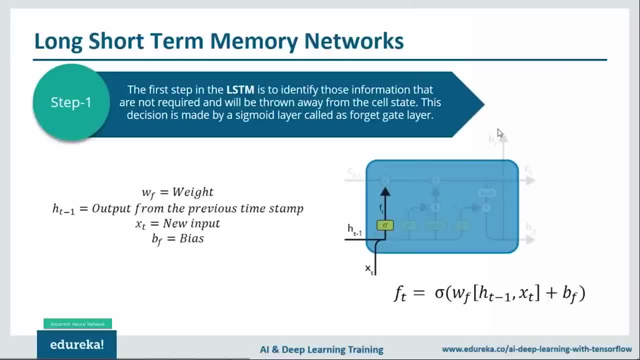 We want to use the gender of the new subject, so we'll forget the gender of the previous subject here. This is just an example to explain you what is happening here. Now let me explain you the equations which I've written here. So FT will be. 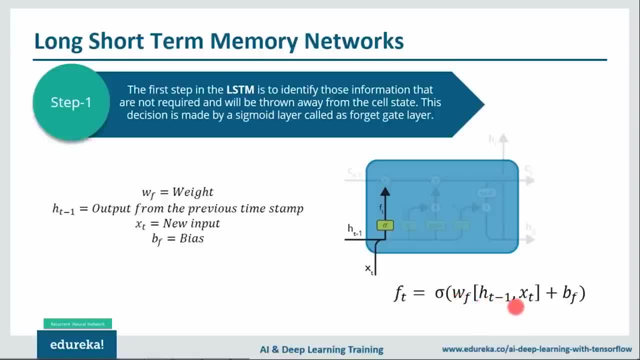 combining with the cell state. later on that I'll tell you. So currently FT is a велicode with a 0 and a 1. So this is what happens basically in the first step. Now let us see what happens in the next step. 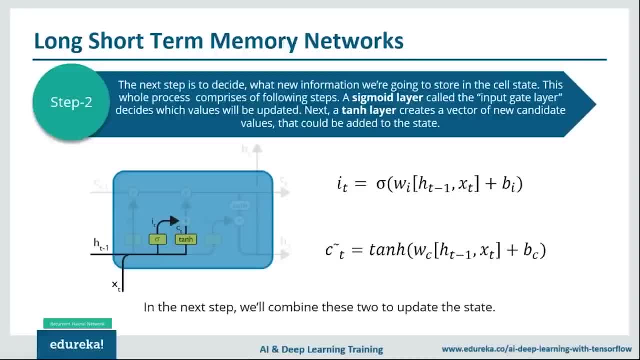 So the next step is to decide what information we are going to store. In the previous step we decided what information we are going to keep, but here we are going to decide what information store in the cell state. now this has two parts. first, a sigmoid layer. this is called a sigmoid. 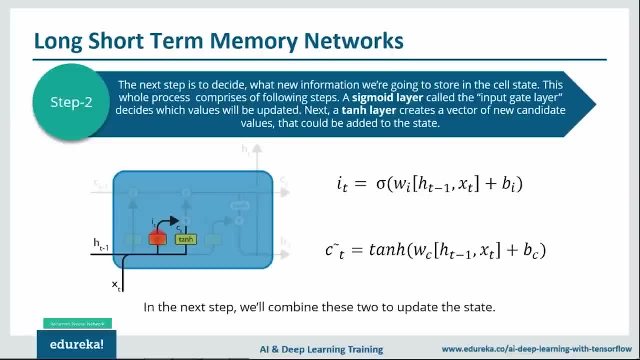 layer, and which is also known as an input gate layer, decide which values we'll update. all right, so what values we need to update? then there's also a tanhash layer that creates a vector of the candidate values: c bar of t minus one that will be added to the state later on. all right, so 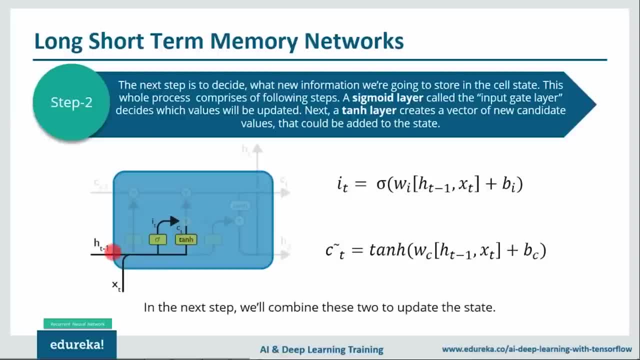 let me explain it to you in a simpler terms. so, whatever input that we are getting from the previous timestamp and the new input, it will be passed through an sigmoid function which will give us i of t, all right, and this i of t will be multiplied by ct, which is nothing but the input. 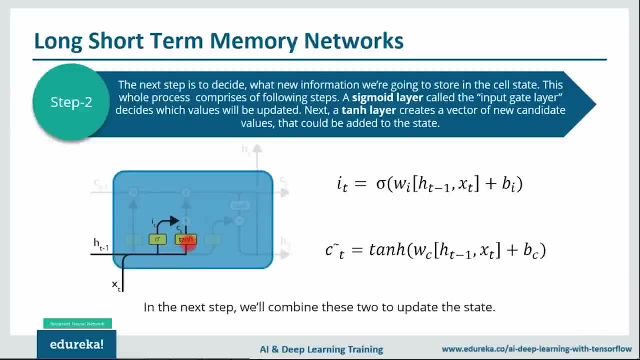 coming from the previous timestamp and the new input with that is passed through a tanh. that will result in ct and this will be later added on to our sales state and the next step will combine these two to update the states. now let me explain the equations. so i of t will be what weight matrix? 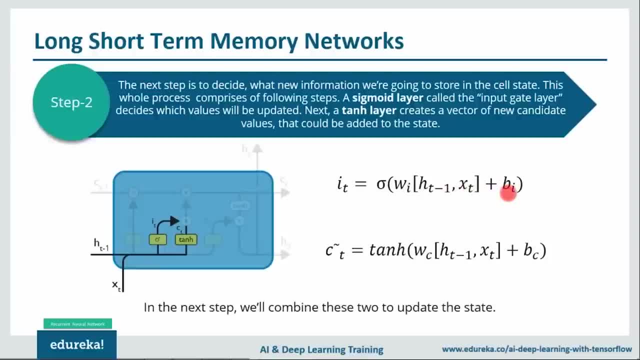 and then we have ht minus one comma xt multiplied by the weight matrix plus the bias. pass it through a sigmoid function. we get i of t. c bar of t will get, by passing a weight matrix, ht minus one xt plus bias, to a tanh squashing function. 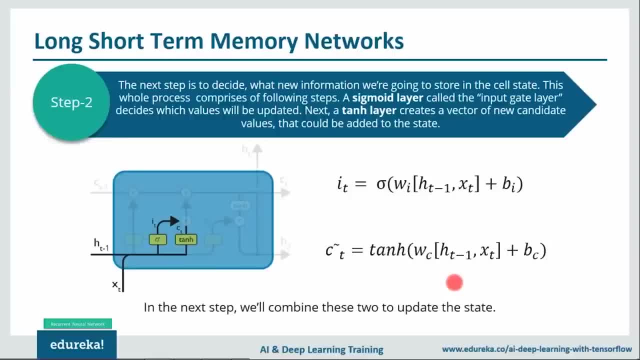 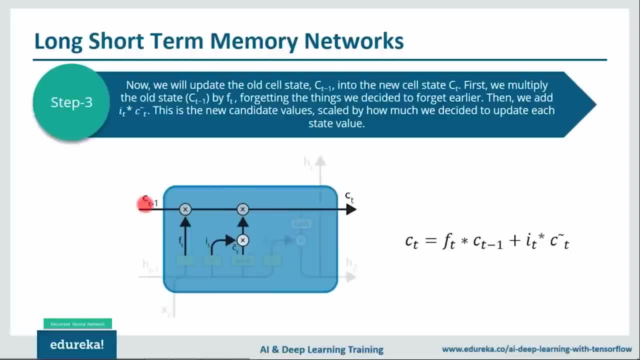 And we'll get c bar of t. all right. So, as I've told you earlier as well, in the next step we'll combine these two to update the state. Let us see how we do that. So now is the time to update the old cell state, ct minus one. 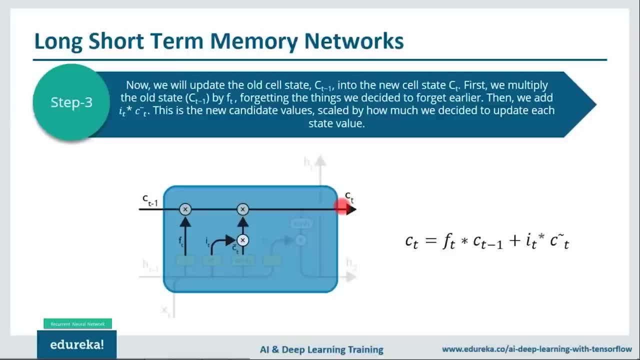 with the new cell state ct, all right- And the previous steps. we have already decided what to do. We just need to actually do it. So what we'll do? we'll multiply the old cell state ct minus one with ft that we got in the first step. 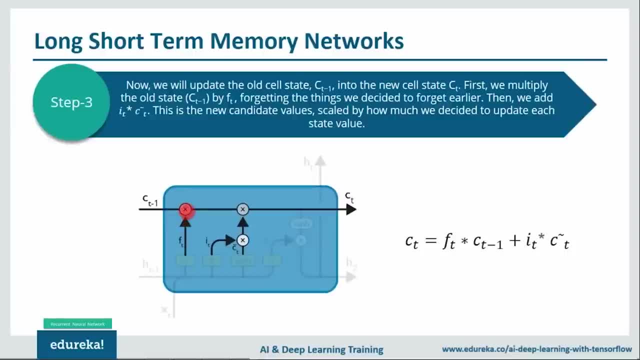 forgetting the things that we decided to forget earlier in the first step. if you can recall, Then, what we do: we add it to it and ct, then we add it by the term that will come after multiplication of it and c bar t. 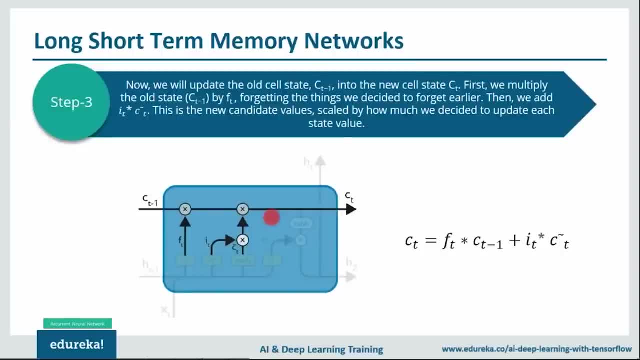 And this new candidate value scaled by how much we decided to update each state value. all right, So in the case of the language model that we were discussing, this is where we would actually drop the information about the old subject- gender- and add the new information. 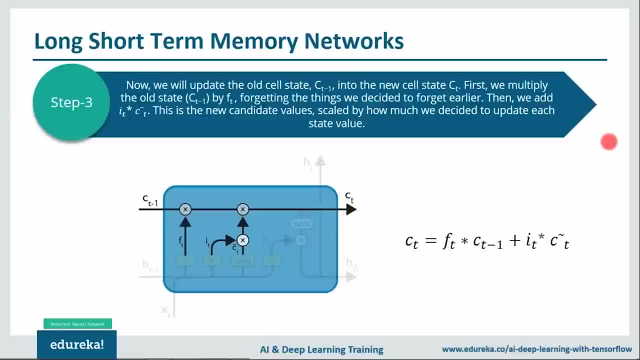 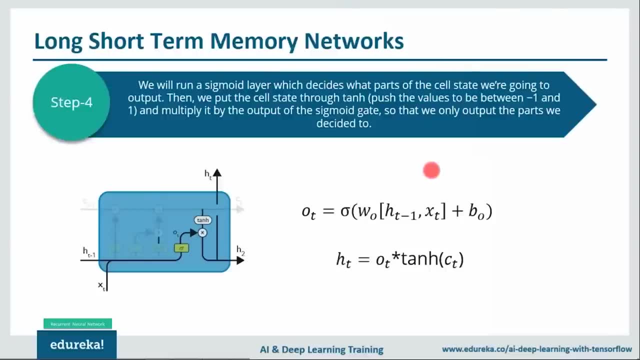 as we decided in the previous steps. So I hope you are able to follow to me, guys. all right, So let us move forward and we'll see what is the next step. Now our last step is to decide what we are going to output. 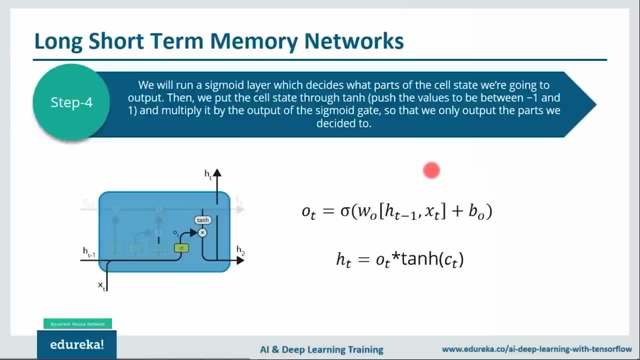 And this output will depend on our cell state, but it will be a filtered version. Now, finally, what we need to do is we need to decide what we are going to output, And this output will be based on our cell state. First, we need to pass ht minus one and x three. 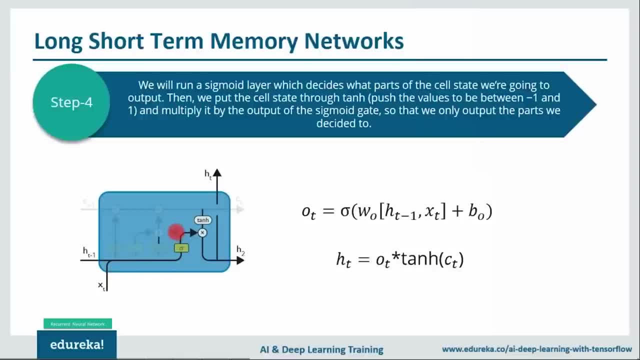 through a sigmoid activation function so that we get an output that is ot- all right, And this ot will be in turn multiplied by the cell state after passing it through it. So this will be a tanh squashing function or an activation function. 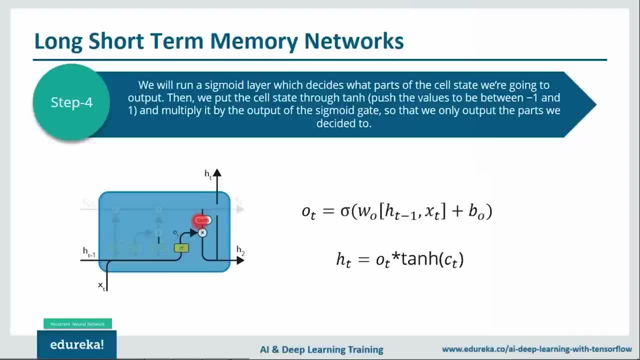 And why we do that Just to push the values between minus one and one. So after multiplying ot, that is, this value and a tanh ct, we'll get the output h two, which will be our new output, And that will only output the part that we decided to. 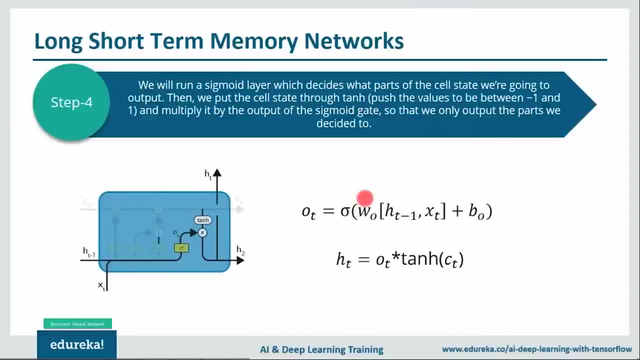 Whatever we have decided in the previous steps, it will only output that value. All right, now I'll take the example of the language model again. Since it just saw a subject, it might want to output information relevant to a verb, And in case that's what is coming next. 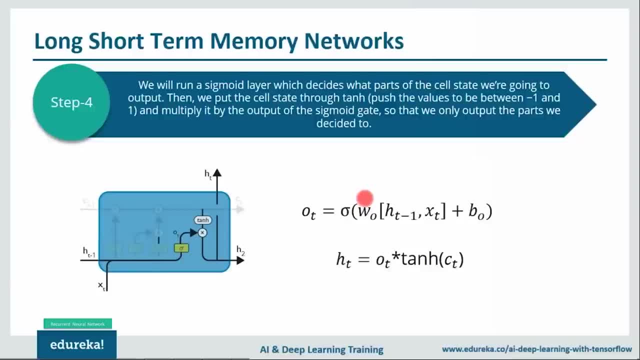 For example, it might output whether the subject is singular or plural, So that we know what form of a verb should be conjugated into. all right, And you can see from the. you can see the equations as well. Again, we have a sigmoid function. 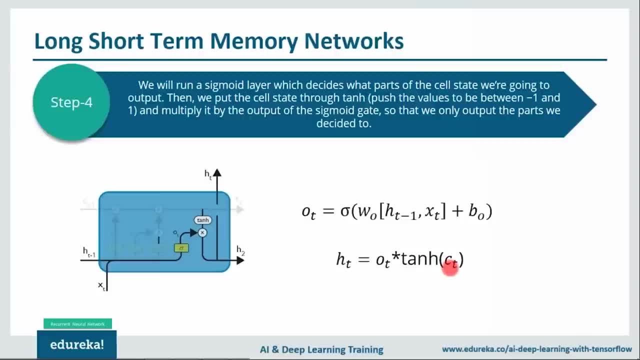 Then that whatever output we get from there, we multiply it with tanh ct to get the new output. All right, guys, so this is basically LSTMs in a nutshell. So in the first step, we decided what we need to forget. In the next step, we decided what are we going to add? 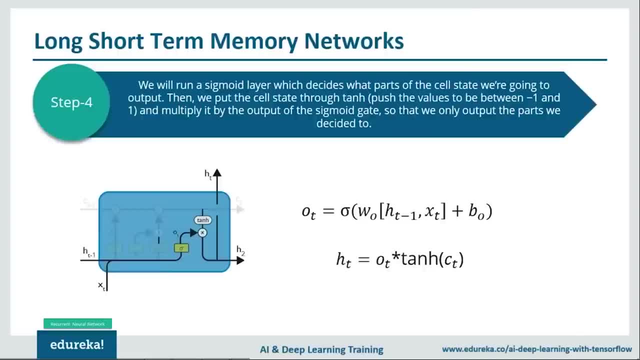 to our cell state, what new information we are going to add to our cell state, And we were taking an example of the gender throughout this whole process. all right, And in the third step, what we do. we actually combined it to get the new cell state. 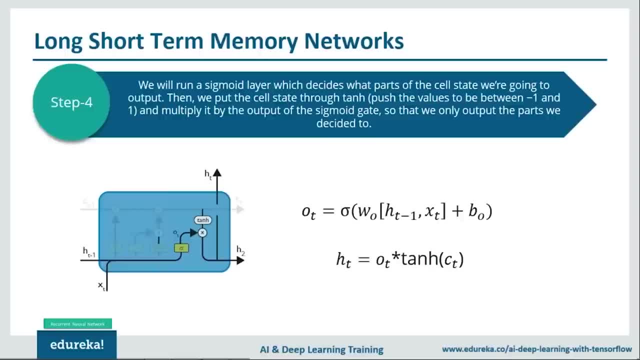 Now, in the fourth step, what we did? we finally got the output that we want. And how we did that? Just by passing ht minus one and xt through a sigmoid function, multiplying it with the tanh ct, the tanh new cell state. 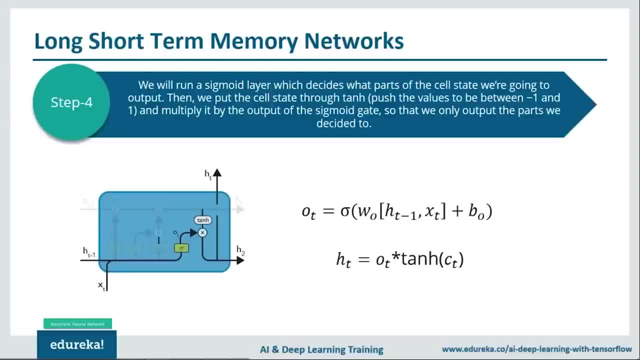 and we get the new output. Fine guys, That's basically LSTMs. guys. Now we'll look at a use case where we'll be using LSTM to predict the next word in a sentence. All right, let me show you how we are going to do that. 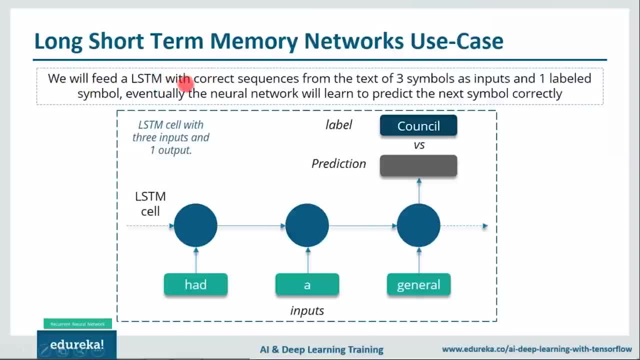 So this is what we are trying to do in our use case, guys. We'll feed our LSTM with correct sequences from the text of three symbols. For example, had a general and a label, that is, council in this particular example. Eventually, our network will learn to predict. 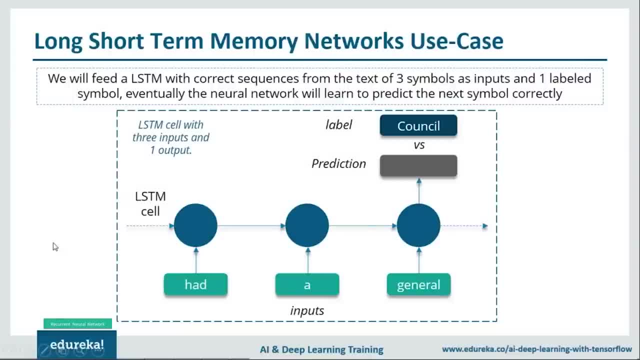 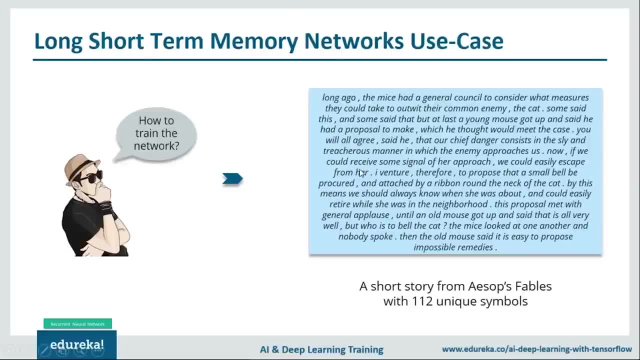 the next symbol correctly, So obviously we need to train it on something. Let us see what we are going to train it on. We'll be training our LSTM to predict the next word using a sample short story that you can see over here. All right, so it has basically 112 unique symbols. 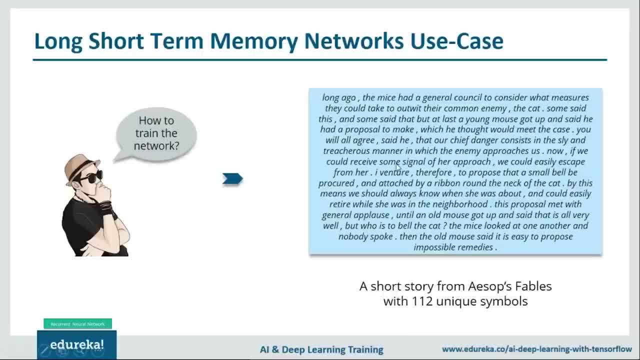 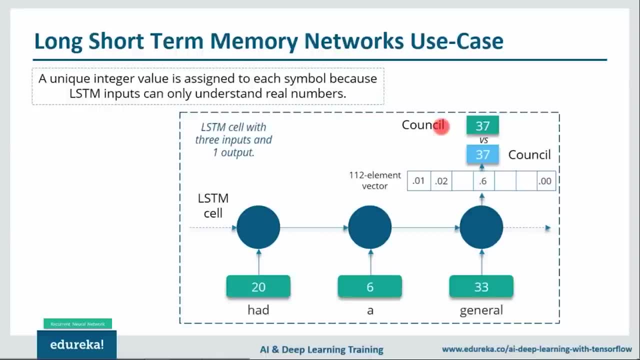 So even comma and full stop are considered as symbols. All right, so this is what we are going to train it on. So, technically, we know that LSTMs can only understand real numbers. all right, So what we need to do is we need to convert. 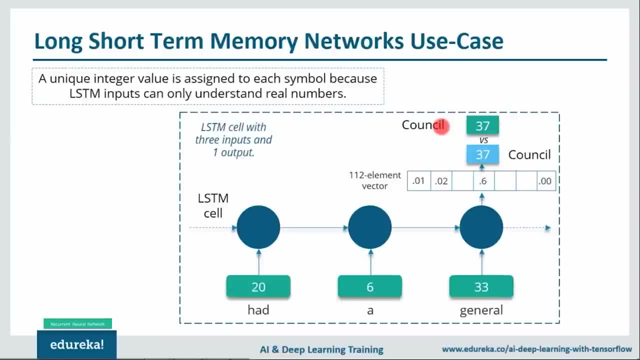 these unique symbols into a unique integer value based on the frequency of occurrence. And like that we'll create a dictionary. For example, we have had a dictionary that will have value 20.. A will have value six. general will have value 33.. 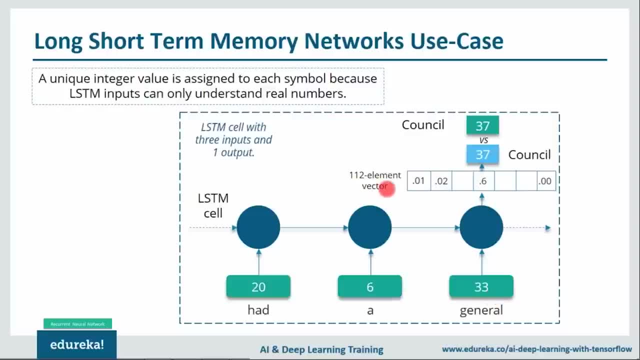 All right, and then what happens? our LSTM will create 112 element vector that will contain the probability of each of these words or each of these unique integer values. all right, So, since 0.6 has the highest probability in this particular vector, 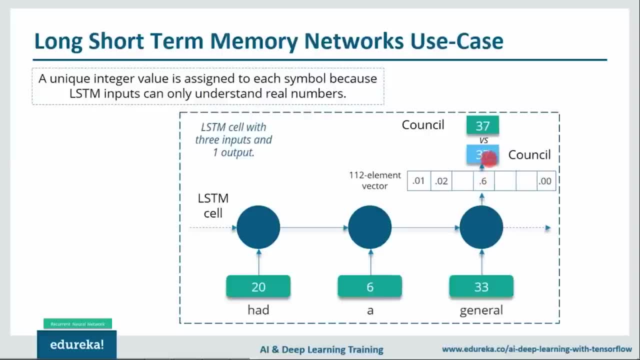 it will pick the index value of 0.6.. Then it will see what symbol is attached to that particular integer value. So 37 is attached to council. So this will be our prediction, which is absolutely correct, as a label is also council, according to our training data. 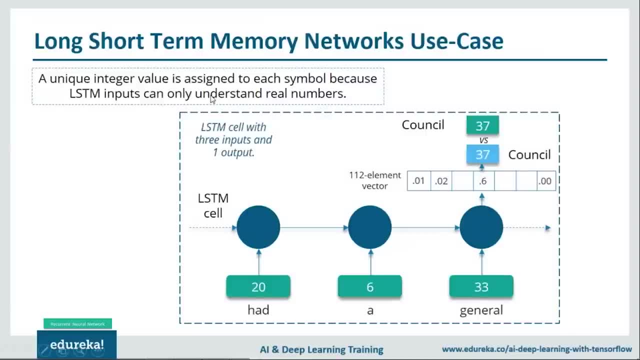 All right, so this is what we are going to do in our use case. So, guys, this is what we'll be doing in today's use case. Now I'll quickly open my PyCharm and I'll show you how you can implement it using Python. 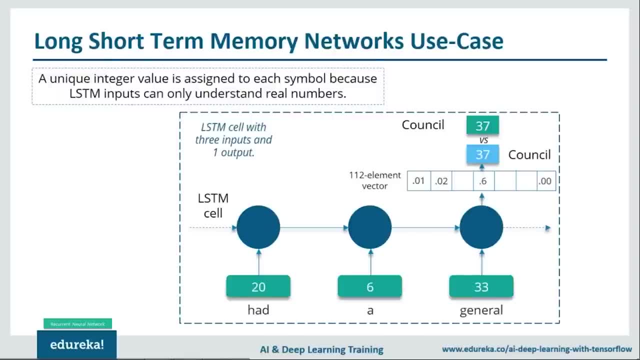 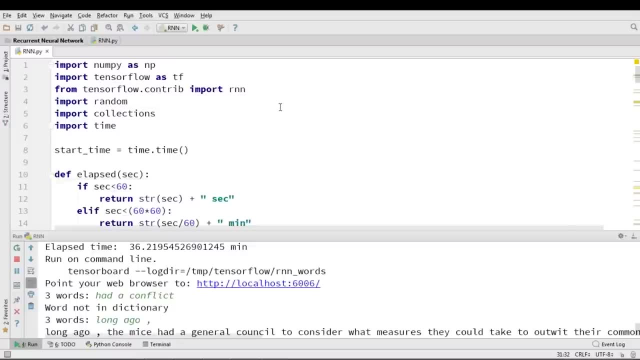 We'll be using TensorFlow, which is a popular Python library for implementing deep neural networks or neural networks in general. All right, so I'll quickly open my PyCharm now. So, guys, this is my PyCharm, and over here I've already written the code in order to execute. 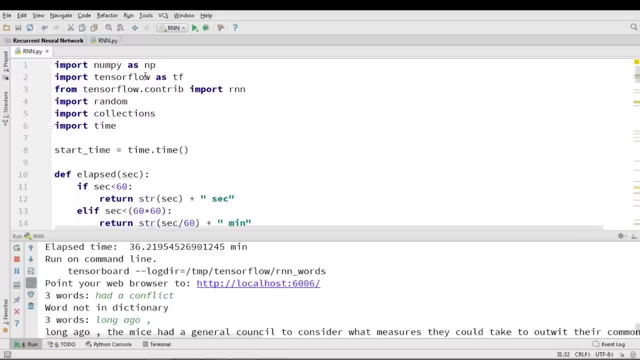 the use case that we have. So what we need to do is import the libraries NumPy, Ferraris, TensorFlow- we know TensorFlowcontra From that. we need to import RNN in random collections in time. All right, so this particular block of code. 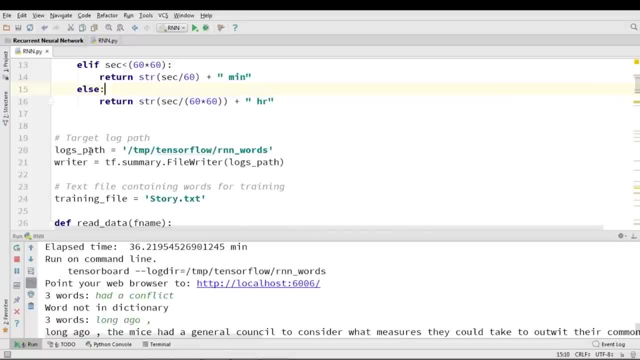 is used to evaluate the time taken for the training. After that, we have log underscore path, and this log underscore path is basically telling us the path where the graph will be stored. All right, so there will be a graph that will be created, and then that graph will be launched. 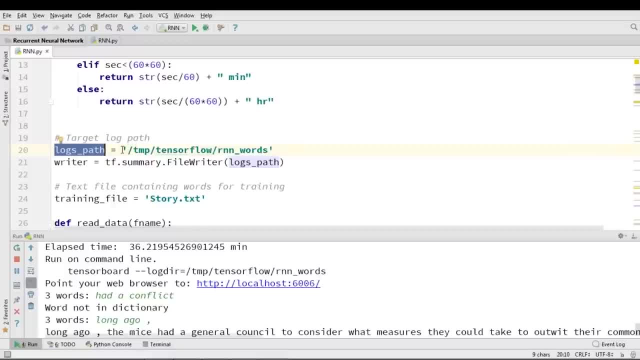 Then only our RNN model will be executed. Then that's how TensorFlow works, guys. All right, so that's how we're going to do it. All right, so that's how we're going to do it. So we're going to do it in this particular path. 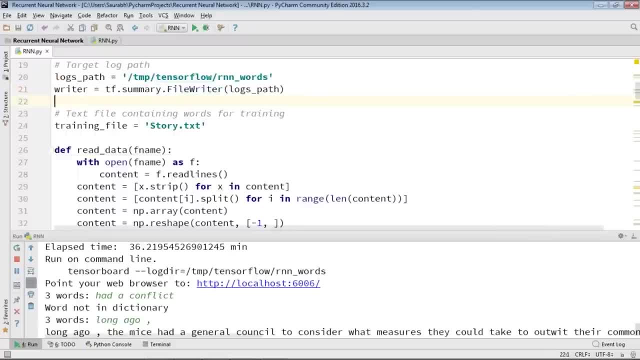 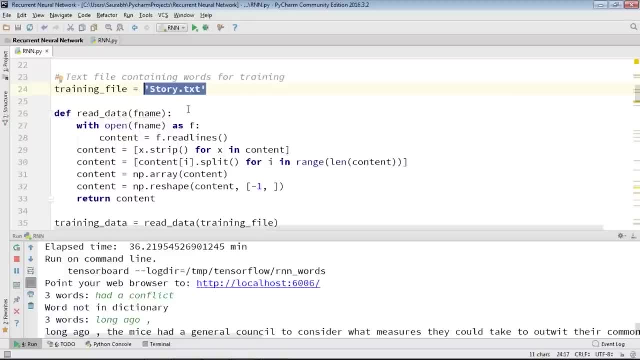 All right, and we are using summary writer, So that will actually create the log file that will be used in order to display the graph using TensorFlow. All right, so then we have defined training underscore file, which will have our story, on which we'll train our model on. 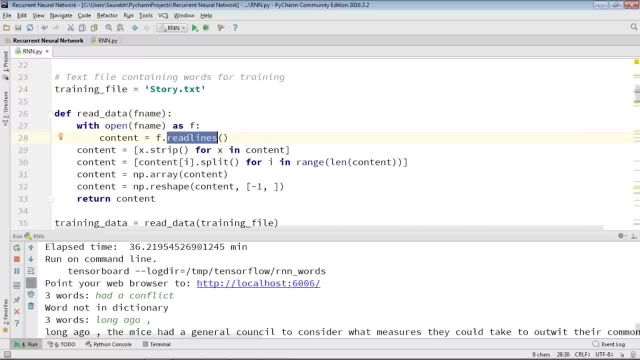 Then what we need to do is read this file. So how are we going to do that? First is read line by line whatever content that we have in our file. Then we are going to strip it. That means we are going to remove the first and the last white space. 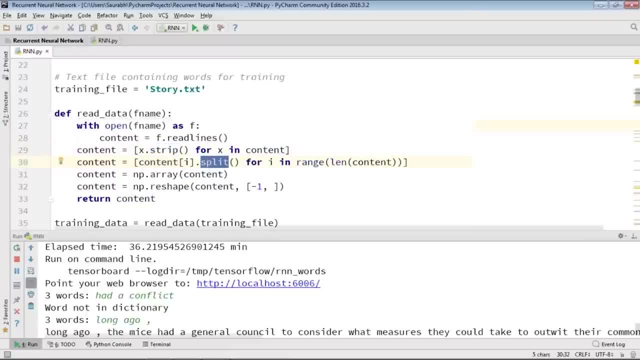 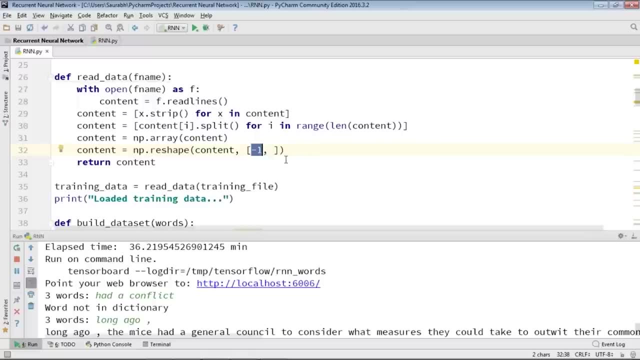 We are splitting it just to remove all the white spaces that are there. After that, we're creating an array and then we are reshaping it. Now, during the reshape, if you notice this minus one value tells us the compatibility. All right, so when you're reshaping it, 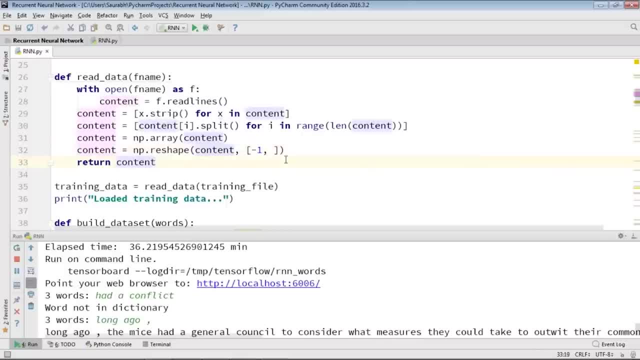 you need to make sure that we are providing in the correct parameters to reshape it So you can convert a three cross two matrix to a two cross three matrix, right? So just to make sure that it is compatible enough, we add this minus one and it'll be done automatically. 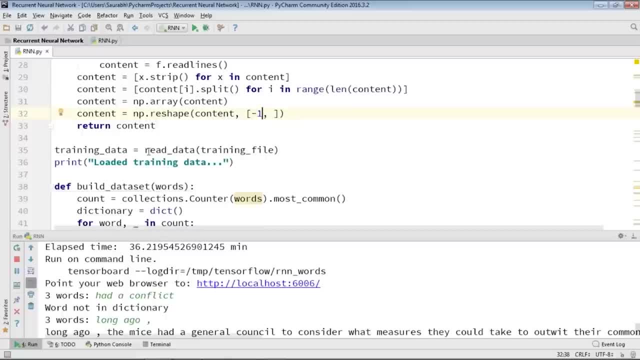 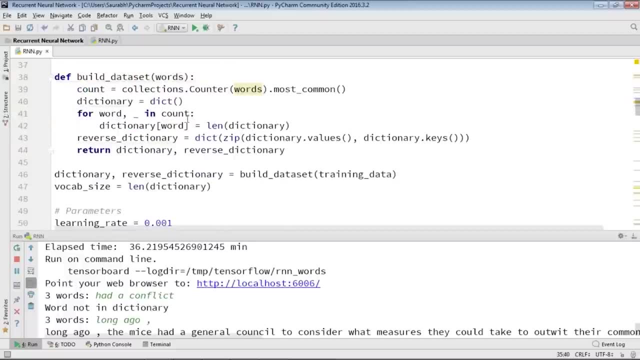 All right, then return content. After that, what we are doing, we are feeding in the training data that we have training underscore file. We are feeding in our story and calling the function: read underscore data. Then what we are doing: we are creating a dictionary. 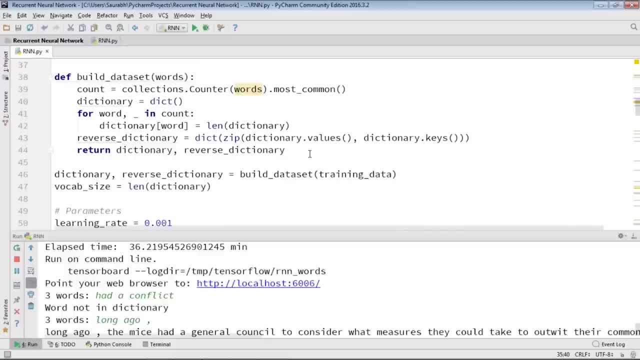 What is a dictionary? We all know key value pairs based on the frequency of occurrences of each symbol. All right, so from here, collectionscounterwordsmostcommon, So most common words with their frequency of occurrence, there'll be a dictionary created. 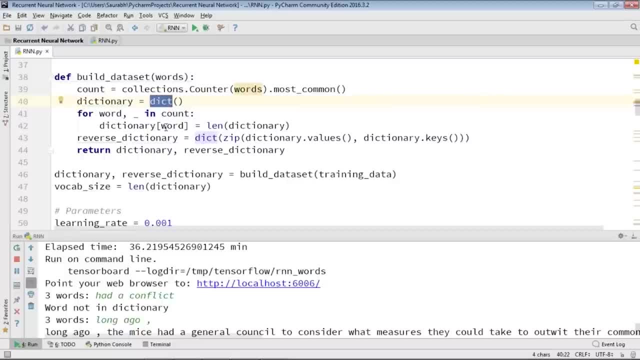 And after that we'll call this dict function And this dict function will feed in word, and which is equal to the number of words, equal to length of dictionary. That means whatever the length of that particular dictionary is, how many time it is repeated. 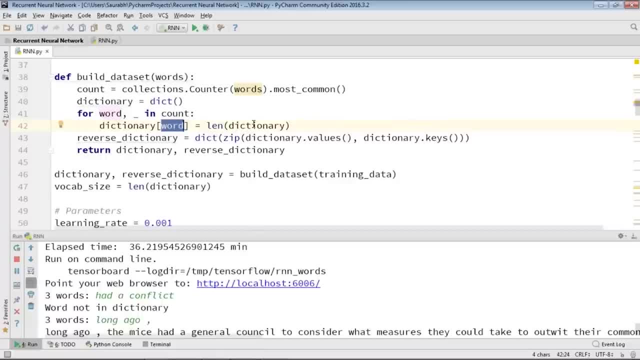 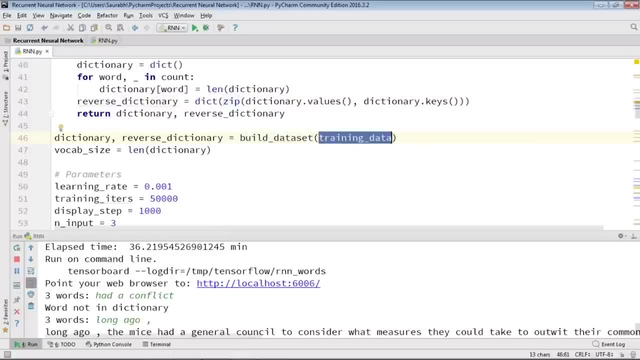 So we'll have the frequency as well as a symbol. that will be our key value pair, and we are reversing it as well. Then what we are doing? we are calling it build underscore data set and we're feeding in our training data there. This is our vocabulary size. 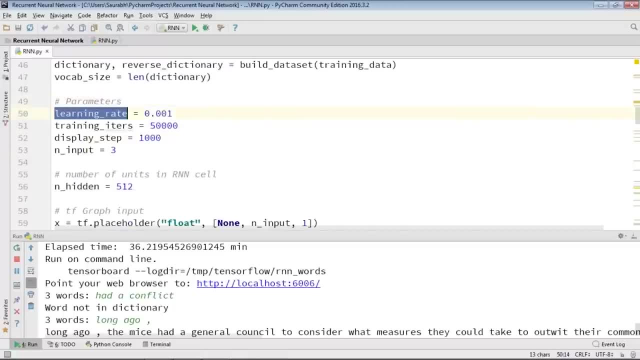 which is nothing but the length of your dictionary. Then we have defined various parameters, such as learning rate, iterations or epochs. Then we have display, step and underscore input. Now, learning rate. we all know what it is, The steps in which our variables are updated. 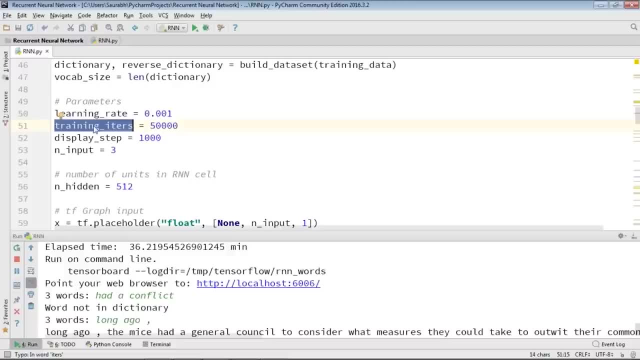 Training. underscore iterations is nothing but your epochs, the total number of iterations. So we have given 50,000 iterations here. Then we have display underscore step. that is thousand, which is basically your batch size. So batch size is what? After every thousand epochs you'll see the output. 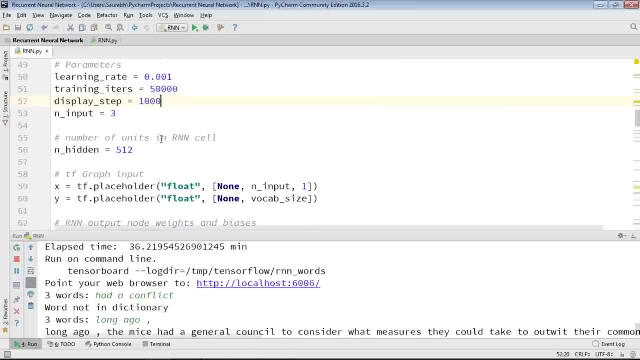 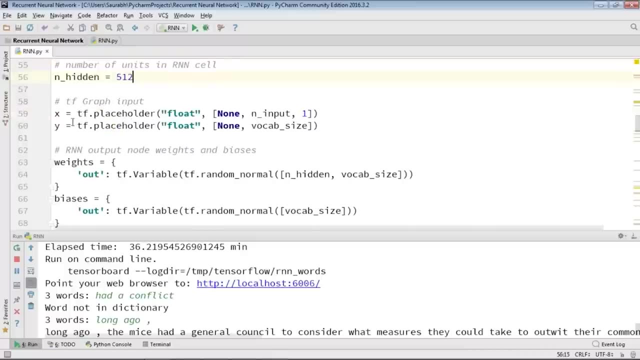 All right, so it'll be processing it in batches of thousand iterations. Then we have n underscore input as three. Now the number of units in the RNN cell will keep it as 512.. Then we need to define x and y, So x will be our placeholder. 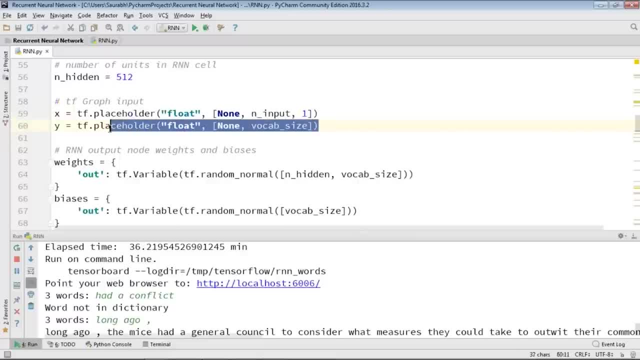 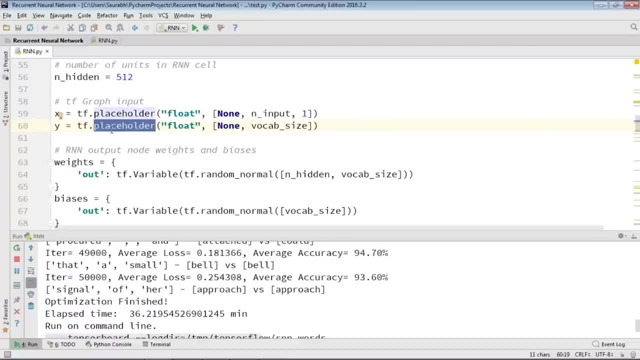 That will have the input values And y will have all the labels. all right. vocab size. So x is a placeholder where we'll be feeding in our input dictionary. Similarly, y is also one word placeholder And it'll have a shape of none comma. vocab size. 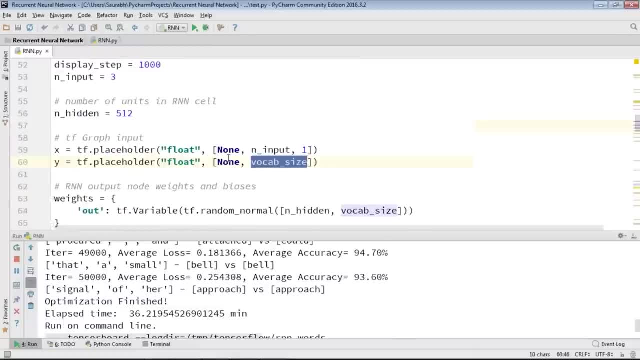 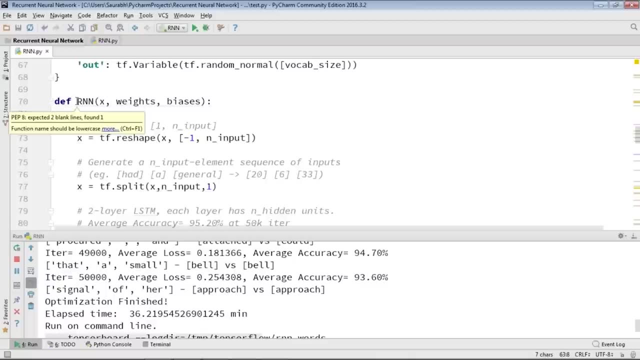 Vocab size we have defined earlier, as you can see, which is nothing but the length of your dictionary. Then we are defining weights as well as biases. After that, we have defined our model, All right, so this is how we are going to define it. 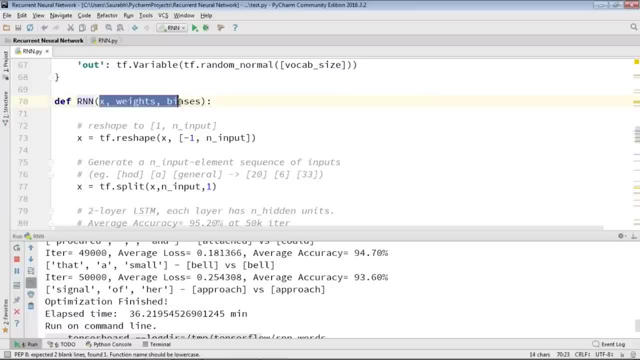 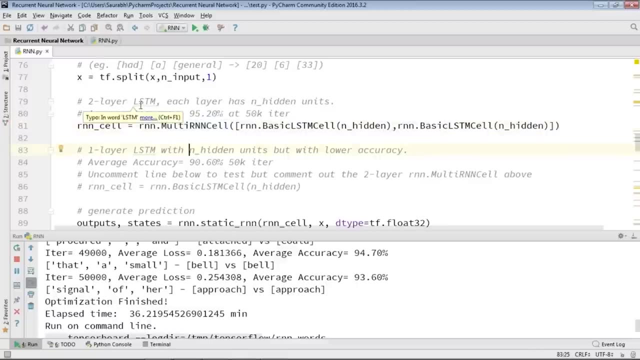 We'll create a function RNN, then we'll have x, weights and biases And after that we are calling in RNN, dot, multi, RNN, cell function. And this is basically to create a two-layer LSTM And each layer has n underscore- hidden units. 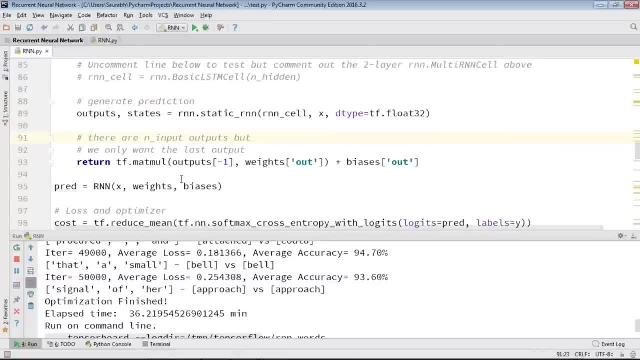 After that, what we are doing? we are generating the predictions. But once we have generated the prediction, there are n underscore input outputs, but we only want the last output, all right, So for that we have written this particular line. 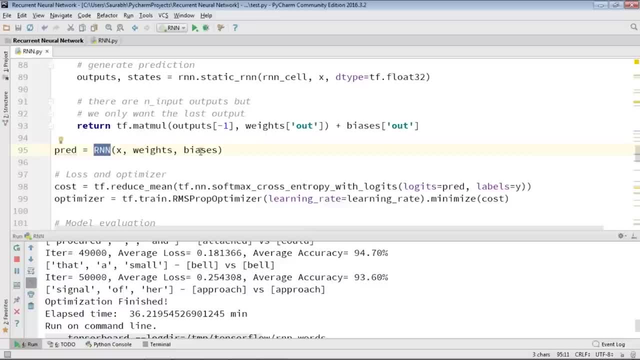 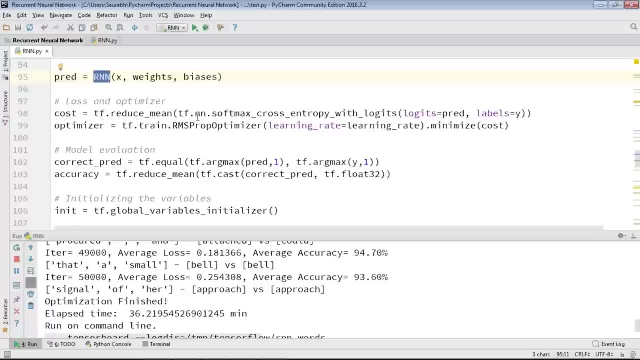 And then, finally, we are making a prediction. We are calling this RNN function, feeding in x weights and biases. After that, we are calculating the loss, we are optimizing it. For calculating the loss, we are using: reduce, underscore, mean, softmax, cross entropy. 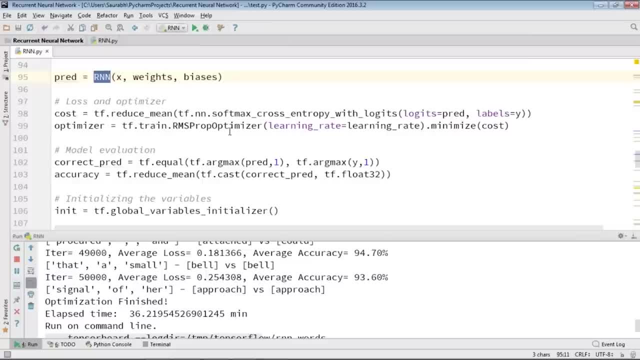 And this will give us basically the probability of each symbol. and then we are optimizing it using RMS prop optimizer. all right, And this gives actually a better accuracy than Adam optimizer, and that's the reason why we are using it. Then we are going to calculate the accuracy. 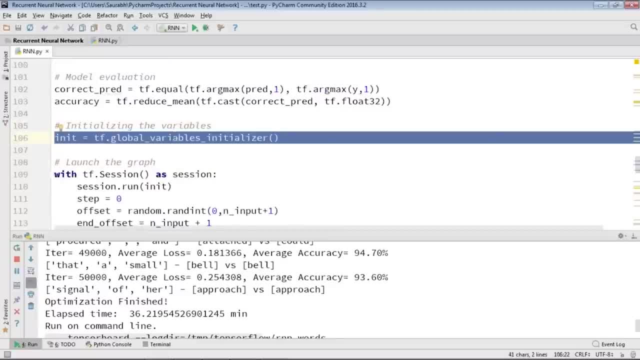 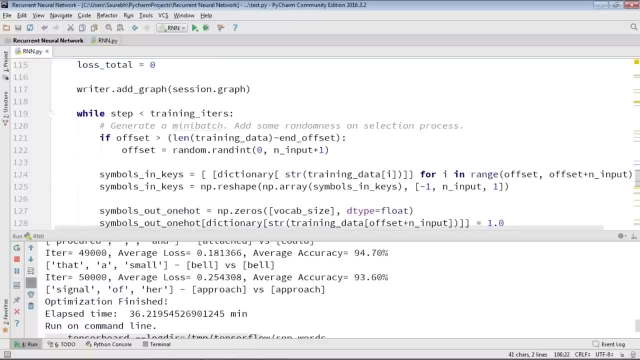 And after that we are going to initialize the variables that we have used, As we have seen in TensorFlow that we need to initialize all the variables, unlike constants and placeholders in TensorFlow, All right, And once we are done with that, we are feeding in our values. 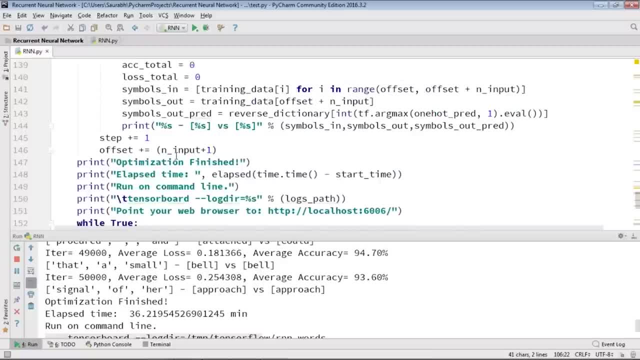 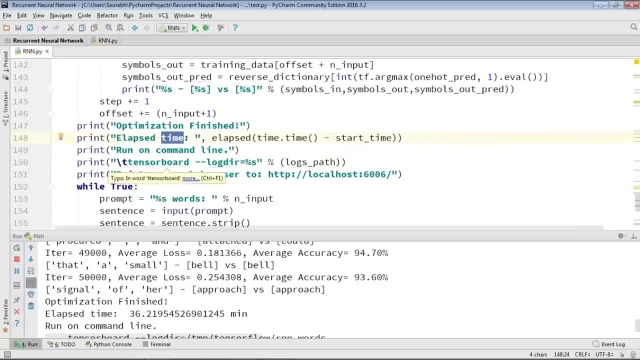 then calculating the accuracy, how accurate it is, And then, when optimization is done, we are calculating the elapsed time as well, So that will give us how much time it took in order to train our model. Then this is just to run the tensor board. 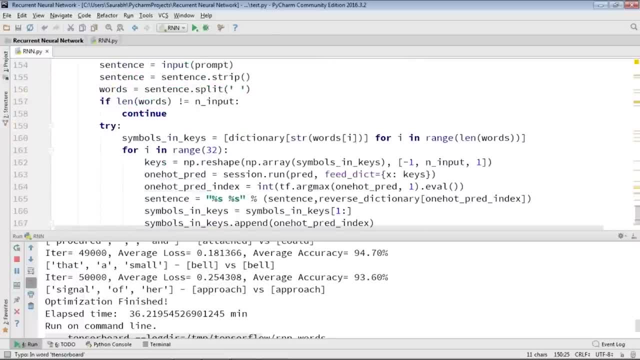 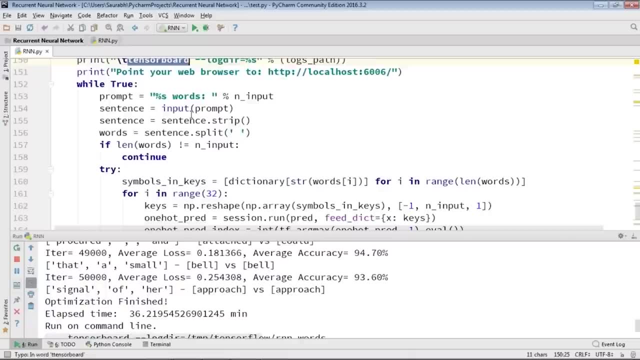 on local host 6006.. And yeah, and this particular block of code is used in order to handle the exceptions, So exceptions can be like whatever word that we are putting in might not be there in our dictionary or might not be there in our training. 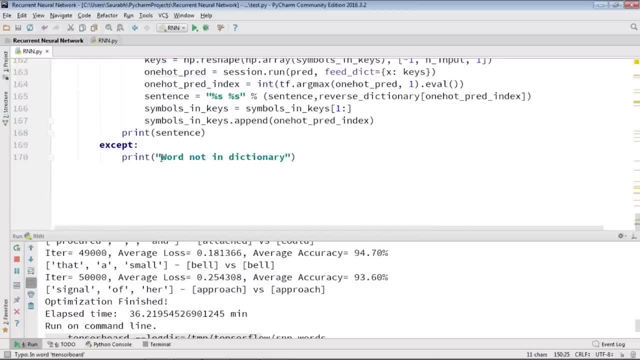 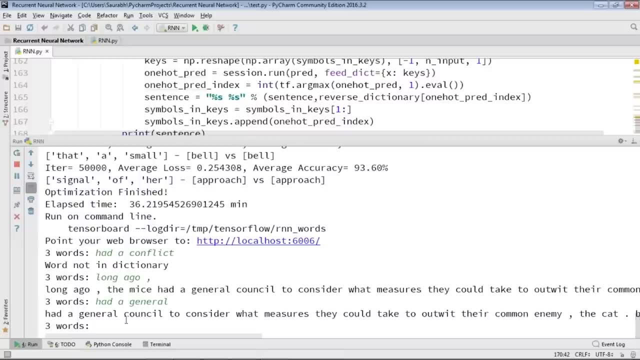 So those exceptions will be handled here, And if it is not there in our dictionary, then it will print word not in our dictionary, All right. So, fine guys, let's input some values and we'll have some fun with this model, All right? 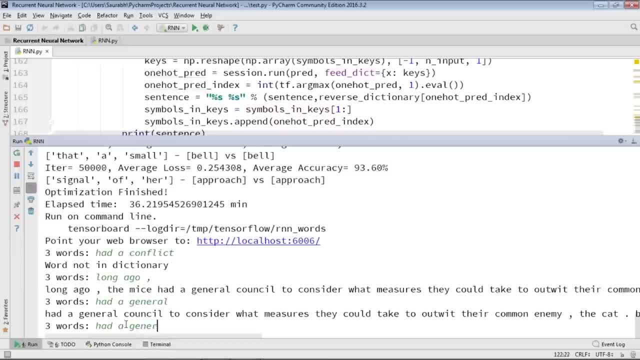 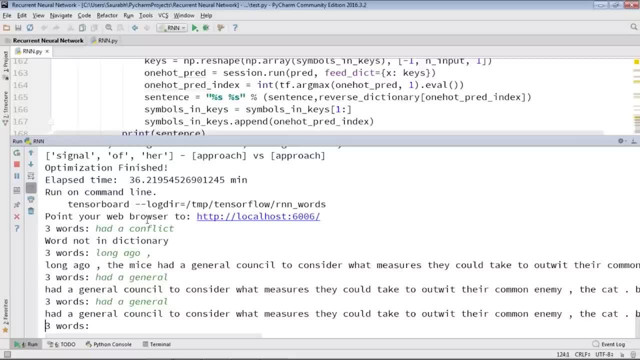 So the first thing that I'm gonna feed in is had a general. So whenever I feed in these three values had a general, there will be a story that will be generated by feeding back the predicted output as the next symbol in the inputs. 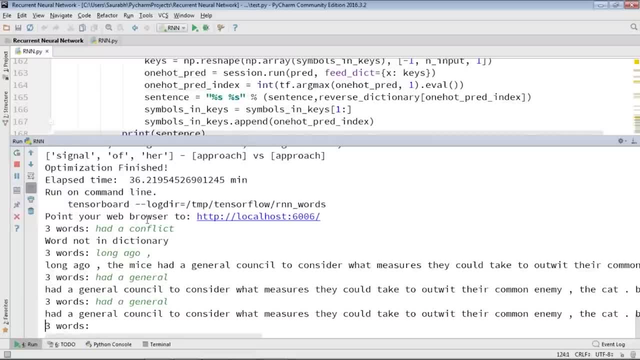 All right. So when I feed in, had a general, so it will predict the correct output of this council And this council will be fed back as a part of the new input and our new input will be a general council, So it will be a general council. 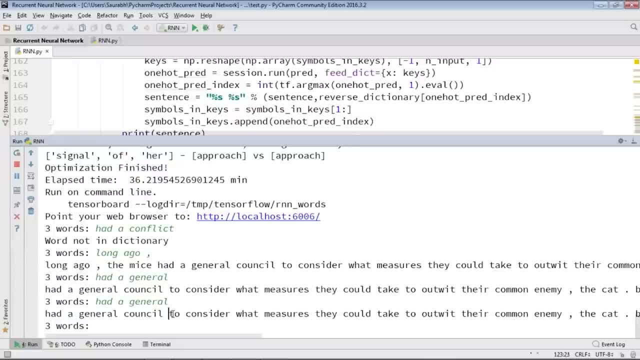 All right. So these three words will become a new input to predict the new output, which is two All right And so on. So, surprisingly, LSTM actually creates a story that somehow makes sense. So let's just read. it Had a general council to consider what measures. 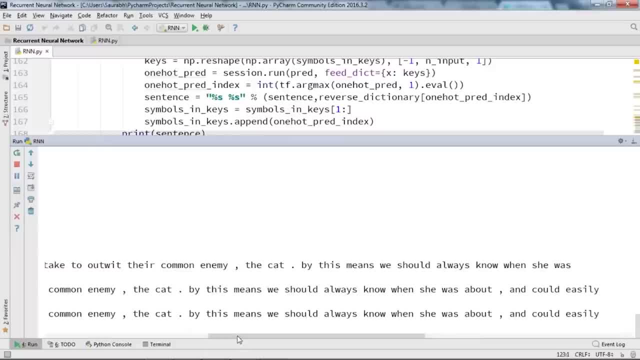 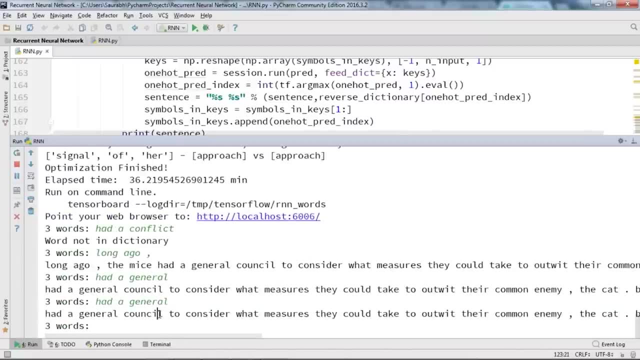 they could take to outwit their common enemy, the cat. By this means we should always know when she was about and could easily All right, So somehow it actually makes sense when you feed in that. So what'll happen when you feed in these three inputs? 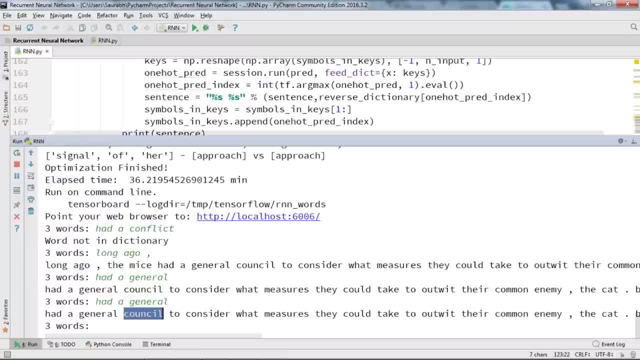 it'll predict the next word, that is, council. After that it will take council and it will feed back as an input along with a general. So a general council will be your next input to predict two. Similarly, in the next iteration it will take general council two. 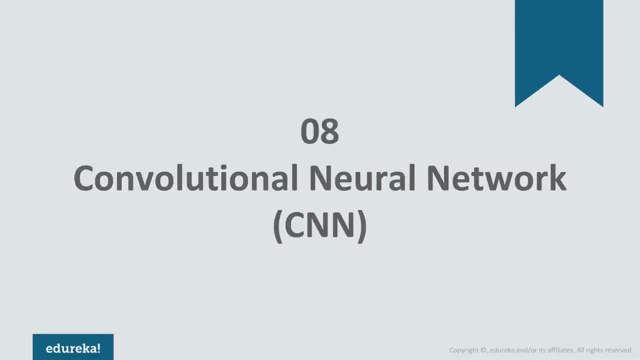 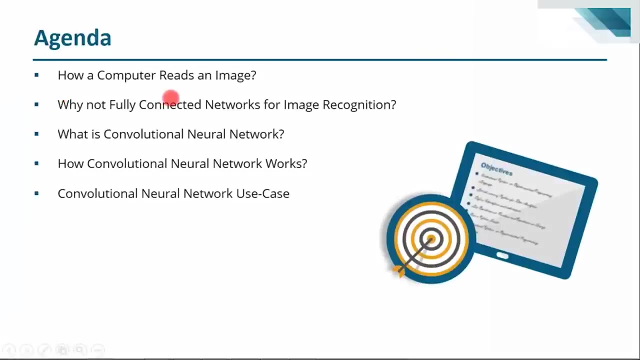 and predict, consider for us, And this will keep on repeating. Today we'll be discussing about convolutional neural networks. So, without any further ado, let us move forward and have a look at the agenda for today. So we'll begin by understanding how a computer reads an image. 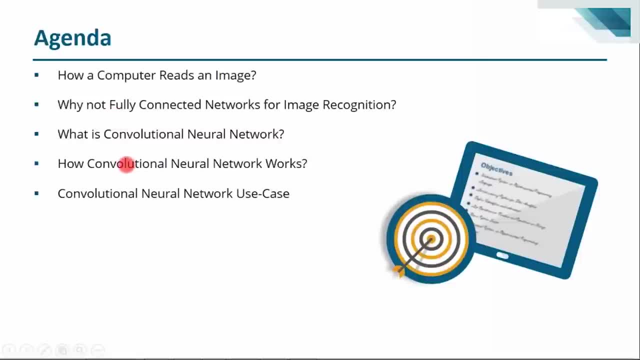 Then we'll see why can't we use fully connected networks for image recognition. After that we'll understand what exactly is convolutional neural network and how it works, And finally we'll be looking at a use case. So let's begin, guys. 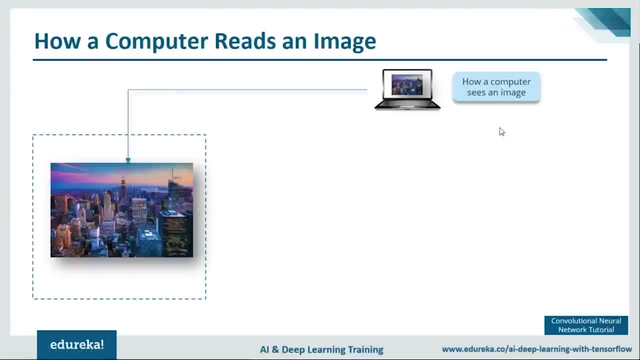 We'll understand how exactly a computer reads an image. So this is an image of New York skyline. I personally love this picture. So when a human will see this image he'll first notice there are a lot of buildings in different colors and stuff like that. 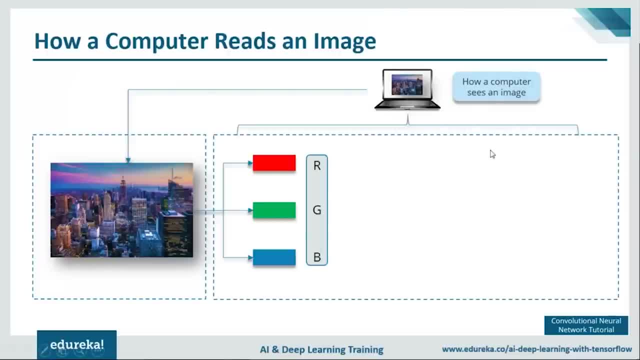 But how a computer will read this image. So basically, there'll be three channels: One will be red, another will be green and finally we have blue channel, which is popularly known as RGB. So each of these channels will have: 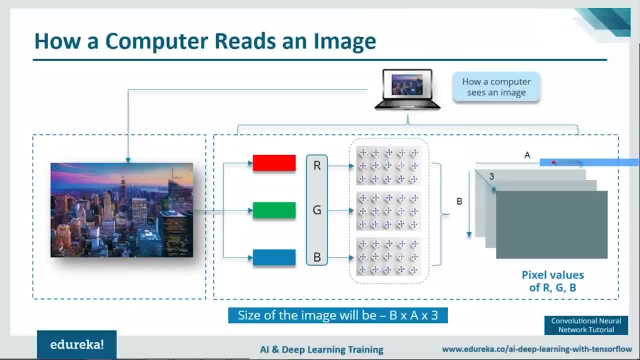 their own respective pixel values, as you can see it over here. So when I say that image size is B cross A cross three, it means that there are B rows, A columns and three channels. all right, So if somebody tells you that the size of an image 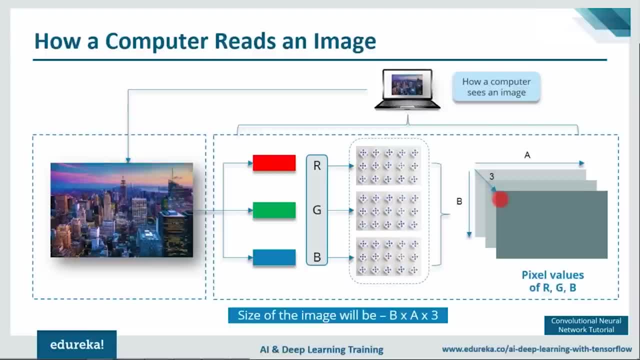 is 28 cross, 28 cross, three pixels. it means that it has 28 rows, 28 columns, 28 pixels. It means that it has 28 columns and three channels. So this is how a computer sees an image, And this is for colored images. 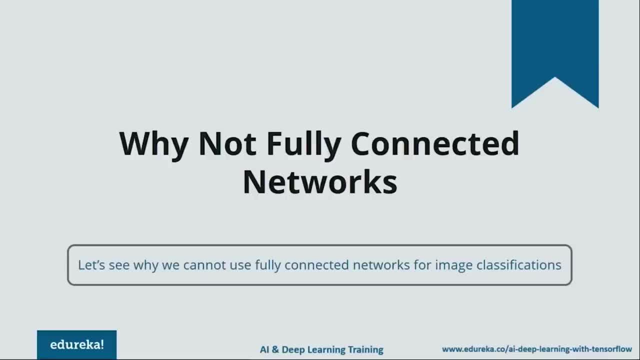 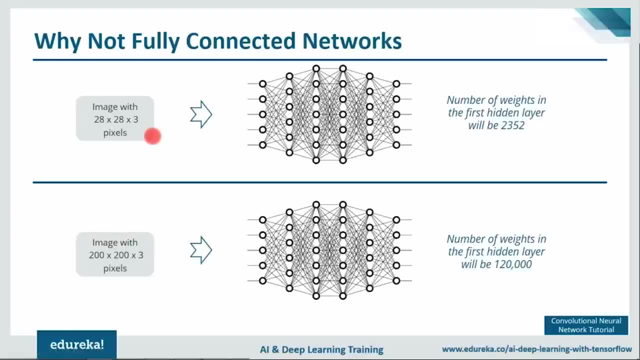 For black and white images we have only two channels. So let's move forward and we'll see. why can't we use fully connected networks for image classification? So consider an image which has 28 cross, 28 cross three pixels. So when I feed in this image, 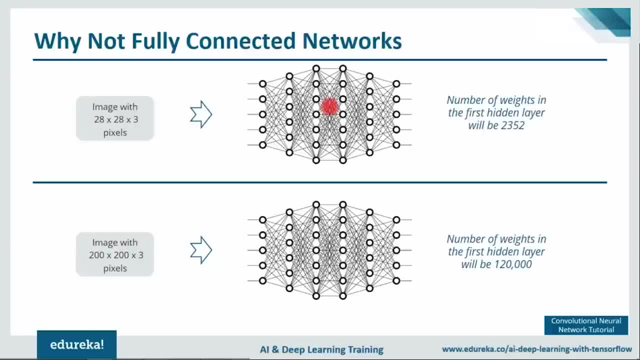 to a fully connected network like this, then the total number of weights required in the first hidden layer will be 2,352.. You can just go ahead and multiply it yourself, all right, But in real life the images are not that small, all right. 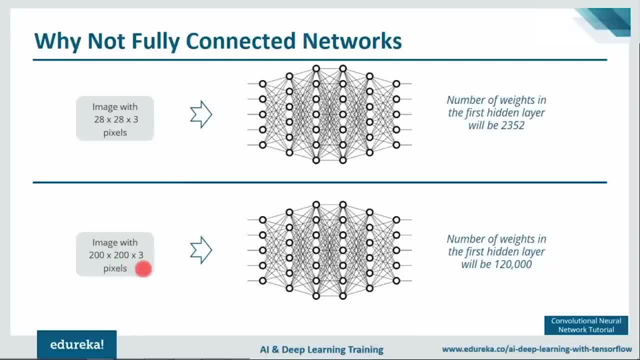 So whatever images that we have, they are definitely above 200 cross, 200 cross three pixels. So if I take an image which has 200 cross 200 cross three pixels and I feed it to a fully connected network, so at that time the number of weights required 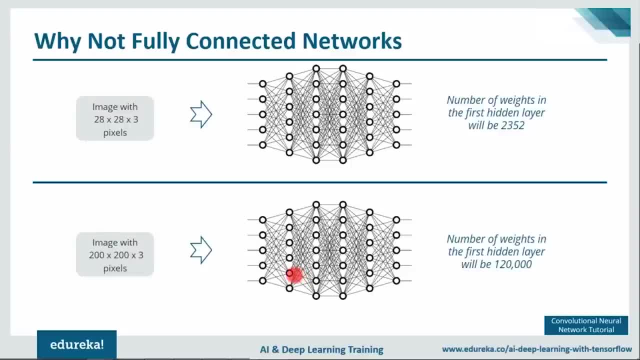 at the first hidden layer itself will be 120,000, guys. So we need to deal with such huge amount of parameters and obviously require more number of neurons, So that can eventually lead to overfitting. So that's why we cannot use fully connected network. 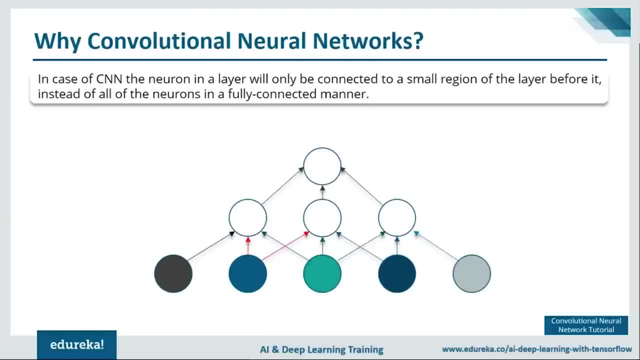 for image classification. Now let's see why we need convolutional neural networks. So basically, in convolutional neural network, the neuron in the layer will only be connected to a small region of the layer before it. So if you consider this particular neuron, 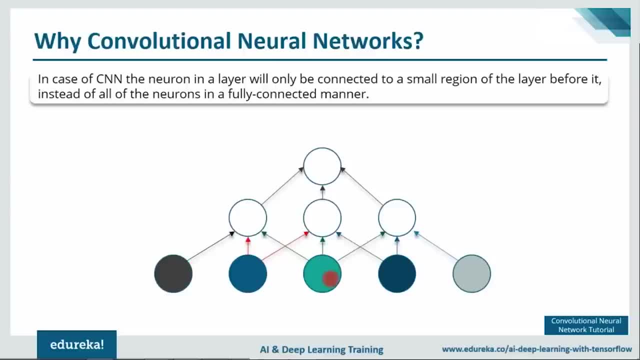 which I'm highlighting right now, is only connected to three other neurons, Unlike the fully connected network, where this particular neuron will be connected to all these five neurons. Because of this, we need to handle less amount of weights and, in turn, we need less number of neurons as well. 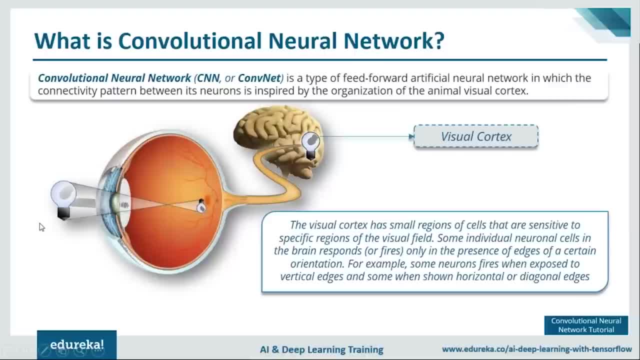 So let us understand what exactly is convolutional neural network? So convolutional neural networks are special type of feed forward, artificial neural networks, which is inspired from visual cortex. So visual cortex is nothing but a small region in our brain, Brain, which is present somewhere here. 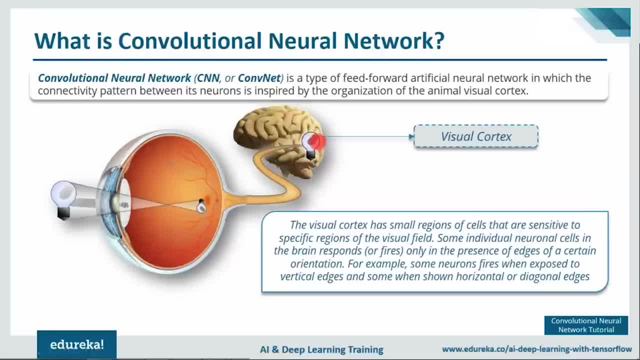 where you can see the bulb, And basically what happened. there was an experiment conducted and people got to know that visual cortex is small regions of cells that are sensitive to specific regions of visual field. So what I mean by that is, for example, 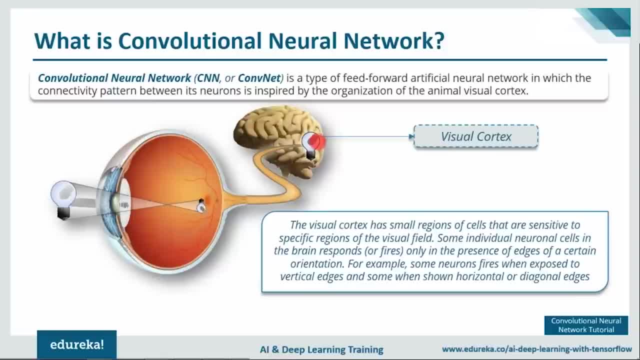 some neurons in the visual cortex fires when exposed to vertical edges, Some will fire when exposed to horizontal edges, Some will fire when exposed to diagonal edges, And that is nothing but the motivation behind convolutional neural network. So now let us understand how exactly a convolutional neural network works. 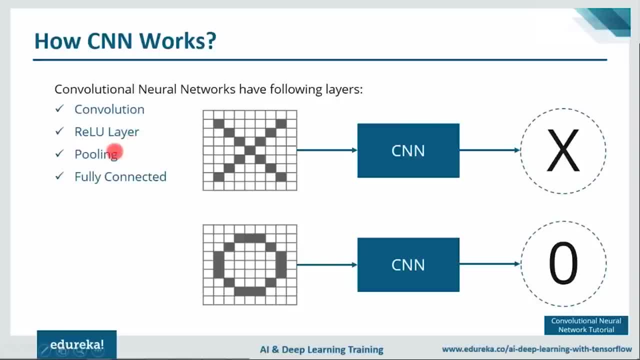 So, generally, a convolutional neural network has three layers: convolutional layer, ReLU layer, pooling layer and fully connected layer. We'll understand each of these layers one by one. We'll take an example of a classifier that can classify an image of an X as well as an O. 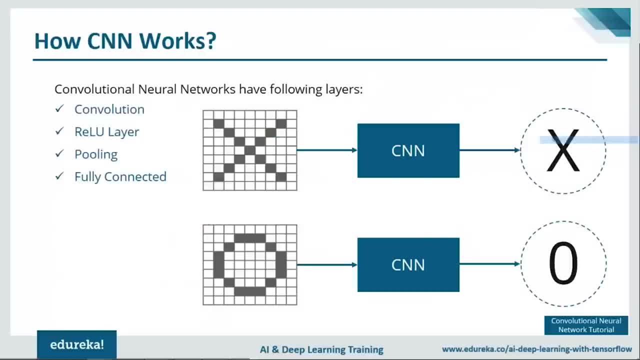 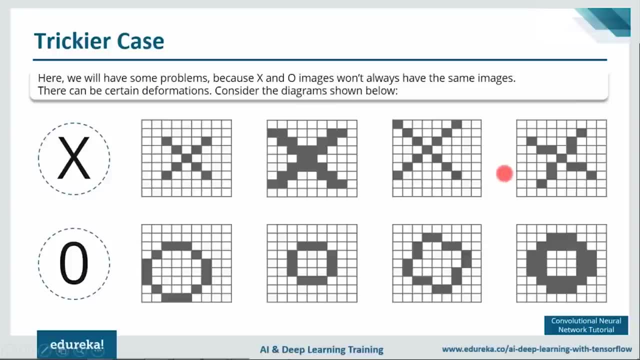 So with this example, we'll be understanding all these four layers. So let's begin, guys. Now there are certain trickier cases. So what I mean by that is X can be represented in these four forms as well. right? So these are nothing but the deformed images of X. 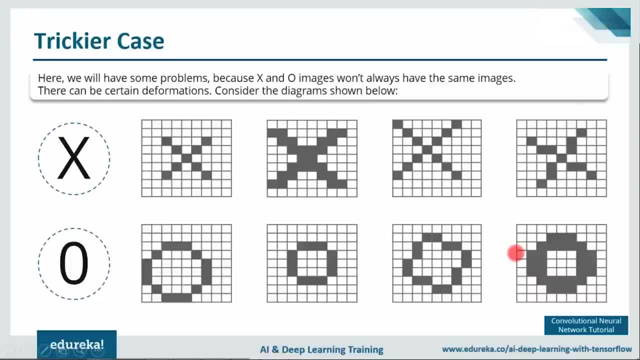 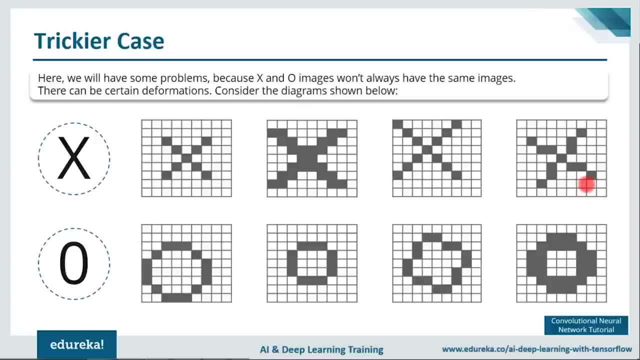 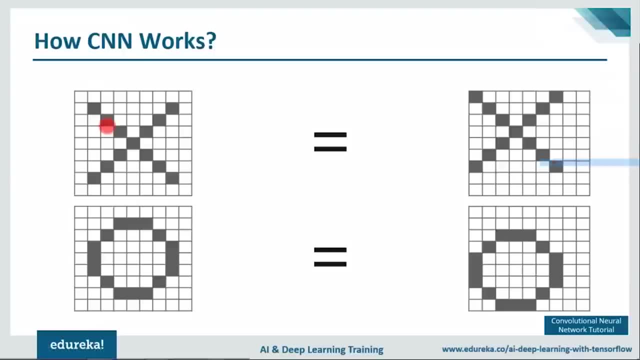 But all these are deformed images, But they are in turn, X, right? So I want my classifier to classify them as X. So, basically, that's what I want. So, if you can notice, here, this is a proper image of an X. 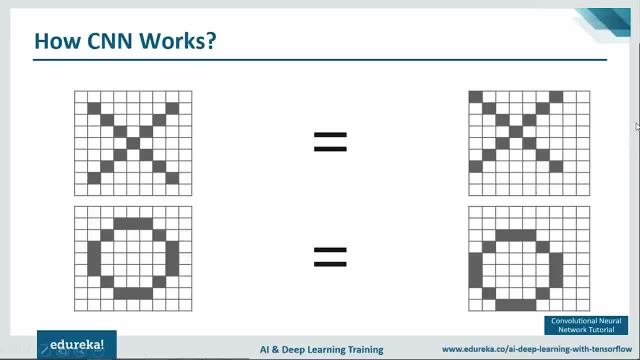 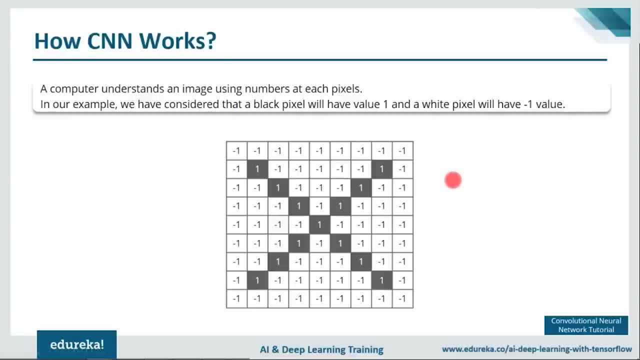 and which is actually equal to this particular X, which is a deformed image. Same goes for this O as well. So now what we are going to do is we know that a computer understands an image using numbers at each pixels. So what we'll do, 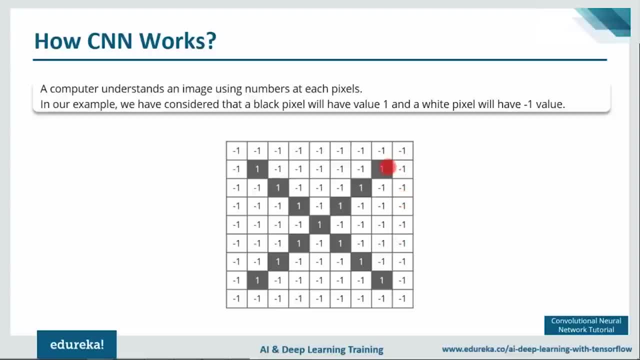 whatever the white pixels that we have, we are going to assign a value minus one to it, And whatever black pixels we have, we are going to assign a value one to it. When we use normal techniques to compare these two images, one is a proper image of X. 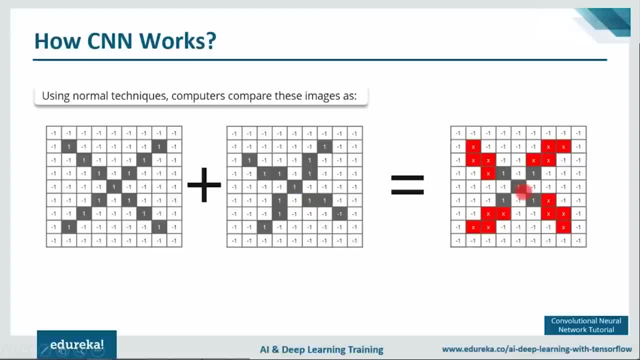 and another is a deformed image of X. we got to know that a computer is not able to classify the deformed image of X correctly. Why? Because it is comparing it with the proper image of X, right? So when you go ahead and add the pixel values, 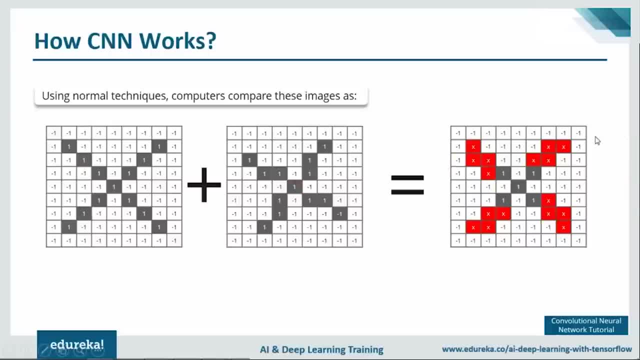 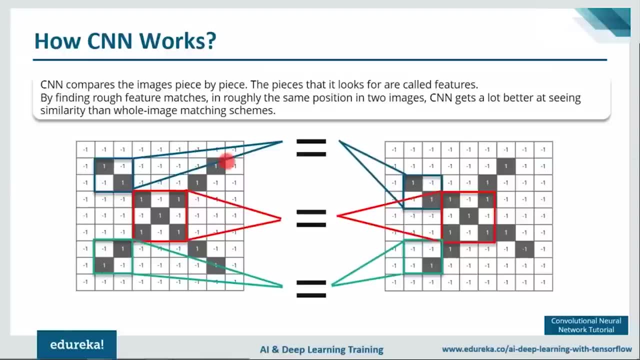 of both of these images, you get something like this: So, basically, our computer is not able to recognize whether it is an X or not. Now what we do with the help of CNN, we take small patches of our image. So these patches- 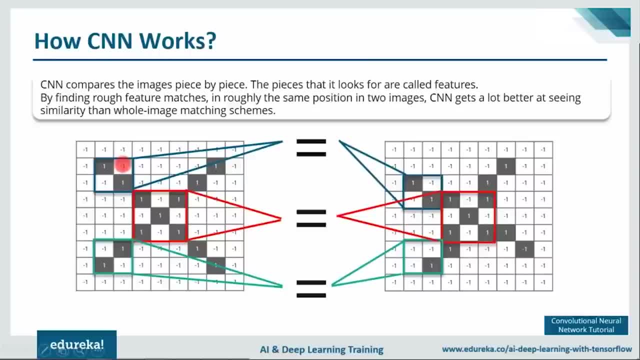 or these pieces are known as nothing but features or filters. So what we do? by finding rough feature matches in roughly the same positions in two images. CNN gets a lot better at seeing the similarity between the whole image matching schemes. What I mean by that is: 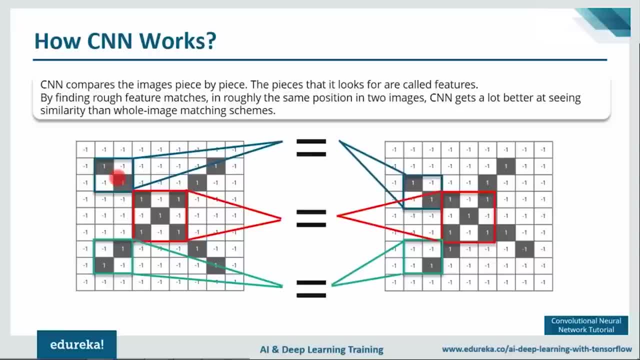 we have these filters, right, We have these filters that you can see. So consider this first filter. This is exactly equal to the feature or the part of the image in the deformed image as well. So this is our proper image and this is our deformed image, all right. 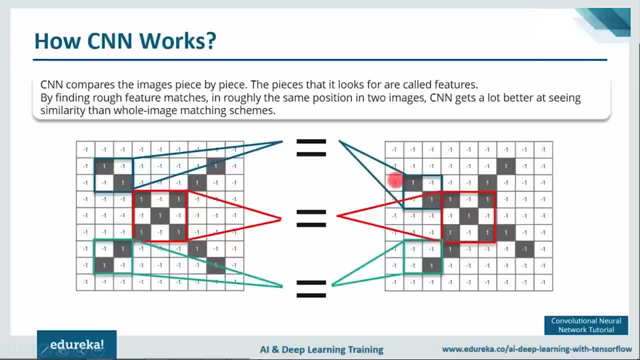 So this particular feature or this particular part of the image is actually equal to this particular part of the image. Same goes for this particular feature or filter as well, And similarly we have this filter as well, which is actually equal to this particular part. 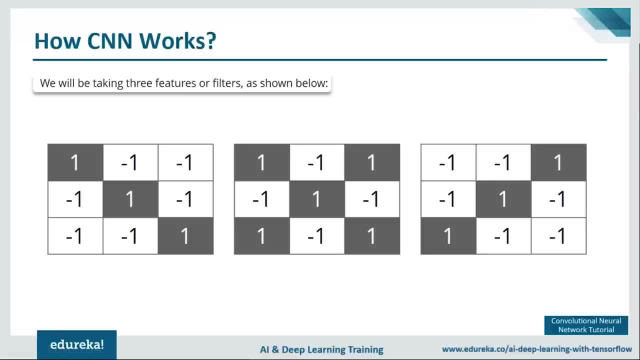 of the deformed image. all right, So let's move forward and we'll see what all features that we'll be taking in our example. So we'll be considering these three features, or filters. This is a diagonal filter. This is, again, a diagonal filter. 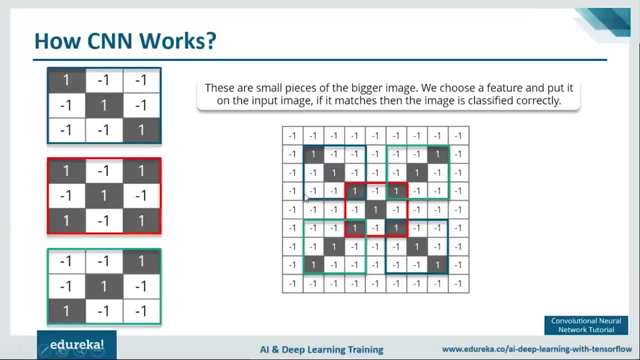 and this is nothing but a small X. So we'll take these three filters and we'll move forward. So what we are going to do is we are going to compare these features, the small pieces of the bigger image We are going to put it. 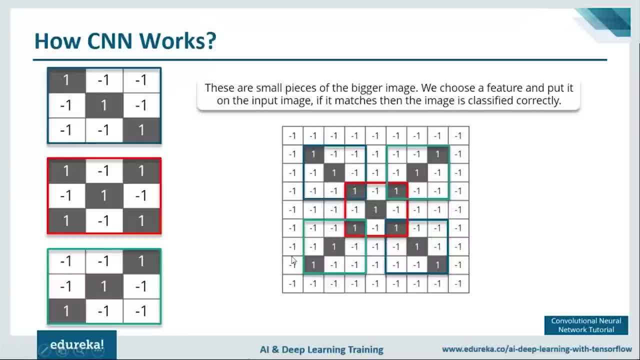 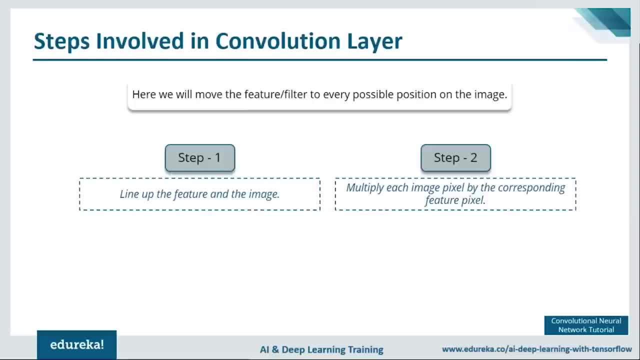 on the input image and if it matches, then the image will be classified correctly. Now we'll begin, guys. The first layer is convolution layer. So these are the beginning two steps of this particular layer. First, we need to line up the feature in the image. 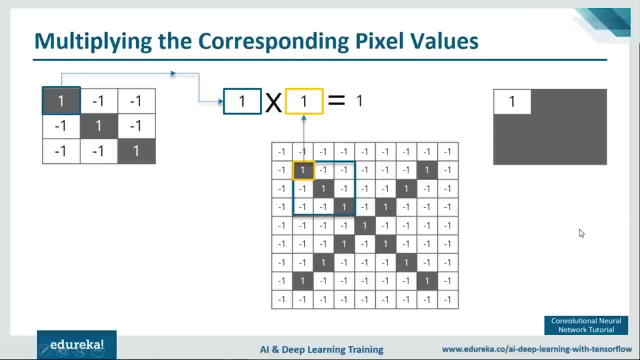 and then multiply image by the corresponding feature pixel. Now let me explain you with an example. So this is our first diagonal feature that we'll take. We are going to put this particular feature on our image of X, all right, And we are going to multiply. 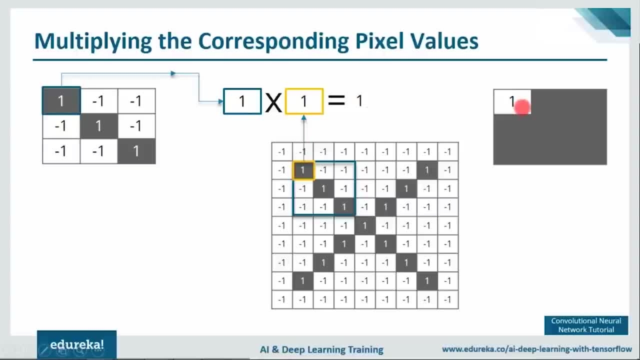 the corresponding pixel value. So one will be multiplied with one, we'll get one and we'll put it in another matrix. Similarly, we're going to move forward and we're going to multiply minus one with minus one. We're going to multiply minus one with minus one. 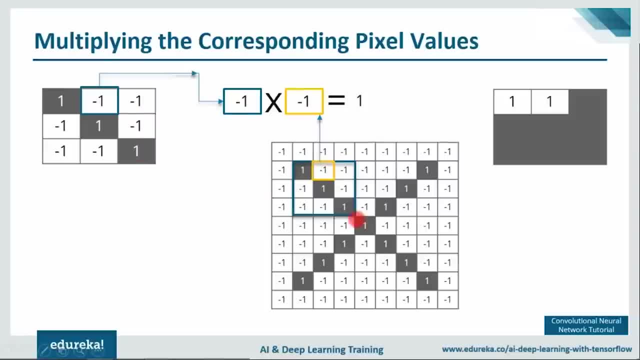 as you can see. Similarly, we multiply this result minus one into minus one, then again minus one into minus one. So we are going to complete this whole process when we are going to finish up this matrix, all right, And once we are done finishing up the multiplication, 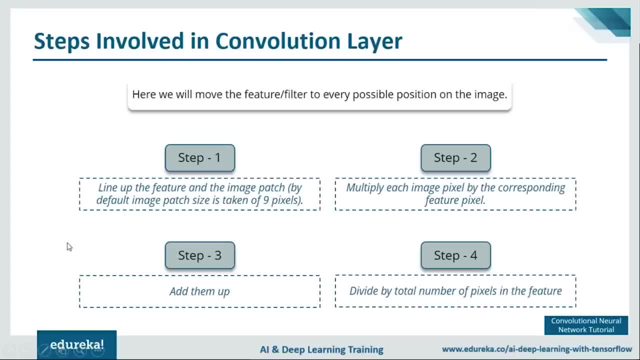 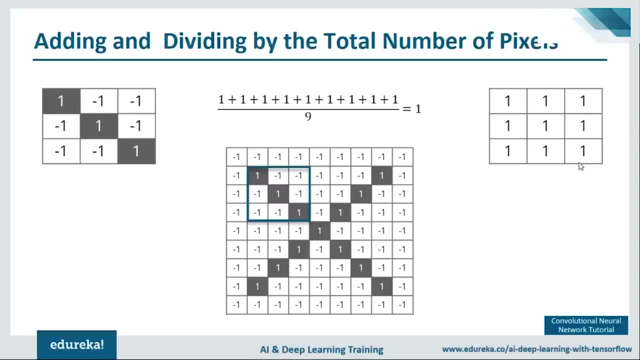 of all the corresponding pixels in the feature as well as in the image. we need to follow two more steps. We need to add them up and divide by the total number of the pixels in the feature. So what I mean by that is after the multiplication of the corresponding pixel values. 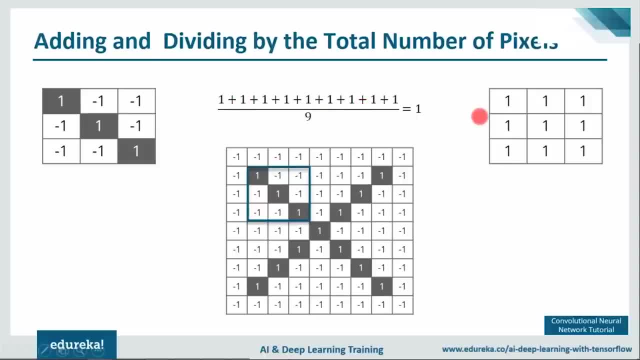 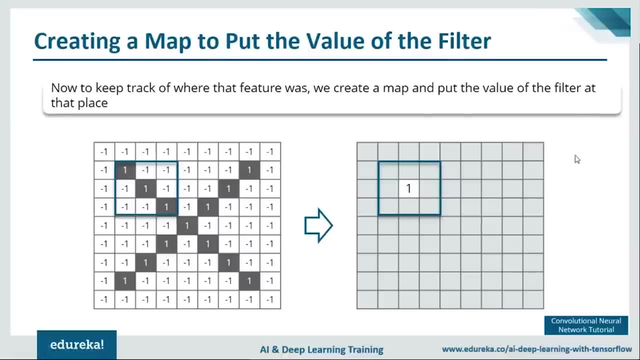 what we do. we add all these values, we divide it by the total number of pixels and we get some value right. And then now our next step is to create a map and put the value of the filter at that particular place. 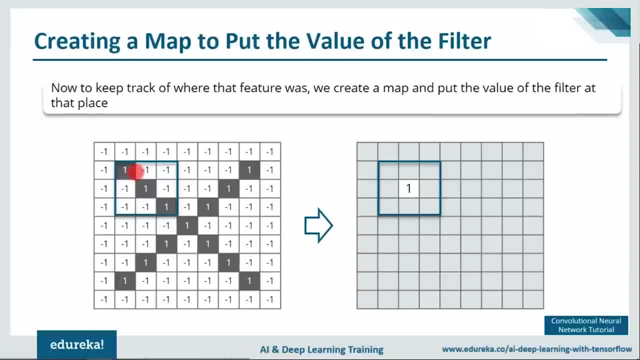 We saw that after multiplying the pixel value of a feature with the corresponding pixel value of that of our image, we get the output, which is one. So we place one here. Similarly, we are going to move this filter throughout the image Next up. we are going to move this filter here. 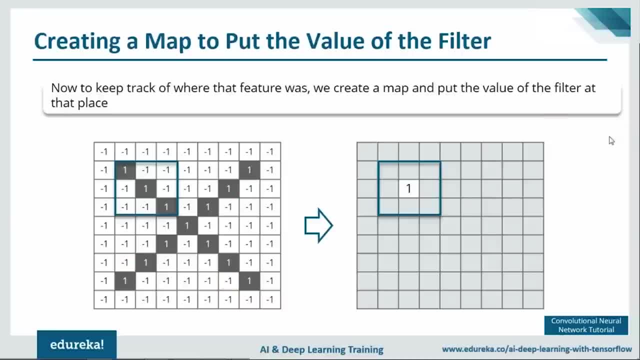 After that, we are going to move it here, here, here, everywhere on the image, we are going to move it and we are going to follow the same process. All right, so yeah, this is one more example where I've moved my filter in between. 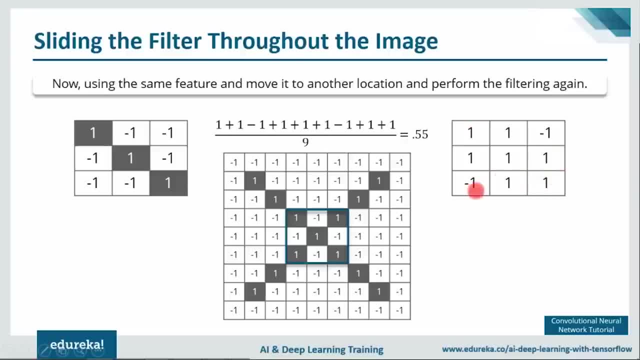 and after doing that, I've got the output something like this: one one minus one and all So over here, if you notice, I've got a couple of times minus one as well, due to which my output that comes is 0.55, right. 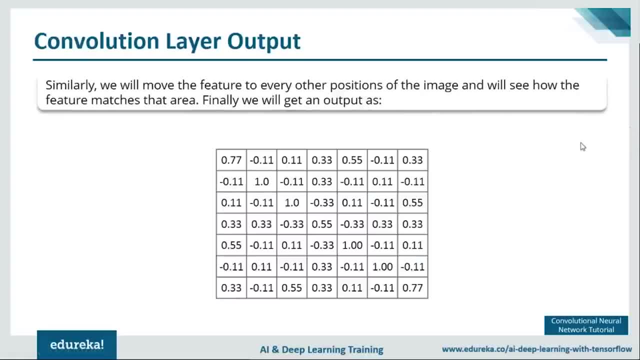 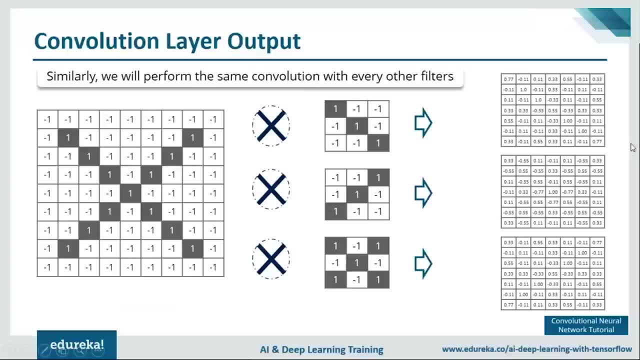 So I'm going to place 0.55 here. Similarly, after moving the pixel, after moving the filter, throughout the image, I got this particular matrix all right, And this is for one particular feature, After performing the same process for the other two filters as well. 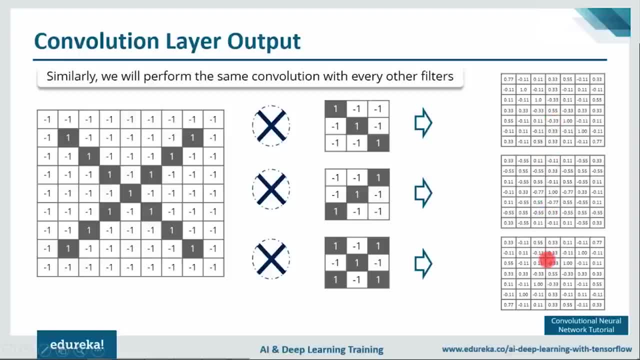 I've got these two values, So we have these three values after passing through the convolution layer. Let me give you a quick recap of what happens in convolution layer. So basically, we have taken three features, all right, And one by one we'll take one feature. 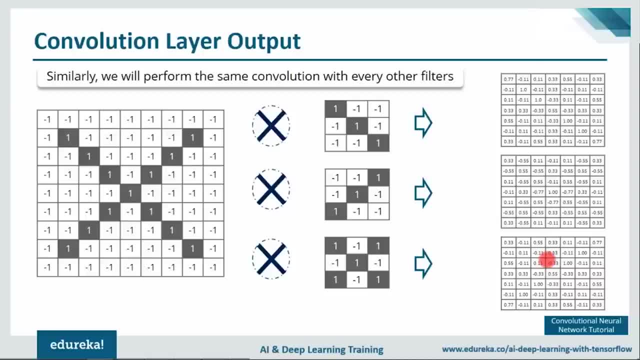 move it through the entire image. and when we are moving it, at that time we are multiplying the pixel value of the image with that of the corresponding pixel value of the filter, adding them up, dividing by the total number of pixels to get the output. 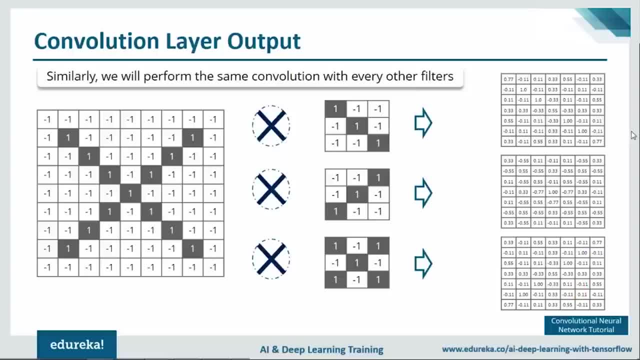 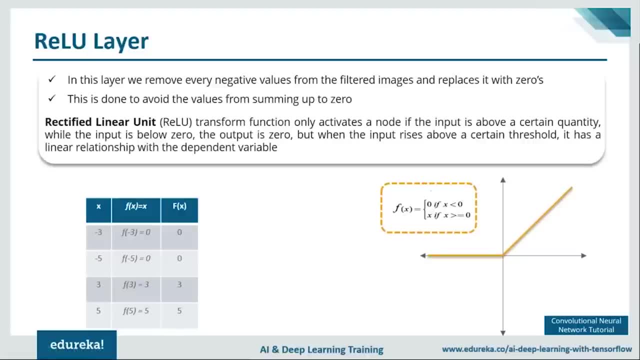 So when we do that for all the filters, we got these three outputs all right. So let's move forward and we'll see what happens in ReLU layer. So this is ReLU layer. guys and people who have gone through the previous tutorial. 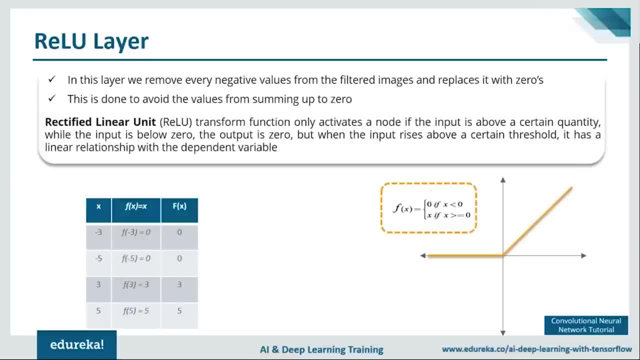 actually know what it is. So let me just give you a quick introduction of ReLU layer. So ReLU is nothing but an activation function, all right. So what I mean by that is it will only activate a node if the input is above a certain quantity. 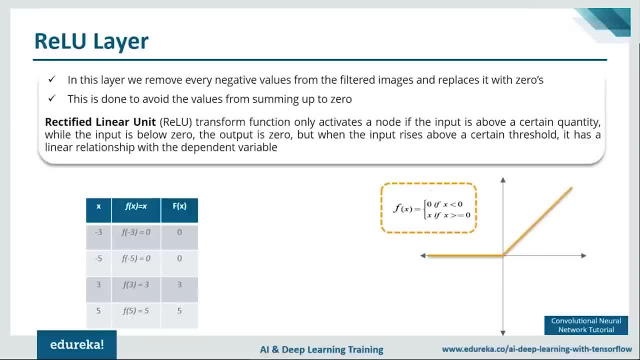 While the input is below zero, the output is also zero, All right. and when the input rises above the certain threshold, it has a linear relationship with the dependent variable. Now I'll explain you with an example. We have a graph of ReLU function here. 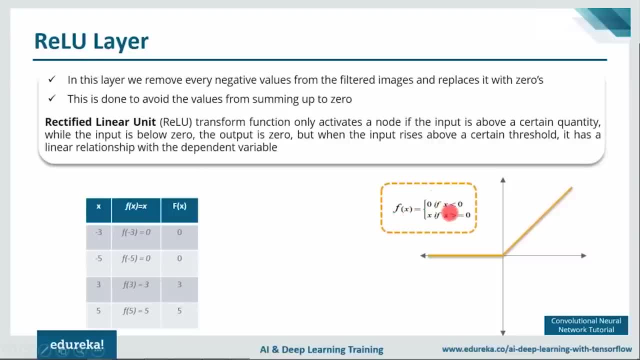 So let's say that when f of x is equal to zero, if x is less than zero, and it is equal to x when x is greater than zero. all right, So whatever values that I have which are below zero will actually, in turn, become zero. 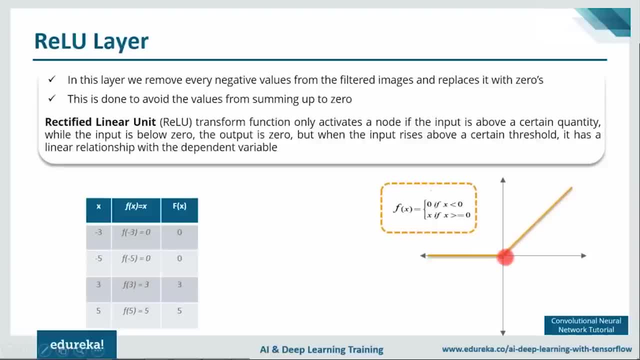 and whatever values that are above zero, our function value will also be equal to that particular value. So f of x will be equal to x if it is greater than or equal to zero, and it will be zero if it is less than zero. 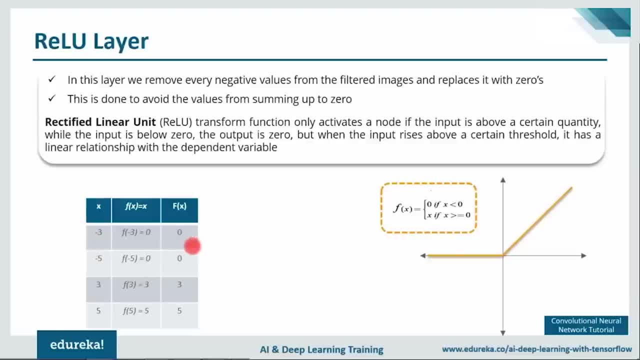 So if I have x value as minus three, so definitely it is less than zero, so f of x becomes zero. Similarly, if I have minus five x value, then again it is less than zero, so my f of x value becomes zero. 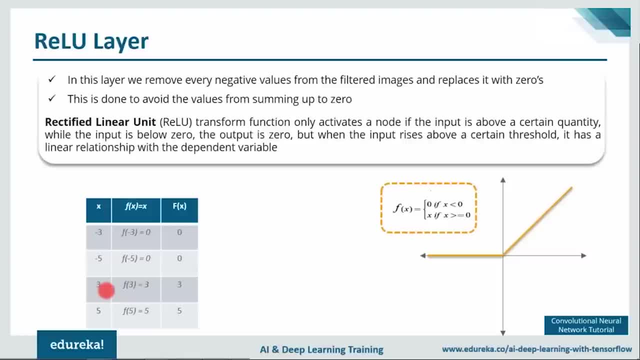 But when I consider three as my x value, then my f of x becomes equal to x, which is nothing but three. So over here I'll have three Again. if I take my x value as five, then obviously it is greater than or equal to zero. 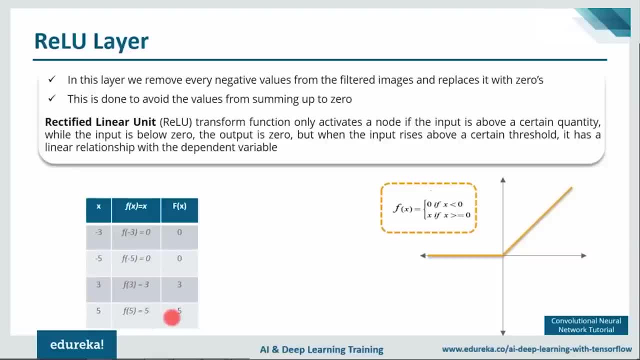 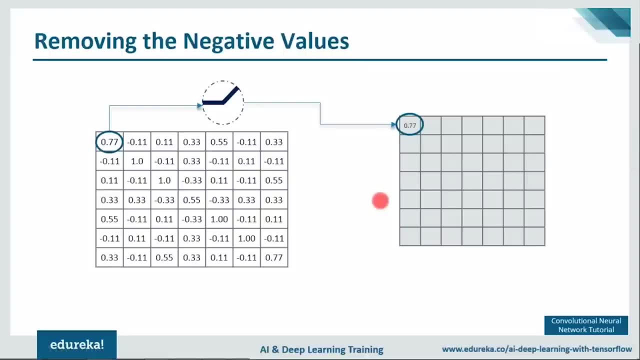 then my f of x becomes equal to x, so my f of x value becomes five. So this is how a ReLU function works. So why are we using ReLU function here? is we want to remove all the negative values from our output that we got through the convolution layer. 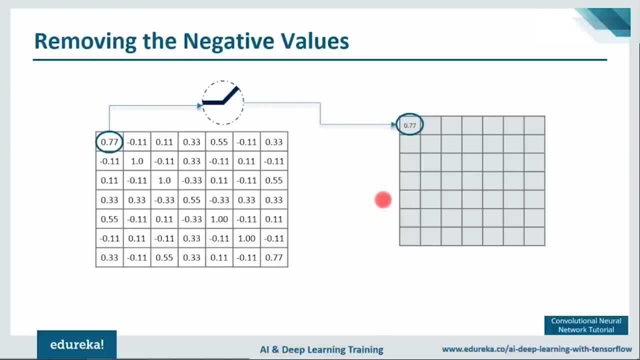 So we'll only take the first output that we got by moving one feature throughout the image. So this is the output that we have got for only one filter, all right, So over here I'm going to remove all negative values. So over here you can see that it was minus 0.11 before. 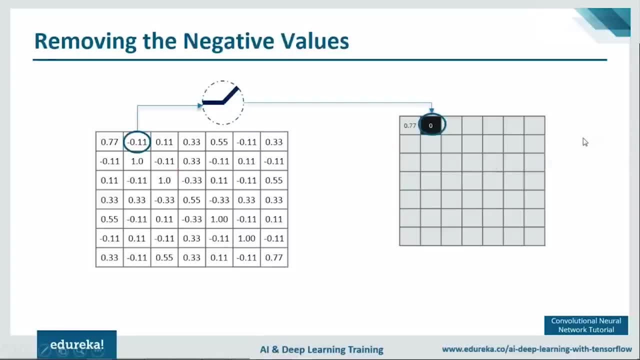 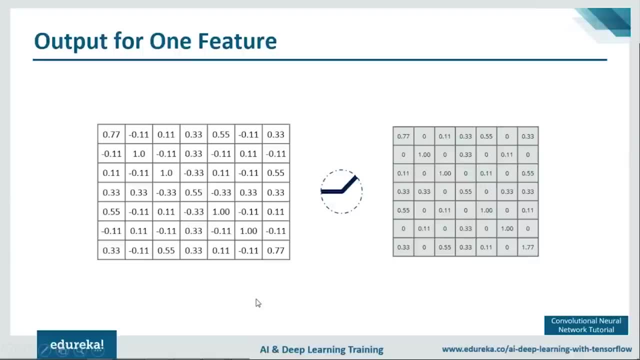 and I've converted that to zero. Similarly, I'm going to repeat the whole process for the entire matrix And once I'm done with that, I get this particular value. Now, remember, this is only for the output that we got through. one feature, all right. 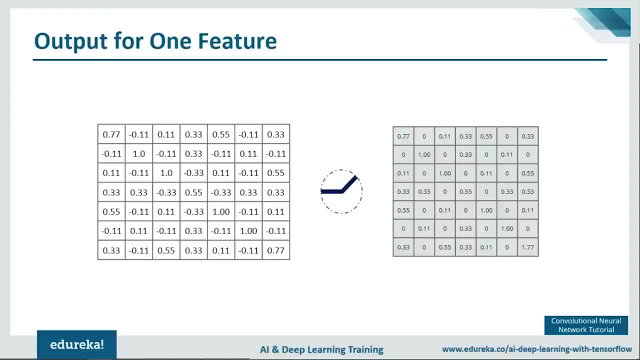 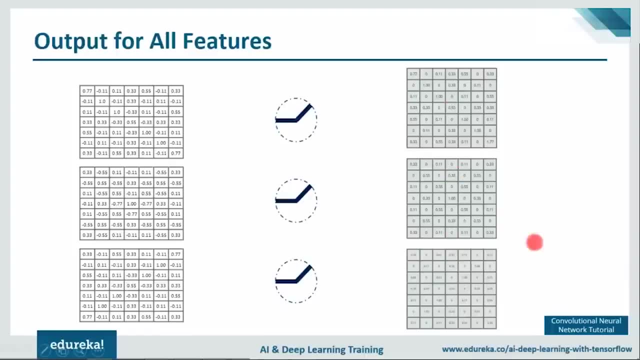 So when we were doing convolution, at that time we were using three features, right. So this is output only for one filter. After doing it for the output of the other two filters as well, we have got these two values more. So, totally, we have these three values. 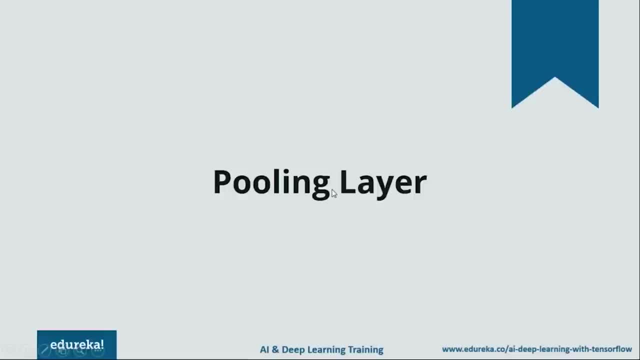 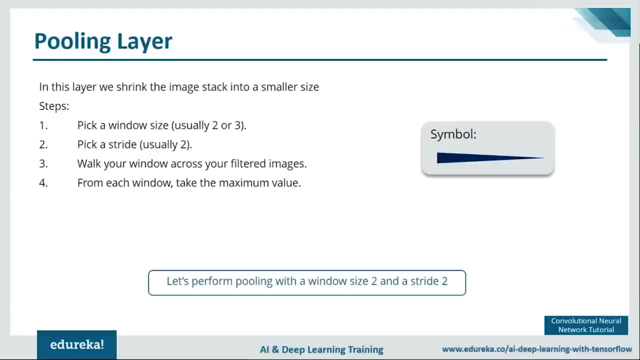 after passing through ReLU activation function. Next up we'll see what exactly is pooling layer. So in pooling layer, what we do? we take a window size of two and we move it across the entire matrix that we have got after passing through ReLU layer. 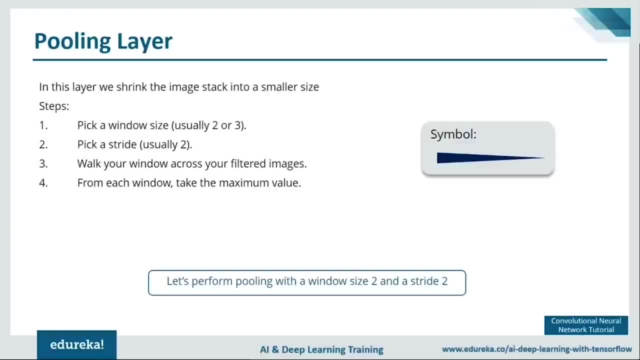 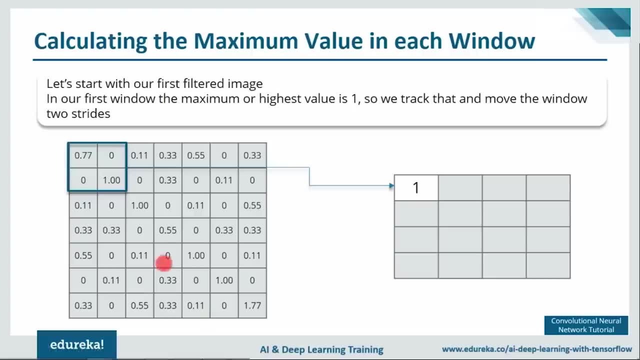 And we take only the maximum value from there so that we can shrink the image. So what we are actually doing is we are reducing the size of our image. So let me explain you with an example. So this is basically one output that we have got. 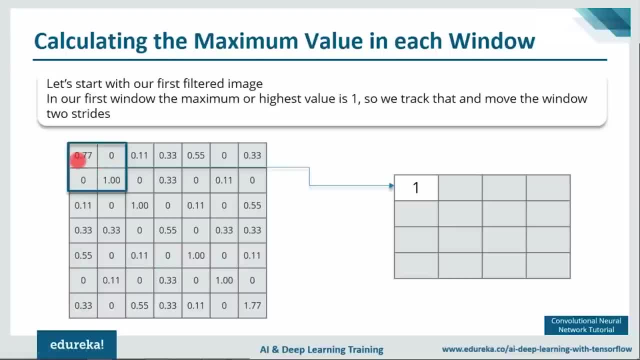 So this is basically one output that we have got. So this is basically one output that we have got. after passing through ReLU layer And over here, we have taken a window size of two cross two. So when we keep this window at this particular position, 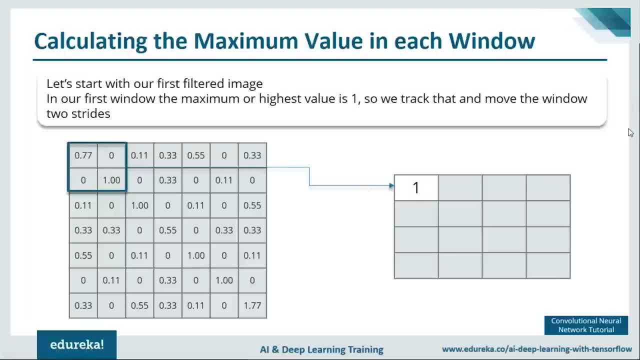 we see that one is the highest value, So we are going to keep one here And we are going to repeat the same process for this particular window as well. So over here the maximum value is 0.33, so 0.33 will come. 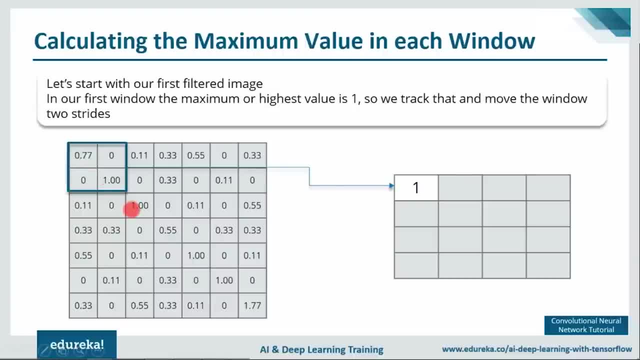 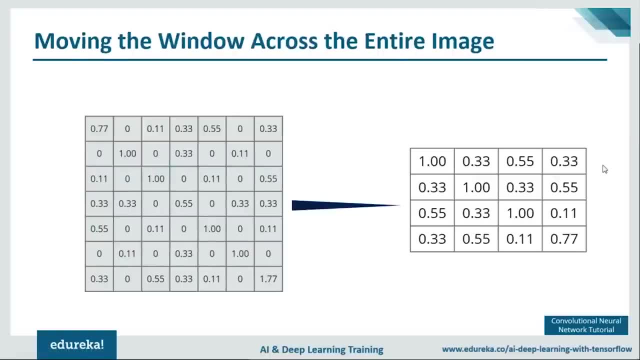 So, if you notice here, earlier we had seven cross, seven matrix, and now we have reduced that to four cross, four matrix. So after doing that, for the entire image, we have got this as our output. This output we have got after moving our window. 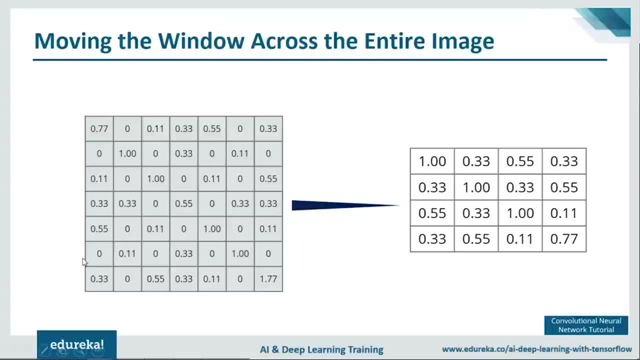 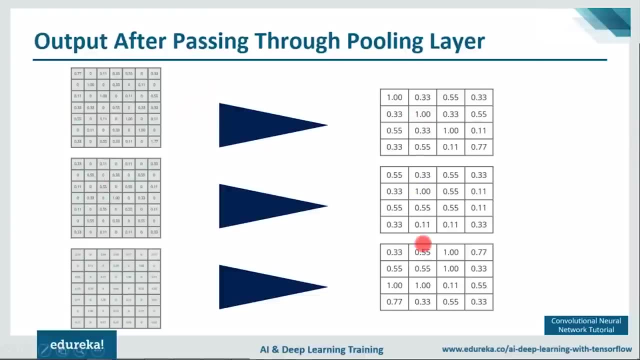 throughout the image that we have got after passing through ReLU layer. And when we repeat this process for all the three outputs that we have got after the ReLU layer, then we get this particular output after pooling layer. So basically, we have shrinked our image. 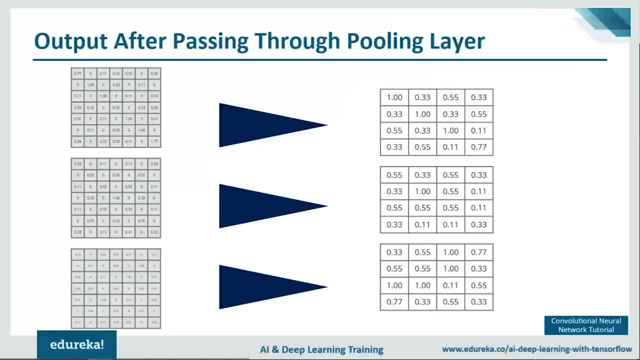 to a four cross four matrix. Now comes the tricky part. So what we are going to do now is stack up all these layers. So we have discussed convolution layer, ReLU layer and pooling layer. So I'll just give you a brief recap. 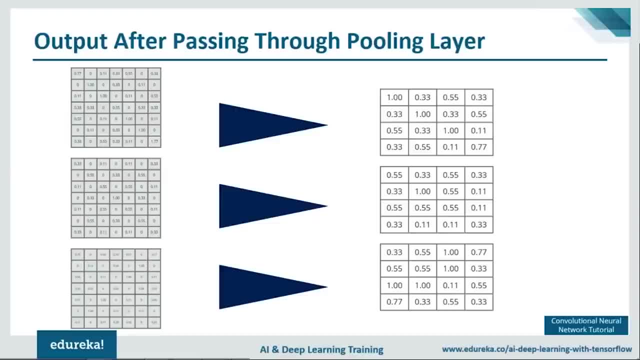 of what all things we have discussed In convolution layer. what we did? we took three features And then, after that, one by one, we moved each filter throughout the image, And when we were moving it, we are continuously multiplying the image pixel value with that of the corresponding filter. 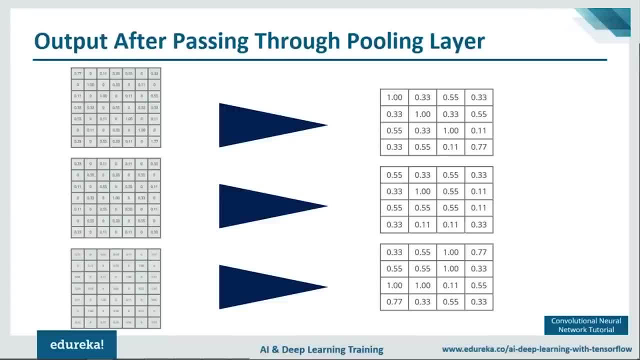 pixel value And then we were dividing it by the total number of pixels. All right, with that, we got three output after passing through the convolution layer. Then those three output, we pass through a ReLU layer where we have removed the negative value. 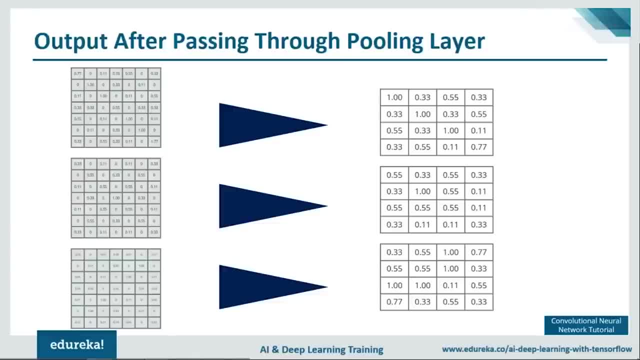 All right, and after removing negative value again, we have got the three outputs. Then those three outputs we pass through pooling layer. So basically, we're trying to shrink our image And what we did? we took a window size of two cross two. 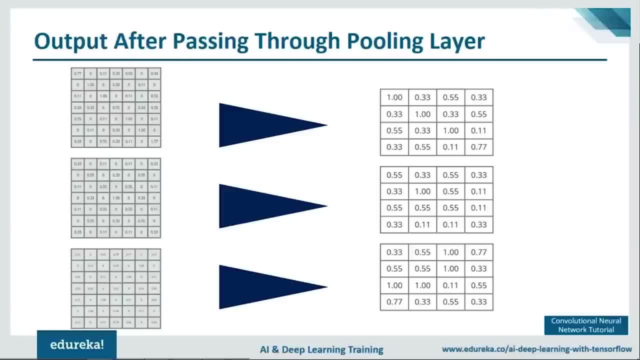 moved it through all the three outputs that we have got through ReLU layer And after doing that we were only taking the maximum value, pixel value, in that particular window, And then we are putting it in a different matrix so that we get a shrink image. 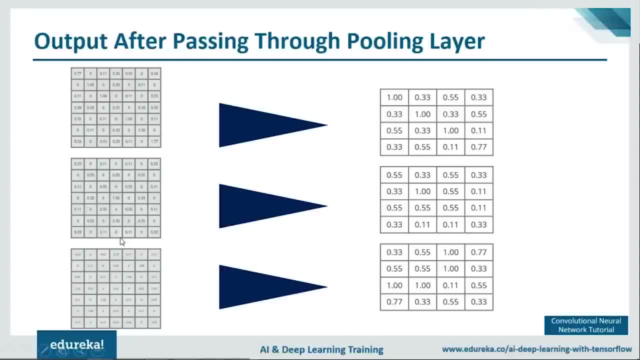 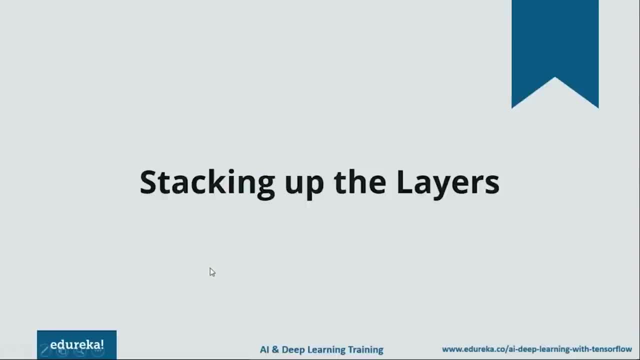 And after passing it through pooling layer, we have got a four cross, four matrix And since we took three features at the beginning, so therefore we have got three outputs after passing through pooling layer. All right, next up, we are going to stack up all these layers. 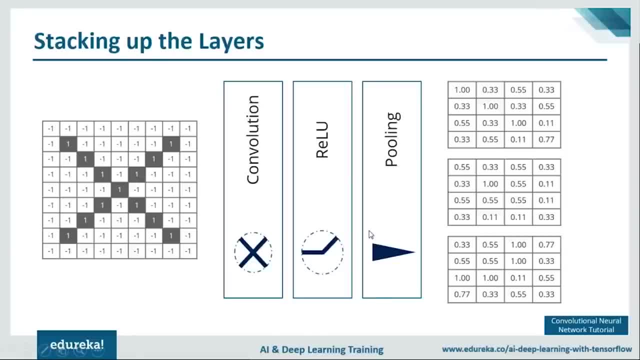 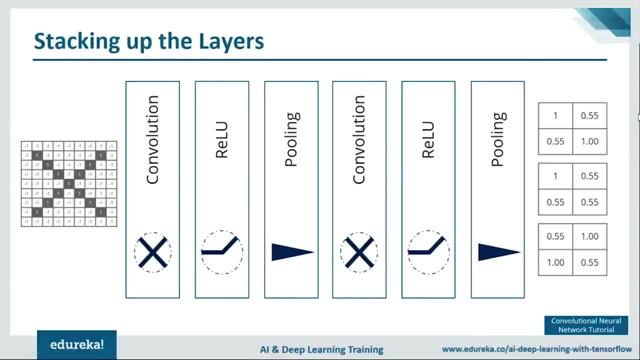 All right, so let's do that. So, after passing through convolution, ReLU and pooling, we have got this four cross, four matrix. This was our input image. Now, when we add one more layer of convolution, ReLU and pooling, we have shrinked our image. 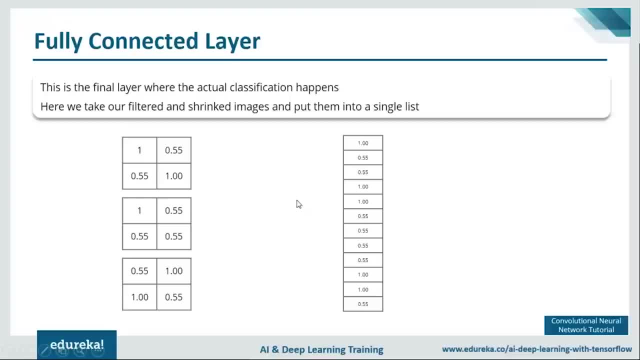 from four cross four to two cross two, as you can notice here. Now we are going to use fully connected layer. Now, what happens in fully connected layer? The actual classification happens here, guys, okay, So what we are doing here is we are going to take 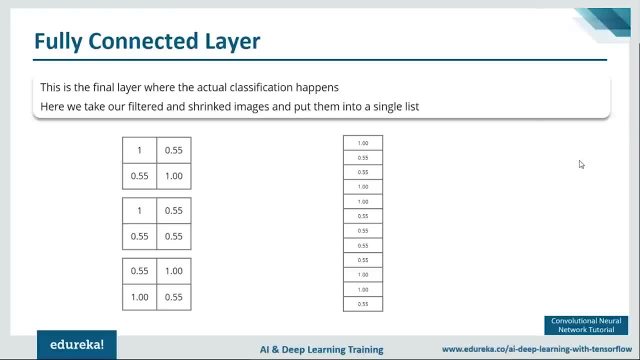 the shrinked images and put it into a single list. So, basically, this is what we have got after passing through two layers of convolution, ReLU and pooling, and this is what we have got. So, basically, we are converting into a single list. 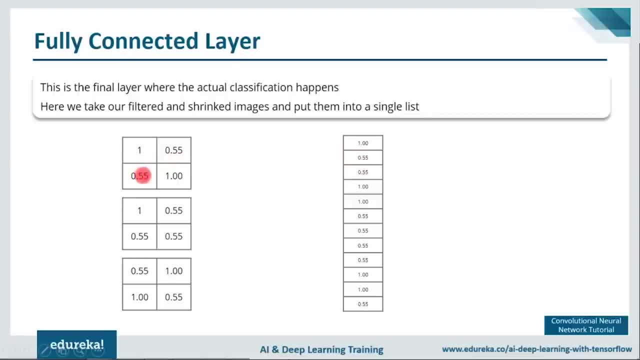 or a vector. How we do that. we take the first value one, then we take .55,, then we take .55,, then we take one again, Then we take one, then we take .55,, .55,, .55.. 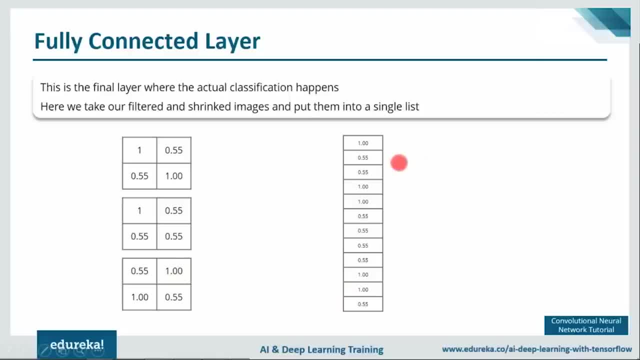 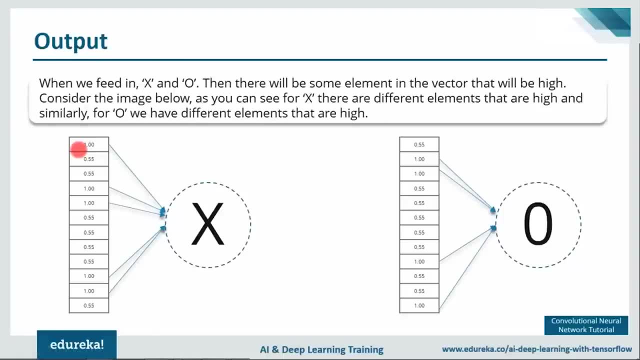 Then we again take .55, one one and .55.. So this is nothing but a vector, or you can say a list, If you notice here that there are certain values in my list which are high for x, and similarly, if I repeat. 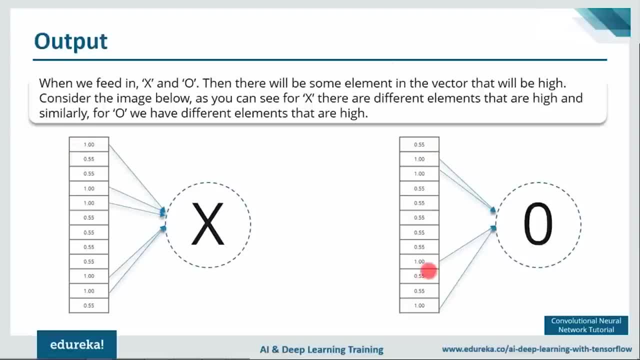 the entire process that we have discussed. for o, there are different values which will be high. So for x we have first, fourth, fifth, tenth and eleventh element vector values are high. For o, we have second, third, ninth and twelfth. 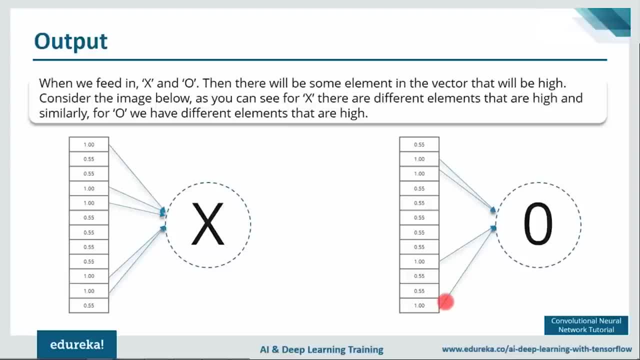 element vector which are high. So basically we know now, if we have an input image which has first, fourth, fifth, tenth and eleventh element vector values high, we know that we can classify it as x. Similarly, if our input image has a list which has: 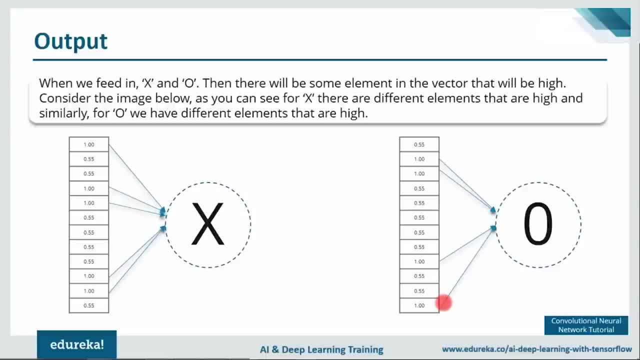 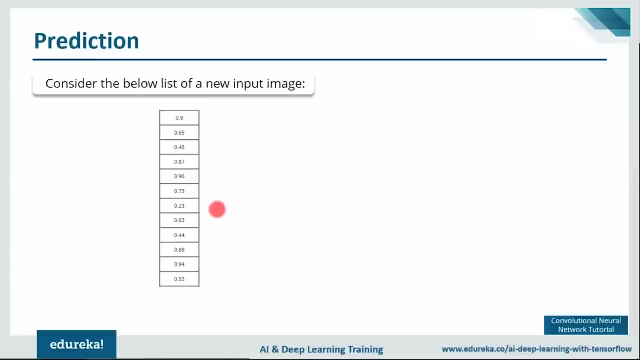 the second, third, ninth and twelfth element vector values high, then we can classify it as zero. Now let me explain it with an example. So after the training is done, after doing the entire process for both x and o, you know that our model 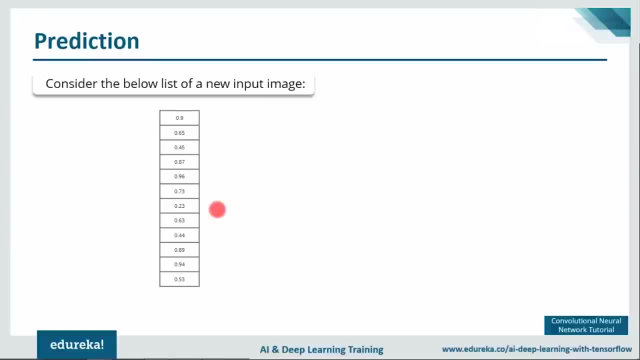 is trained now. okay, So we have given a new input image and that input image passes through all the layers and once it has passed through all the layers, we have got this 12 element vector. Now it has .9,, .65, all these values, right? 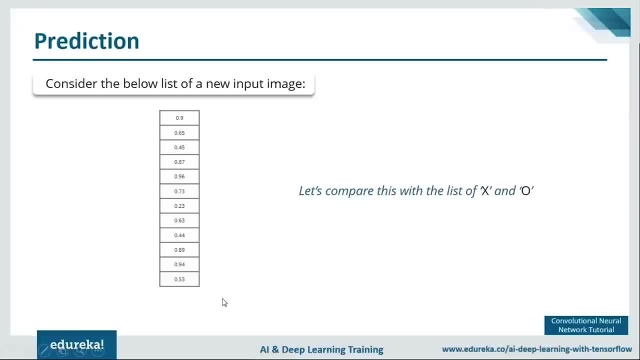 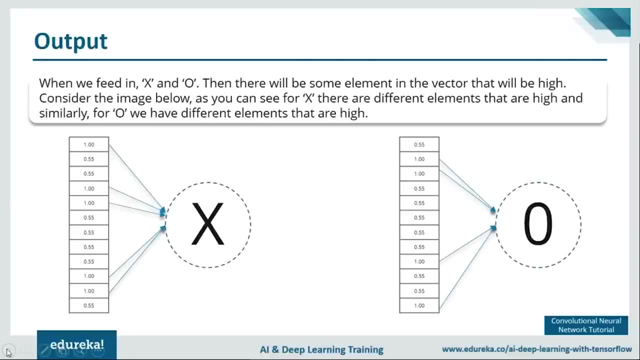 Now, how do we classify it, whether it is an x or o? So what we do? we compare this with a list of x and o, Right? So we have a list. in the previous slide, if you notice, We have got two different lists for x and o. 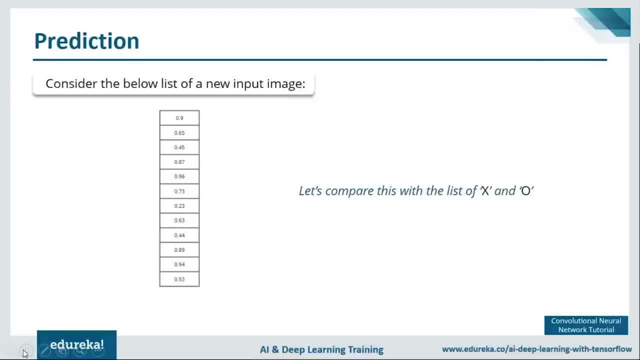 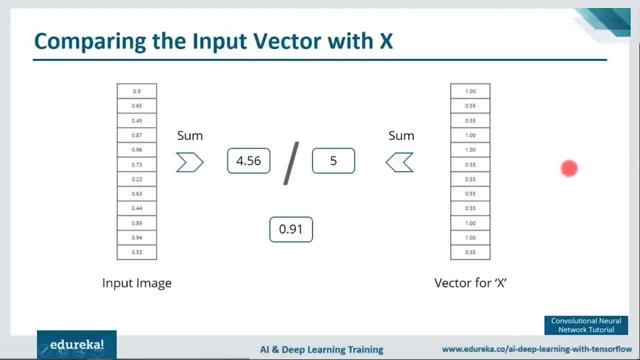 We are going to compare this new input image list that we have got with that of x and o, Right, so first let us compare that with x. Now, as I've told you earlier as well, for x there are certain values which will be high, which is nothing. 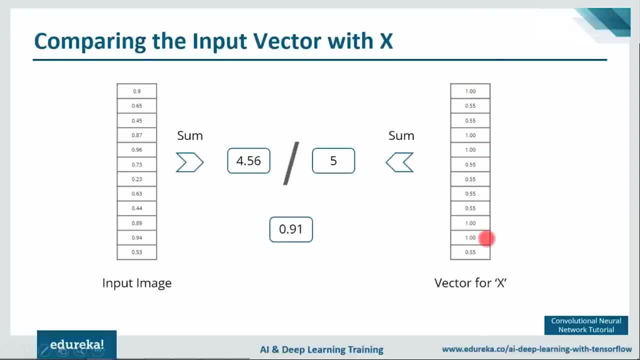 but first fourth, fifth, tenth and eleventh value, right, So I'm going to sum first fourth, fifth, tenth and eleventh value, and I've got five, One plus one plus one plus one and plus one. 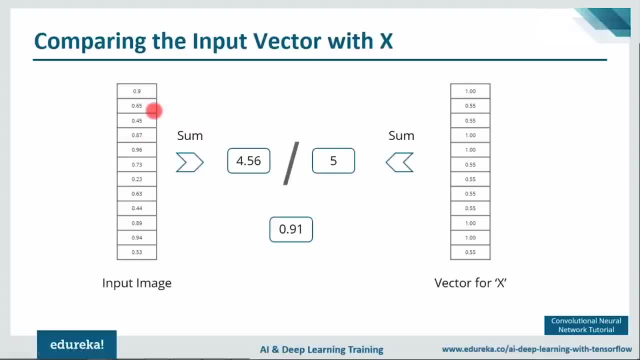 So five times one, I've got five. And now I'm going to sum the corresponding values of my input image vector as well. So the first value is .9, then the fourth value is .87,. fifth value is .96,. tenth value is .89,. 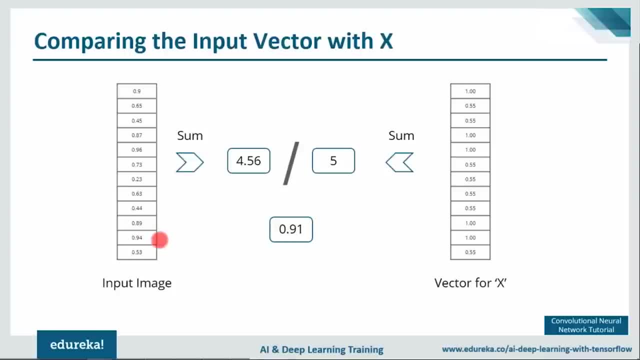 and the eleventh value is .94.. So after doing the sum of these values, I've got 4.56.. When I divide this by five, I've got .91,. right Now, this is for x. Now, when I do the same process for o, so in o, 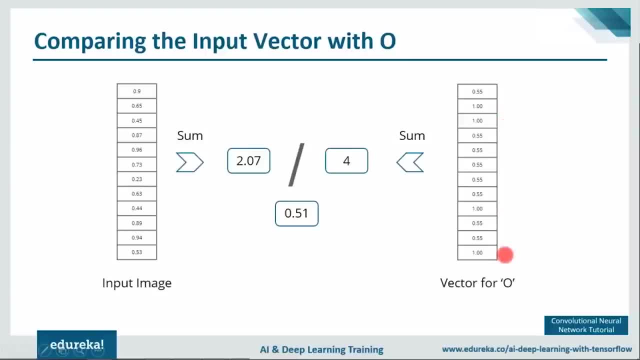 if you notice, I have second, third, ninth and twelfth element vector values as high. So when I sum these values I get four, And when I do the sum of the corresponding values in my input image I've got 2.07.. 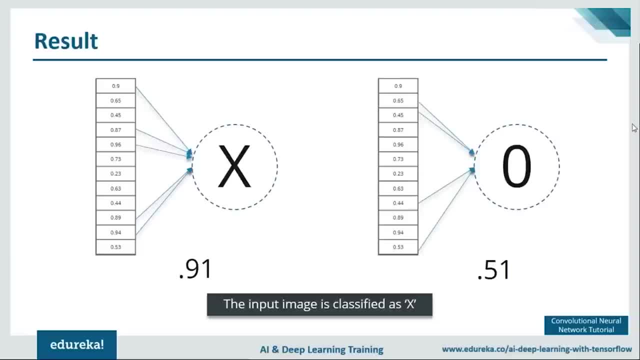 When I divide that by four, I got .51.. So now we notice that .91 is a higher value compared to .51.. So when we have compared our input image with the values of x, we got a higher value than the value that we have got after comparing. 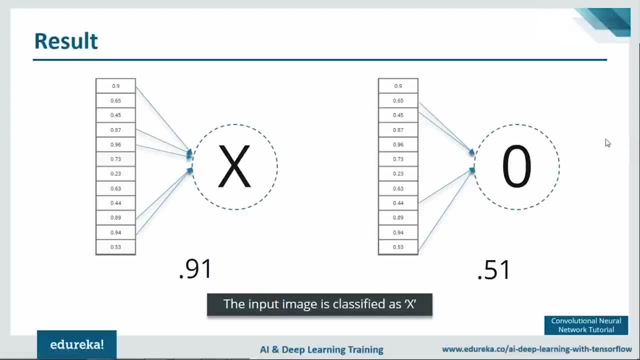 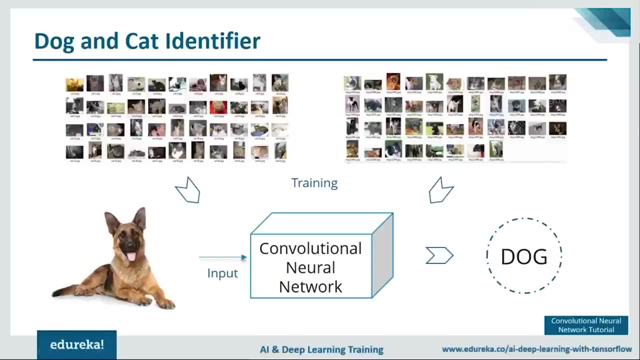 the input image with the values of four. So the input image is classified as x. All right, so now let us move towards our use case. So this is our use case, guys. So over here, what we are going to do is we are going to train. 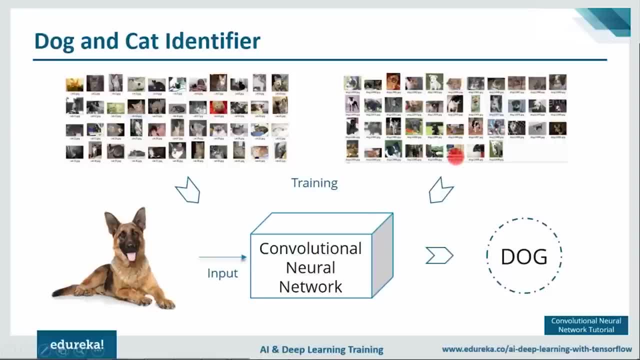 our model on different types of dogs and cat images And once the training is done, we are going to provide it an input and it will classify whether the input is of a dog or a cat. Now let me tell you the steps involved in it. 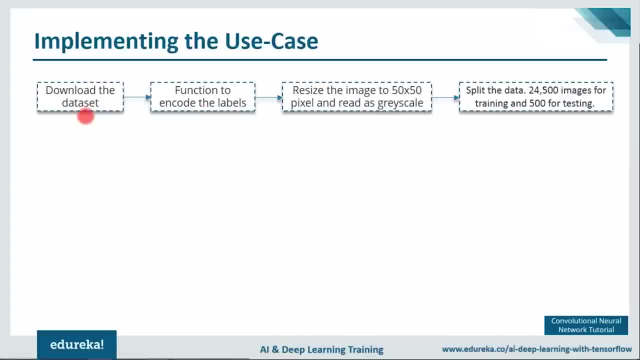 So what we are going to do in the beginning is obviously: first we need to download the data set. After that we are going to write a function to encode the labels. Labels are nothing but the dependent variable that we are trying to predict. So in our training data and testing data, 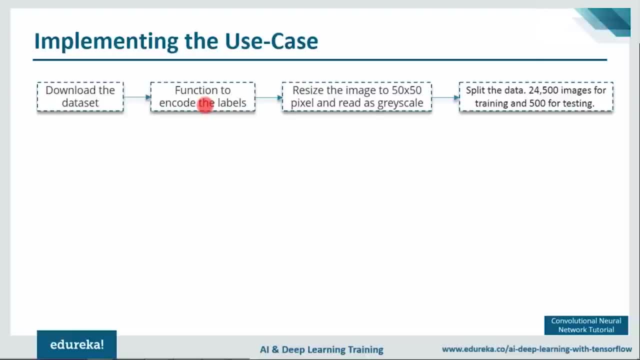 obviously we know the labels right. So on that basis only we are going to encode those labels. After that we'll resize the image to 50 cross 50 pixel and we are going to read it as a grayscale image. Then we are going to split the data. 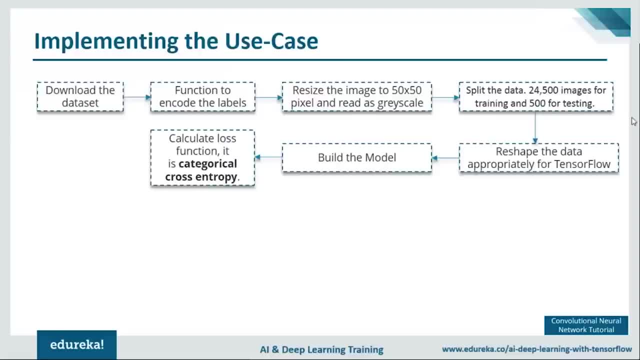 24,000 images for training and 50 for testing. Once this is done, we are going to reshape the data appropriately for TensorFlow. Now TensorFlow: I think everyone knows about TensorFlow. TensorFlow is nothing but a Python library for implementing deep learning models. 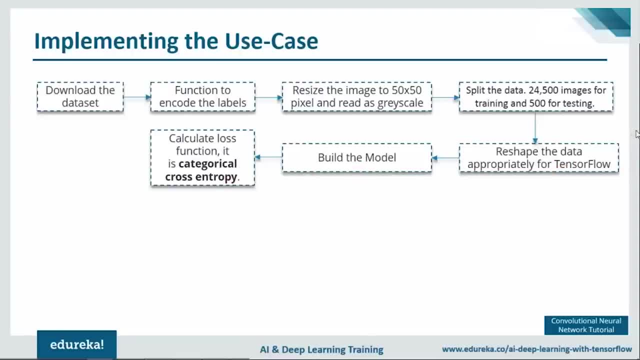 Then we are going to build the model, calculate the loss. It is nothing but categorical cross entropy. Then we are going to reduce the loss by using Adam Optimizer with a learning rate set set to 0.001.. Then we are going to train the deep neural network. 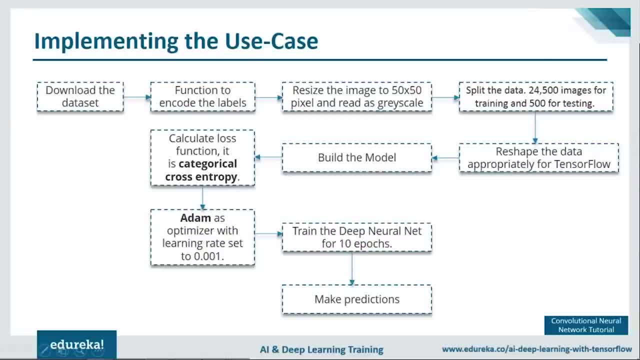 for 10 epochs. And finally, we are going to make predictions. All right, so I'll just quickly open my PyCharm and I'll show you the code how it looks like. So this is a code that I've written in order to implement the use case. 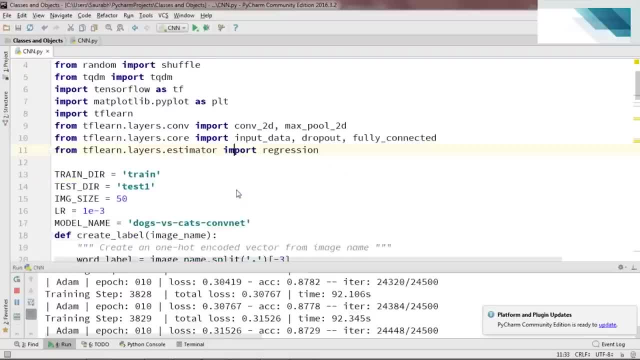 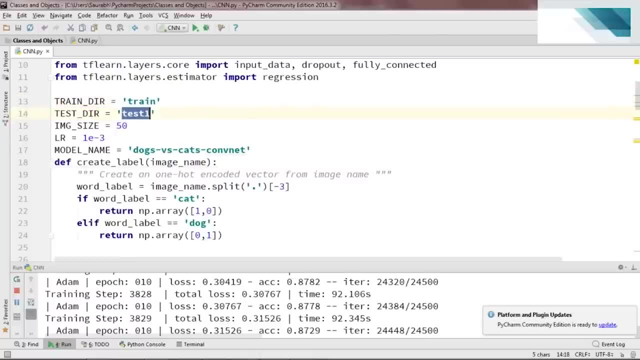 In the beginning, I need to import the libraries that I require And once it is done, what I'm doing? I'm defining my training data and the testing data. So train and test one contains the training data. It contains both my training data. 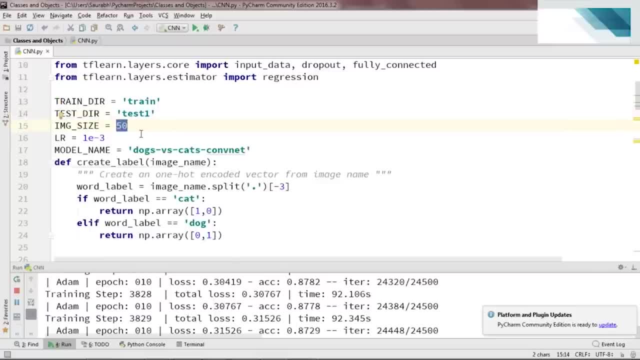 as well as testing data respectively. Then I've taken my image size as 50 and learning rate I've defined here And I've given a name to my model. You can give whatever name you want. All right, the first thing that we saw. 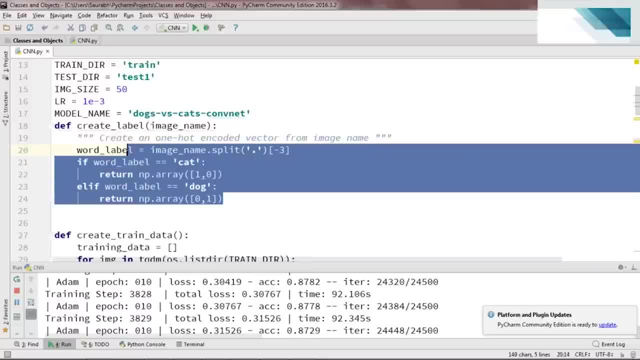 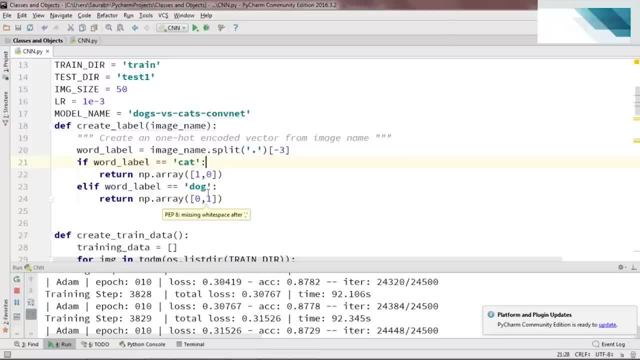 we need to encode the dependent variable. That's what we are doing here. We are encoding our dependent variable. So whenever the label is cat, then it will be converted to an area of 1,0.. And when it is dog, it will be converted. 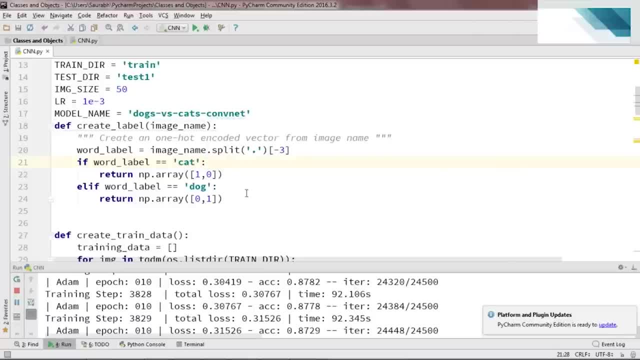 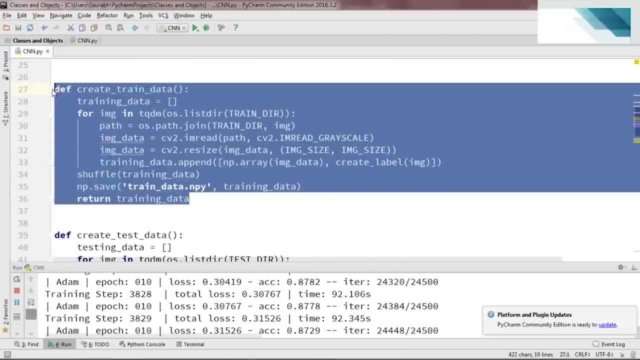 to an area of 0,1.. So why we're actually encoding the label? Because our code cannot understand the categorical variable, so we need to encode it right. Next, what I'm doing is I'm resizing my image to 50 cross 50. 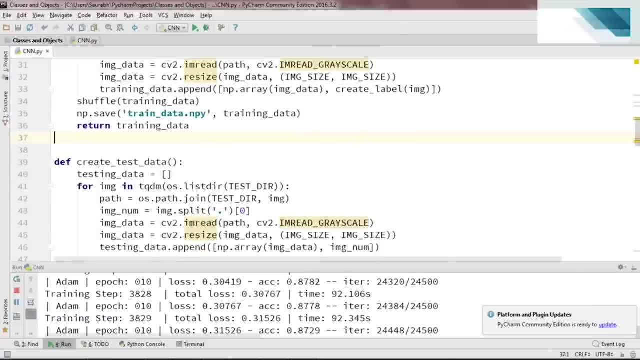 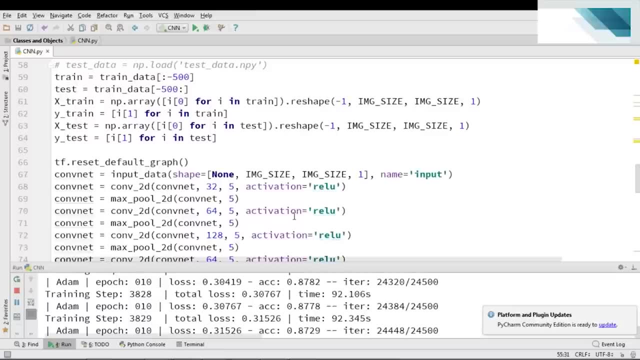 and I am converting it to a grayscale image, right, And once this is done, I'm going to split my data set into training and testing parts. So yeah, we are basically splitting the data set into two parts for training and testing, And here we are defining a model. 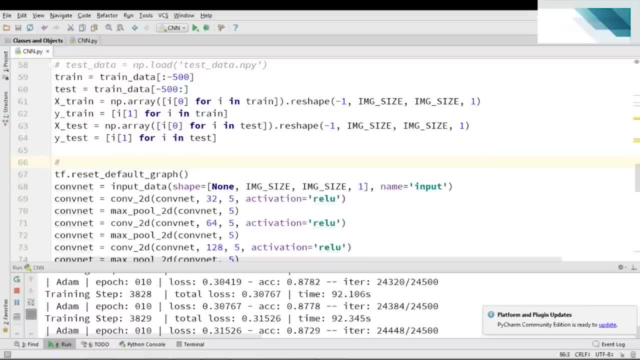 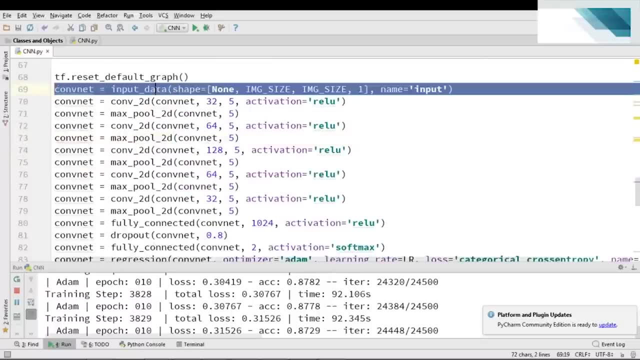 So you can just- I can just- go ahead and throw in a comment here Building a model, yeah, So this is where we are building the model. So, basically, what we have done here is we have resized our image to 50 cross, 50 cross one matrix. 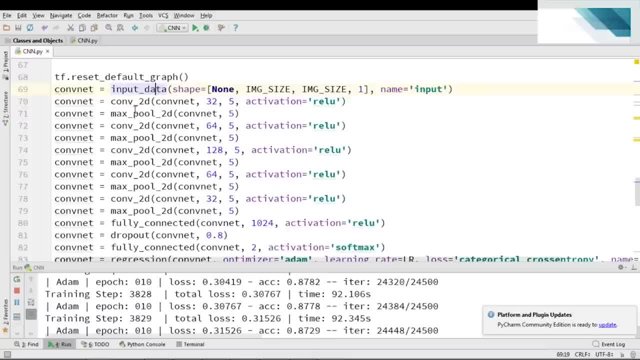 and that is the size of the input that we are using, right, This input that I'm talking about. Then what we have done: a convolution layer we have defined with 32 filters and a stride of five with an activation function, a ReLU. 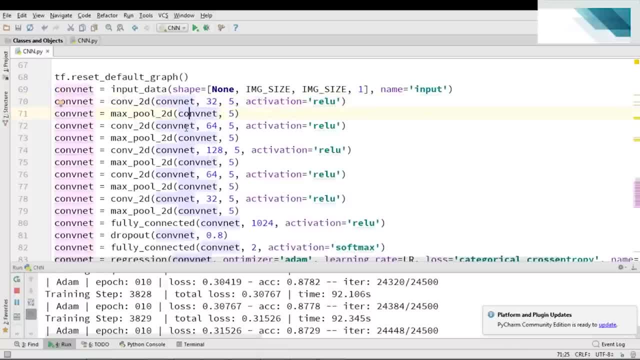 And after that we have added a pooling layer, max pool layer. okay, Again what we have done. we have repeated the same process, but over here we are taking 64 filters and five stride, passing it through a ReLU. 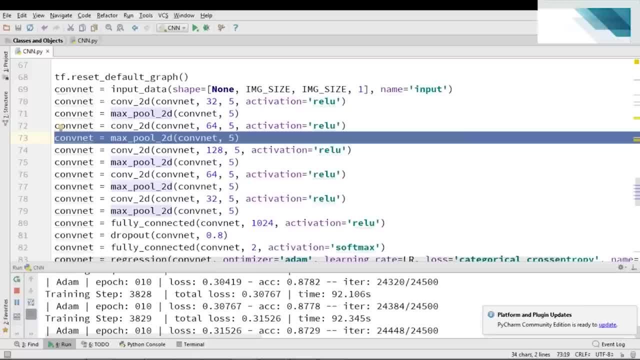 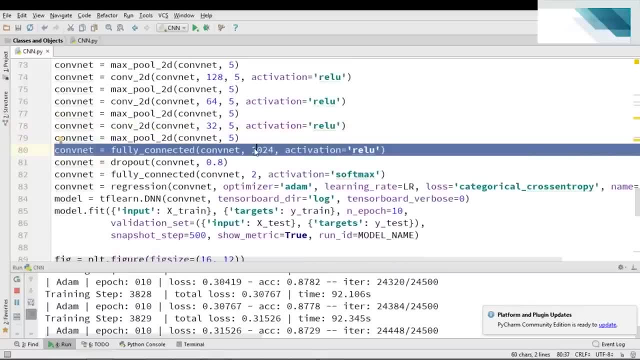 and after that we have a pooling layer- max pool layer- Then we have repeated the same process for 128 filters. After that we have repeated for 64 filters, then for 32 filters, Then after that we are using a fully connected layer. 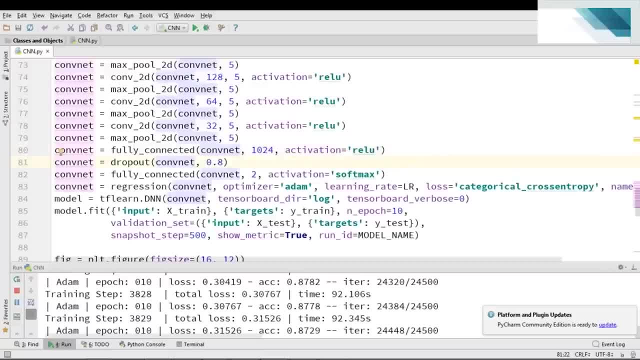 with one zero, two, four neurons. And finally, we are using the dropout layer, with key probability of 0.8, to finish our models. This is where our model is actually finished, And then what we are doing is we are using the Adam optimizer. 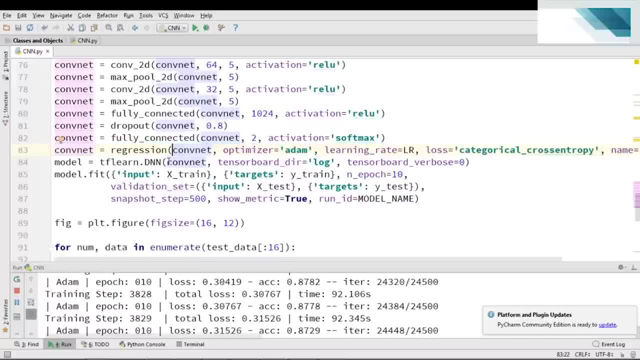 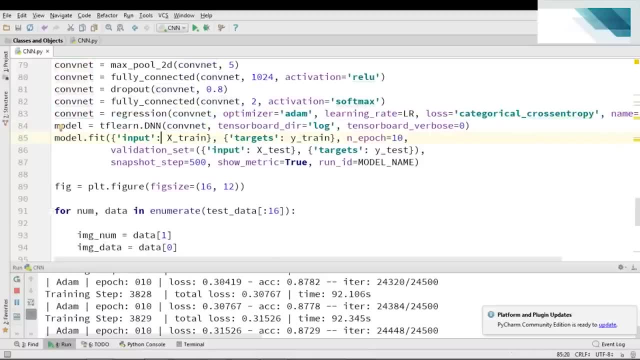 to optimize our model. So, basically, whatever the loss that we have, we are going to reduce it, And this is basically for your TensorBoard. So we are creating some log files and then, with that log file, TensorBoard will create a pretty fancy graph for us. 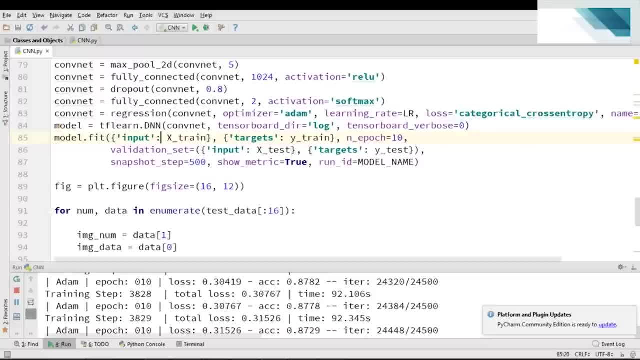 that helps us to visualize the entire model. And then what we are doing is we are trying to fit the model And we have defined epochs as 10, that is, the number of iterations that will happen will be 10.. And yeah, so this is pretty much it. 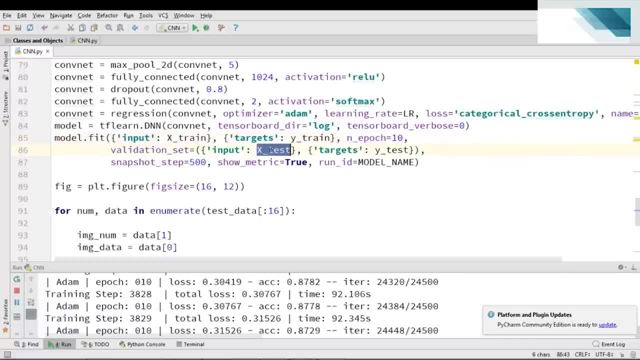 Model name we have given. Then input is X underscore test to check the accuracy. Similarly, the target will be Y underscore test. labels associated with that test data will be Y underscore test and which we have encoded basically. So this is how we are going to actually calculate. 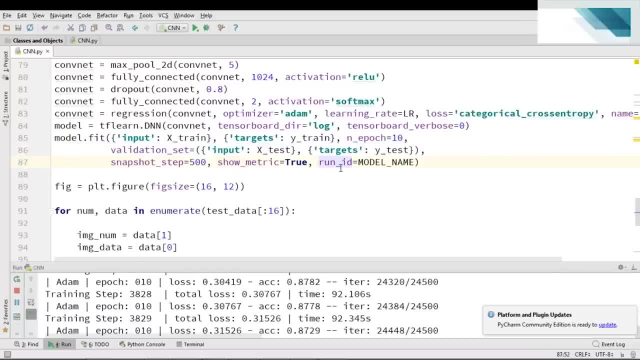 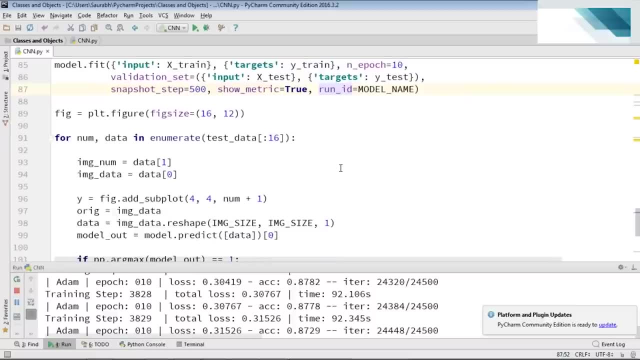 the accuracy and we'll try to reduce the loss as much as possible in 10 epochs. So till now, our model is complete. we are done with it. Next, what I'm doing is I'm feeding in some random input from the test data and I'm validating. 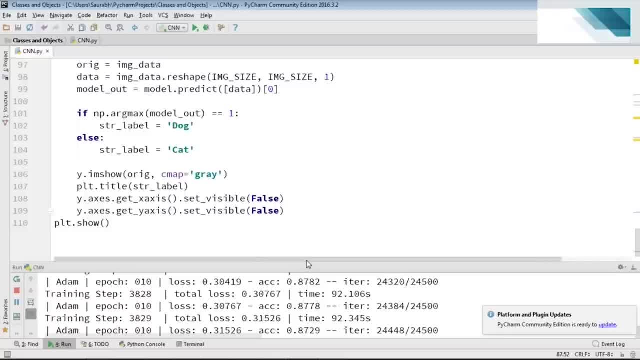 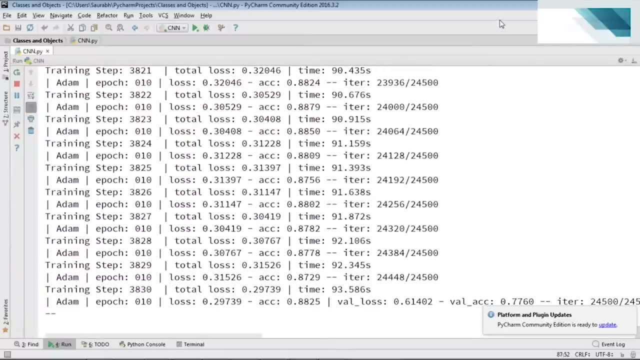 whether my model is predicting it correct or not. All right, so I've already trained the model, because it takes a lot of time and, yeah, I cannot do it here. So I've already trained the model and you can see that the loss that came after the 10th epoch. 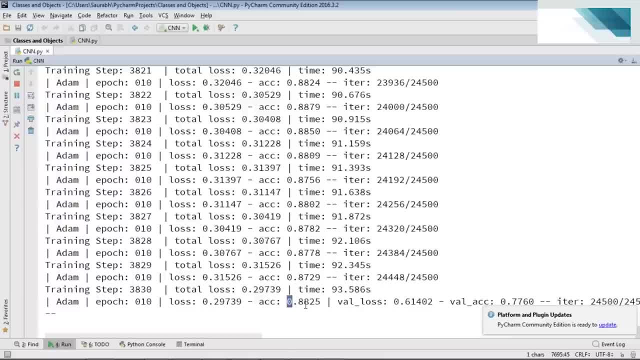 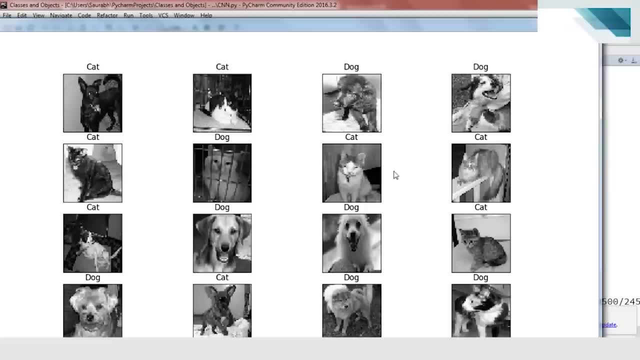 is 0.2973 and the accuracy is somewhere around 88%, which is pretty good guys. And yeah, and I've done the prediction on the test data as well, So let me just show it to you that. So this is the prediction that it has done. 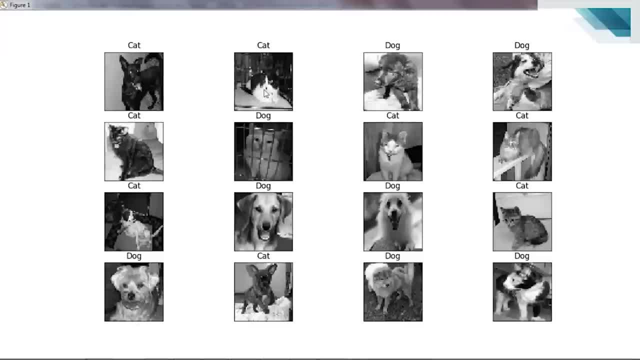 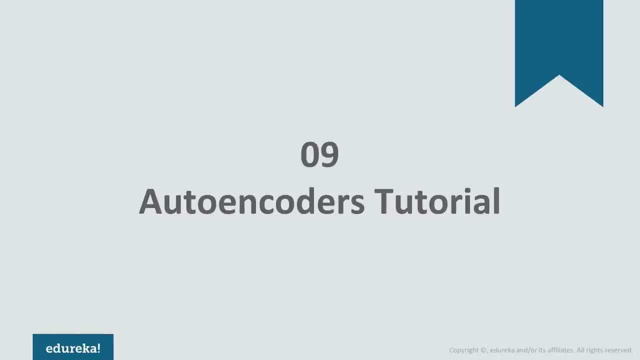 on a few of the images in the test data. So yeah, it is a cat predicted as cat, cat predicted as a cat, cat, cat, cat and dogs as well. There are certain dogs as well. Welcome to today's tutorial session based on the auto encoders. 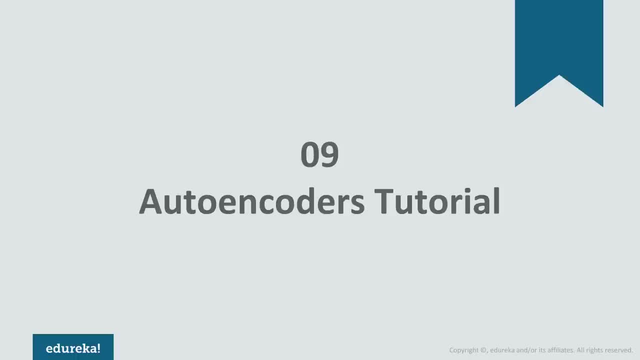 Now in this session you will have a deeper insight into the working of auto encoders. that will help you build a strong fundamental knowledge about the topic. So let's move forward and look at the agenda of today's session. So we will begin with the fundamental query. 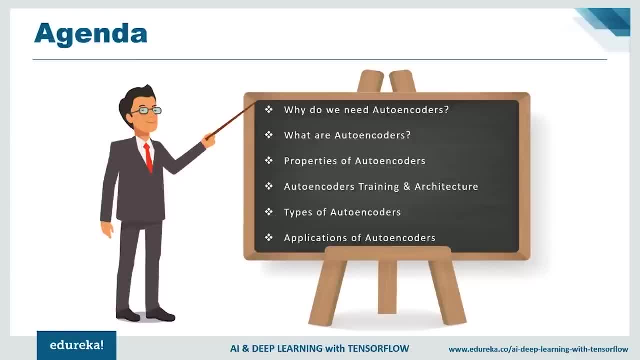 that. why do we need auto encoders? next We will start with the introduction to what are auto encoders and the various components of these. then we will move on to the various properties of auto encoders. next We will see how the training is done. 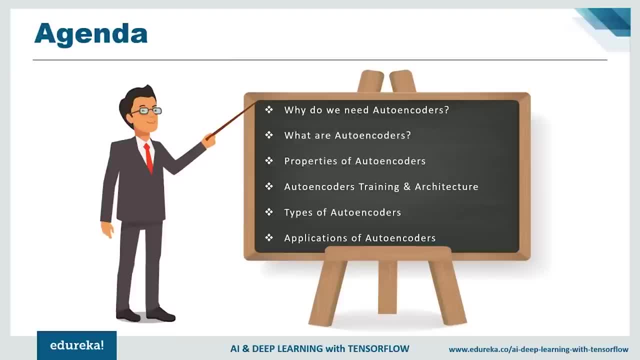 and discuss the architecture of auto encoders. moving on, We will have a detailed discussion about the various types of auto encoders, such as convolution auto encoders, parse auto encoders, deep auto encoders and contractive auto encoders, and we shall also see how do they work, along with a short demo. 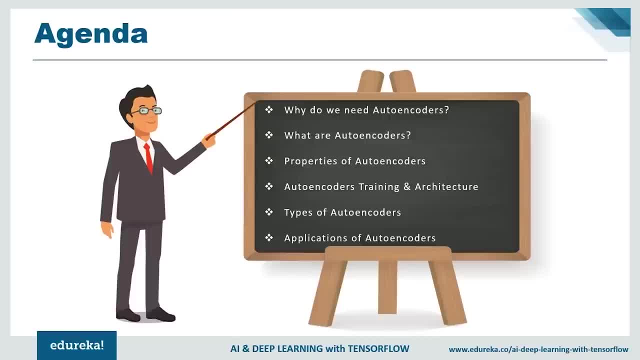 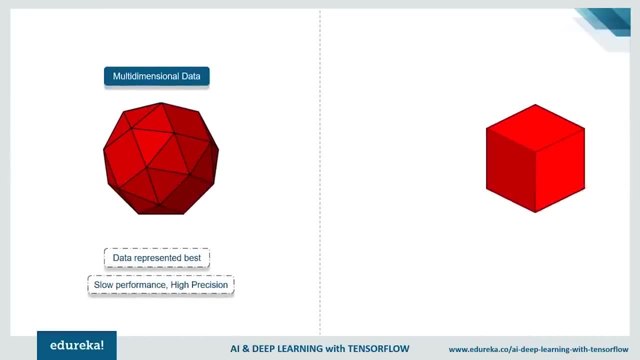 Now, finally, we will have a look at all the applications of auto encoders. So let's get started. data compression is a big topic that's used in computer vision, computer networks and many more. Now the point of data compression is to convert our input. 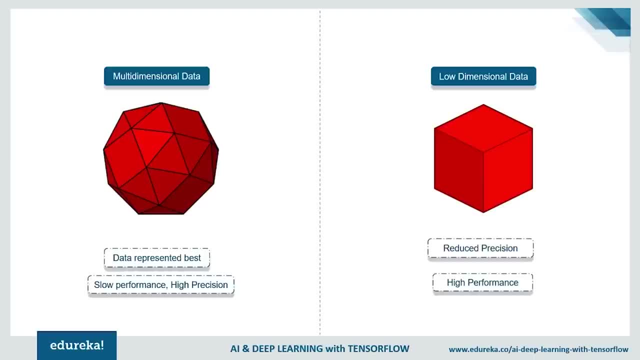 into a smaller representation that we recreate to a degree of quality. the smaller representation is what would be passed around, and when anyone needed the original, they would reconstruct it from the smaller representation. Now, auto encoders are unsupervised neural networks that use machine learning to do this compression for us. 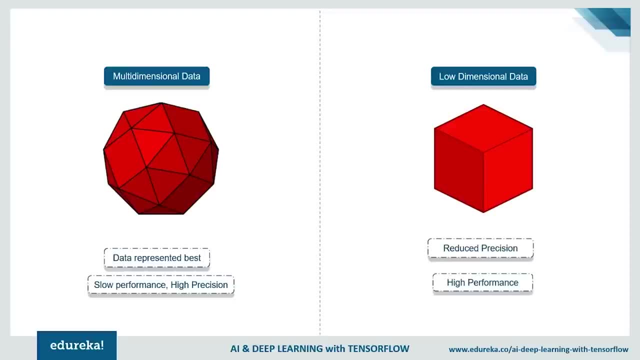 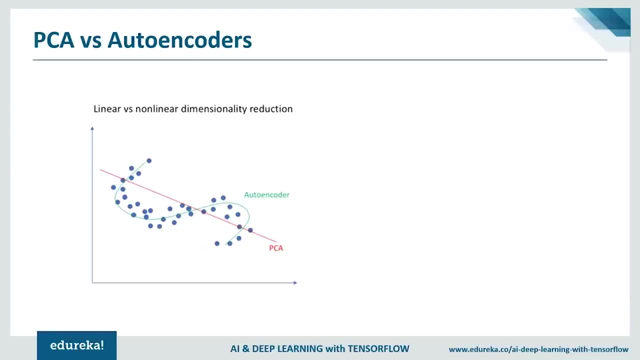 The aim of an auto encoder is to learn a compressed, distributed representation for the given data, typically for the purpose of dimensionality reduction. now, for that we already have principal component analysis. Then why do we need auto encoders? So an auto encoder can learn nonlinear transformations. 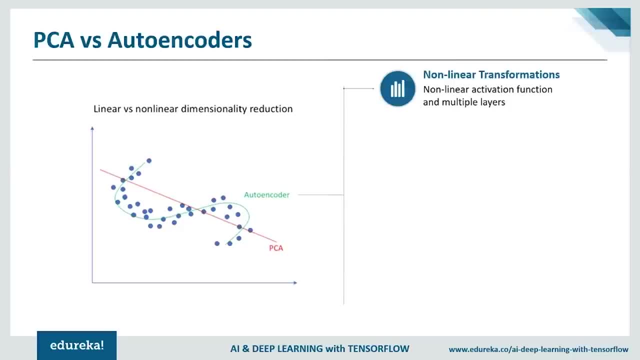 unlike PCA, with a nonlinear activation function and multiple layers. now it doesn't have to learn dense layers, So it can use convolutional layers to learn to, which could be better for video image and series data. Now it may be more efficient in terms of model parameters. 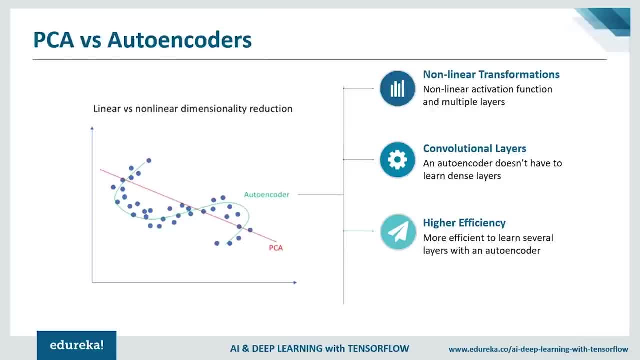 to learn several layers with an auto encoder rather than learn one huge transformation with PCA. and auto encoder also gives a representation as the output of each layer, and having multiple representations of different dimensions is always useful. So an auto encoder could let you make use of pre-trained layers. 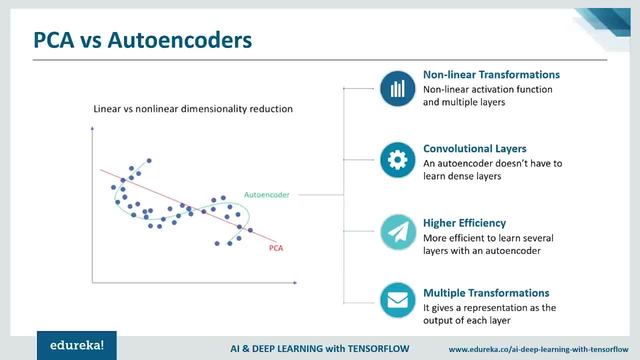 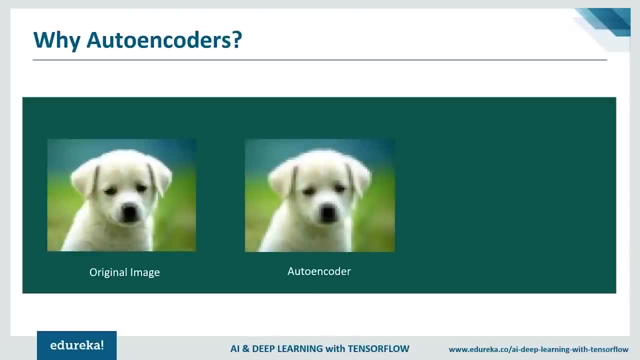 from another model to apply transfer learning, to prime the encoder or the decoder. despite the fact that the practical applications of auto encoders were pretty rare sometime back today, data denoising and dimensionality reduction for data visualization are considered as two main interesting practical applications of auto encoders. 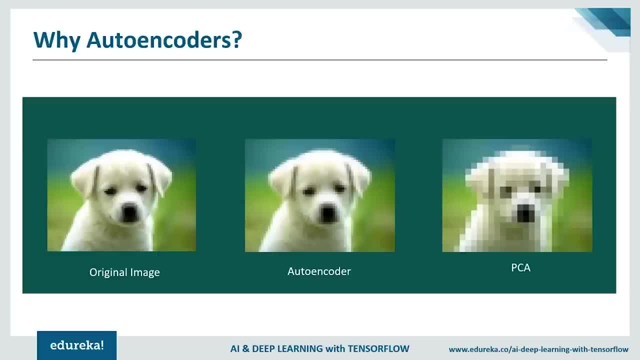 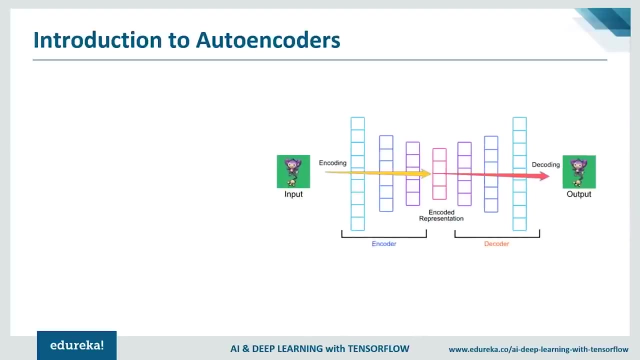 Now, with appropriate dimensionality and sparsity constraints, auto encoders can learn data projections that are more interesting than PCA or other basic techniques. It also provides a more accurate output when compared to PCA. Now, auto encoders are simple learning networks that aim to transform inputs into outputs with the minimum possible error. 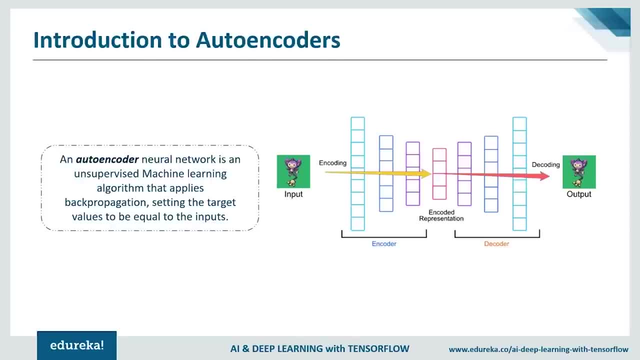 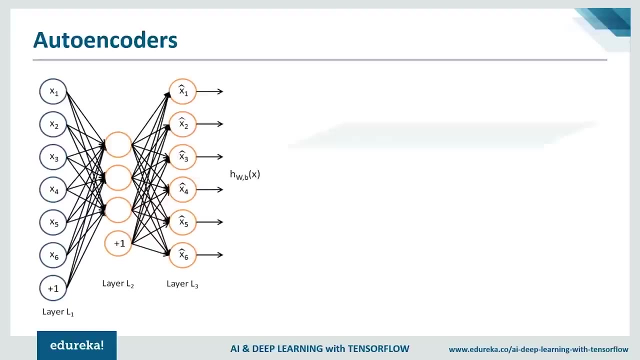 This means that we want the output to be as close to input as possible, and auto encoder neural network is basically an unsupervised machine learning algorithm that applies back propagation, setting the target values to be equal to the inputs. So let's have a look at some of the key features about auto encoders. 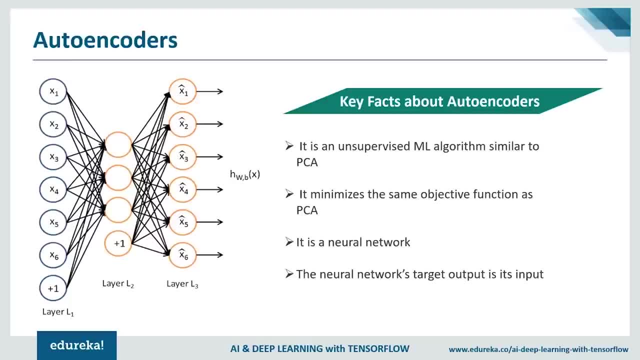 So it is an unsupervised machine learning algorithm that is similar to PCA but minimizes the same objective function, and auto encoder is a neural network whose target output is its input. auto encoders, Although, is quite similar to PCA, But they are more flexible when compared to the other auto encoders. 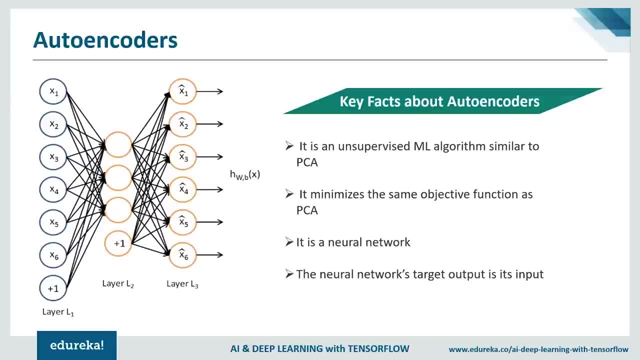 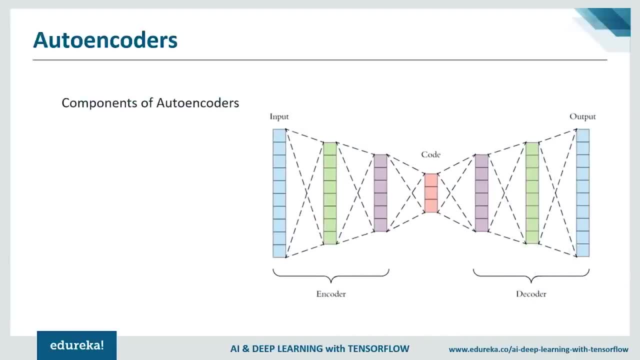 can represent both linear and nonlinear transformation in encoding, but PCA can only perform linear transformation. So now let's have a look at the components of auto encoders. So there are basically three main layers. The first one is the encoder, then code and decoder, the first component. 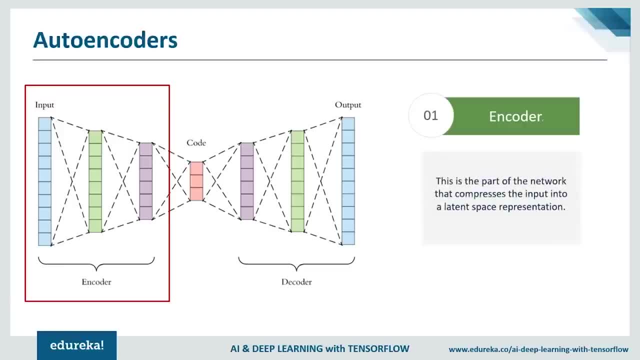 that is, the encoder is the part of the network that compresses the input into a latent space representation. The encoder layer encodes the input image as a compressed representation in a reduced dimension. Now the compressed image typically looks garbled, nothing like the original image. the next component represents the latent. 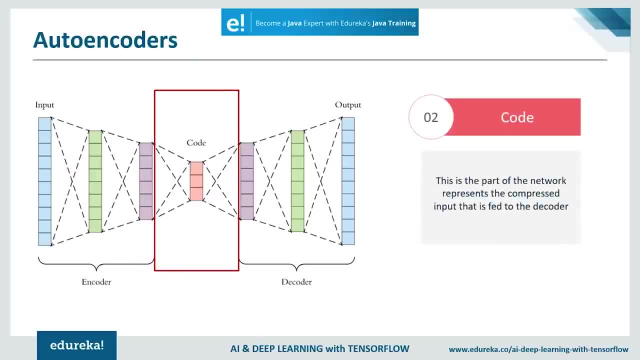 space. now code is the part of the network that represents the compressed input fed to the decoder. The third component is a decoder. Now this layer basically decodes the encoded image back to the original dimension. The decoded image is a lossy reconstruction of the original image. 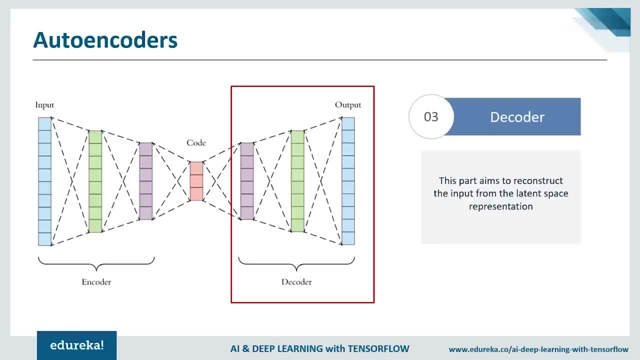 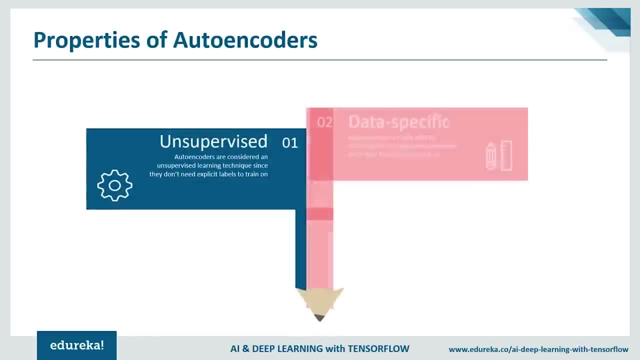 Now it reconstructs the input from the latent space representation. So now let's talk about some of the properties of auto encoders. They are only able to compress data similar to what they have been trained on an auto encoder which has been trained on human. 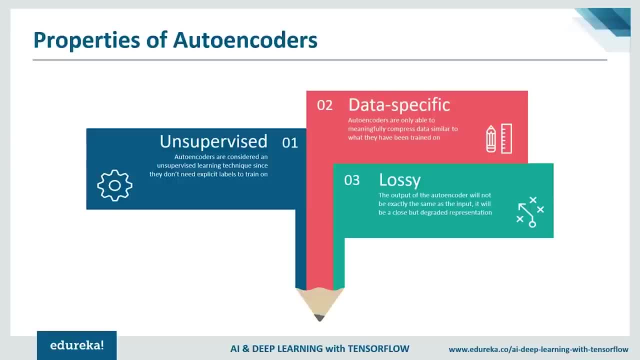 faces would not be performing well with images of modern buildings. This improvises the difference between the auto encoders and mp3 kind of compression algorithms, which only hold assumptions about sound in general but not about specific types of sounds. auto encoders are lossy. 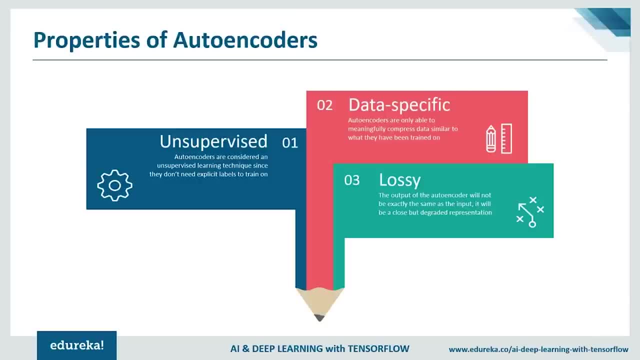 which means that the decompressed outputs will be degraded compared to the original inputs, just like what you see in jpeg or mp3. now, if you have appropriate training data, it is easy to train specialized instances of the algorithm that will perform well on a specific type of input. now, 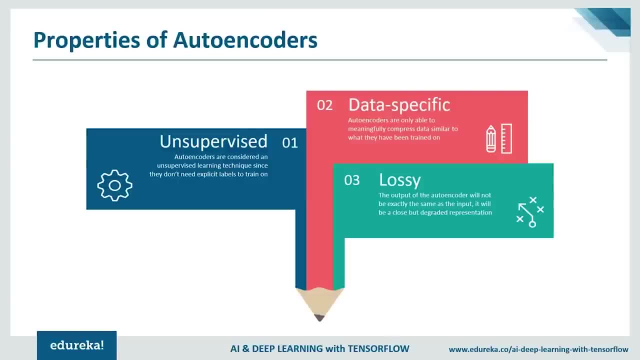 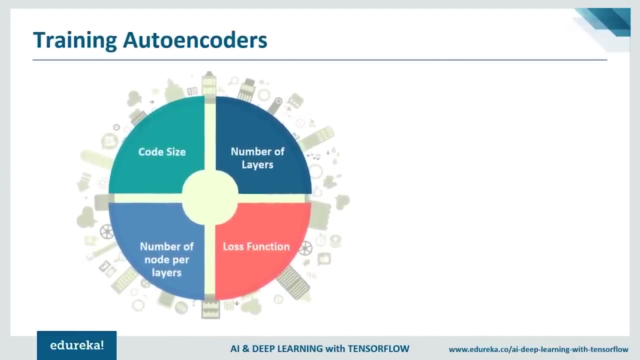 it doesn't require any new engineering. additionally, in almost all context Where the term auto encoder is used, the compression and decompression functions are implemented with neural networks. So now let's have a look at the training of an auto encoder. Now There are four hyper parameters that we need to set before training. 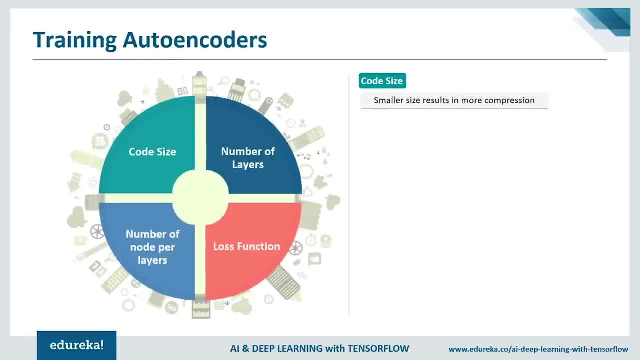 them. The first one is the code size. The code size represents the number of notes in the middle layer. smaller size results in more compression. The second parameter is the number of layers. now the auto encoder can be as deep As we want it to be. we can have two or more layers in both. 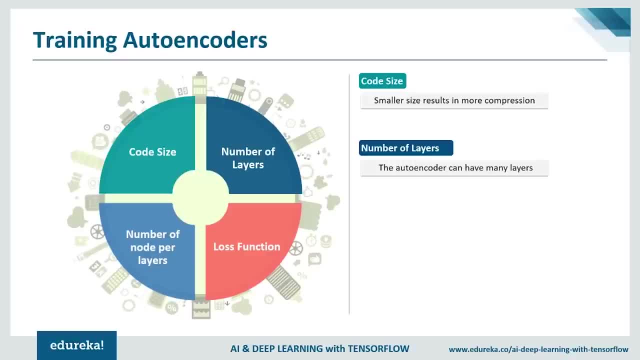 the encoder and decoder, without considering the input and the output. next is the loss function. So we either use mean squared error or binary cross entropy. Now, if the input values are in the range 0 to 1, then we typically use cross entropy. 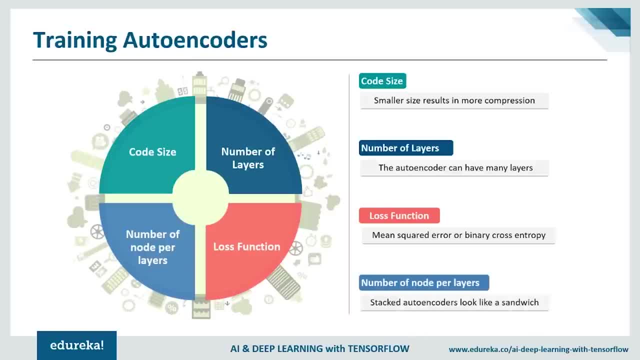 Otherwise we use the mean squared error. next is the number of notes per layer. So the number of nodes per layer decreases with each subsequent layer of the encoder and increases back in the decoder. Also, the decoder is symmetric to the encoder in terms of layer. 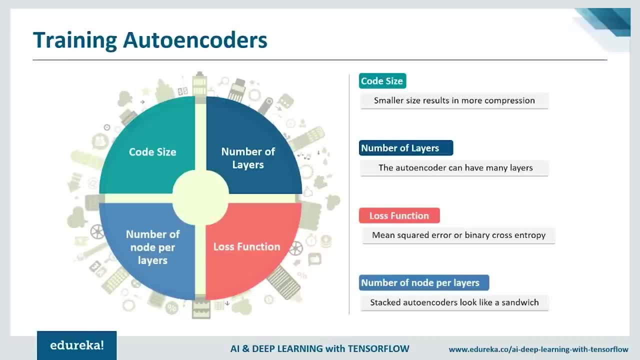 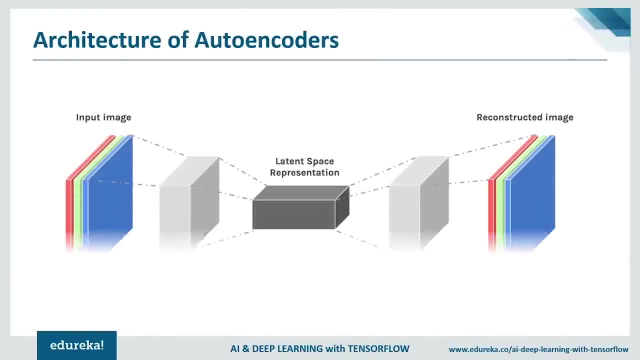 structure, but this is not necessary and we have total control over these parameters. Now let's have a look at the architecture of an auto encoder and have a deeper insight about the hidden layers. So in an auto encoder, we add a couple of layers in between. 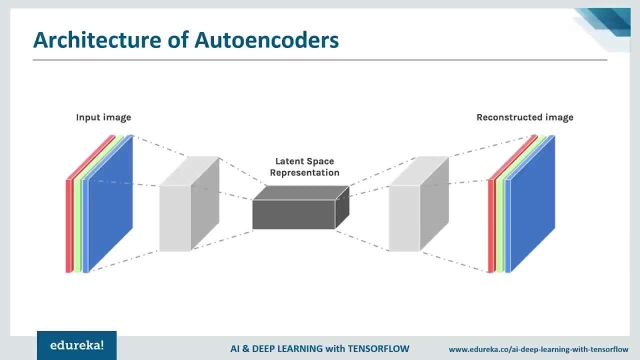 the input and output, and the sizes of these layers are smaller than the input layer. Let's say the input Vector has a dimensionality of n, which means that the output will also have a dimensionality of n. now we make the input go through a layer of size P, where the value 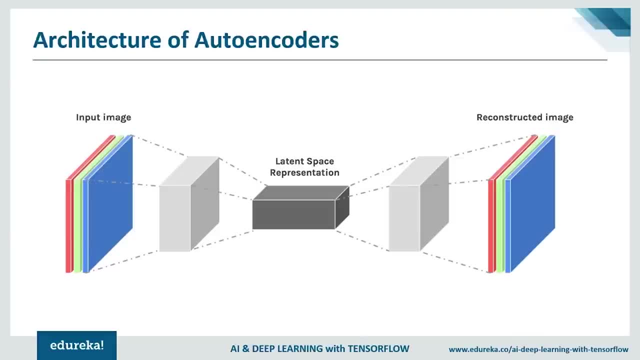 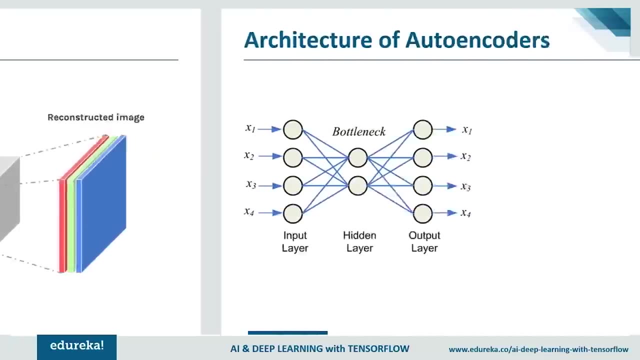 of P is less than n and we ask it to reconstruct the input. Now the auto encoder receives unlabeled input, which is then encoded to reconstruct the input. one important part of the auto encoders is the bottleneck. Now the bottleneck approach is a beautifully elegant approach. 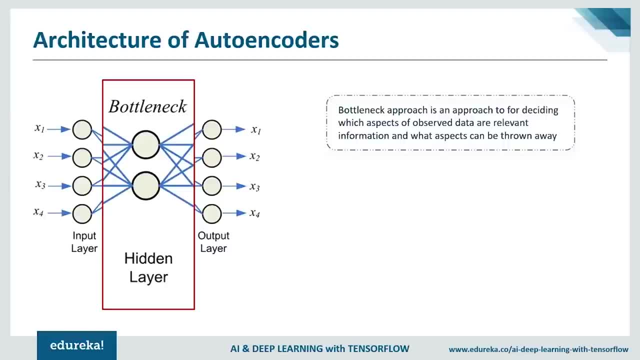 to a representation learning specifically for deciding which aspects of observed data are relevant information and what aspects can be thrown away. It does this by balancing two criteria, that is, the compactness of representation, measured as the compressibility- number of bits needed to store the representation, and the second 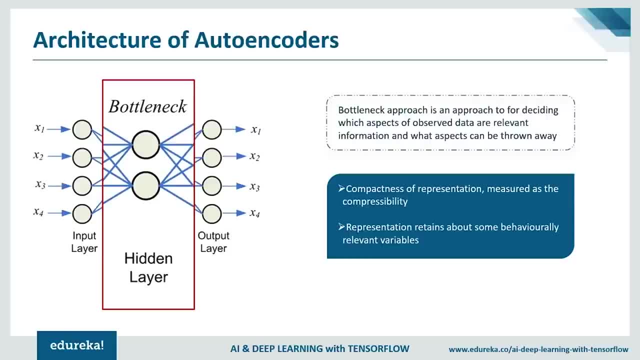 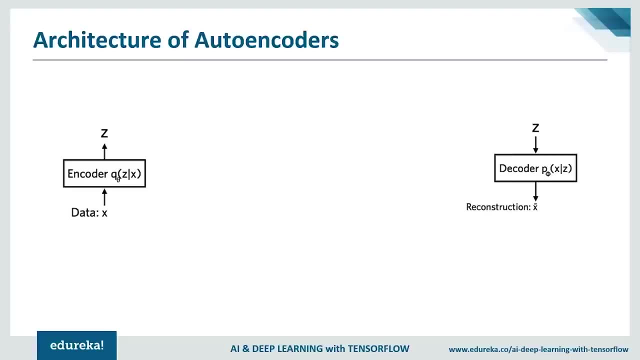 one information the representation retains about some behaviorally relevant variables. Now it assumes we know what the behaviorally relevant variables are and how they are, Are related to observe data, or at least we have to have data to learn or approximate the joint distribution between observed 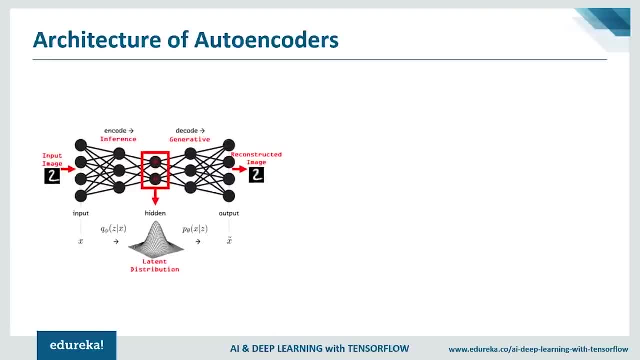 and relevant variables. Now let's have a detailed description about the encoder. The encoder is a neural network. Its input is a data point X, its output is a hidden representation, Z, and it has weights and biases- Theta. now, to be concrete, Let's say X is a 28 by 28 pixel photo of a handwritten number. 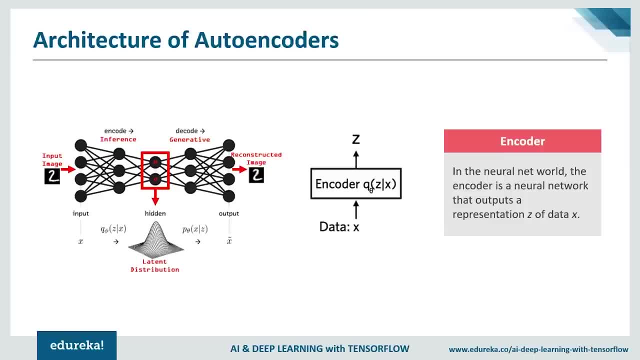 the encoder Encodes the data, which is 784 dimensional, into a latent representation space Z, which is much less than 784 dimensions. Now, this is typically referred to as a bottleneck, because the encoder must learn an efficient compression of the data into this lower dimensional space. 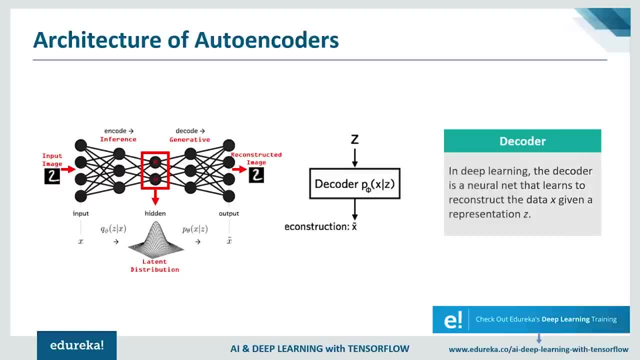 Next is the decoder. The decoder is another neural net. its input is the representation Z. it outputs the parameters to the probability distribution of the data and has weights and biases as five, running with a handwritten digit example. Let's say the photos are black and white. 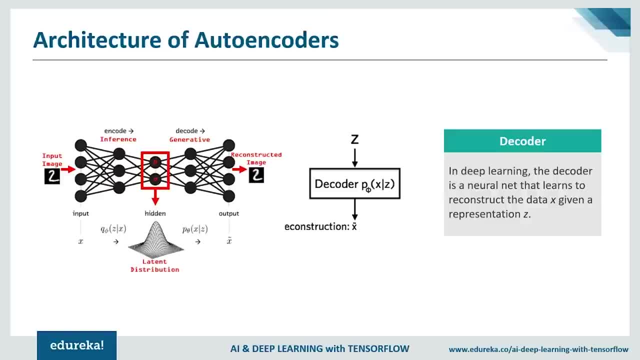 and represent each pixel as 0 or 1. now the probability distribution of a single pixel can be then represented using a Bernoulli distribution. the decoder gets as input the latent representation of a digit Z and outputs 784 Bernoulli parameters, one for each of the 784 pixels in the image. the decoder 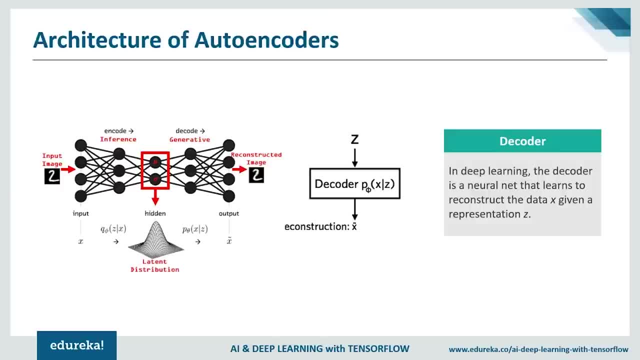 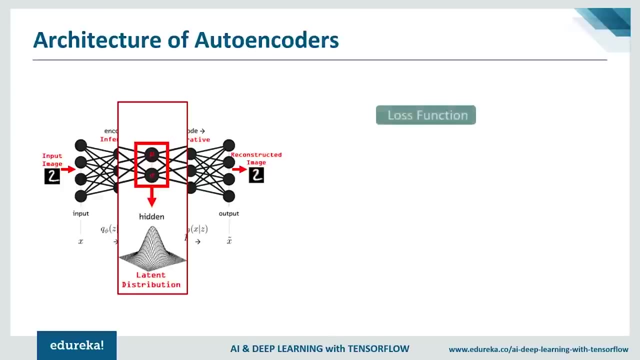 The decoder decodes the real valued numbers in Z into 784 real valued numbers between 0 and 1. information is lost because it goes from a smaller to a larger dimensionality. Now how do we find out how much information is lost? The loss function equation helps us find the value. 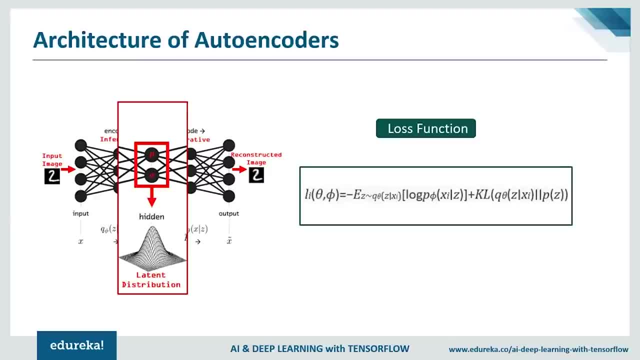 Now this measure tells us how effectively the decoder has learned to reconstruct an input. image X, given its latent representation. Z. The loss function of the variational autoencoder is the negative log likelihood with a regularizer, because there are no global representations that are shared by all data points. 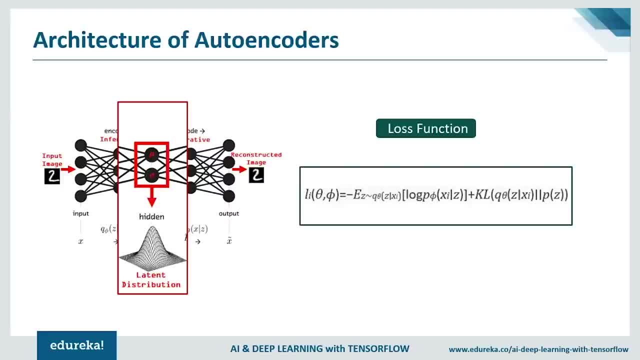 We can decompose the loss function into only terms that depend on a single data point. So the loss function, the first term is the reconstruction loss or expected negative log likelihood of the i-th data point. the expectation is taken with respect to the encoders distribution. 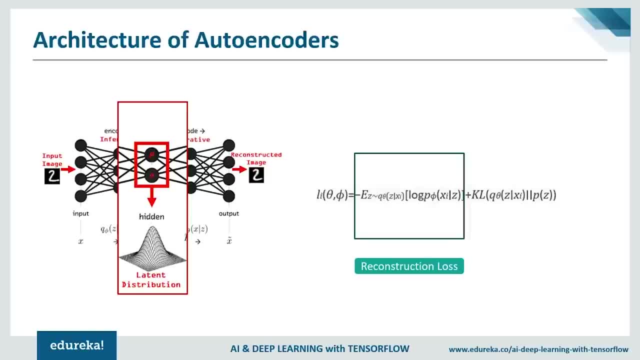 over the representation. This term encourages the decoder to learn to reconstruct the data. Now, if the decoders output does not reconstruct the data Well, it will incur a large cost in the loss function. The second term is a regularizer that we throw in. this is: 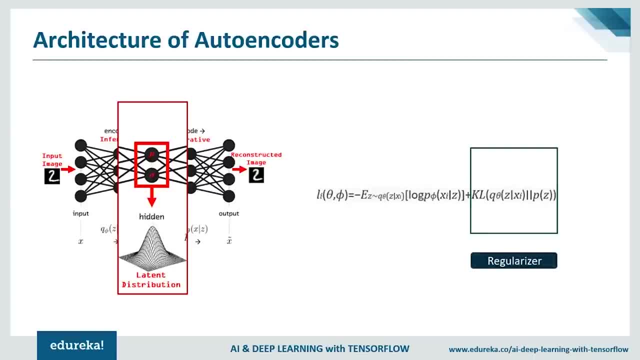 the callback labeler. divergence between the encoders distribution. Now this divergence measures how much information is lost when using Q to represent P. It is one measure of how close Q is to P if the encoder is encoder outputs representations said that are different than those from a standard, normal distribution. 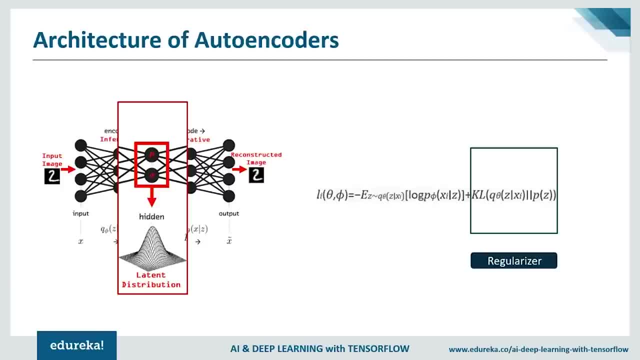 It will receive a penalty in the loss. this regularizer term means keep the representation Z of each digit sufficiently diverse. If we didn't include the regularizer, the encoder could learn to cheat and give each data point a representation in a different region of Euclidean space. 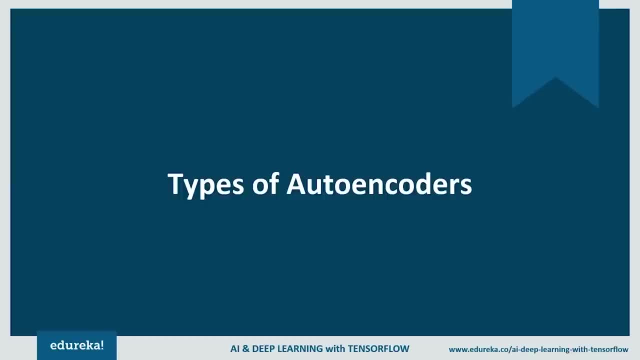 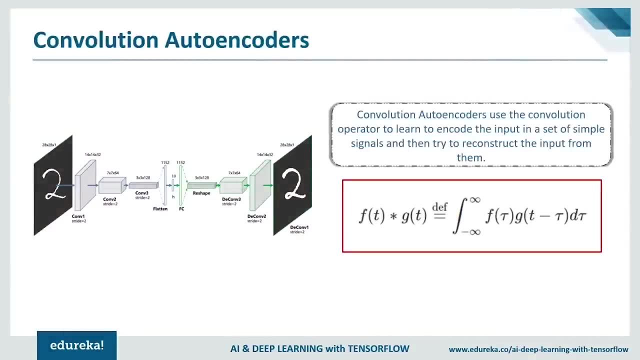 So now let's move on and have a look at the different types of autoencoders. The convolution An operator allows filtering an input signal in order to extract some parts of its content. autoencoders, in their traditional formulation, do not take into account the fact that the signal can be seen as a sum of other signals. 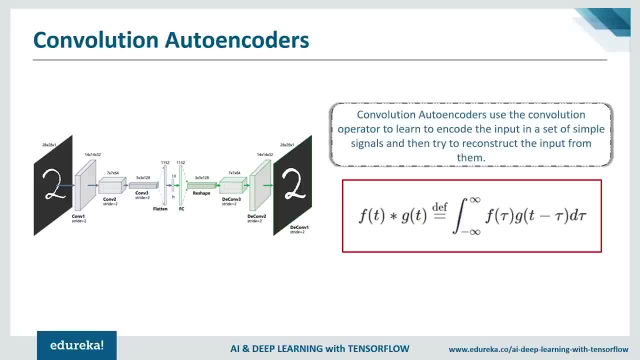 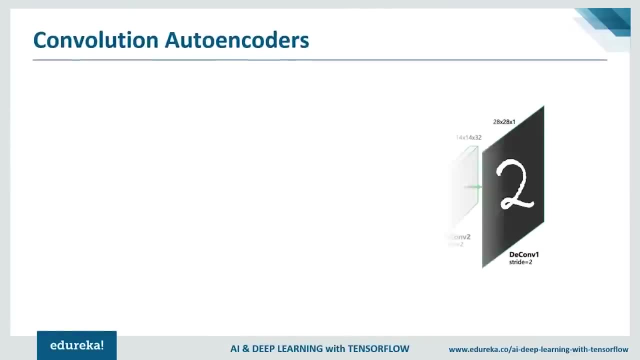 convolution. autoencoders use the convolution operator to exploit this observation. Basically, they learn to encode the input in a set of simple signals and then try to reconstruct the input from them, modify the geometry or the reflectance of the image. Now the encoder consists of three: convolutional, less the number. 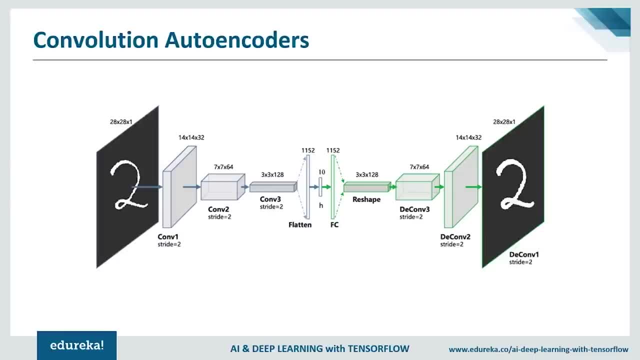 of features changes from one- the input data- to 16 for the first convolutional layer, then from 16 to 32 for the second layer and finally from 32 to 64 for the final convolutional layer. now, while transacting from one convolutional layer to another, 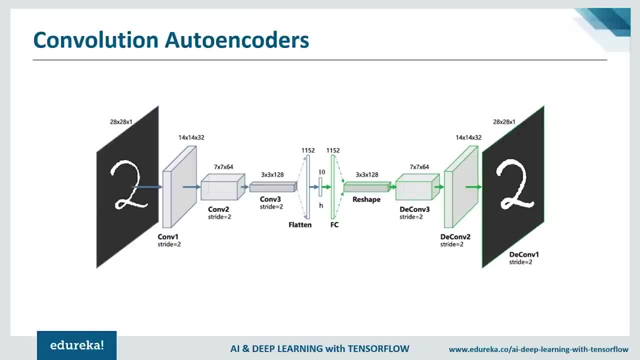 the shape undergoes an image compression. So the decoder consists of three deconvolution layers, arranged in sequence. for each deconvolution operation We reduce the number of features to obtain an image that must be the same size as the original image. So, in addition to reducing the number of features, deconvolution 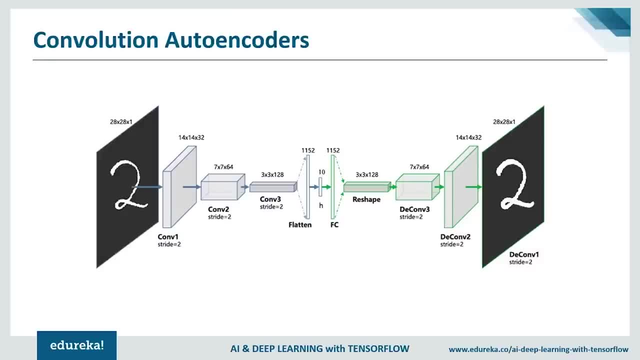 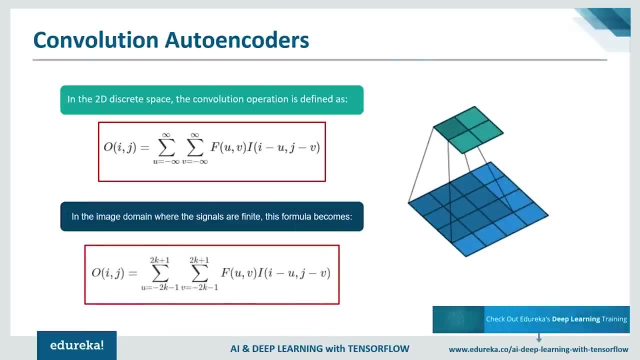 involves a shape transformation of the images. a convolution is the general continue case defined as the integral of the product of two functions, after one is reversed and shifted as a result, a convolution produces a new function and it is a commutative operation, now in the 2d discrete space. 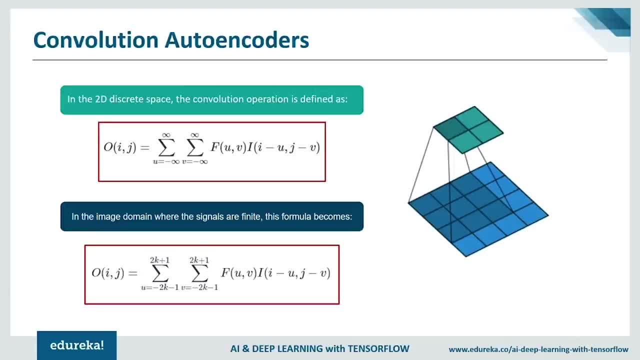 The convolution operation is defined as the following equation: and in the image domain, where the signals are finite, this formula becomes as such: where o of i, j is the output pixel in position i, n, j and 2 k plus 1 is the side of a square, that is the odd. 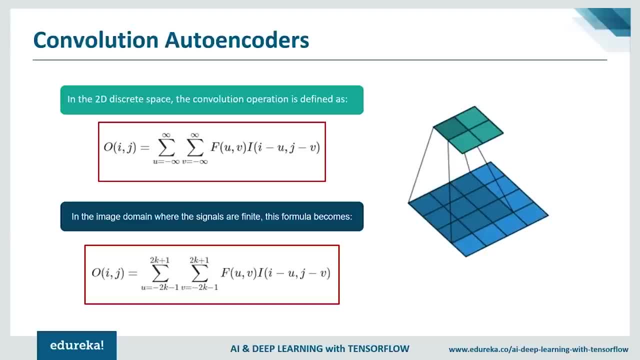 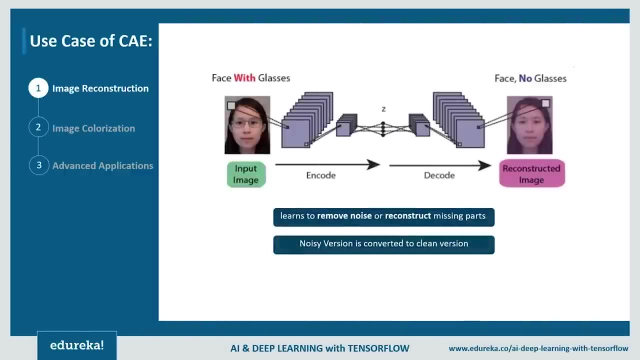 convolutional filter. F is the convolutional filter and I is the input image. Now this operation is done for every location of the input image that completely overlaps with the convolution Filter. now let's see the use cases of convolution auto encoders. The first one is image reconstruction. 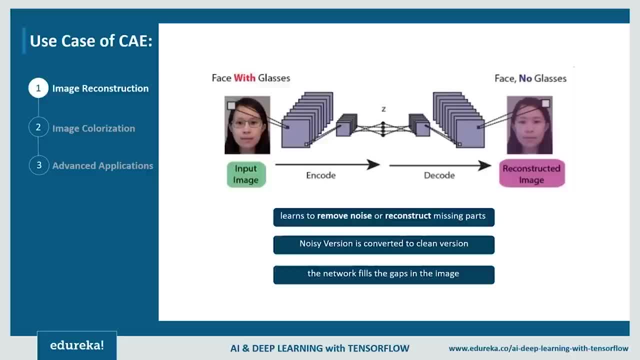 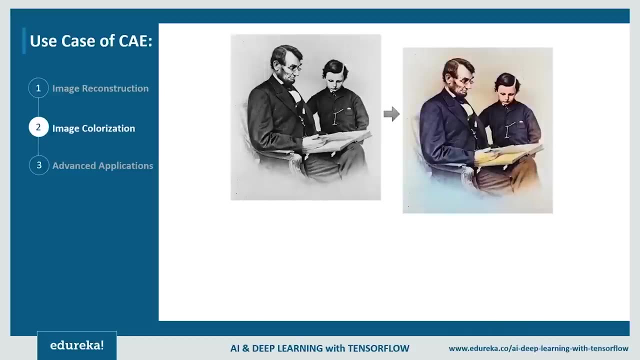 Now the convolution auto encoders learn to remove noise from a picture or reconstruct the missing parts. So the input noisy version becomes the clean output version. the network also fills the gap in the image. next is image colorization. now convolution auto encoders Maps, circles and squares from an image to the same image. 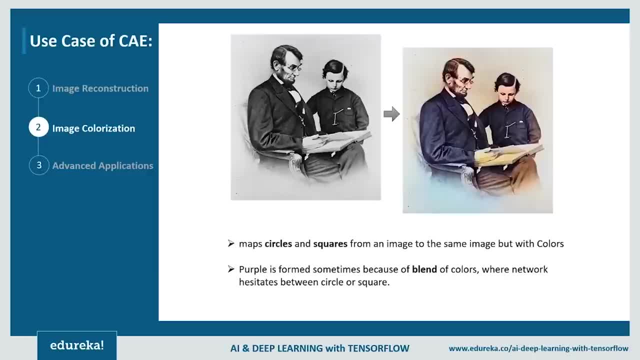 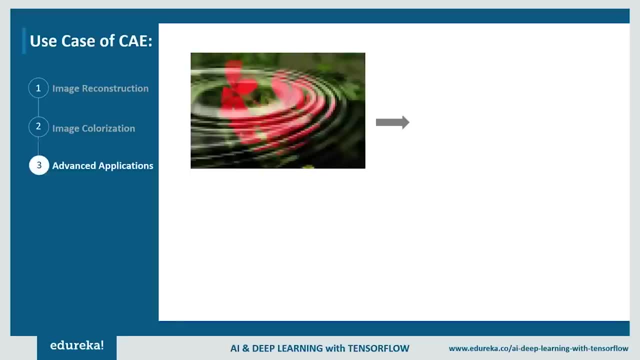 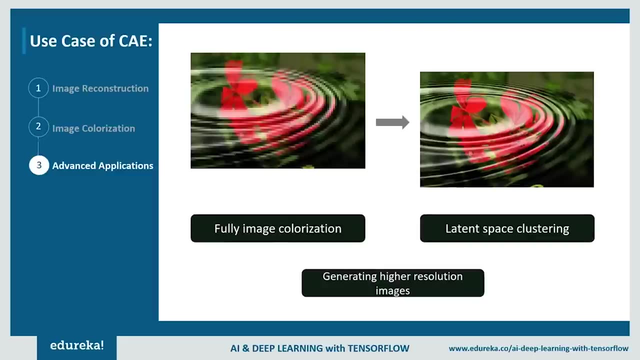 But with red and blue respectively. purple is formed sometimes because of blend of colors where Network hesitates between circle or square. next up are some of the advanced applications, such as fully image colorization, latent space clustering and generating higher resolution images. moving on to the next type of auto, 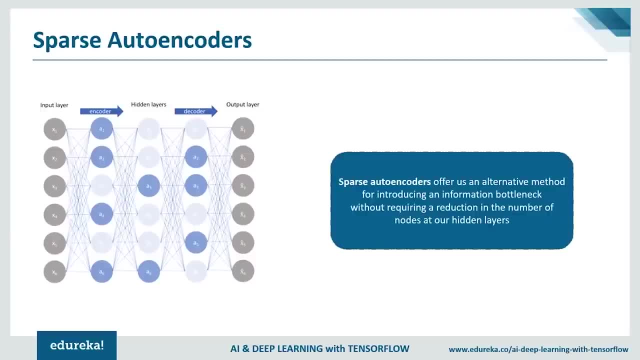 encoders. sparse auto encoders offer us an alternative method for introducing an information bottleneck without requiring a reduction In the number of notes at our hidden layers. rather, we will construct our loss function such that we penalize activations within a layer. So for any given observation, we will encourage our network. 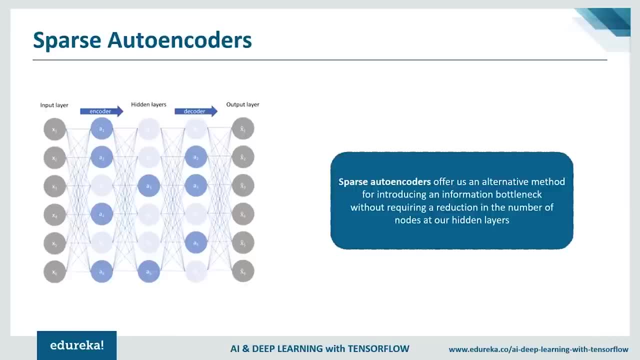 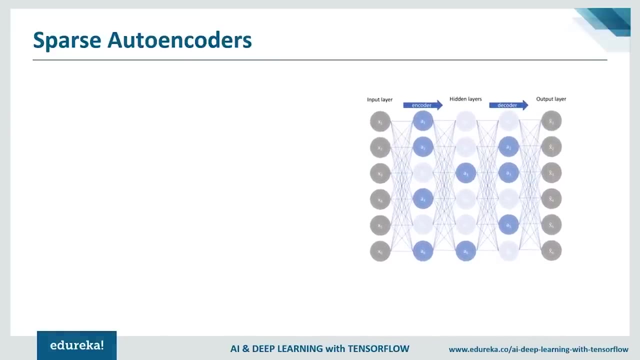 to learn an encoding and decoding which only relies on activating a small number of neurons. Now, this is a different approach towards regularization, as we normally regularize the weights of a network, not the activations. now there are two main ways by which we can impose: 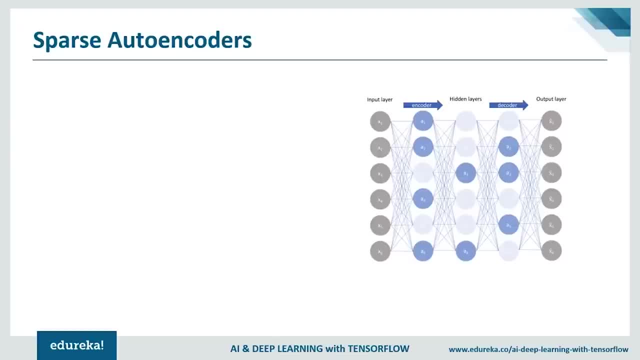 this parsity constraint. both involve measuring the hidden layer activations for each training batch and adding some term to the loss function in order to penalize excessive activations. The first one is the l1 regularization. Now we can add a term to our loss function that penalizes the 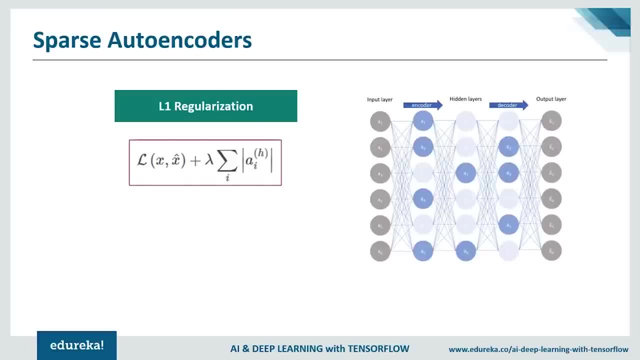 absolute value of the vector of activations a in layer H for observation. I now scaled by a tuning parameter, lambda. the next one is the KL divergence. in essence, KL divergence is a measure of the difference between two probability distributions. We can define a sparsity parameter row which denotes the average. 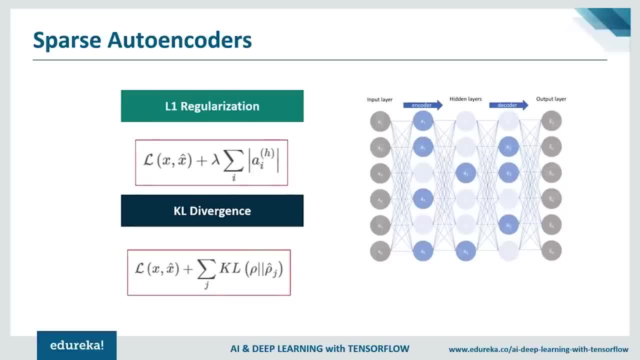 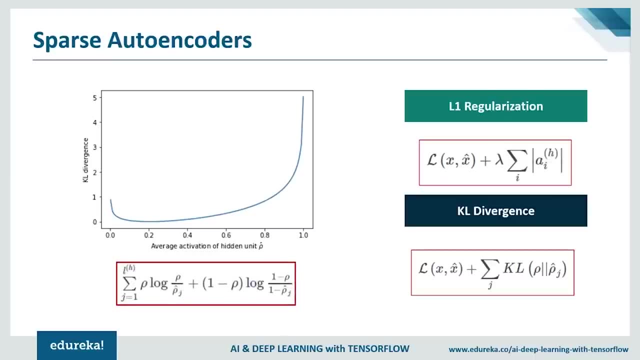 activation of a neuron over a collection of samples. This expectation can be calculated in the following equation: Now the KL divergence between two Bernoulli distributions can be written as such. now This loss term is visualized below: for an ideal, distribution of row equals to zero. 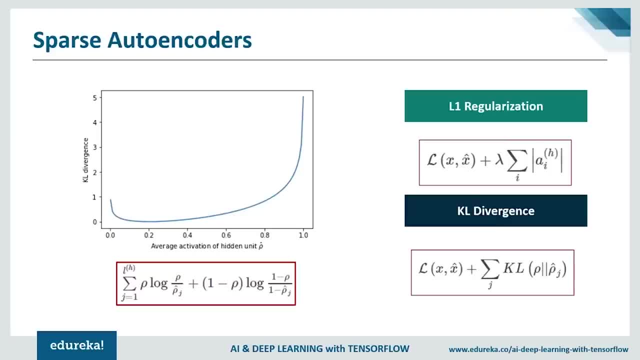 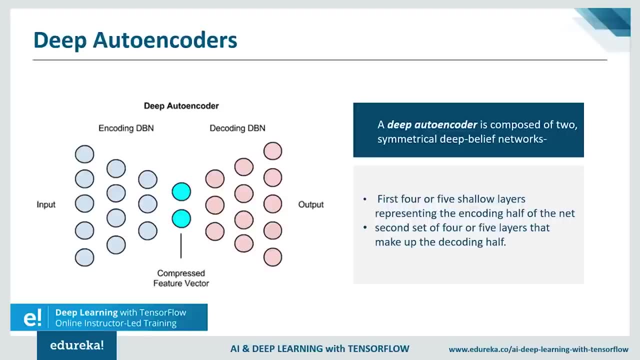 Point two, corresponding with the minimum penalty at this point. The next one is the deep Auto encoders. Now, the extension of the simple Auto encoder is basically the deep Auto encoders. Now, the only difference to its simpler counterpart is number of hidden layers. 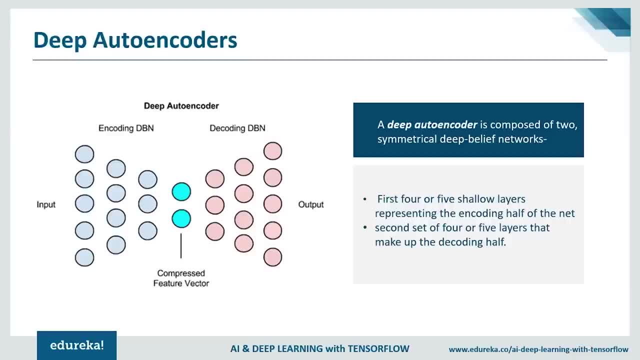 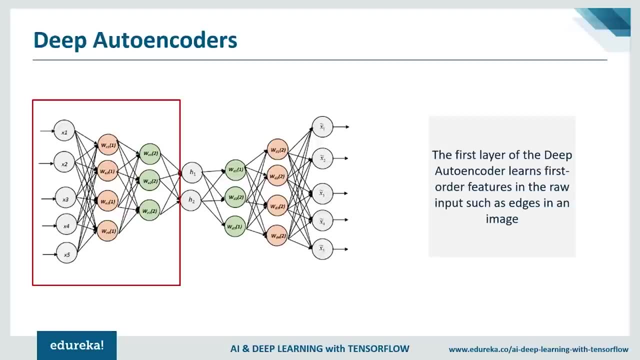 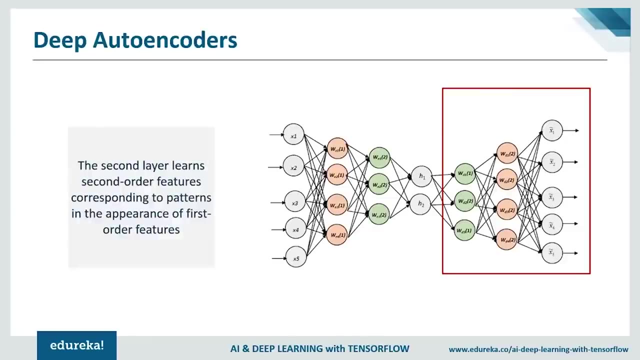 The additional hidden layers enable the Auto encoder to learn mathematically more complex underlying patterns in the data. the first layer of the deep Auto encoder may learn first order features in the raw input. The second layer may learn second order features corresponding to patterns in the appearance of first order features. deeper layers: 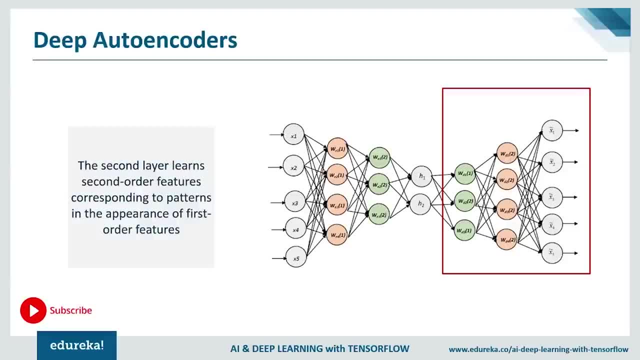 of the deep Auto encoder tend to learn even higher order features. to put everything together, We need additional layers to be able to handle more complex data, such as the data we use in collaborative filtering. So let's have a look at some of the use cases of deep Auto encoders. 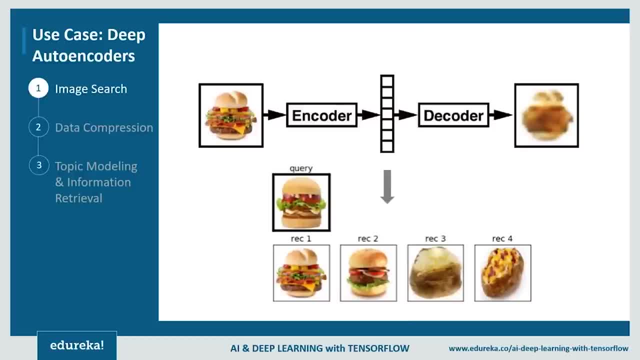 The first one is image search. deep Auto encoders are capable of compressing images into 30 number vectors. image search therefore becomes a matter of uploading an image, which the search engine will then compress to 30 numbers and compare that vector to all the others in its index vectors containing. 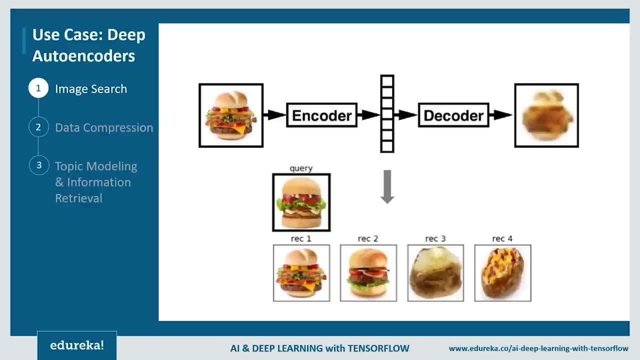 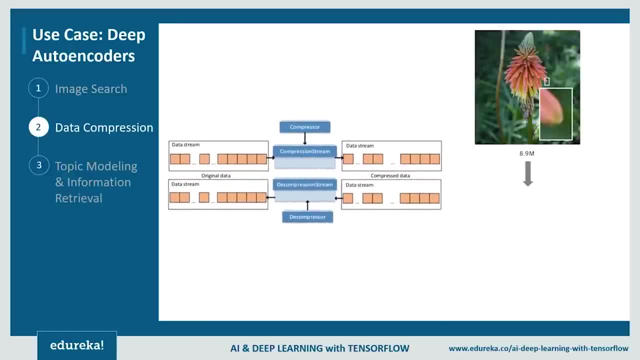 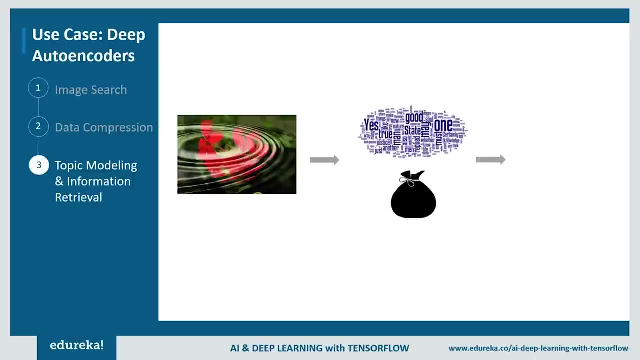 similar numbers will be returned for the search query and translated into their matching image. a more general case of image compression is data compression, and deep Auto encoders are useful for semantic hashing. Next up is the topic modeling and information retrieval. So deep Auto encoders are useful in topic modeling or statistically. 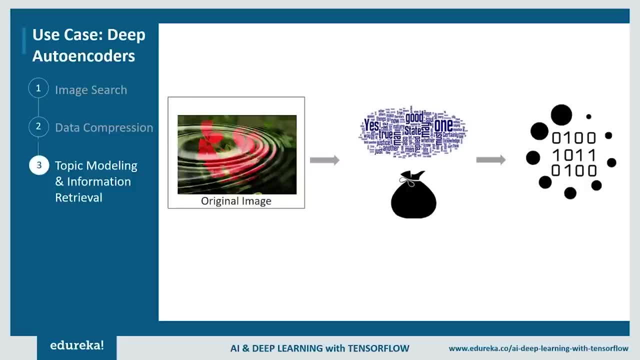 modeling abstract topics that are distributed across a collection of documents. in brief, each document in a collection is converted to a bag of words and those word counts are scaled to decimals between 0 and 1, which may be thought of as the probability of a word occurring in the document. 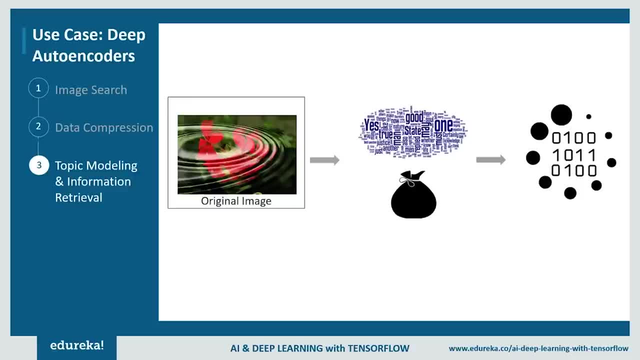 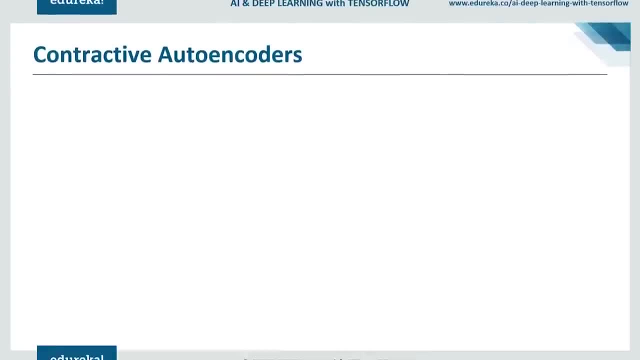 For example, one document could be the question and other others could be the answers. now a match the software would make using vector space measurements. The next type of Auto encoders is the contractive Auto encoders. one would expect that for very similar inputs, the learned. 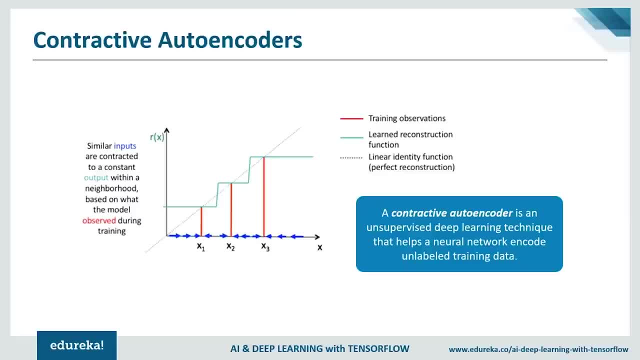 encoding would also be very similar. We can explicitly train our model in order for this to be the case by requiring that the derivative of the hidden layer activations are small with respect to the input. In other words, for small changes to the input, We should still maintain a very similar encoded state. 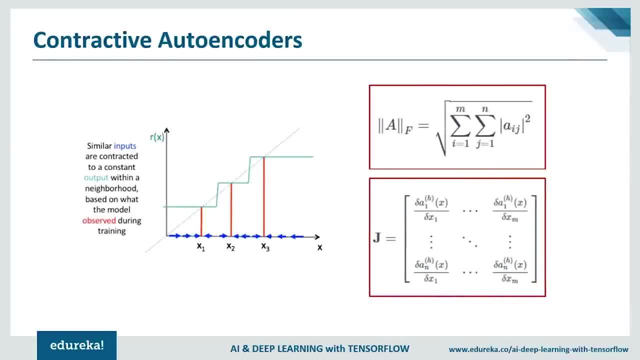 Now This is quite similar to a denoising Auto encoder, in the sense that these small perturbations to the input are essentially considered noise and that we would like our model to be robust against noise. Now we can accomplish this by constructing a loss term, which 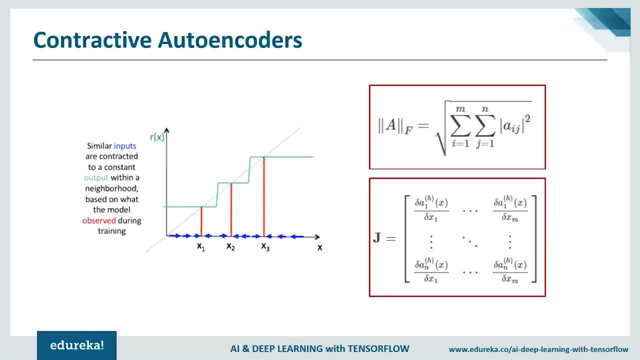 penalizes large derivatives of our hidden layer activations with respect to the input, training examples, essentially penalizing instances where a small change in the input Leads to a large change in the encoding space. Now, in fancier mathematical terms, We can craft our regularization loss term as the squared. 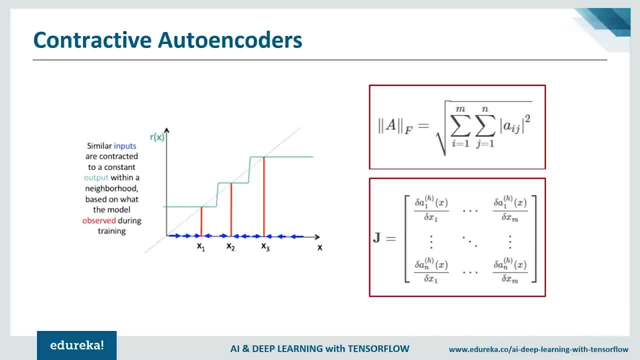 Frobenius norm of the Jacobian mattress. J for the hidden layer activations. with respect to the input observations, a Frobenius norm is essentially an L2 norm for a matrix and the Jacobian matrix simply represents all first-order partial derivatives of a vector valued function. now for M- observations and n- hidden. 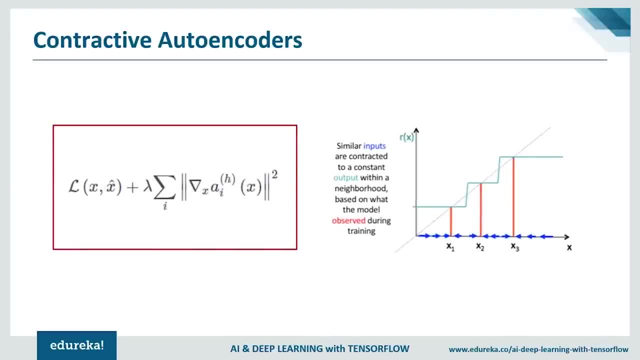 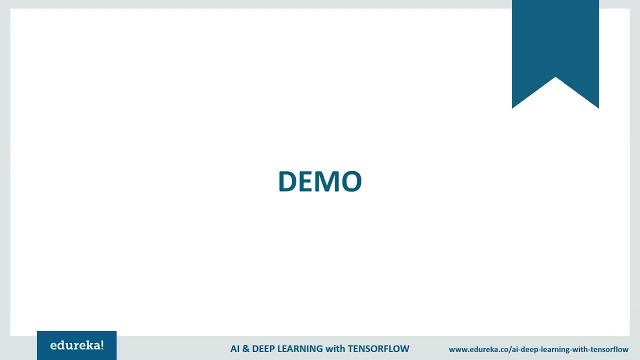 layer nodes. We can calculate the values using the following equations: So now that we know the various types of Auto encoders, let's have a look at how it actually works. So let's see the code that provides us with a reconstructed image. 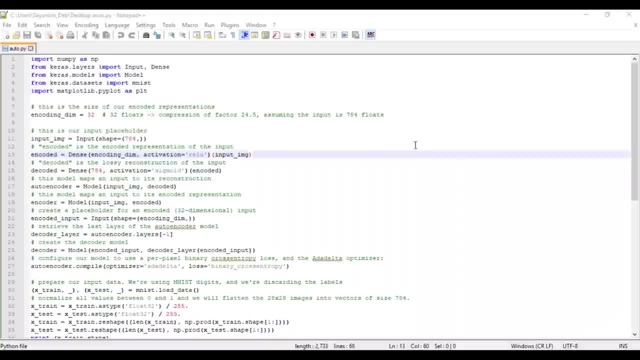 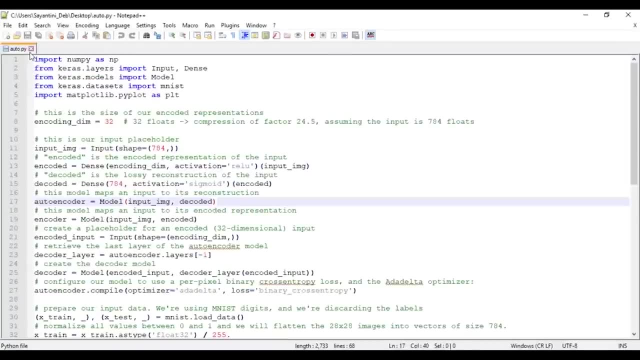 So this is the code for Auto encoder that generates a similar output as the input with reduced dimensions. The packages that are needed to be pre-installed are numpy, Keras and matplotlib. So first we define the size of our encoded representations. the encoded representation. 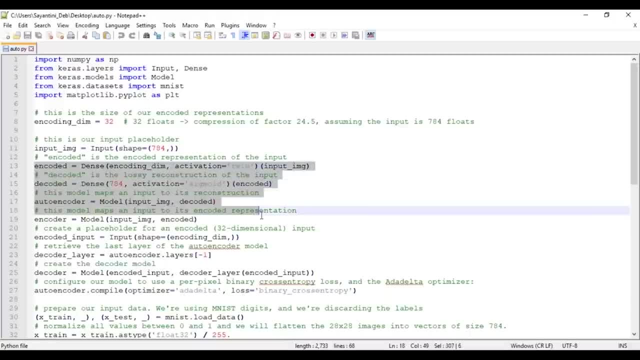 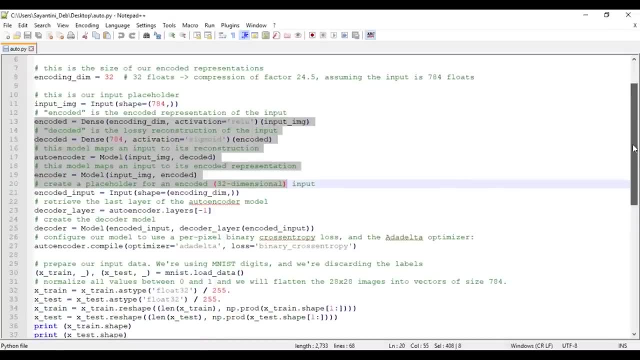 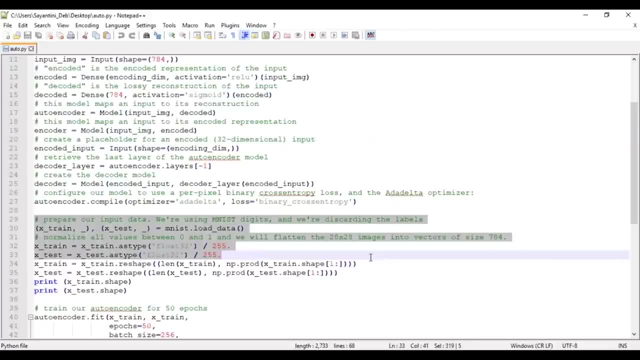 of the input is declared as encoded, while the lossy reconstruction of the input is declared as decoded. The input is then mapped to its encoded representation in order to create the decoder model. Next, we have to prepare our input data and normalize all the values between 0 and 1. the 28 by 28 images will be then flatted. 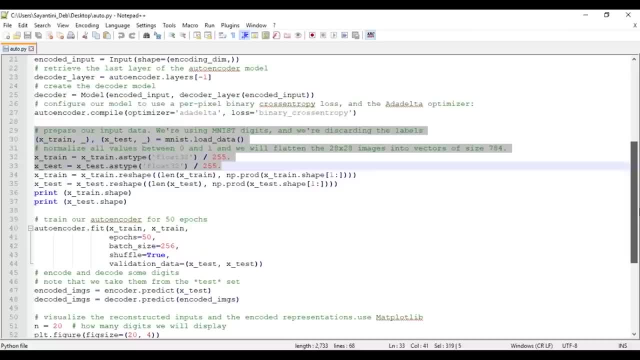 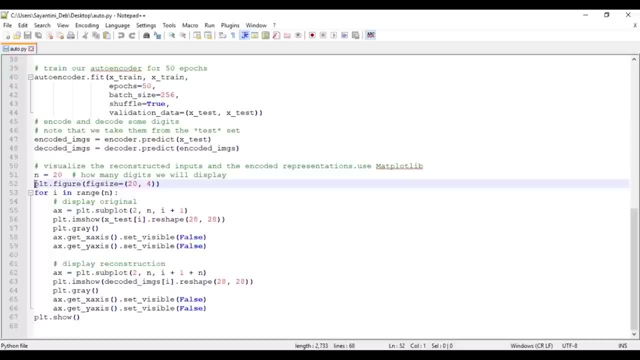 into vectors of size 784.. Now, once the data is trained And tested- the Auto encoder is trained- It will take certain values from the test set, encode and decode them. now for the visualization of the reconstructed inputs and the encoded representations: It is done with the help of matplotlib library. 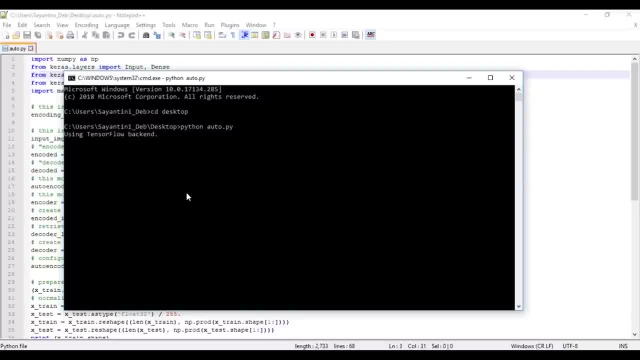 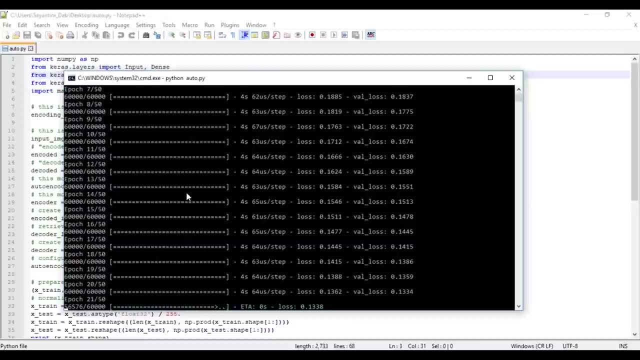 So let's see what happens when we execute this code. So now we can see that the data is being trained and tested, and this will take a few minutes to complete. Now, once we are done with the training of the data, we will have an original image and a reconstructed image as our output. 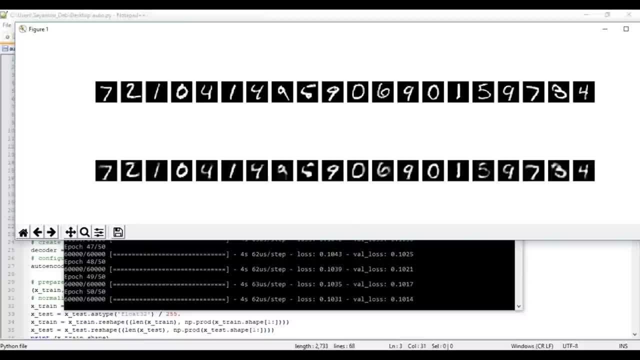 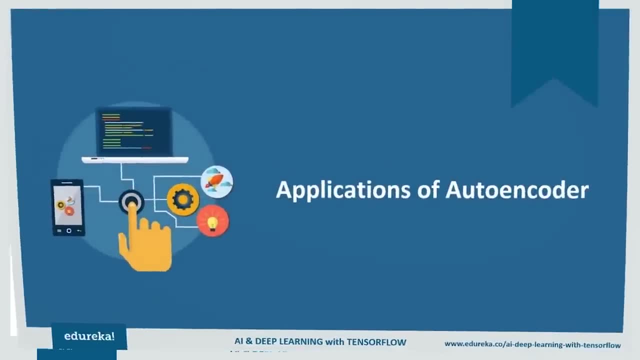 Our output will look like this. So the first row shows the original input image and the second row shows the reconstructed image with reduced dimensions. So now we have seen how an autoencoder actually works and how it provides us a reconstructed image. So now let's move on to some of 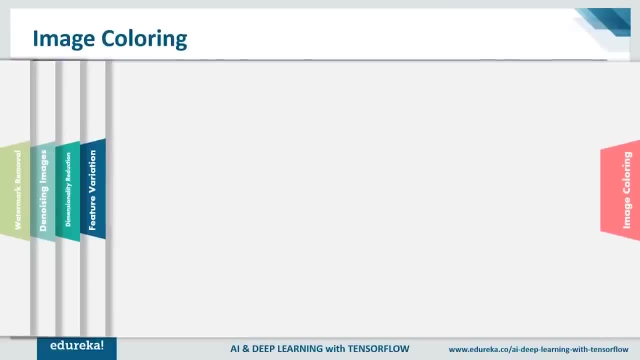 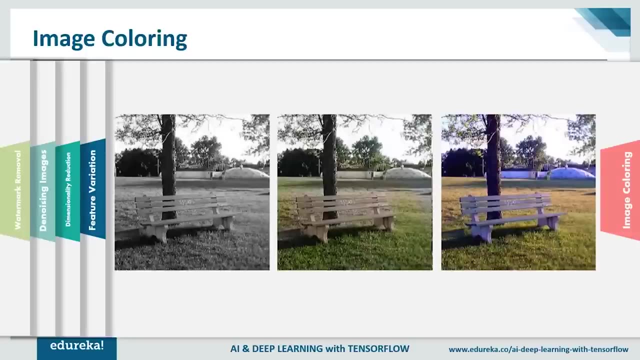 Applications of autoencoders. now, autoencoders are used for converting any black and white picture into a colored image. depending on what is in the picture, It is possible to tell what the color should be. For example, the leaves of trees are generally green. 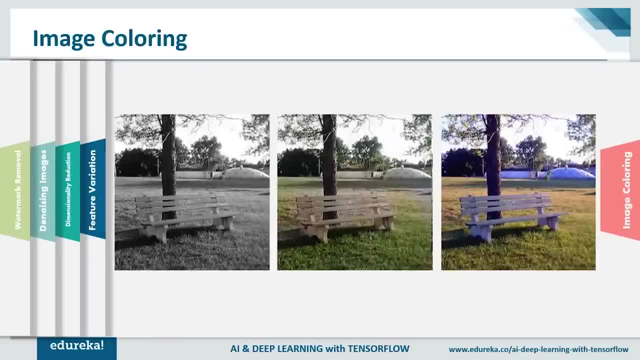 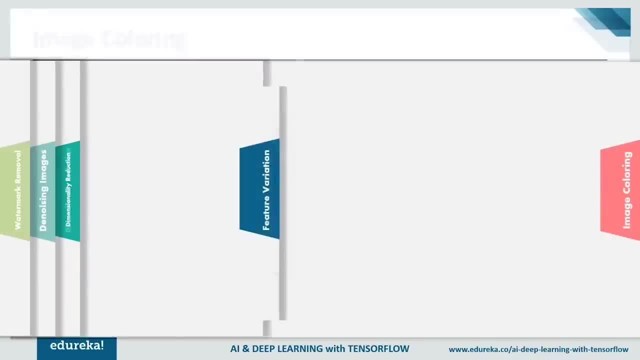 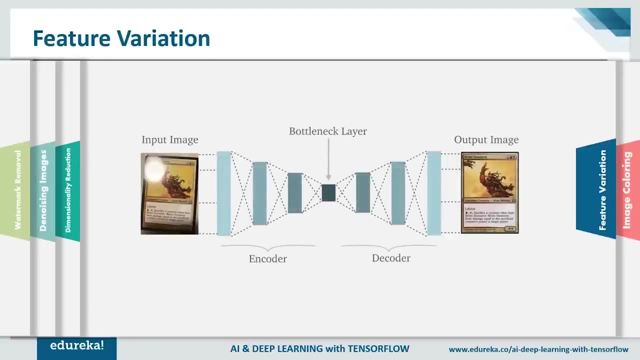 The sky is blue and the clouds are white, So all that is needed to be done is to make a computer be able to do this, and that is where autoencoders step in. the next application is the feature variation. It basically extracts Only the required features of an image and generates the output. 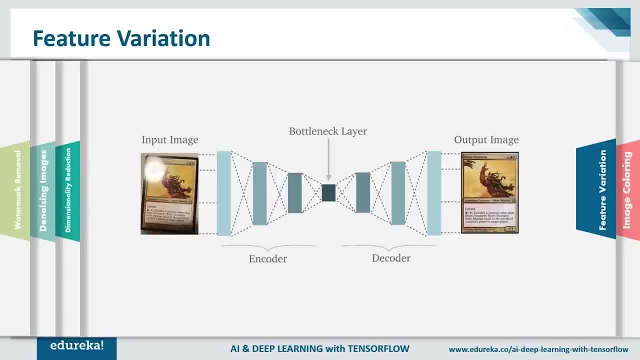 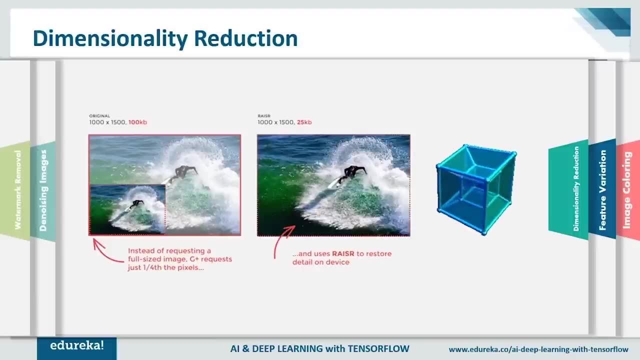 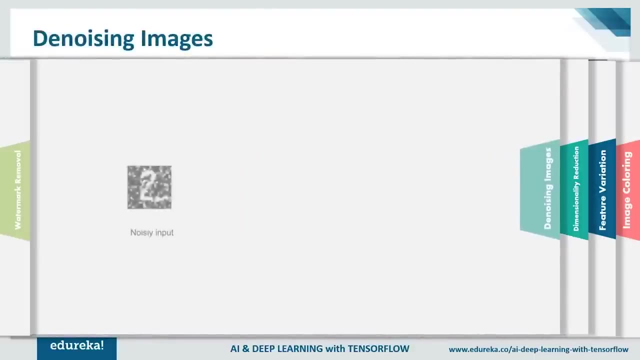 by removing any noise or unnecessary interruption. now, using autoencoders, We receive the same image as the input, but with reduced dimensions. it helps in providing the similar image, along with a reduced pixel value. now, during the training, the autoencoder learns to extract important features from input images and ignores 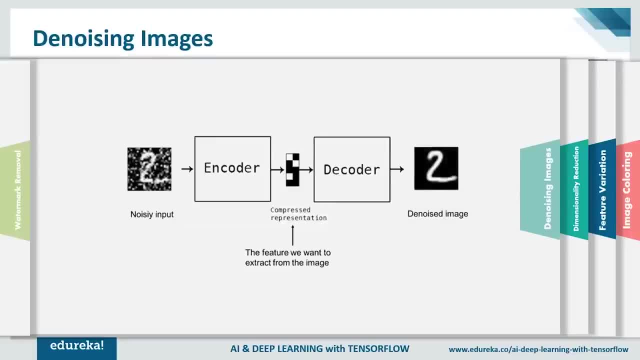 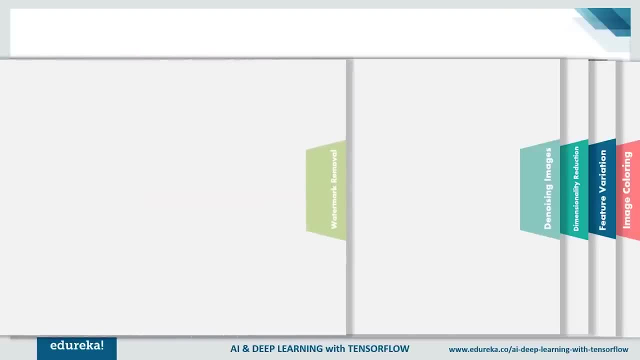 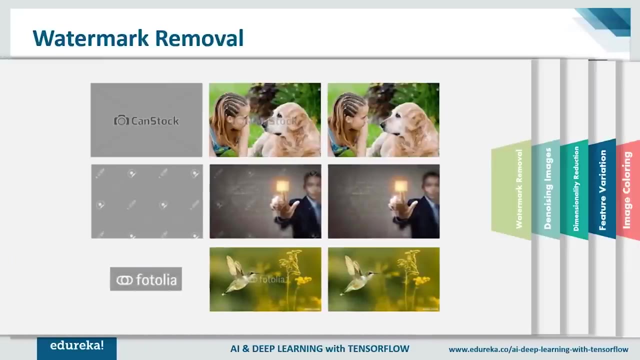 the image noises because the labels have no noises. the input seen by the autoencoder Is not the raw input, but a stochastically corrupted version. now, autoencoders are also used for removing watermarks from images or to remove any object while filming a video or a movie. 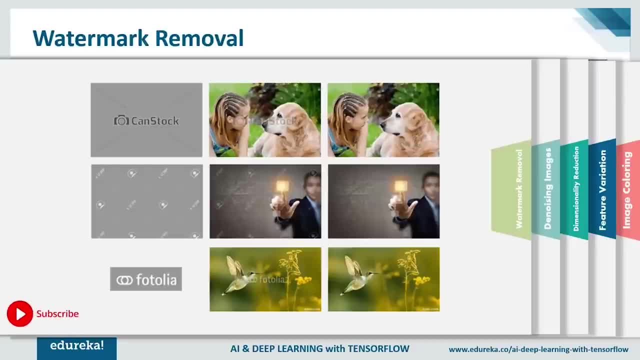 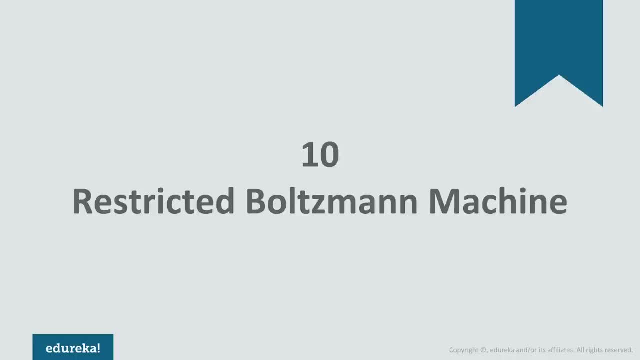 So now we have reached the end of today's session and I hope you have a clear idea about what are autoencoders and how do they actually work in the era of machine learning and deep learning. In today's session, we will learn about how functionality reduction 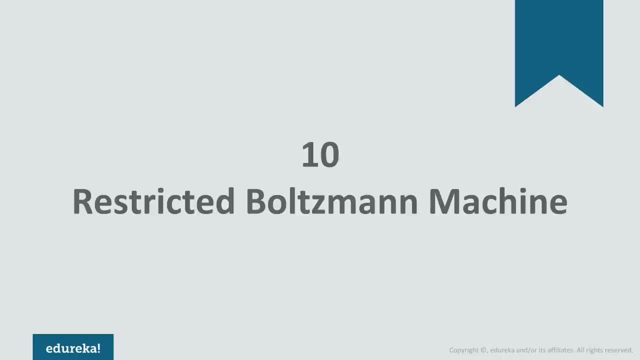 classification, filtering and regression play a very important role in feature selection and extraction. Now we have a number of algorithms that can perform these functions, But what if we have just one single algorithm that can perform all of these together? in today's session, we will learn about 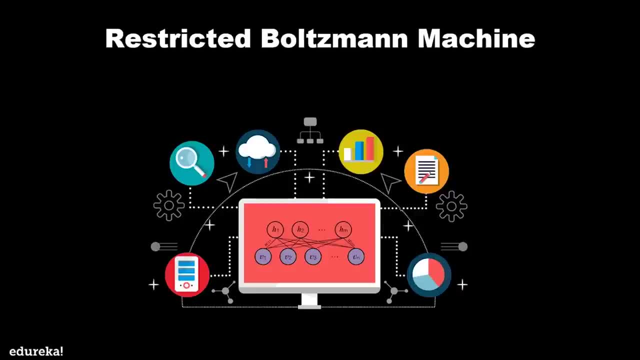 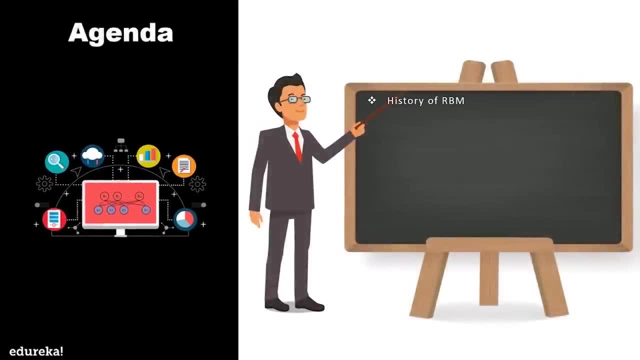 such an algorithm, known as the restricted Boltzmann machines algorithm, and we will see how do they actually work. So let's move on and have a look at today's agenda. So first we will begin with a short history about restricted Boltzmann machines. 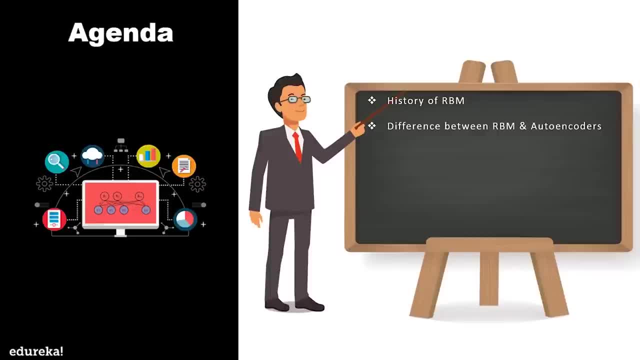 Then we will move on and have a look at the difference between autoencoders and rbm's. next up We will see what are restricted Boltzmann machines and how do they actually work. in the next section We will see one energy based model and probabilistic model. 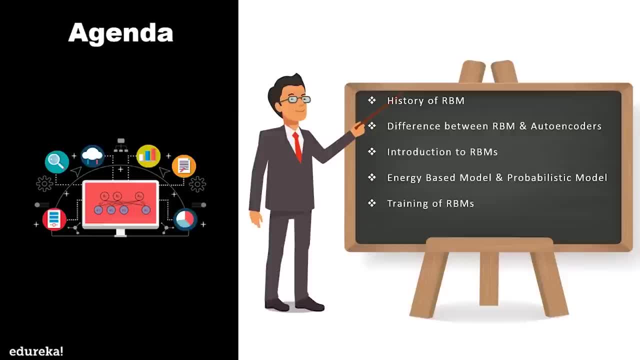 of rbm. moving on, We will have a look at the training of restricted Boltzmann machines. in the final section, We will see one example of restricted Boltzmann machines Using collaborative filtering. So let's begin the session now. restricted Boltzmann machine. 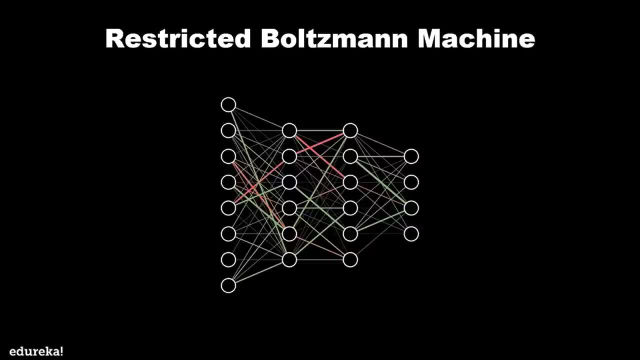 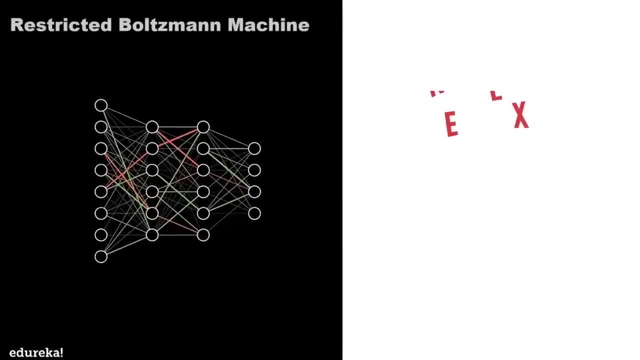 is an undirected graphical model that plays a major role in deep learning framework nowadays. Now it was introduced as harmonium initially, and it gained big popularity in recent years in the context of the Netflix price, where rbm's achieved state-of-the-art performance in 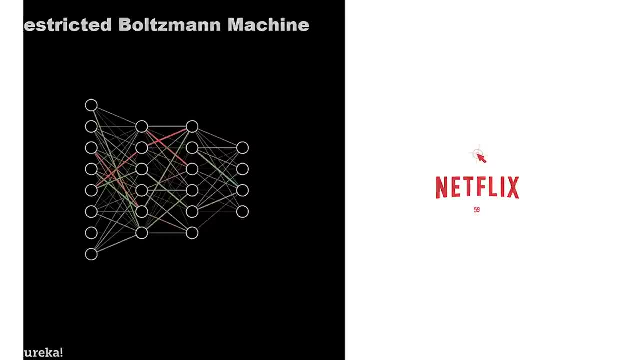 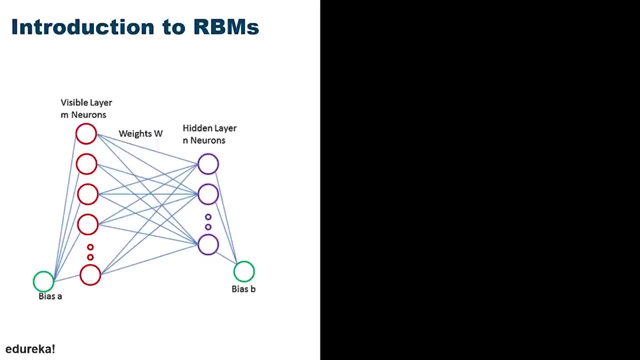 collaborative filtering and have beaten most of the competition. many hidden layers can be learned efficiently by composing restricted Boltzmann machines using the feature activations of one as the training data for the next. these are basically the neural networks that belong to so-called energy based models, and it is an algorithm which is used for dimensionality reduction. 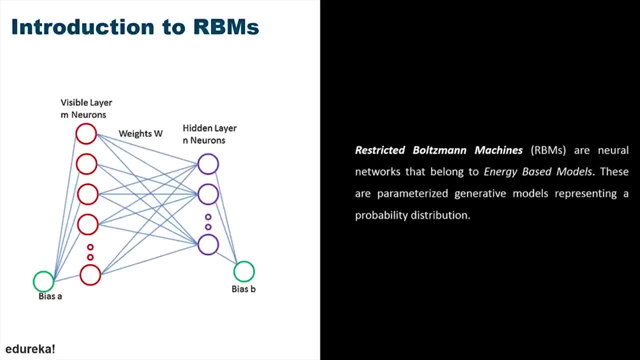 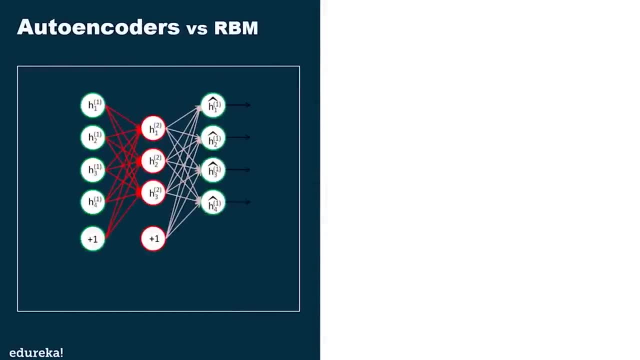 classification, regression, collaborative filtering, feature learning and topic modeling. Now let's see how our autoencoders and rbm's different from each other. So autoencoders are a simple three-layer neural networks where output units Are directly connected back to input units, typically number. 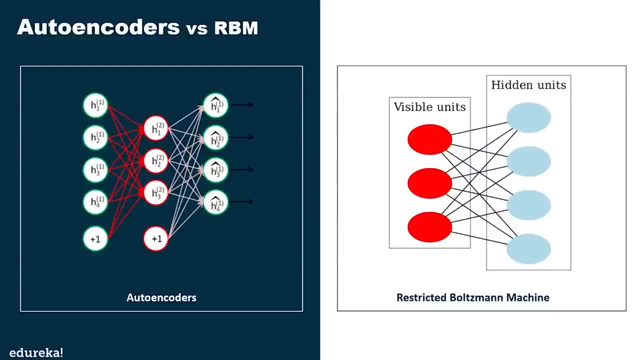 of hidden units is much less than number of visible ones. rbm also shares a similar idea, but it uses stochastic approach instead of deterministic. It uses stochastic units with particular distribution. Now you will notice that rbm's have two biases. This is one aspect that distinguishes them from other. 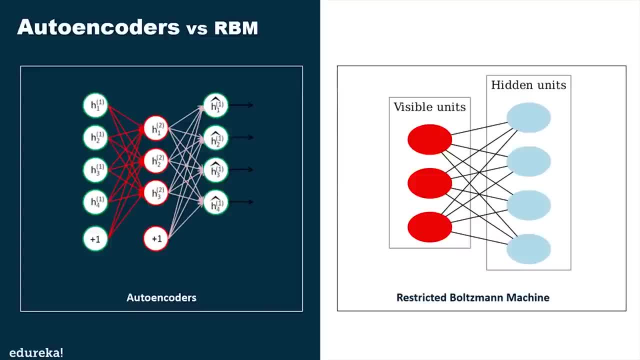 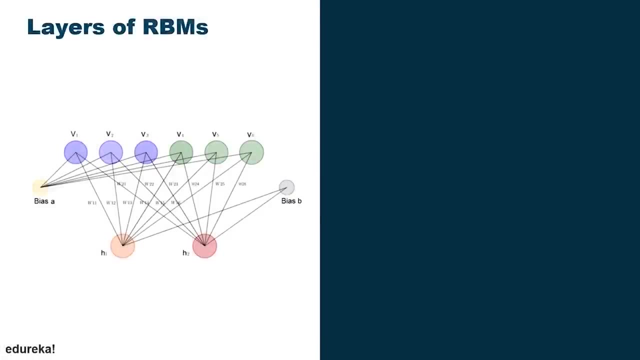 autoencoders. Now, the hidden bias helps the rbm provide the activations on the forward pass, While the visible layers biases help the rbm learn the reconstructions on the backward pass. restricted Boltzmann machines are shallow. They basically have two layer neural nets that constitute the 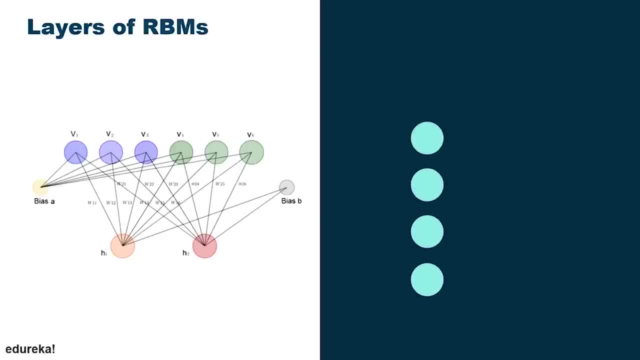 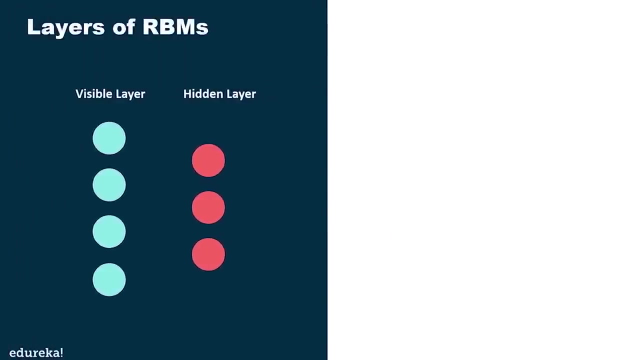 building blocks of deep belief networks. Now the first layer of the rbm is called the visible or input layer, and the second is the hidden layer. each circle here represents a neuron like unit called a node, and nodes are simply where calculations take place. Now the nodes are connected to each other across layers. 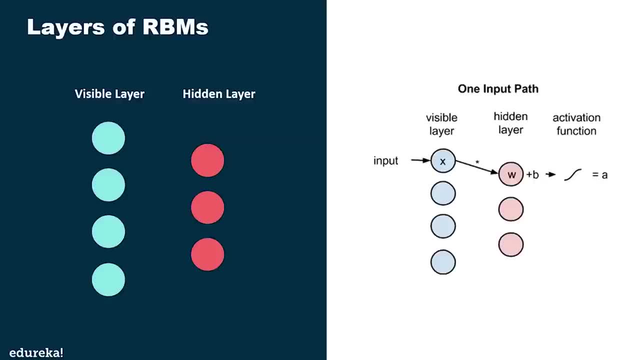 But no two nodes of the same layer are linked, which means that there is no intra layer communication. Now, This is the restriction. in a restricted Boltzmann machine, Each node is a locus of computation that processes input and begins by making stochastic decisions about whether to 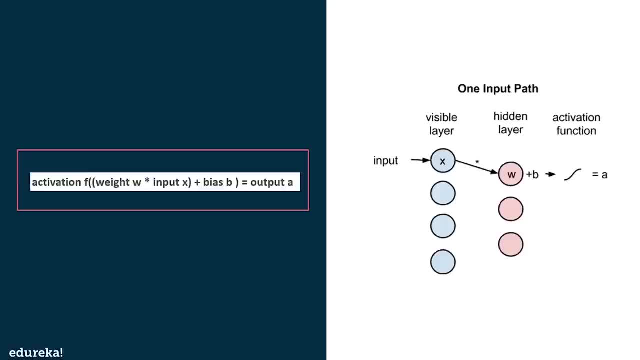 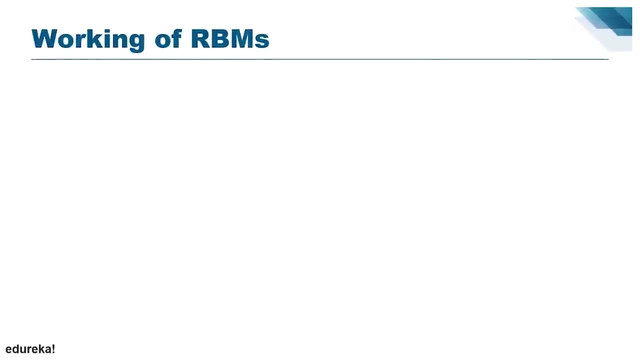 transmit the input or not. Now each visible node takes a low-level feature from an item in the data set to be learned, For example, from a data set of grayscale images. each visible node would receive one pixel value for each pixel in one image. Now let's follow that single pixel value X through the two. 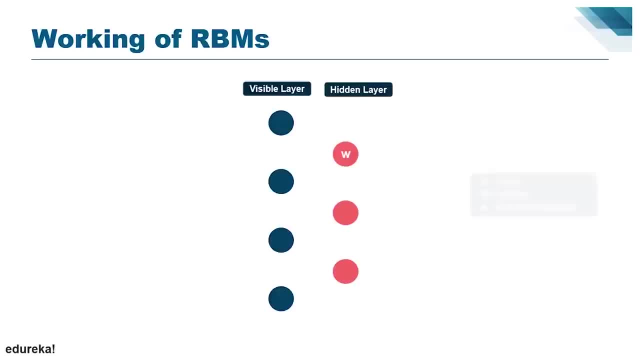 layered net. at node one of the hidden layer X, is multiplied by a weight and added to a so-called bias. The result of those two operations is fed into an activation function which produces the nodes output or the strength of the signal passing through it. given input X. 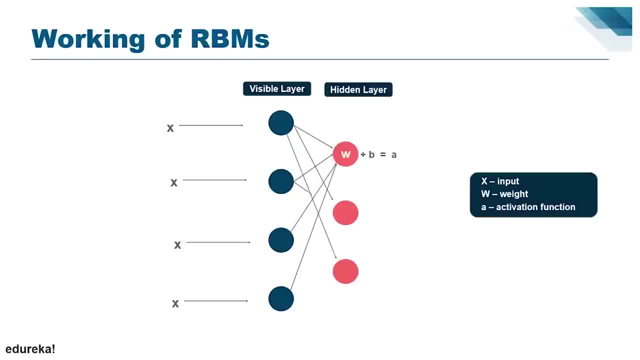 Now let's look at how several inputs would combine at one hidden node. Each X is basically multiplied by a separate weight, The products are summed, added to a bias and again the result is passed through an activation function to produce the nodes output. Now each hidden node receives the four inputs multiplied by. 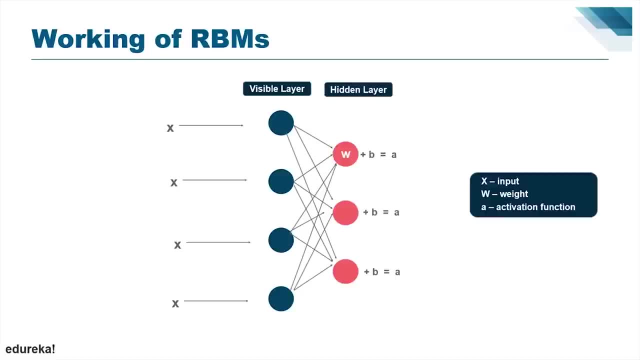 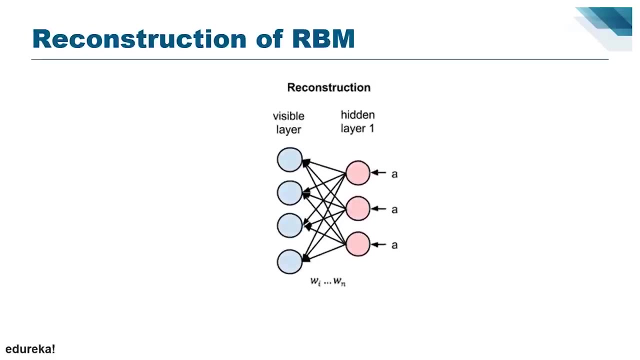 their respective weights. The sum of those products is again added to a bias and the result is passed through the activation algorithm, producing one output for each hidden node. Now, in the reconstruction phase, the activations of hidden layer become the input in a backward pass. Now they are multiplied by the same weights, one per inter node. 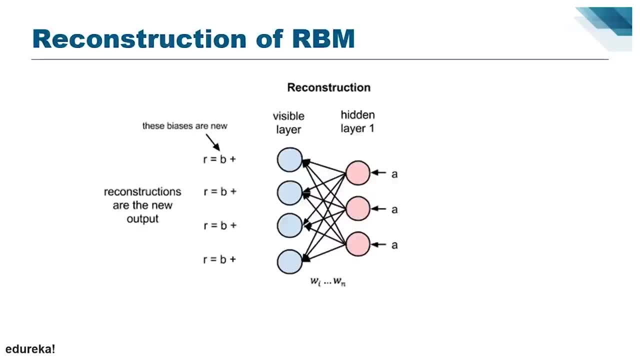 edge, just as X was weight adjusted on the forward pass. the sum of those products is added to a visible layer, bias at each visible node, and the output of those operations is a reconstruction that is, an approximation of the original input. now, because the weights of the RBM are randomly initialized, the difference? 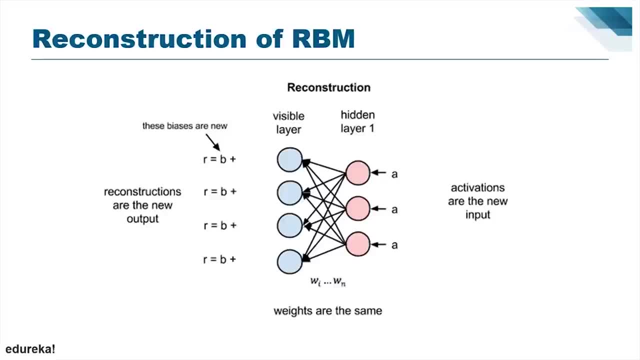 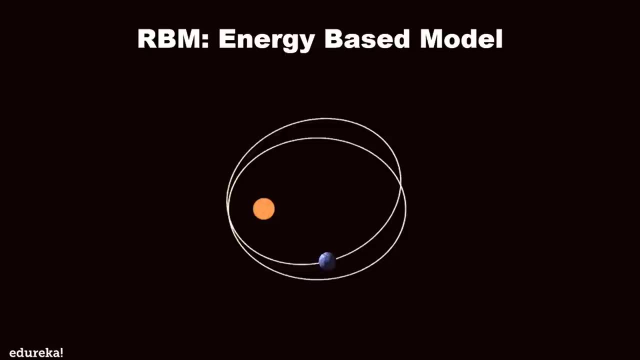 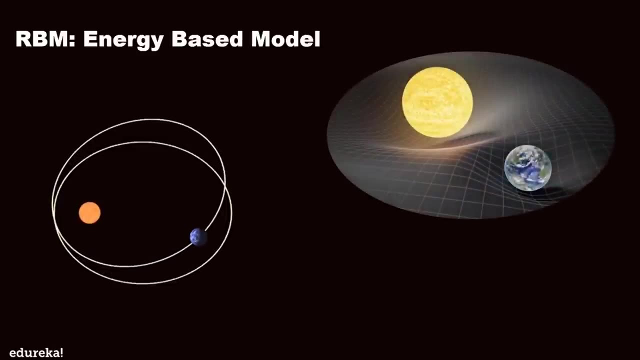 between the reconstructions and the original input is often large. Now let's move on and have a look at the energy based model. Now, energy is a term that may not be associated with deep learning in the first place. Rather, energy is a quantitative property of physics. yet some 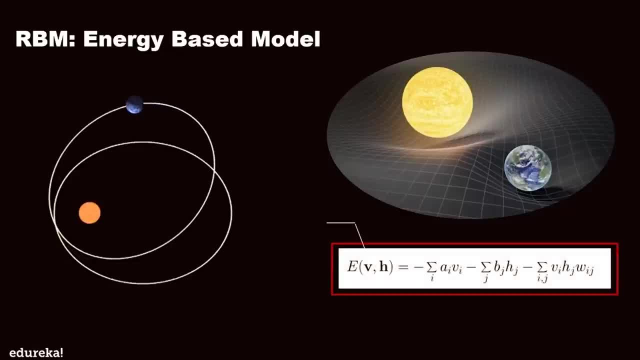 deep learning architectures use the idea of energy as a metric for measurement of the models quality. Now, one purpose of deep learning models is to encode dependencies between variables. the capturing of dependencies happen through associating of a scalar Energy to each configuration of the variables, which serves 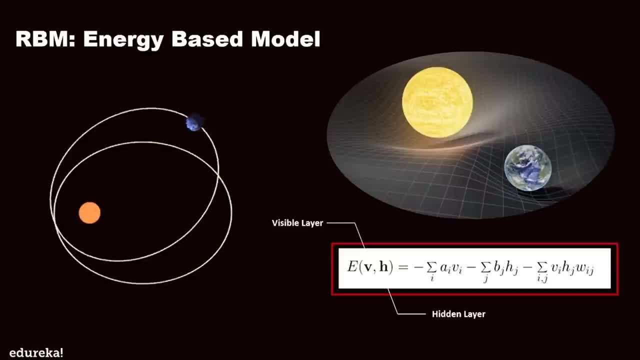 as a measure of compatibility. now, a high energy means a back compatibility, and energy based model always tries to minimize a predefined energy function. Now the energy function for the rbm's is defined using the following equation: We can see that the value of the energy function depends on: 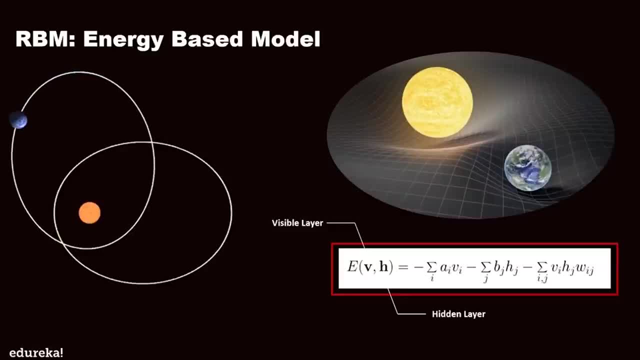 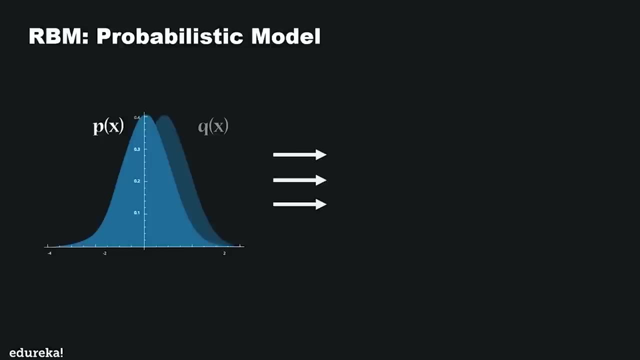 the configurations of visible States, hidden States, weights and biases. the training of RBM consists and finding of parameters for given Input values so that the energy reaches a minimum. Now let's have a look at the probabilistic model. rbm's are basically probabilistic, as opposed to assigning discrete values. 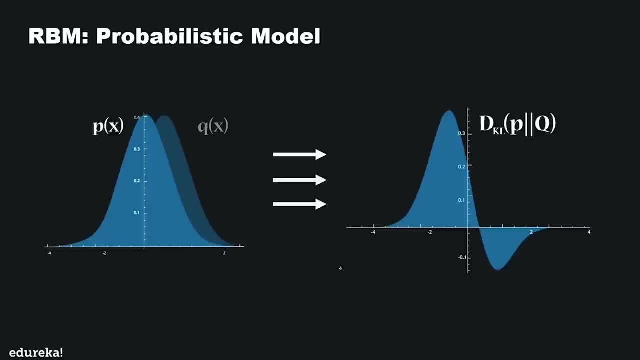 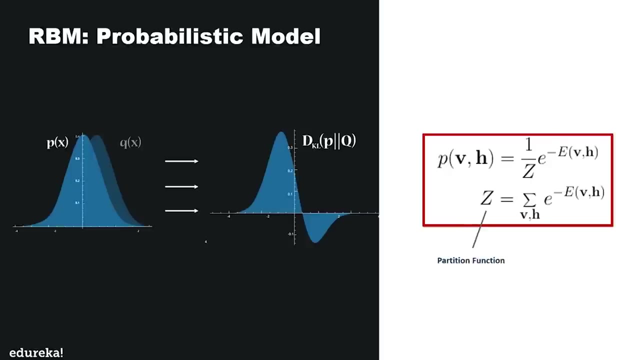 the model assigns probabilities. now, at each point in time The rbm is in a certain state. Now the state refers to the values of neurons in the visible and hidden layers V and H. now the probability that a certain state of V and H can be observed is given by the following joint: 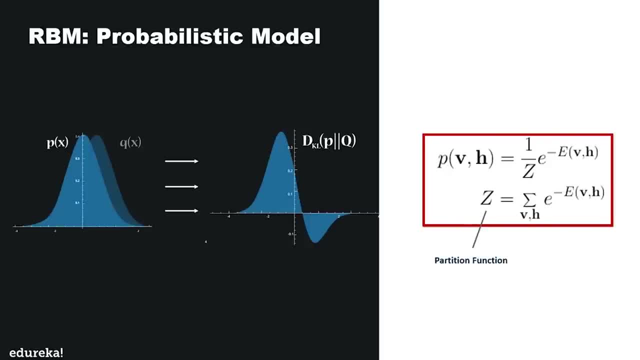 distribution. here Z is called the partition function, That is the summation over all possible pairs of visible and hidden vectors. Now this is the point where restricted Boltzmann machines meet physics for the second time. the joint distribution is known in physics as the Boltzmann distribution, which gives 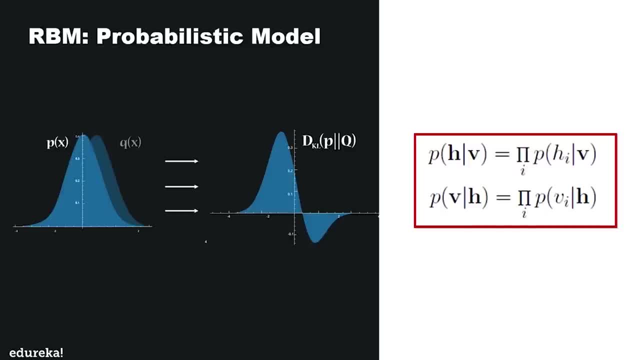 the probability that a particle can be observed in the state with the energy E. as in physics, We assign a probability to observe a state of V and H that depends on the overall energy of the model. Unfortunately, It is very difficult to calculate the joint probability. 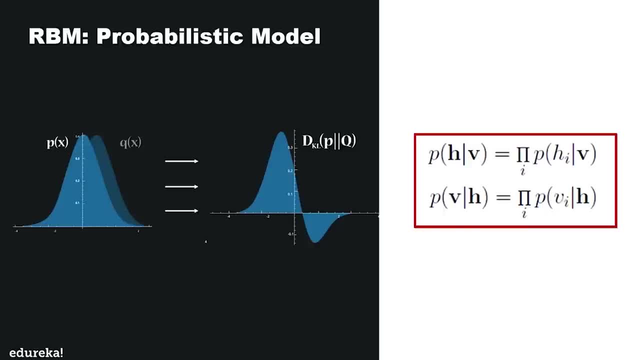 due to the huge number of possible combination of V and H in the partition function Z, much easier is the calculation of the conditional probabilities of state H given the state V and conditional probabilities of state V given the state edge, which is represented using the following equation: 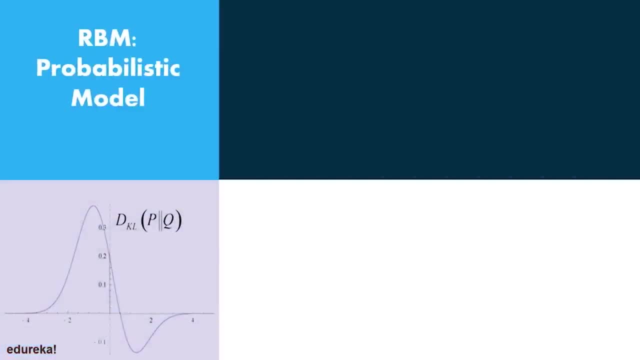 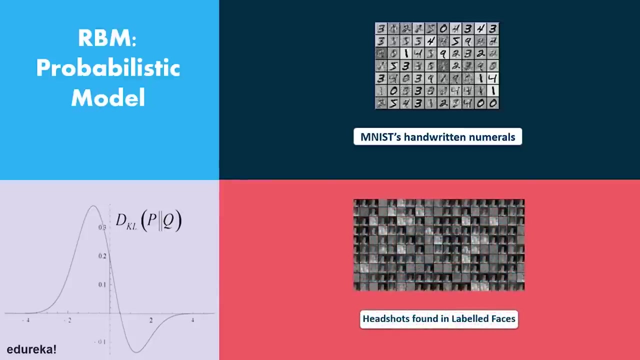 Now the image data sets have unique probability distributions for their pixel values depending on the kind of images in the set. pixel values are distributed differently, differently Depending on whether the data set includes MNI, STS, handwritten numerals or the headshots found in labeled faces in the wild. 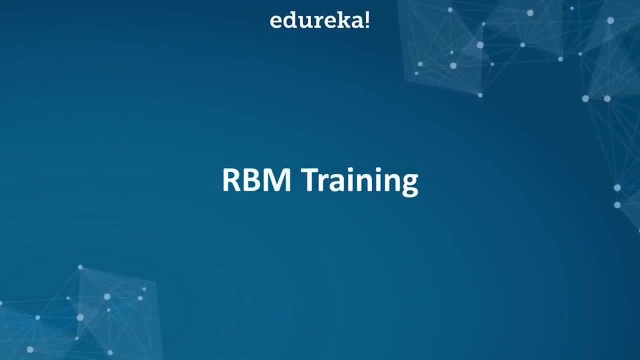 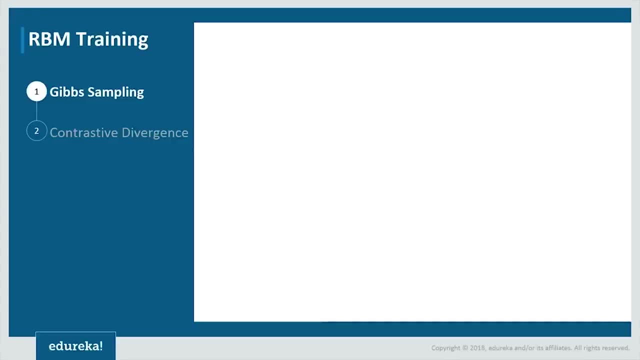 Now let's have a look at the training of restricted Boltzmann machines. Now the training of RBM differs from the training of a regular neural networks via stochastic gradient descent. Now, the two main training steps include Gibbs sampling and contrastive divergence. 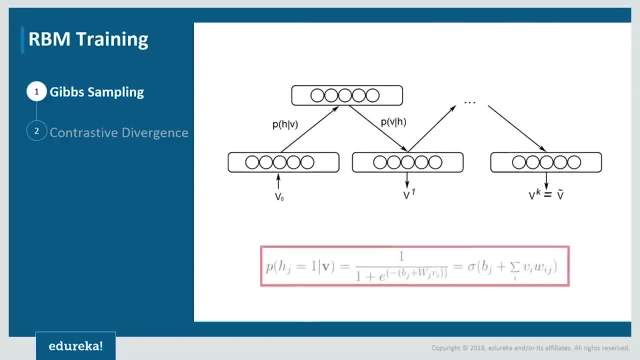 Now the first part of the training is called Gibbs sampling. given an input vector V, We are using the following equation for prediction of the hidden values H. Now knowing the hidden values, we use the next equation for prediction of new input values V. This process is repeated a number of times and after each, 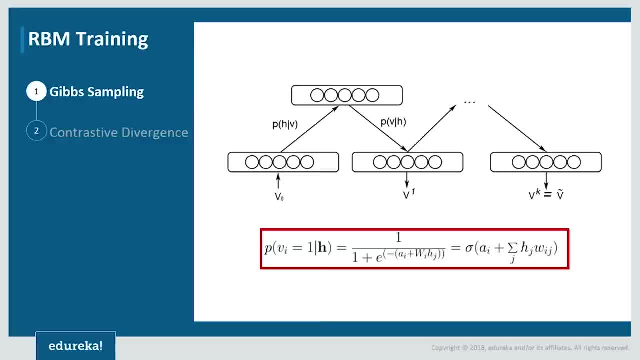 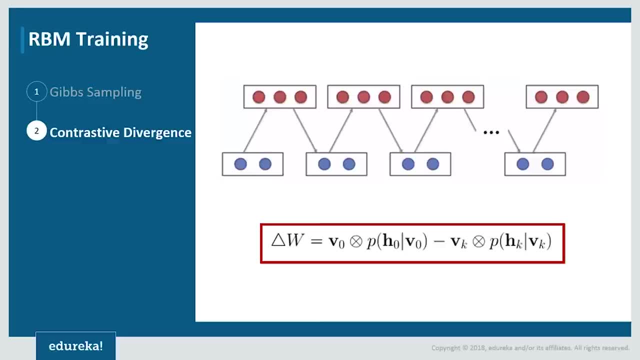 iteration we obtain another input which is recreated from the original input value. Now the update of the weight matrix happens during the contrastive divergence step. Now both the vectors are used to calculate the activation probabilities for the hidden values, Now the difference between the outer products of those 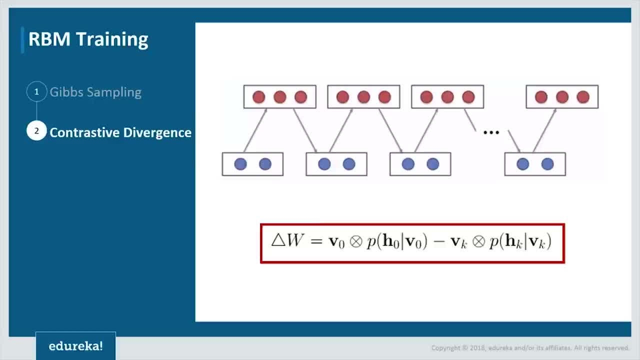 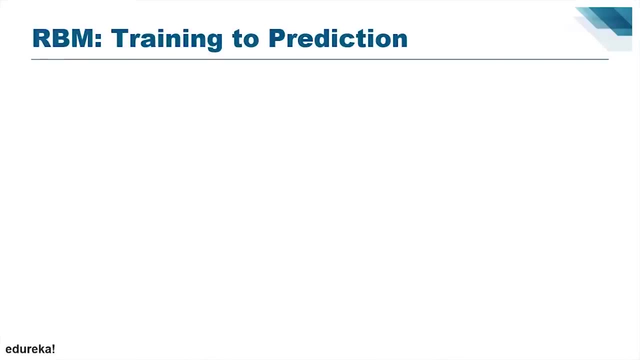 probabilities with input vectors results in the updated matrix, which is represented using the following equation. Now, using the updated matrix, the new weights can be calculated with gradient ascent, which is given by the next equation. Now let's have a look at the steps involved in the process. 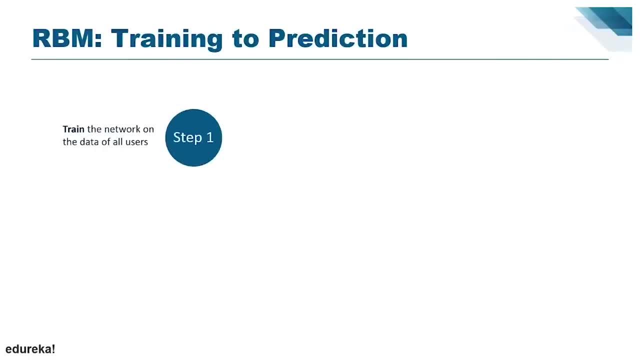 of training to prediction in RBM. So the first step is to train the network on the data of all users. In the next step, take the training data of a specific user during the inference time. Now use this data to obtain the activations of hidden neurons. 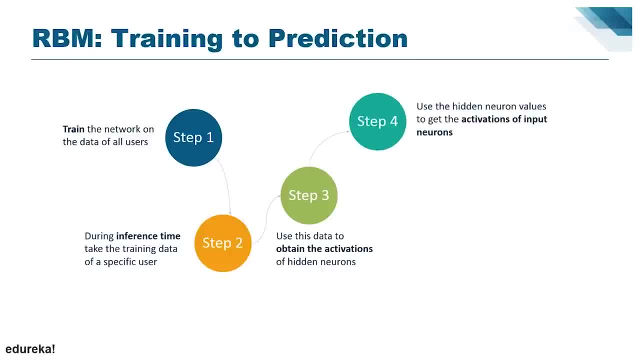 in step 3.. In step 4, use the hidden neuron values to get the activations of input neurons. Now, finally, the new values of input neurons show the rating the user would give. So now that we have seen how a restricted Boltzmann machine 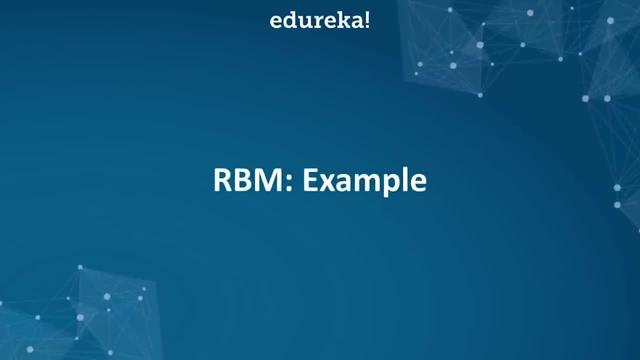 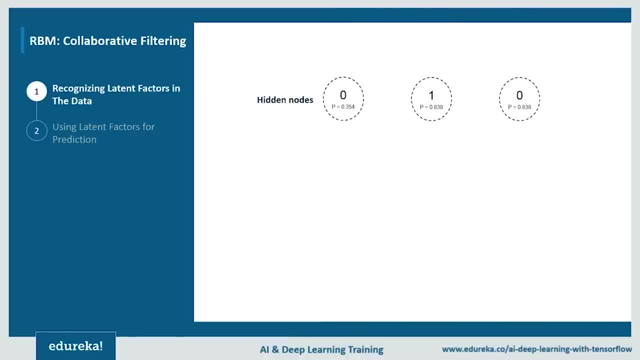 works. So let's move on and have a look at the example of RBM using collaborative Filtering. Now let's assume some people were asked to rate a set of movies on a scale of 1 to 5 stars In classical factor analysis. 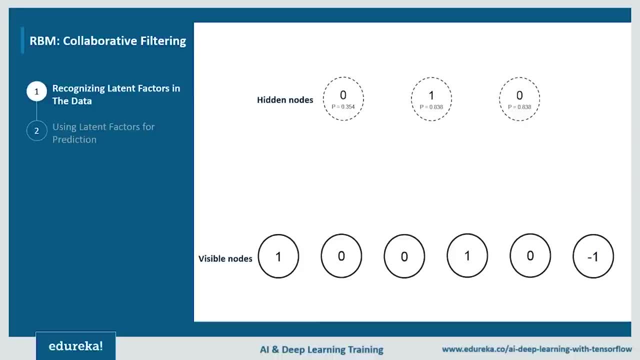 Each movie could be explained in terms of a set of latent factors. For example, movies like Harry Potter and Fast and the Furious might have strong associations with the latent factor of fantasy and action. On the other hand, users who like Toy Story and Wall-E might. 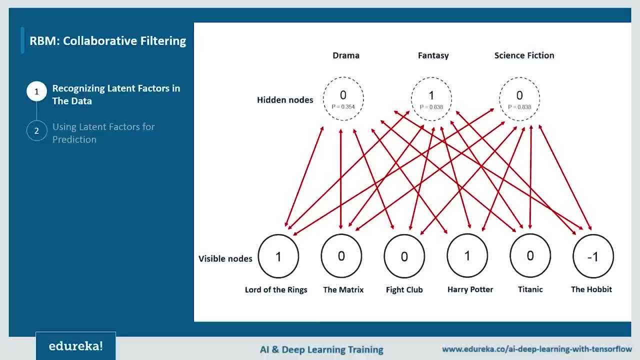 have strong associations with latent Pixar factor. Now RBMs are used to analyze and find out the underlying hidden factors, based on user preferences and corresponding collaborative movie tastes of all users. Now let's consider the following example where a user likes Lord of the Rings and Harry Potter but does not like 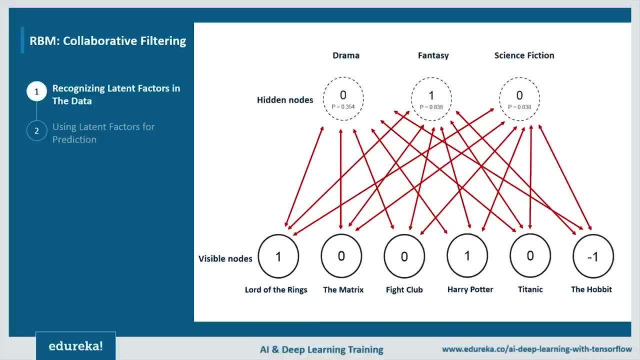 The Matrix, Fight Club and Titanic. The Hobbit has not been seen yet, So it gets a minus 1 rating. Given these inputs, the Boltzmann machine may identify three hidden factors: drama, fantasy and science fiction, which correspond to the movie genres. 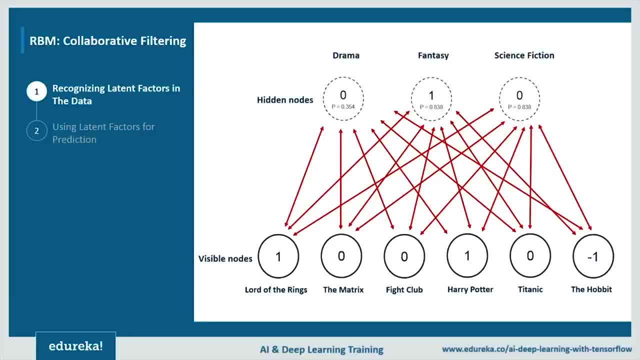 Now, in this example, only the hidden neuron that represents the genre fantasy becomes activate. Given the movie ratings, the restricted Boltzmann machine recognized correctly that the user likes fantasy the most. Now, after the training phase, the goal is to predict a binary rating for the movies that had not been seen yet. 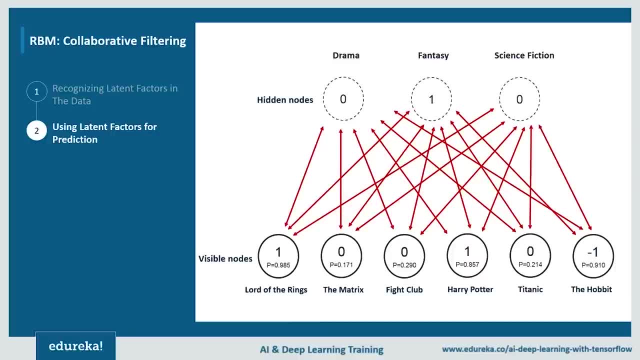 Given the training data of a specific user, the network is able to identify the latent factors based on the user's preference. Now the latent factors are represented by hidden neurons, So we can use all our previous equations and sample from Bernoulli distribution to find out which of the visible neurons 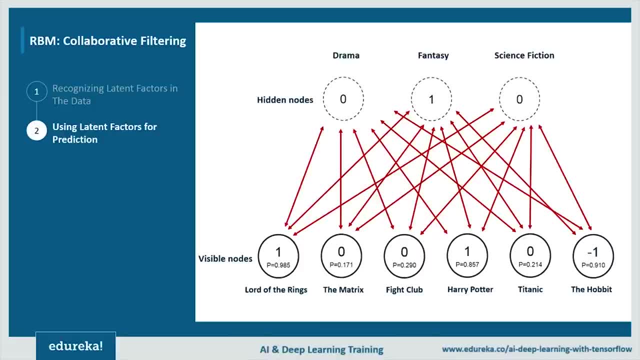 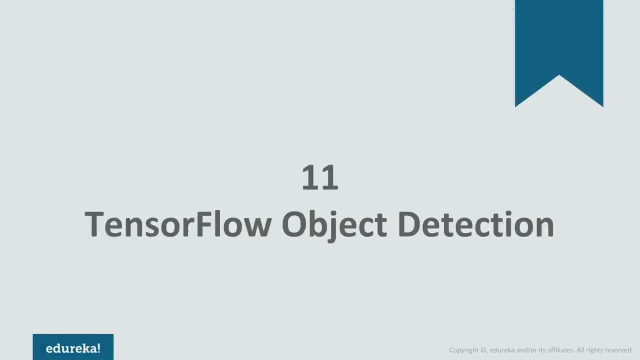 will become active. Now. that's exactly how an RBM would help you identify which movie genre would the user prefer. Creating accurate machine learning models capable of localizing and identifying multiple objects in a single image remained a core challenge in computer vision. But with recent advancement in deep learning and deep learning, 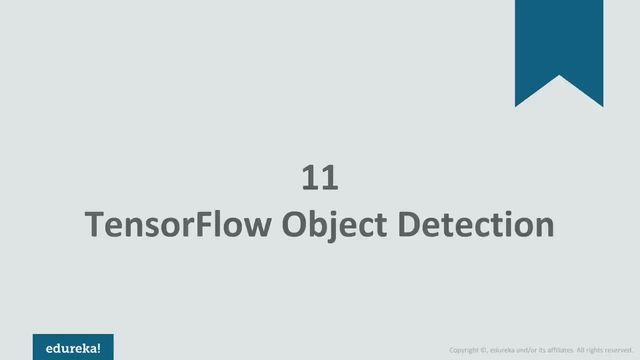 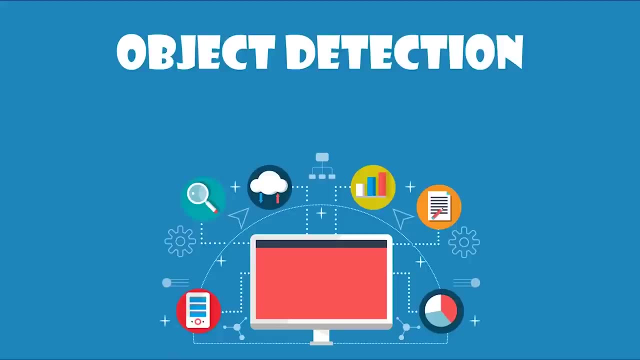 based computer vision models, object detection applications are easier to develop than ever before. welcome you to this session on object detection using tensorflow. So before moving forward, let's have a quick look at the agenda of this session. So first of all I'll be starting with explaining you guys. 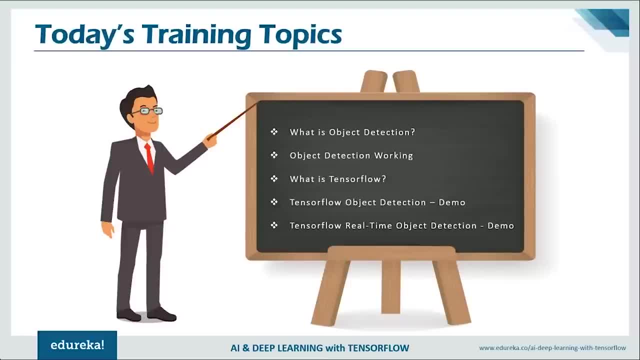 What is exactly object detection? then we'll have a look at the object detection workflow, How exactly it works, and the various industrial use cases of object detection. Then we'll understand what is tensorflow, and I'll end this video with two demos, the first one being the tensorflow object. 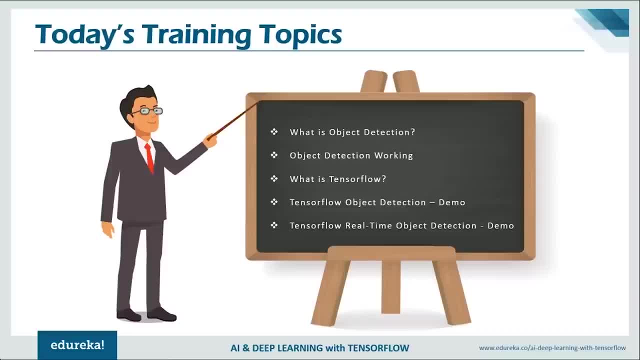 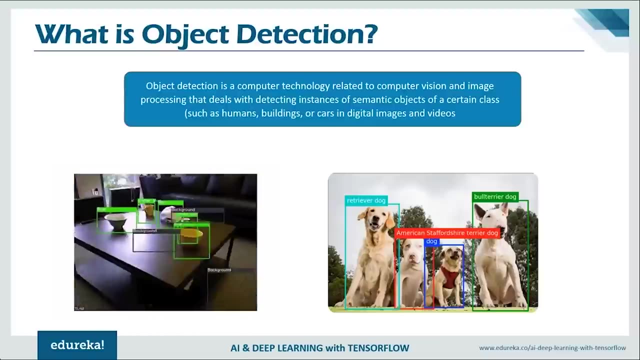 detection, where we can detect objects using our own input images, and the second demo is based on the live object detection, where we'll detect objects in real time. So, without wasting any time, let's go ahead and start now. object detection allows for the recognition, detection and the 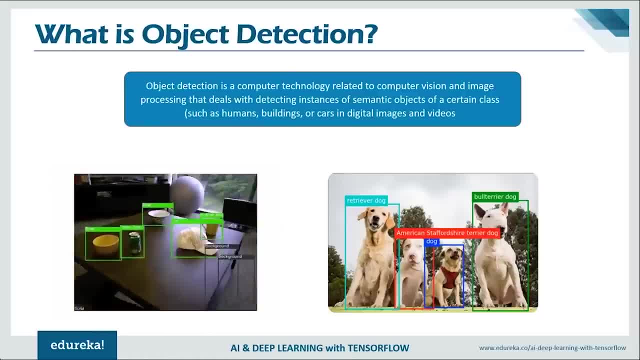 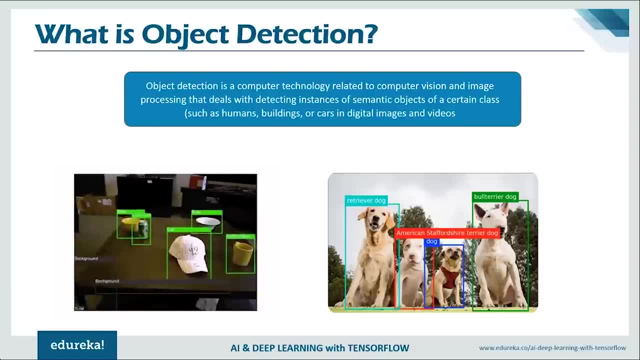 localization of multiple objects within an image. It provides us a much better understanding of an image as a whole, as opposed to just visual recognition. In addition, with current approaches focusing on full end-to-end pipelines, performance has also improved significantly, enabling real-time use cases. 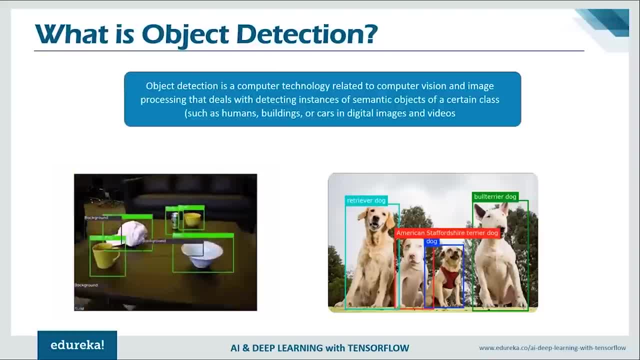 Object detection is the process of finding instances of real world objects such as faces, bicycles and buildings in images or videos. Now, object detection algorithms typically use extracted features and learning algorithms to recognize instances of an object category. It is commonly used in applications such as image. 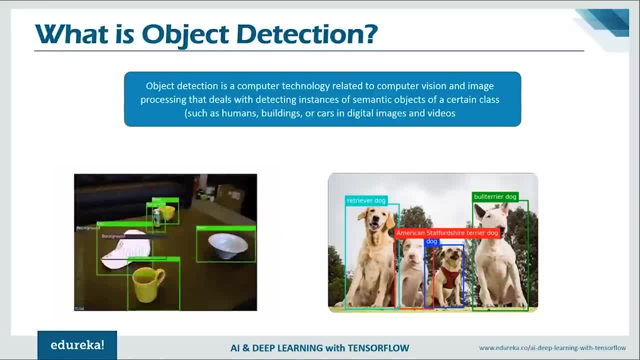 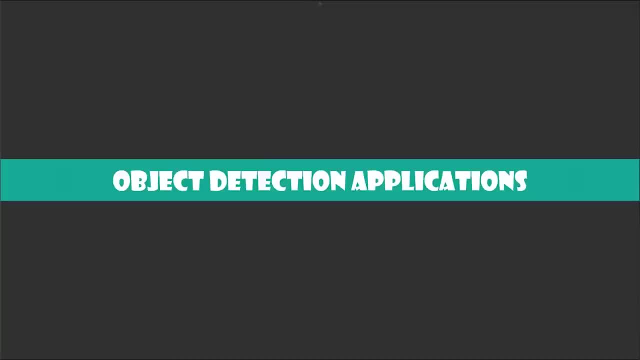 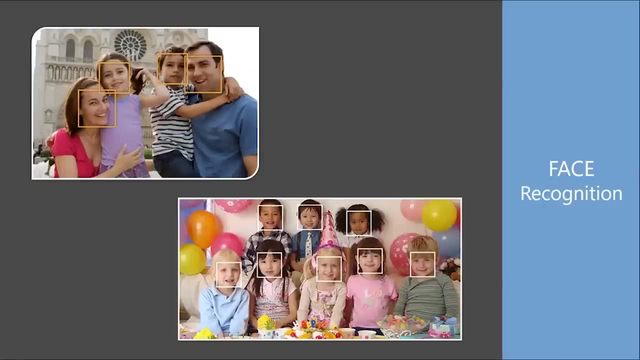 retrieval, security, surveillance and advanced driver assistance system, which is known as ADAS. Now let's have a look at few of the object detection application Now. the first use case is the facial recognition Now popular application include face detection and people counting. 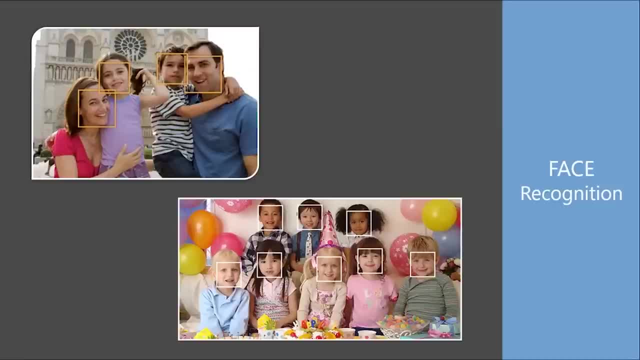 Have you ever noticed how Facebook detects your face when you upload a photo? that is due to their facial recognition algorithm. Now, this is a simple example of object detection that we can see in our daily life. Even the DSLR cameras and our phone cameras also detect the. 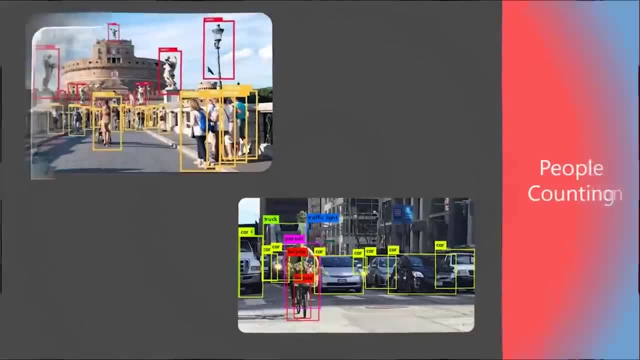 faces. Object detection can also be used for people counting. It is used for analyzing store performance or crowd statistics during festivals, where people tend to get lost easily. Now, these tend to be more difficult as people move out of the frame quickly and also because people are non-rigid. 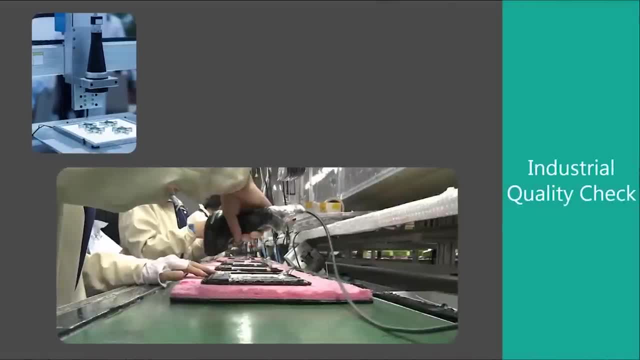 objects. Object detection is also used in industrial process to identify products. finding a specific object through visual inspection is a basic task that is involved in multiple industrial processes like sorting, inventory management, machining, quality management, packaging and much more. inventory management can be very tricky as items are hard to track in. 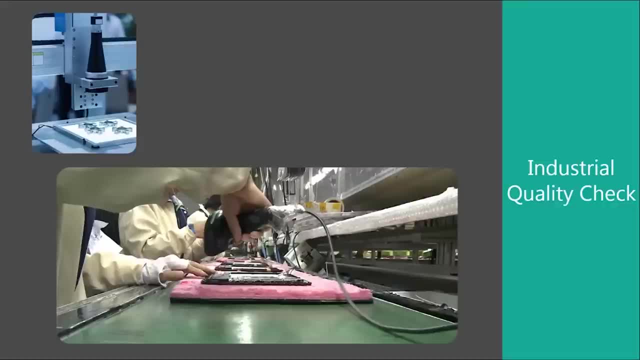 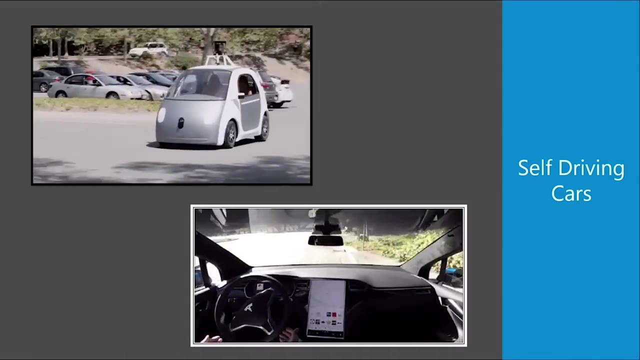 real-time. something is always added, removed and moved every day. systems can perform automatic object counting and localization. that will allow you to improve inventory accuracy. Now this is one of the most recent and, I should say, one of the most exciting use cases of object detection, which is the 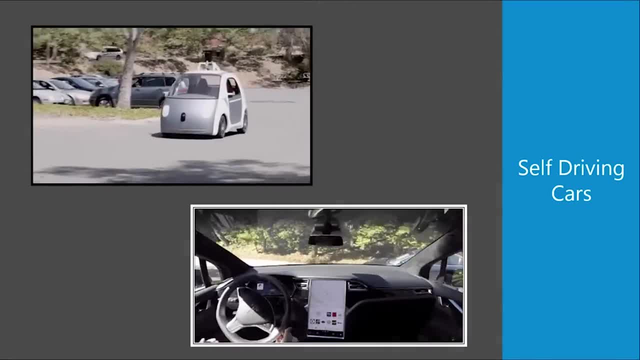 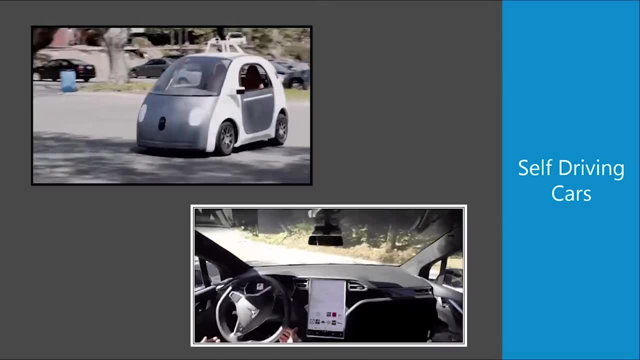 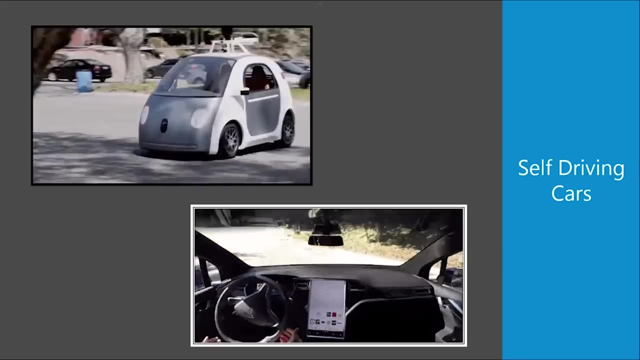 self-driving car. It is a vehicle that is capable of sensing its environment and navigating without human input. Now, how is it done? Now, it combines a variety of techniques to perceive the surroundings, including the radar, laser light, GPS and also computer vision. Now here is where the object detection comes in place. 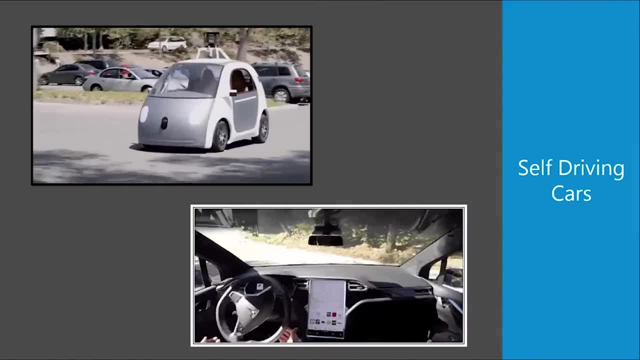 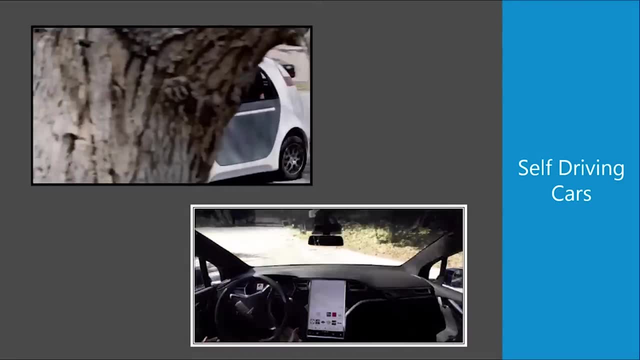 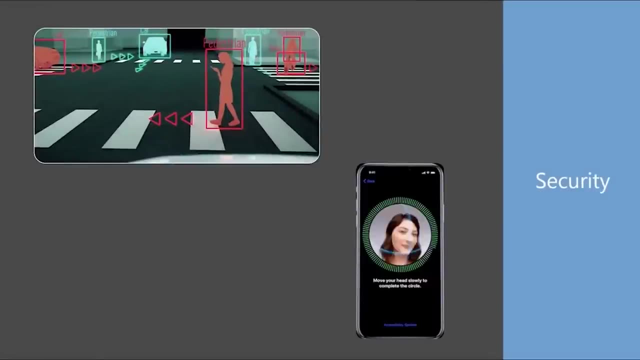 So the moment it senses a person on the road on its way, the car automatically stops. advanced control system interprets sensory information to identify appropriate navigation paths as well as obstacles. Now our final use case is the most important one, which is the security. Now it is used in the banking industry as well as the phone. 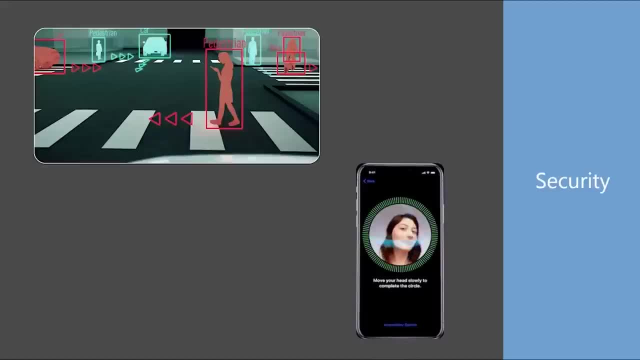 industry, or I should say the technologically industry, a lot. So it is using the banking industry to identify If I fraud, the forgery of notes or the currency and also theft. Now, one of the most important use of object detection is the facial recognition used in the smartphones nowadays, which is 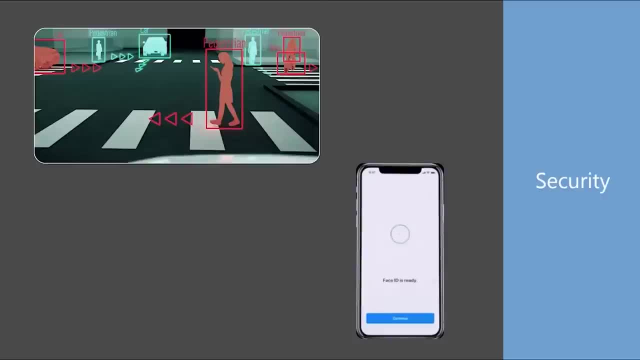 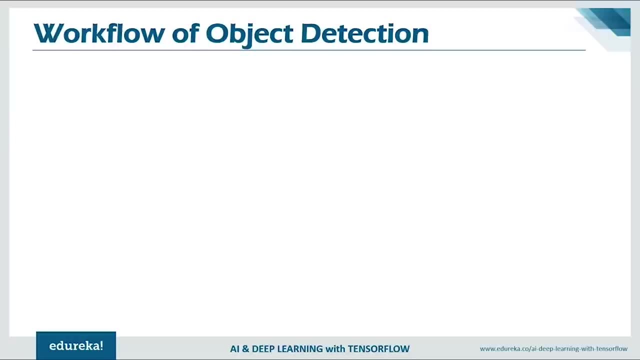 popularly known as face unlock. Now that we have understood What are the various industrial use cases of object detection, Let's have a look at the object detection workflow. Not typically, There are three steps involved in object detection workflow. First of all, we have the training data which we input. 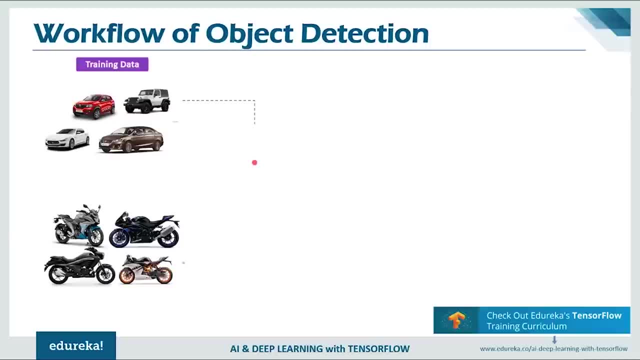 and create Our model. Now, this model is created using the visual features which are extracted from the images or the digits or whatever be your input of the training data. Now these are evaluated and is determined whether which objects are present in the proposal based on the visual. 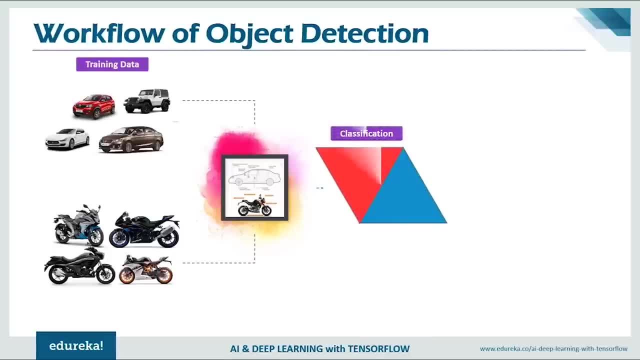 features. Now, upon extracting these features, we have a classification model created. Now, after that, we have the testing data. in our final post-processing step, We use the testing data and we extract all the features and then we move on to our model to see which all 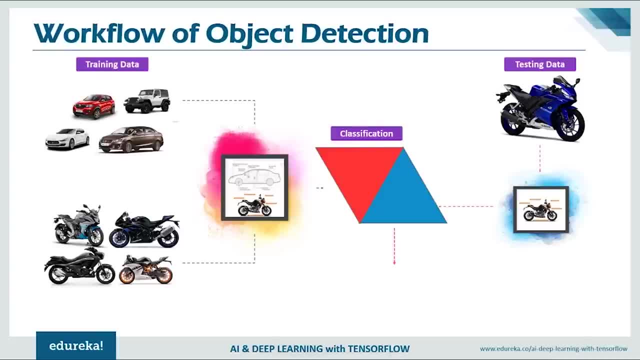 features are matching which type of class and finally, after the computation is done, We finally get our results. Now there is an important trade-off being made here, which is between the number of regions versus the computational complexity. We learn more about these later in this video. 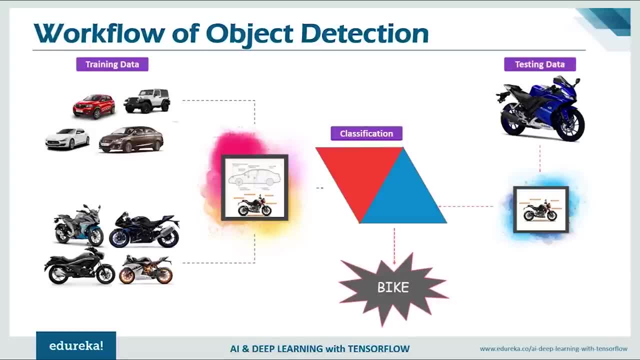 Now in object detection frameworks. people typically use pre-trained image classification models to extract visual features, as these tend to generalize fairly well. The goal of feature extraction is to reduce a variable sized image to a fixed set of visual features. Image classification models are typically constructed using 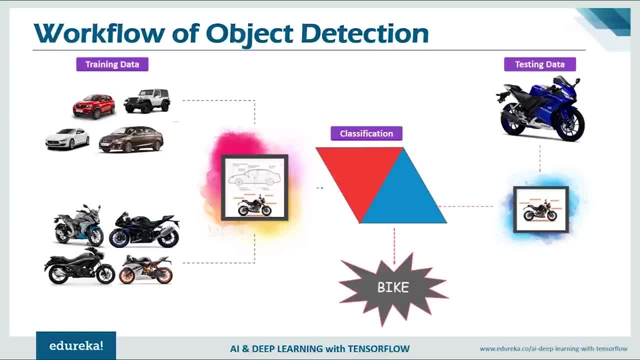 strong visual feature extraction methods. whether they are based on traditional computer vision approaches such as the filter based approach, the histogram methods or the deep learning methods, They all have the exact same objective: extracting features from the input image that are representative for the task at hands and use these. 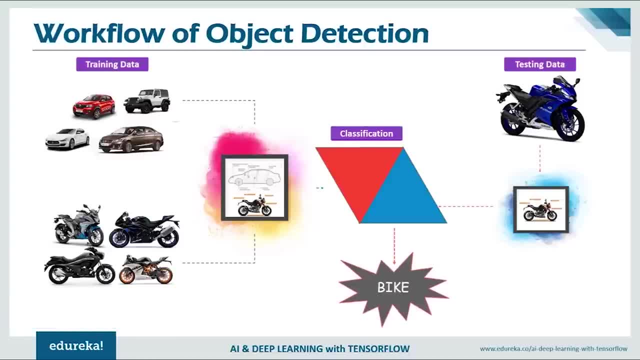 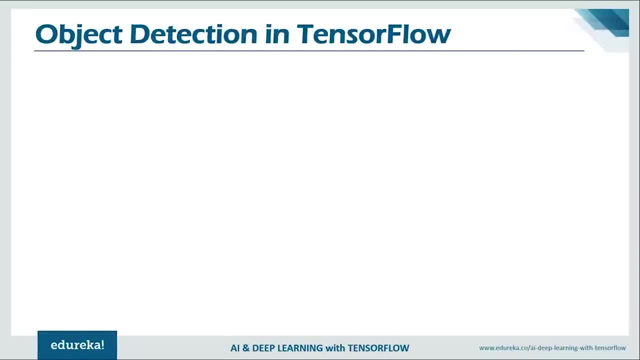 features to determine the class of the image. Now that we have understood the basic workflow of an object detection algorithm, Now let's see how object detection can be performed in TensorFlow. So first of all, we provide our input data, which is a set of 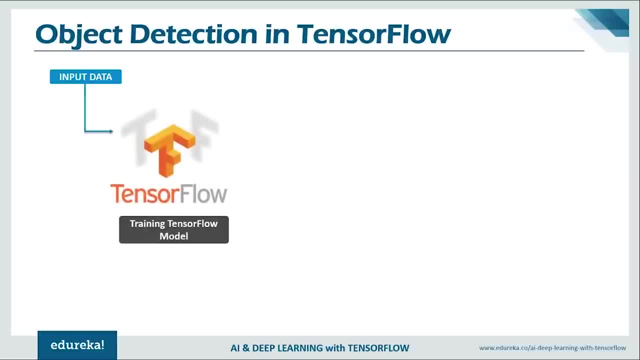 images and using TensorFlow, we train our model. Now this model is trained using deep learning and the main objective of this model is to extract the features. Now these are visual features which are based on edge detection, the HA features, the facial recognition and many more. 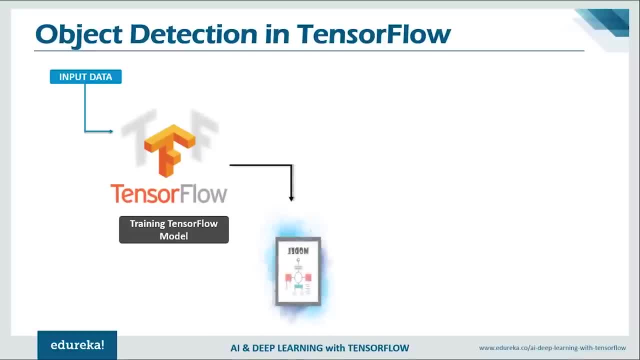 Now, when these features are extracted and then the model is created. to test this model, we provide our test data, which is again a set of images in our case, and using this model, we get our final output, in which we have the objects detected in an image. 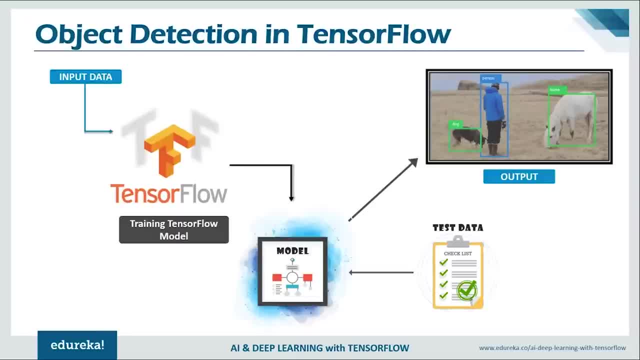 Now the image are converted into a numpy array in the TensorFlow object detection. So that the computation can be made easy, We also use the TF record, which is the TensorFlow record, which contains the record of the image along with the tags, such as, as you can see here: 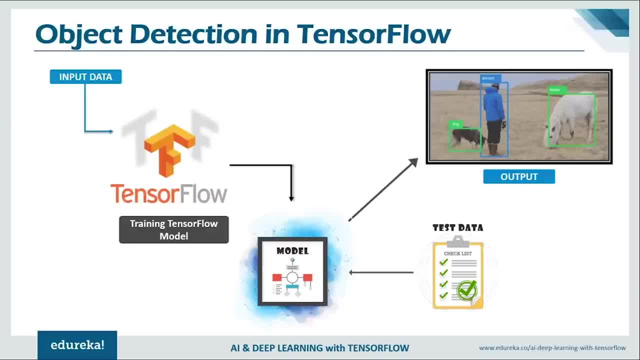 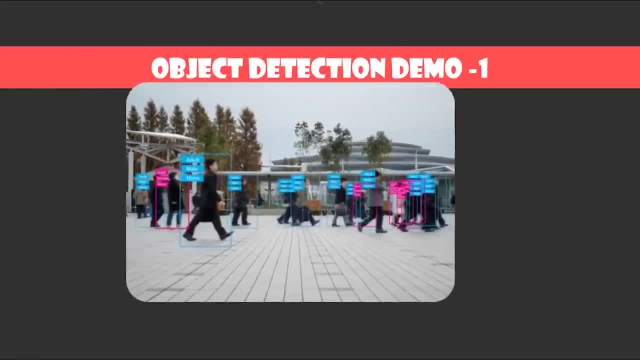 We have the person tag, We have the dog tag and the horse tag. Now, these tags are just labels which are provided in the input data. Now let's go ahead and start our demo and see how we can perform object detection using TensorFlow. 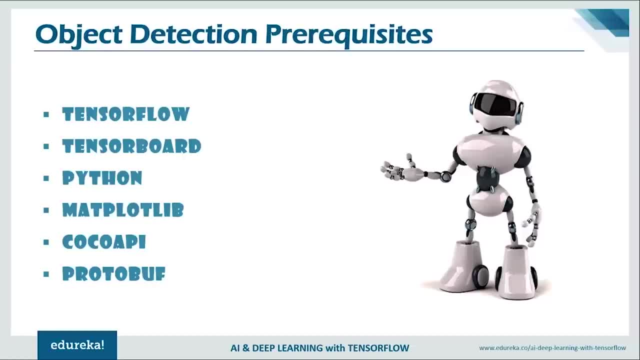 Now, to begin with, you want to make sure that you have TensorFlow installed with all of its dependencies, Like the TensorBoard, Python, matplotlib. We have the Cocoa API and the protobuf. Now I'll explain you guys what all steps are needed. 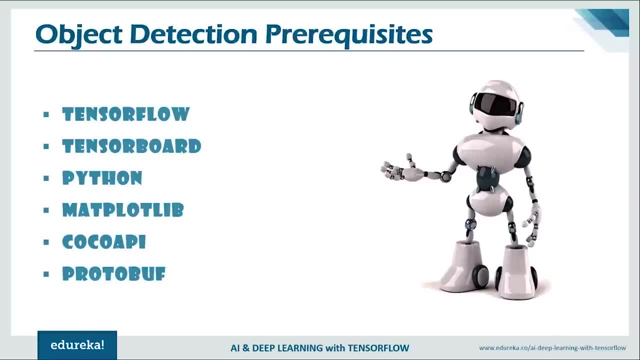 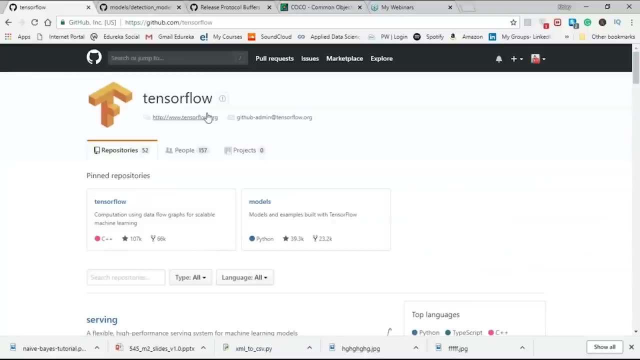 So for CPU TensorFlow you can just do pip install TensorFlow. But of course the GPU version of the TensorFlow is much faster at processing, So it is ideal. Now, next we need to do is to clone the GitHub repository of TensorFlow. So for that just go to GitHub and type TensorFlow, which is: 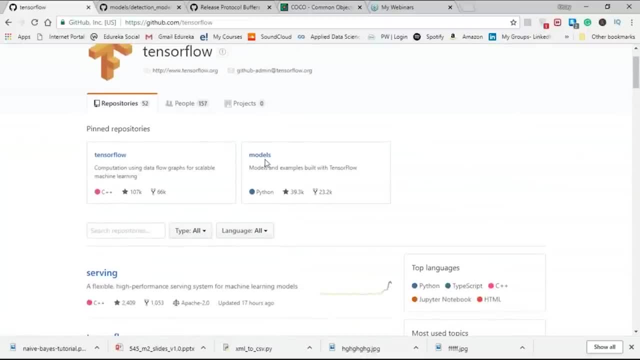 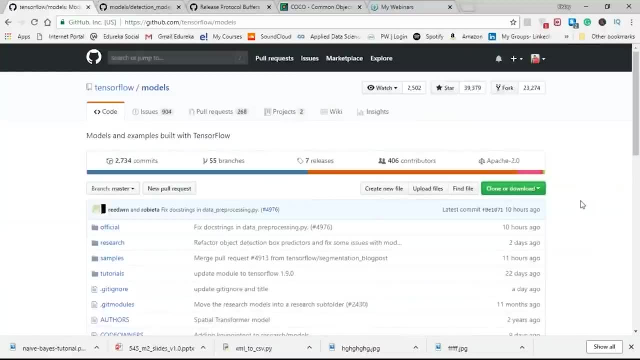 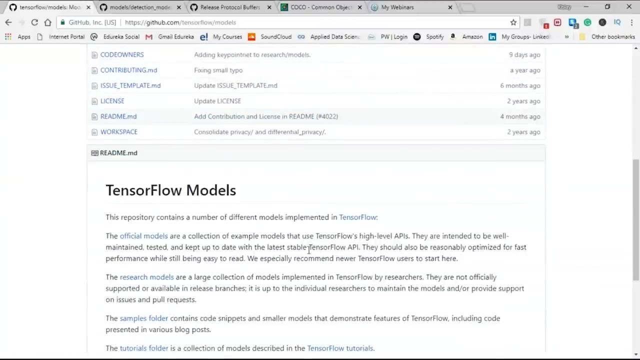 the official GitHub repository of TensorFlow And inside that we have the model section. Just go to this models. You can either clone this TensorFlow model or download it as per your wish. So I have already downloaded the TensorFlow model. Now the TensorFlow object detection model uses protobuf. 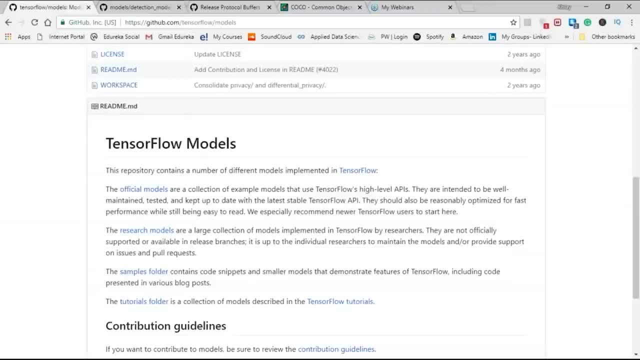 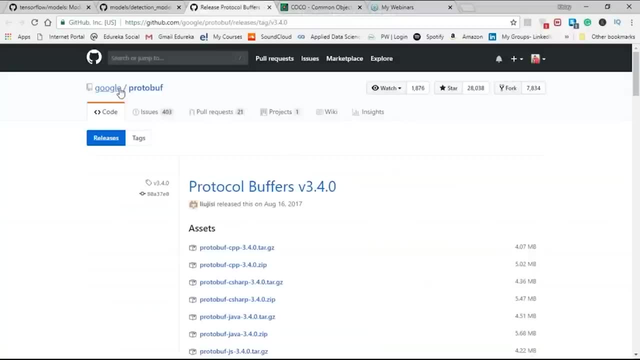 to configure model and the training parameters. before the framework can be used, The protobuf libraries must be compiled Now. to download protobuf, All you need to do is go to Google slash protobuf in GitHub and here you will have all the different versions of protobuf. 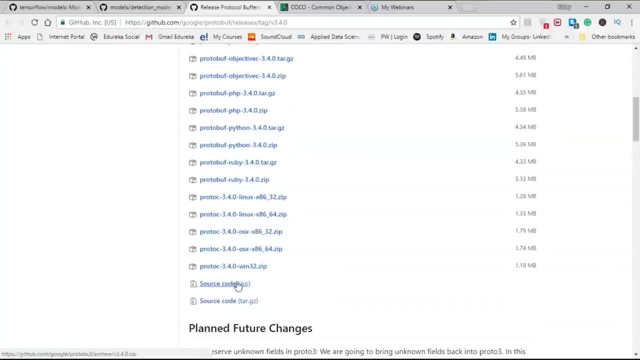 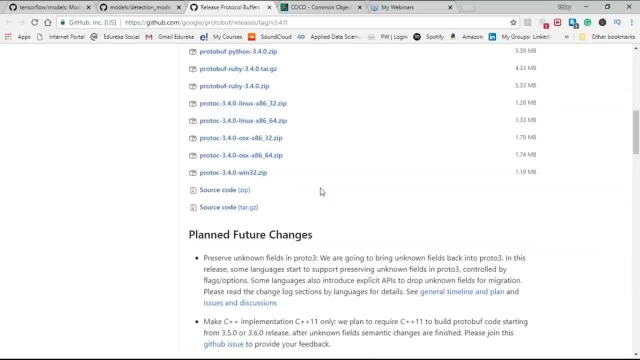 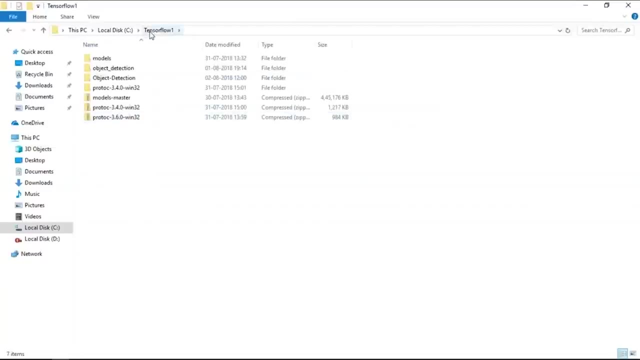 So, according to your OS, which is Linux, Mac OS or the Windows OS, or if you are using only the python, you can download the required protobuf. So, once you have downloaded TensorFlow and protobuf, create a folder in just see which is known as TensorFlow, and in this 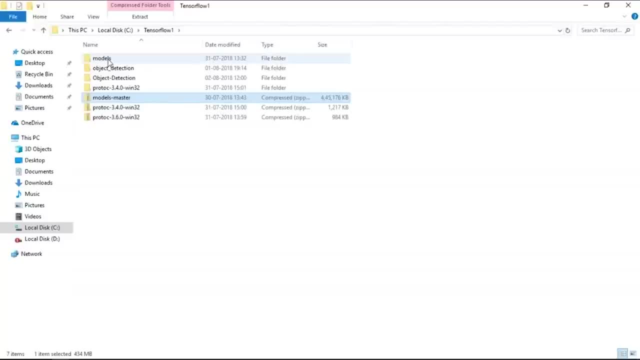 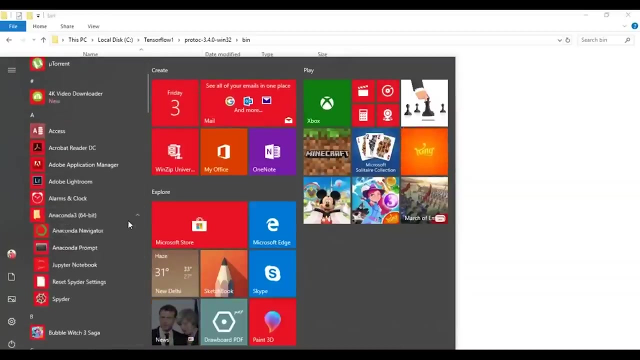 you will have the models master. extract this and rename it as models And extract the protobuf. now inside protobuf You have the bin folder. Now all you need to do is go to this bin folder. So let me just open the command prompt here. 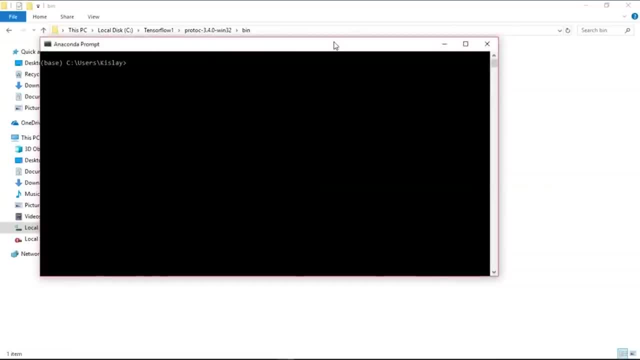 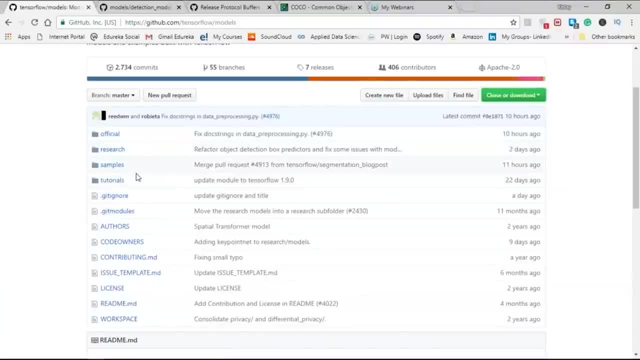 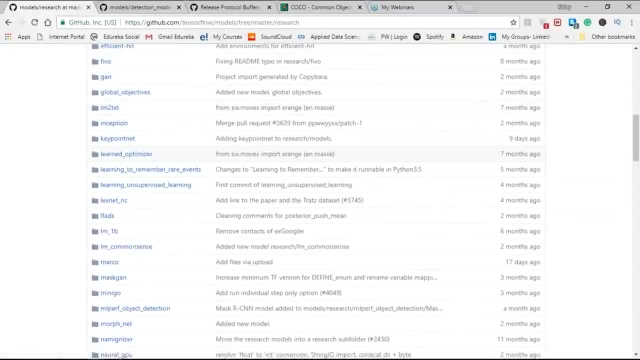 I'm using the anaconda prompt, but you can use the command prompt as well. So, once you have downloaded and renamed the models, master as models go back to the GitHub repository. and inside models you have the research. and inside research There is the object detection model, which we are interested in. 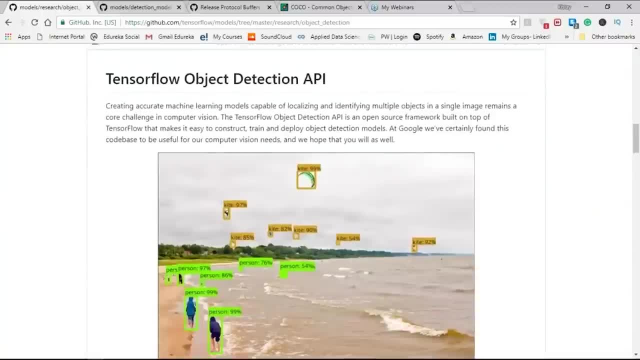 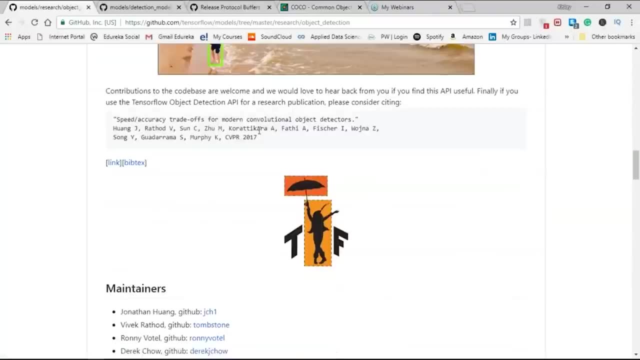 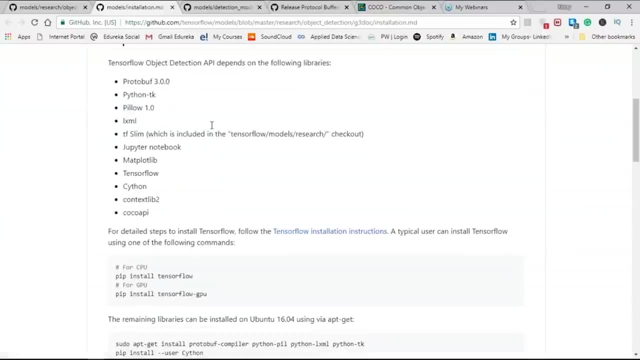 So let's go to the object detection model here Now. as you can see, this TensorFlow object detection API gives an accurate machine learning model, description of how the objects are detected, and here you have the steps for the setup. So in the installation, as you can see, we have the prerequisites. 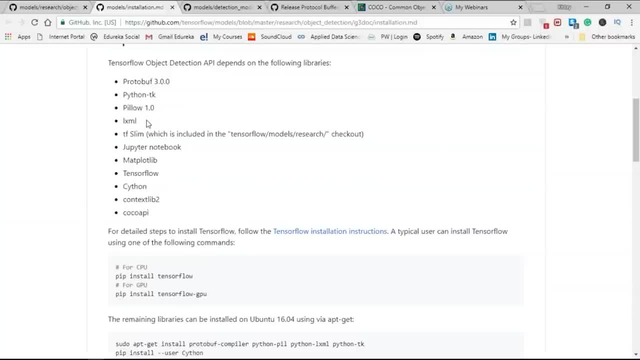 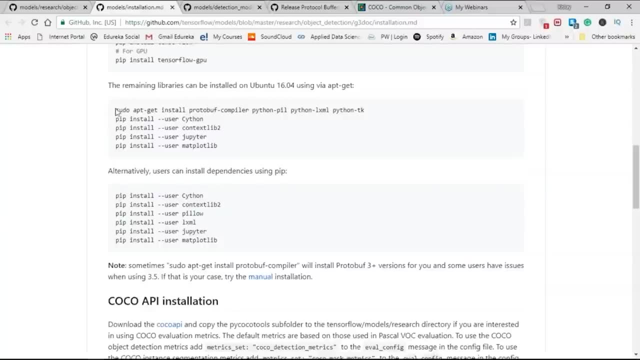 or the dependencies, which are the protobuf python pillow. You can install all of these using the pip or the conda command. Okay, so to download the protobuf on Ubuntu you can do the sudo apt-get install. then you can use the Cython. the context: 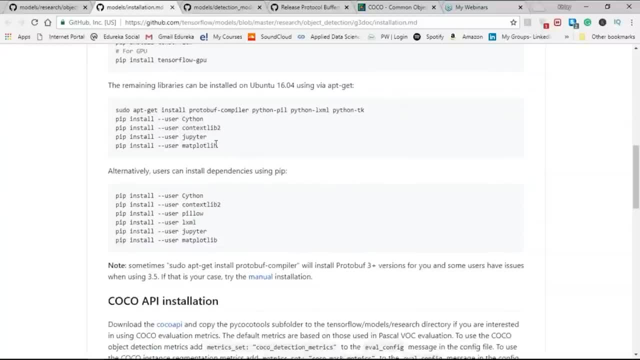 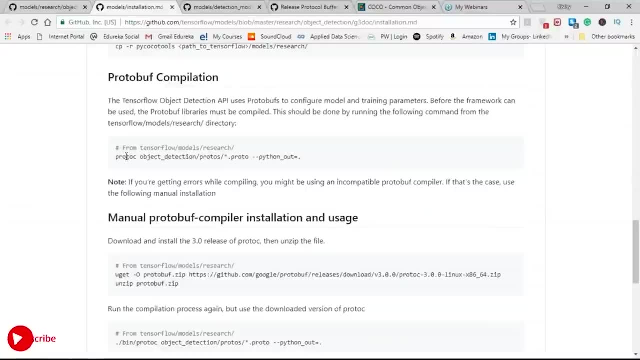 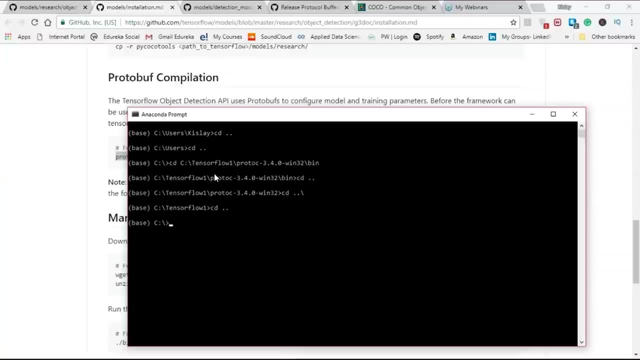 lib, the Jupiter and the matplotlib. Alternatively, you can also use the pip and the conda commands. And next, what we need to do is, once you have downloaded and extracted the protobuf, you need to copy this command Now. then you need to go into the test. 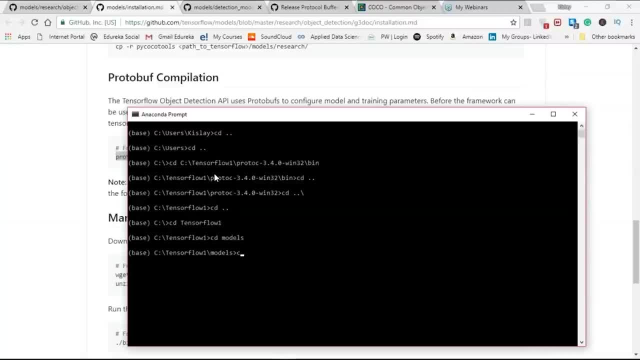 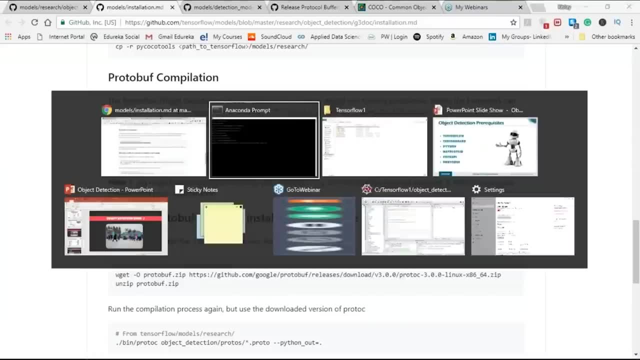 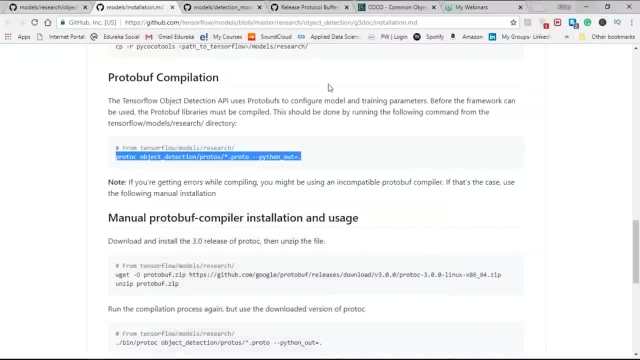 TensorFlow, then you need to go into the models and then inside that, you need to go into the research. Now, once you are inside the research, what you need to do is copy this command and paste it and run this command here. So what it will do- is I'll explain here- is that it will take. 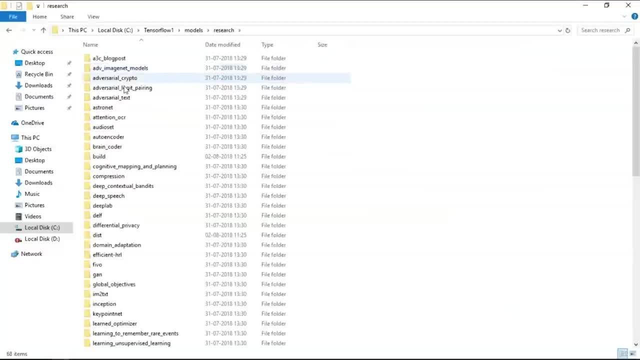 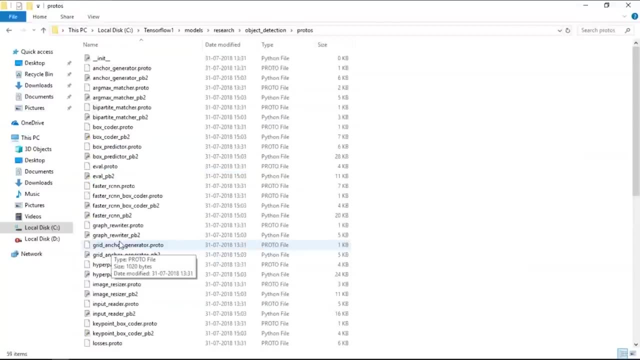 all the object. if you go inside the models research, and inside if you go to the object detection, you can see there's a folder named protos. So once you have compiled that code, all the proto files are then converted into the python files. 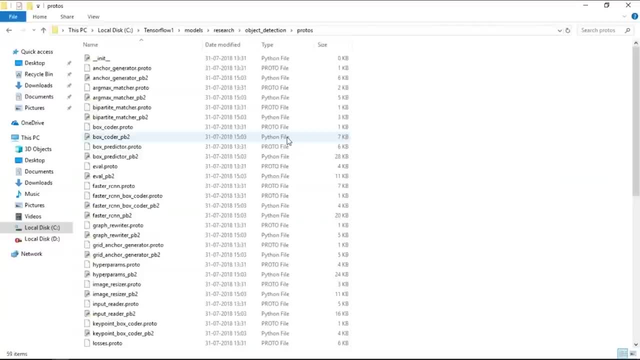 Now, in order to have a better understanding of what the different supported components are, inside the protos folder, which contains the functional definition, especially the train, the eval, the SSD, the faster, our CNN and the processing Protos, which are important while joining of model all these. 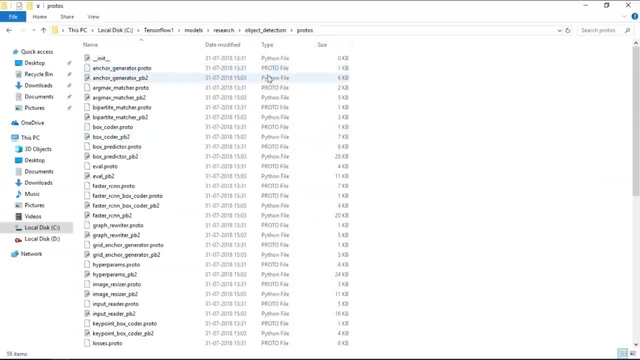 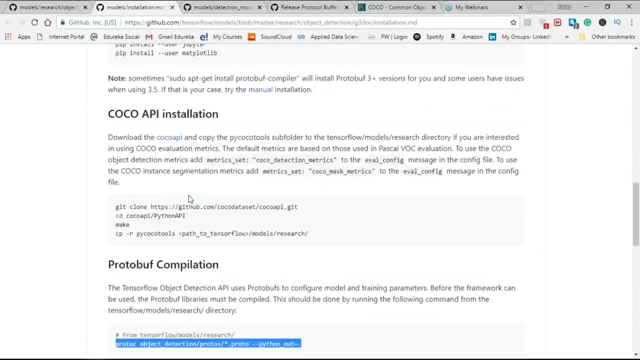 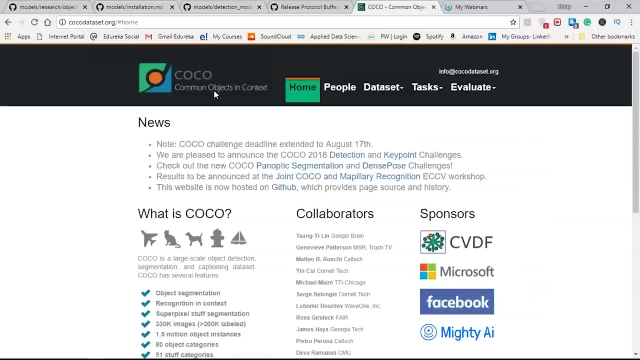 proto files are present here. What you need to do is that. run that command. All the protos file will be converted into python executable files. Now, after that, what we need to do is Cocoa API installation. Now let's understand What is Cocoa now. Cocoa refers for common objects. in context, 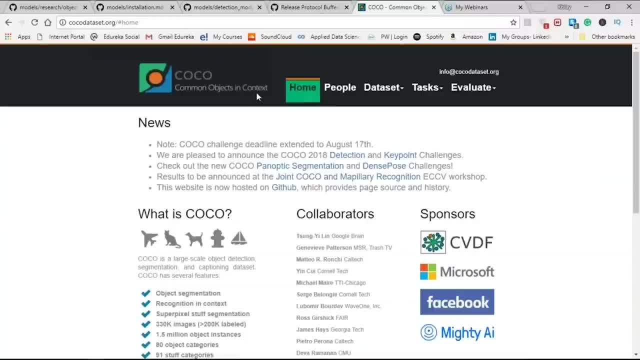 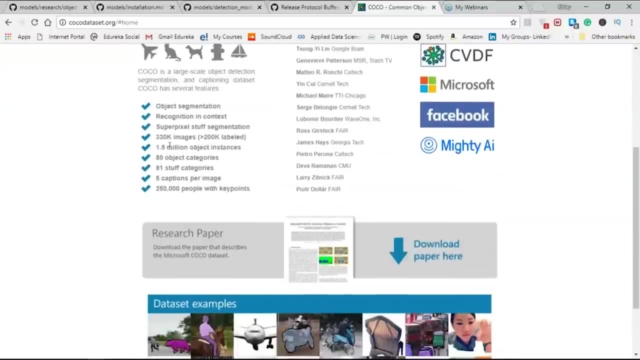 It is a large image data set designed for object detection, segmentation, person key points detection, stuff segmentation and caption generation. Now this package provides MATLAB, python and Luna APIs that assist in loading, Passing and visualizing the annotations in Coco. as you can see, we have 330 K images, in which we have more than 200 K. 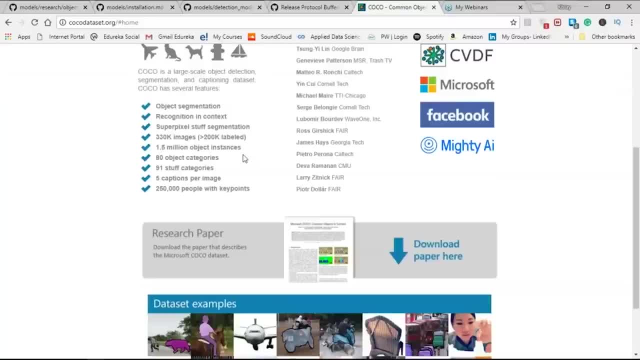 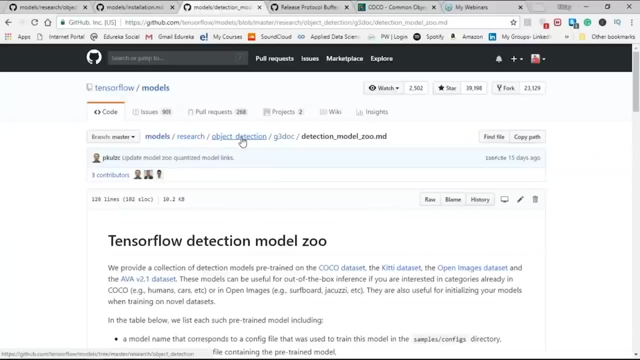 labeled images. We have 1.5 million objects, instances, 80 object categories, We have 91 stuff categories, 5 captions per image and we have 250 people with this key points. Now, when you have downloaded the models, inside models, research and inside the object direction, you need to go to the G3. 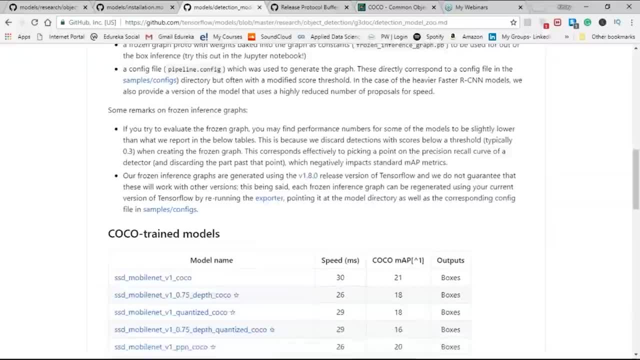 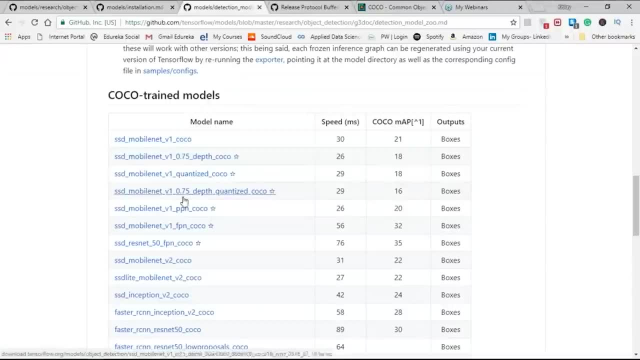 doc in which we have the tensorflow detection models. do now, here We have all the list of models which are trained on the Cocoa data set. So, as you can see, we have the SSD mobile net version 1.. We have the SSD mobile net version 1: PPN Coco depth Coco. 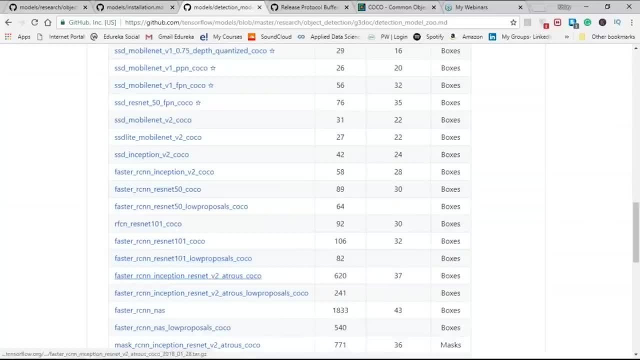 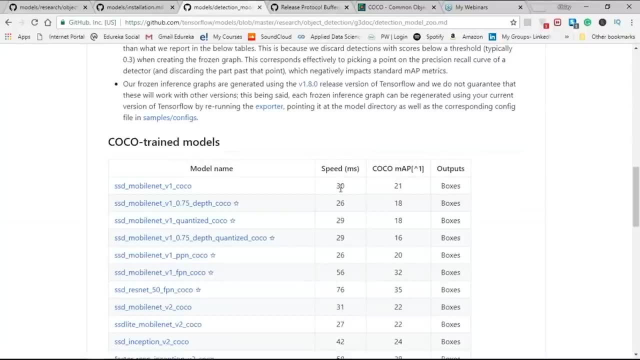 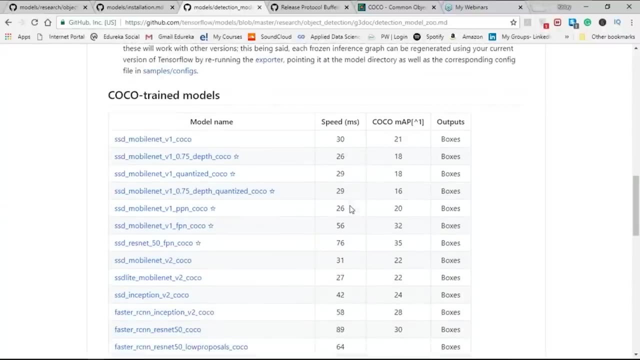 We have the SSD inception, We have faster RCNN, We have different mask RCNN inception. now, an important thing to consider here while selecting a model is that it depends on your system which model you should use. suppose, if your system is low on GPU but has higher RAM, you can go for a. 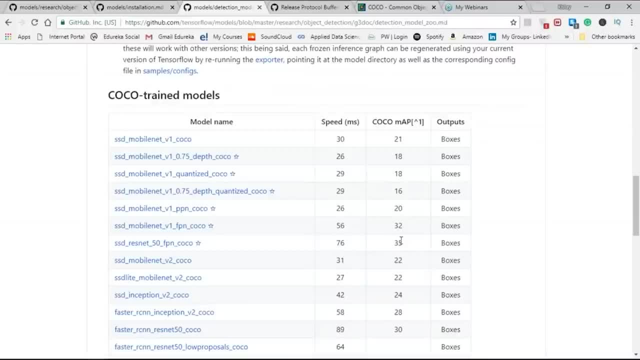 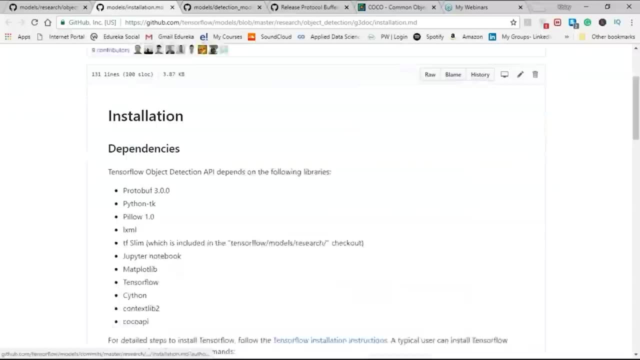 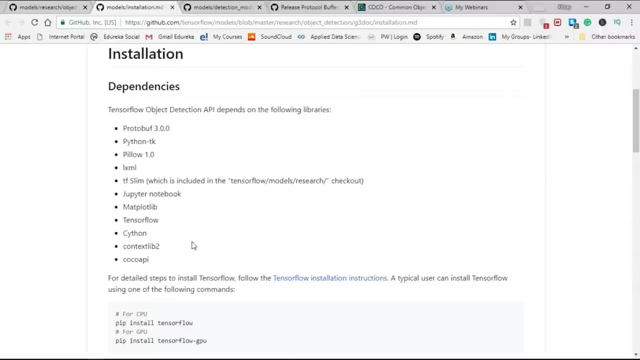 model which has a higher speed and a higher MAP. point Now, this value should always be high if you are looking for a more accurate prediction in your images. So once all your dependencies are downloaded and you have installed tensorflow and protobuf, Let's go ahead and see how we can do the coding now inside. 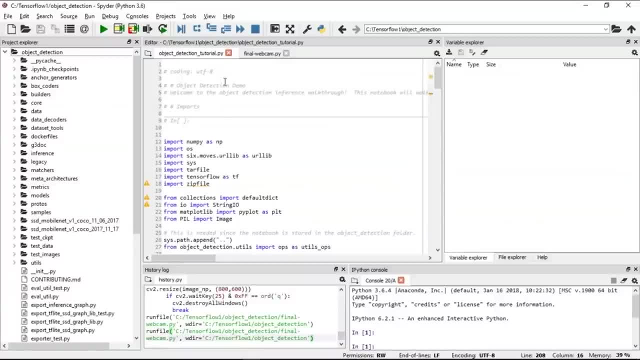 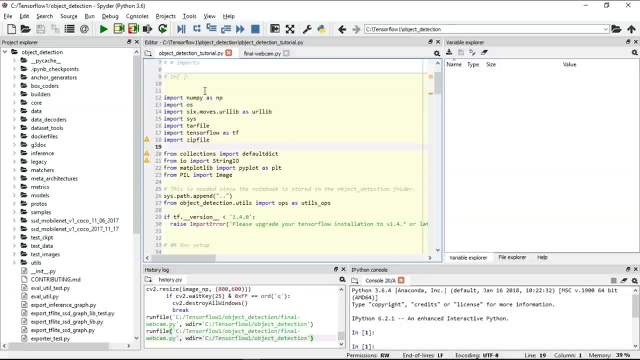 the object detection folder. There is an object detection tutorial. Now, first of all, what we need to do is import all the libraries: the numpy, the OS, the SOS star file. We are importing tensorflow as well. We are operating the collections and the various imports, which. 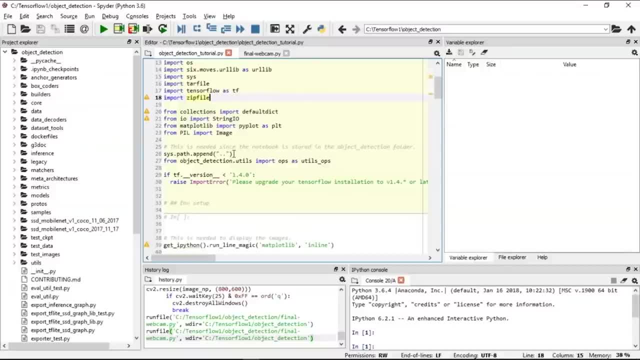 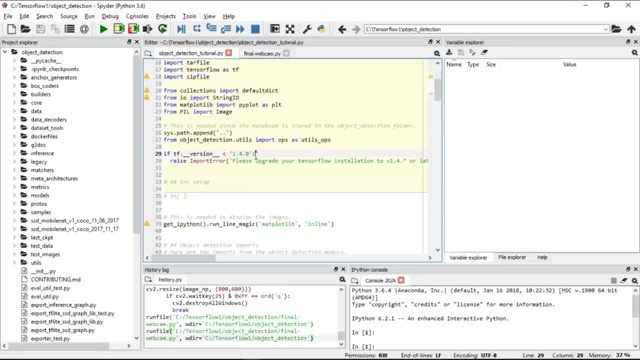 are needed, then we need to append the path of the object detection folder. And finally, if the version of tensorflow is less than 1.4, we need to upgrade, as the latest tutorial suppose the tensorflow object 1.4 and above. So let's run this block by block. 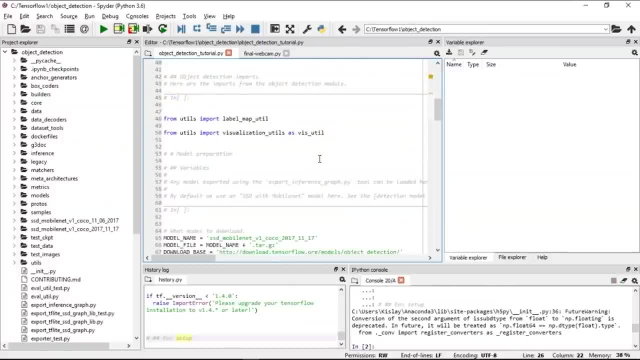 So, first of all, let's load all the libraries Now. next, what we are going to do is import the object detection module, some of the labels, which are the label map util, which will be later used to provide the labels to the input images, and based on that, our model will be created. 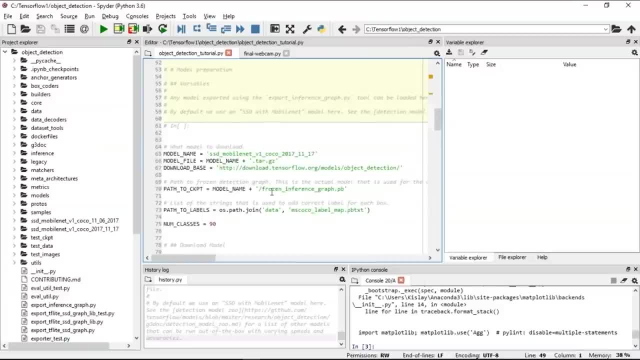 Now, next, what we are going to do is we are going to select which model to download. So, for example, here we are using the SST mobile net, version 1, Cocoa 2007.. So if you go back to the list of the models, you can select any of the given models here. 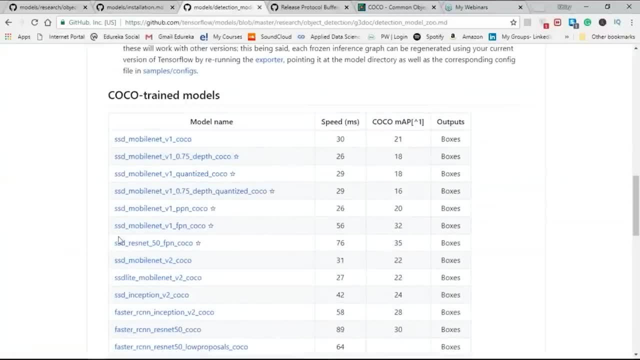 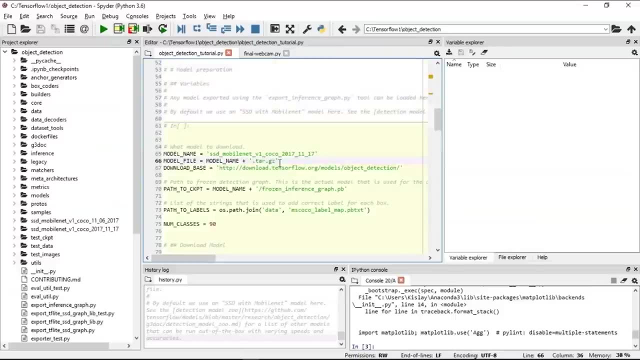 but make sure your system should support the required amount of RAM. I should have the requirement of GPU to support the models which you are selecting. So for this tutorial, I'm using a model which will give me the results faster, So all you need to do is provide the model name, the model. 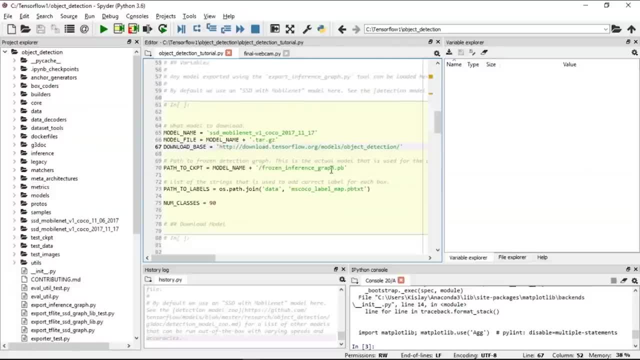 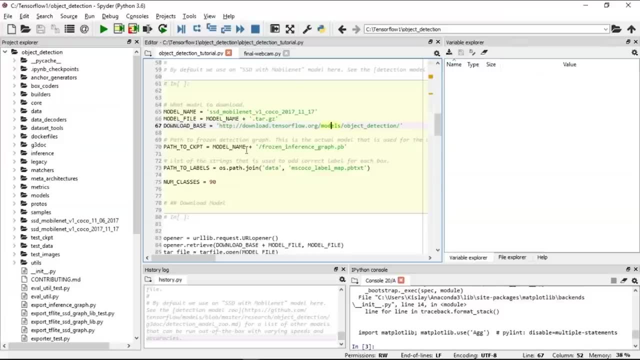 file and the download base from where it should download. Now, as I mentioned earlier that tensorflow works on the graph principle, which is the data flow graph. So what we are going to do is give the part to the detection graph which we are going to use here, which will be supported. 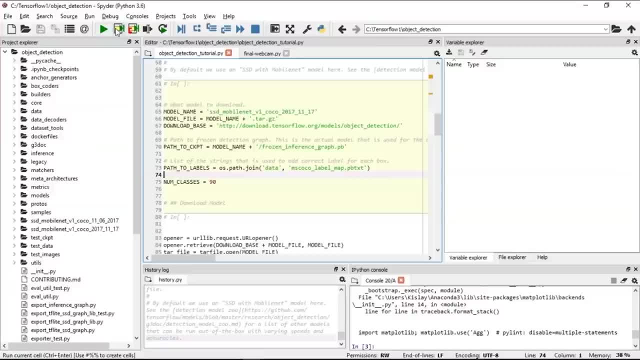 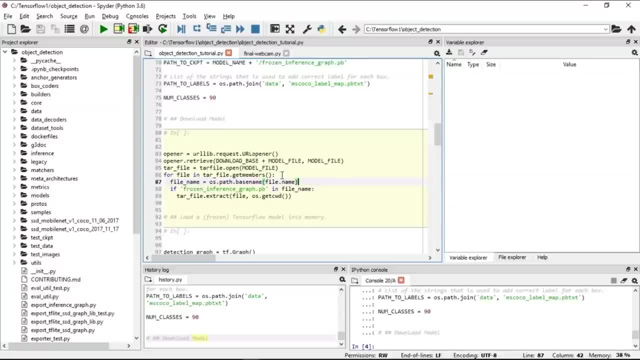 by this model and then we are going to give the part to the labels. Now, to download the models, We have this code which will take the URL and which will download this file and produce the frozen inference graph of that model, which is the SST Cocoa mobile net. 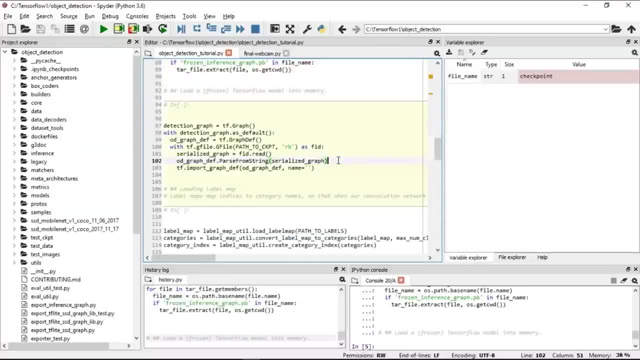 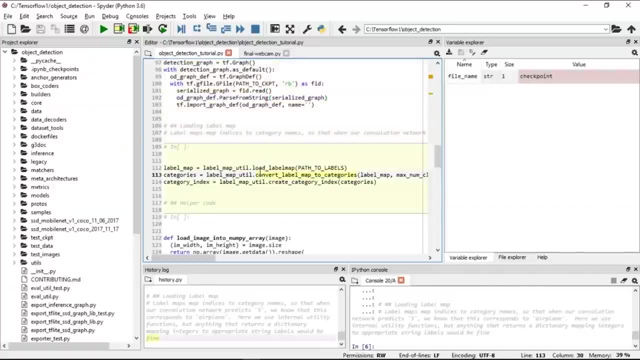 So, once this has been done, we are going to load the graph, which is the frozen inference graph, into the memory. So here we are, using the tfgraph method and tfgraph def to define the graph which we are going to use next. What we need to do is load all the labels and the categories. 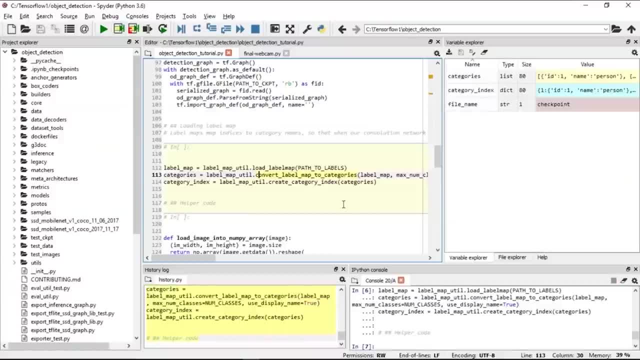 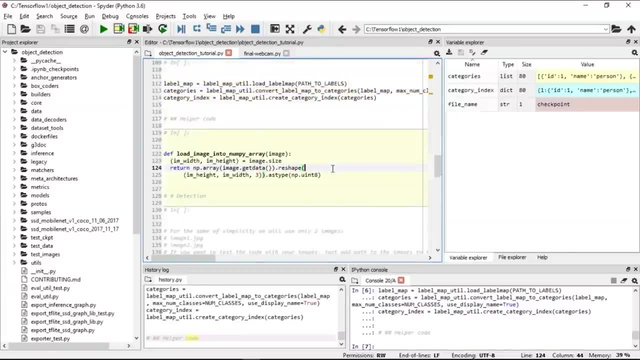 and the category index from our data set. So the data set is Coco. So once we have loaded all the labels and the categories, now is the time to convert all the images Into a numpy array. So this code, which is definition here of the load image into 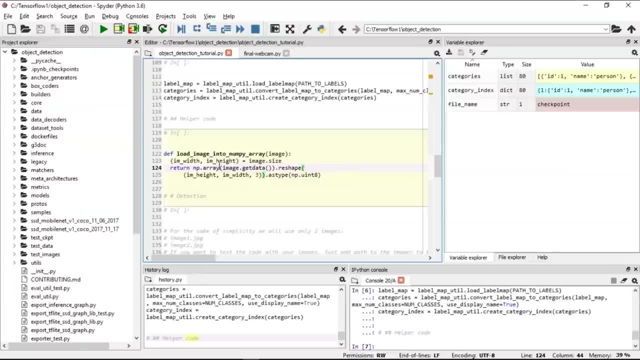 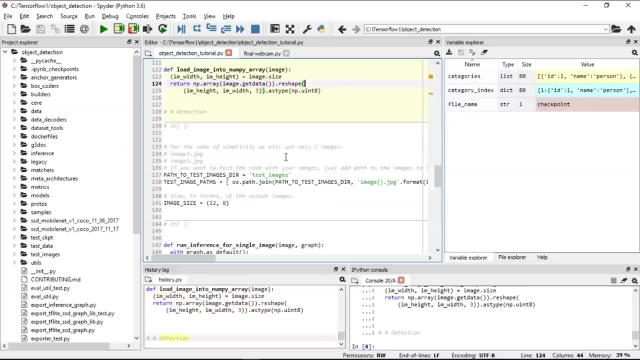 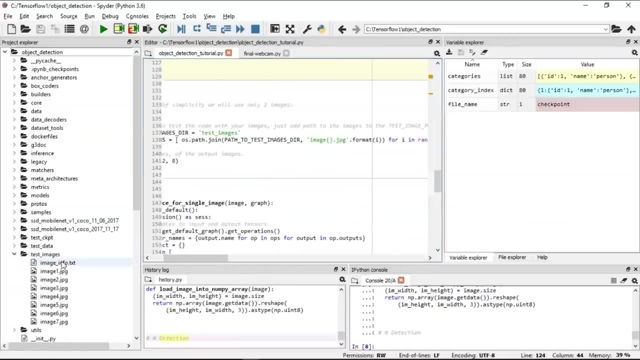 numpy array which we will use later in this code. what it does is takes the images and converts it into a numpy array, So it will be easier for TensorFlow to process it. Now here we are going to provide the images for testing purposes. So, as you can see, we have the test image folder here and 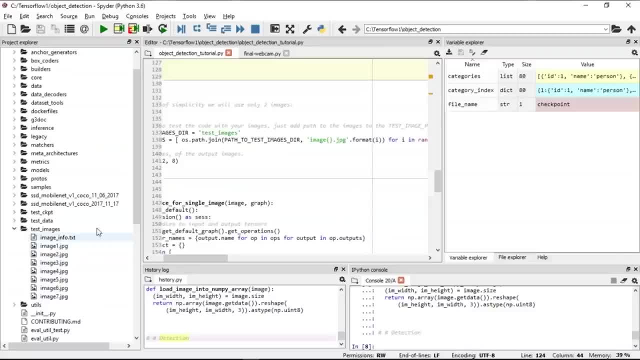 inside that you can input all your images, whichever you want to test upon this model. So, for example, I have taken the range from 1 to 8. it will take all the images named, image 1 to image 7.. So let's load this. 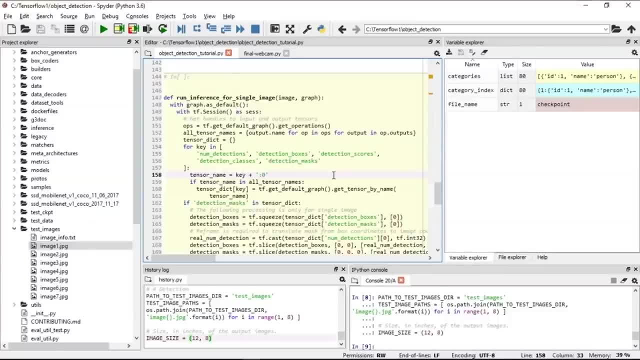 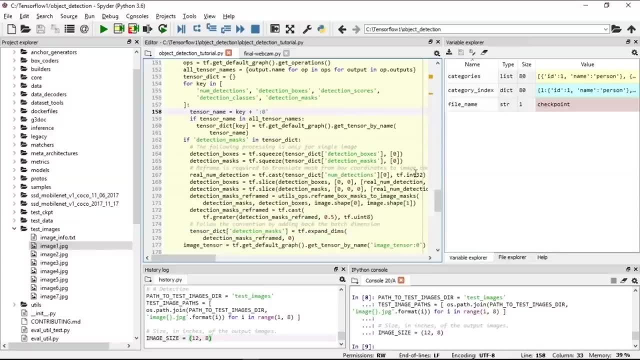 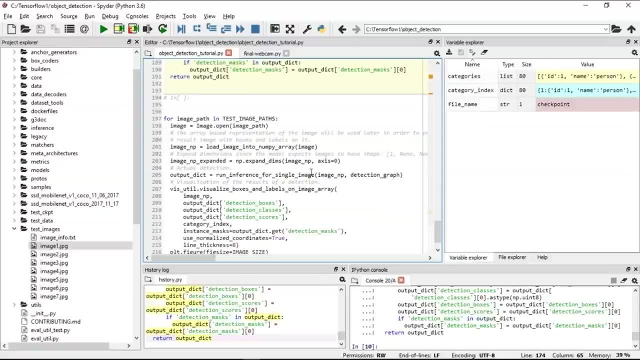 Now this function. what it does is run the inference for a single image. now for a single image. First of all, it detects all the boxes, the detection mask, and provides a certain box on the object it detects. And finally, we have the for loop, the main for loop, in which 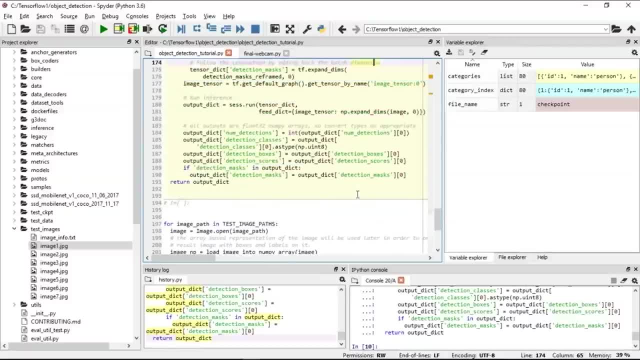 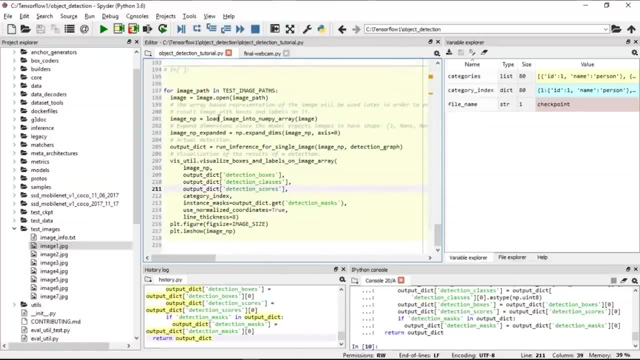 will take the images from the test image path and open them and, one by one, will take all the images and do the inference for a single image, one by one. So, as you can see, we are using the load image into numpy array. We are using the NP dot. expand novel. expand the dimensions. 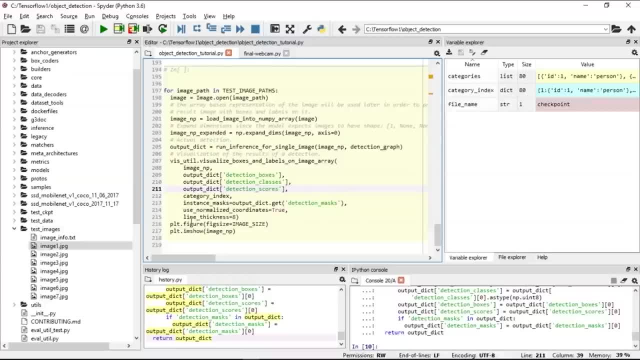 since the model expects images to have the shape, which can be 1, 2, 3, based upon the categories and you can see the output- will get the detection boxes, the detection classes and the detection score And, finally, we are using the matplotlib to show us the image. 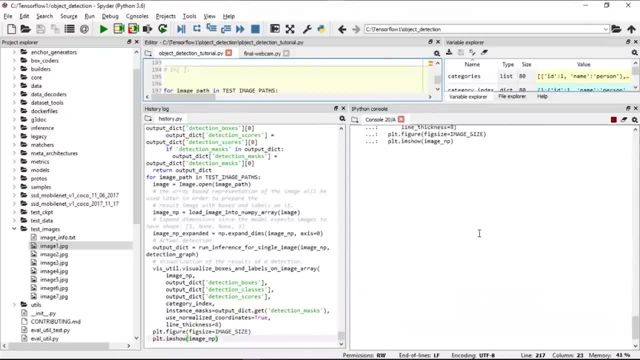 So let's run this. We'll get our output here, So this might take time, depending upon the processor which you are using or the system which you are using. So since we have taken the model which will take the least amount of time, this shouldn't take much time. 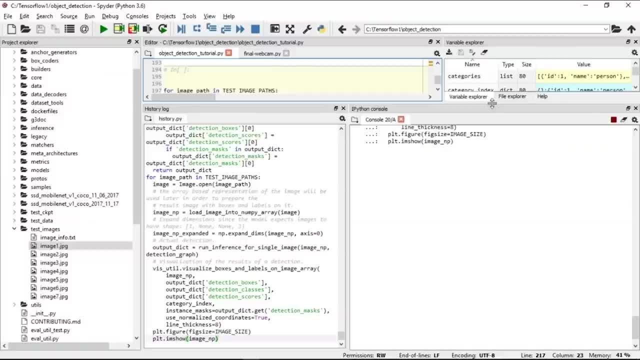 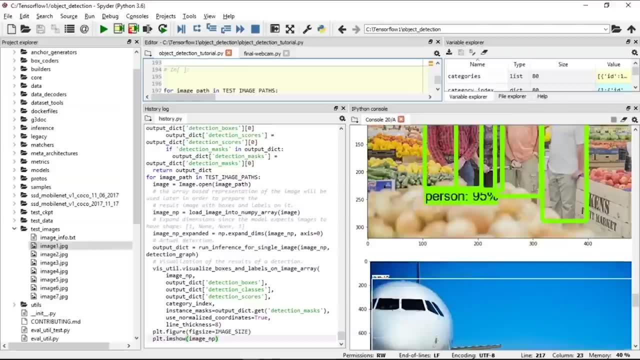 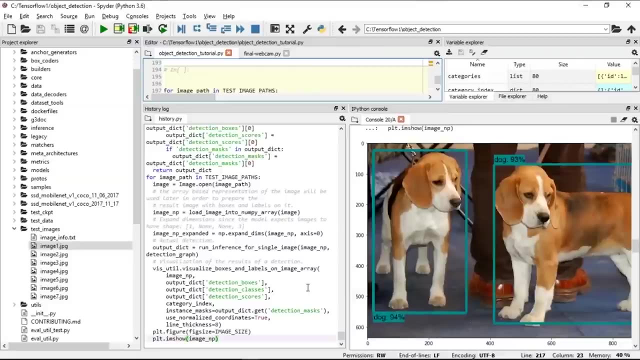 But then again, tensorflow is heavy and the tensors are multi-dimensional arrays, as I explained, which do all the heavy computation. So, guys, here we have the results. So, as you can see, let's begin from the start. as you can see, it identified the dog as a 94%. it has provided a box, the label and the score. 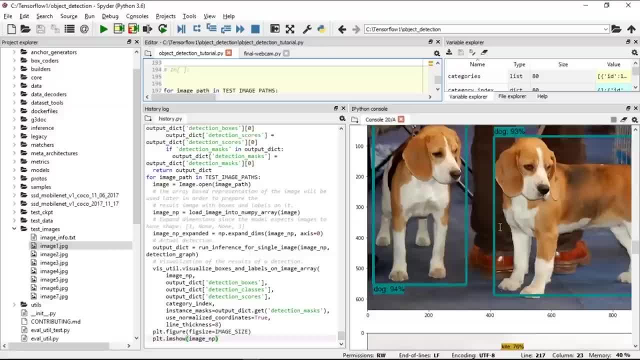 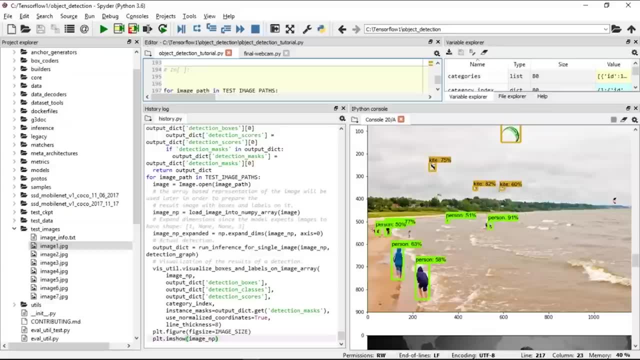 which is the detection score, how much it is similar to all the images which has been imported in the cocoa data set. So, as you can see, here we have the person, the various percentage. we have kite: here We have a tie detected. it can detect objects in. 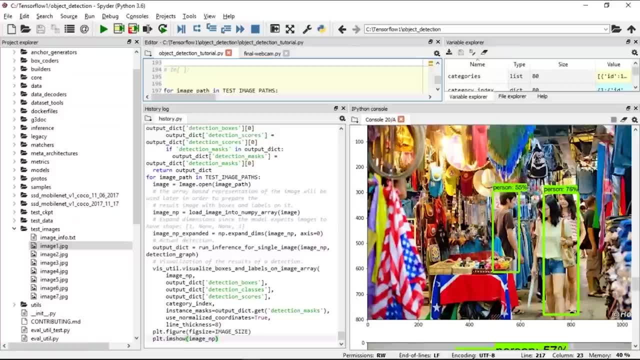 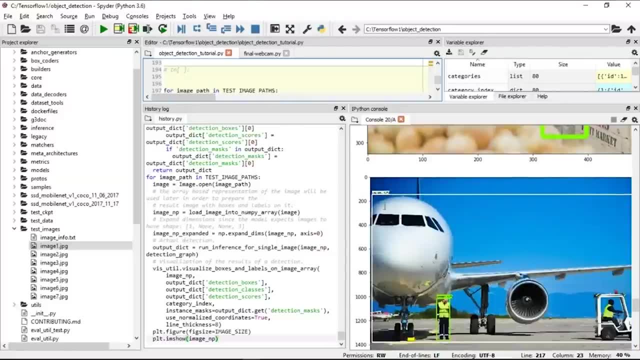 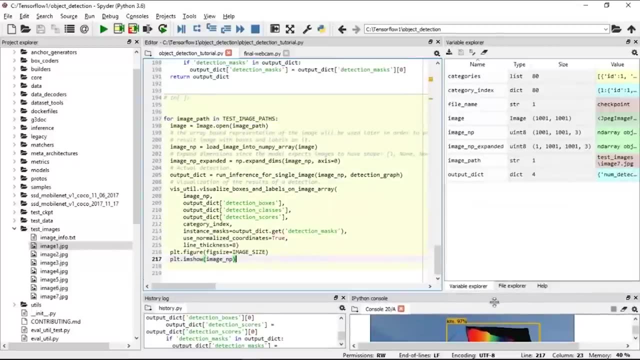 Such a heavy background as you can see the person are so much camouflage in the background, but still it has managed to score that person. As you see here, it has detected an airplane person kite. Now you can use your own images. All you need to do is copy that images into the test image. 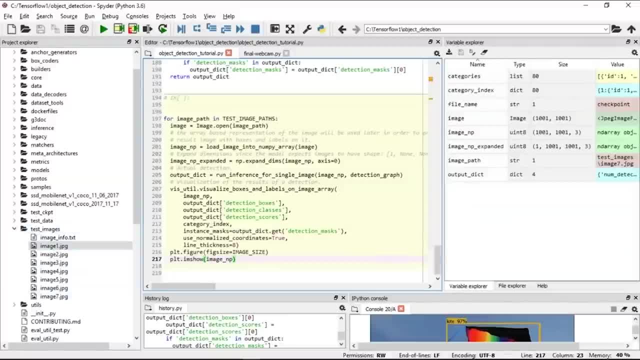 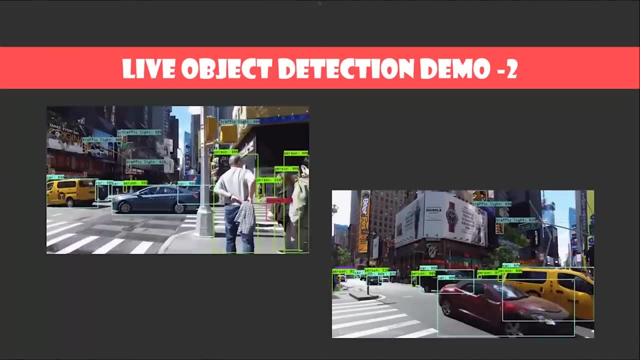 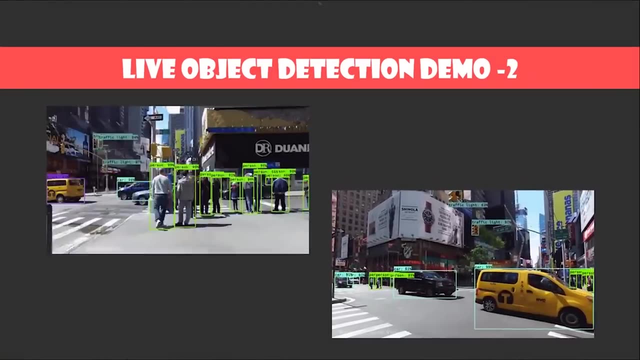 folder and use the naming convention provided here as the image one, image two. So now let's go ahead to our second demo, which is the live object detection. Now in this demo we will use the open CV. So let me show how we can do the coding here. 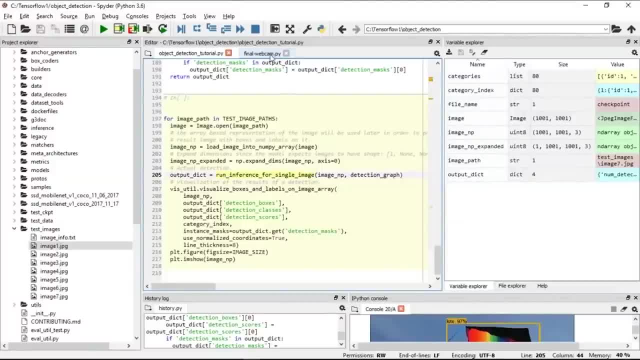 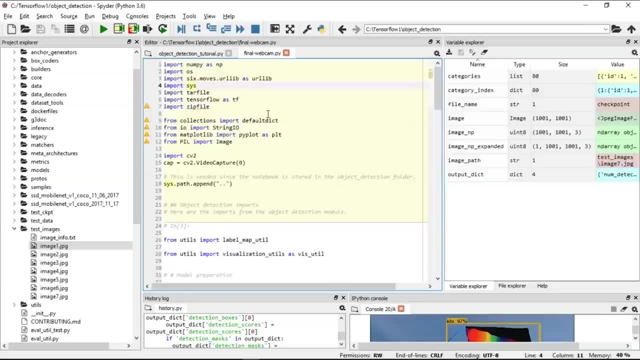 So, first of all, all you need to do is copy all the code and paste it into another python file. So, once you have pasted, the major changes which are involved in the live detection of the images is that we are going to use open CV. 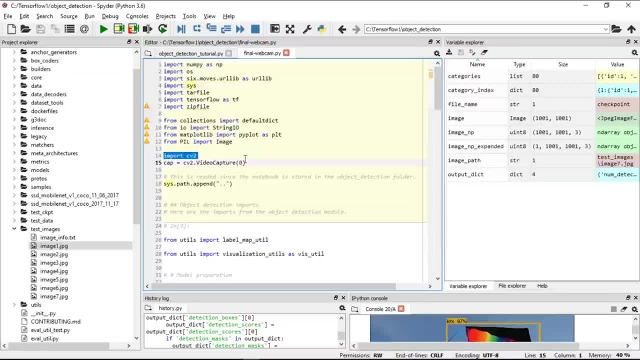 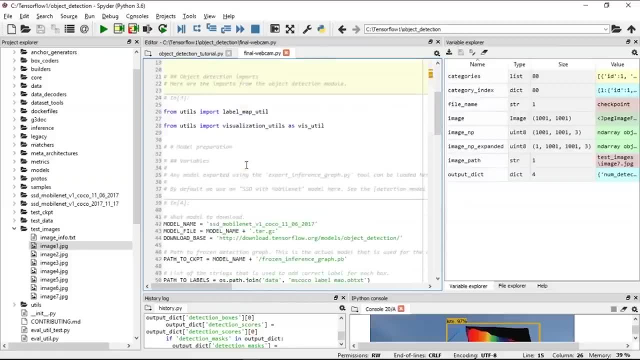 So first of all we need to import CV to here, as you can see, and we have defined an object- CAP- that will capture. So we are going to use CV to dot video capture. Here You can change the model which you want to download, because 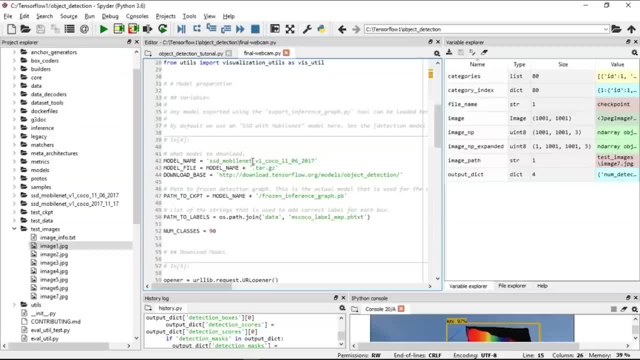 if you have a higher GPU and the refresh rate of the images is also high, You should take a model that has an equal balance among the speed and also the accuracy of the image detected. So all this will remain same, and I'll show you what all changes. 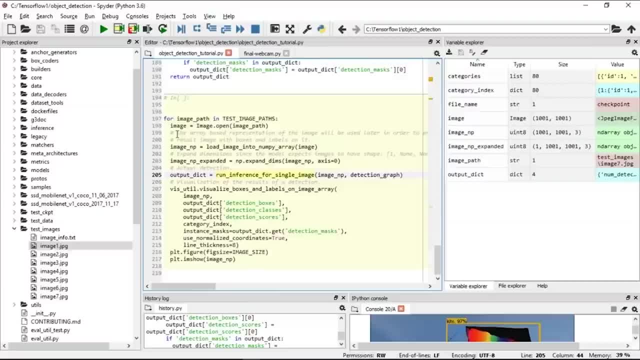 we need to make. So what you need to do is for image path in test images. As you can see, we do not need this code, because our images will be not coming from the test image folder, as it will be coming from our webcam. 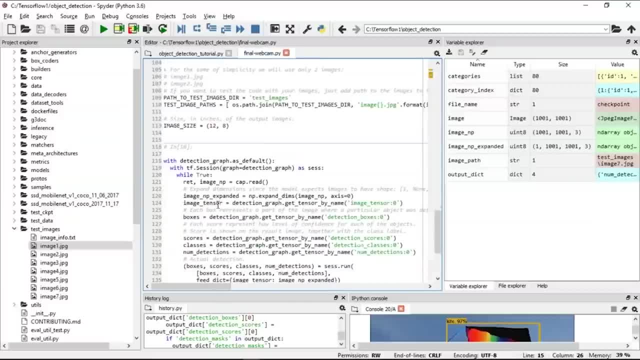 So you need to remove these codes and instead of that, you need to do is input these line of code, which is: while true return, and we'll use image NP, as that's the exact name which is being used here by the tensorflow code, and we are going to use CAP dot read. 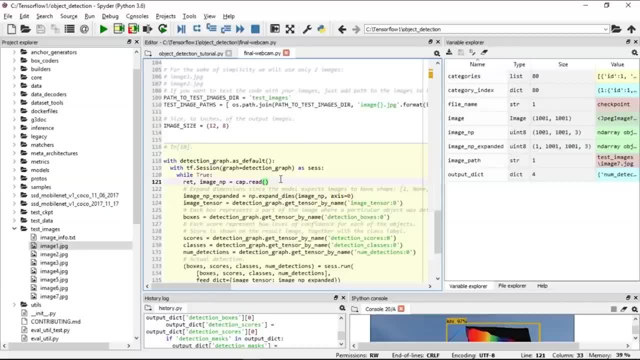 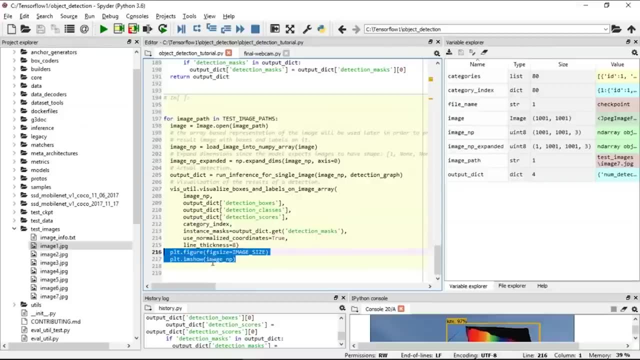 So what it will do is it will take the input of the video which is coming through the webcam, and then we need to remove these two lines as well, which is the PLT dot figure and the PLT dot image show, because we are not using matplotlib anymore and we'll be using the 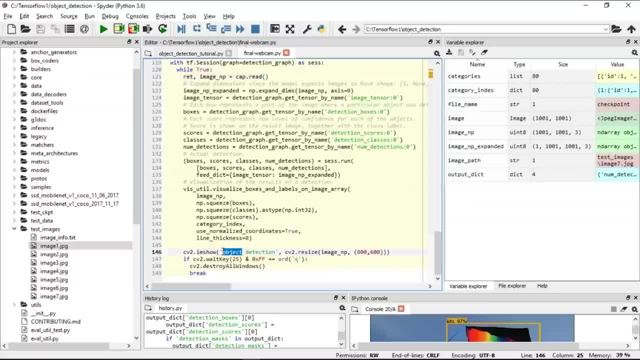 open CV. So we'll do CV to dot M show and this is the name of the window which will come up and, for instance, we are resizing The image to 800 is to 600.. Now we need to provide this code as well. 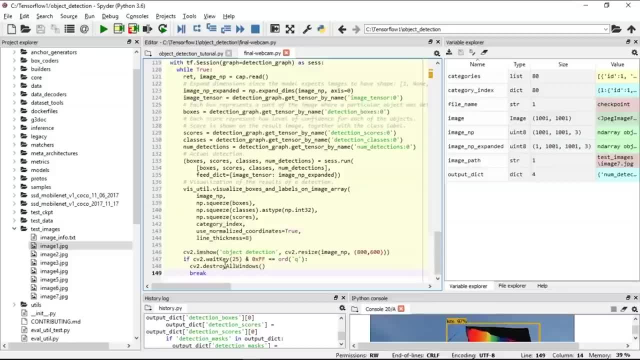 Now what we'll do? it is the wait key option of 25 seconds, And if we press Q or for 25 seconds, the screen is black. It will automatically destroy all the windows and break out of the loop. So here you do not need to run this code, which is the path. 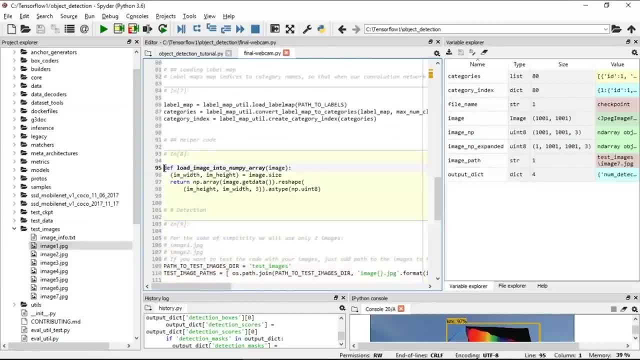 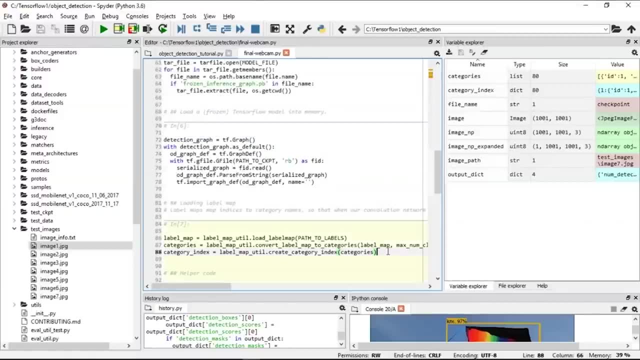 to the test image because it's not needed. you do not need to convert the images into the numpy array, because all the images coming through the open CV is already in an array format or a structured format. So let me just open another console for you. 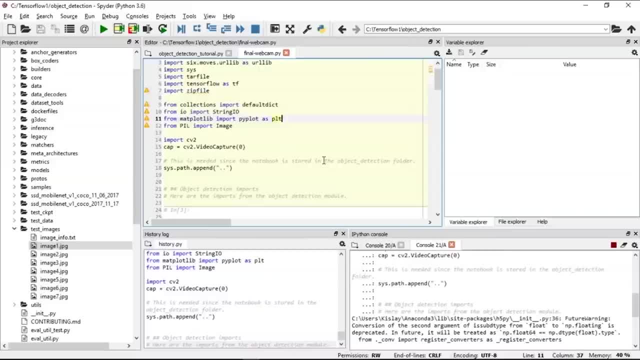 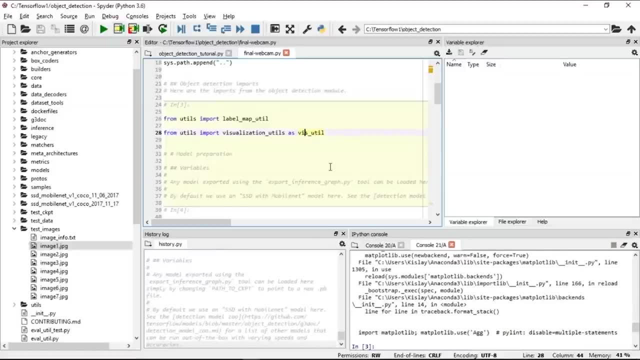 So, first of all, we'll import all the necessary libraries, the CV to. we have the tensorflow. We are going to import the label apis and the label frameworks which are used here. Now we have already downloaded this model. What you can do is again run this code. 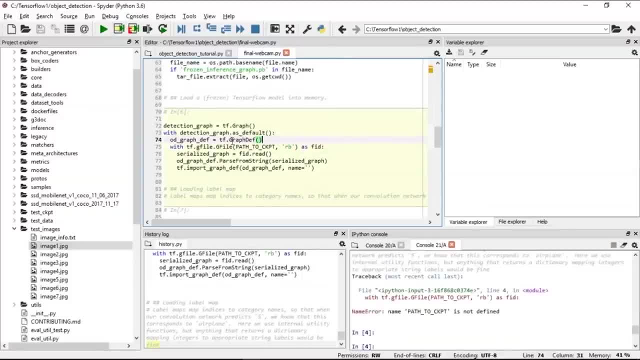 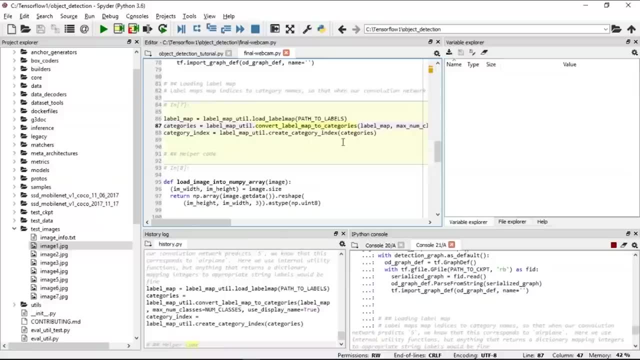 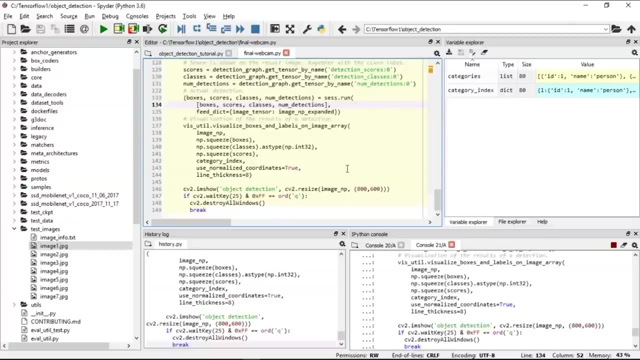 but that won't help either. Next, you need to load the frozen inference graph. After that we need to load all the labels And finally, we need to run our final code block, which is the object detection, which will call all the definitions which have provided earlier. 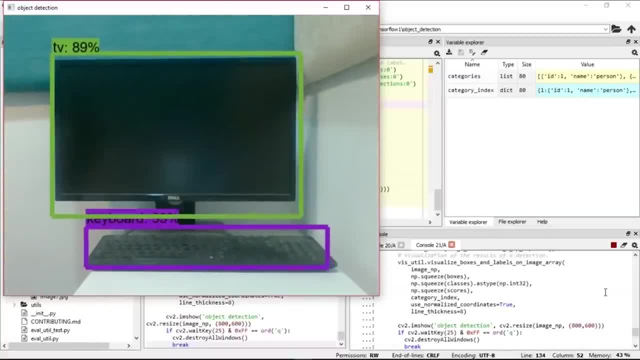 So, guys, as you can see here, it has opened up a window of 800 cross 600 and, as you can see, it has successfully detected the TV, as 92% of TV, and keyword also has been detected at 90%. So, as you can see, it is also detecting the bottle which we. 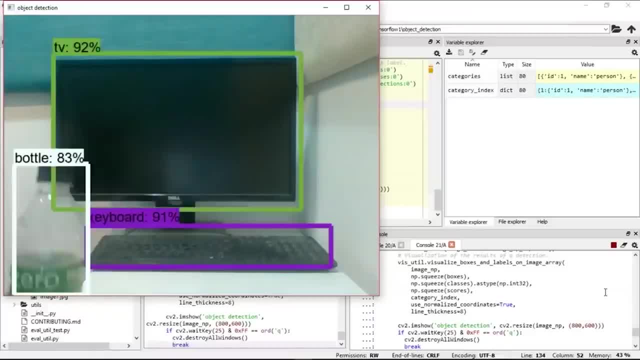 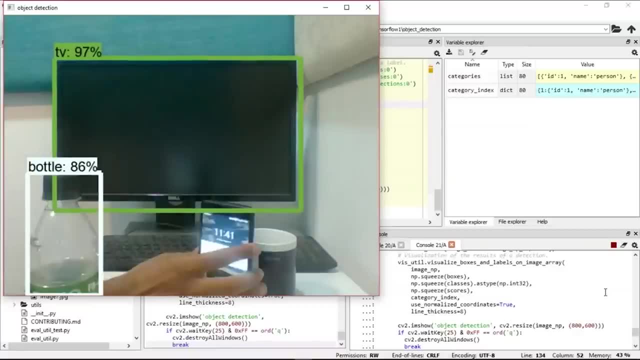 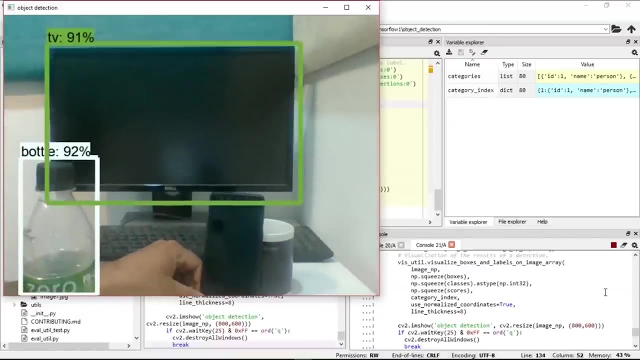 have provided here as 92%. It is also detecting the cup as well. So what about the phone? Let's see if it detects it as a cell phone or not. Let me just keep it in the frame. As you can see, it has detected cell phone. 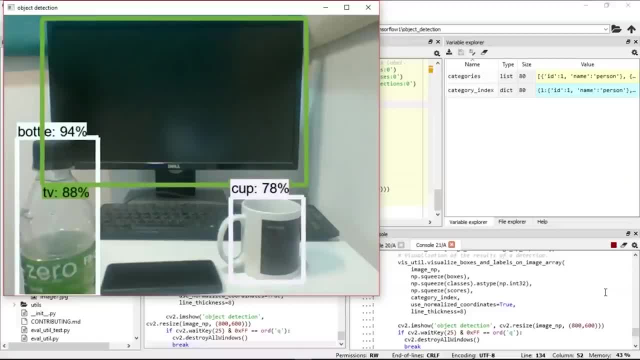 Now the refresh rate of this particular model is slow because we needed the result fast. But if you have a higher GPU system and the CPU is good, you can use more advanced model with the higher refresh rate. So, as you can see here, it has detected clock. 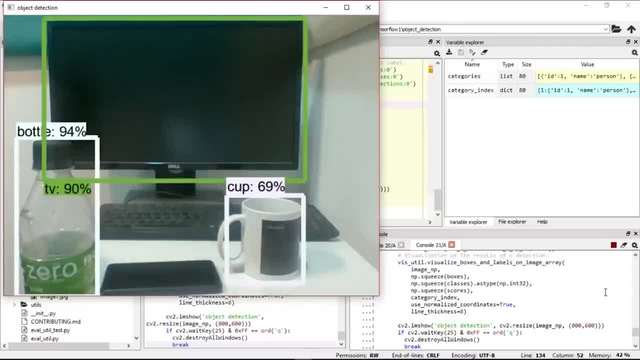 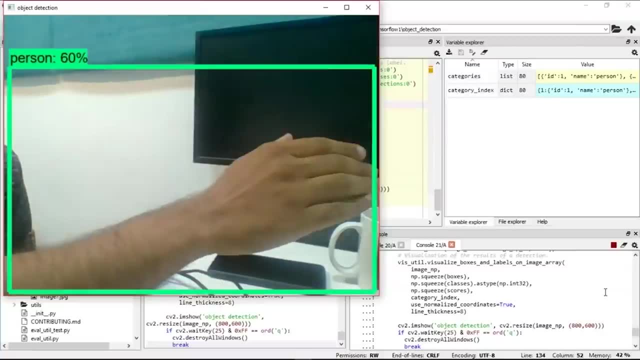 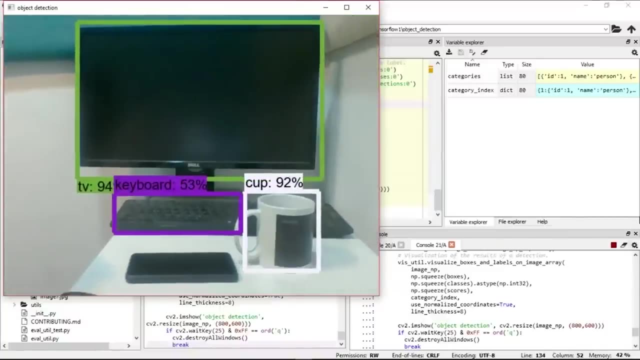 the watch as clock and the moment it receives any part of human Body in the frame. as you can see, If my hand is there, it will detect it as a person. Okay, You can see. it is detecting the TV, the cup. It will also detect the phone as well. 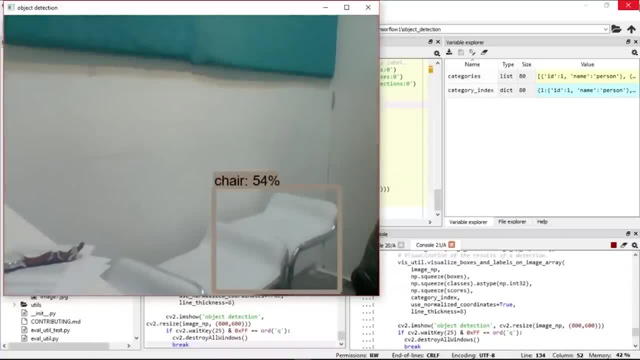 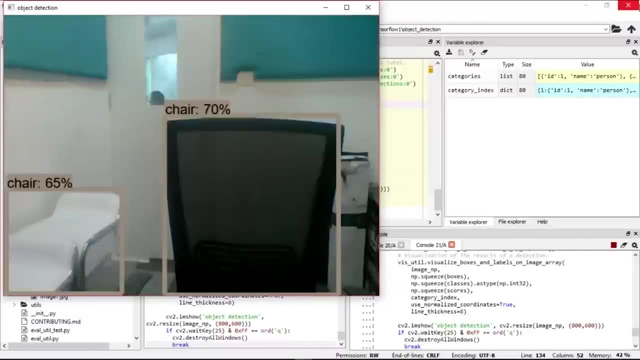 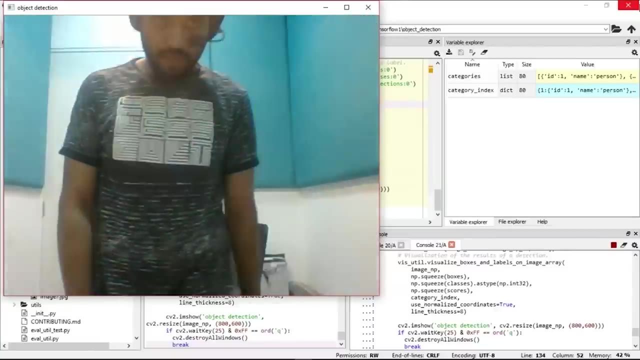 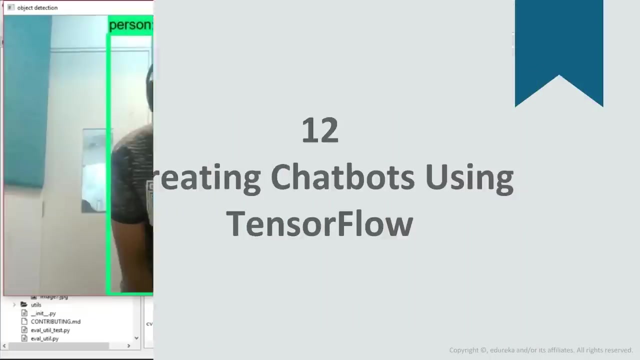 Cell phone. So, as you can see here, it is also detecting the chairs. So you can see it has also detected my chair as well. So, guys, as you can see, it has also detected me as a person. that is good to know In today's session. 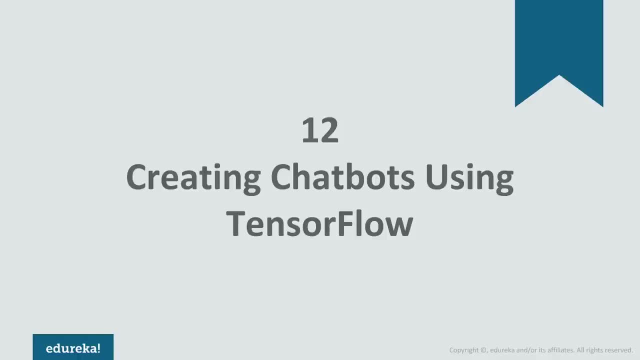 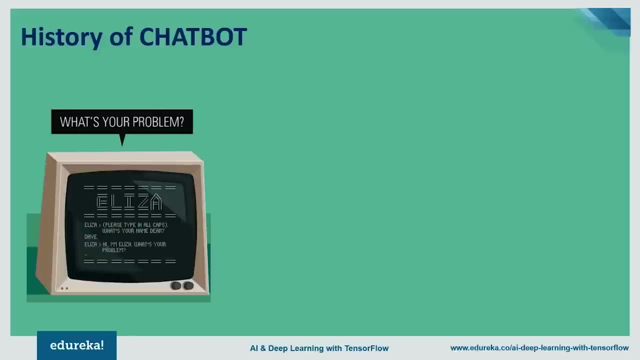 we will learn how to create a chat bot using tensorflow. Now, before we get into the details of chat bot, let's first find out. why do we need them Now? the first chat bot was named Eliza. that blurted out canned lines. 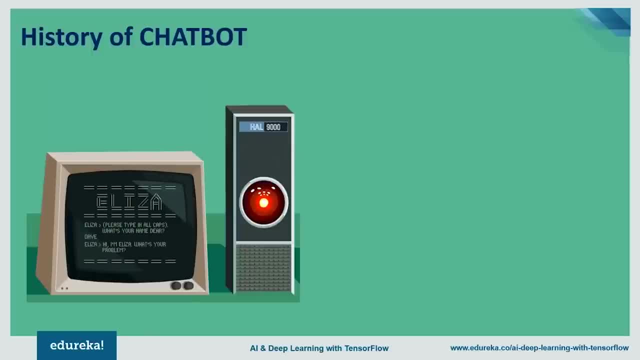 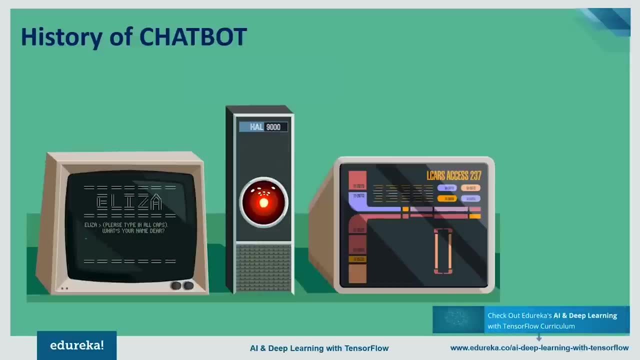 for certain keywords using programmed scripts. Many users developed an affinity towards her, even after knowing that the program simply followed a script. since then, chat bots have advanced beyond scripts and rules. the new generation chat bots can encourage human like conversations with the help of artificial intelligence. 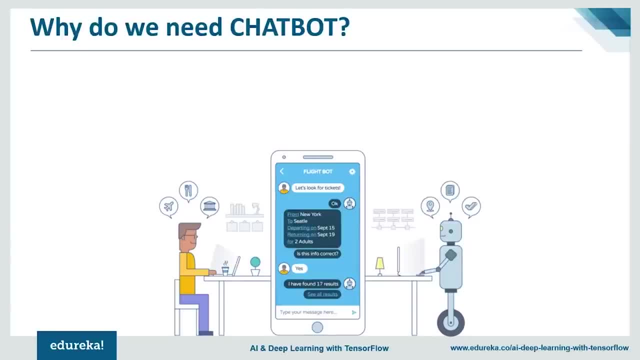 Now, it all started with one question: can machines think? the concept of chat Bots came into existence to check whether the machines could fool users and make them think that they are actually talking to humans and not robots. on the other hand, with the success rate of chat bots, different companies started using the machines. 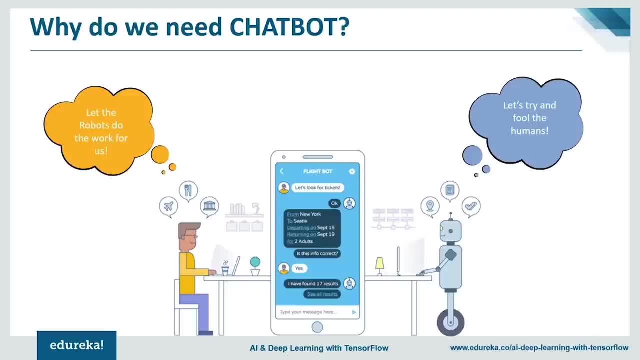 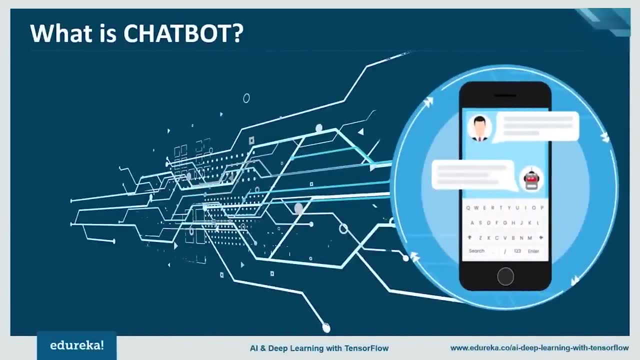 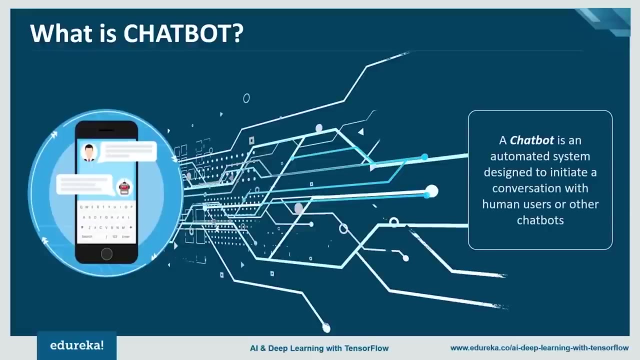 for having conversations with their customers about everything which made their work simpler and reduced the need of manpower. So now that we know the importance of chat bots, Let's have a deeper insight about what are these and how do they work. The evolution of artificial intelligence has seen its peak. 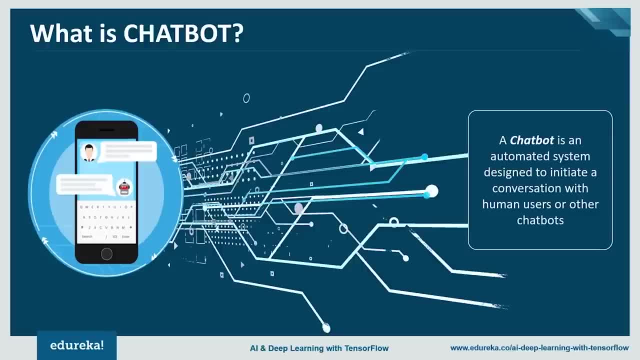 in the recent times, and chat bots are a faint splash on a huge wave of progress. A chat bot is an assistant or an automated system that communicates with us through text messages. It integrates into websites, applications or instant messengers and helps entrepreneurs get closer to customers. 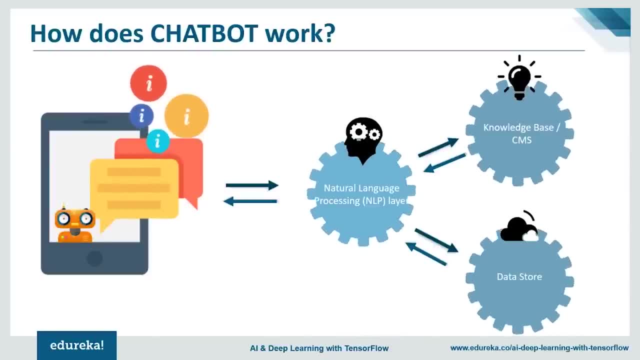 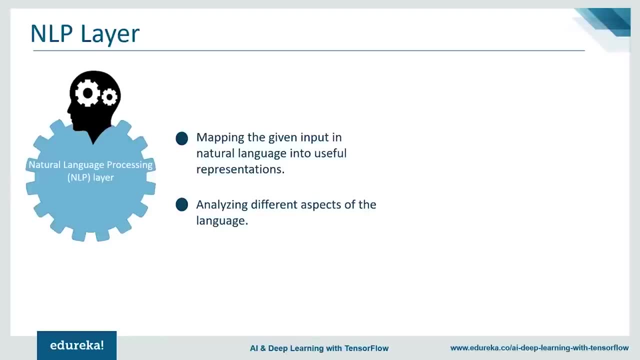 Now let's have a look at the number of steps involved in the working of a chat bot. Now, the first step is to convert the user Text or speech into structured data in order to find the related answers. Some of the natural language processing steps include sentiment. 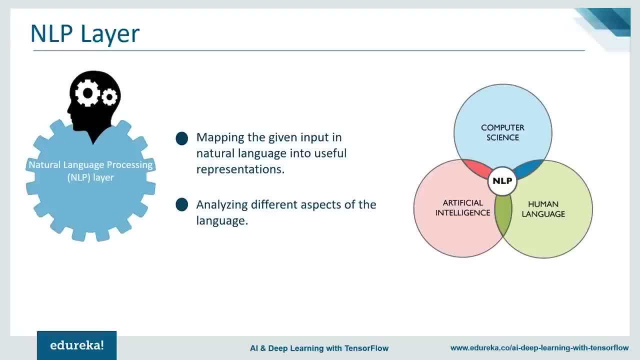 analysis, tokenization, normalization and dependency. passing now, chatbots process the text presented to them by the user before responding according to a complex series of algorithms that interprets and identifies what the user said, then infers what they mean and determine a series of appropriate responses based on. 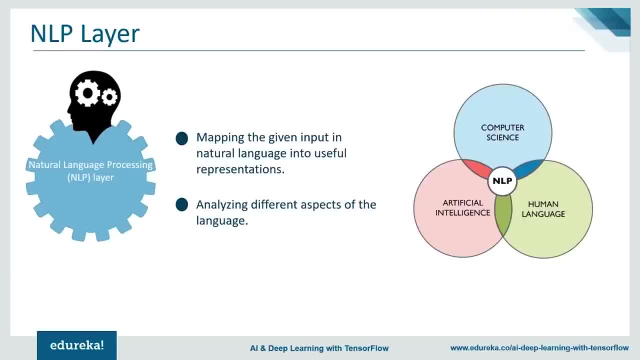 Information. any system or application that relies upon a machine's ability to parse human speech is likely to struggle with the complexities inherent in elements of speech such as metaphors and similes. now, despite these considerable limitations, chatbots are becoming increasingly sophisticated, responsive and more human-like. now, 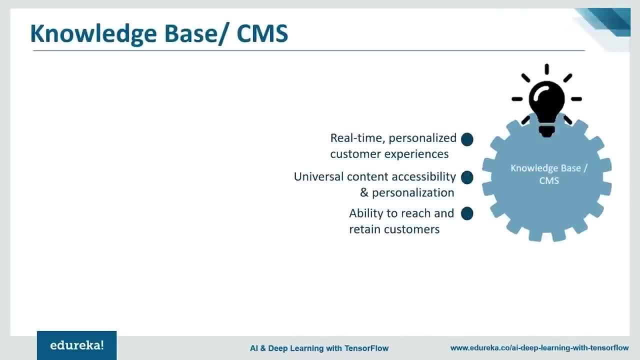 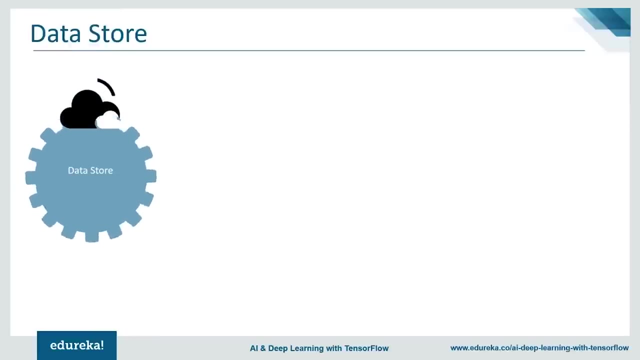 it provides a real-time customer experience along with universal content accessibility. It is believed that chatbots Will take over almost 85% of all customer service interactions by 2020. now, training a chat bot happens at much faster and larger scale than teaching a human humans customer service. 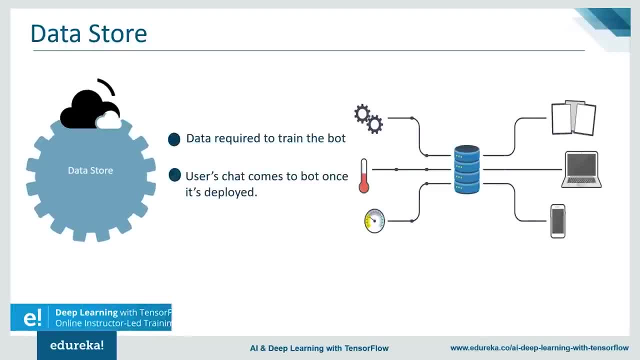 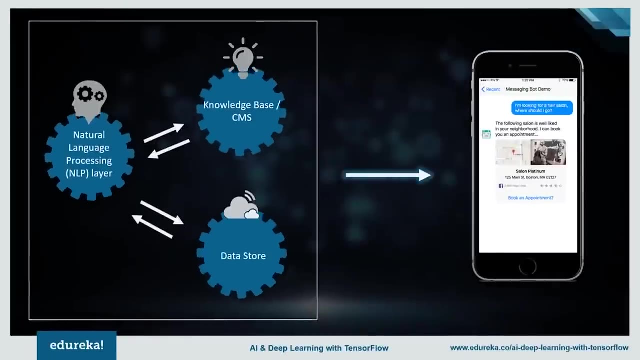 representatives are given manuals, while the customer support chat bot is fed with thousands of conversation logs, and from those logs the chat bot is able to understand what type of question requires what type of answers. now, the working of all these steps together Provides us the required chat bot, which response to the users. 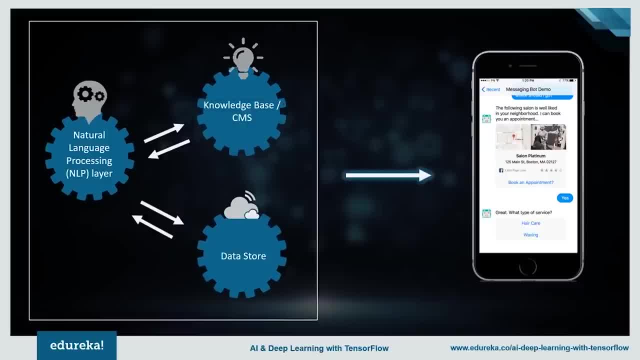 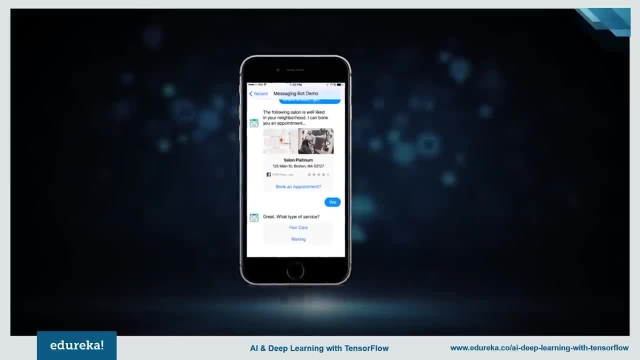 or customers and makes them believe that they are talking to humans and not robots. So we have talked about the steps involved in the working of a chat bot, but there are certain things that need to be kept in mind while creating one the five important key points that should be: 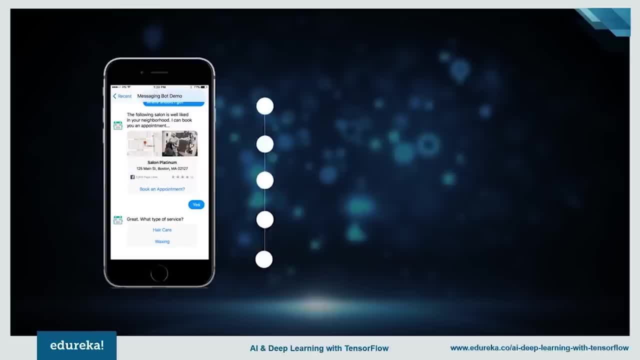 considered for a chat bot to work perfectly or more like a human includes the volume of conversations, consistency of the agents, training the agents, Length of conversations and complexity of the incoming and outgoing questions. So far we have talked about how the chatbots work and how they 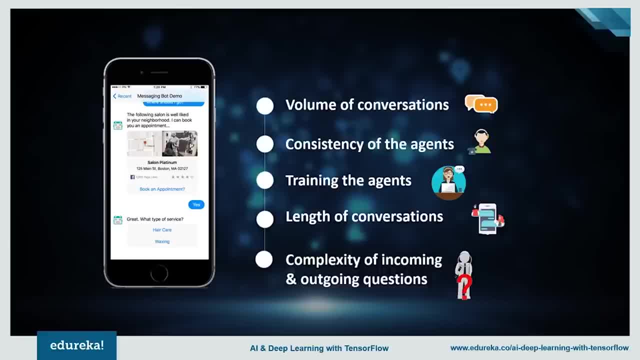 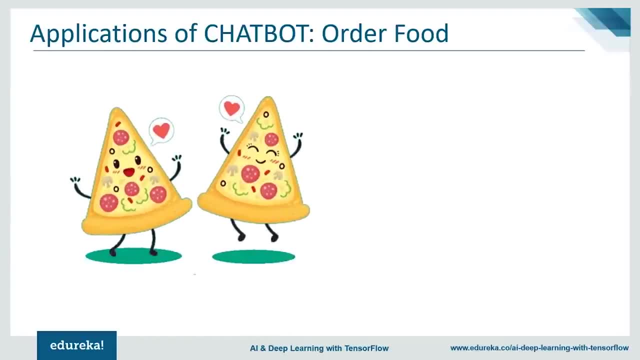 are used to initiate conversations with users or customers. Now let's take a look at some of the applications of chat bot. in our everyday life, ordering our favorite food has become much easier Now. we can take help from the online assistant and select our option for delivery. a few quick steps through Messenger and 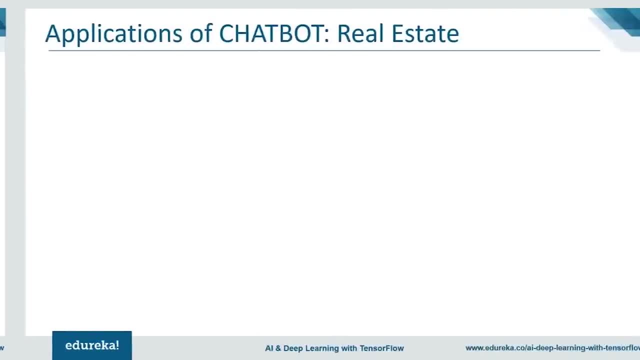 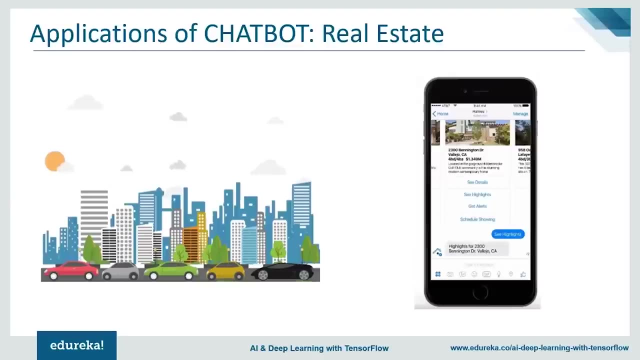 your pizza Will be delivered at your doorstep. If you're looking for the perfect house or a society, the chat bot will also work as your personal assistant to find that perfect house for you in your desired locations, without much hard work. Now we all have booked flight tickets online, but with the 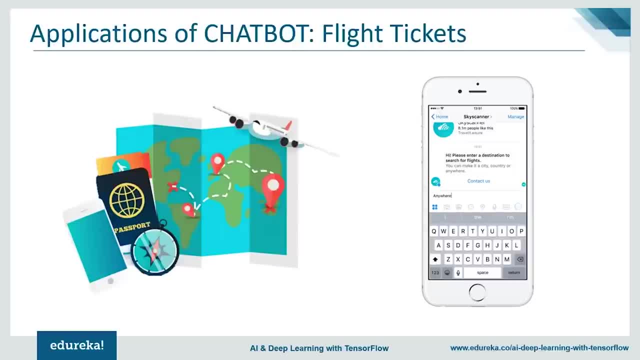 help of a chat bot, the work has become even more simple. All you have to do is provide your destination, and it will find you the flights suitable for your journey, and you can book your tickets with just one click. not just that it, It can also help you in selecting the dress you want, or the 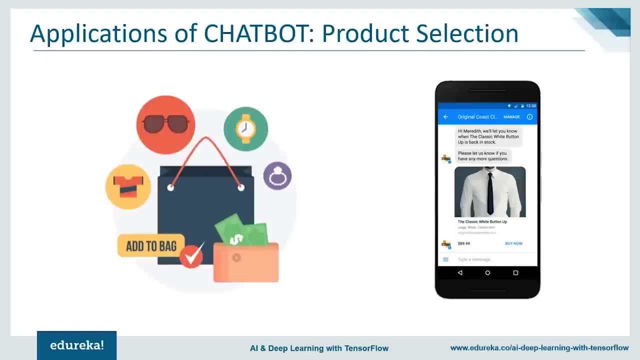 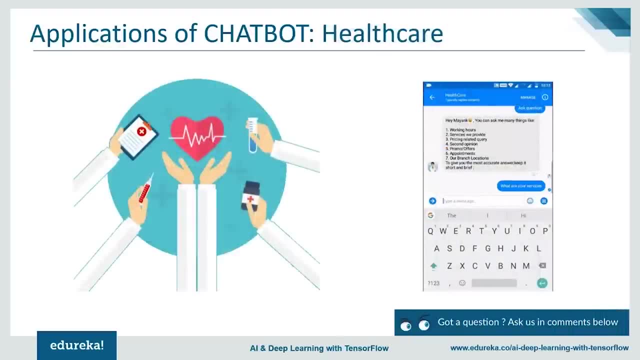 shirt that will fit you. They can help you in finding the right product based on your preferences. The chatbots are not only helpful in case of food delivery or booking flight tickets. They provide a great assistance in case of emergency as well. It provides you with all the information that you would need. 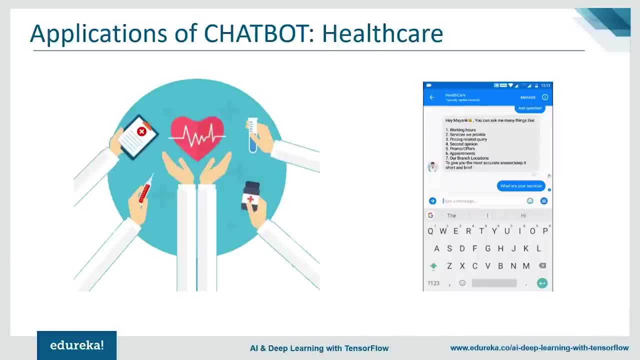 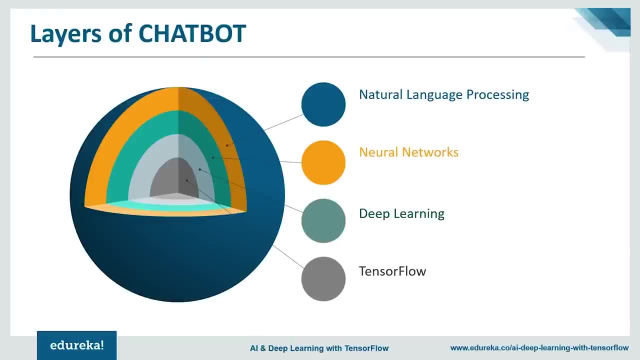 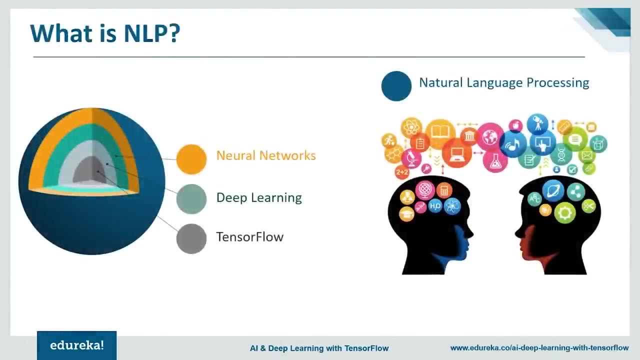 during a medical emergency, such as nearest hospitals working hours, medicine delivery and a lot more. now let's discuss the layers of chat bot In details. The first layer is the natural language processing layer. now it is the ability of a computer program to understand human. 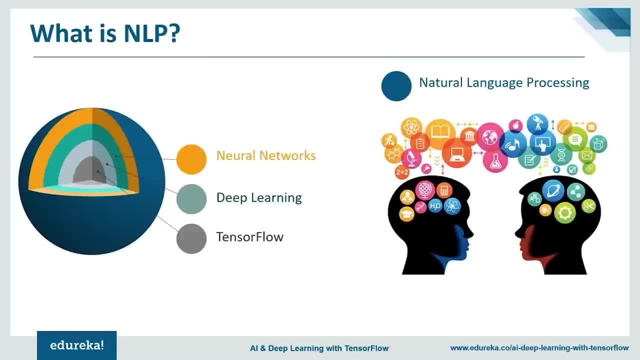 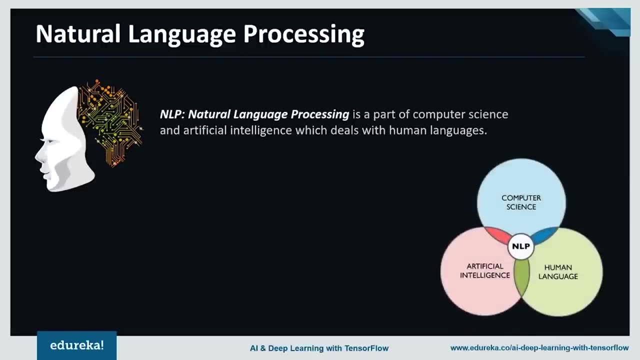 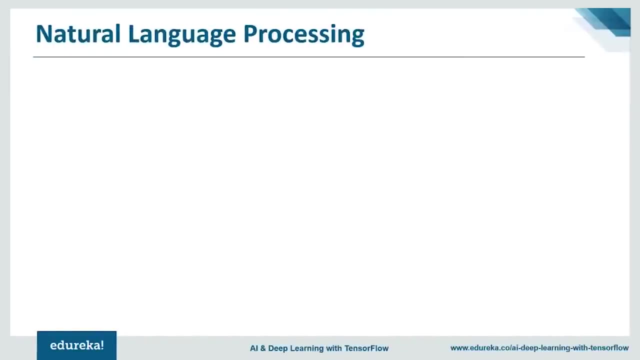 language as it is spoken, and it is a component of artificial intelligence. Now the machine interprets the important elements of the human language sentence, such as those that might correspond to specific features in a data set, and returns an answer. Now there are two main components of NLP. 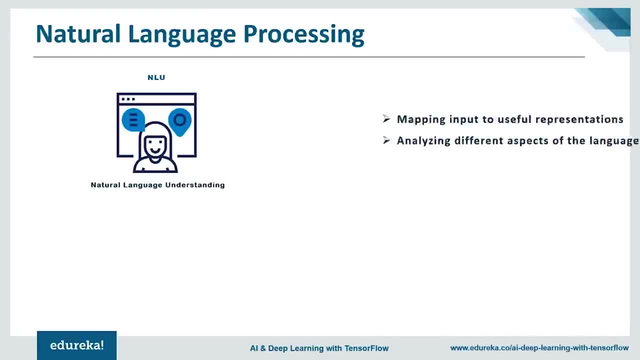 The first one is the natural language understanding. It Maps the given input in natural language into useful representations and analyzes different aspects of the language. The second component, natural language generation, is the process of producing meaningful phrases and sentences in the form of natural language from some internal representation. 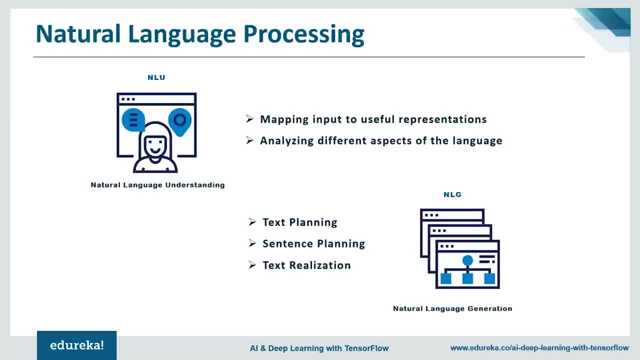 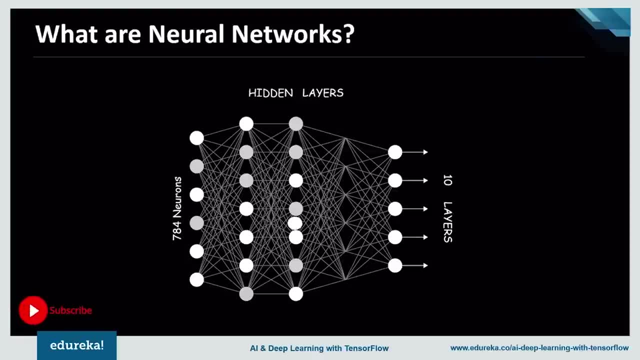 Now this involves text planning, sentence planning and text realization. The next layer is the neural networks. It is an information processing Paradigm That is inspired by the way brain processes information. Now neural depicts neurons, and Network is the connection between them. It has the remarkable ability to derive meaning from complicated 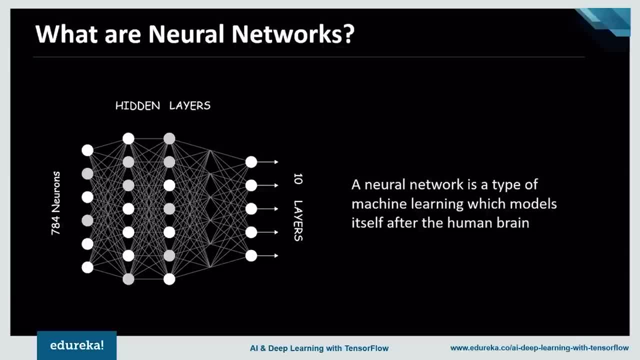 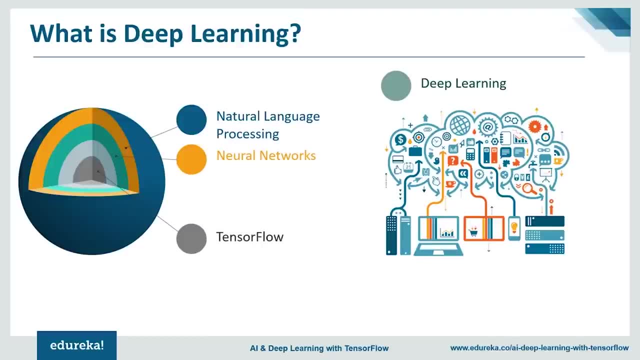 or imprecise data and can be used to extract patterns and detect trends that are too complex to be noticed by either humans or other computer techniques. Now the next layer is deep learning. It is a subset of machine learning and artificial intelligence that has networks capable of learning. 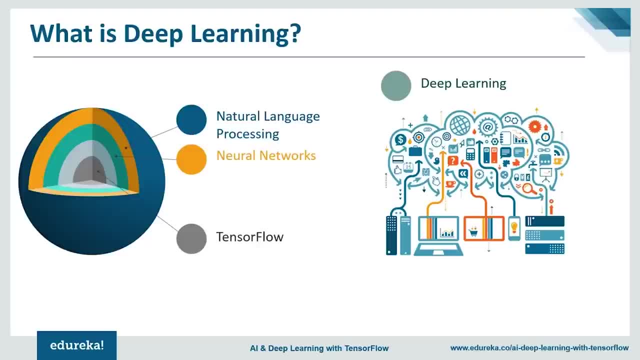 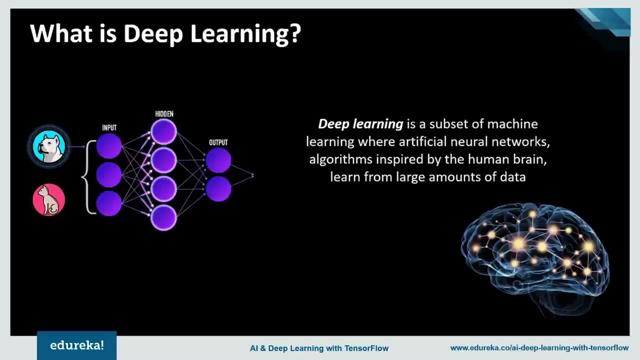 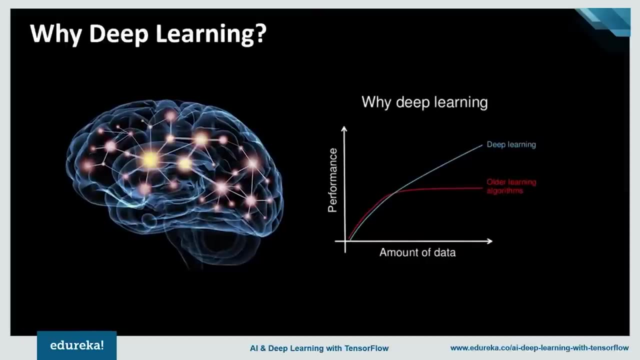 Unsupervised form of data that is unstructured or unlabeled. It is a subfield of machine learning concerned with algorithms inspired by the structure and function of the brain, called the artificial neural networks. now, in traditional machine learning techniques, Most of the applied features need to be identified by a domain. 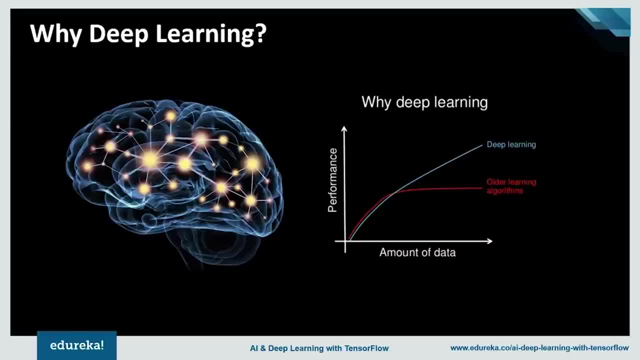 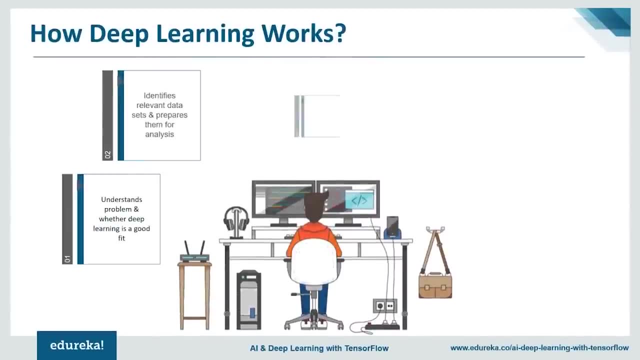 expert in order to reduce the complexity of the data and make patterns more visible to learning algorithms to work. the biggest advantage of deep learning algorithms is that they try to learn high-level features from data in an incremental manner. Now, this eliminates the need of domain expertise and hardcore. 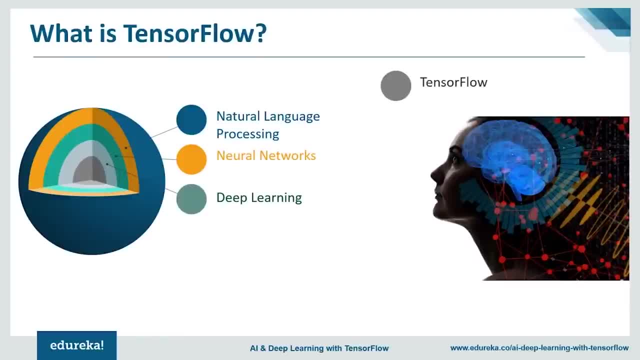 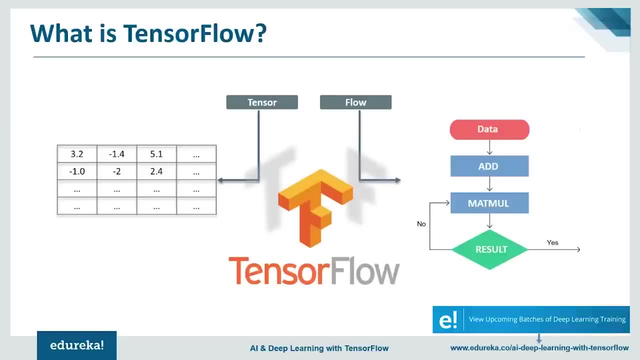 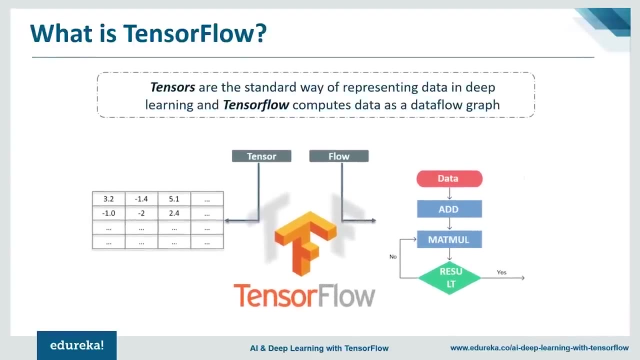 feature extraction. Now, another important layer is tensorflow. machine learning is a complex discipline, but implementing machine learning models is far less daunting and difficult than it used to be, thanks to machine learning frameworks such as Google's tensorflow. that is the process of acquiring data, training models serving 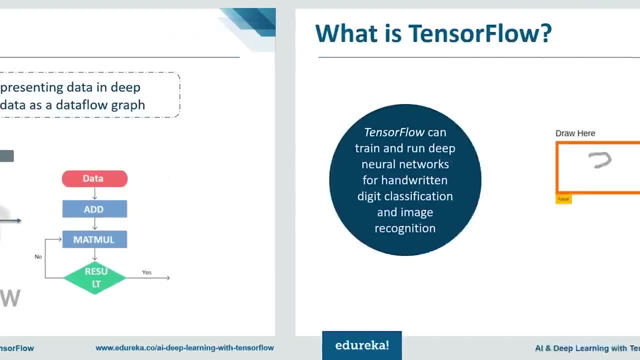 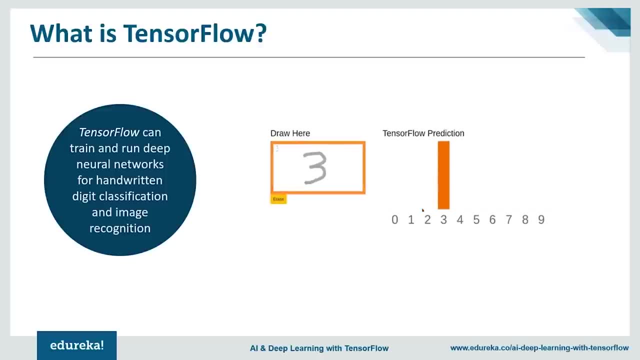 predictions and refining future Results. it is an open-source library for numerical computation and large-scale machine learning. tensorflow bundles together a slew of machine learning and deep learning models and algorithms. that makes them useful by way of a common metaphor. So now let's see how all these layers combined together and set. 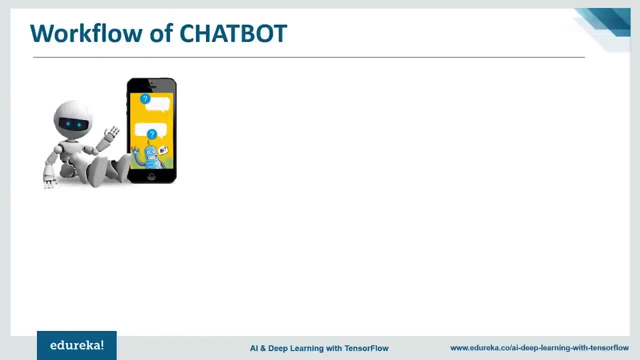 the workflow of chatbots. The first step is to determine the role of your bot and set goals, be specific about what you want your bot to do, and then evaluate And pick a channel. the next step is to create the conversational architecture. It basically organizes the content and finds the best way. 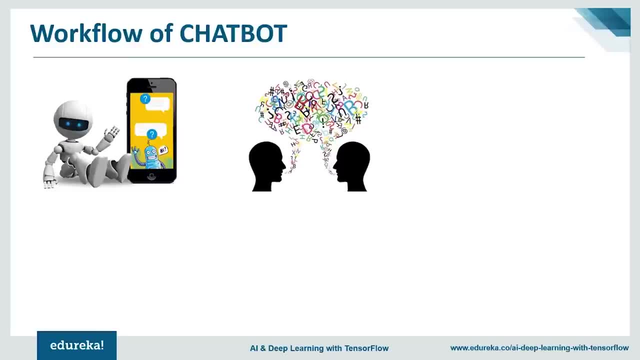 toward the bots answers. The dialogue flow goes into the detail. to implement the bot Now, one of the most important resources you will need to assemble is a collection of question variations reflecting the different ways your customer can ask for something. Now the next step is to pick a platform and a development approach. 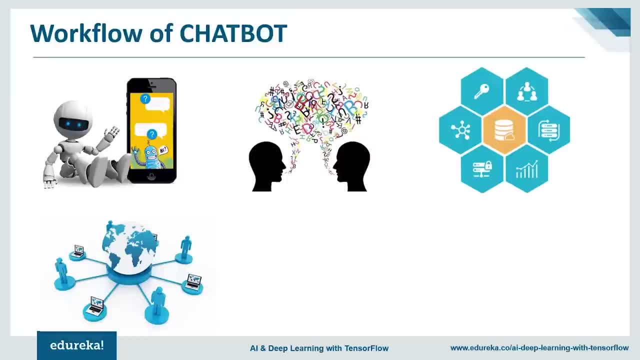 the chatbot. It needs to determine the intent of the sentence and extract data from the sentence. Next is the implementation of the dialogue flow and to engineer the natural language understanding. If you have a platform based on machine learning, you will provide it with example sentences for each possible intent. 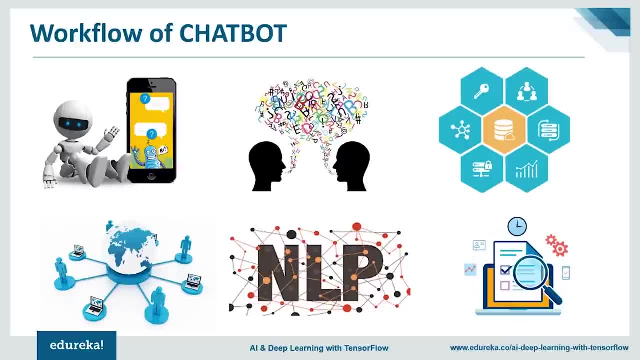 So now, in the final step, you have to perform internal testing and revise your use case detection now to ensure a successful outcome of your chatbot deployment. view the creation as a iterative process now, because of the nature of human language and the infinite possible expressions of every question or 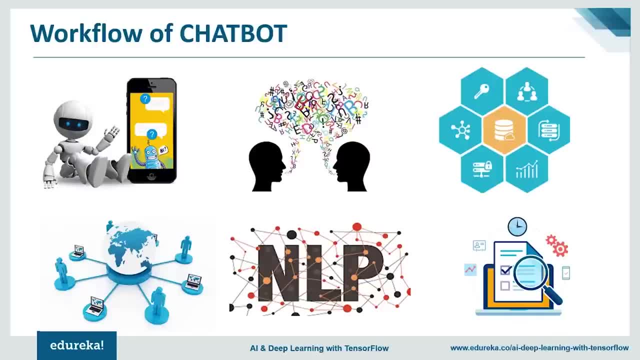 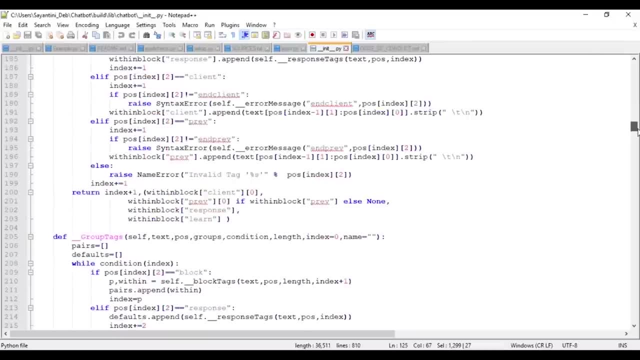 intent. the goal of hundred percent accuracy is an unattainable one, even for a human being. So let's have a look at the code that will make our chat bot talk to us. So here we have a set of reflections that trains the chat. 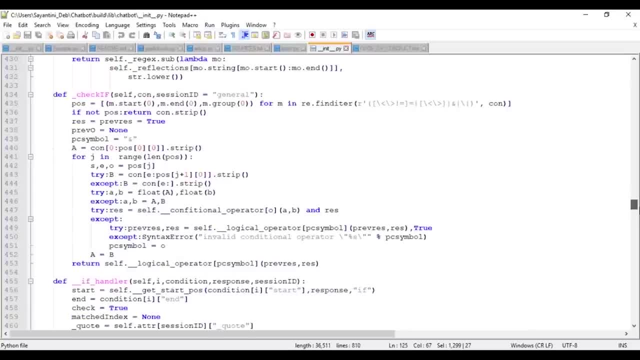 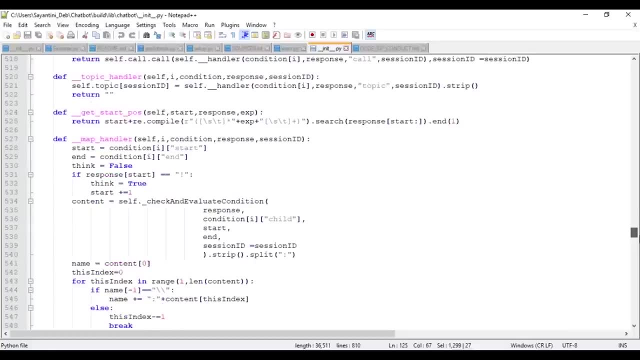 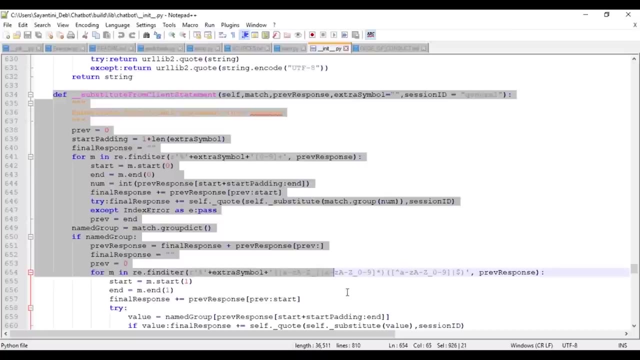 bot to reply in a particular manner. now, in the multifunction called class, We generate the session ID for any string in order to join or split the sentences, which is then matched with the trained data set for similar answers. So once we are done normalizing now, we will substitute words. 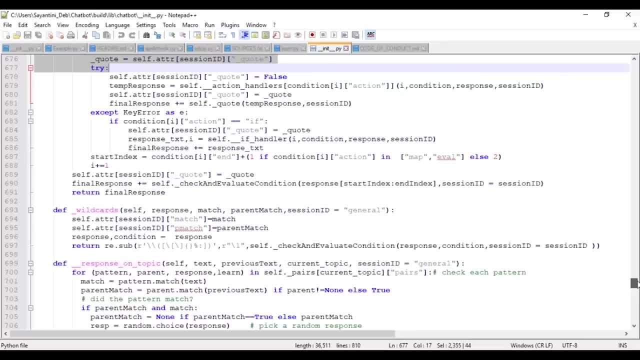 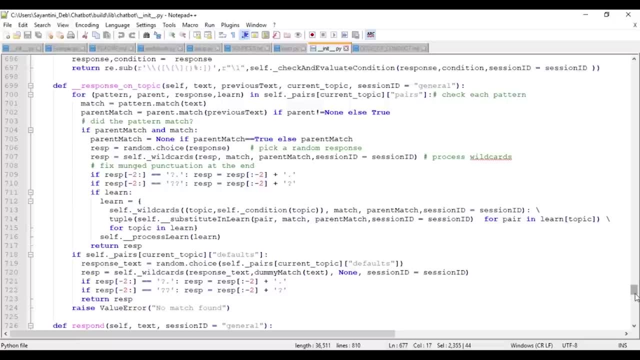 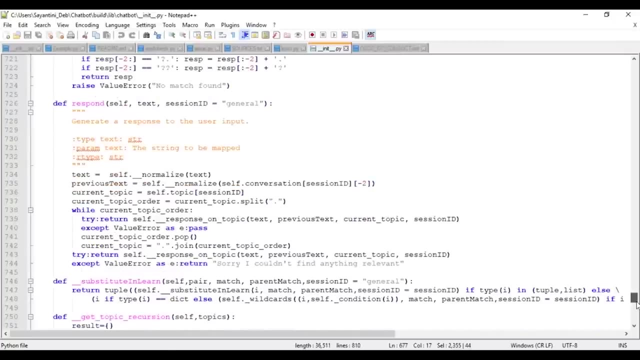 in the string according to the specified reflections. now, after this, the client statements will be substituted into responses so that the chat bot can answer according to a particular query. once we are done with this, now it's time to generate a response to the user. The user would be expecting an accurate answer from the chat. 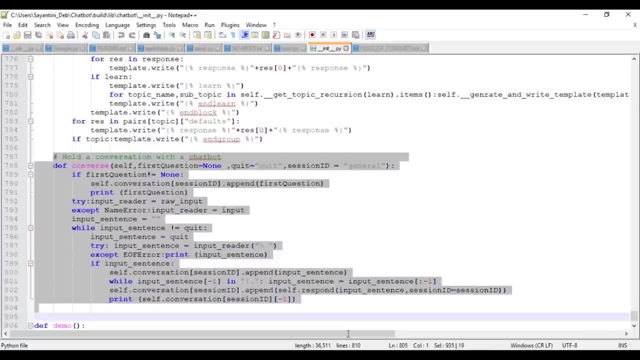 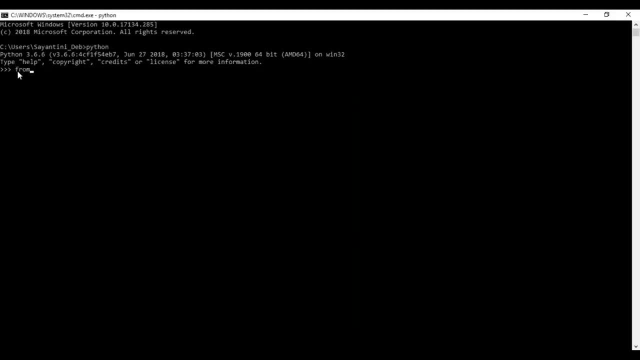 bot. Now, once the mapping of the words and the strings are done, the chat bot is ready to hold a conversation with a human being and reply to all the queries. So now let's see how the demo of our chat bot works. So let me start by responding to its question and then see how. 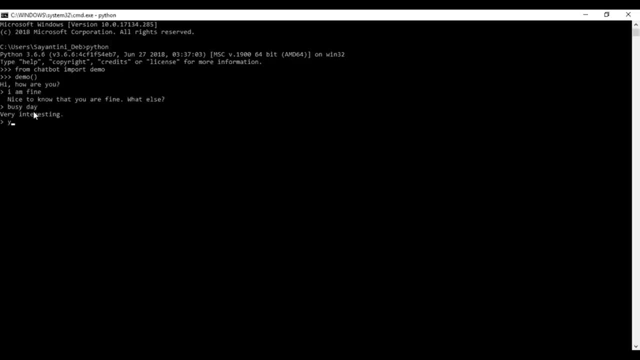 it responds to my queries. So we can see that the chat bot will not provide a hundred percent accurate response Or exactly the way we wanted to reply, but it must understand the question and provide a satisfying response. Now we can see that our chat bot is up and running and it is. 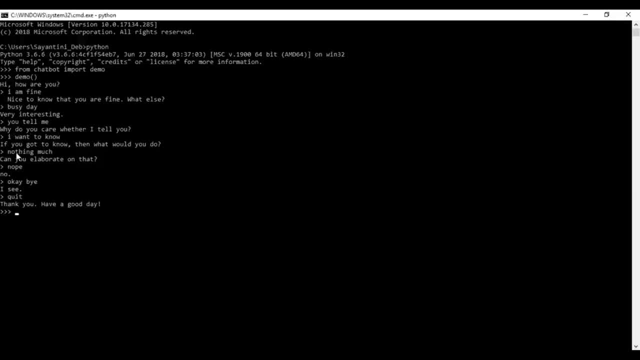 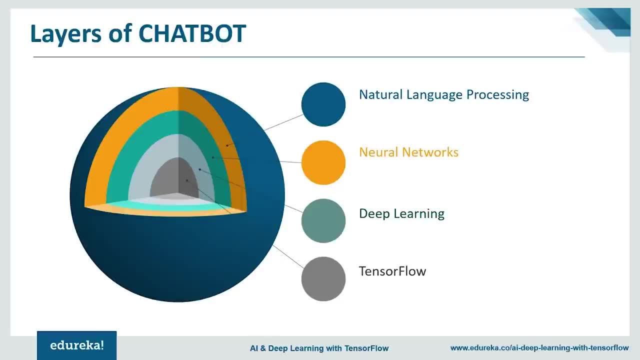 able to hold a conversation with us with the help of all the layers involved in the working of our chat bot, such as NLP, neural networks, deep learning and tensorflow. So I hope you all understood how all these layers work together in machine learning and helps in building a robot that can. 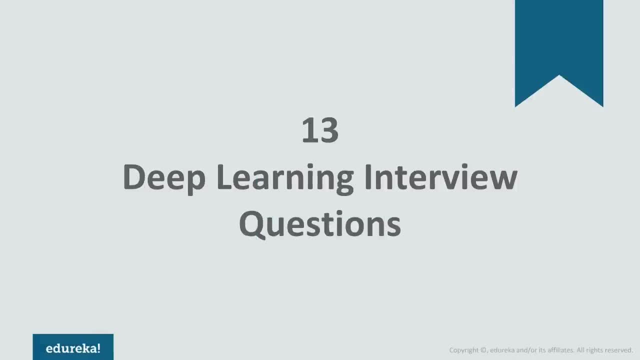 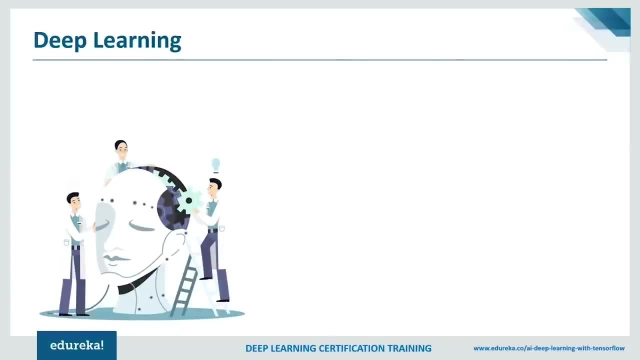 almost talk like a human being. Now. deep learning is a hot buzzword nowadays and has firmly put down its root in a vast multitude of Industries that are investing in fields like artificial intelligence, big data and analytics. For example, Google is using deep learning in its voice and 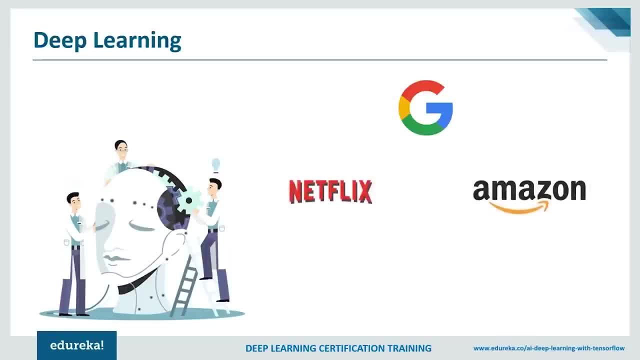 image recognition algorithms, whereas Netflix and Amazon are using it to understand the behavior of their customers. even Tesla is using deep learning in their self-driving cars. Now imagine how much potential deep learning has in revolutionizing the world and the way we work around things. Now this growth of deep learning and its application has led to 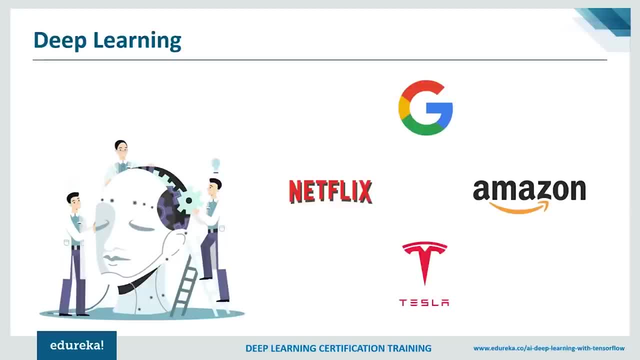 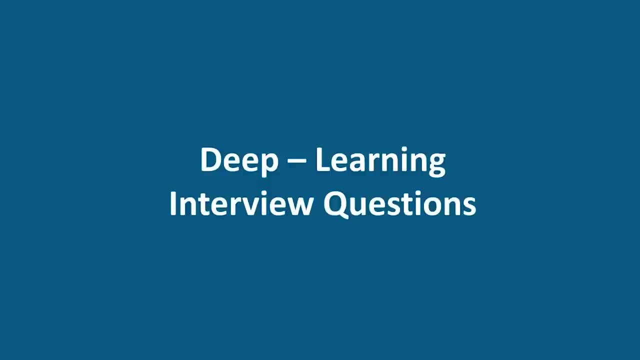 the growth of deep learning jobs even, for example, we have the data scientists, We have machine learning engineer, We have artificial intelligence engineer and much more rules. So let's begin our deep learning interview question and answer session and understand what are the typical questions, which are: 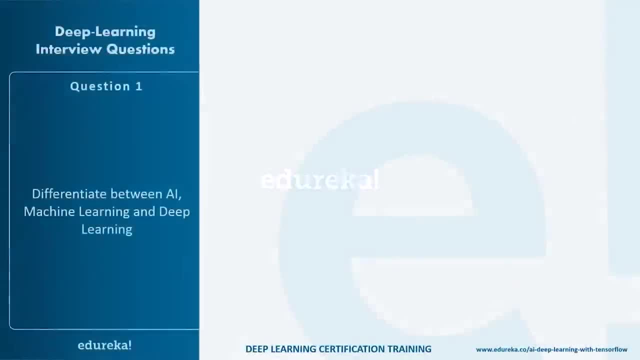 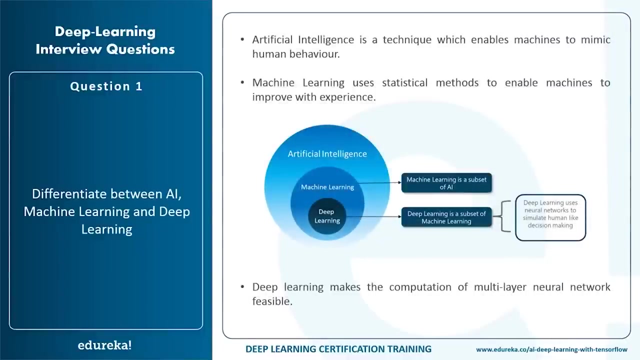 being asked in deep learning interview. So the first and foremost question, what any deep learning interviewer ask is the basic understanding of the relationship between machine learning, artificial intelligence and deep learning. So basically, artificial intelligence is a technique which enables machine to mimic human behavior and machine learning. 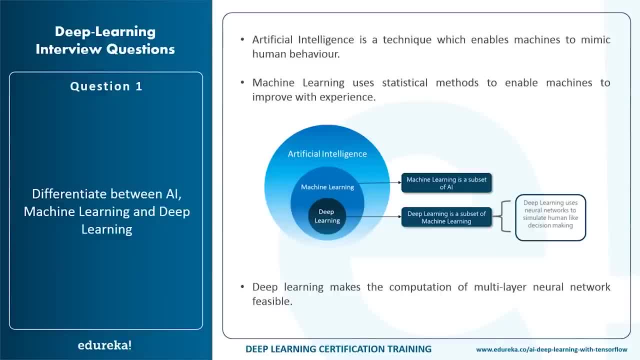 is a subset of artificial intelligence technique which uses statistical methods to enable machines to improve with experience. not deep learning, On the other hand, Is a subset of machine learning which makes the computation of multi-layer neural network feasible. It uses neural networks to simulate human-like decision-making. 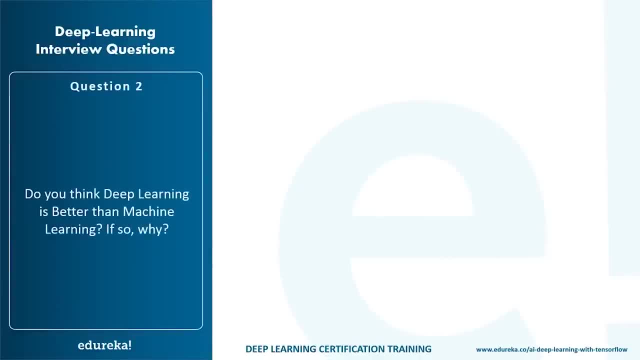 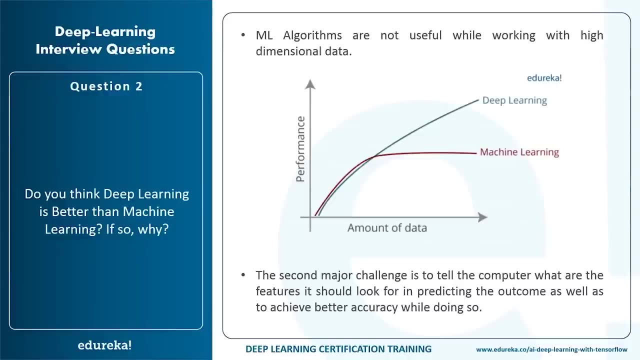 not coming to the second question, Do you think deep learning is better than machine learning? And if so, why not though machine learning algorithms? the traditional machine learning algorithms solve a lot of our cases, but they are not very useful while working with high dimensional 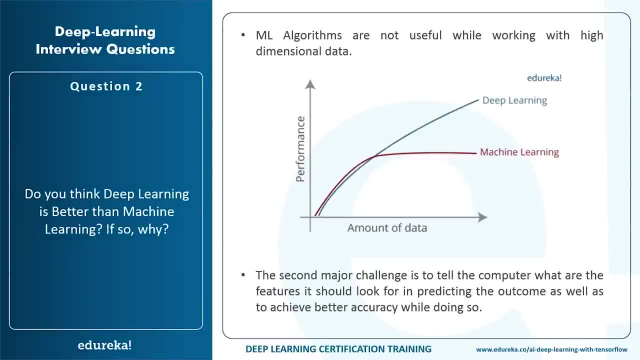 data. Now that is where we have a large number of inputs and outputs. For example, in case of handwriting recognition, We have large amount of inputs where we have different types of input associated with different types of handwriting. Now another major challenge is to tell the computer what all. 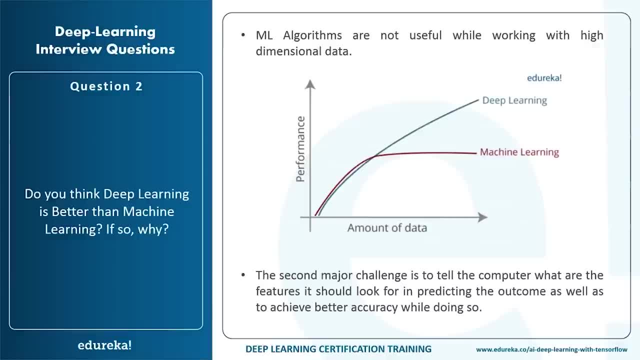 features it should look for that will play an important role in predicting the outcome, as well as to achieve better accuracy while doing so. So these are some of the few shortcomings what machine learning have, and deep learning overcomes all of these shortcomings. Now, coming to our third question, which is what? 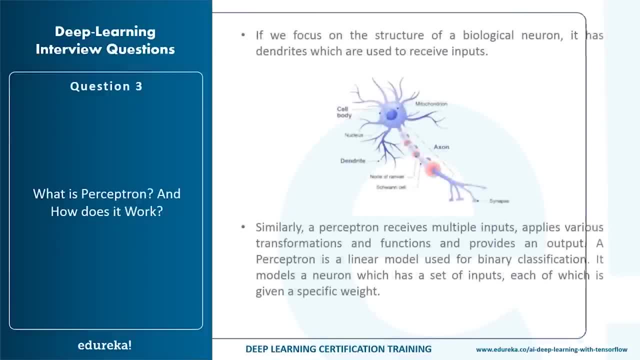 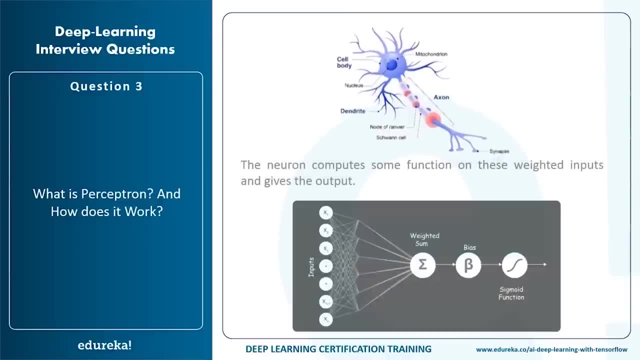 What is a perceptron and how does it work Now, actually, our brain has subconsciously trained itself to do a lot of things over the years. Now the question comes: how does deep learning mimics the functionality of the brain? Well, deep learning uses the concept of artificial neuron. that 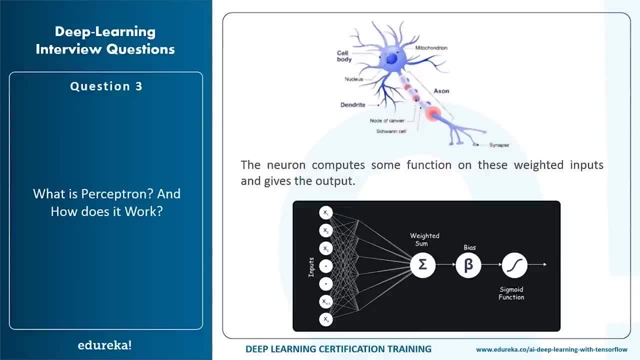 functions in a similar manner as the biological neuron present in our brain. Therefore, we can say that deep learning is a subfield of machine learning concerned with algorithms inspired by the structure and the function of the brain, called artificial neural networks. Now, if you focus on the structure of a biological neuron, it has 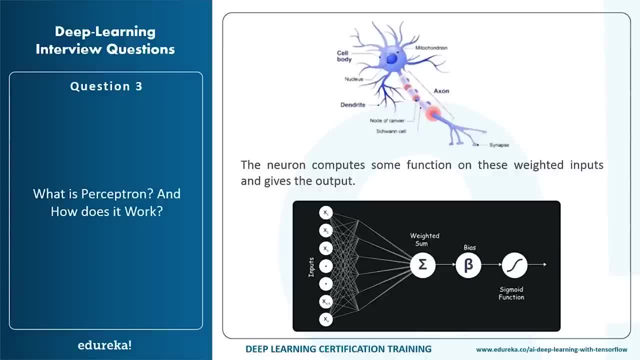 dendrites, which is used to receive inputs, But these inputs are summed in the cell body and, using the axon, it is passed on to the next biological neuron. But similarly, a perceptron receives multiple inputs, applies various transformations and functions and provides an output. 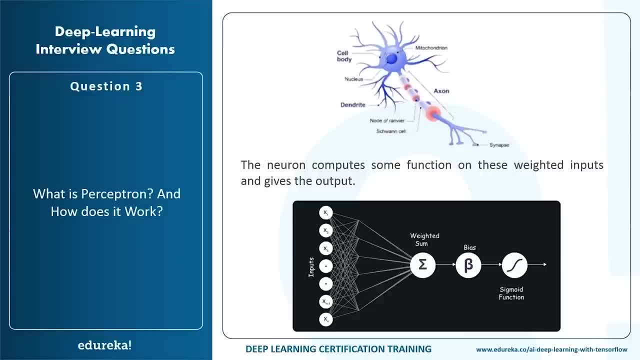 Now, a perceptron is a linear model used for binary classification. It models a neuron which has a set of inputs, each of which gives a specific weight. Now the neuron computes some function on these weighted inputs and then, finally, it provides the output, As we know that our brain consists of multiple connected neurons. 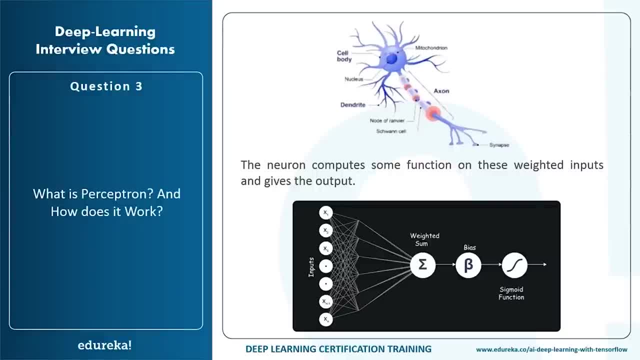 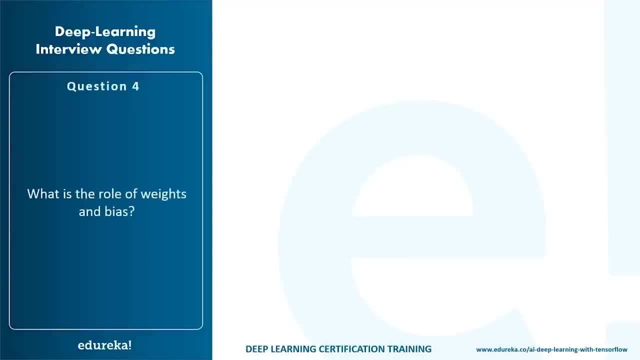 called the neural network. We can also have a network of artificial neurons called the perceptron to form a deep neural network. Now, coming to the next question: What is the role of weights and biases? Now for a perceptron, they can have one or more input called bias. 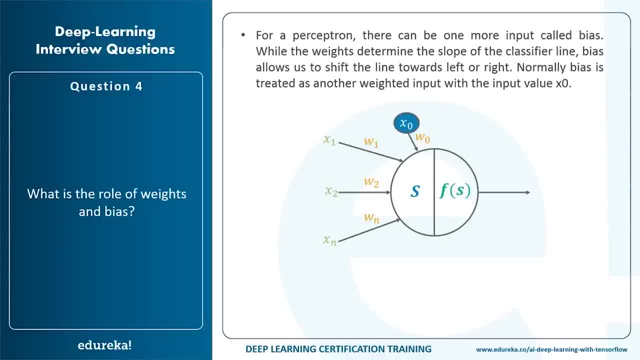 while the weights determine the slope Of the classifier line, the bias allows us to shift the line towards left or right. Normally, bias is treated as another weighted input, with the input value X in our case. If you have a look at a typical perceptron, what it receives is a. 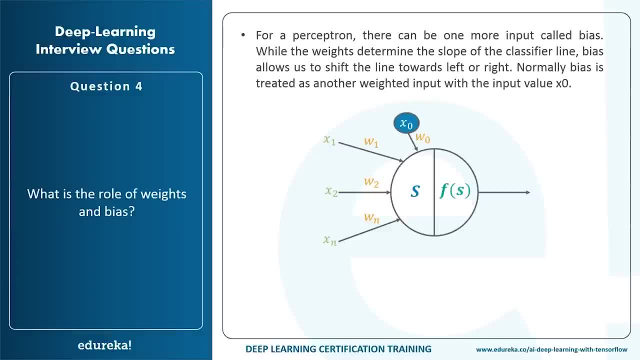 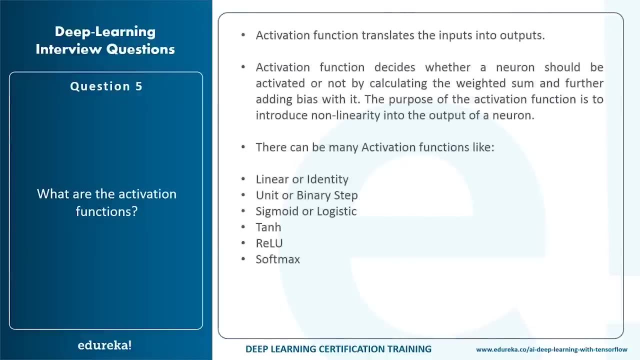 set of input. but these inputs are not just input which it gathers. So weights are an additional input which it takes and according to that it computes and provides an output. Now, which brings us to the next question, which is: what exactly are activation functions? So activation function translates the inputs into outputs and it uses 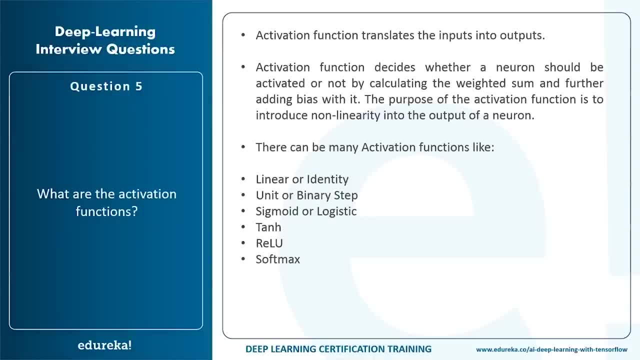 a threshold to produce an output. So the activation function decides whether a neuron should be activated or not by calculating the weighted sum and further adding the bias with it, and the purpose of the activation function is to introduce a non-linearity into the output of a neuron. 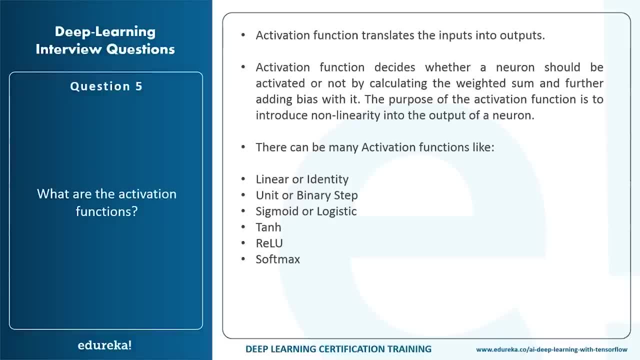 There can be many activation functions like linear or identity. We have the binary step, We have sigmoid, We have the tanh, We have relu and softmax. These are a lot of activation functions which are being heavily used in the deep learning industry. 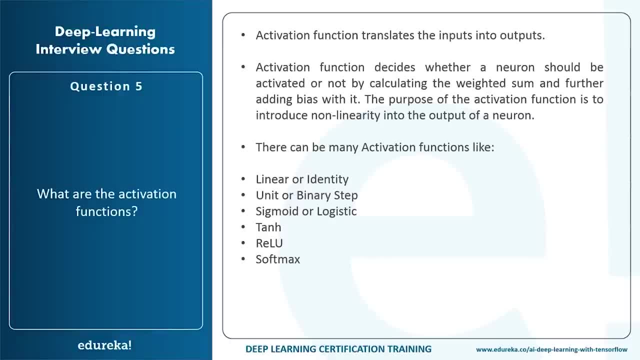 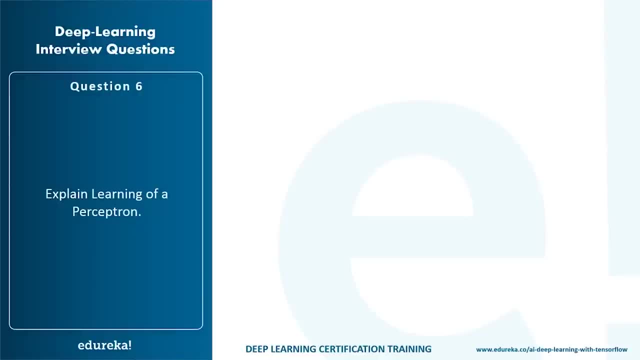 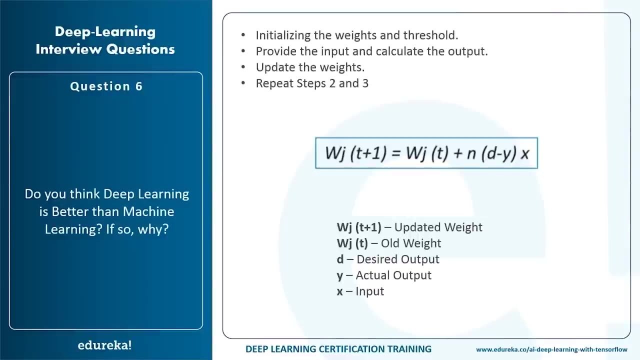 So one should actually know about all of these things. Now, talking about perceptron, our next question, what an interviewer might ask, is explain the learning of a perceptron. So basically, a perceptron has four steps of learning. So the first steps is initializing the weights and threshold. so just 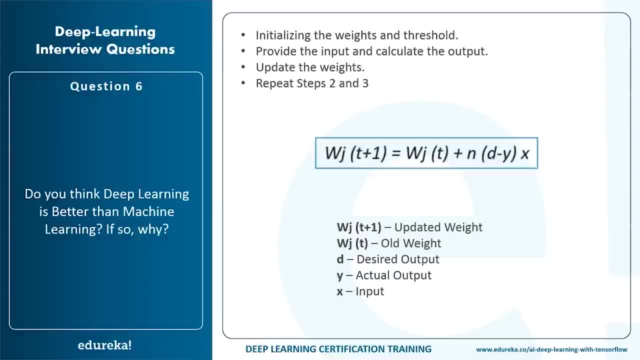 now, as I mentioned, Initializing the weights and threshold, so to the perceptron, so that it can activate a neuron by calculating the weighted sum and further adding the bias in. and all this is the first step and the second step is providing the input and calculating the output using the 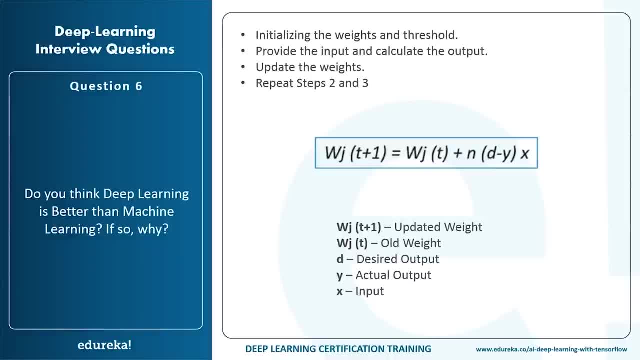 activation functions. And according to that, what we do is the third step, inverse updating the weights. Now, once a particular perceptron learns something, it has to update the weights so that it could learn Much more things in a new manner. and the next step: 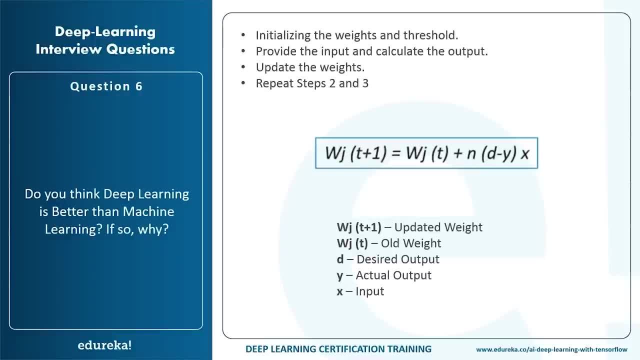 What comes is just repeat the step number two and three, which is provide the input and calculate the output, and then update the weights accordingly. If we have a look at the equation here, we have wjt plus one. that equals wj of t plus n of t minus y x. the wj of t plus one is the. 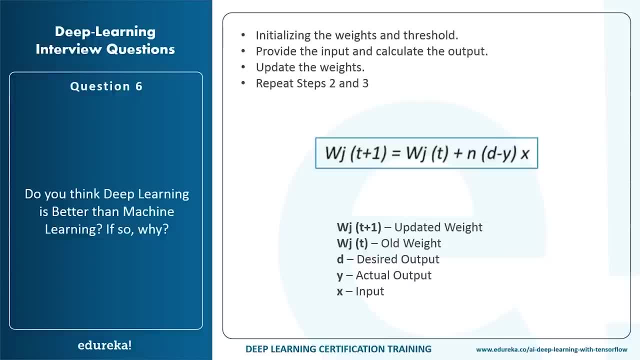 updated weight, whereas wj of t is the old weight, d is the desired output, y is the actual output and x is the input. So this is the equation of the learning of a perceptron. Now the next question is: what is the significance of a cost or a? 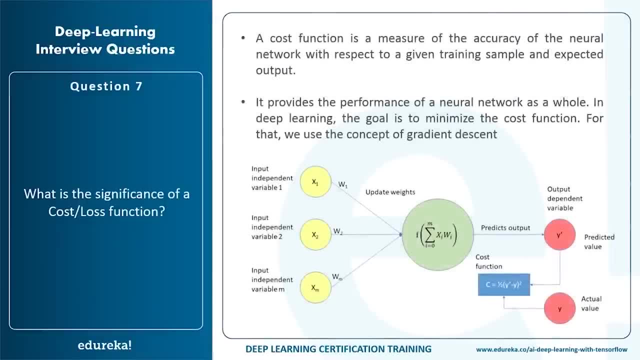 loss function. So a cost function is a measure of accuracy of the neural network with respect to a given training sample and expected output. it provides the performance of a neural network as a whole. and in deep learning the goal is to minimize the cost function, So for that we use the concept of radian descent now, which brings 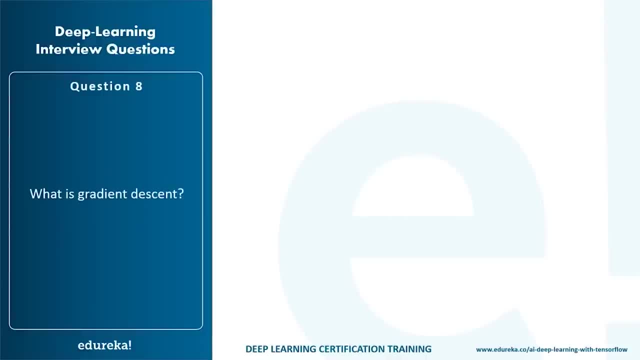 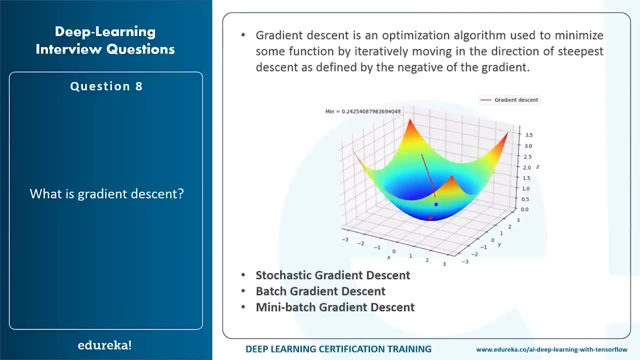 us to the next question, Which is: what exactly is gradient descent and what are its various types? So gradient descent is an optimization algorithm which is used to minimize some function by iteratively moving in the direction of the steepest descent, as defined by the negative of the gradient. 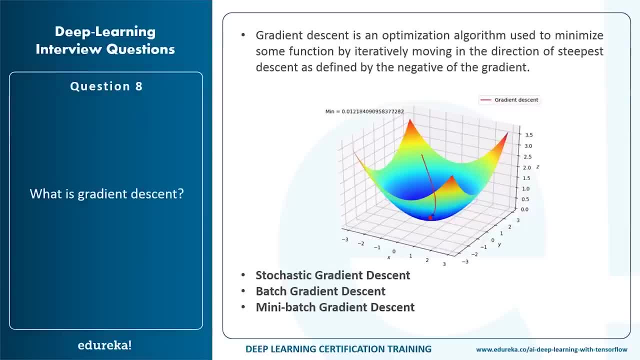 Now think of it as a bowl in which you start from any particular point and the goal is to reach the bottom of the bowl, which is the gradient descent. So there are three types of gradient descents, which are the stochastic batch And the mini batch. so stochastic gradient descent it uses only. 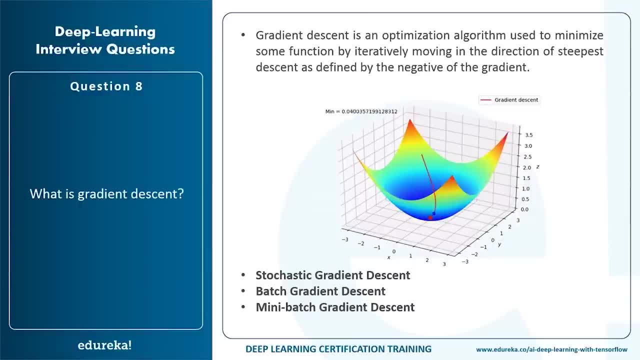 single training example to calculate the gradient and update the parameters accordingly, whereas the batch gradient descent calculates the gradients for the whole data set and performs just one update at each iteration. Now, mini batch gradient descent is a variation of the stochastic gradient descent where, instead of single training example, mini batch. 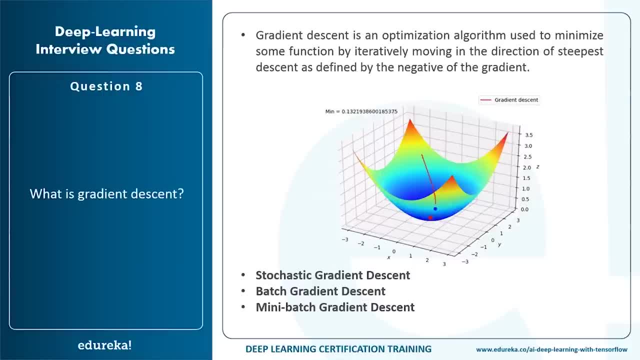 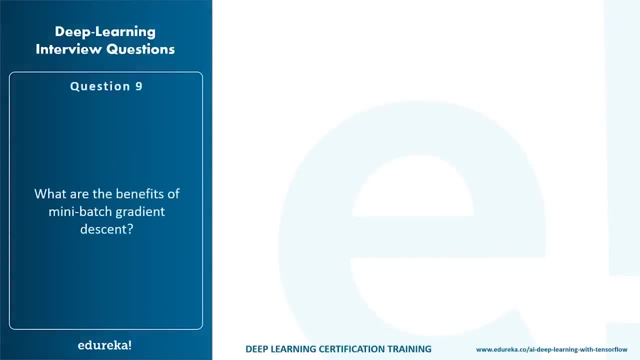 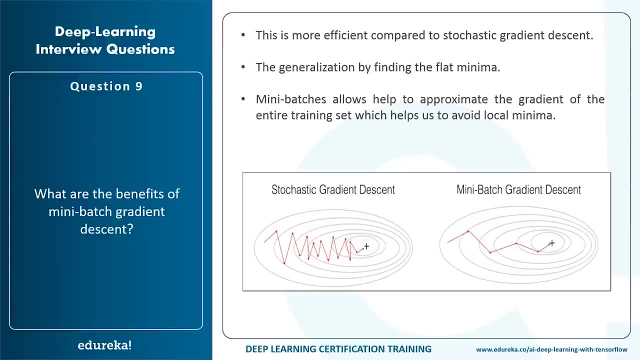 of samples are used and it is one of the most popular optimization algorithm. Now, if we talk about mini batch gradient descent, what might ask is: what are the benefits of the mini batch gradient descent, or how is it useful than the others? Now, the mini batch gradient descent is more efficient when compared. 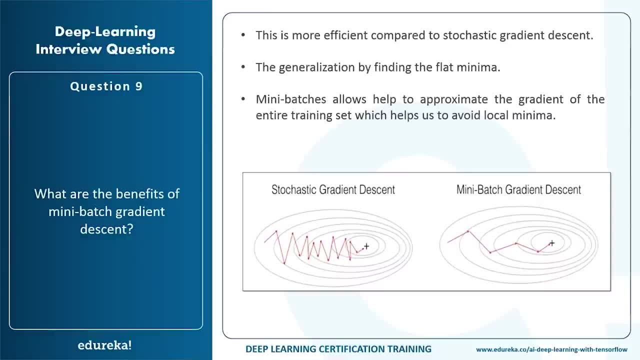 to the stochastic gradient descent and the generalization is done by finding the flat minima, which allows to help approximate the gradient of the entire training set, which help us to avoid the local minima. Now, this is why the mini batch gradient descent is considered. 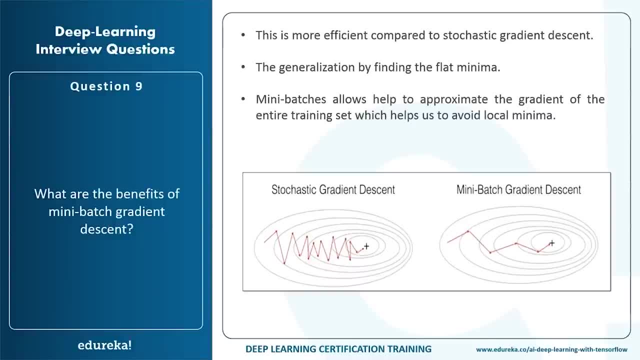 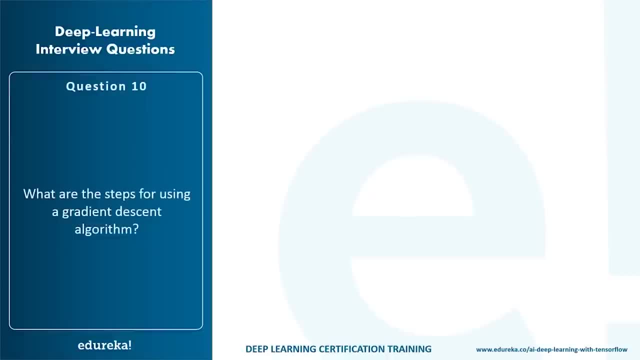 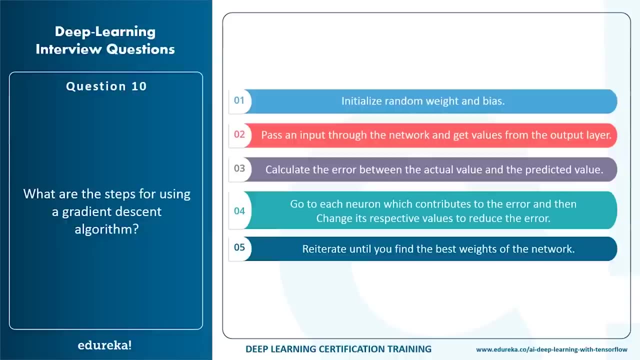 or is preferred over the regular gradient descent algorithm, which is the stochastic gradient descent. Now one might ask: what are the steps for using a gradient descent algorithms? So, first of all, what you need to do is initialize some random weight and bias, and after that you need to do is pass an input. 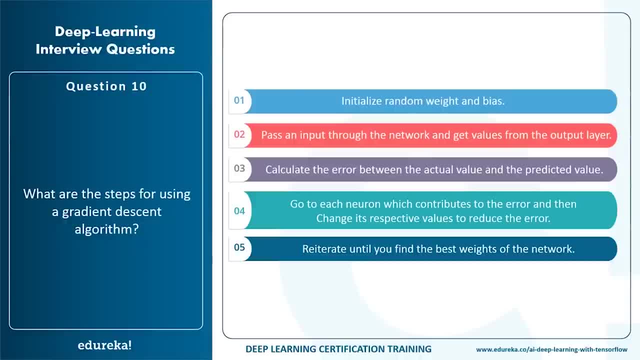 through the network and get values from the output layer. Next, what you're going to do is calculate the error between the actual value and the predicted value, but this can be done in a number of ways. Now the next step involves is to go to each neurons which contributes to the error and change. 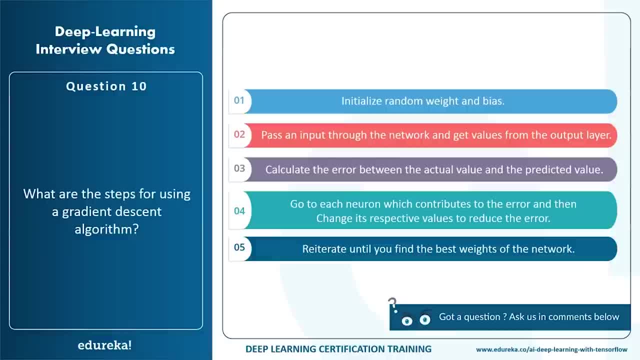 its respective values to reduce the error, which is basically our goal, is to reduce the cost of any particular function or any particular model. So after that, what you do is reiterate until you find the best weights of the network and you find the lowest cost of the particular 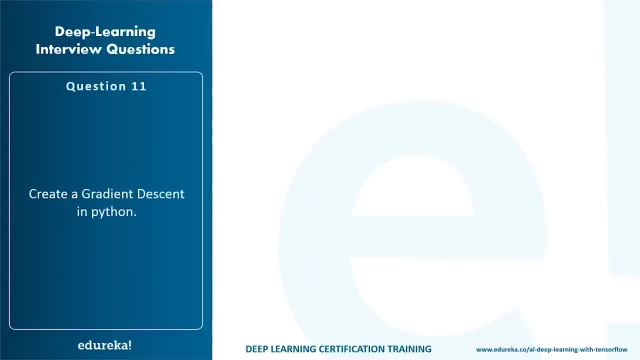 network. So one might ask you to write any gradient descent program or write the pseudo code of a gradient descent program. So what you need to do First of all, what we do, is define the parameters, which are the weights, the hidden weights, the weight output, the bias hidden. 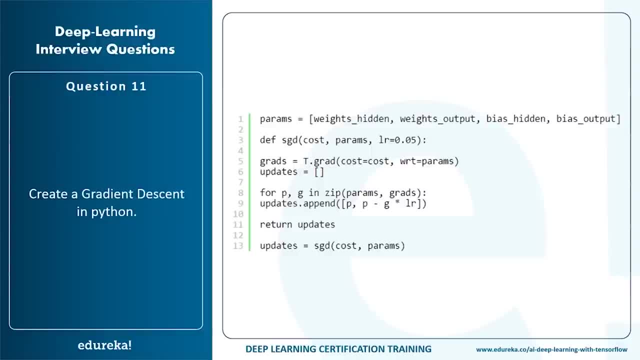 and the bias output. We define a function, STD, with arguments as cost, the parameters- what we have discussed- and the learning rate. Now, what we do is then we then define the gradients of our parameters with respect to the cost function. So here we use the Theano library. 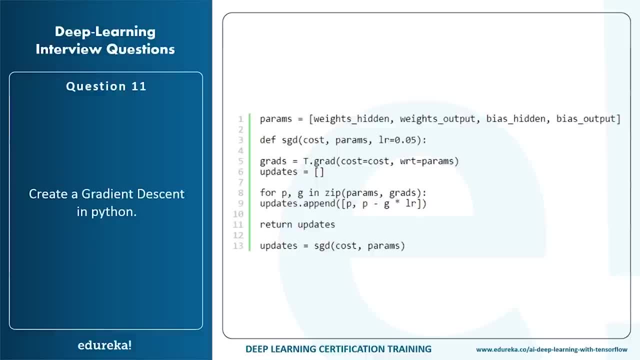 To find the gradients and we import Theano, STD and finally iterated through all the parameters to find out the updates for all the possible parameters. So you can see that we use vanilla gradient descent here and, as you can see, it returns the updates and what we do is update the parameters. 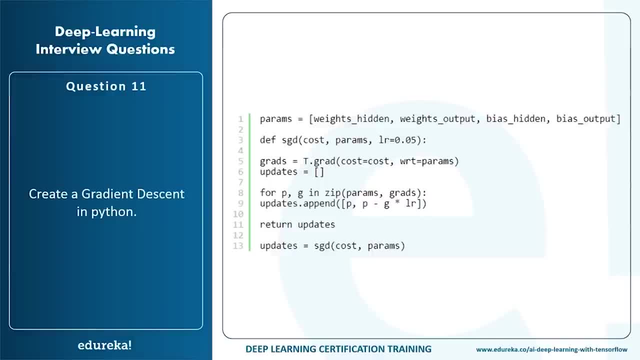 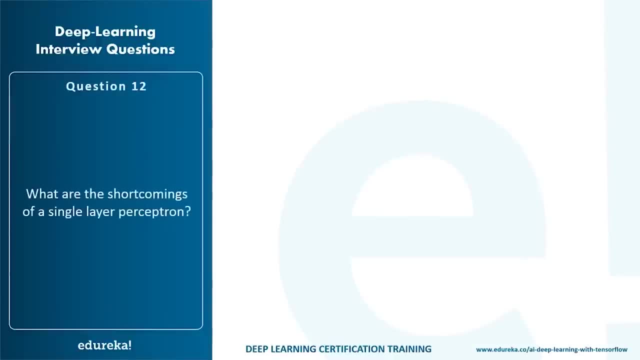 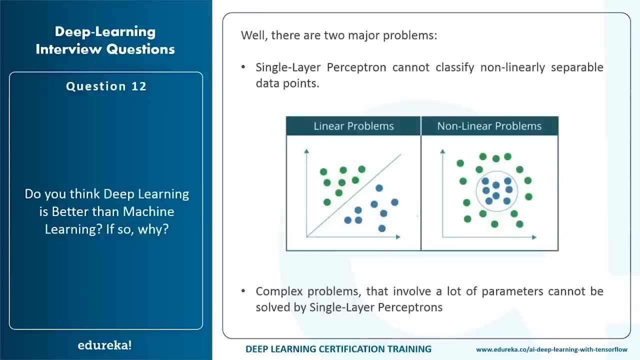 and the cost in this particular equation. The ultimate goal of any gradient descent algorithm is to minimize the cost. Now, talking about perceptron, What are the shortcomings of a single layer perceptron? So well, there are two major problems Now. first of all is that the single layer perceptron cannot classify 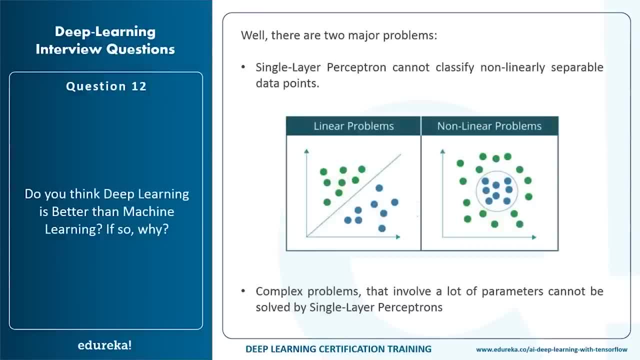 non-linear, separable data points. And the second point is that the complex problems that involve a lot of parameters cannot be solved by a single layer perceptron. Now consider an example here and the complexity which arises when the parameters are involved to take a decision by a marketing team. 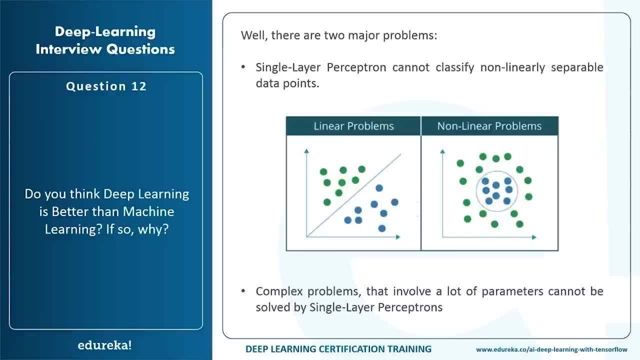 So first of all we have the categories, which are the email direct paid reflare program or the organic, and inside this category We have subcategories which are the Google, Facebook, LinkedIn, Twitter. We have Instagram now, and inside that we have the type of subcategory. 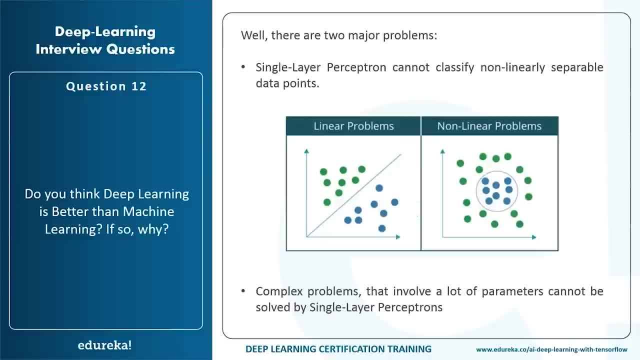 which are the search as remarketing ads, interested as look-alike ads. And again, if we do a subdivision, we have the parameters to consider, which are the customer acquisition cost. We have the money spent, the click Rate or the lead generated, the customer generated and the time. 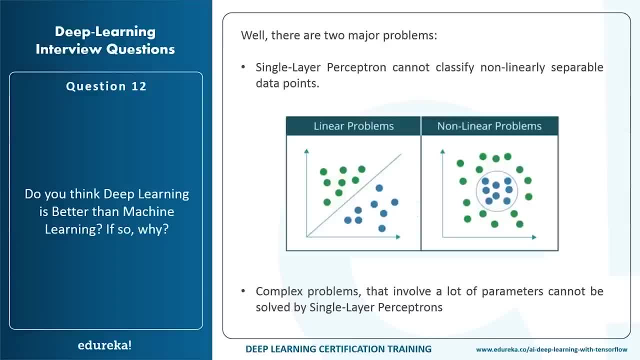 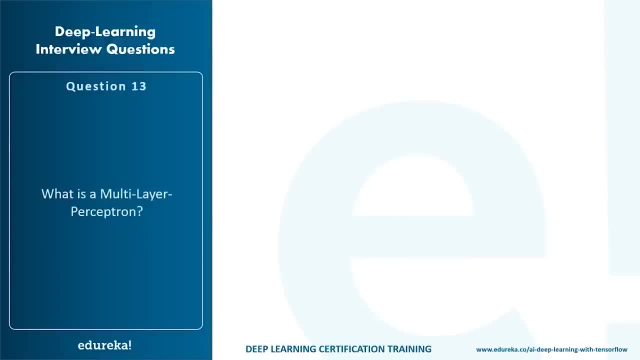 taken to become a customer. So one neuron cannot take in so many inputs, and that is why more than one neuron would be used to solve this problem. Now, which brings us to the question: What is a multi-layer perceptron? So a multi-layer perceptron, or MLP, is a class of feed forward, artificial. 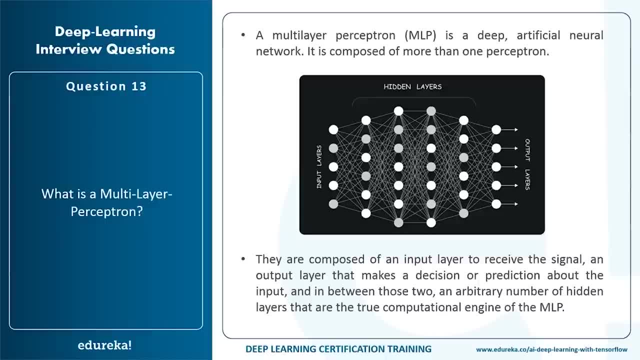 neural network and it is composed of more than one perceptron. They are composed of an input layer to receive the signal, and output layer that makes a decision Or the prediction about the input and in between these two and arbitrary number of hidden layers that are the true computational engine of any. 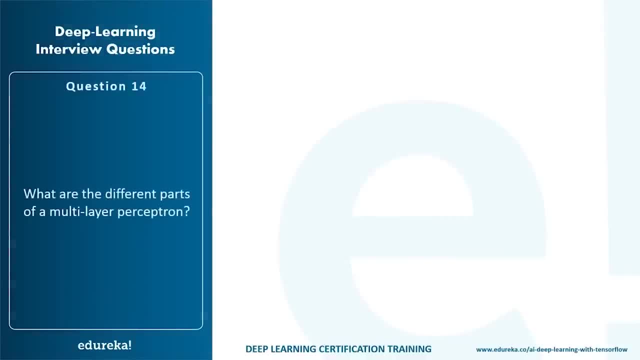 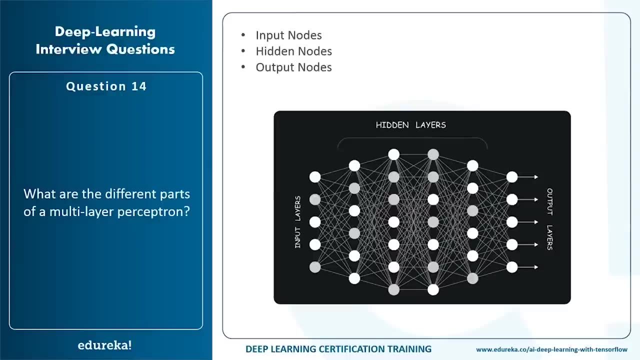 multi-layer perceptron. Now one might ask: what are the different parts of any multi-layer perceptron or a neural network? So, first of all, what we have, our input notes. So the input notes provide information from the outside world to the network and are together referred as the input layer. 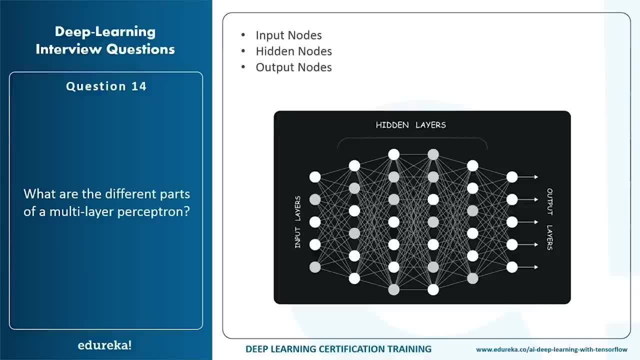 No computation is performed in any of the input notes. They just pass the information to the hidden layers. Now, hidden nodes have no direct connection with the outside world, Hence the name hidden. and what they do is they perform computation and transfer the information from the input nodes to the output nodes. 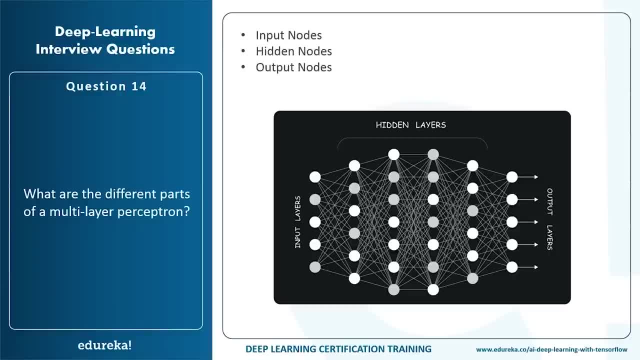 Now, a collection of hidden nodes forms the hidden layer, and while a network will only have a single input layer and a single output layer, it can have 0 to n number of hidden layers, and a multi-layer perceptron has more than one hidden layer. Now, if we talk about output nodes, the output nodes are collectively. 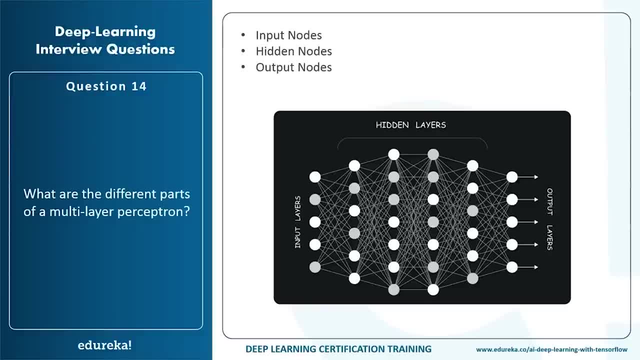 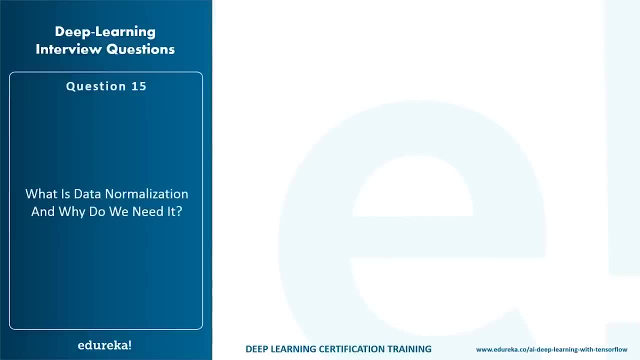 referred to as the output layer, and are responsible for the computation and transferring information from the network to the outside world and hence and hence, they are also responsible for the prediction. Now, coming to our next question: What exactly is data normalization and why do we need it? 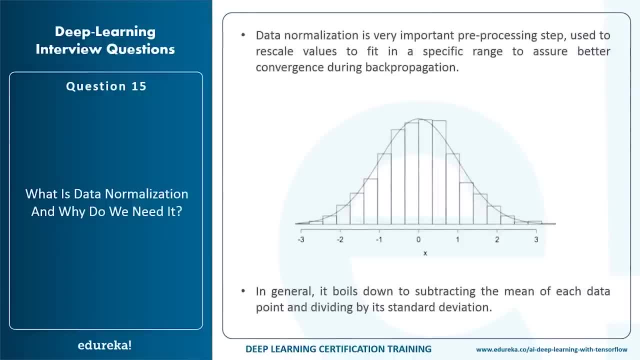 Now data normalization is a very important pre-processing step, which is to normalize the data. The data should not be either left skewed or right skewed- It should be normal and is used to rescale the values to fit in a specific range to assure the better convergence during back propagation. 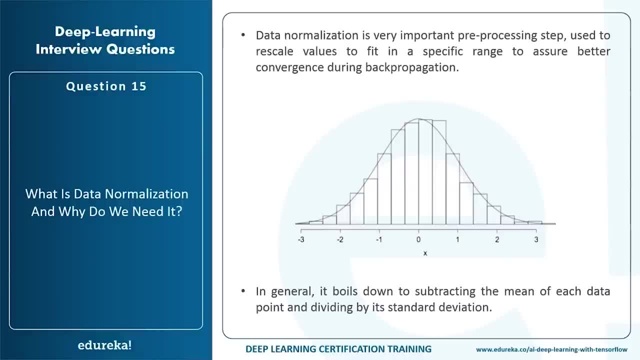 and in general it boils down to subtracting the mean of each data point and dividing by its standard deviation so that we get a normally distributed data, and it makes computation easy in terms of the back propagation in case of a neural network. So This is a very important part of any deep neural network. now talking, 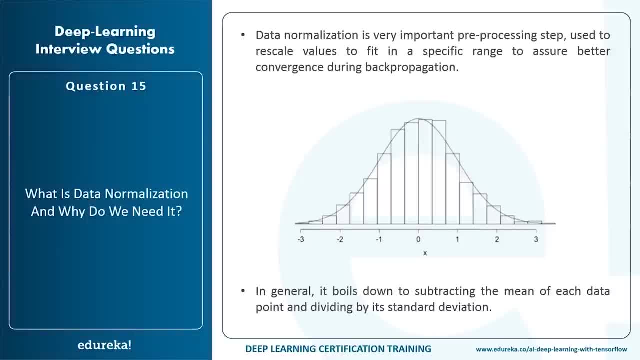 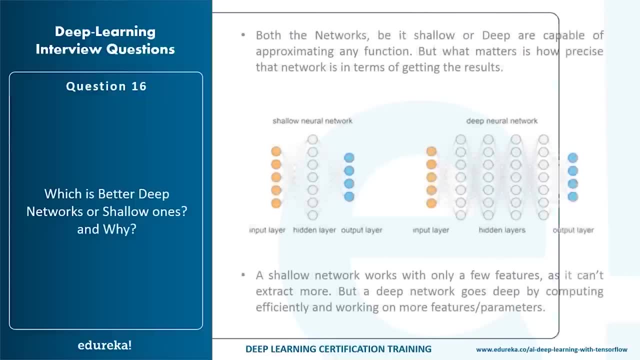 about deep neural networks, So our neural networks in general. coming to our next question, which is now: what is better, the deep networks or the shallow ones, and why? now, both the networks, be it shallow or deep, are capable of approximating any function. what matters is how precise that network is in terms of 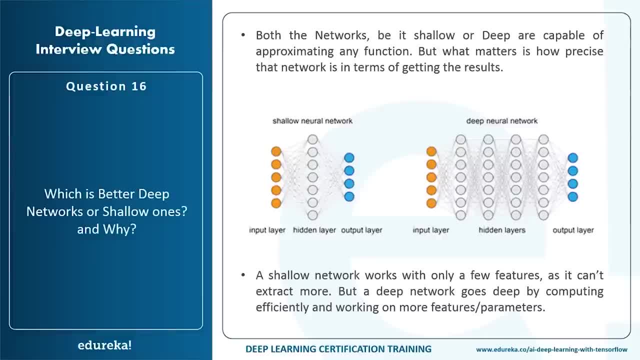 getting the result now. a shallow network works with only a few features, as it cannot extract more, but a deep network goes deep by computing efficiently and working on more features or the parameters. now deeper networks are able to create deep representation at every layer. The network learns a new, more abstract representation of the input. 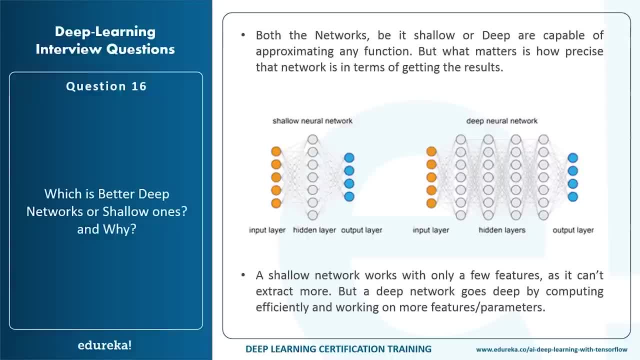 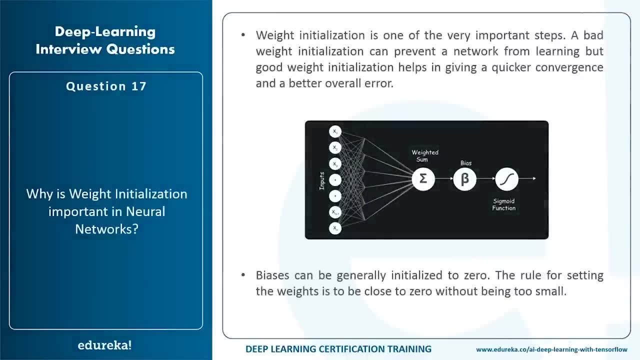 and hence deep neural networks are better than the shallow ones. So what exactly is weight initialization in a neural network? Now, as we saw, we had weight initialization in perceptron, So weight initialization is one of the very important steps. a bad weight initialization can prevent a network from learning, but good. 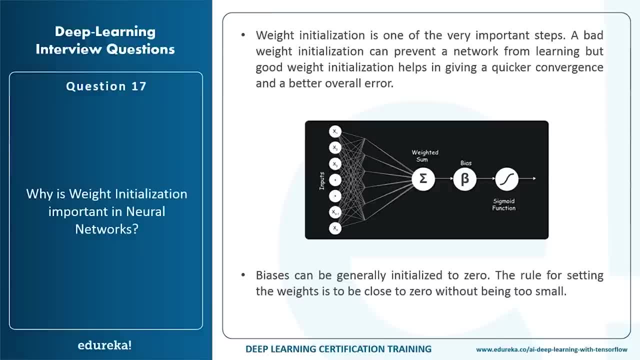 weight initialization can help it in giving quicker convergence and a better overall error. now biases can be generally initialized to 0. the rule for setting the weights is to be close to 0, without being too small, because every time the weight is being multiplied to the inputs. 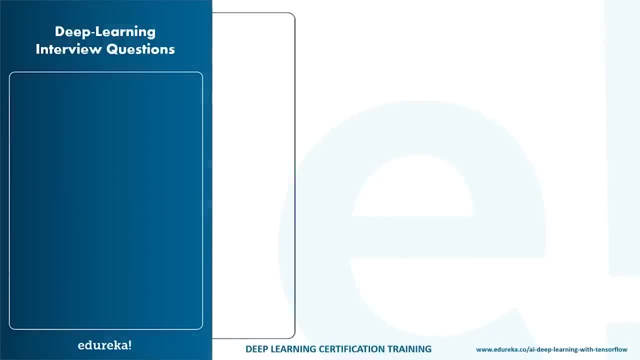 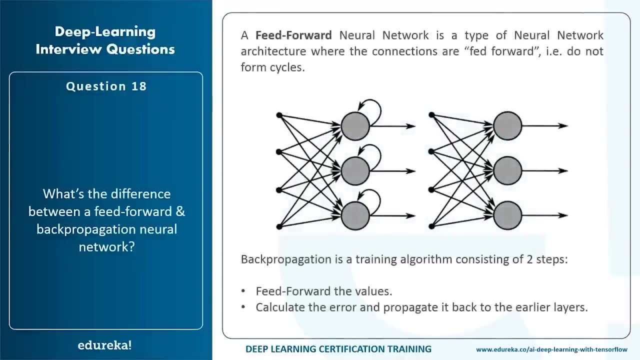 the results get smaller and smaller. but talking about neural networks, What is the difference between a feed forward and a back propagation neural network? now, a feed forward neural network is a type of neural network architecture where the connections are fed forward, that is, they do not form cycles. 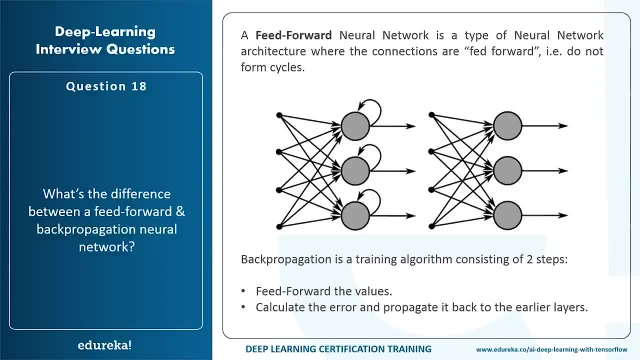 The term feed forward is also used when you input something at the input layer and it travels from the input to the hidden and from the hidden to the output layer. Values are fed forward. now, back propagation is a training algorithm which consists of two steps. majorly, 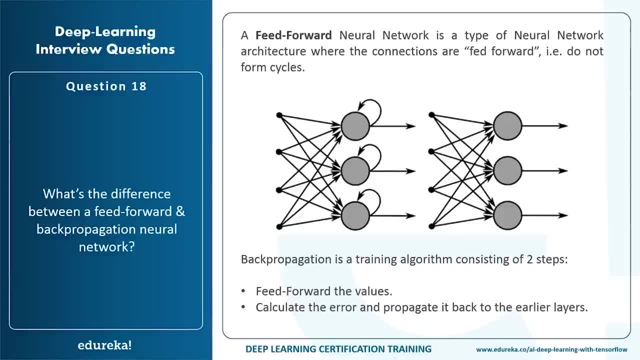 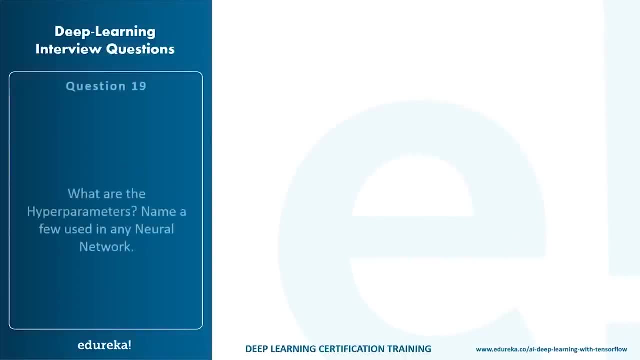 The first one is feed forwarding the values, and the second one is to calculate the error and propagate it back to the earlier layers. So, to be precise, forward propagation is a part of back propagation algorithm, but it comes before the back propagation. So one might ask the question, which is one of the most important questions. 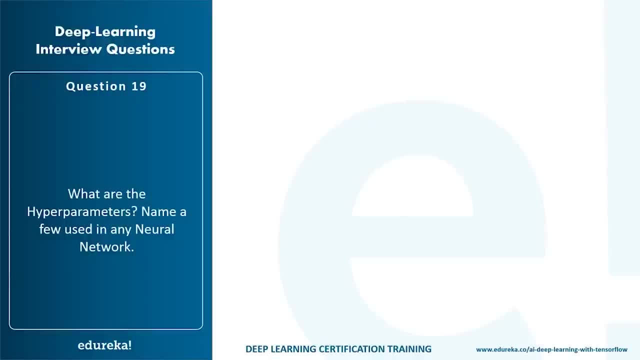 is that? what are the hyperbolic, What are the hyper parameters in the neural networks, and name a few of these hyper parameters. So hyper parameters are the variables which determine the network structure, that is, for example, the number of hidden units and all the hidden layers. 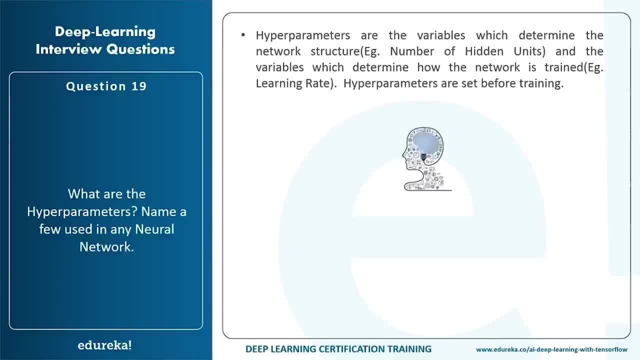 and the variables, which is to mind how the network is trained, For example the learning rate. but there are two types of hyper parameters. usually one are the network parameters which are associated to the network, and that case We have The number of layers. 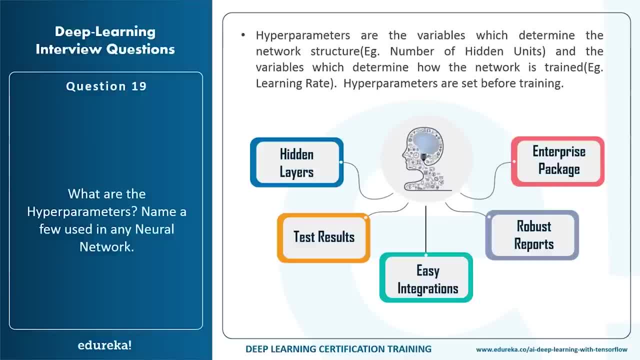 We have the network weight initialization, We have the activation function and in the training parameters, We have the learning rate, We have momentum number of epochs, We have the bath size and much more. now a lot of hyper parameters also differ when we work along with different types of neural networks. 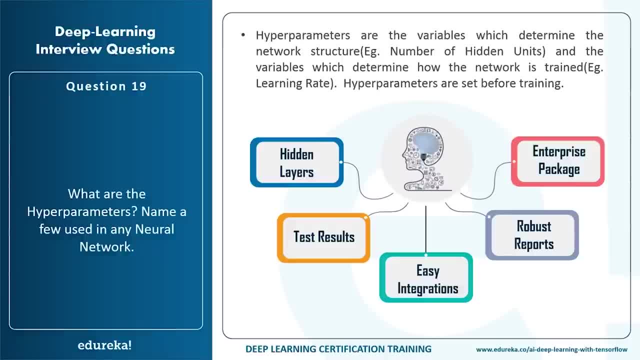 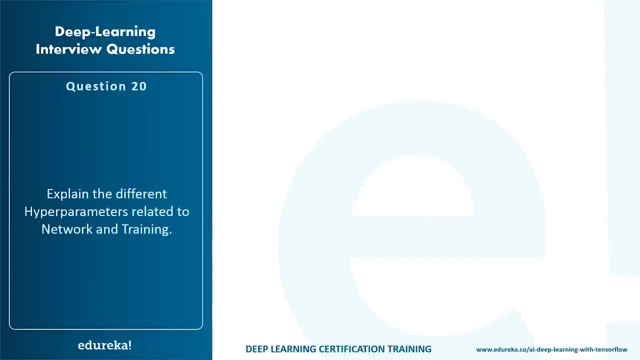 So, as in CNN, we get extra parameters to work on when considering CNN, which are the convolutional neural networks, and sometimes we have to deal with less number of hyper parameters. It all depends upon the type of neural network which you are using. So, which brings us to the next question: is that explain the different? 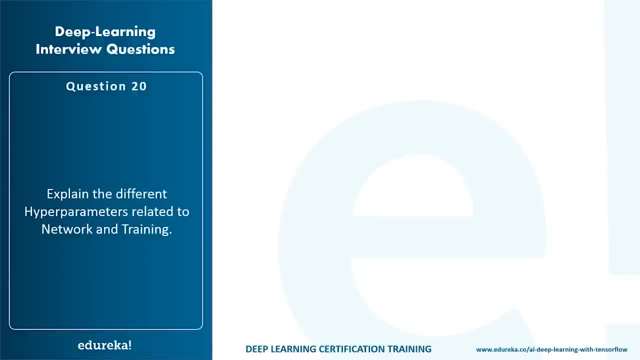 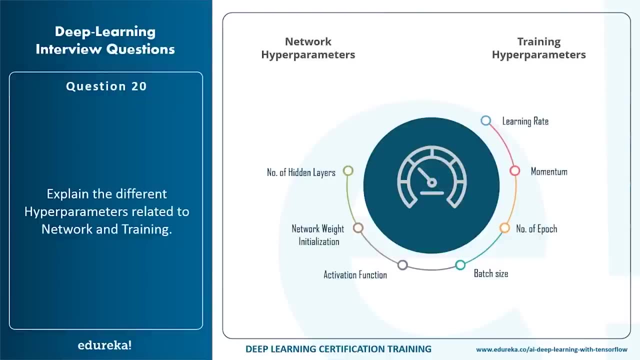 hyper parameters. we did to networking and training. So in training we have: first of all we have the number of hidden layers. So hidden layers are the layers between the input and the output layers, as we just discussed, and many hidden units within a layer with regularization. 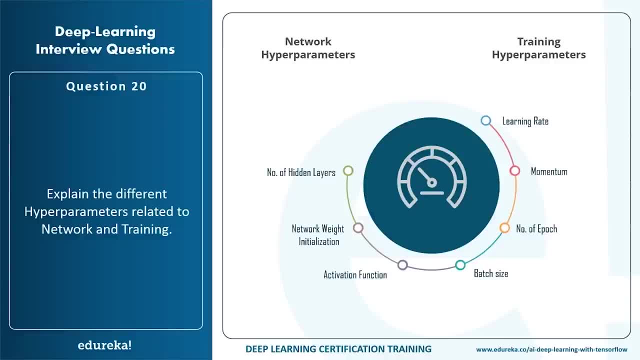 technique can increase the accuracy as smaller number of units It may cause under fitting. now another important aspect is network weight initialization. So ideally it may be better to use different weight initialization schemes according to the activation function used on each layer. mostly uniform distribution is used or the normal distribution. 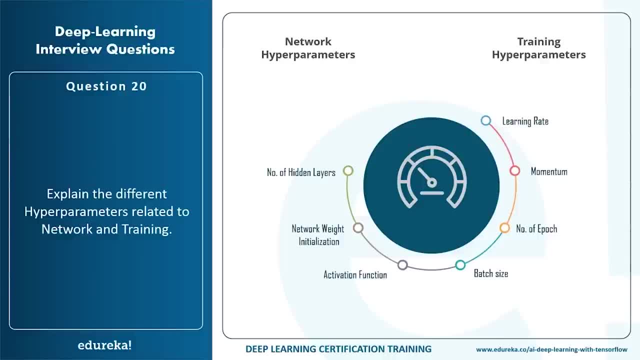 Now, if we talk about activation function, so they are also used to introduce non-linearity to the models. They are also used to introduce non-linearity to the models, which allows deep learning models to learn. nonlinear Boundaries are generally the rectifier. activation function or the relu is 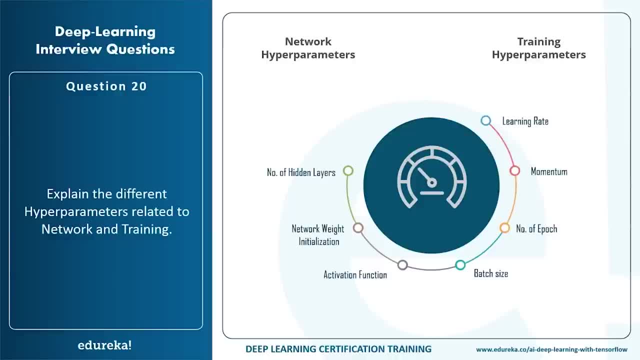 the most popular. Now if you talk about the training parameters. so these were the network parameters which have to be initialized to a deep neural network before the training begins, and just before the training we have the training parameters, which are the learning rate. So the learning rate defines how quickly a network updates its parameter. 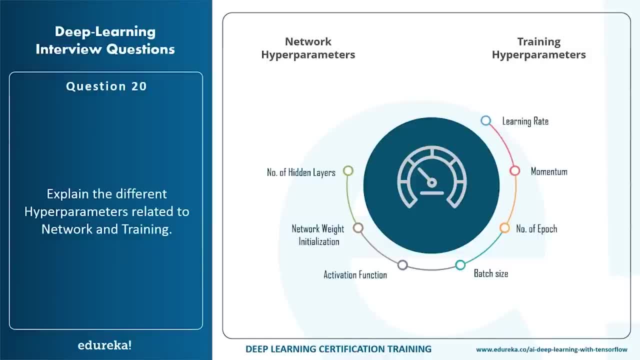 low learning rates slows down the learning process but converts smoothly. A larger learning rate speeds up the learning but may not converge as smooth as a low learning rate. Usually a decaying learning rate is preferred so that we get the best of both worlds and we get the best expected output. 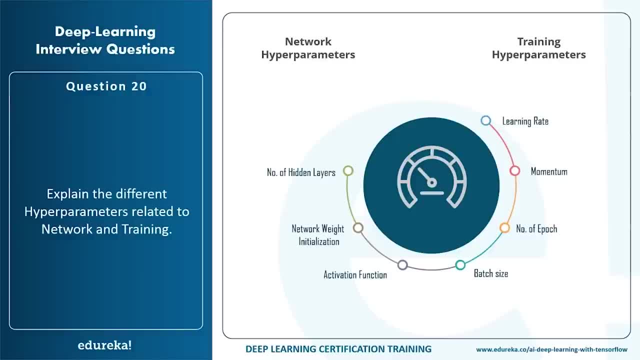 Now another hyper parameter is momentum. So momentum helps us to know the direction of the next step with the knowledge of the previous step. Now it helps to prevent oscillation, and a typical choice of momentum is between 0.5 to 0.9.. 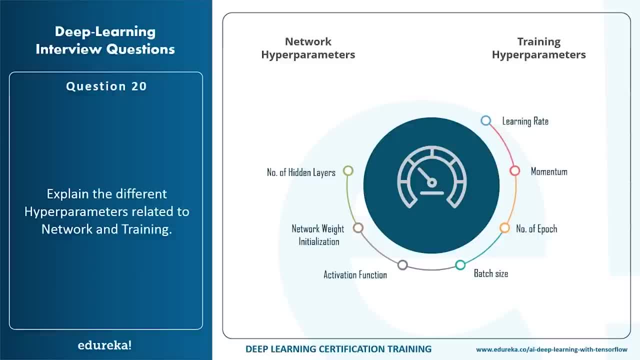 Now, if we talk about the number of epochs, so epochs is basically iterations, So a number of epochs is the number of times the whole training data is shown to the network while training. So increase the number of epochs until the validation accuracy starts decreasing, even when tearing accuracy is increasing. 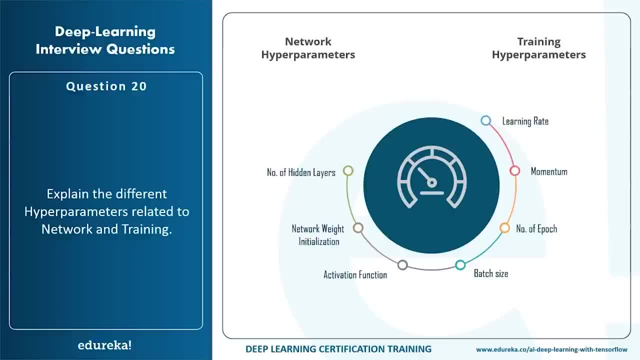 So that results in sometimes overfitting. and if you talk about the batch size, so mini batch size is the number of sub samples given to the network After which parameters update happen. So a good default for batch size might be 32 or 1664.. 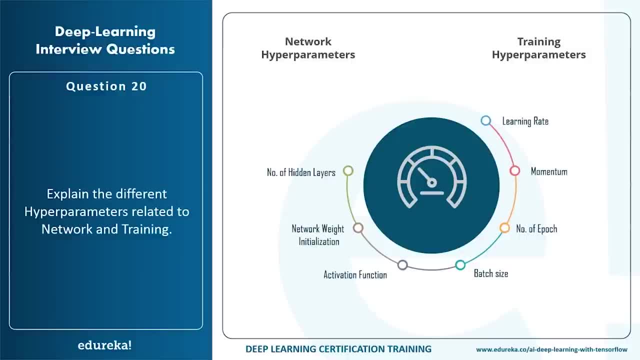 It depends upon the size of, you know, the data you have. it can be any arbitrary number, but it's always better to have it in the power of two right. So while we were talking about overfitting, which brings us to our next question, 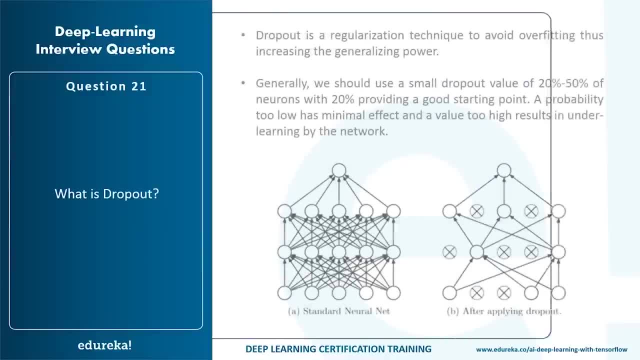 which is what exactly is a dropout. So dropout is regularization Technique to avoid overfitting, which is to increase the validation accuracy, thus increasing the generalization power. now generally use a small dropout value of 20% to 50% of the neurons fit 20%, providing a good starting point and a 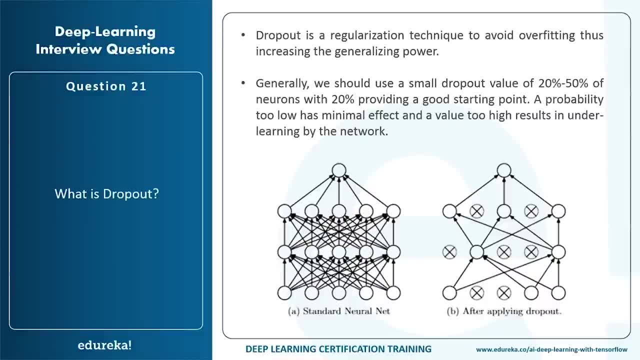 priority too low has minimal effect and a value too high results in under learning by the network. So, first of all, what you need to do is use a large network and you are likely to get better performance When the dropout is used on larger Network, giving the model more of an 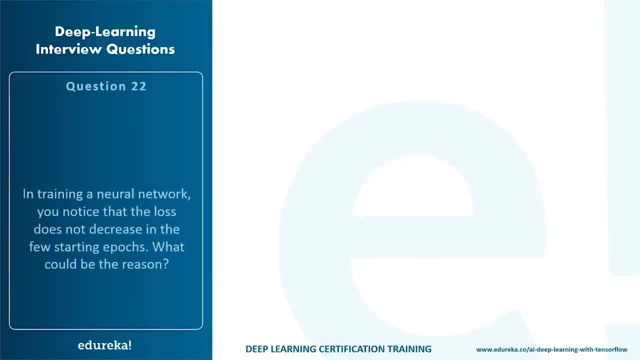 opportunity to learn independent representation. Now our next question is: in a neural network, You notice that the loss does not decrease in the few starting Epochs, So what could be the possible reason for this to happen? Now the correct answer is: the reason for this could be the learning rate is. 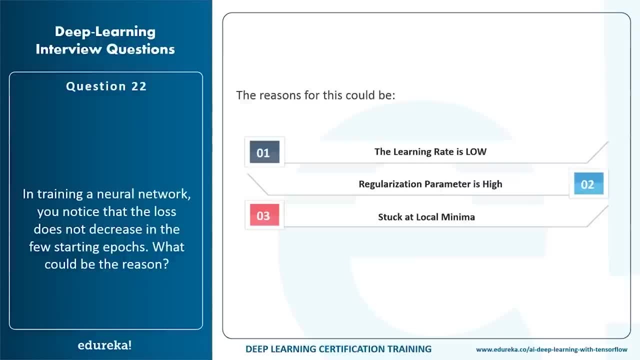 low. First of all, or it might be the regularization parameter is high, or it can be it is stuck at local minima. So it might take certain iteration to go out of the local minima and finally reach the lowest point. So it might happen in some cases that is a stuck at local minima. 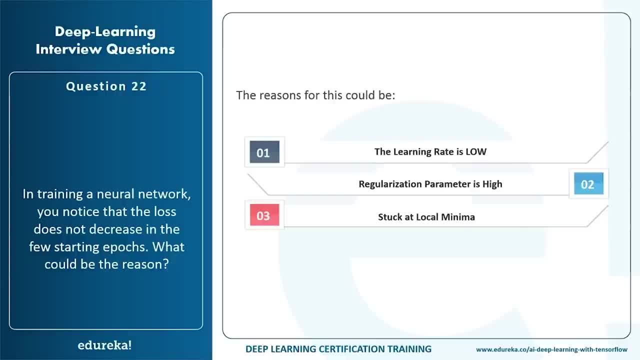 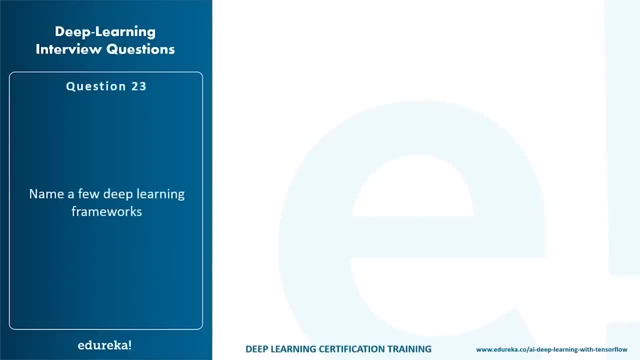 So another approach to that sort of problem must be initiated at that particular point of time. not talking about deep learning, fun might ask to name you a few deep learning frameworks which are being used in the industry. So, first of all, the foremost and the most amazing deep learning library is 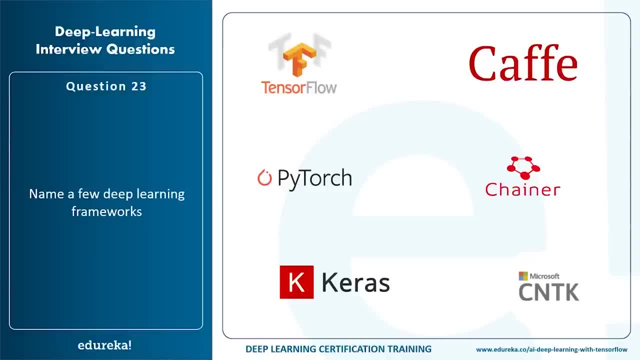 the tensorflow followed by. we have cafe. We have the Microsoft Cognitive Toolkit, which is the CNTK. We have torch, or pie torch, which is giving a good battle or it's standing out from the crowd and people are sometimes preferring by torch over. 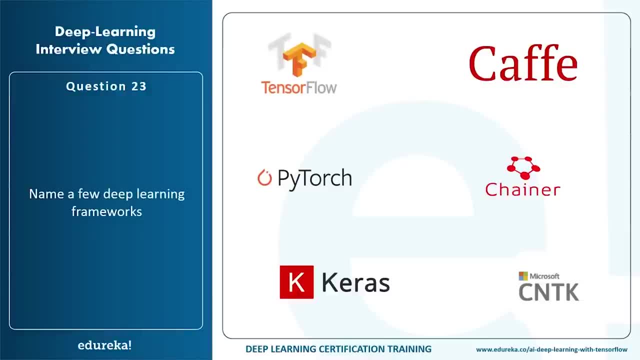 tensorflow. Now MX net is another deep learning framework. We have Chainer and we have Keras. Now Keras, as you know, can be integrated with piano as well as tensorflow, and Keras has been considered one of the best or the simplest deep learning framework. when it comes to deep learning, 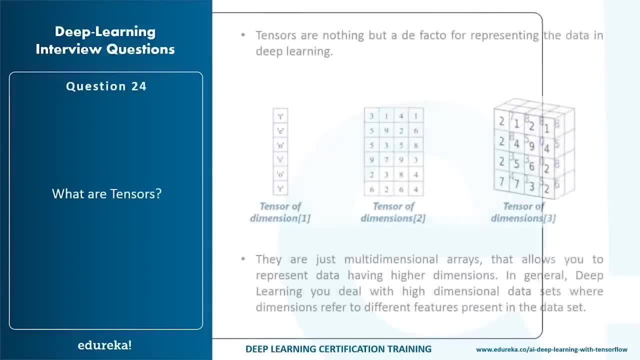 Now one might ask: what exactly are tensors? so tensors are nothing but a de facto for representing the data and deep learning what I meant to say? that tensors are just multi-dimensional arrays that allows you to represent the data having higher dimensions. in general, deep learning you deal with. 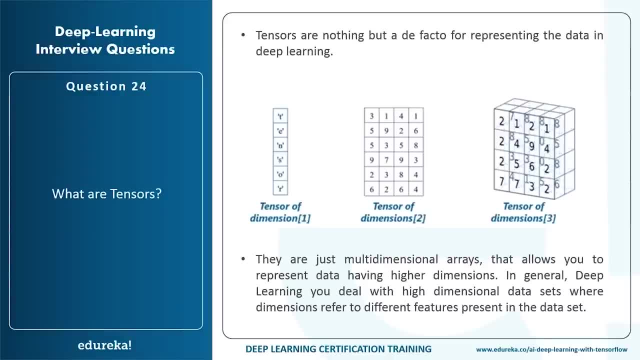 high dimensional data sets. We are dimensional To the different features present in the data set, So what you need is a multi-dimensional sort of array or a data structure, what you could say, so that what exactly tensor is, and in fact the name tensorflow has been derived from the operations which the neural network. 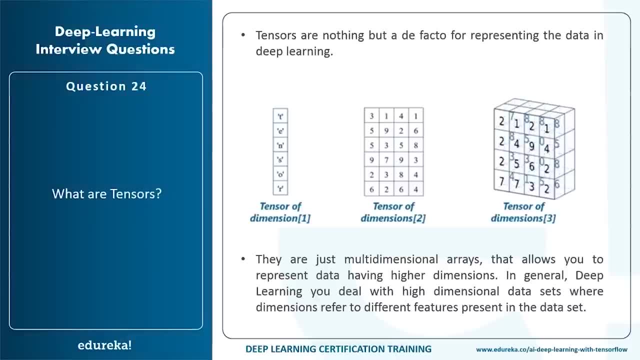 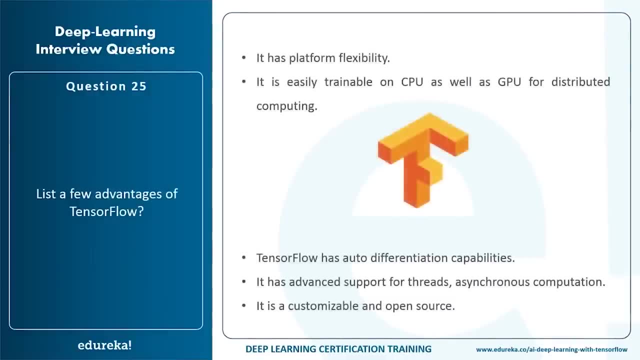 perform on tensor. So it's literally a flow of tensor. the talking about tensorflow, one might ask, since it's the most popular deep learning framework and companies prefer people having the knowledge of tensorflow and been working on it. So what are the few advantages of tensorflow? 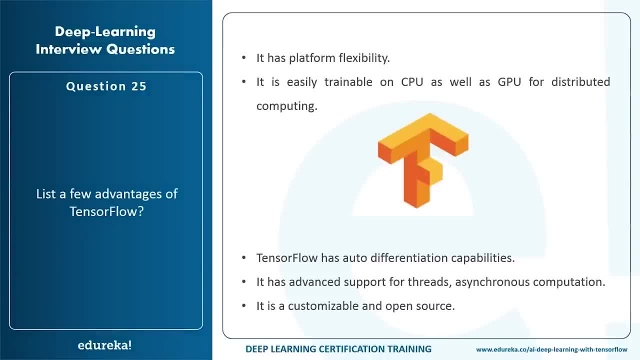 So, first of all, it has the platform flexibility. It is easily trainable on CPU as well as GPU for distributed computing not as a flow- has Auto differentiation capabilities and it has advanced support for threats, asynchronous computation and it is a customizable and open-source framework and, most importantly, if we talk about the latest tensorflow 2.0,. 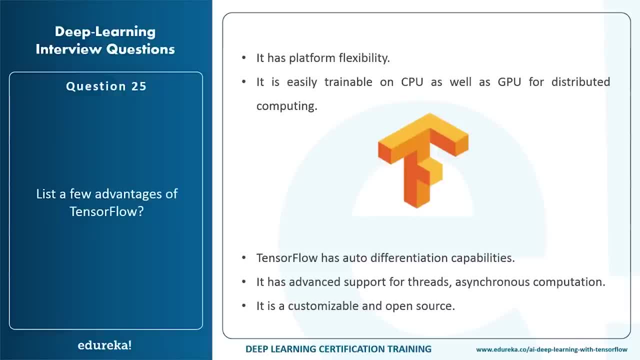 which has just been released. So those come up with a lot of interesting features, and it has adopted Keras as its high-level API fully so that the coding aspect of it is much simplified and eager. execution is now by default, so that you do not have 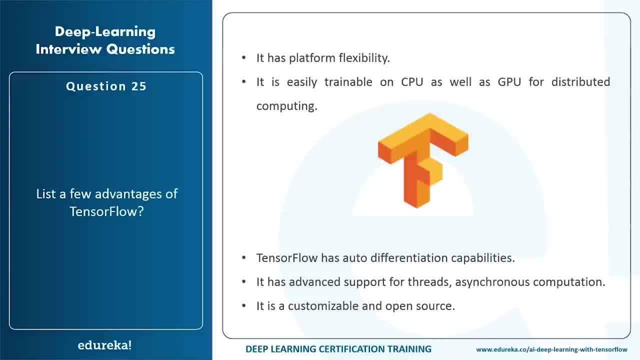 to write loads and loads of line of code. and if you want to know more about tensorflow 2.0 and why it's the best deep learning framework in the industry right now, just go ahead and check our tensorflow 2.0. Video. 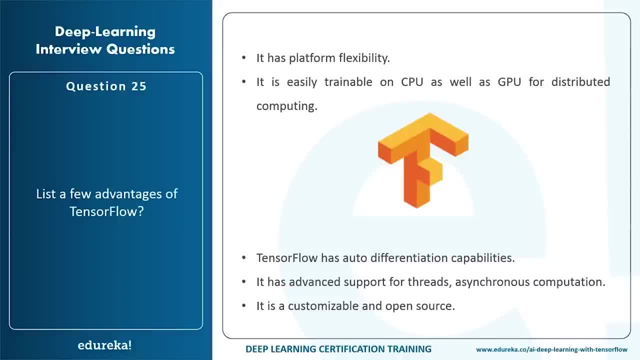 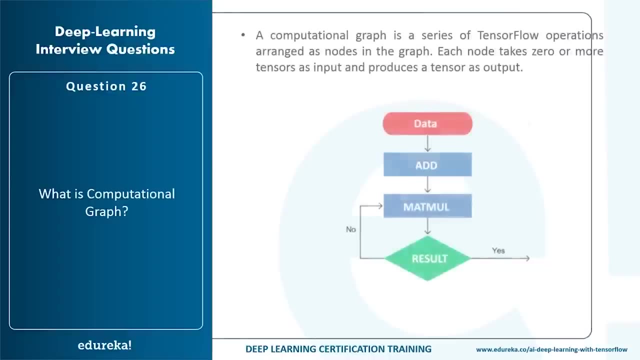 I'll leave the link in the description box below. go check it out, guys, and understand how exactly is it better from the previous version and why it is the best deep learning framework right now. not talking about computational graphs. what might ask what exactly they are So well? a computation graph is a series of tensorflow operations arranged. 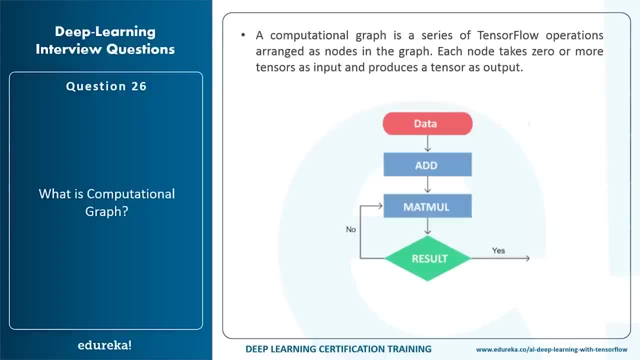 as notes in the graph. now, each note takes zero or more tensors as input and produces a tensor as Output. now, basically, one can think of a computational graph as an alternative way of conceptualizing mathematical calculation that take place in a tensorflow program. Now the operations assigned to the referent nodes of a computational graph: 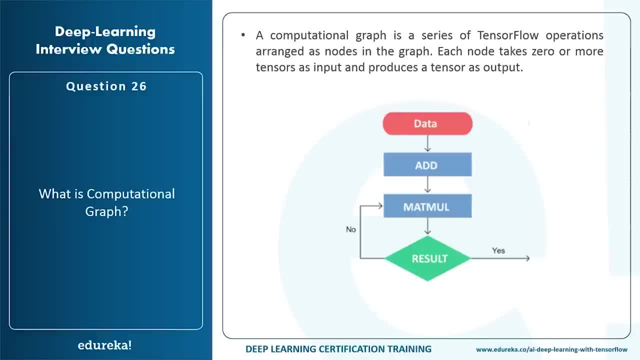 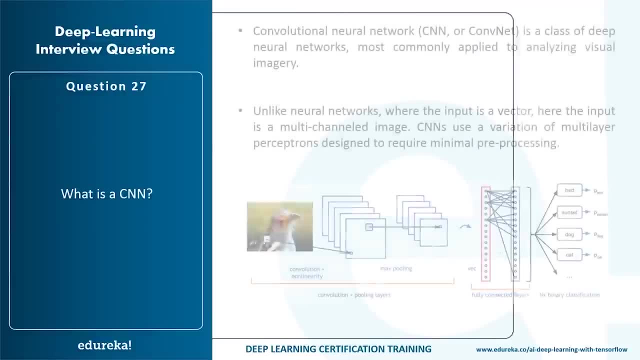 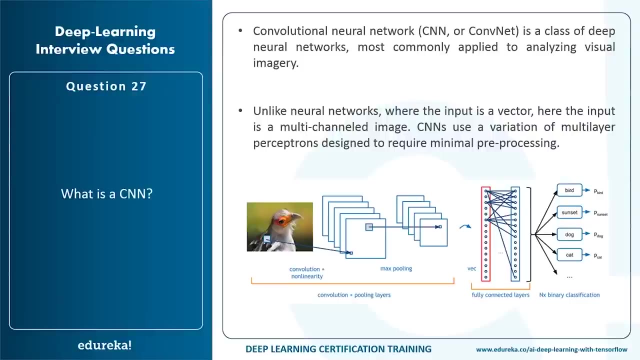 can be performed in parallel, thus providing better performance in terms of computation. So one might ask: what exactly is a convolutional neural network? now, a convolutional neural network or CNN or cornet? It's a class of deep learning neural networks which is most commonly applied to analyzing the visual imagery. 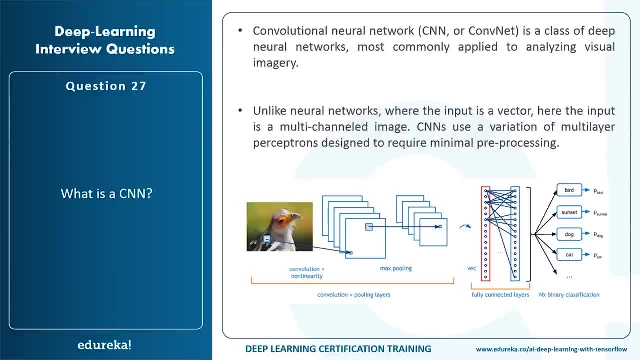 So CNN use a variation of the Monday layer perceptron designed to require minimal processing. Now one might ask the next question if you are going for an interview which requires you to work with a lot of images or videos, So in that case CNN's are very much used. 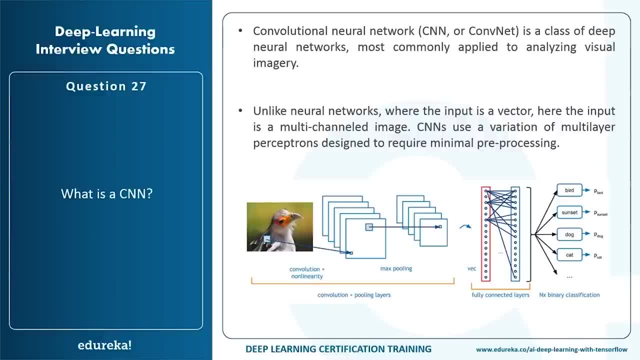 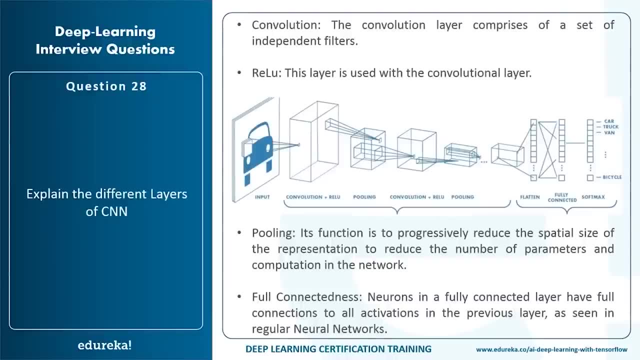 So having a good knowledge of CNN is always better in that case. So the next question which we have here is: What are the various layers of CNN? but there are four layered concepts Everyone should understand in convolutional neural networks are first the convolutional layer. 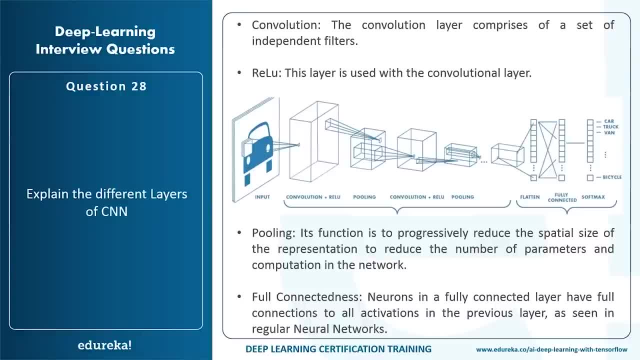 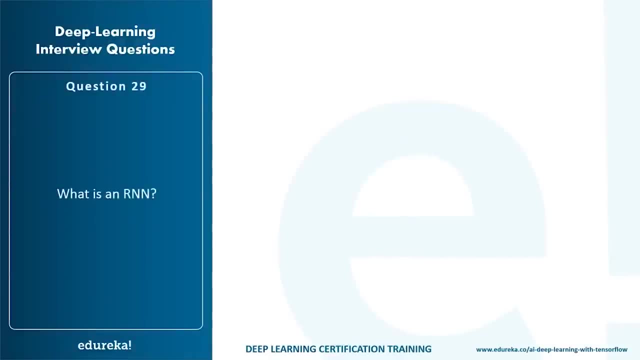 The second is the relu layer, And finally we have the pooling layer and finally we end up with the full connectedness or the full connected layer. Now, if we talk about CNN, we have to talk about iron also. So one might ask: what exactly is iron? and so iron or the regular networks? 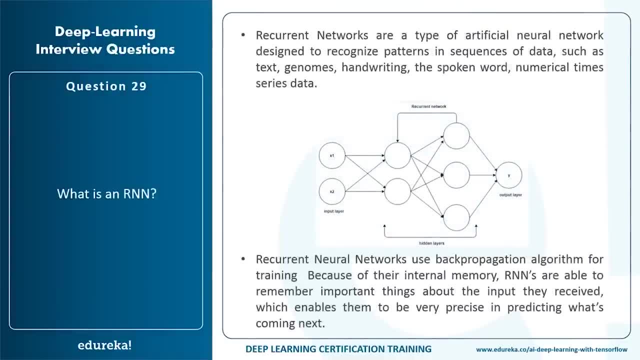 Are a type of artificial neural networks which are designed to recognize the patterns in the sequence of data such as text, genomes, handwriting the spoken word, numerical time series, data from sensors, the stock markets and the government agencies. So recurrent neural networks use back propagation algorithm for training. 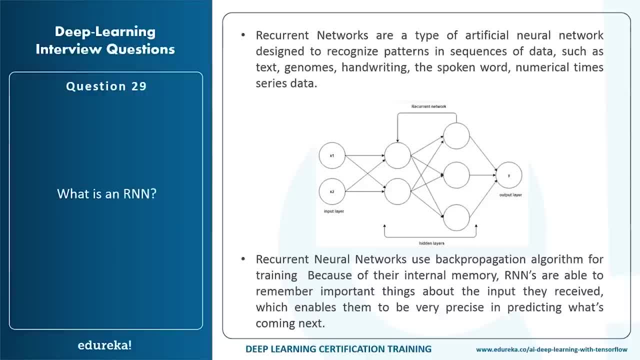 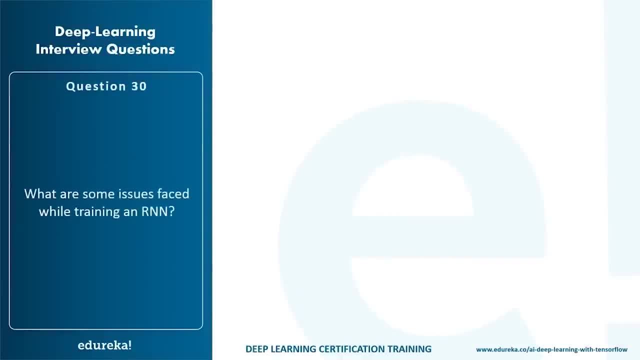 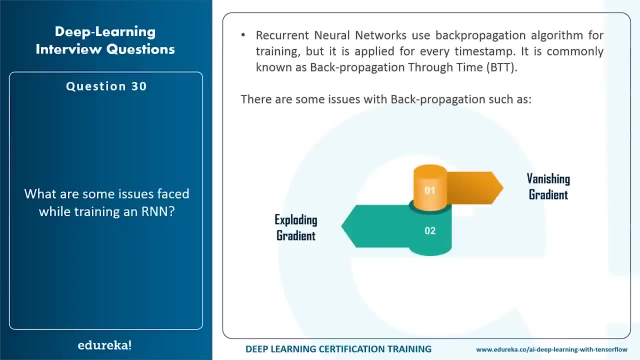 but it is applied for every time stamp. It is commonly known as back propagation through time, which is BTT. Now our next question is: what are some issues faced while training and iron in so recurrent neural networks use back propagation algorithm, as I just mentioned? 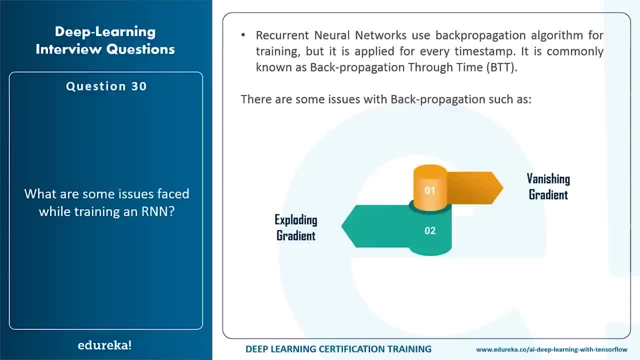 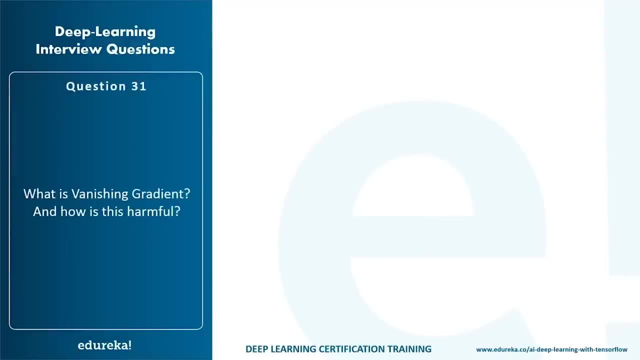 for training, but it is applied for every time stamp and there are some issues with back propagation, such as vanishing gradient or the exploring gradient, where the gradient vanishes or it is too much to handle, which brings us to the next set of questions, The first of which is: what exactly is a vanishing gradient? 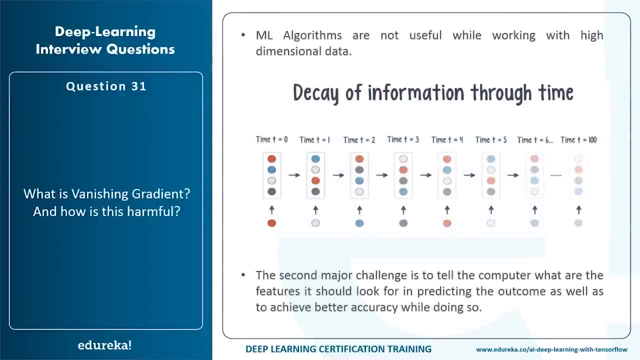 And how is it harmful now when we do back propagation, that is, move backward in the network, and calculating gradients of loss, which is the error? with respect to the weights, the gradients tend to get smaller and smaller as we keep on moving backward in the network. 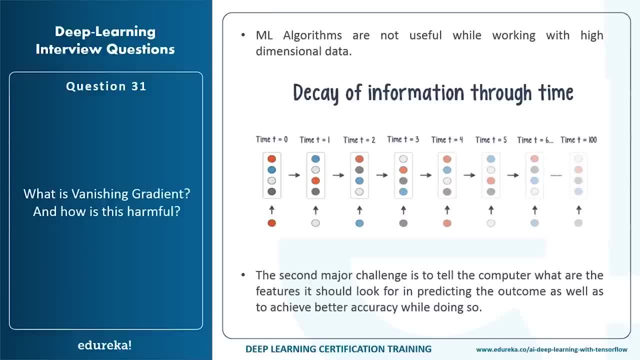 Now this means that the neurons in the earlier layers learn very slowly as compared to the neurons in the later layers in the hierarchy, or the earlier layers in the networks are the slowest to train. now How is this harmful? so earlier layers in the neural 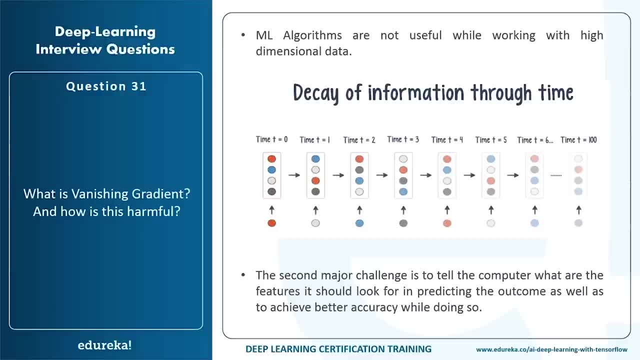 Networks are important because they are responsible to learn and detect the simple patterns and are actually the building blocks of our neural network. Obviously, if they give improper and inaccurate result, then how can we expect the next layer and the complete network to perform nicely and produce the accurate result? 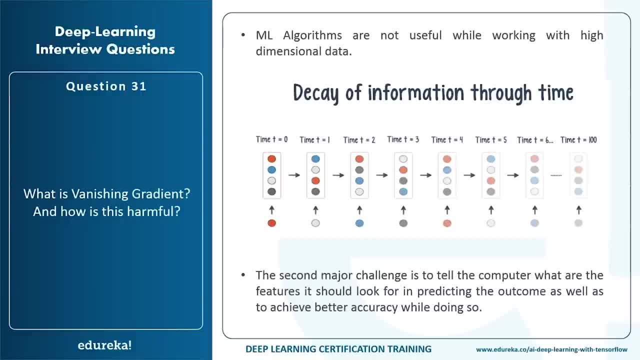 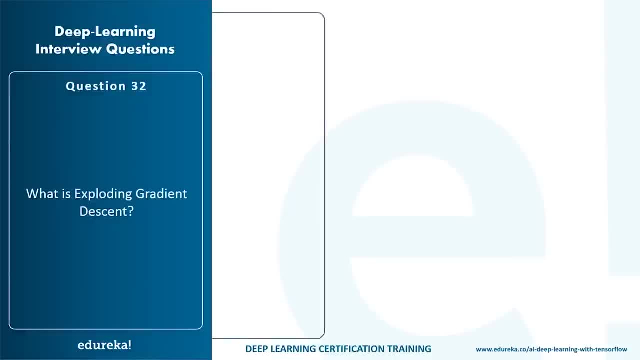 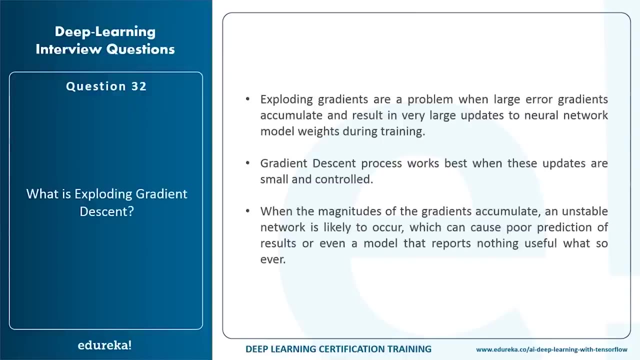 So the training process takes too long and the prediction accuracy of the model will decrease. Now another question here arises is what exactly is then exploding gradient descent? Now, this is just the opposite of vanishing gradient descent. So exploding gradients are a problem when large error gradients accumulate. 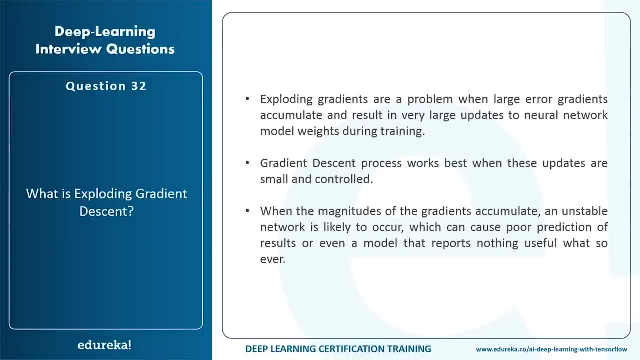 and result in very large updates to the neural network model weights during training. So the gradients are used during the training to update the network weights, but typically when this process works best is when this weights are small and controlled when the magnitudes of the gradients accumulate. 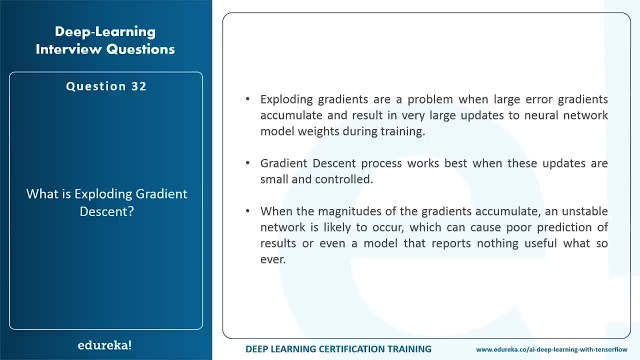 and the unstable network is likely to occur Now, which causes a poor prediction and results or even a model that reports nothing useful whatsoever. So vanishing gradient and the exploding gradient are two problems which occur while the back propagation happens in a recurrent neural network. 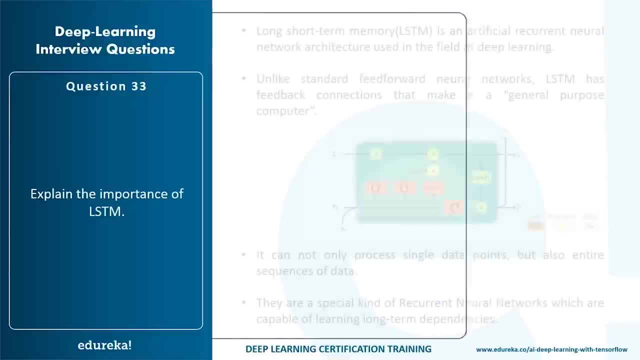 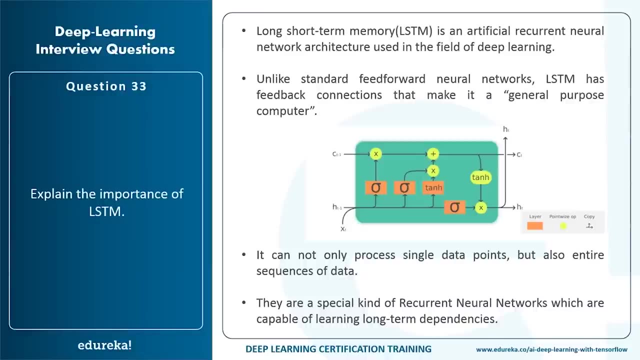 So our next question is: what are LSTM So long short-term memory, which are? the LSTM is an artificial recurrent neural network architecture used in the field of deep learning and, unlike standard feed forward neural networks, The LSTM has feedback connection that make it a general-purpose computer. 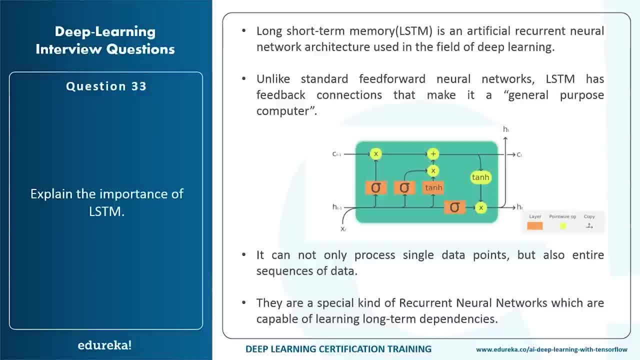 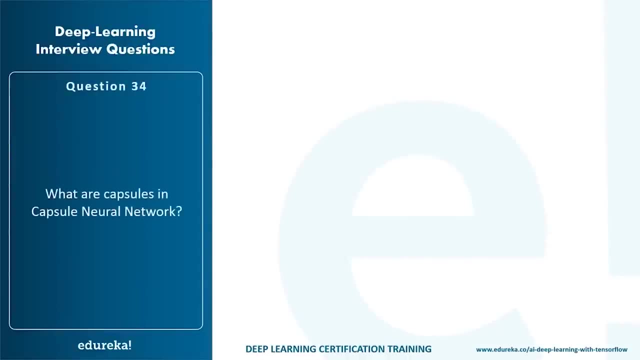 Now it can not only process single data points but also the entire sequence of data. They are a special kind of ordinance or the recurrent neural network which are capable of learning long-term dependencies. Now one might ask: what are capsules in a capsule neural network? 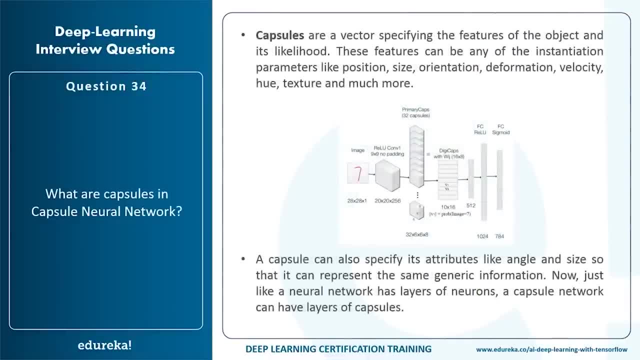 So capsules are vector, or what we can say, an element With a size and a direction specifying the features of the object and its likelihood that these features can be any of the instantiation parameters, like the pose we are: the position, size, orientation, deformation velocity, the albedo. 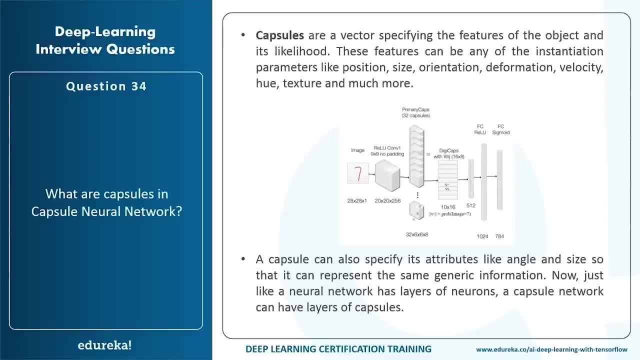 which is the light reflection, hue, texture and much more. a capsule can also specify its attributes, like angle and size, so it can represent with the same genetic information. Now, just like a neural network has layers of neurons, a capsule network can have layers, capsules. So there could be had capsules representing the group of objects or the capsules below them. 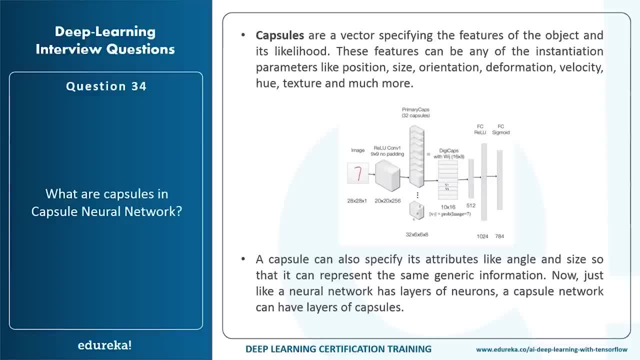 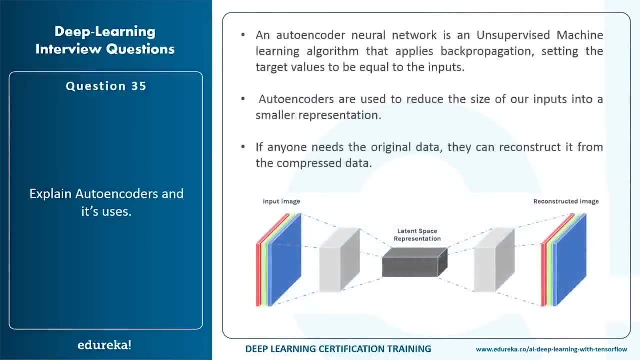 Now this helps in getting deeper knowledge of a particular object or a particular data set and having the knowledge from different aspects or different angles. So the next question arises is explain auto encoders and its uses. so an auto encoder neural networks is an unsupervised machine learning algorithm that applies the back propagation, setting the target values, 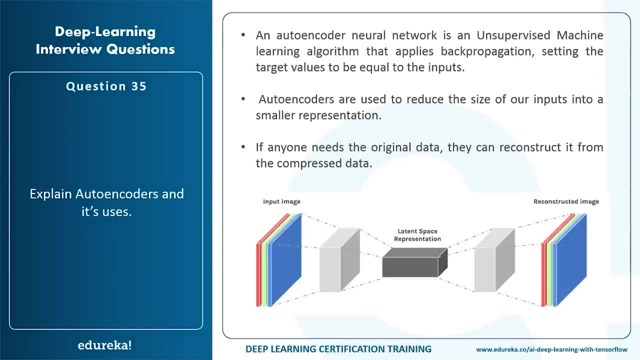 to be equal to the inputs. So auto encoders are used to reduce the size of our inputs into smaller representation, and if anyone needs the original data, they can reconstruct it from the compressed data. Now one might ask the question: How does auto encoder differ from PCA? 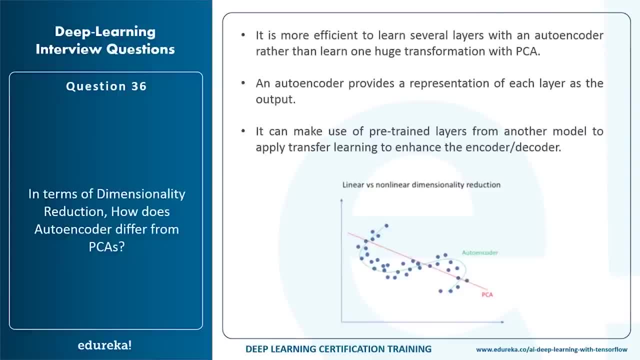 So an auto encoder can learn from nonlinear transformation with a nonlinear activation function and multiple layer. It does not have to learn dense layers. It can use convolution layers to learn, which is better for video image and series data. It is more efficient to learn several layers with an auto encoder rather than learn one huge transformation. 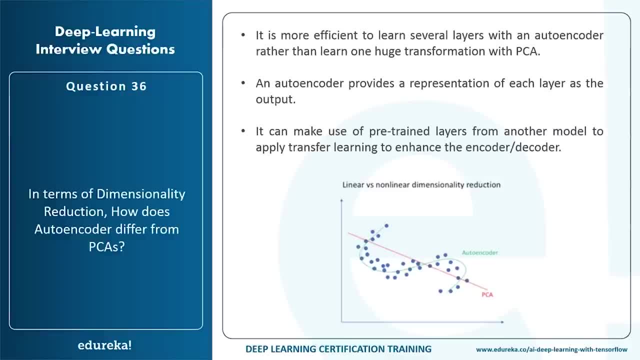 with the PCA and auto encoder provides a representation of each layer as the output and can take the use of pre-trained layers from other model to apply, transfer the learning to enhance the encoder or the decoder. So these are few of the reasons why auto encoders are better from PCA. 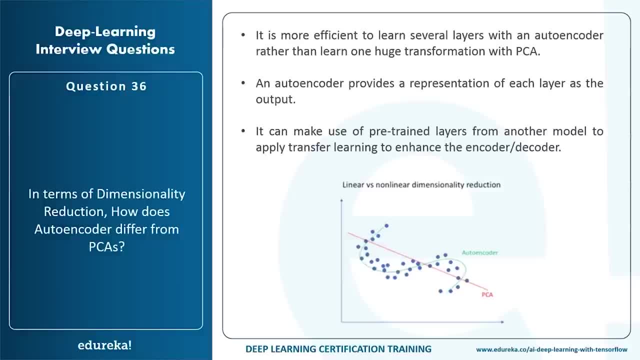 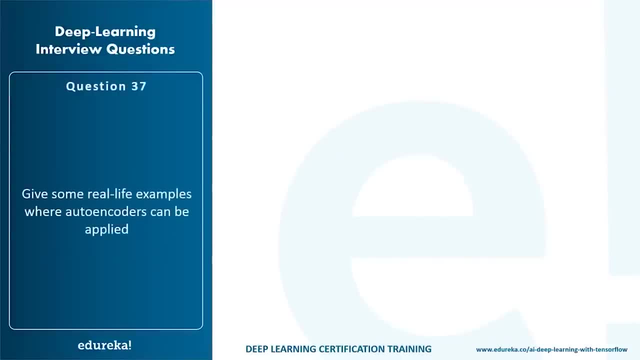 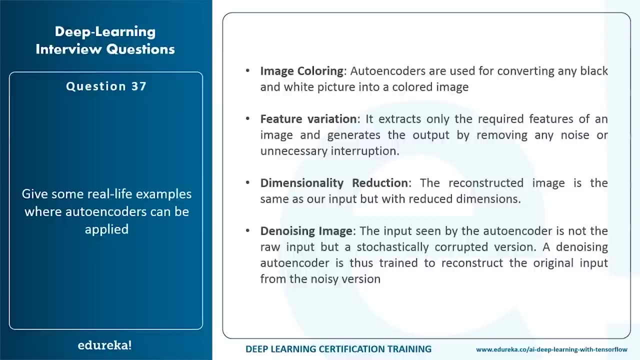 as we know, both of them perform the same task, which is mostly dimensionality reduction. Now give some real-life examples where auto encoders can be applied. So the first of all we talk about dimensionality reduction, or the first thing that should pop up in your mind is dimensionality reduction. 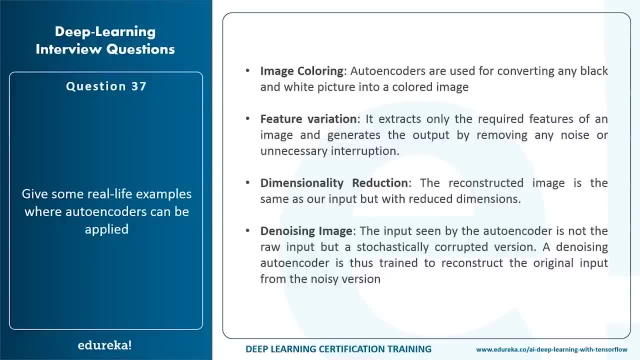 So the reconstructed image is the same as our input image, but with reduced dimensions. Now it helps in providing similar image with reduced pixel value, and it can be used in various areas where we have limited storage or we have limited processing power. So when there is a high input or an image, 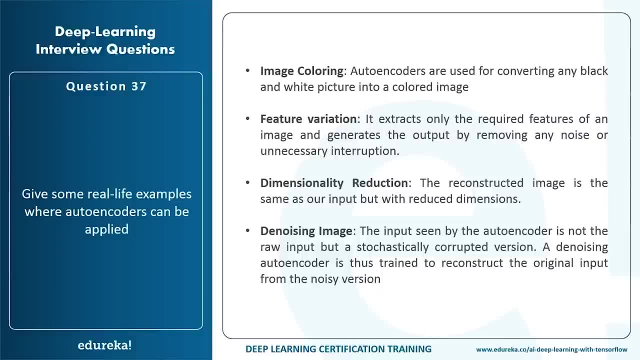 or a data with high dimension or which has higher values- pixel values- it can compress and provide the same image with a lower pixel value. Now, auto encoders are used for converting any black and white picture into a colored image, believe it or not, and depending on what is in the picture. 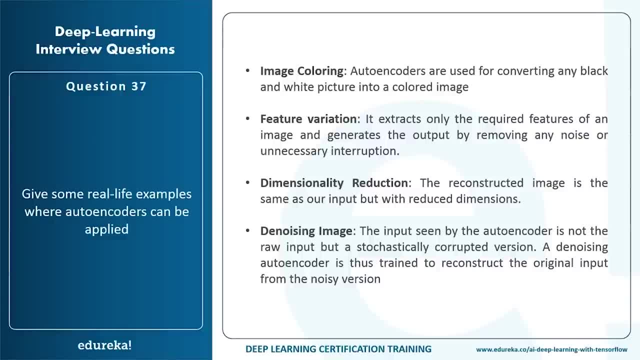 It is possible to tell what the color should be now feature variation. If we talk about feature variation, it attracts only the required features of an image and generates the output by removing any unnecessary noise or unnecessary interruption. And if we talk about denoising image, 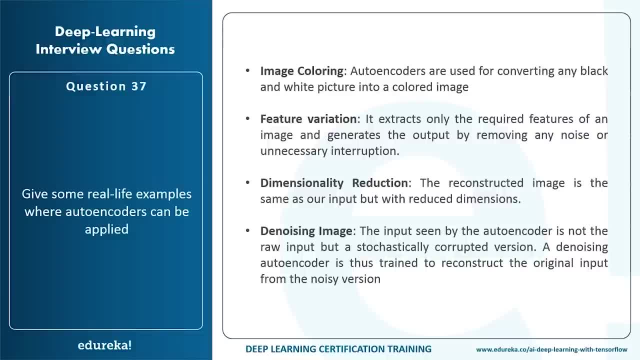 the input seen by an auto encoder is not the raw input but a stochastically corrupted version or denoising. auto encoder is the strain to reconstruct the original input from the noisy version. Not talking about auto encoders. ask about the different layers of the auto encoders. 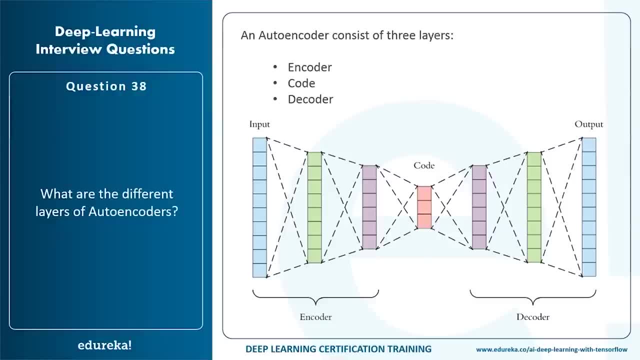 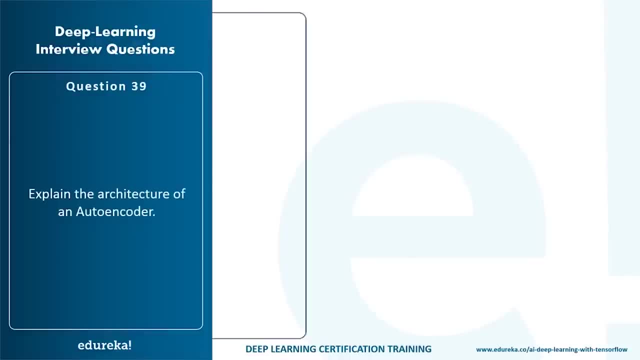 So, basically, an auto encoder consists of three layers, which is the encoder. We have the code and the decoder, which brings us to the next question. Explain the architecture of an auto encoder If you talk about the three layers which are encoder, code and decoder. 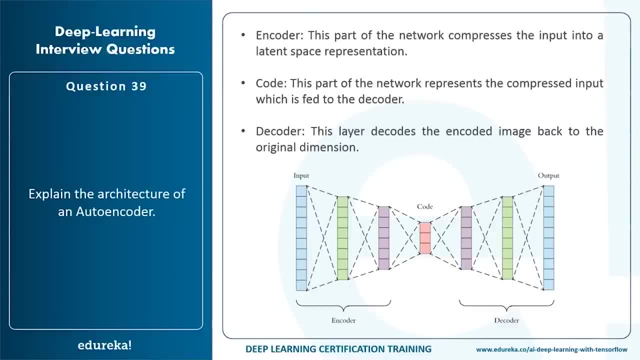 So if we talk about encoder, this part of the network compresses the input into a latent space representation. Now the encoder layer encodes the input images as a compressed representation in a reduced dimension, And the compressed image is the distorted version of the original image. 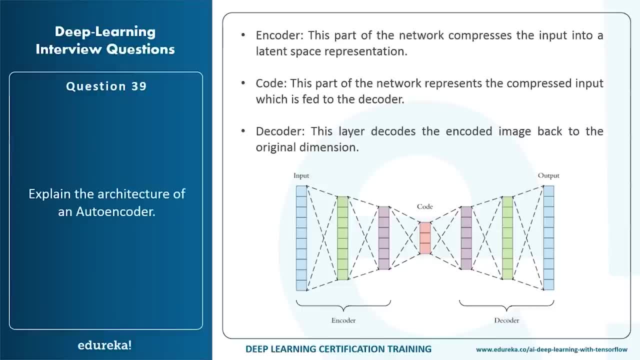 Now coming to the middle part, which is the code. So this part of the network represents the compressed input which is fed to the decoder. It is basically the channel and if you talk about decoder, this layer decodes the encoded image back into the original dimension. 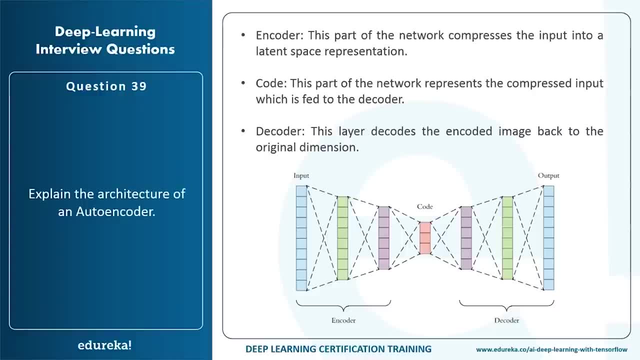 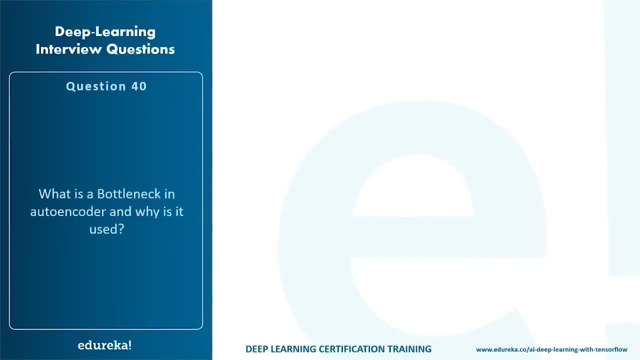 and a decoded image is a lossy reconstruction of the original image and it's reconstructed from the latent space representation. Now one might ask what exactly is bottleneck in an auto encoder and why is it used? Now, the layer between the encoder and the decoder. 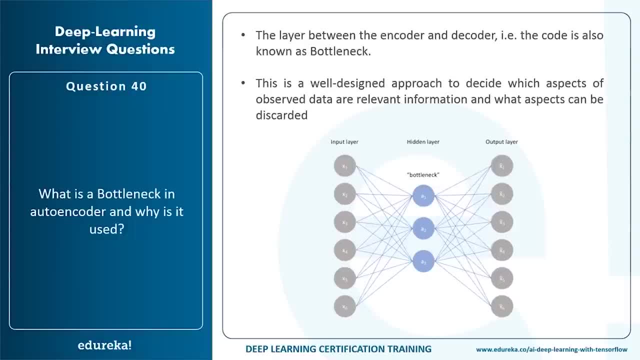 that is, the code, is also known as bottleneck. So this is a well-designed approach to decide which aspect of the observed data are relevant information and what aspects can be discarded. It does this by balancing two criterias. The first, the compactness of the representation, measured as the compressibility. 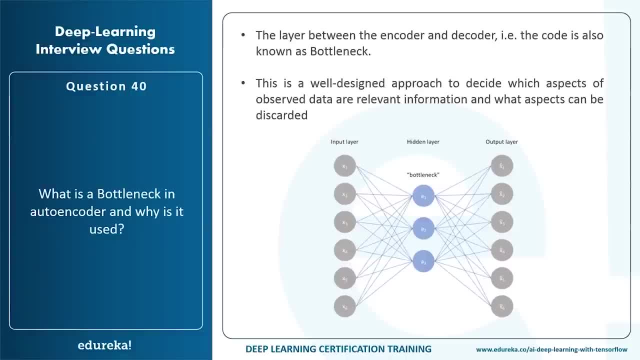 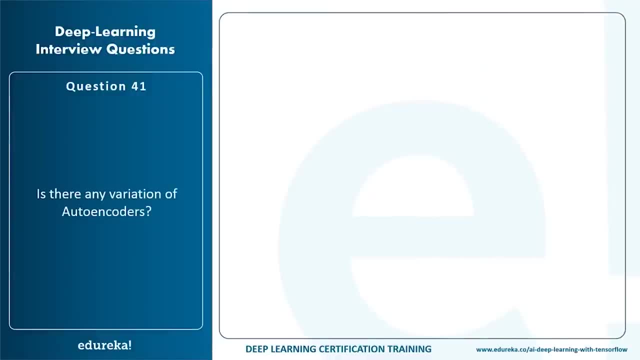 and second, it retains some behaviorally irrelevant variables from the input. Now one might ask: are there any variation of auto encoders? Surely there are. so there are convolutional auto encoders, We have sparse auto encoders, We have deep auto encoders. 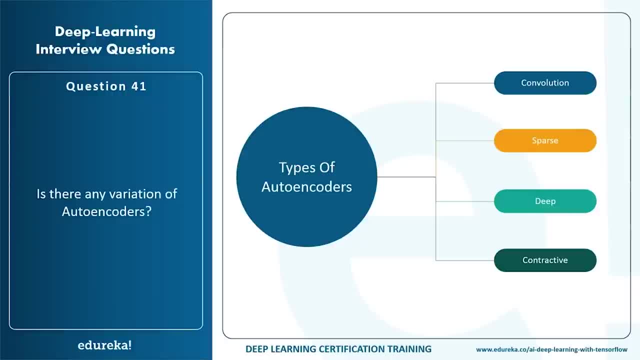 We have contractive auto encoders. All of these auto encoders have a different structure or the different code layer. If you talk about the convolutional auto encoder, we have the convolutional CNN algorithm sort of structure In that particular auto encoder with encoder in one side. 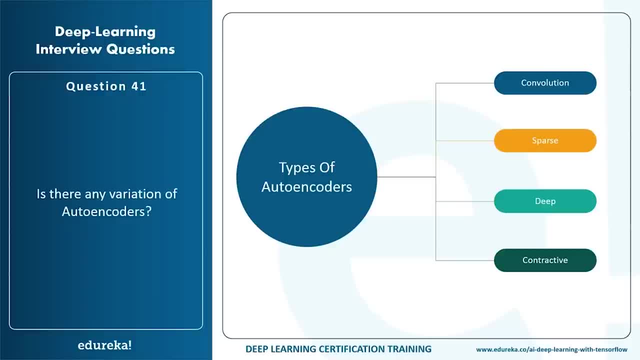 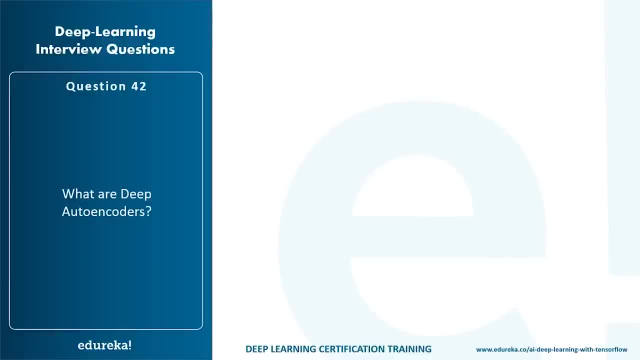 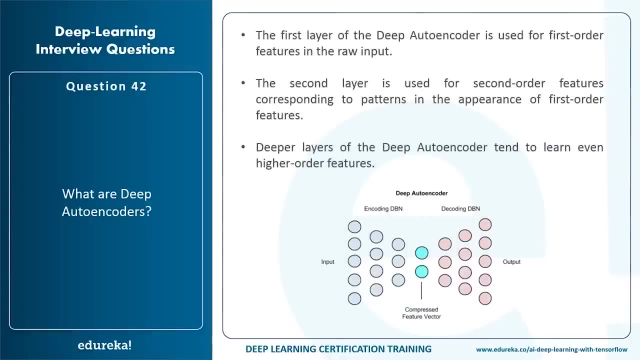 we have the convolution layers, the relu layer, the pooling layer inside it, And then finally we have the decoding layer. So another question what might pop into the interviewers mind is: what are deep auto encoders? So the extension of simple auto encoders is a deep auto encoders. 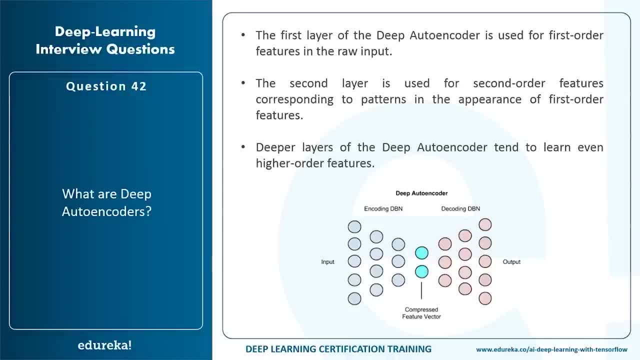 The first layer of the deep auto encoders is used for first order features in the raw input. Now the second layer is used for second order features corresponding to the patterns in the appearance of the first order features. So the deeper layers of the deep auto encoders tend to learn even higher order features. 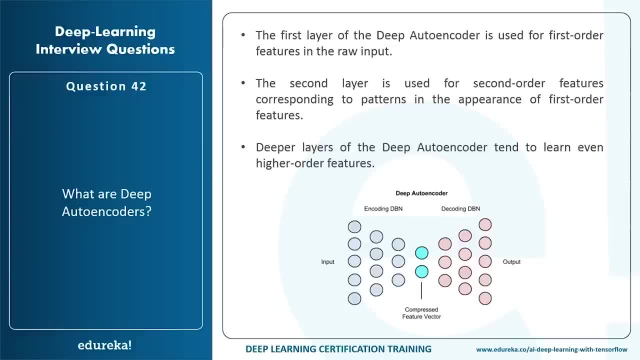 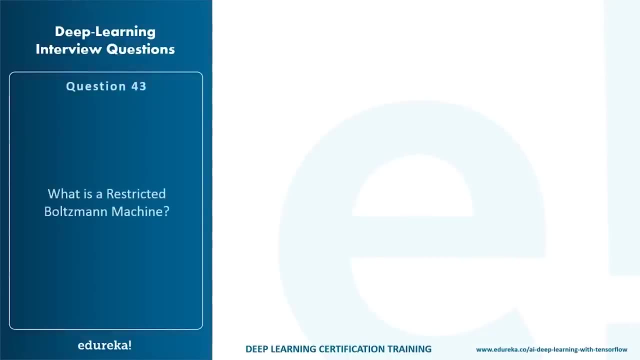 So our deep auto encoders is composed of two symmetrical deep belief networks: First, four or five shallow layers representing the encoding half of the net, and the second, set of four or five layers that make up the decoding half. Interesting right, So another important topic in deep learning. 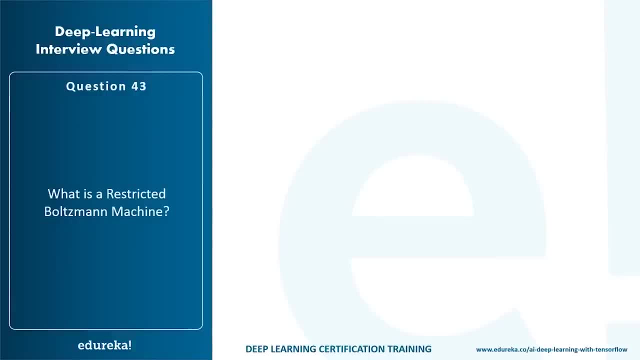 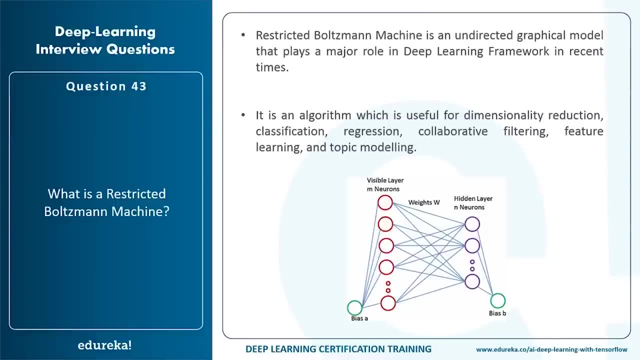 are the Restricted Boltzmann machines. So one might ask: what exactly is an RBM or Restricted Boltzmann machine? So RBM is an undirected graphical model that plays a major role in deep learning framework in recent times and it is an algorithm which is used for dimensionality reduction. 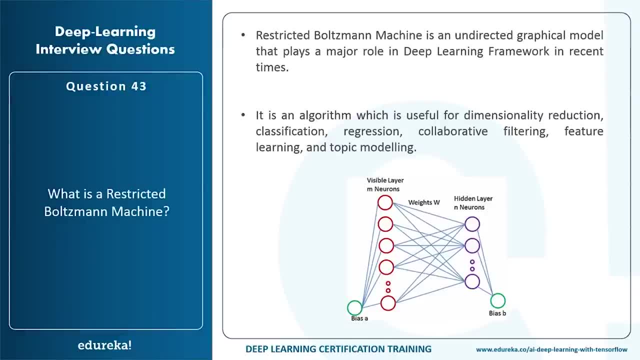 Not only that, it is used for classification, regression, collaborating, filtering, feature learning and topic model. So when we talk about RBM being useful for dimensionality reduction, another question might arise is: how does RBM differ from the auto encoders? 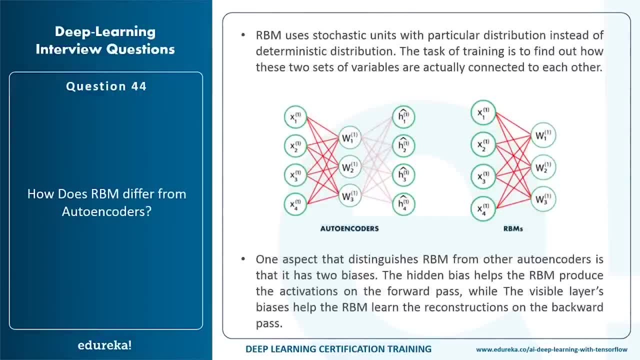 So auto encoders is a simple three-layer neural network where output units are directly connected back to the input units. Typically, the number of hidden units is much less than the number of visible ones, and the task of training is to minimize an error or the reconstruction, that is, find the most efficient compact representation for the input data. 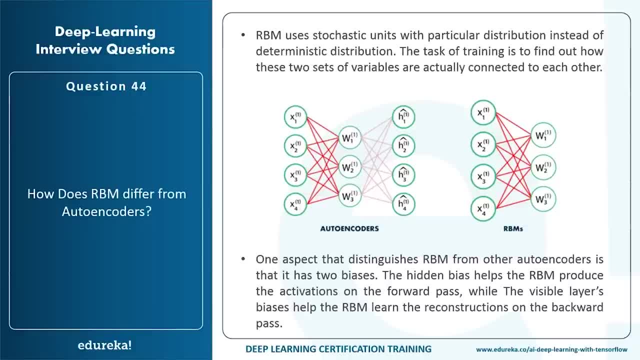 So RBM shared a similar idea, but it uses stochastic units with particular distribution instead of deterministic distribution. The task of our training is to find out how these two set of variables are actually connected to each other. One aspect that distinguishes RBM from the auto encoders is that it has two biases. 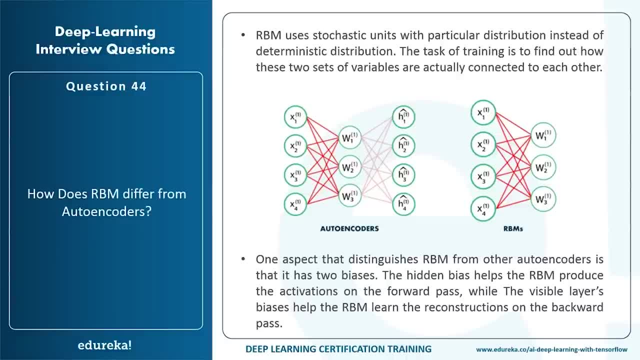 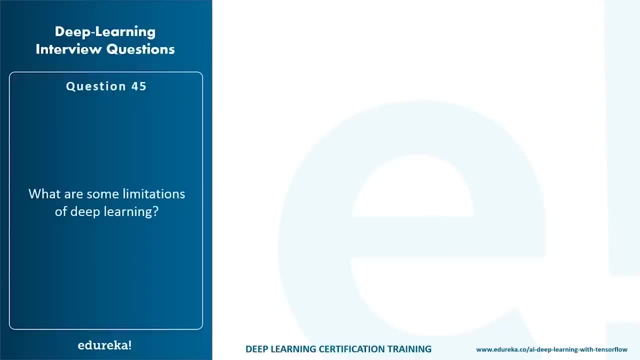 The hidden bias helps the RBM produce the activations on the forward pass, while the visible layer biases help the RBM learn the reconstruction on the backward pass. Now this brings us to the final questions of our deep learning interview. is that, what are some limitations of deep learning? 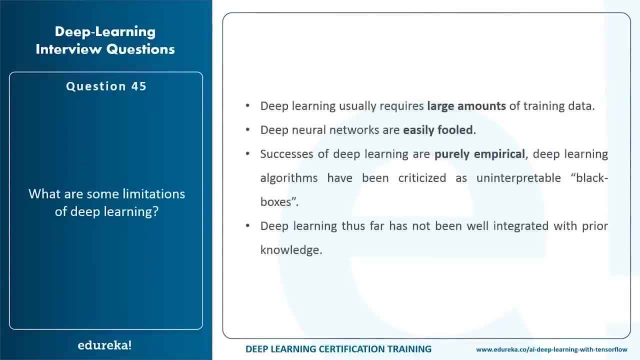 I bet you weren't thinking of this one. but there are some limitations, So deep learning usually requires large amounts of training. data and deep neural networks are easily fooled. Now the success of deep learning are purely imperial. deep learning algorithms have been criticized as uninterpretable black boxes. 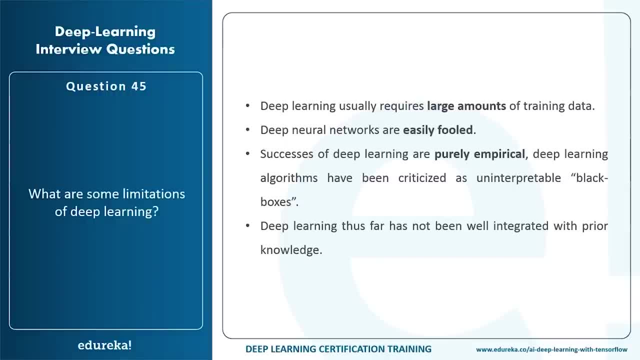 because one important thing about deep learning is that you do not specify What you are looking for right. The algorithm learns on its own. That is one of the shortcomings of deep learning, and deep learning thus far has not been well integrated with prior knowledge. 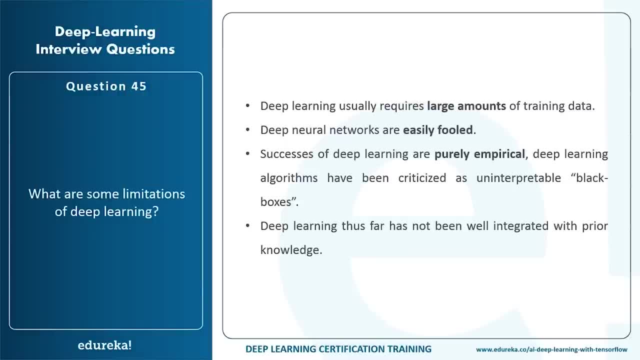 So a lot of people still don't feel it as a way to solve their problem, as a way to approach to their problems, because a lot of people don't understand what exactly is deep learning, how it works, how to initialize all of the variables.